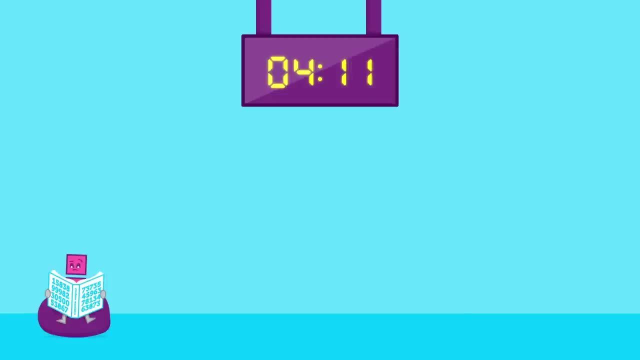 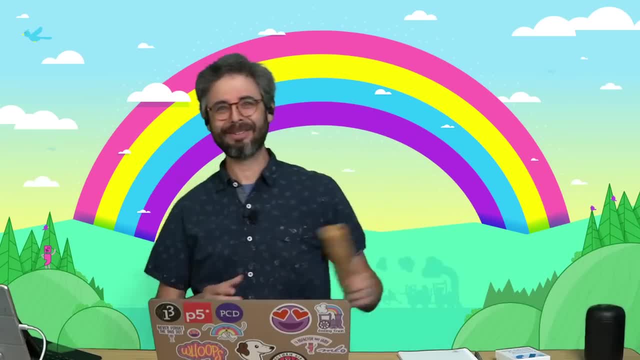 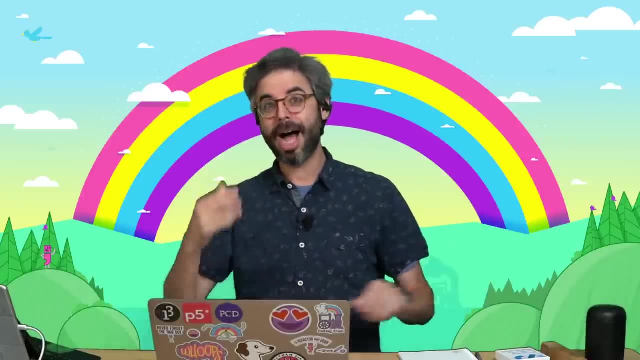 Thank you All right. Hello, I'm live. Look, I'm going to blow the train whistle, which means we're really starting today's live stream. Hello, I'm Dan. Welcome to The Coding Train on a very special Saturday morning. 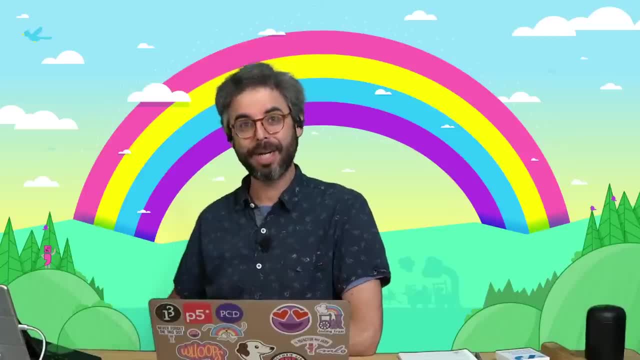 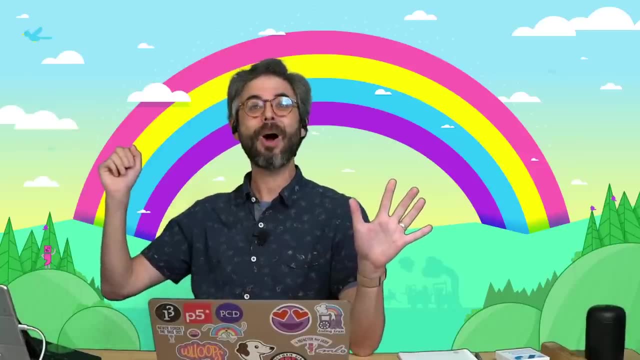 Interesting time to live stream. I hope you're having a nice weekend wherever you are in the world And thank you so much for tuning in, Just in case it's a beautiful day outside, wherever you are and you feel like you know, playing some Frisbee, going for a walk. this will all be archived. 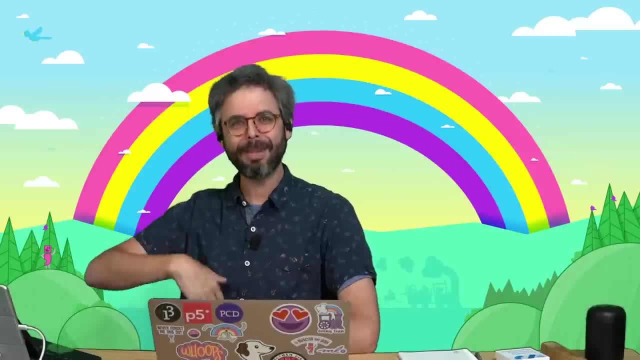 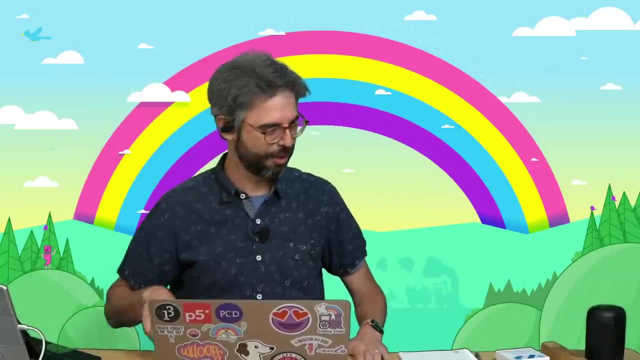 You can watch it all back later. I'll be reviewing any of the comments on YouTube after this gets archived and answering your questions. So but please stay with us. Very excited that you're all here. So I'm just kind of vamping here for a minute to make sure all the everything is going well. 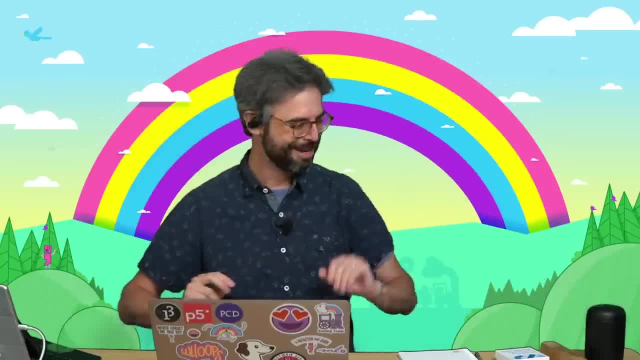 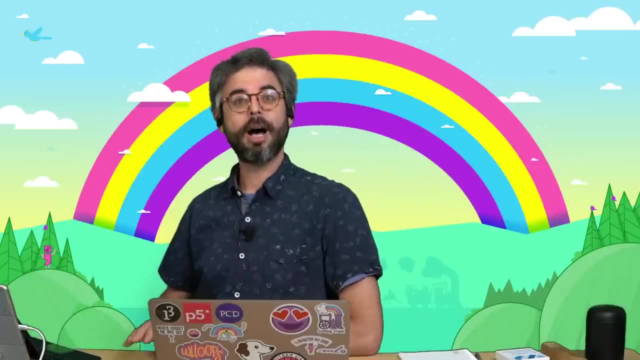 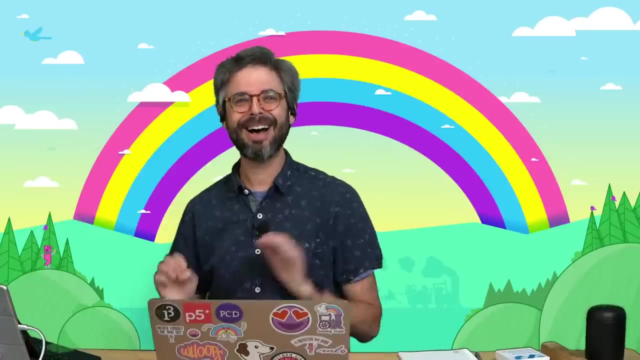 I'm seeing a little flickering on my monitor which is a little disconcerting, But I'm not going to worry about that too much. So first just a couple of housekeeping items. here I have a kind of entirely new tech setup for this stream, because I have a guest which 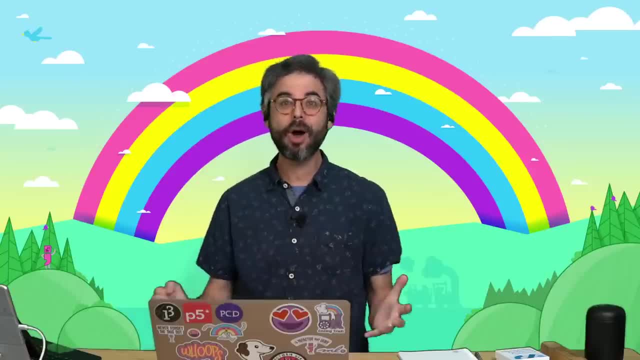 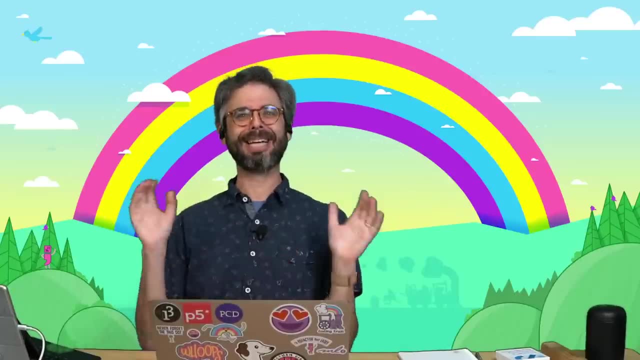 I will introduce in a moment who is going to do a presentation and write some code and really take over for quite a bit of time during this stream. So please bear with me if anything should go awry. I know that that's not going to. that's not a strange thing to happen. 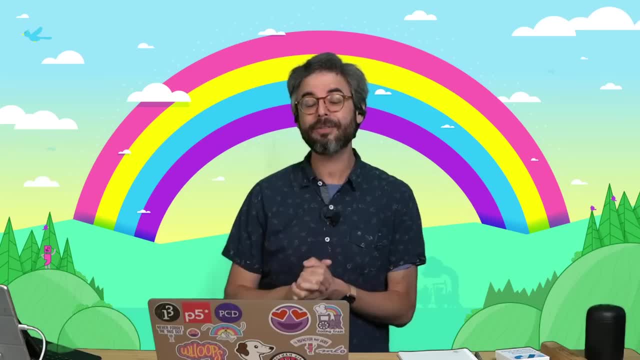 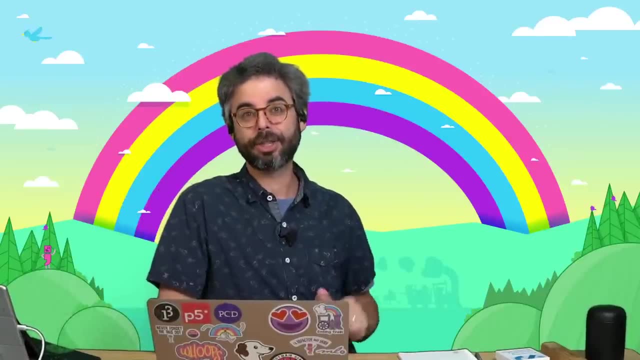 On a coding train live stream. If you happen to have come here- for I don't know why, I'm like burying the lead here- But if you are a, if you came here because you heard about this stream from Dr Christian Hubicki, who is the guest today. 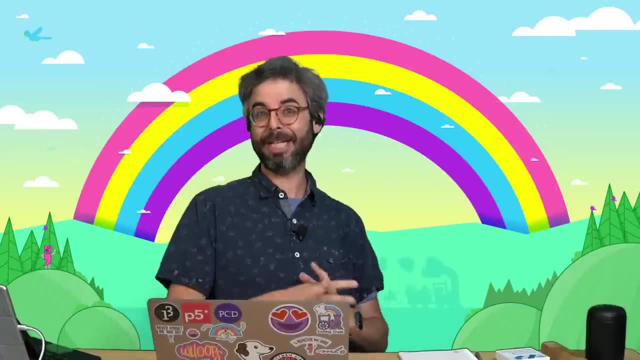 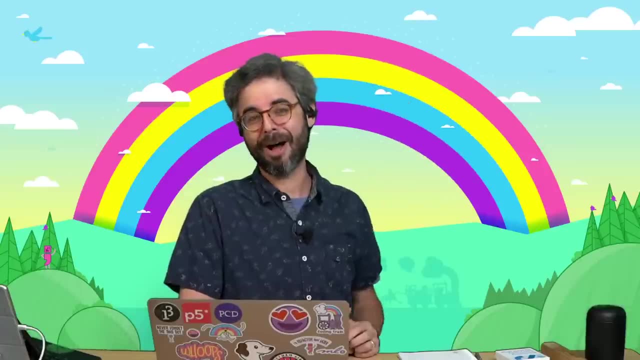 Let me just first briefly introduce myself. My name is Dan. I teach programming and I have so for almost 20 years in various capacities, at schools and workshops and online, now quite often on YouTube. I use a particular piece of software called P5JS, which I will come back to later in this. 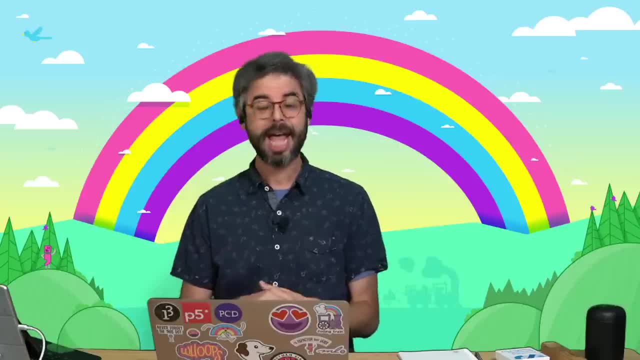 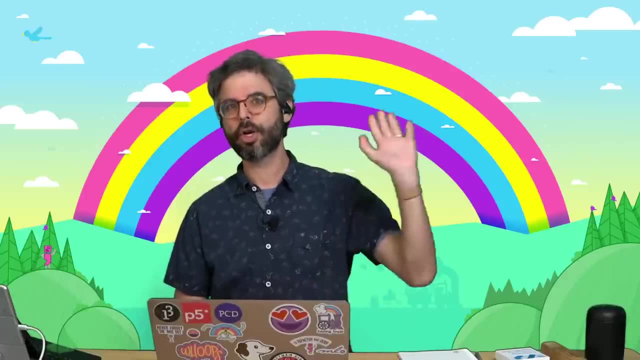 stream. And so if today is one of the first days watching the coding train and you've never coded before, I do have a whole intro set of tutorials that you might want to check out. You can just go to the coding train homepage and find the start learning here. playlist. 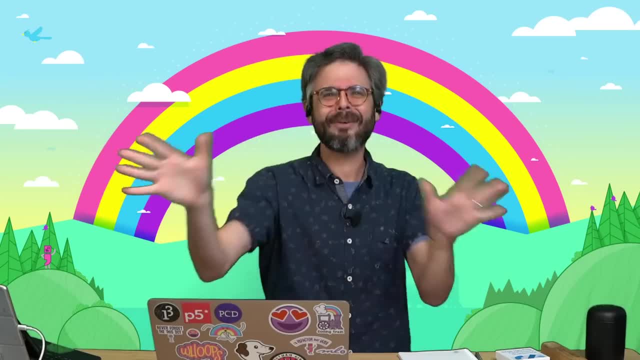 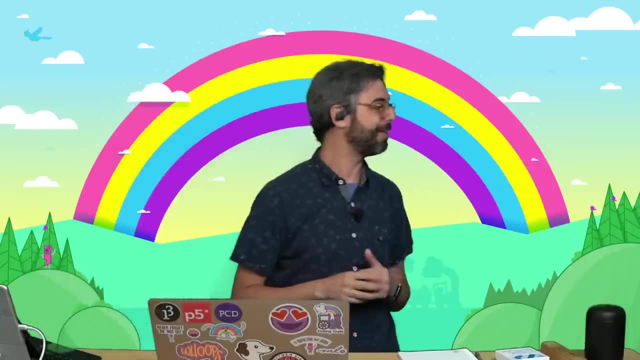 Anyway, I'm not here to promote myself. It's not what I meant to do. I just wanted to sort of set the table. for anybody who might be totally new, Let us know. By the way, I see people already in the chat saying I'm in Poland. 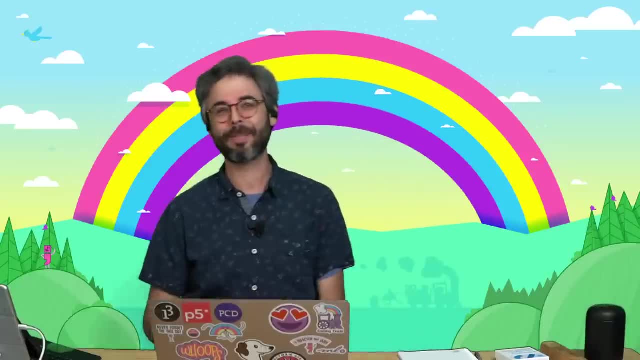 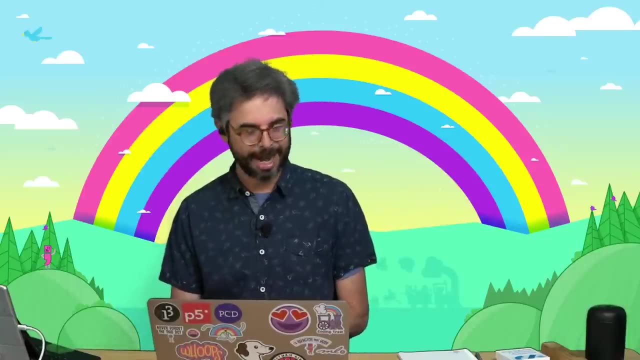 It's evening. It's 1 am Sunday morning here, So I always love to hear what people are watching from. So feel free to drop your location and time zone into the chat, But let me- and Christian, you're still there. 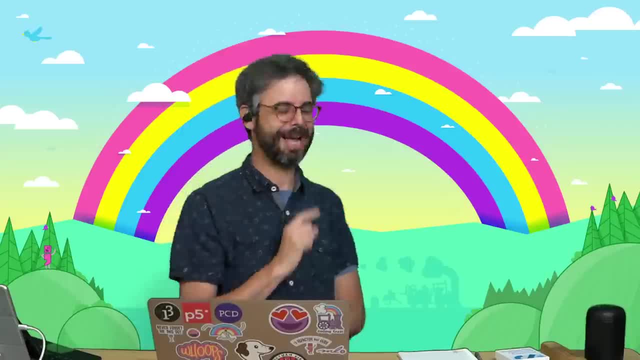 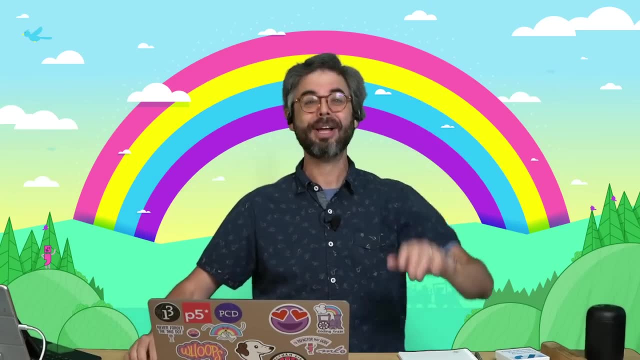 I can hear you in my ear. Yeah, Okay, great, So I'm going to let me. let me, let me get, just jump right in. I have a bad habit on my live streams of going on and on for incredibly long periods of time. 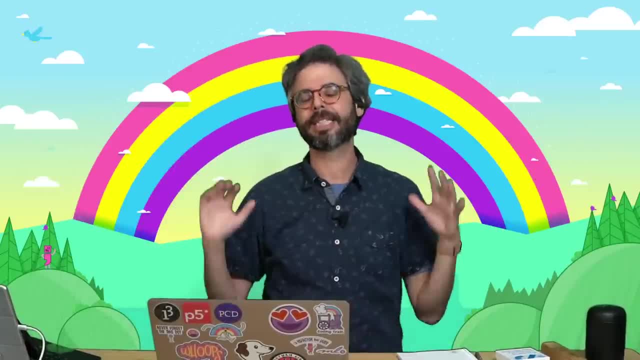 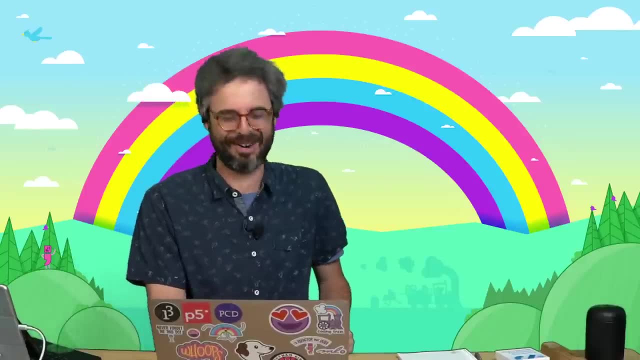 without actually getting to the code, And I do not want to do this today, because this is a really unique and super special opportunity to bring in a real life robot scientist, if that's an appropriate term to use. If you've watched The Coding Train before, you might know that I have a somewhat of a 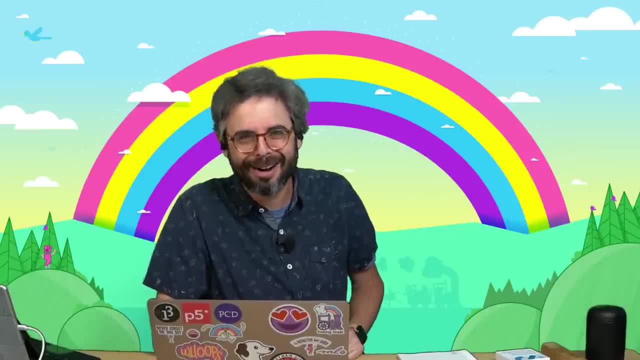 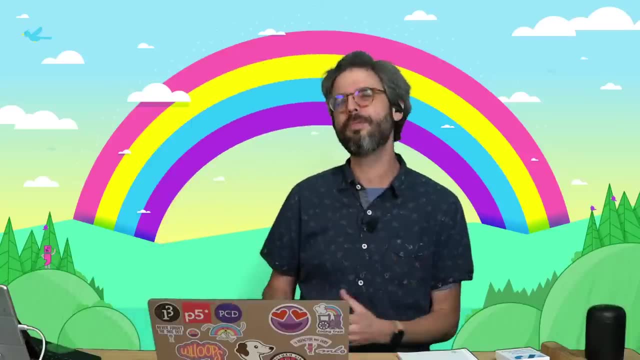 pathological fear of hardware and I'm not so great with soldering and programming microcontrollers and sensors and motors And I always want to do more with that And I hope maybe, maybe 2022 into 2023 will be the year for that. 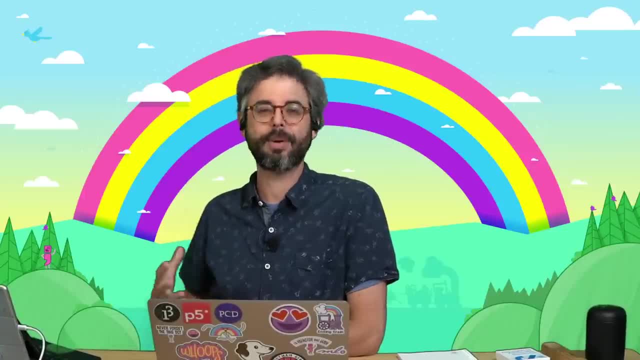 This, I hope, is a little bit of a stepping stone for me to be able to bring a guest who has real expertise in working with real life, moving around physical robots. I first learned about a robot. I first discovered Christian by watching the television show Survivor- American reality. 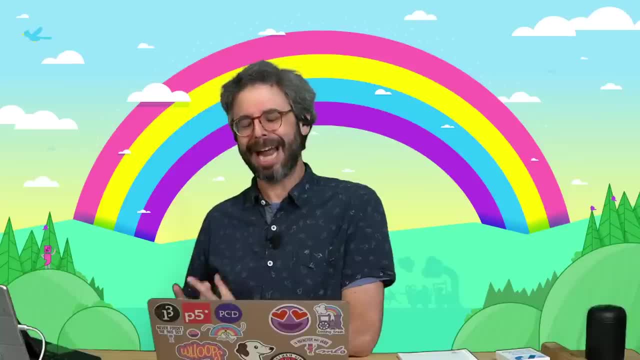 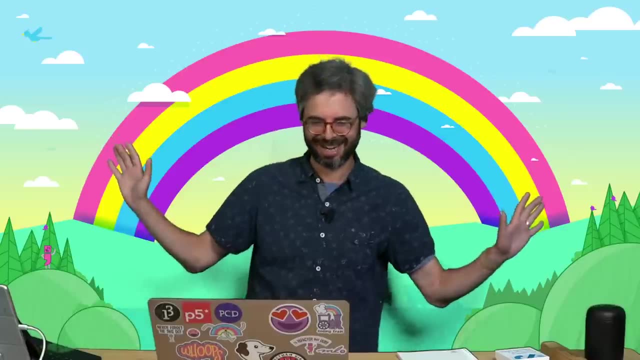 game show where he actually I was like I couldn't believe that a title of an episode of an American reality show was called Breath First Search. And that is all because of the amazing Dr Christian Hubicki. So he's got a bit of a presentation to introduce himself a bit more. 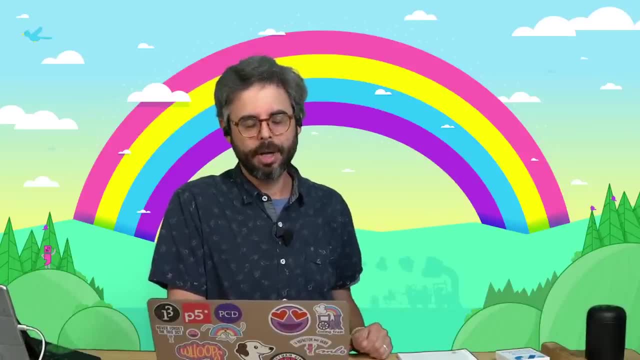 We've been in touch a little bit. Christian helped me. We had some back and forth on Twitter about the Monty Hart All coding challenge that I released where we discussed that a little bit. He did a live stream on Twitch coding the Monty Hall problem in Python. 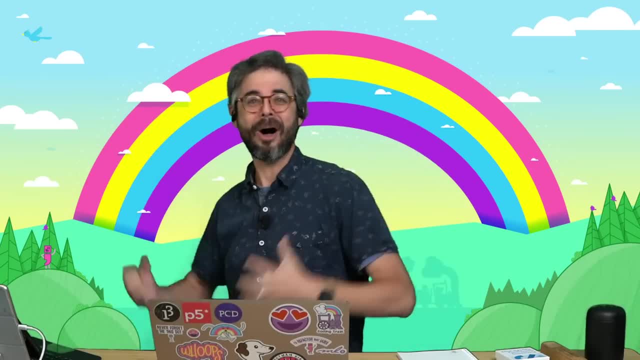 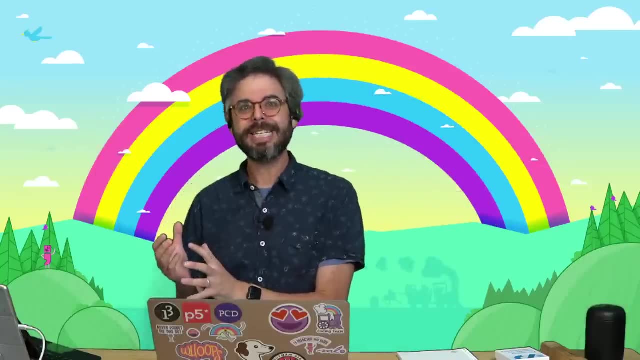 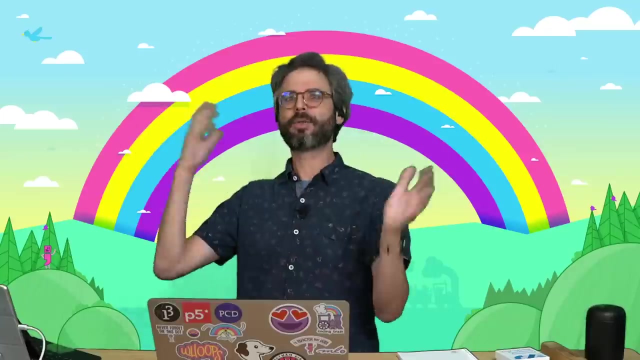 And I thought, ah, we've got to have Christian here on the coding train today. Everybody's always asking for Python, so we could do a little Python. I have all these videos about nature of code, simulation, simulating the movement of natural systems and often very much sort of just trying to create the feeling of those systems, not 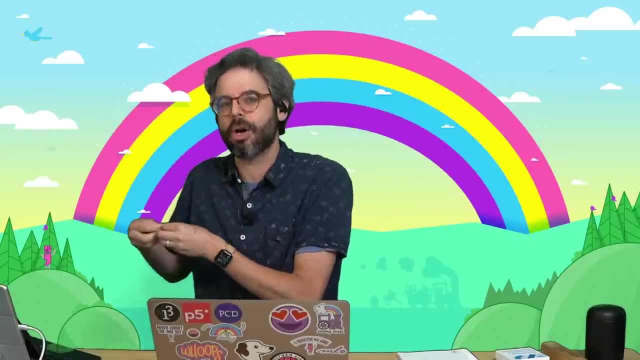 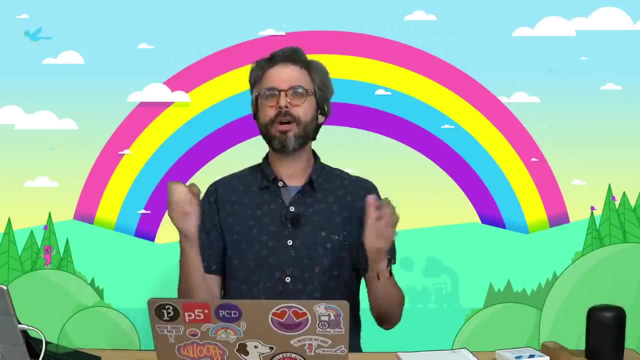 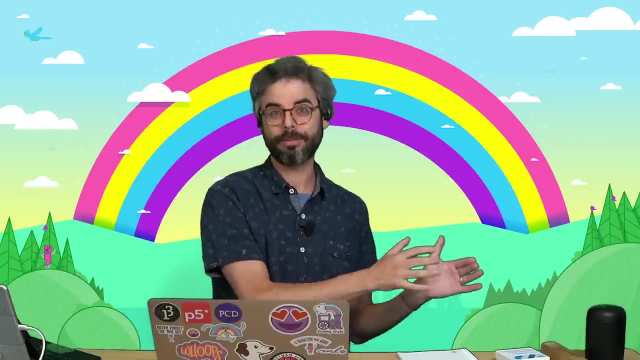 necessarily always reproducing the exact or biological mechanics of those systems through code. And so what I think- and hopefully this will lead to many more videos and coding challenges and things that I do in my own work- to look at: what does it mean to write algorithms to? 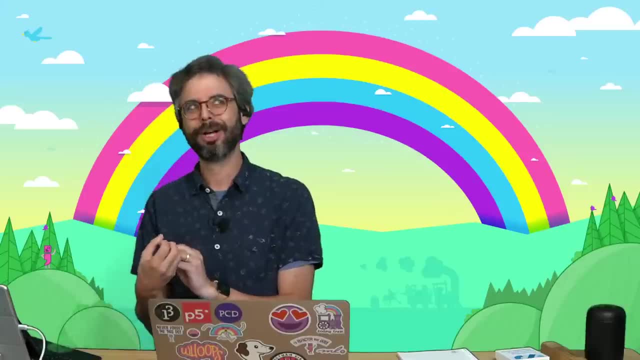 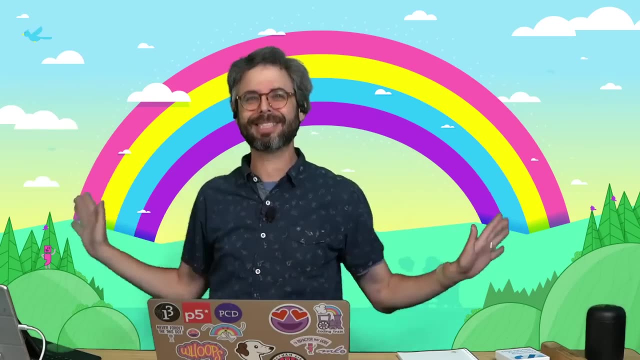 control the motion of robots, How does that relate to the controlling the motion of animated things in generative art systems, And where can we go from there? So there's too much to say about all of that. So that's my quick introduction. 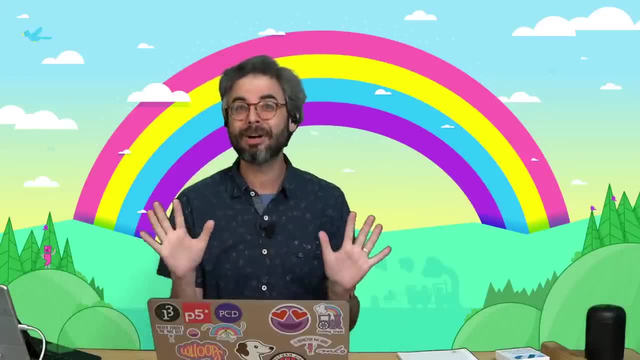 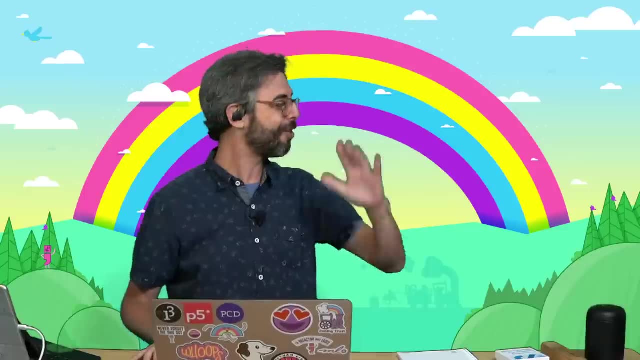 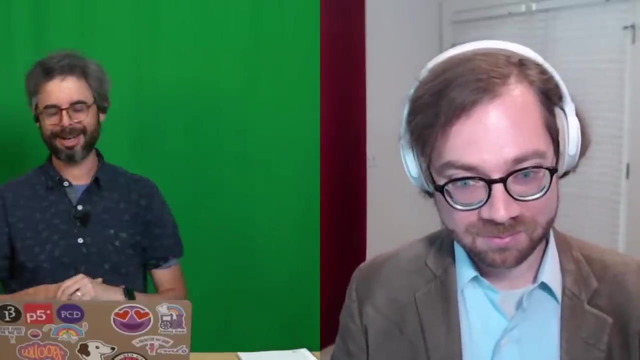 I'm going to press some buttons. Hopefully everything is going to work. You know, if we have to take a five minute break for me to fix audio things, I apologize in advance, But I'm going to turn it over. I'm going to attempt this first button, which will now put both me and here he is, the famous in my world, Dr. 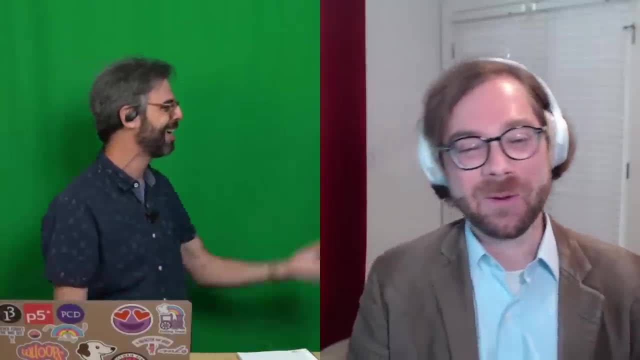 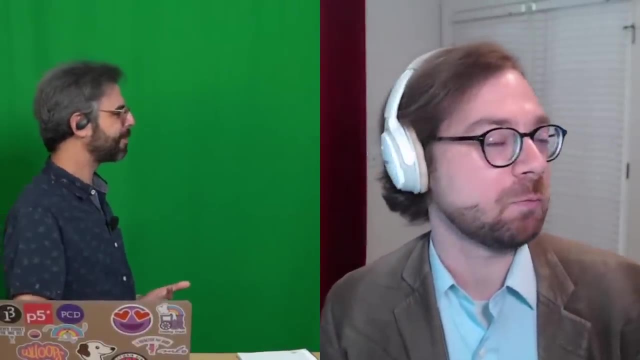 Christian Ubicki. Thanks so much for being on the coding train. It's a real thrill to have you here. Oh, thank you so much, Daniel. It's great to be here. Thank you, You know I what sort of opportunity to do some robot coding in a big public setting. 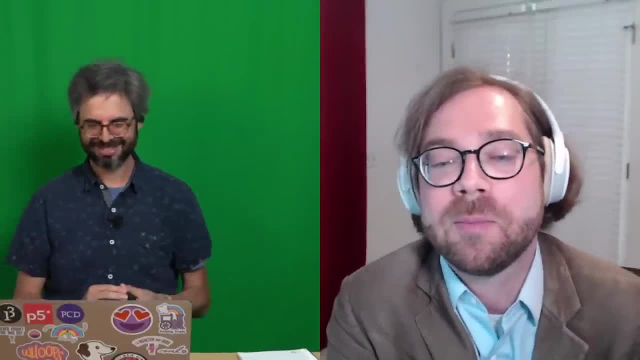 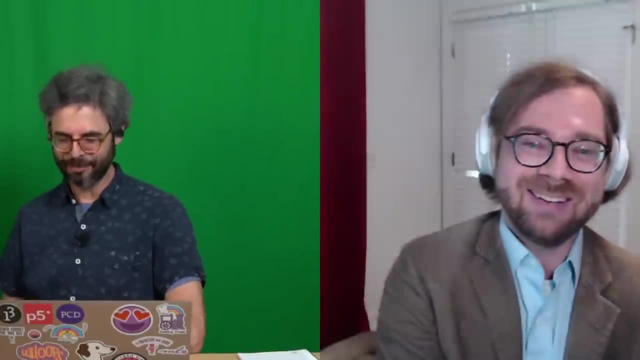 You know I couldn't resist. This is too much fun. So I'm glad to be here and I look forward to this adventure together. This is going to be a fun ride- I would say So awesome. So I just want to make sure that. I want to just see in the chat. 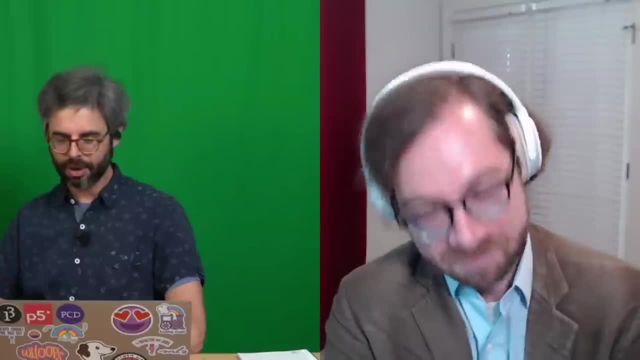 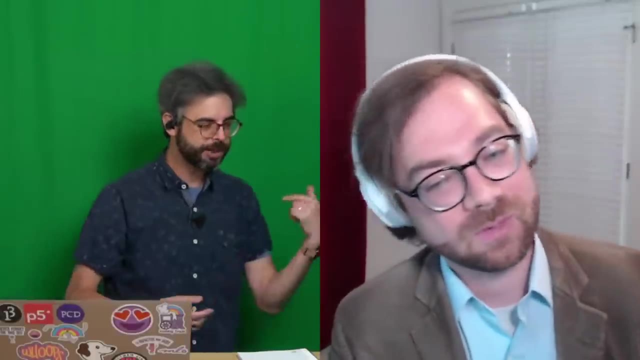 Everybody heard Christian. OK, the audio, the video, is going through. Please let me know. I'm kind of assuming it's fine, because I can see all of the dials and buttons going. So now I'm going to switch over. So now I'm going to switch over and let give Christian the full screen and let you take it away. 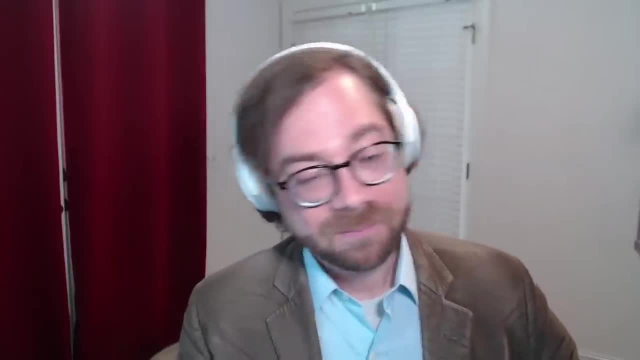 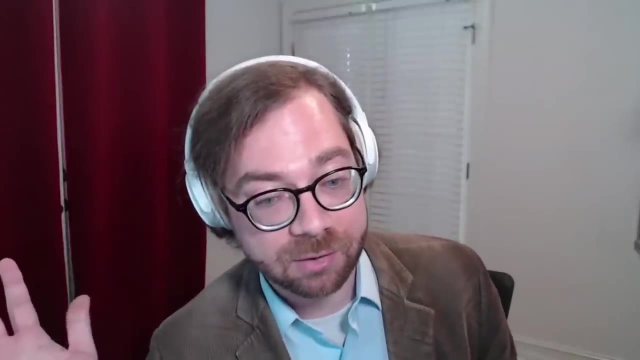 And I will be keeping an eye on the chat and I'll interrupt with any questions or things that come up. Yeah, This is going to be a good time. So, everyone, thank you so much for letting me be here today with you. I'm Christian Ubicki. 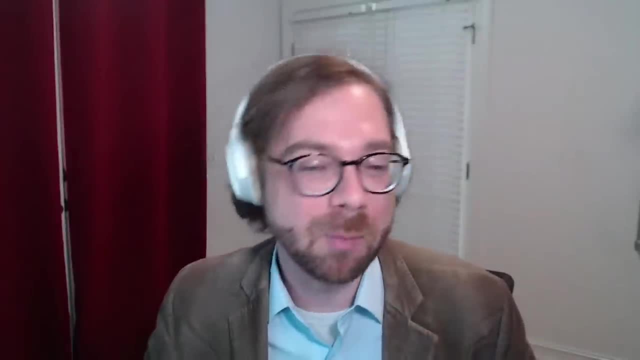 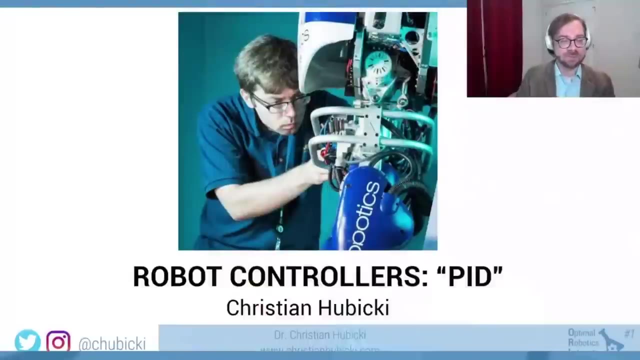 I'm a robotics professor. I have a PhD in robotics and mechanical engineering and I specialize in robot control. So I have a little presentation for you all today. So this, this is kind of me. during my graduate school and undergrad days, You know I like putting robots together, but especially I love coding robot algorithms. 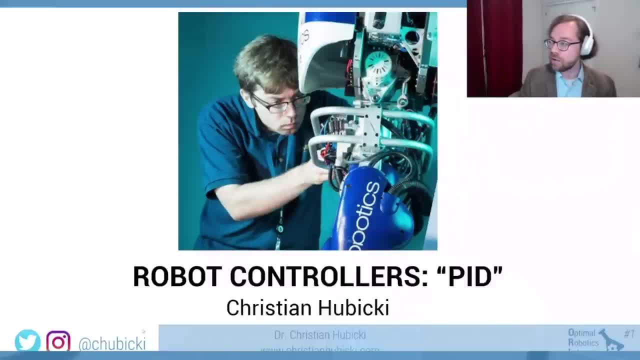 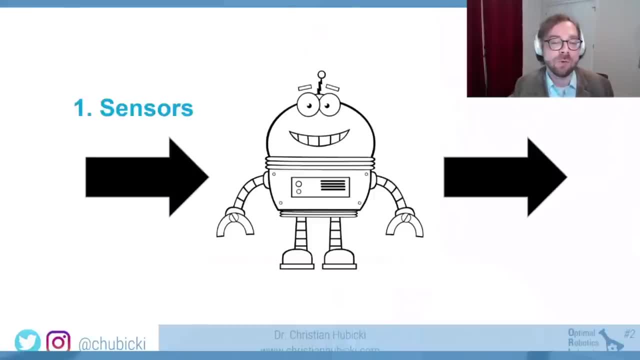 And in my world, when I'm talking about robot, when I talk about robots, I normally break it down into three categories of things that you care about with robots. Right One is that you have sensors that can sense what's going on in the world. 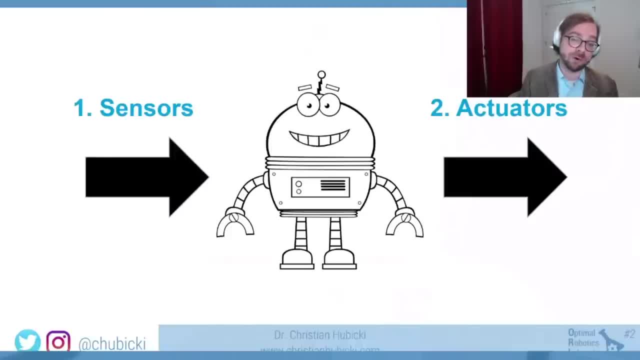 You have actuators that can somehow affect the world, And in the middle is this cool thing called control or a controller, And so my specific subspecialty of controllers that I work with are for robots that walk on two legs- bipedal robots. 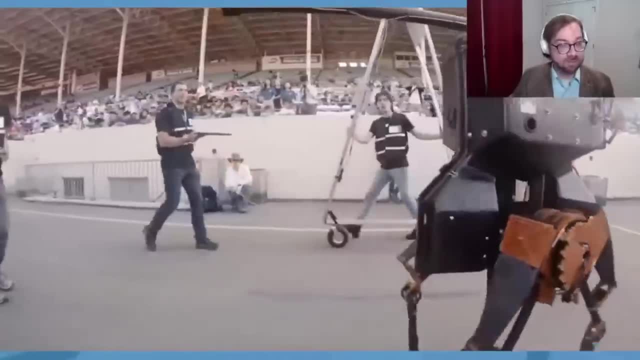 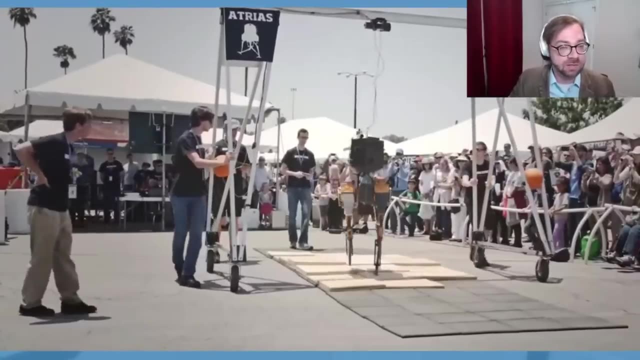 So this is just a little bit of a sample of the work that I've done with my colleagues during my graduate school and postdoc days and currently in my laboratory down at the FAMU FSU College of Engineering in Tallahassee, Florida. 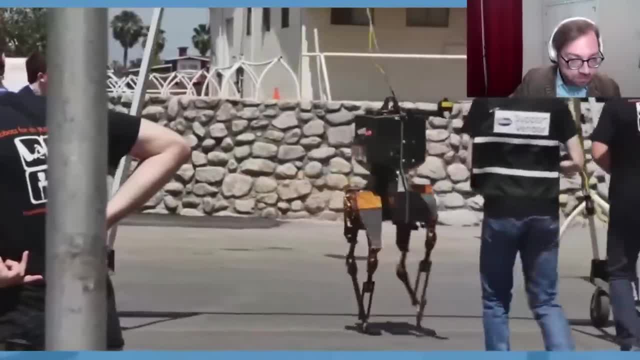 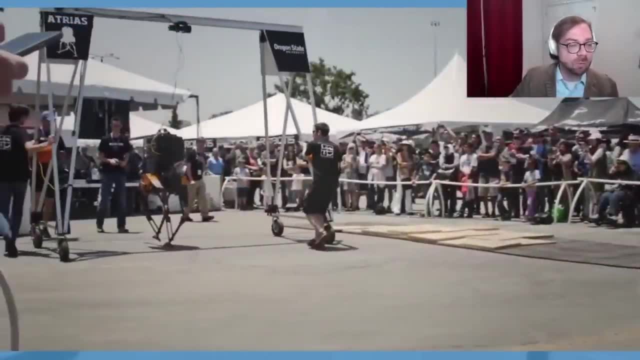 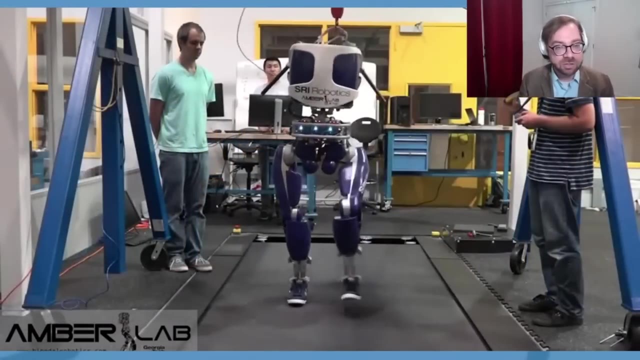 This particular robot. this particular robot is called Atrius. It walks around. It moves around and balances itself completely autonomously. We just tell it which way to walk and it walks in that direction. And here's another example of a robot called Durris that was designed to be a very efficient walking robot. 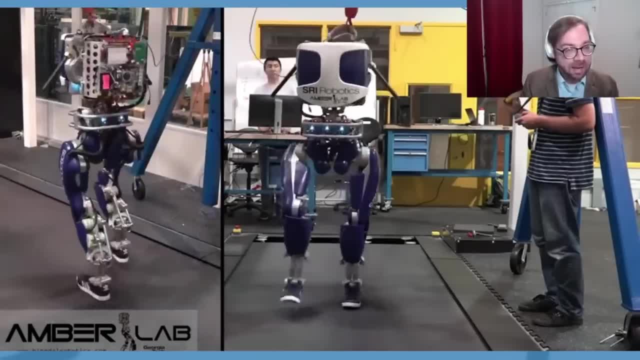 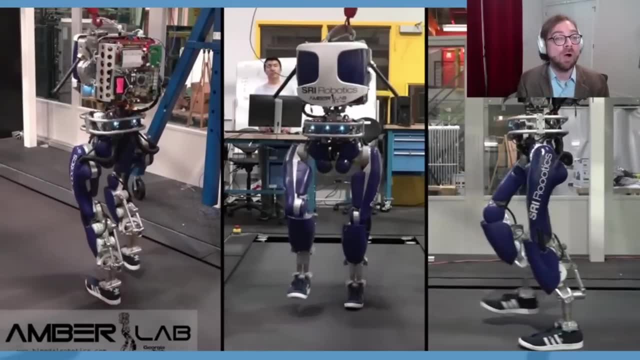 And here it is, striding from heel to toe. And when we were responsible with coming up with the algorithms for this thing to both stay up and also walk while using as little energy cost as possible. It's maximally efficient in how it walks. 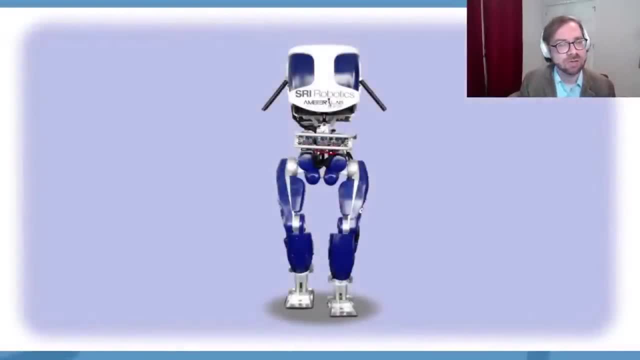 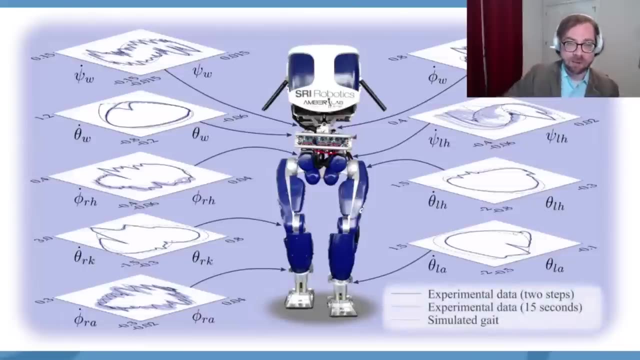 And under the hood there are some pretty fancy looking algorithms that you might expect to make it go. In fact, we would run these big optimization algorithms that would figure out all the ways to move all the little electromechanical joints on the robot to give it that striding motion. 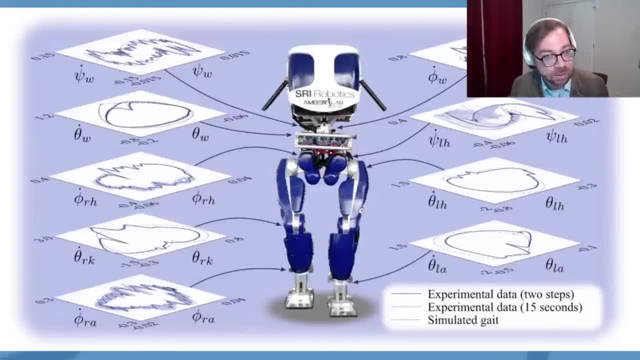 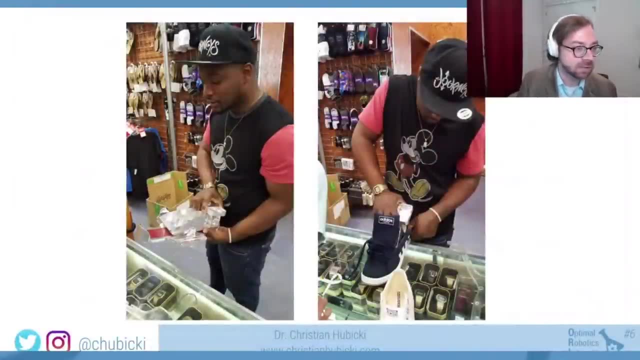 But I'm sure I know what a lot of you are thinking: Where does one buy robot shoes? The answer is the shoe store. like anyone else, In fact, we unbolted the robot's foot and took it the journey And this fine gentleman knew exactly what to do and put it on the shoe sizer and said, ah, size 14 men's. 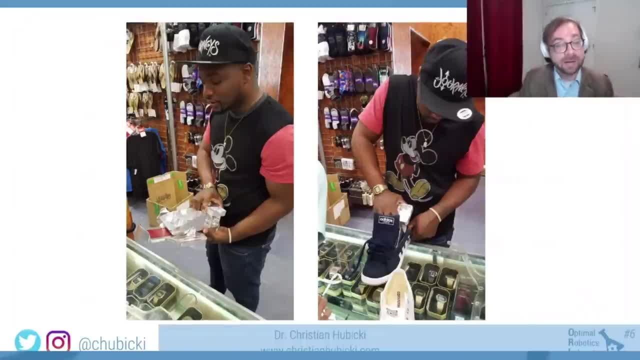 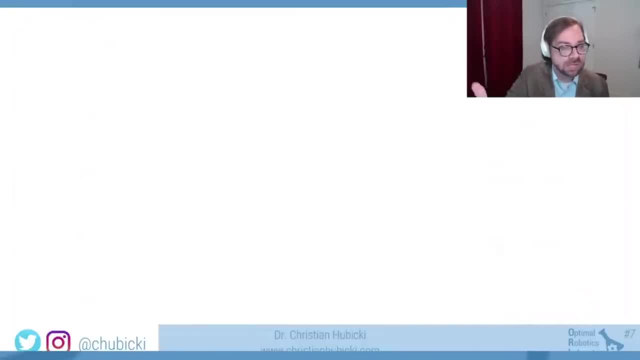 And he was exactly right. So thank you to that professional. But, like I alluded to, many of you are probably wondering how this is put together on a controller side. You think of a controller, you think of control algorithms, you probably think of code. 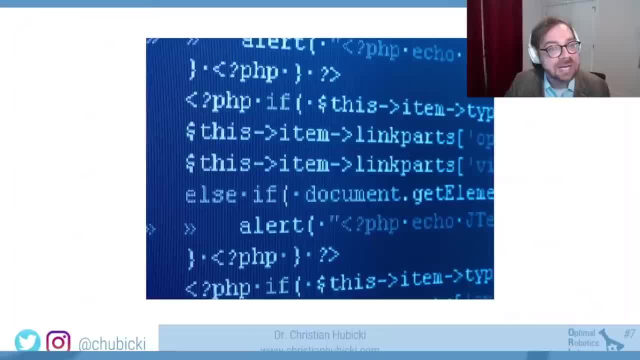 And this is in fact the coding train, And you would not be incorrect in assuming that there's code involved in coding these robots. There absolutely is. But fundamentally, Control algorithms do not need to even be code. They are much more general than that. 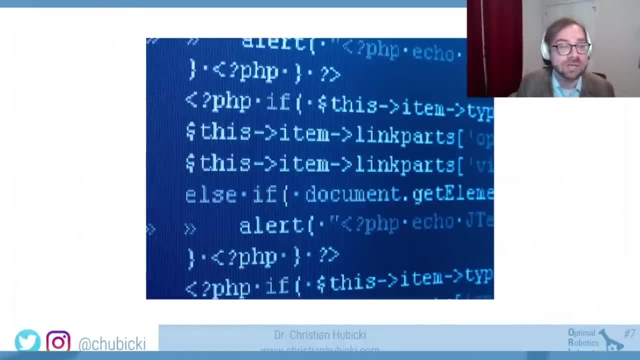 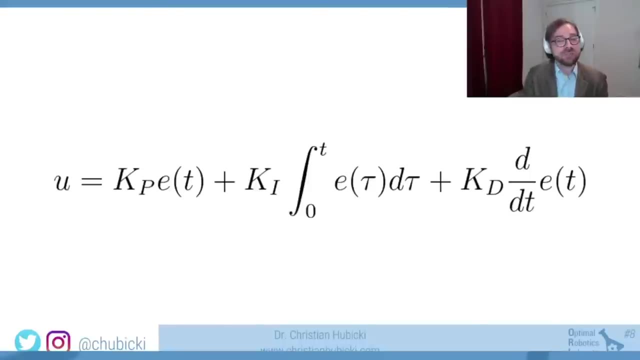 They are typically written as mathematical equations. In fact, when you think of control algorithms, you might want to think a little bit less about lines of code operating in a sequence and more something like this: an equation. Okay, So in fact, a control theory is often considered a subset of mathematics more than it is computer science, even though there are often very much. 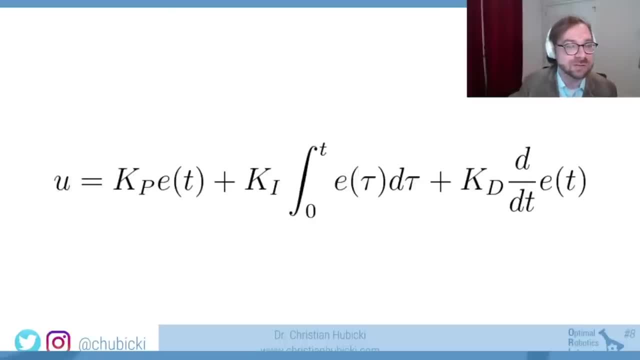 Computers involved in the code execution. So today we're going to break down controllers, specifically this controller. here, And where you can see there's a little P, You can see a little I, You can see a little D, This is called a PID controller. 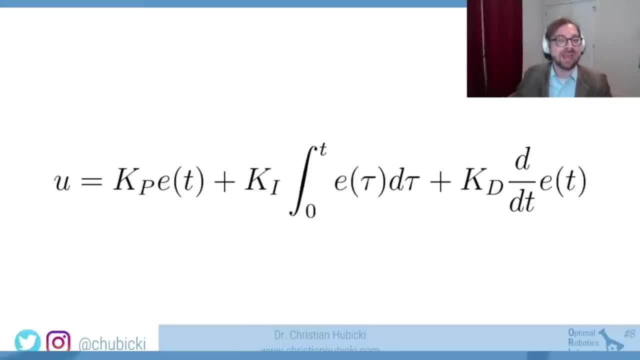 And we're going to break this down for you today- And as to why we use it and why it's so powerful, And why And why And how complicated these robots can seem. At their core, they're using this. Almost certainly the fanciest robot video you've ever seen on YouTube, somewhere down deep in the code, is something like this equation: 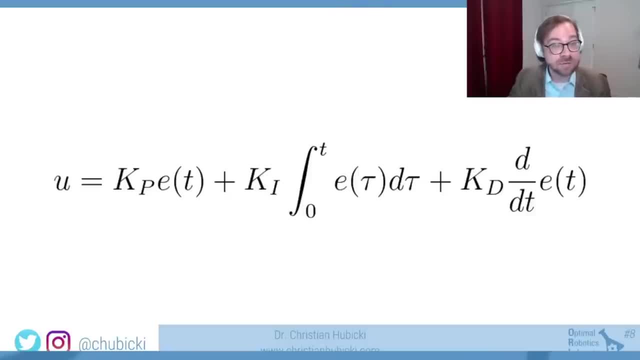 And it's very accessible in that. we're going to try to code it up today, and both in Python and also in these lovely online scripts. I'm looking forward to learning that from you, Daniel. That's going to be a fun time. But to get you started, one thing: I want to point out how to follow along. 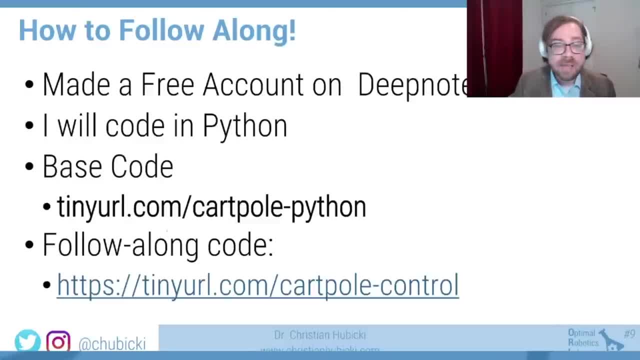 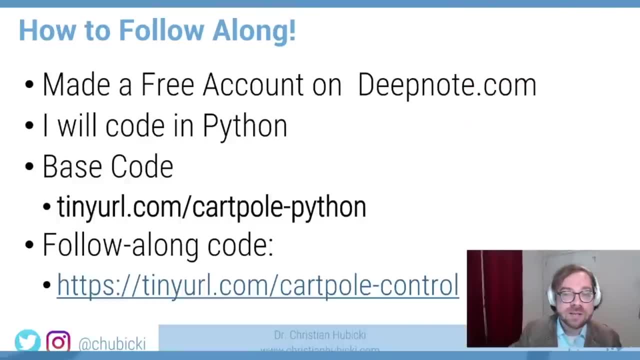 Okay. One is that you can make a free account, And I'm covering up this. I'm doing my own technical issues today. Let me make sure you can read this here. All right, You can make a free account on deepnotecom. 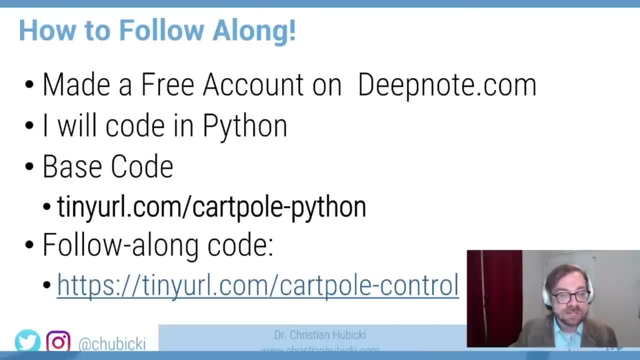 Okay, And if you go to deepnotecom, that is an online notebook that you can start up, that you can run your own Python code from scratch. Okay, And you can code up from scratch, But you can make a free account. 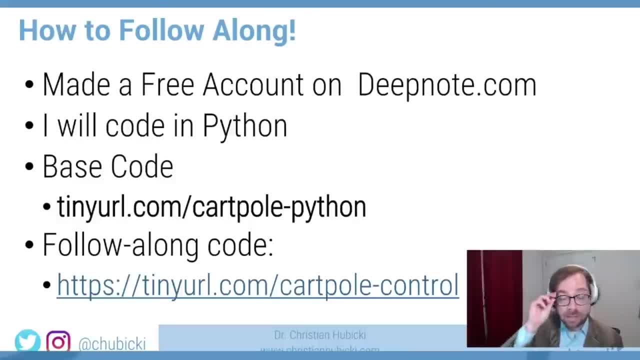 And that will allow you to run your own code and also other people's code. I will be coding in Python today And I have some base code set up here And I just made a quick tiny URL link for you to go to. Go to tinyurlcom. 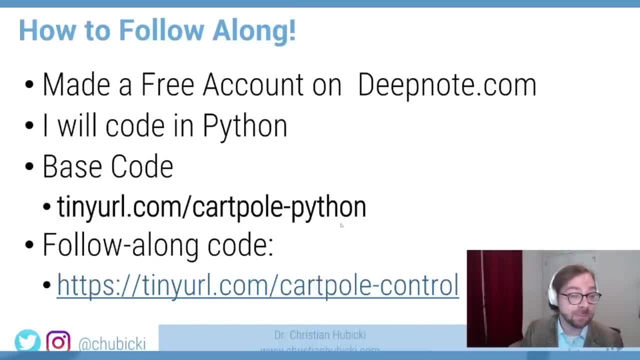 Slash cart poll- hyphen Python. Cart poll- hyphen Python. We'll be controlling this cart poll today And I'll get to that in a minute. If you have any questions, You can actually run this code by hitting the little run button. 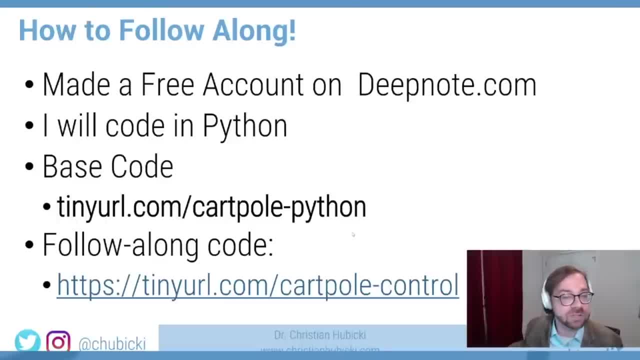 And it should execute. It might take a minute or so And it will create a little video that you can download and watch. Okay, And I will be coding at this link here, cart poll slash control, where you can watch the code change live. 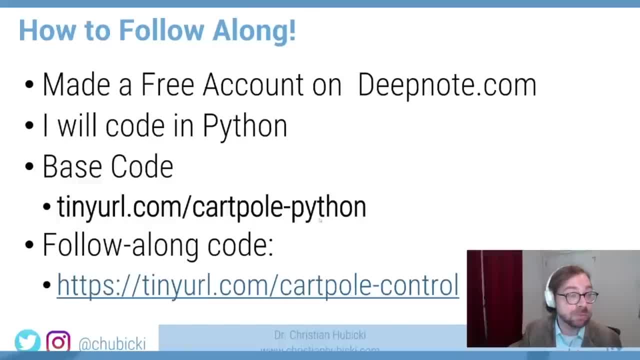 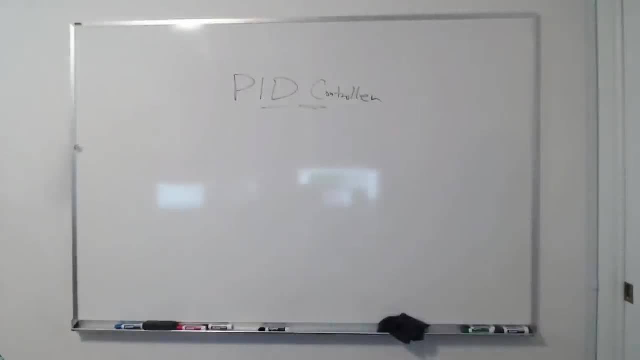 Okay, And you can make your own duplicate copy of it once you make your own deepnote account And that's how I'll be coding today. All right, So with that, I'll go over to my whiteboard and we'll get started covering the basics of the PID controller. 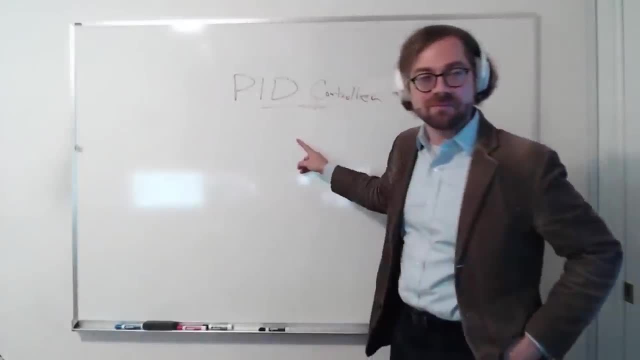 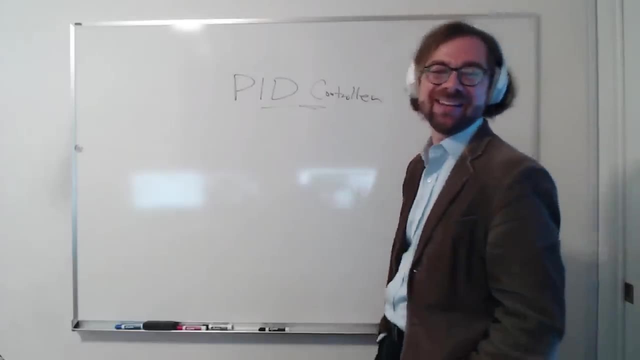 There you go. This is a very exciting moment because I'm constantly using a whiteboard And I think this might be the first remote whiteboard appearance on the coding train. Great, Okay, And, as you can see, graphics design is my passion. 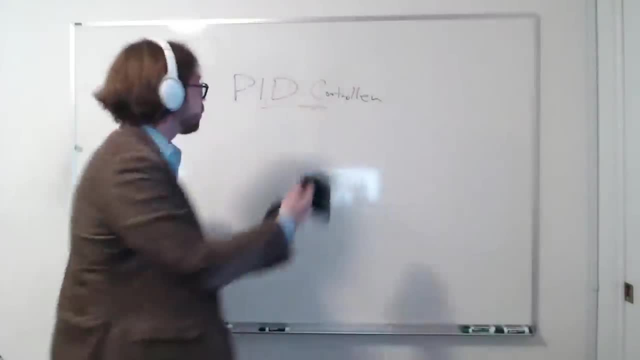 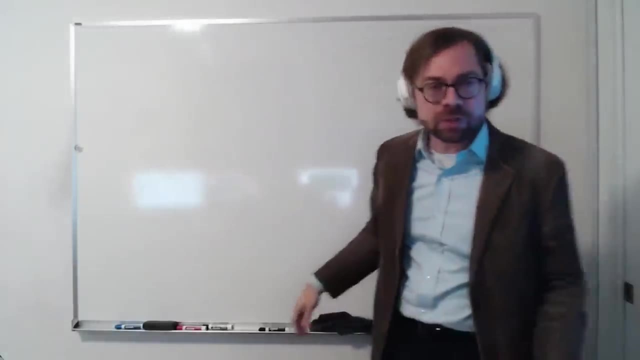 You can tell from how I've set this up for you all. But yeah, PID controller. Let's back up first about what we mean when we want a controller. Well, the first thing we need to ask ourselves is: what do we want to do with a robot? 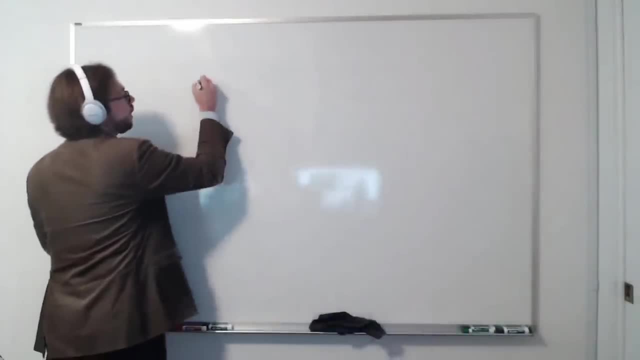 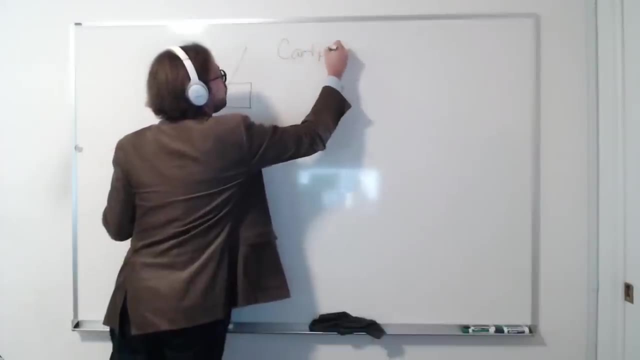 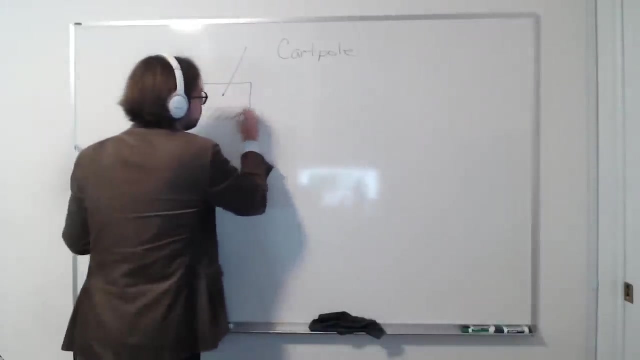 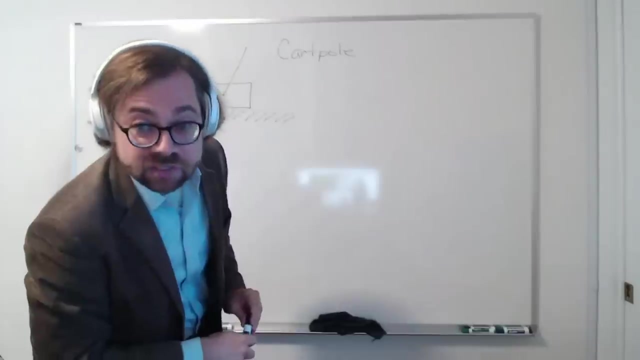 And the example we're going to do today is something called the cart poll. Okay, Classic example. You have a sliding- I don't know what- your whiteboard marker. luck is like here, Daniel, But you know, whenever I go to a marker, I'm like it's never working exactly as I planned it to go. 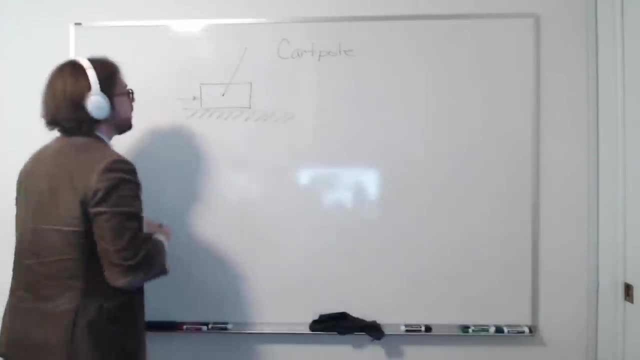 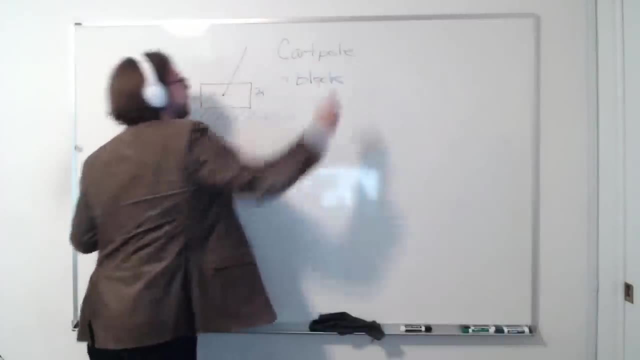 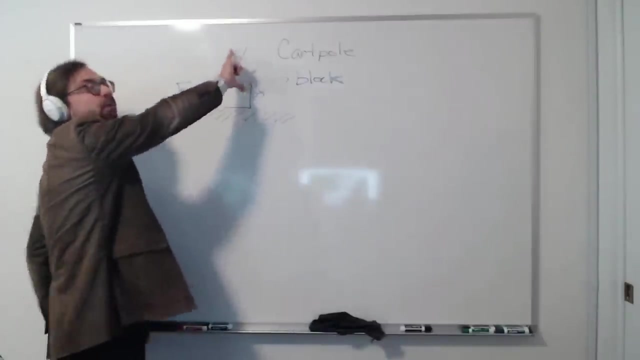 It's almost like a tech check of its own. Let me do my blue here. So this cart poll is this sliding block, Okay, And you can push it around with a force. You can push it like with your finger And you want to balance this poll on top. 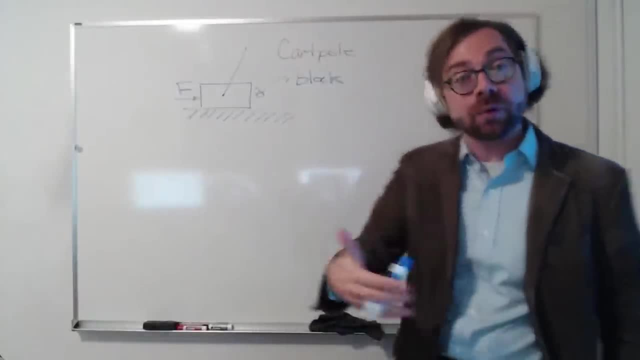 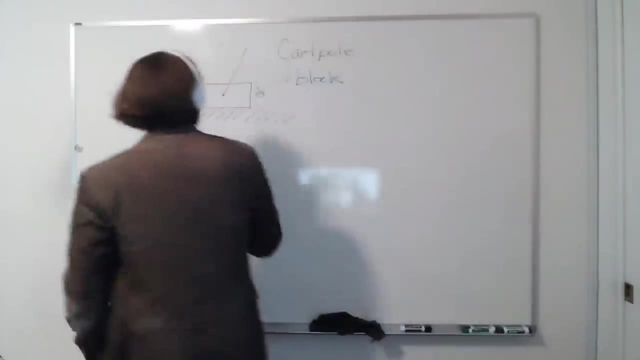 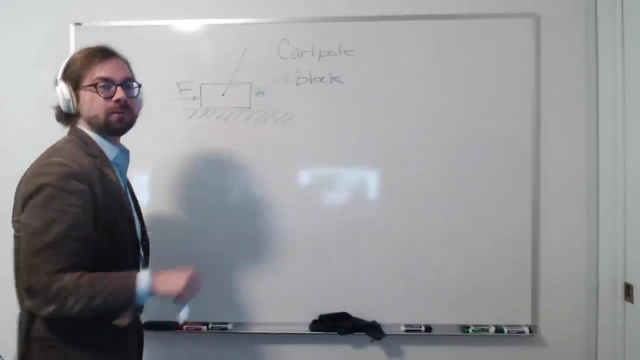 All right, Kind of a classic control that we all learn when we're teaching control theory classes. We're trying to learn the fancy ways to use controllers, Okay, And what we often want to ask ourselves is: what do we want to do? And in this case, we want to balance this poll. 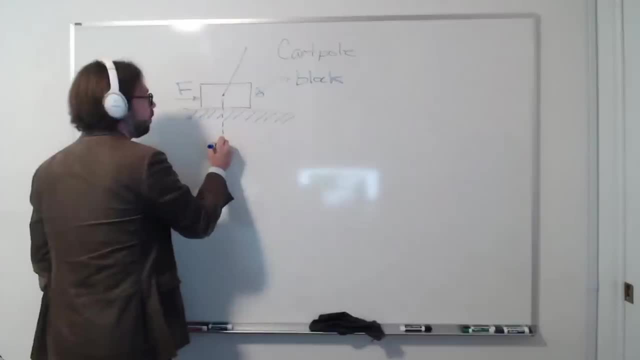 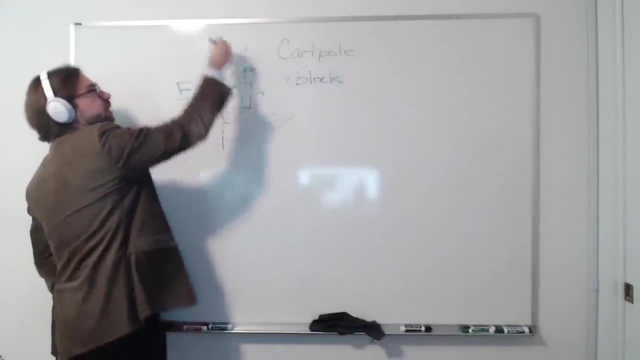 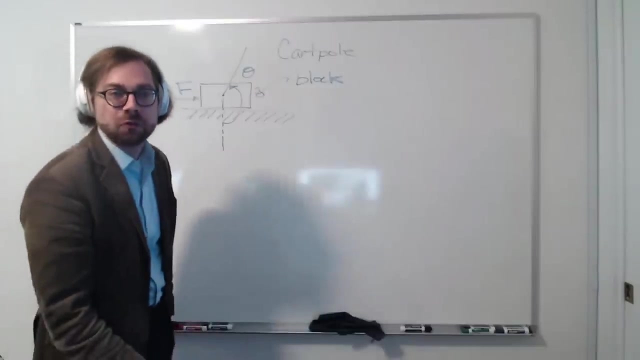 So we might say, hey, If our poll is at this angle, theta- Okay, We want theta to be up. And if you work in radian land, that's pi radians. If you work in degree land, it's 180 degrees. 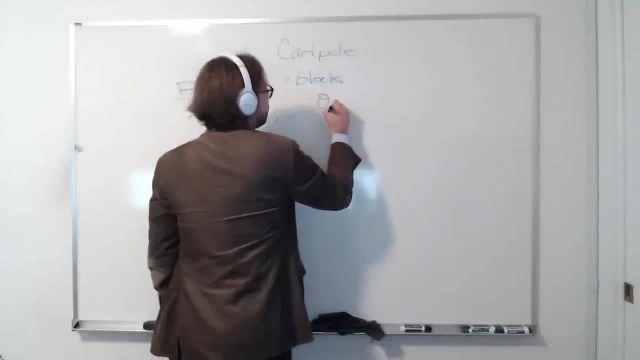 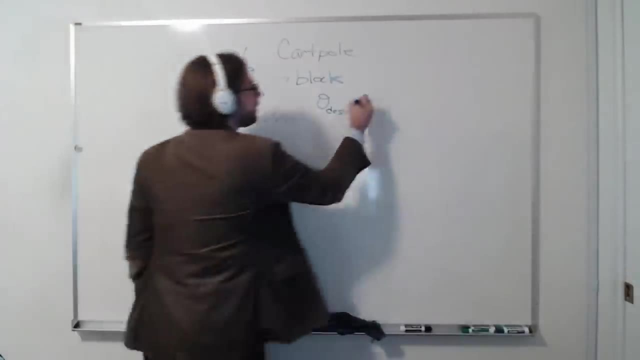 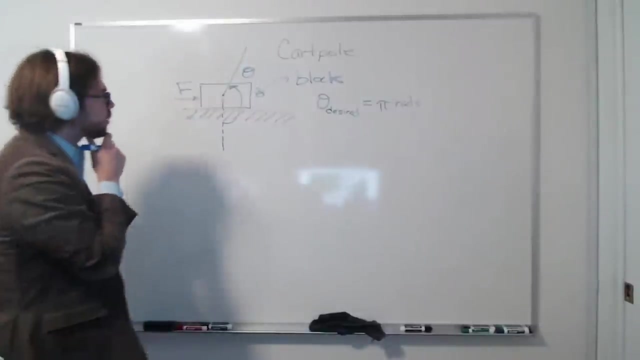 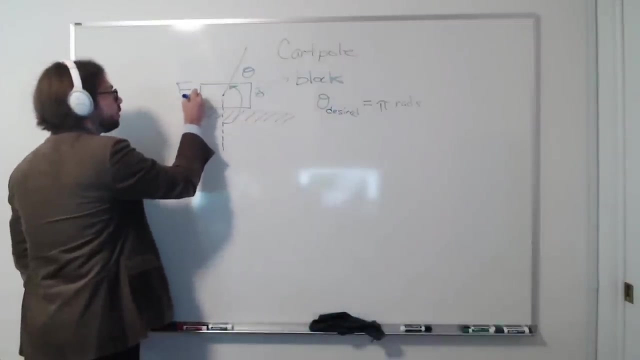 So you would say, hey, I want my theta desired. I desire a theta to be pi radians. Okay, And that is what I consider my output, The thing I want to happen. Okay, And you can also have an input to your system. 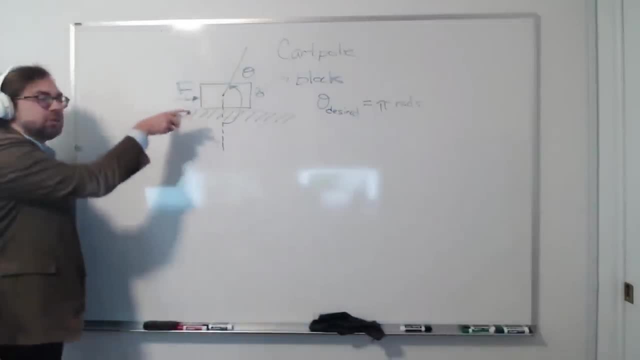 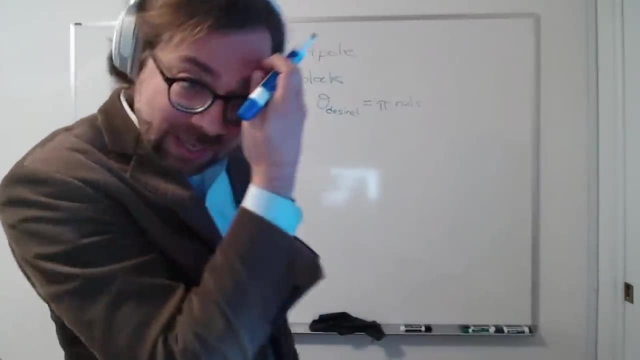 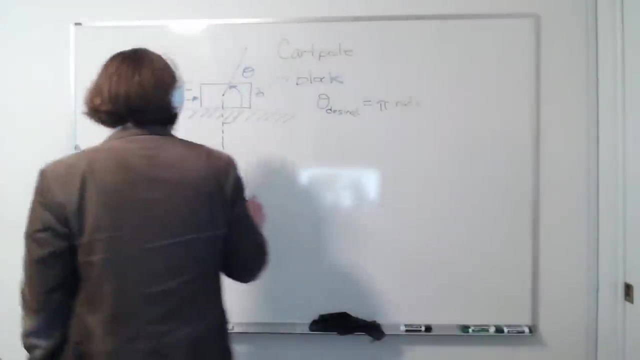 And there are lots of different kinds of inputs to your system, And the most obvious input to this system is this force, The force that we're applying. Okay, And that is true in that that is the physical input to the system, But in the controller we will often say, as our input, our theta desired, 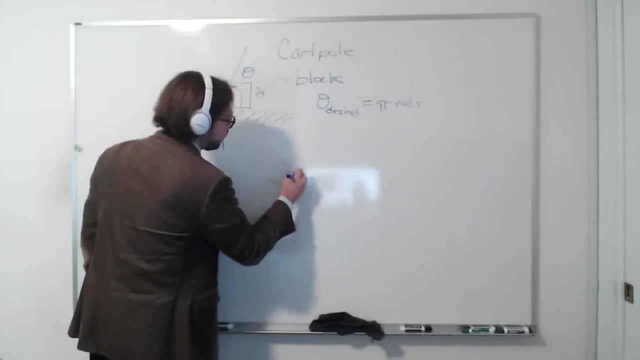 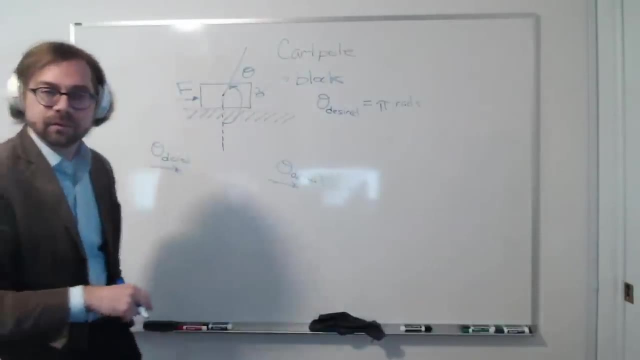 And our output? is our theta actual? So we want to have a desired theta. Let's say it's pi, Okay, And our output? I'll try to block the glare here. I don't know if I can do that or not. 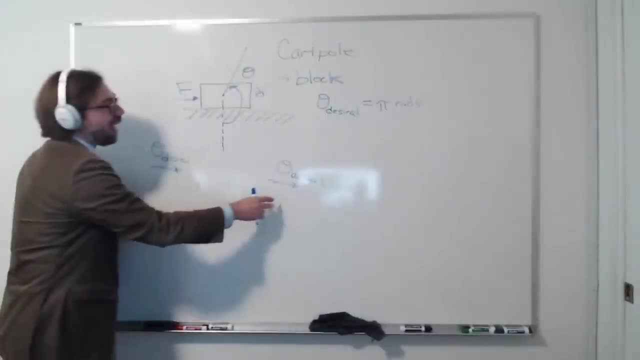 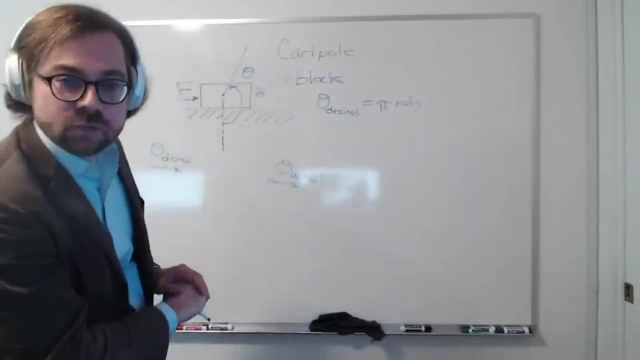 But hopefully So doing my best here. So theta actual, This is where we're actually at And we want to get to our desired angle. So when we've achieved our task in the controller, theta actual, we'll use red. 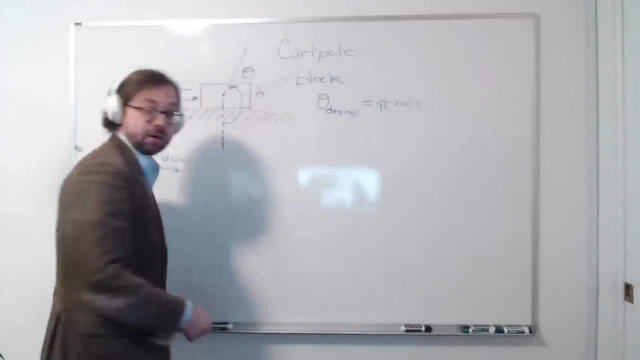 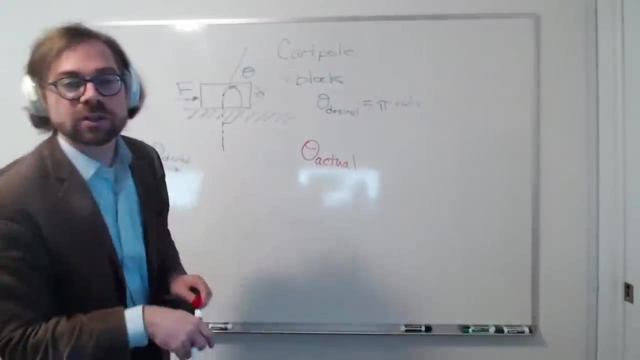 We're on a whiteboard streak here. We're going to try new markers here. By the way, I'm quite familiar with this problem. That red is beautiful though, So you're coming through. Let's go with that red. Let's go with that red. 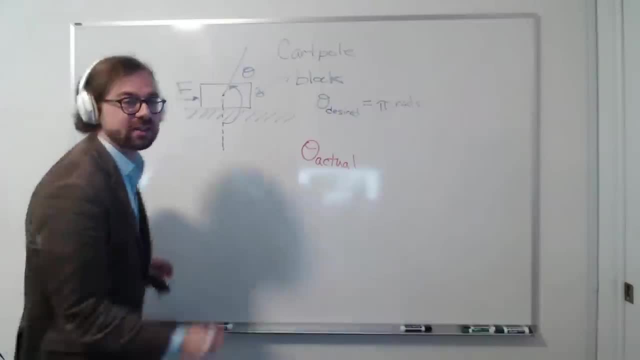 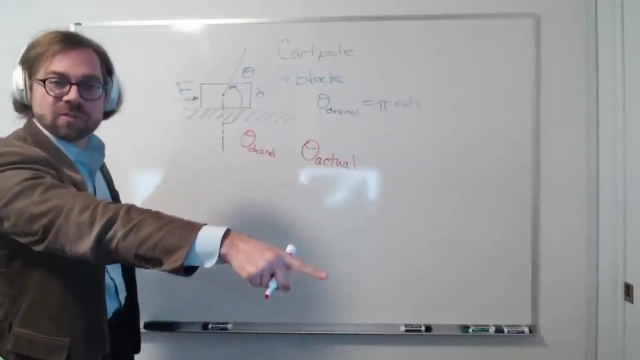 All right. So thanks everyone, as we work through these highly technical difficulties here. We want our theta desired, We will put in our theta desired that we choose, And then we want this system to go to, in actuality, where we want to go. 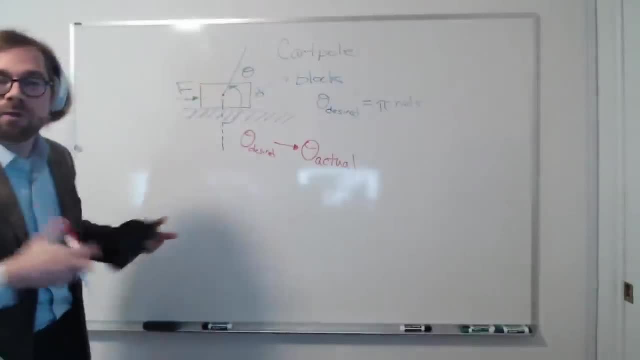 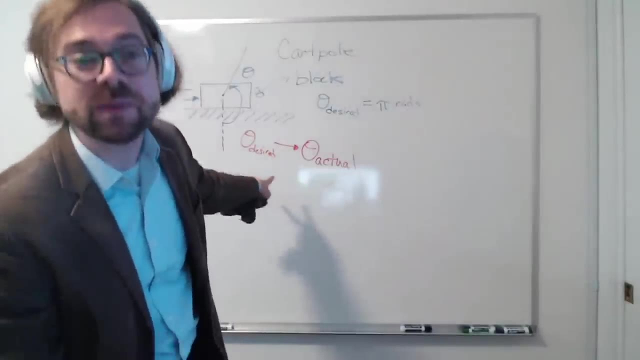 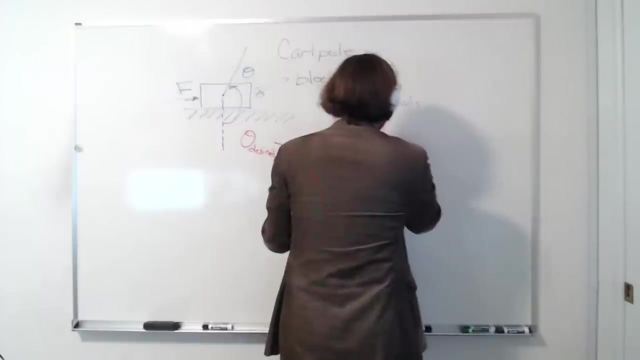 So from one point to the other, Okay, And when we've succeeded, the difference between these things is what? It's zero. We want them to be the same, Okay, So We call the difference between these theta desired minus theta actual as a special name. 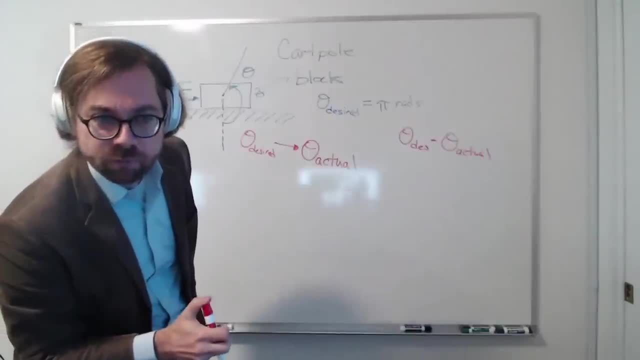 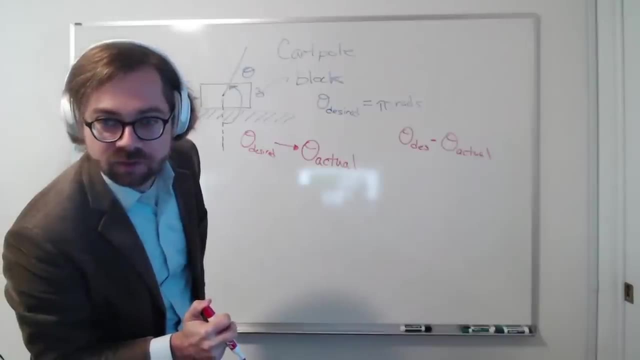 It's called an error. I can't imagine we're familiar with errors here on Coding Train, are we? I'm sure you never get those. We refer to them as happy little accidents. Happy little accidents. Well, here we call them. the technical term is error. 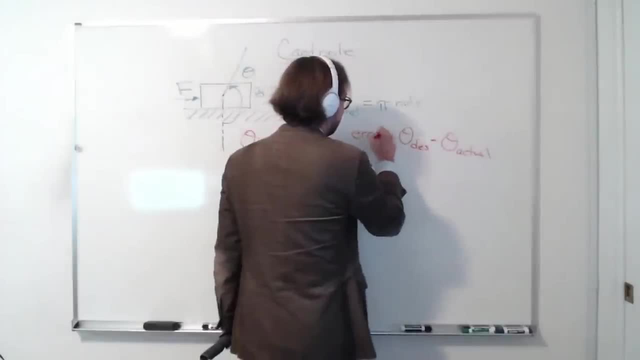 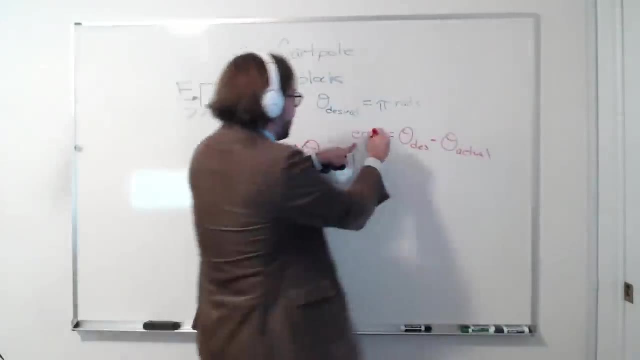 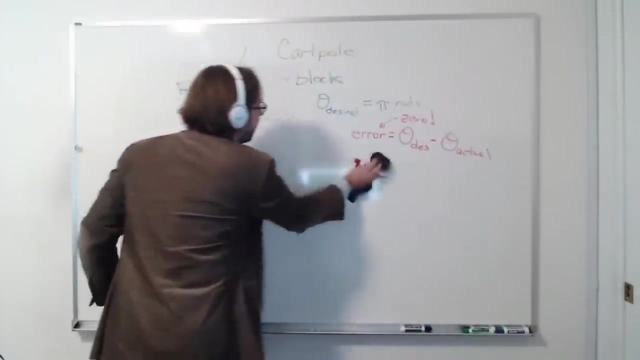 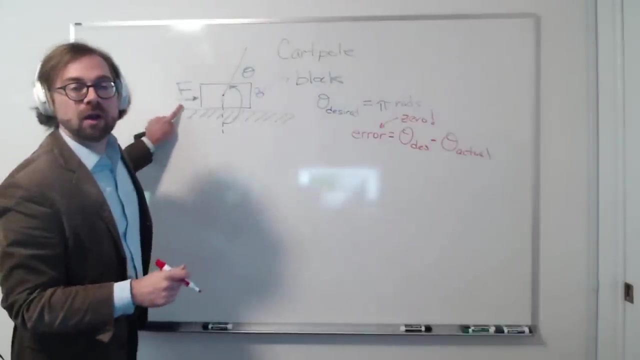 Okay. So we say error is equal to theta, is equal to your desired minus your actual, Okay, And we want to drive that error to zero. We want that to be zero. But how do we do that? Okay, Well, what we do is we decide- is we need to come up with some way of changing our force. 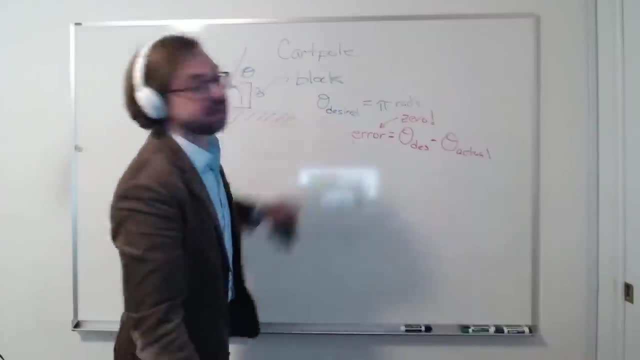 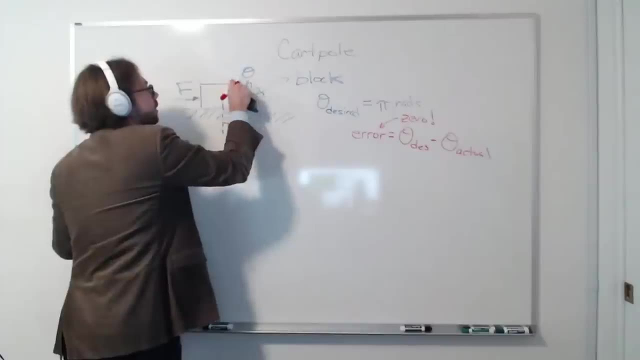 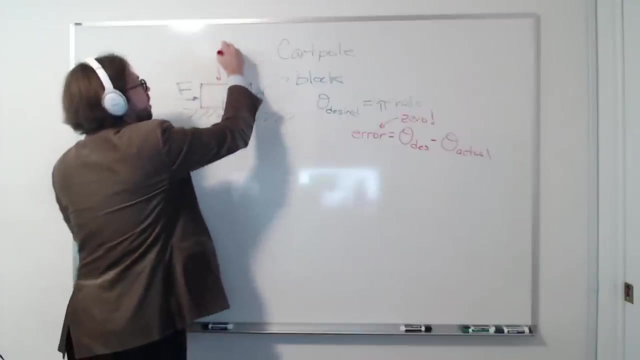 So that way it maneuvers our system to where the error is zero. Okay, And to make this problem even simpler, for explaining what we're going to do, I'm going to get rid of the pole and just do the cart, which has some mass. 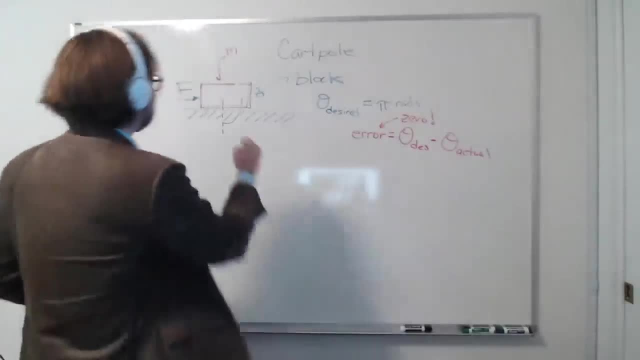 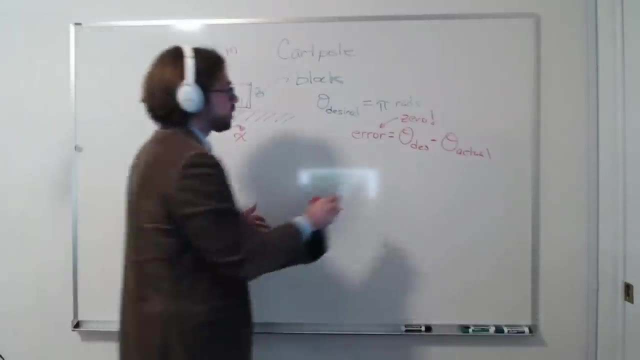 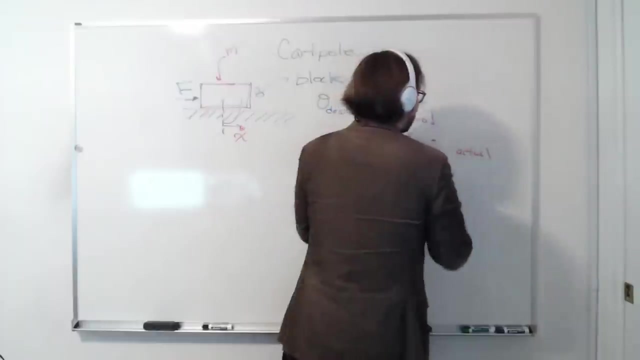 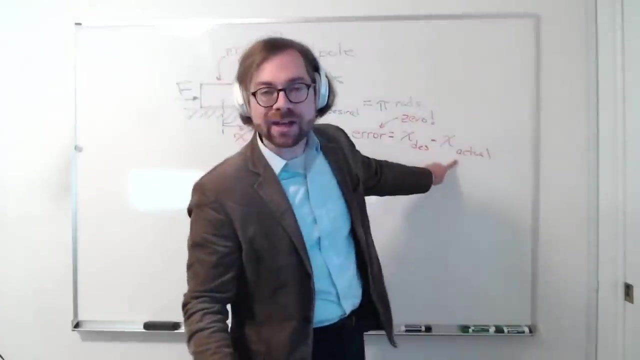 Okay, I'm just going to care about the position of the cart, which I'll call x Okay. So now I'll have some x desired and some x actual Okay. So at any given time we can measure where we're actually at. 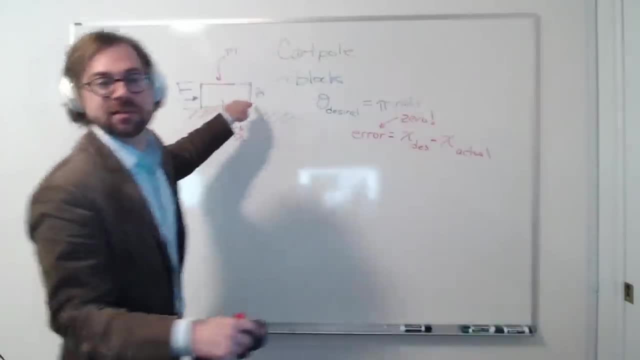 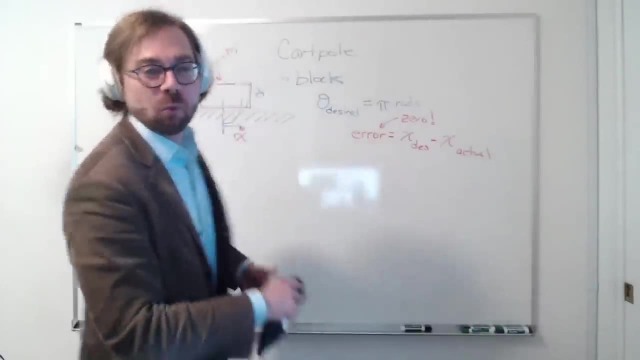 Right, You know, we know it's there, or we know it's there. We know it's there And we know what we want. We get to choose it, So at any given time we can determine what our error is. 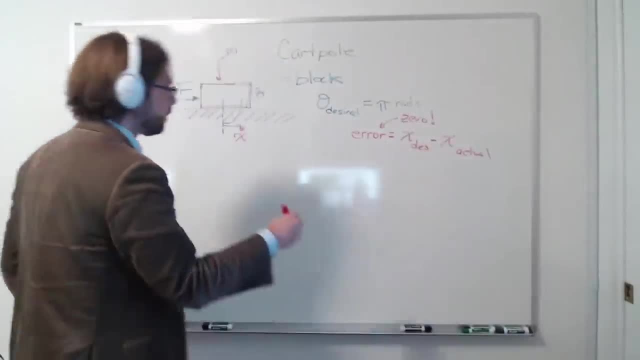 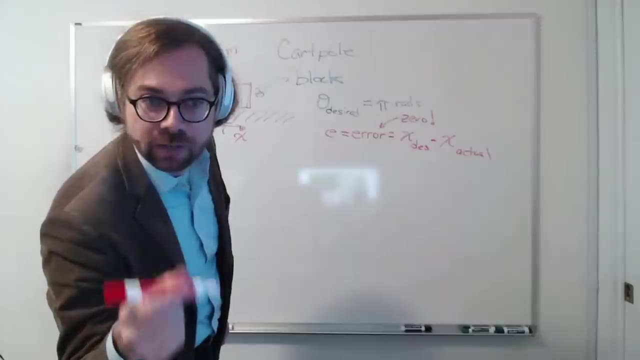 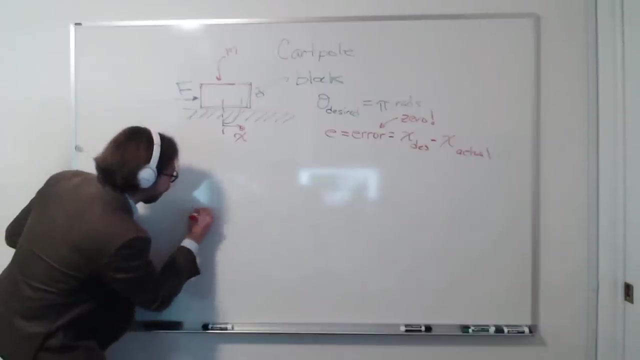 We can take our desired and minus our actual. Okay, And we'll call that e to save me this precious deep-looking marker. Okay, We'll just call it e instead of error. So we need some kind of equation where we assign our force to be equal to something. 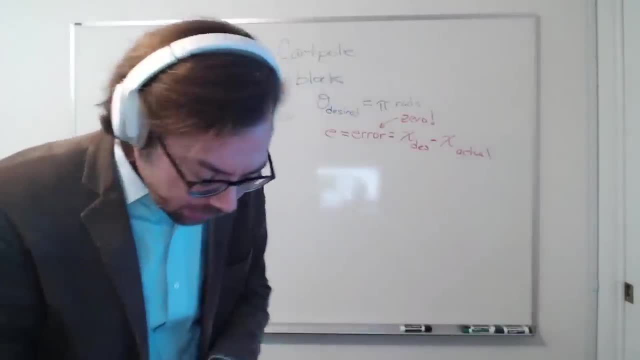 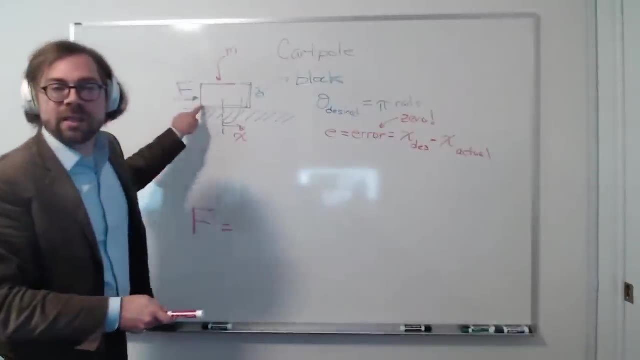 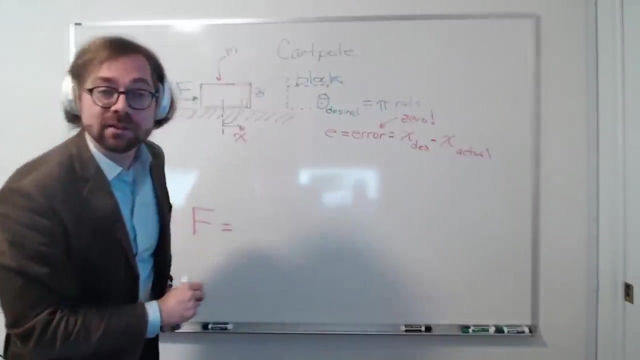 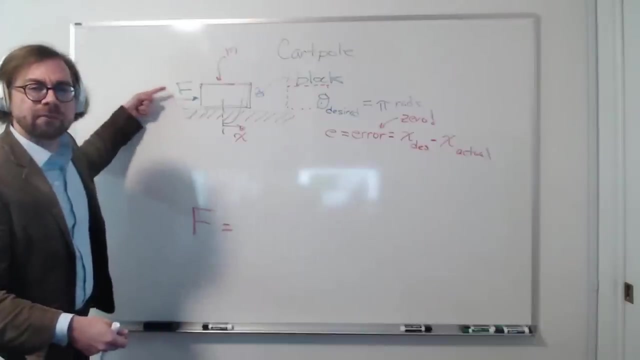 Okay, And one way that we could do this is we could say: hey, I'm currently here, This is my actual position. I want to get over here, which is my desired position. I can subtract them, get my error And I can say: well, my force that I apply should be proportional to how far away I am. 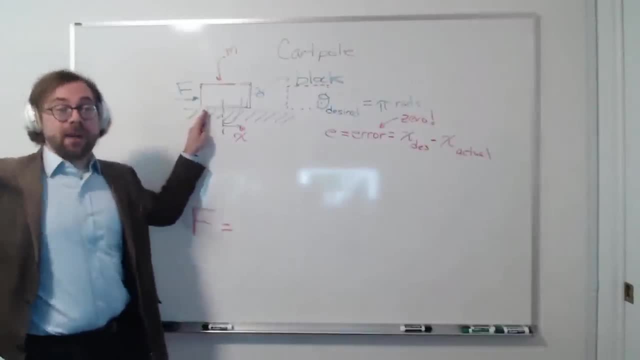 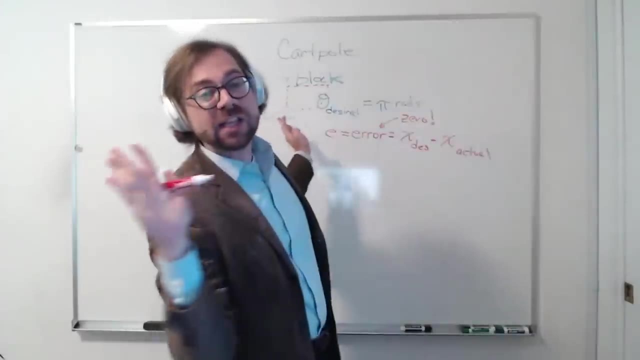 If I'm far away, I'm going to apply a lot of force to book it there. Okay, Once I get closer, closer, closer I release the force. I do less force. So as I get closer, I'm trying less hard. 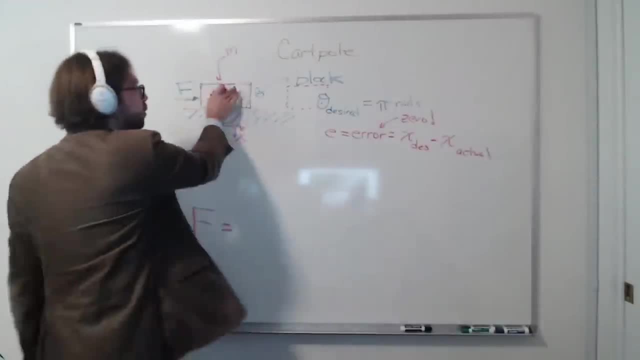 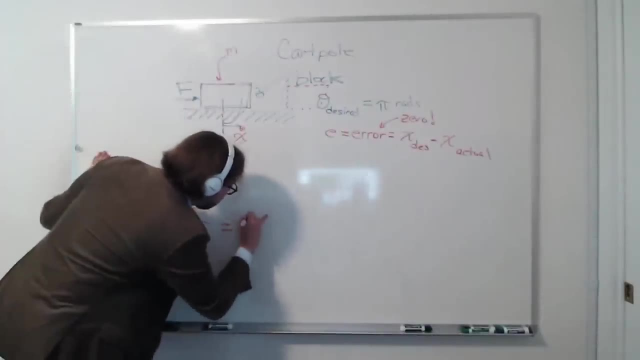 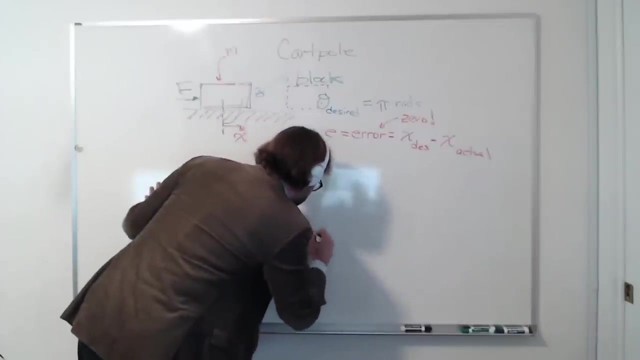 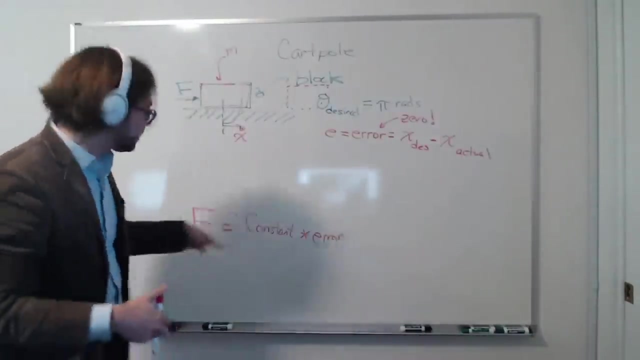 And this, naturally, should drive this block to my desired position. Okay, So I could write that as some constant times your error. Okay, So that constant times that error. if I apply this, if I make this my controller, this equation, 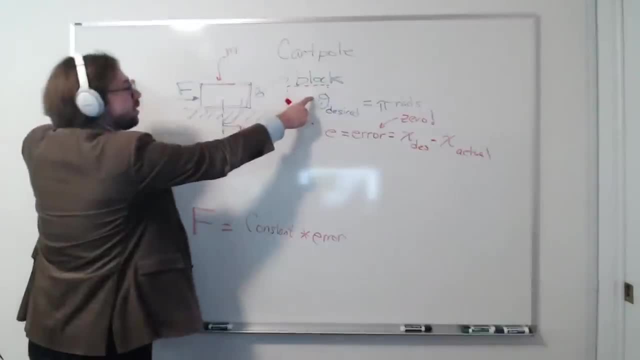 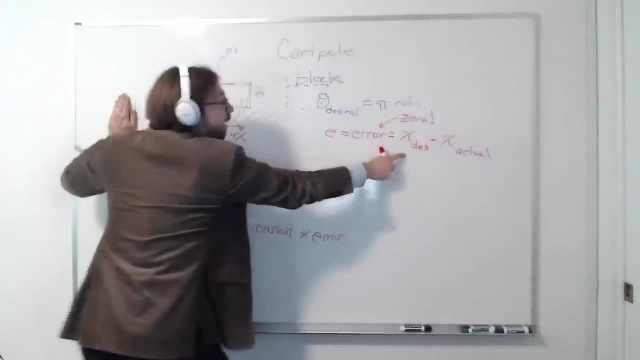 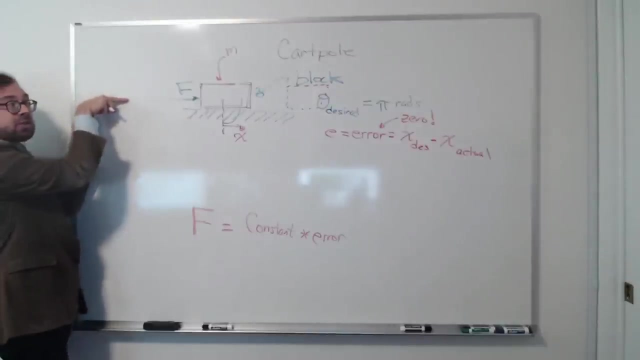 if I start over here, my desired is some large number. My actual is a much smaller number, So desired minus actual is going to be a large positive number. Therefore, I'm going to apply a large positive force and start moving it. 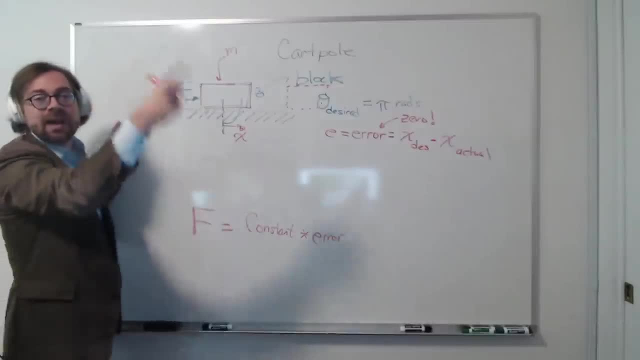 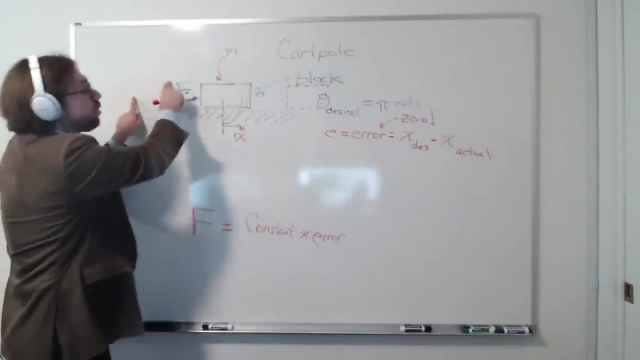 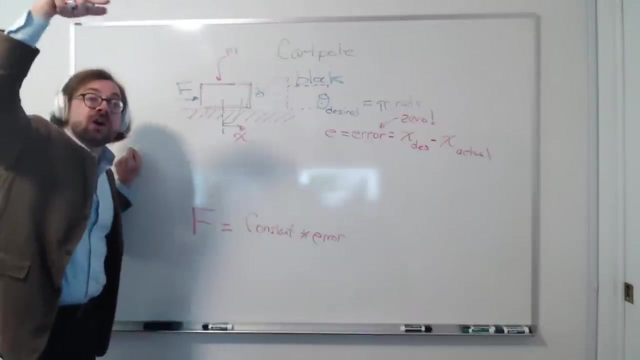 And it starts moving. And then I, every time, every all the time I update what my error is, all a little closer. Now ask yourself, now that I'm a little closer, has my big error gone up or down? Well, it's gone down a little bit. 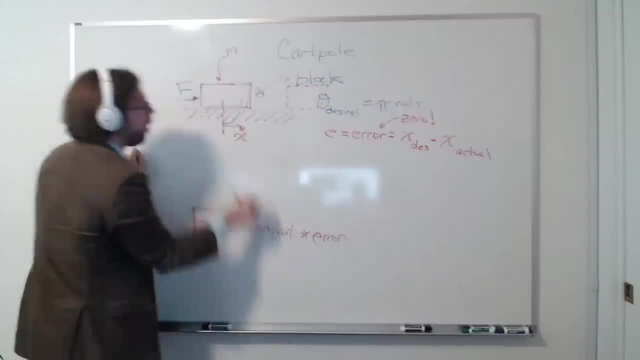 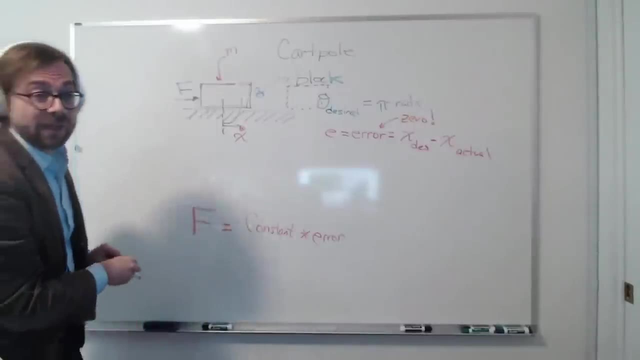 You got a little closer. You're a little closer to your goal. Your error gets smaller. The force you apply gets smaller. You rinse and repeat And you keep running the controller. Just keep running it. Okay, And how is this going to behave? 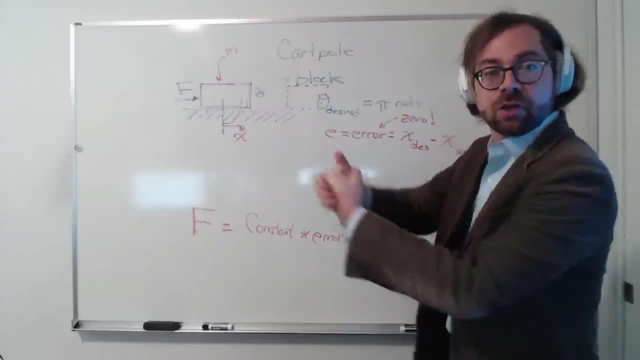 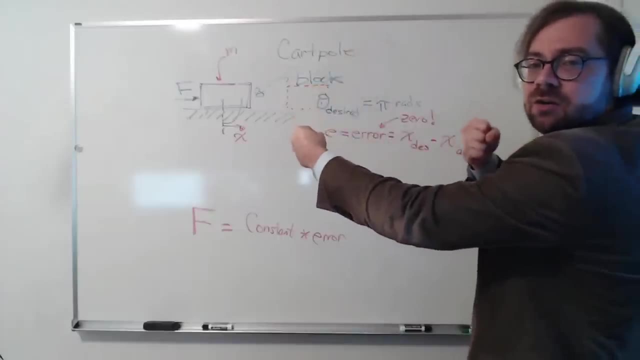 This is going to behave like another device which pushes, pulls on you the further you get away from where you want to go. So let's say: you're here, You want to get here. This is going to change the amount of force you get the more you pull it back. 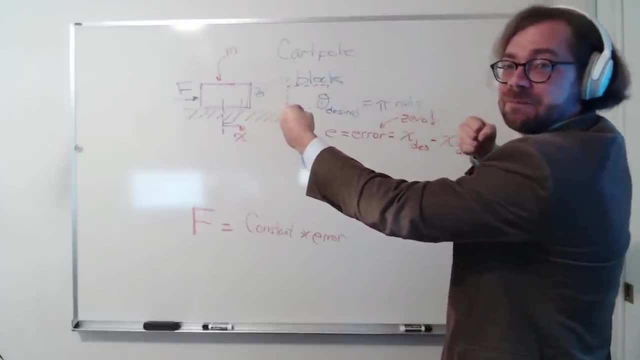 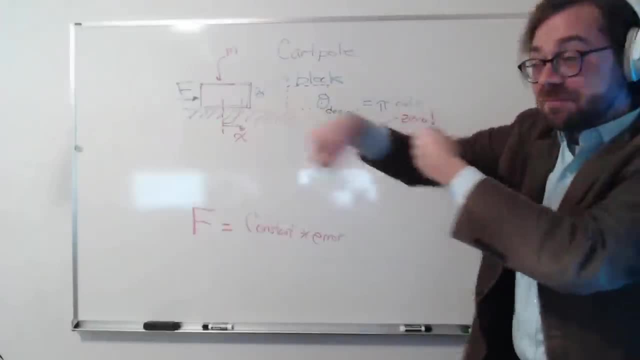 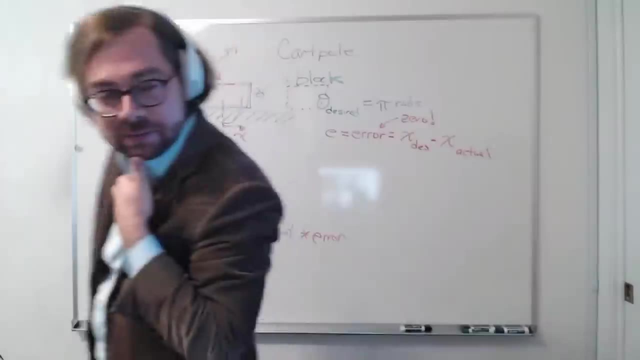 It's going to go. It's going to go, Right. So it's true, It gets us there. I'm not very good about stopping, Okay. So how do we get it? So how do we get it to stop? Well, we don't need. 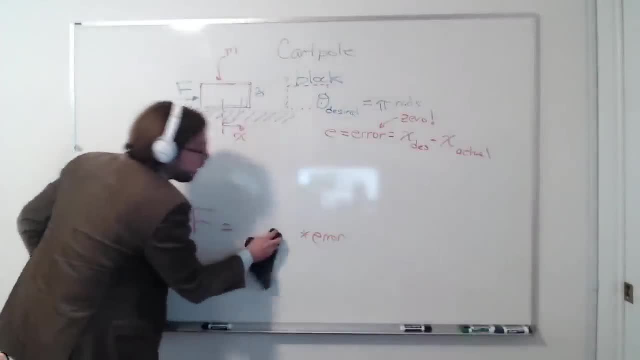 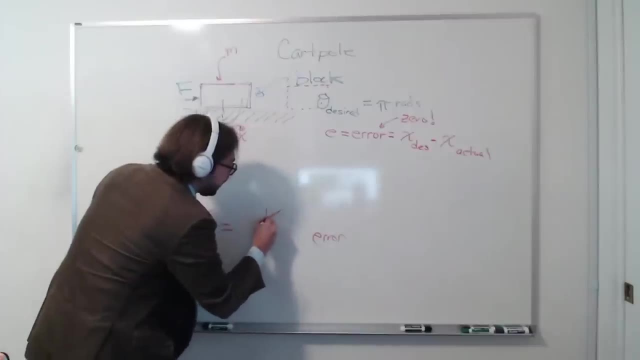 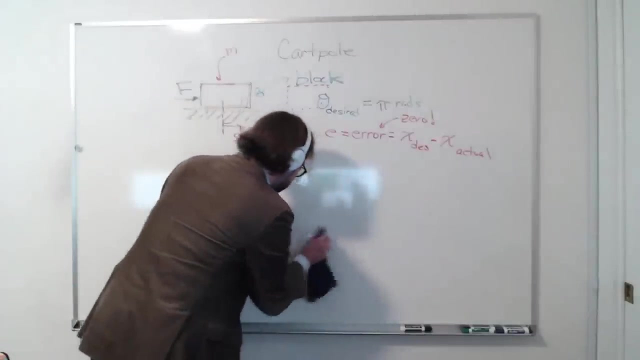 So we need more than just something where you have a constant times your error, which I'm now going to label instead of a constant- Okay, I'm going to call it some constant K, sub P. okay. times your times E, which is your error. 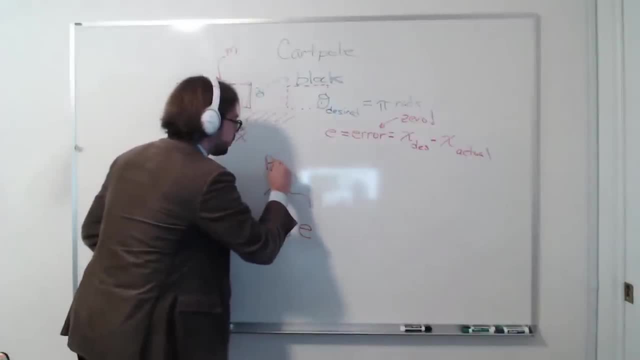 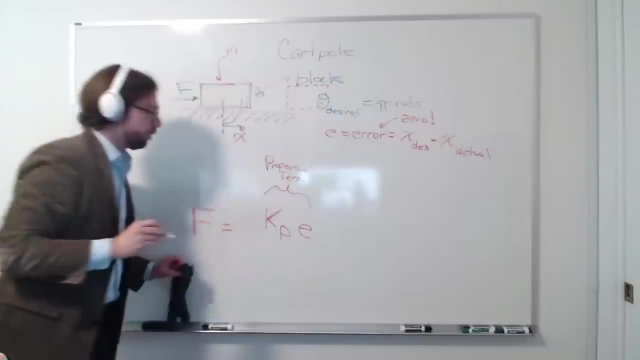 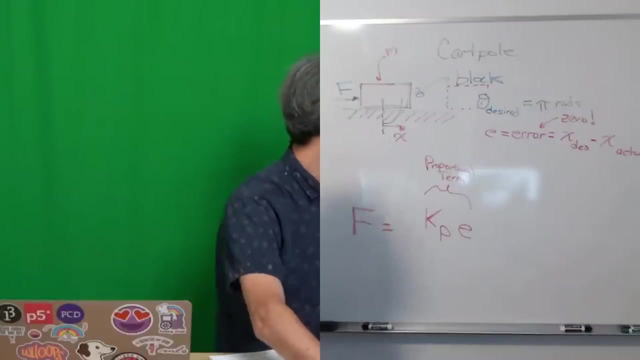 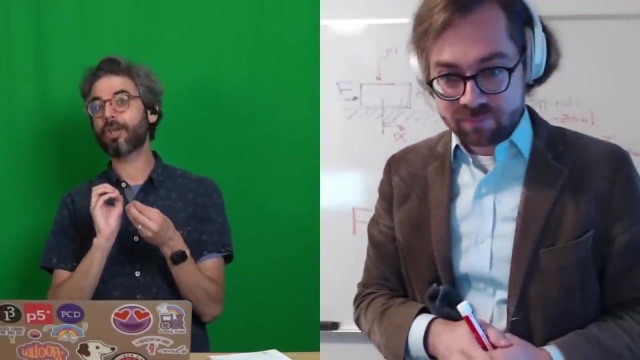 This is our proportional term, So I'm just going to pause you for a second Christian, because a bunch of people in the chat are discussing- And this is the light bulb that went off in my head This week- I guess I can quickly go to this screen here- which is that I have a whole bunch of tutorials about these things called vehicles, which are simulated autonomous agents that steer around a little 2D canvas. 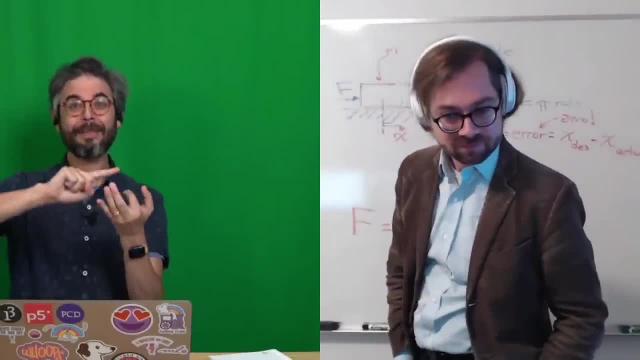 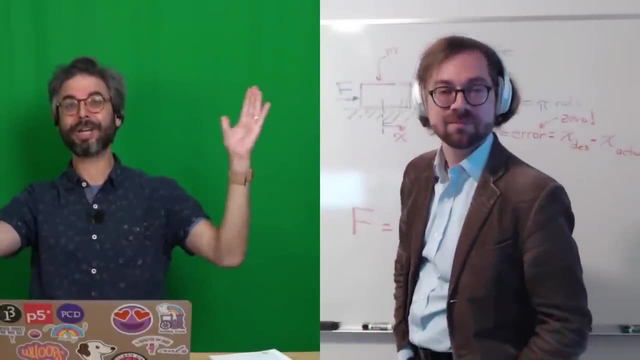 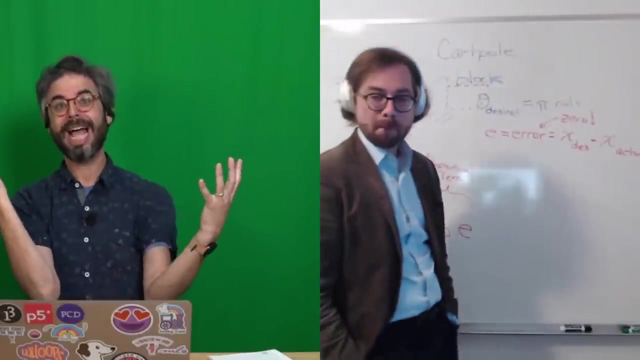 And a bunch of behaviors are things like seek, arrive, path following, And all of those involve this idea of a desired velocity and their current velocity and looking at the error as the difference between the Where, The sort of speed and direction they want to go and where they're currently going, and then applying a steering force in that direction. 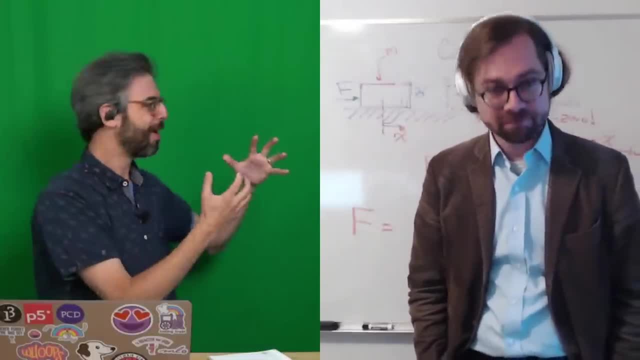 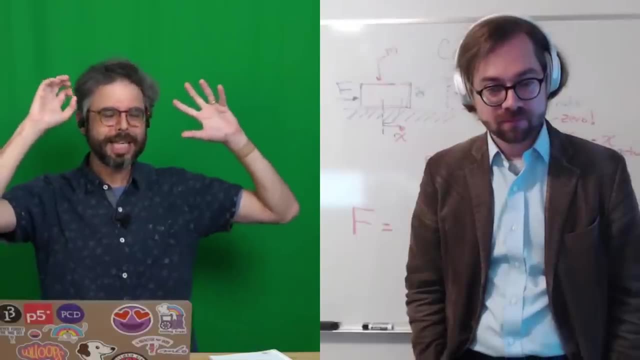 That is exactly the same concept as what Christian is formalizing here in terms of the mathematical equations and applying it to robotics. So this is kind of an amazing thing that happened to me. that made me realize all the ways that I might be able to expand and augment those examples. 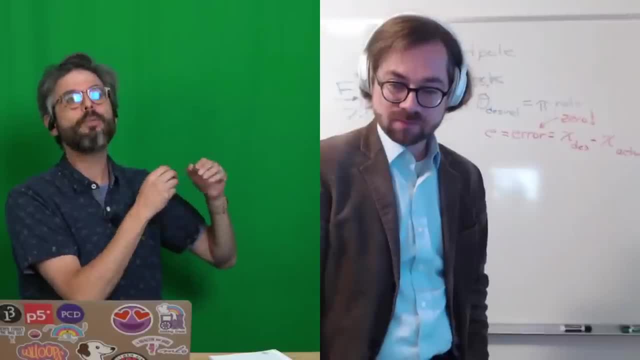 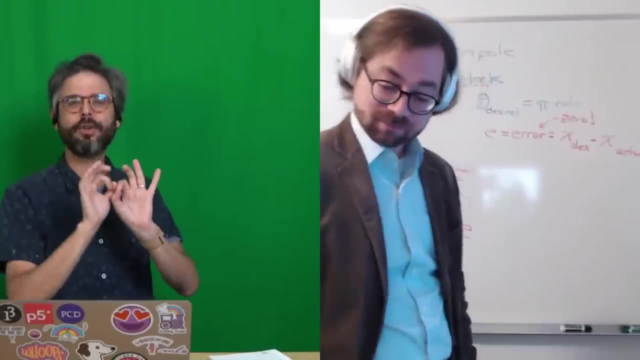 And we're going to get to this. You'll start to see this. But I'm really only scratching the surface by mostly just using this idea of proportion. But I'm really only scratching the surface by mostly just using this idea of proportion. So anyway, I just wanted to make that connection for any of the viewers who have been following the Nature of Code book project and those simulated steering agents. 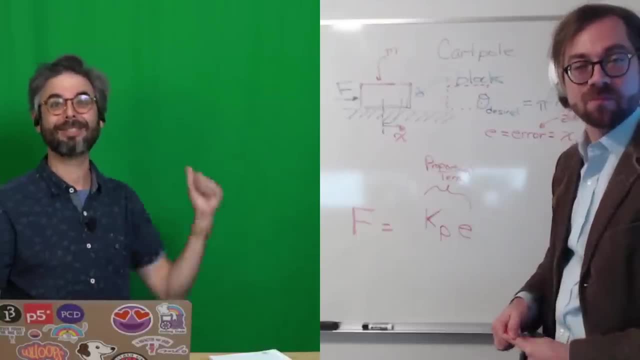 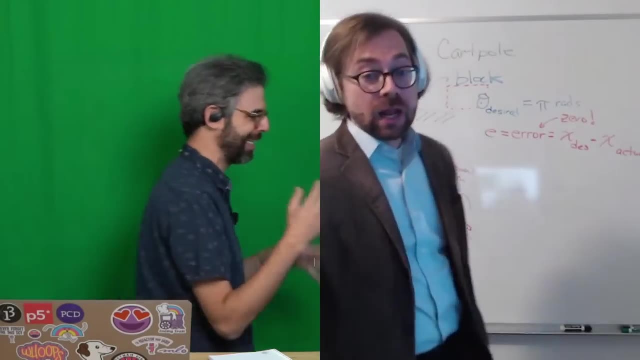 This is like really just sort of peeling back some of the layers of those even further, And we'll see the connections of those more once we bring this code into P5.. Okay, So I just wanted to mention that people were discussing it in the chat. 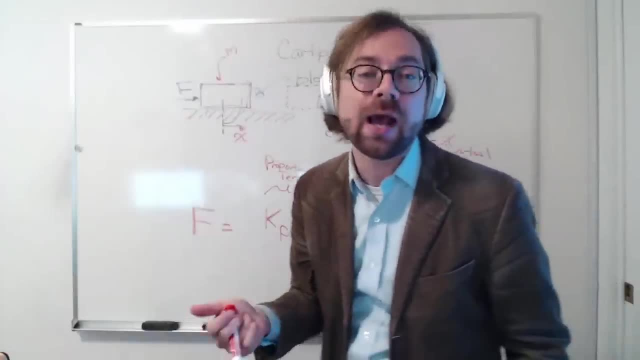 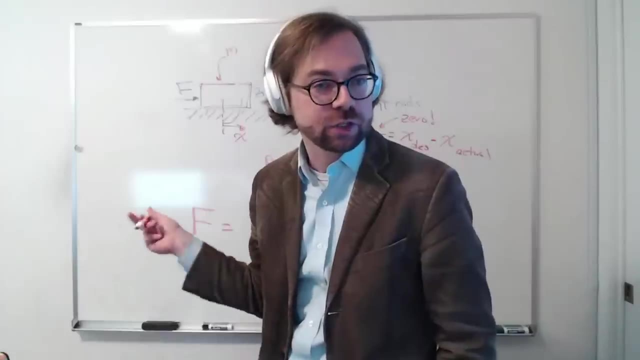 That's awesome. Now, that's exactly the kind of I mean this is kind of a core concept that applies to lots of different fields. I mean, the PID control is well over Absolutely A hundred years, a hundred-ish years old, plus. 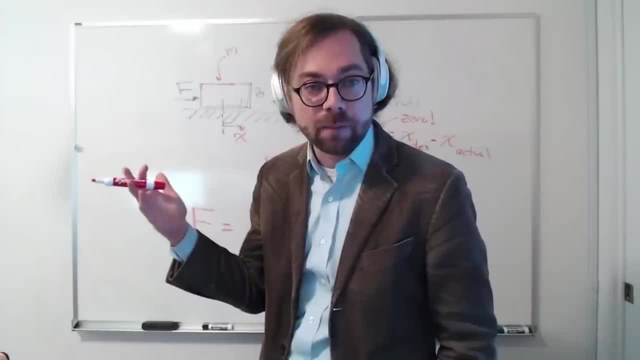 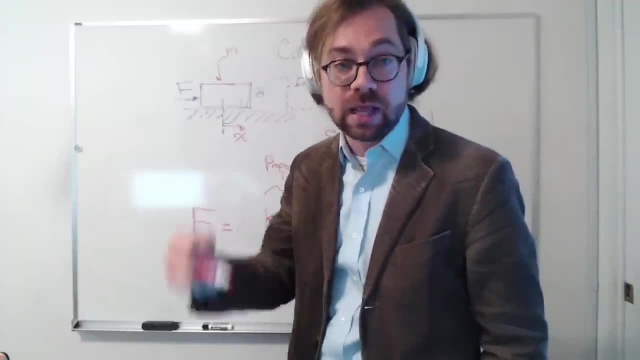 And control theory as a field is. It goes back to especially the 1800s- was a big time for that, And it's so- But these concepts creep into lots of different things. It's really intuitive, right? And let me just break this down a little bit here. 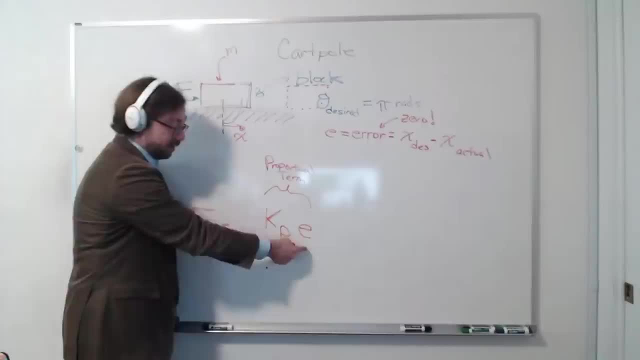 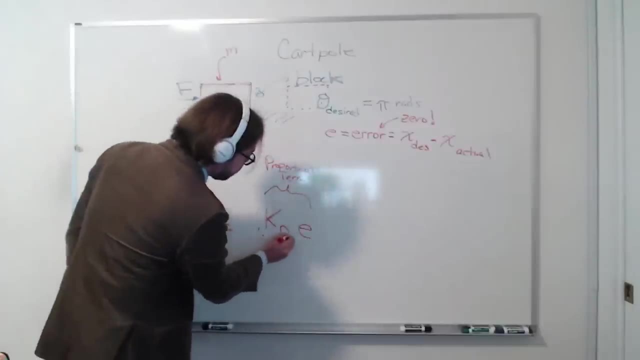 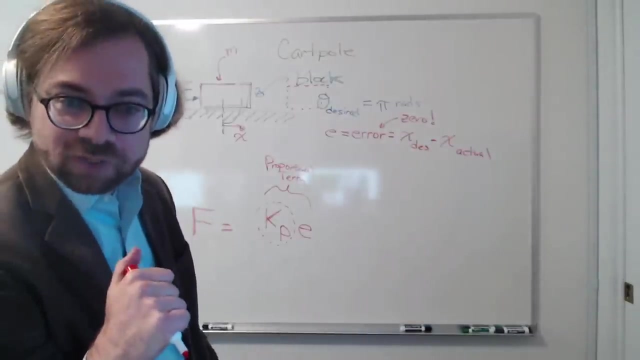 We call this a proportional term because the amount of force you apply is proportional to your error right. And how much is it proportional by? Well, we have this constant right. Who gets to choose that constant? We do. We're the control designers today. 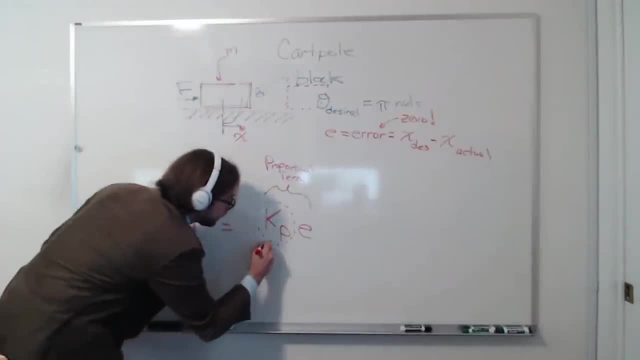 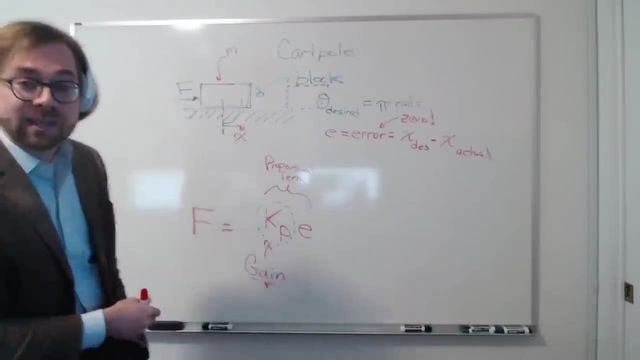 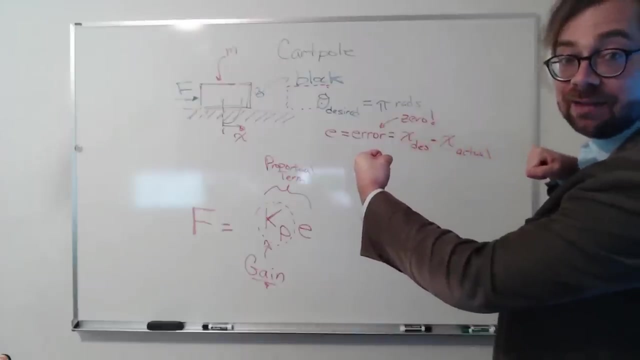 Okay, And this constant has a name. It's called a gain G-A-I-N. Okay, And we get to choose what that is. And in this analogy of the spring, us choosing that gain, if it's really high, that's like a really stiff spring. 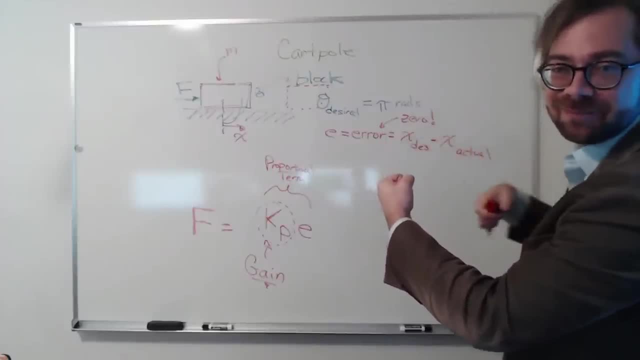 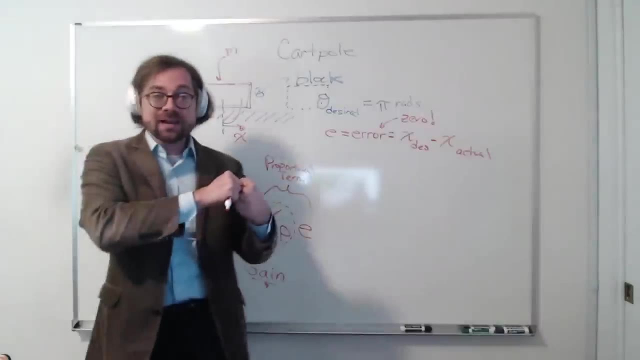 If it's really low, it's a very soft spring, Okay. So that's what that term is, Okay. But like I said, in a lot of systems you know you put a spring in there, it's going to start vibrating right. 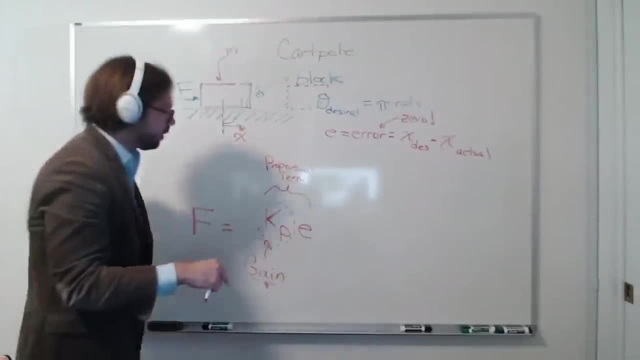 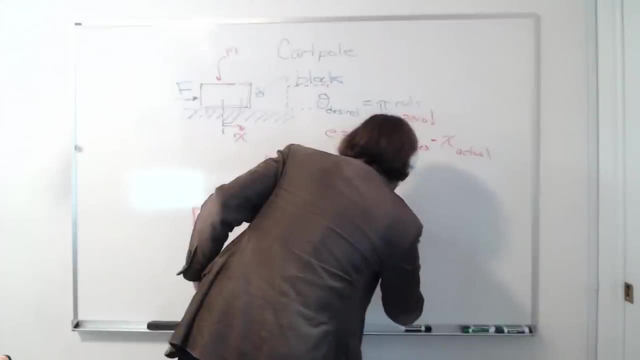 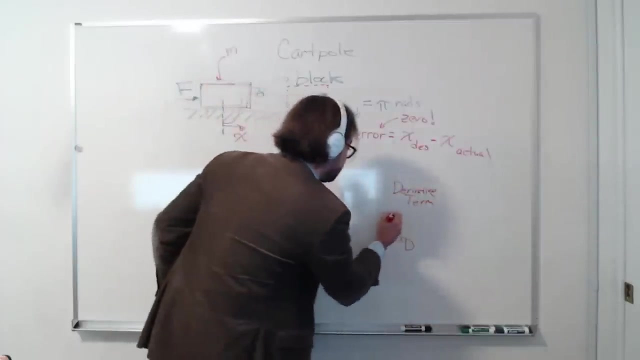 And we don't want this to vibrate, We want it to come to a stop. So we need to add another term, Okay, And call the derivative term, And it's going to be K-D, which is another kind of, which is another gain, that who gets to choose it. 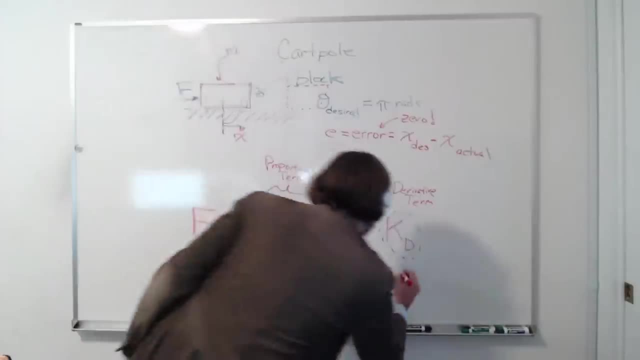 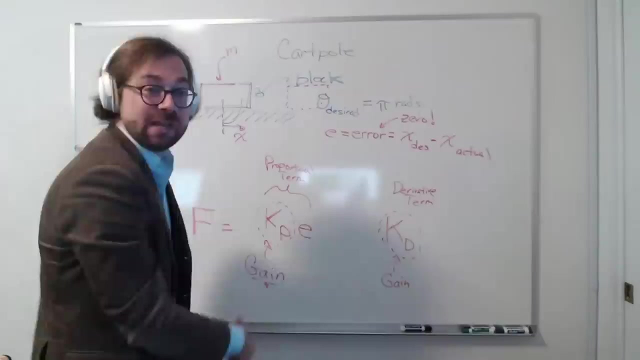 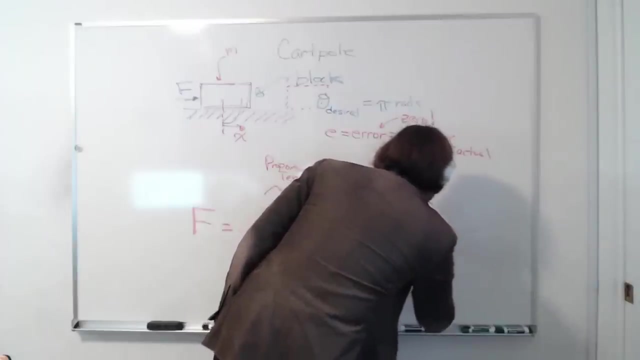 We do. We get to choose it as the control designer. This is another gain. These can be different and almost always will be different. We get to choose Right Times, the derivative Of E with respect to time. Now I know I just jumped into derivatives which are calculus. 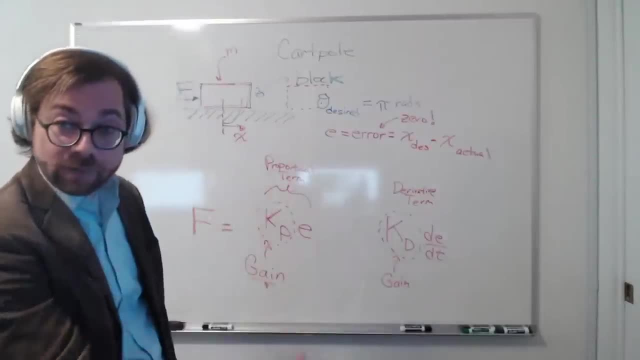 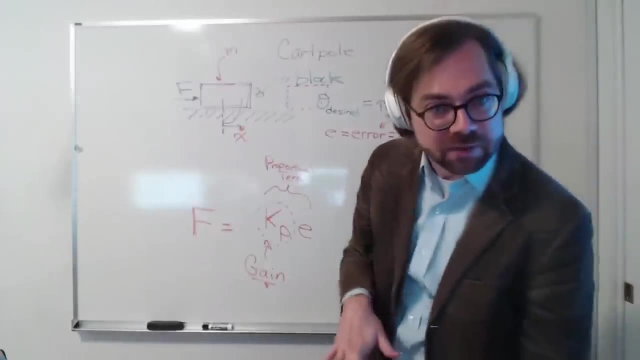 Not, I don't want to scare anyone who hasn't seen calculus or bored anyone who has already. Okay, But all the derivative is in calculus. If you ever had to explain and sound smart to someone who's never heard of calculus before, that calculus is about change. 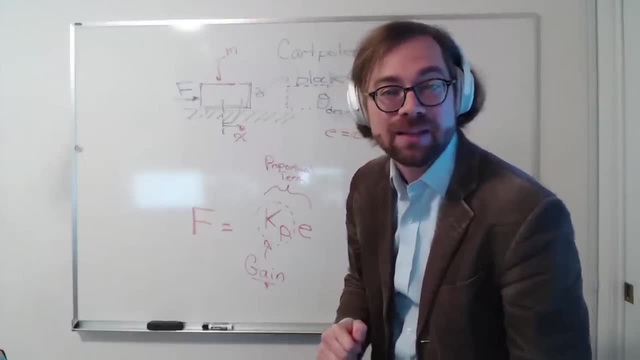 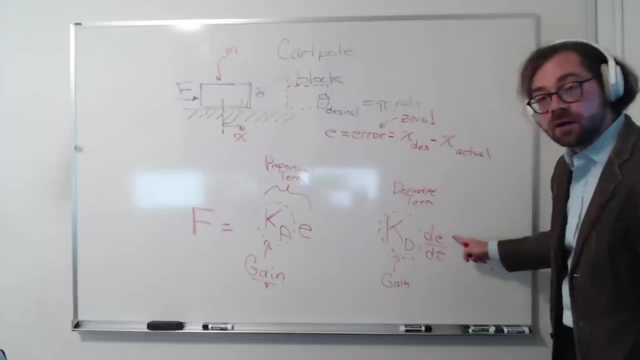 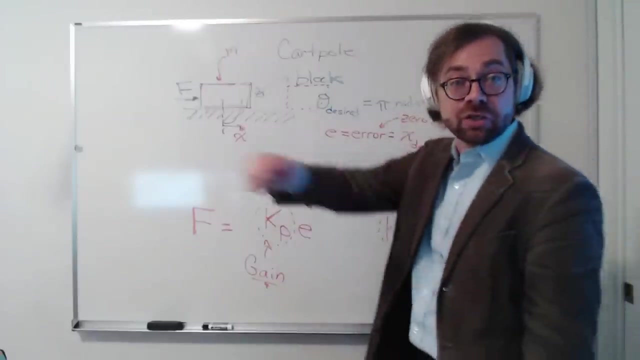 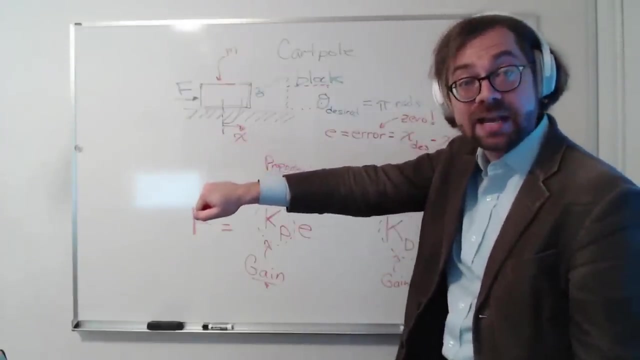 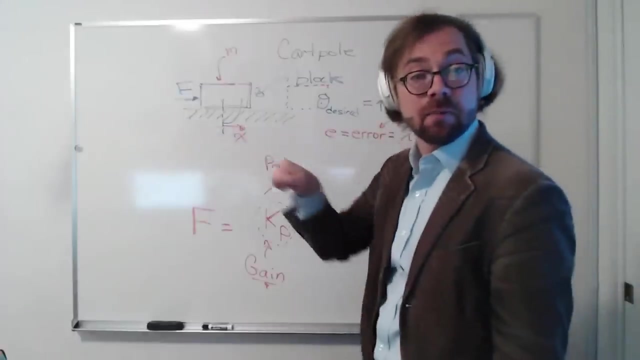 Okay, It's basically the mathematics of change, And so this is a. the derivative is described. It's describing how much your error is changing over time class. The thing we classically say is that a position that's changing over time. If I see, if I want to see how much it's changing over time, I take the derivative with respect to with respect to time, and it gives me my velocity. 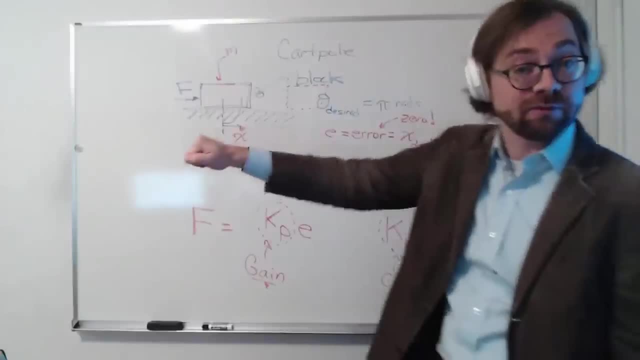 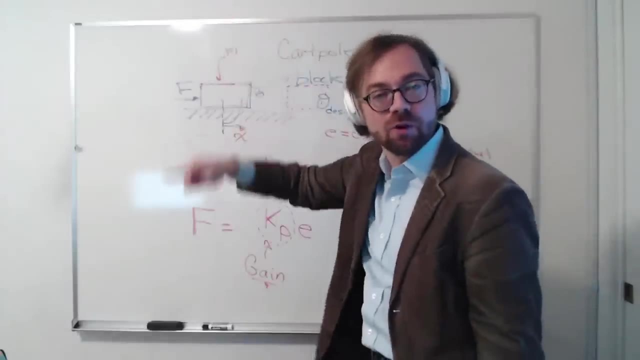 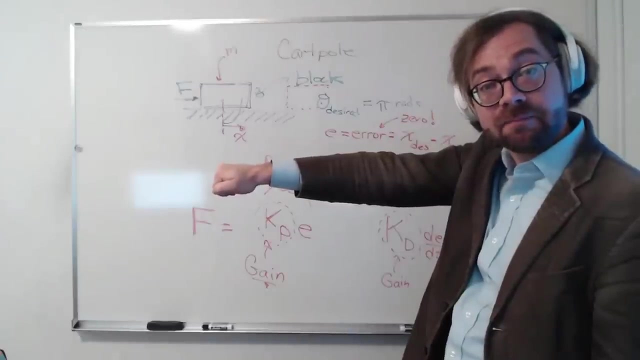 So here I'm moving around. I, if I took the derivative of my Signal here, of me moving back and forth, you would have this velocity going up and down. Always moving is coming to a stop. If I held my arm out constant, took my derivative with respect to time, something that's not changing. 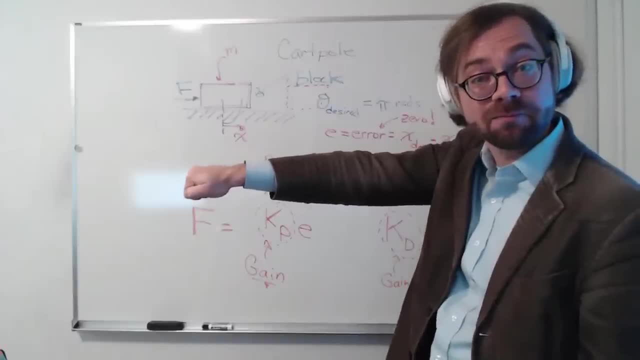 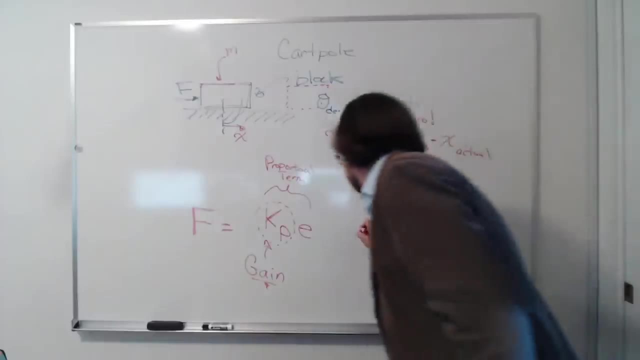 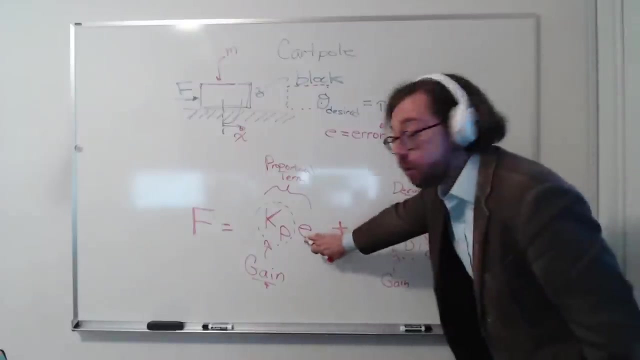 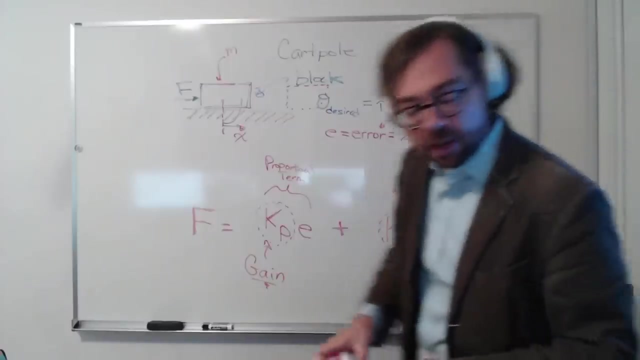 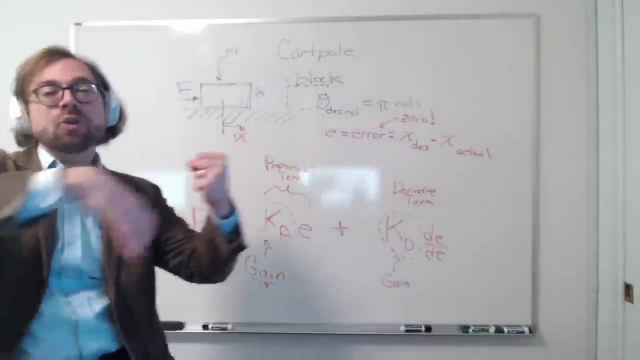 And you're asking how much it's changing. The answer is zero. So this is basically saying that we're going to add a term That's not just looking at how far away we are from where we want to get, but how much that error is changing. now, to give you a little intuition as to how that works, we just talked about a spring, how the proportional terms, like a spring you pull back, that spring wants to go. it's going to try to drive you to where you want to go. 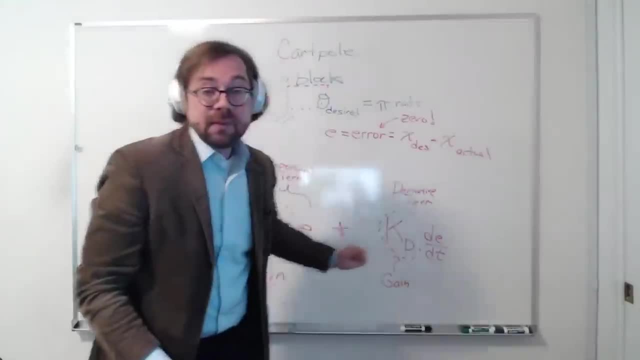 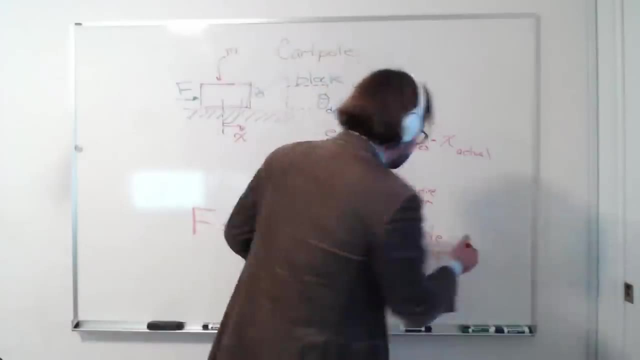 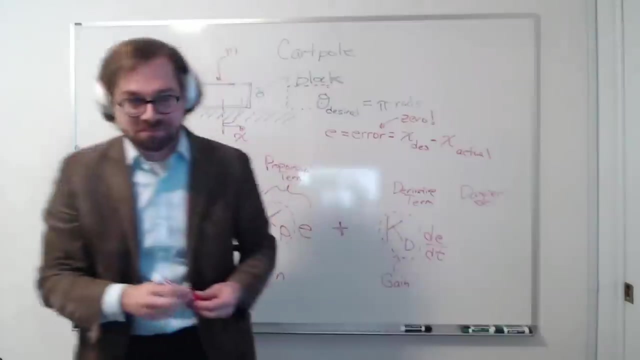 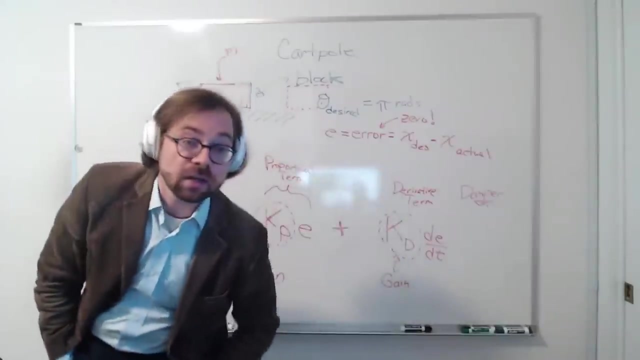 Okay, The derivative term is something like a damper. Now, not everyone has heard of damper, Most people have heard of springs, but dampers are very important mechanical systems. My PhD is in mechanical engineering as well, So I'll wax philosophic and philosophical here. but, like you know, in a car, in a car, if you were driving around you know, and every time you hit a pothole, your whole car goes and it starts bouncing around. 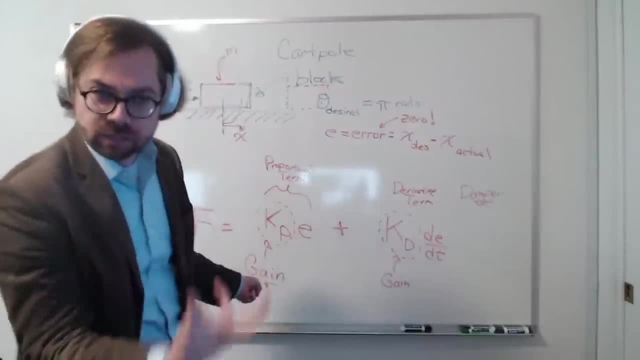 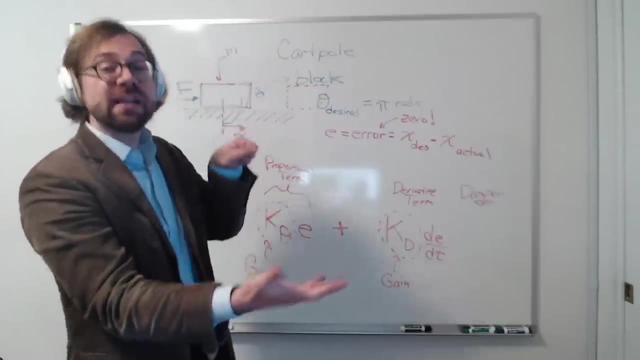 It's bouncing around because there's a spring in your car called the spring, The suspension, but not just a spring. there's something in your car that also makes the. that's that stops this, this, uh the the bouncing, otherwise you'd bounce forever. 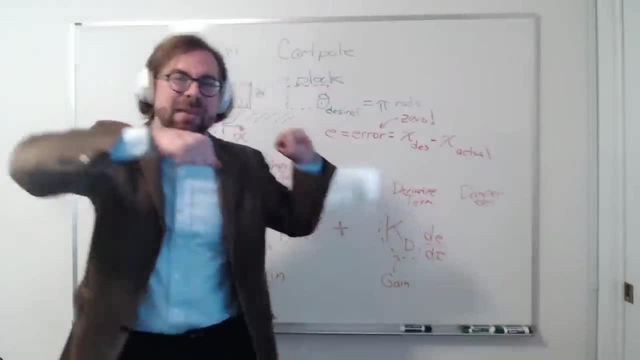 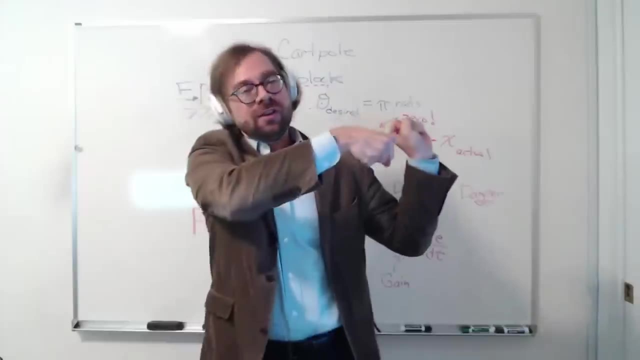 Okay, And that's called a damper, And normally what it is is is a piston. Okay, It's a piston that when you push on it, there's a little fluid that you push through and it resists your motion. Okay, 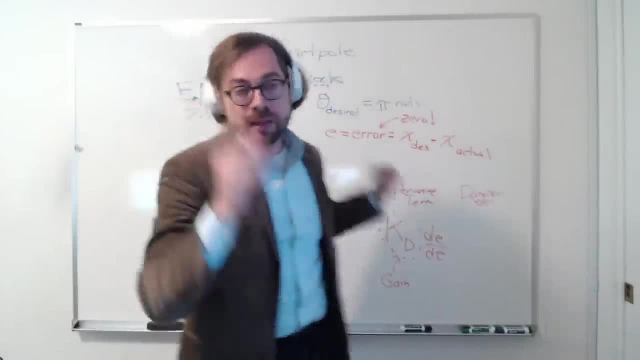 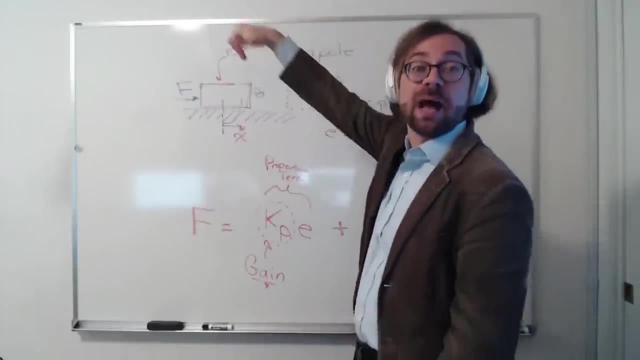 And you might see these in your everyday life when you walk around in a building. if you've ever seen a door, Okay That. if you were to try to slam it shut, all there's like a little mechanism in the door that might try to stop it. 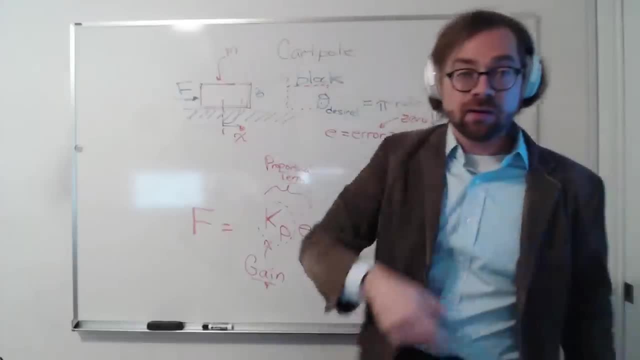 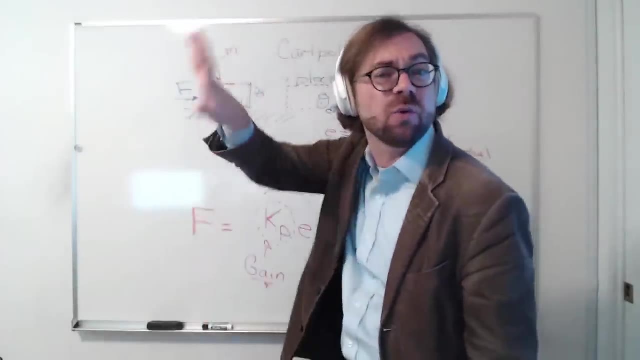 It's up up by the hinge. you know that slows it down, That's a damper And you can even hear the air whistling through it, sometimes right Where the air is the fluid that brings it to a stop. 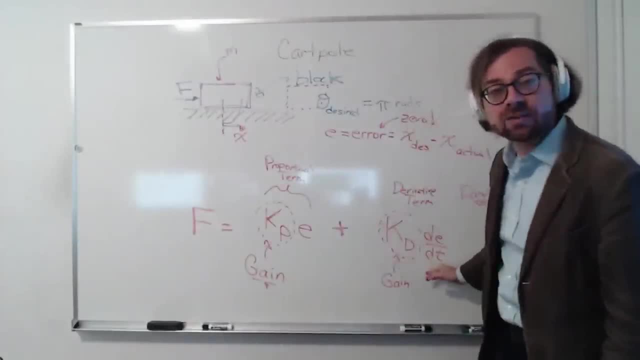 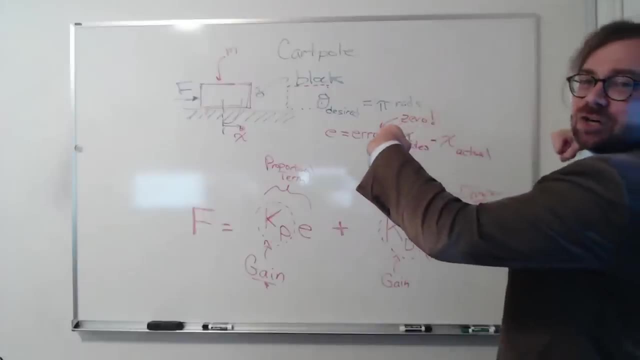 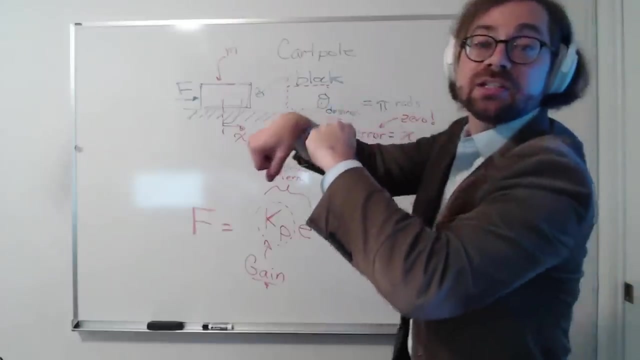 Okay, So the D term acts like this damper which gets rid of oscillations. So where we once before had this P term, That's going to go. if we add this D term, it's going to slow it down So it doesn't oscillate as much or at all, potentially. 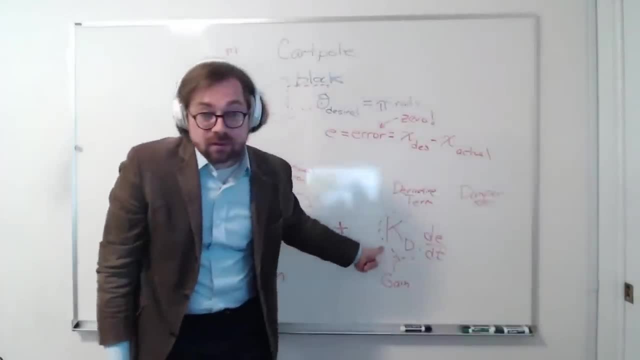 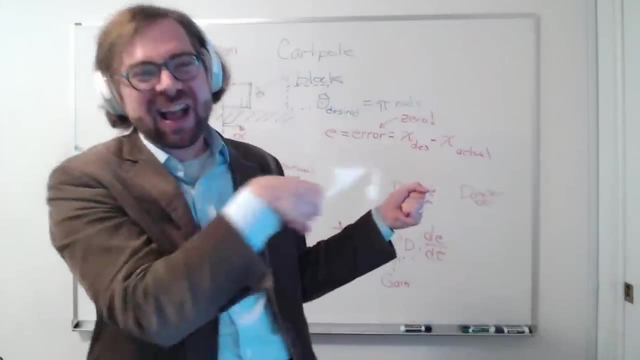 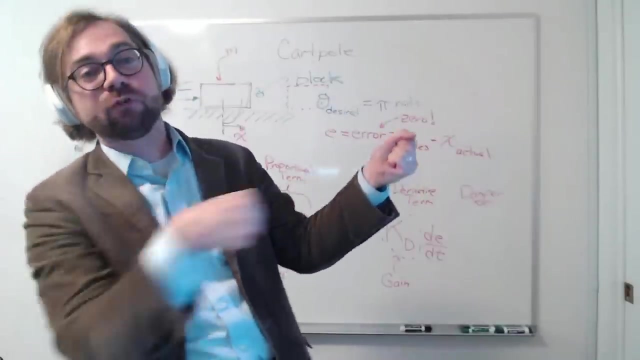 Okay, And how big that D term is. this gain is kind of how goopy our damper is, how much it's going to stop us. If it's very little, it's like pushing through air, not much, you know. if it's, if it's really big, it's like pushing through molasses. 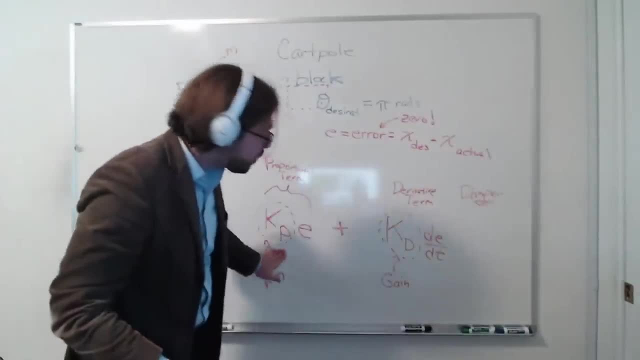 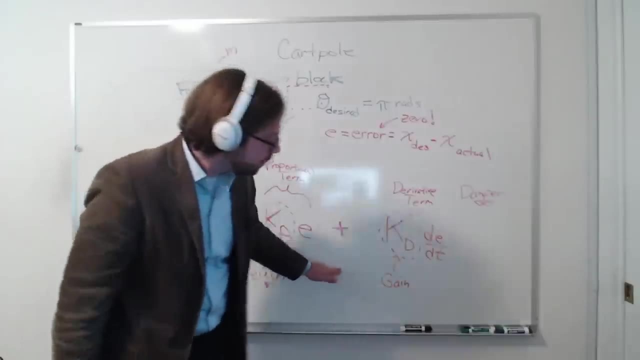 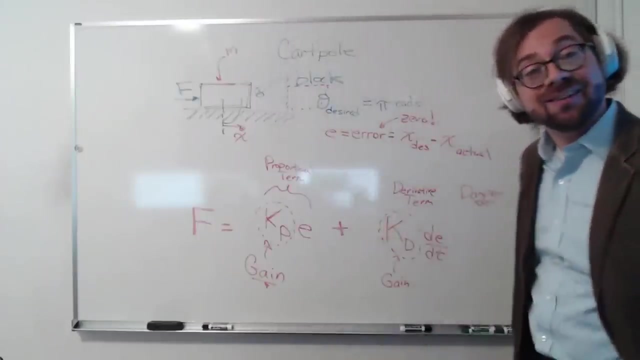 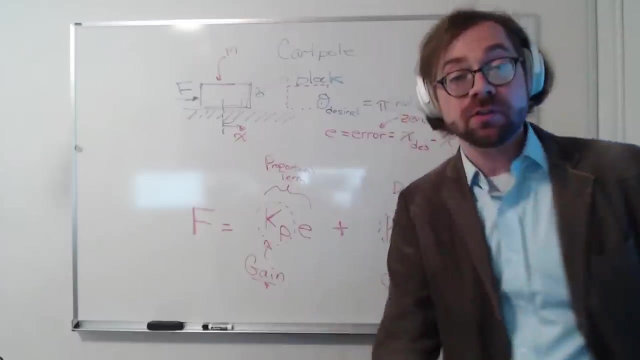 Okay, Those are. so that's a P and a D term and we just add them. Okay, Now, sometimes in control, this will get us a lot of the way to where we want to go. I mean the the blue robot I was showing before the tennis shoes. we use PD controllers on all of the joints of the robot. 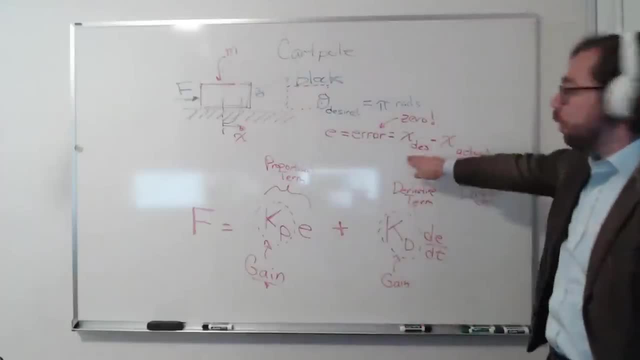 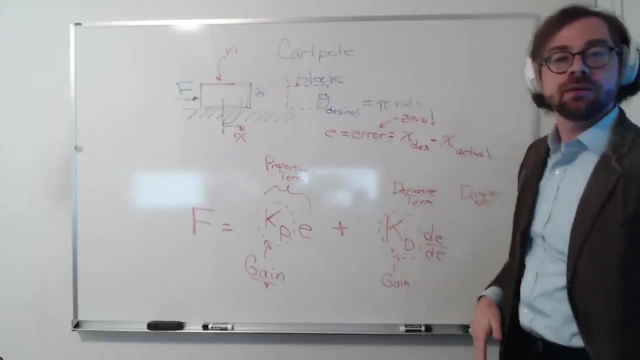 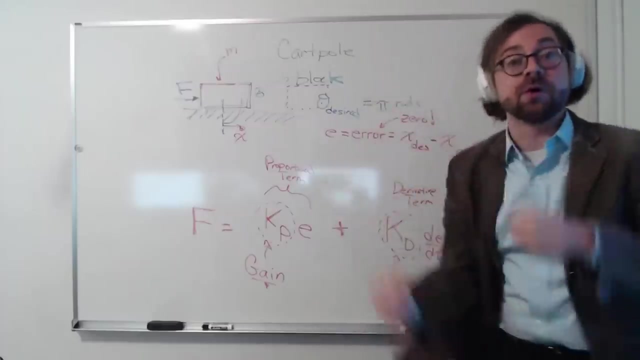 We had a fancy algorithm that would tell us That, oh, what our, what our desired angles are of all of our motors? This algorithm would tell us: oh, we want to make this motion, but onboard the robot, a PD controller, was making the motors drive the joints through those motions. 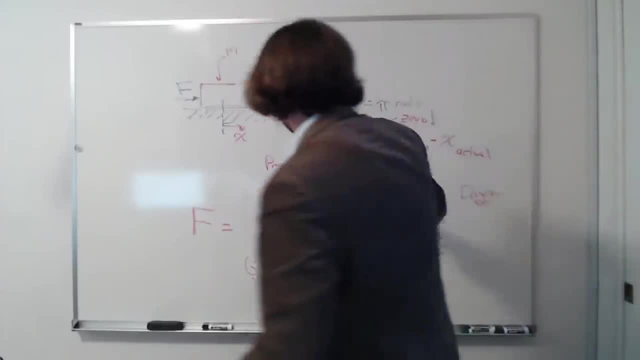 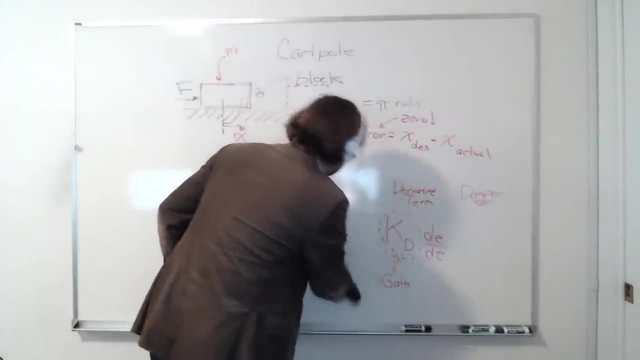 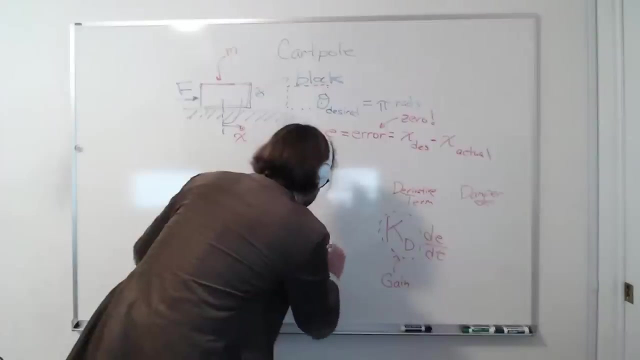 That's how it works. So often a P D control was enough, but sometimes you want another term. Okay, And it's called the integral term. So it's going to be K I integral from zero to T. E of tau, D tau. 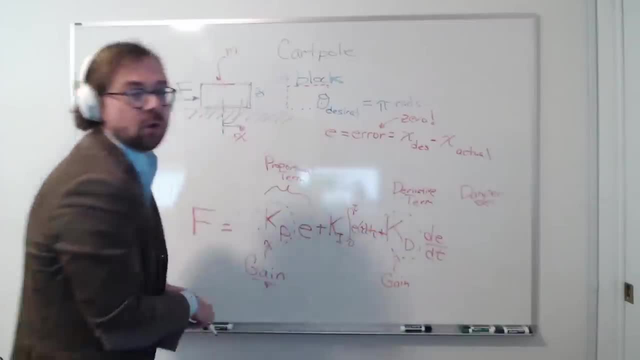 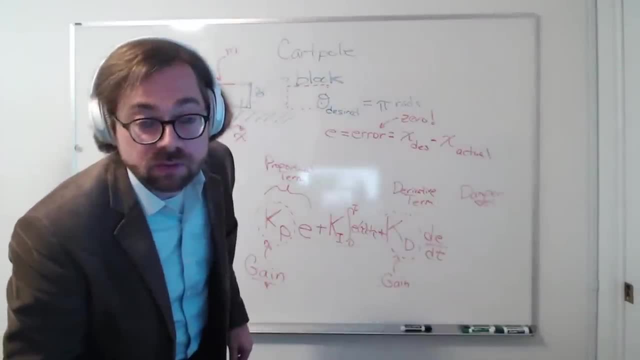 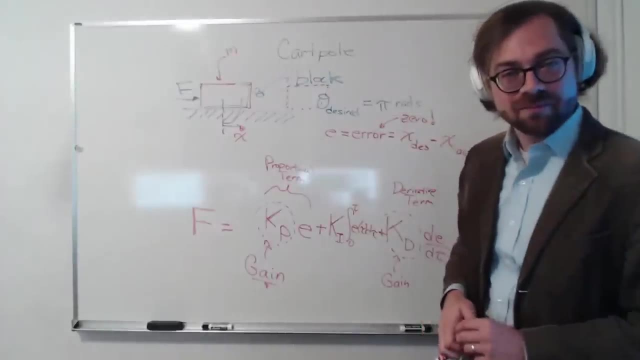 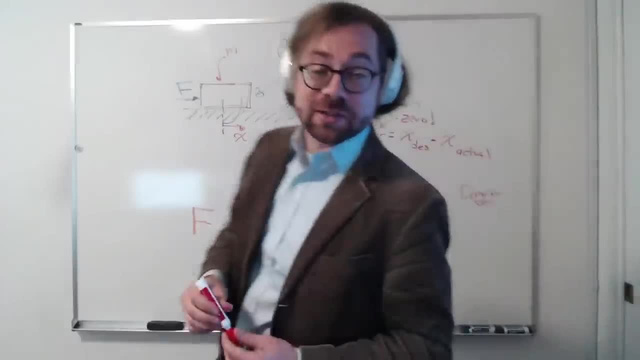 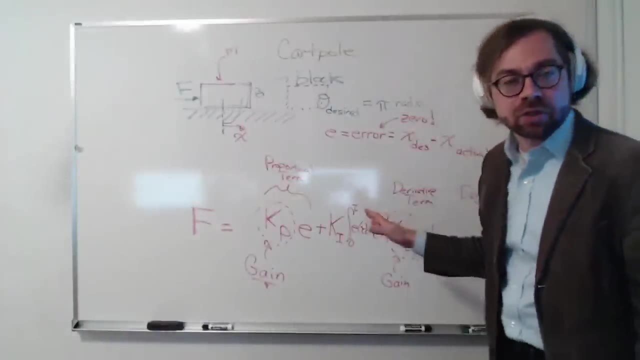 State, Okay, State, I don't like putting Un toppling B like a box to me over all of my non internal long summer. Right, Okay, We need it to be stitch it. stitch it to first, because it's better pain. 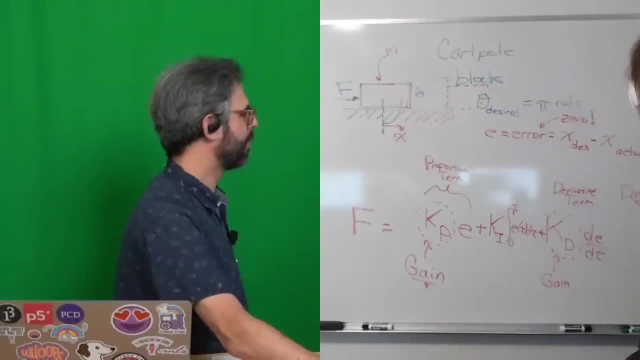 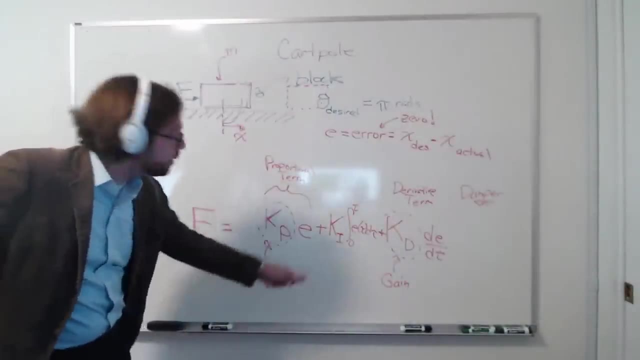 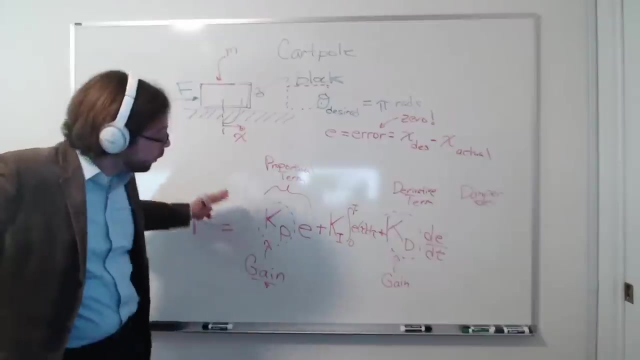 Right, Because That's without. That's what I'm talking about. but no one says PID, People call it PID, People call it PID. But honestly, the I term is the one term I use the least in my work, but it can be really helpful. So the P term gets you to where. 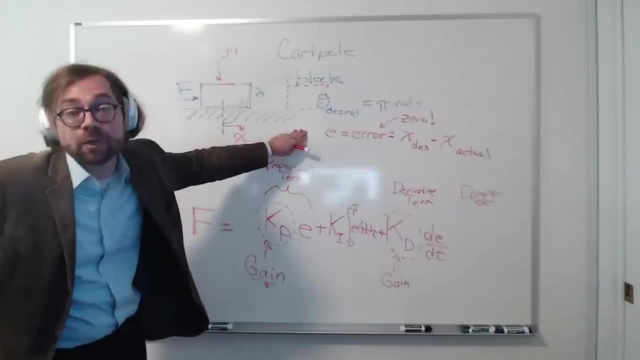 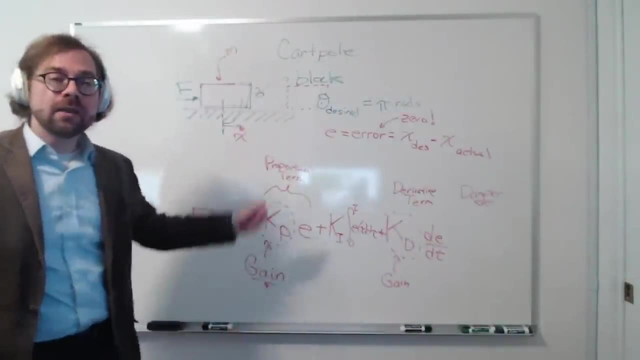 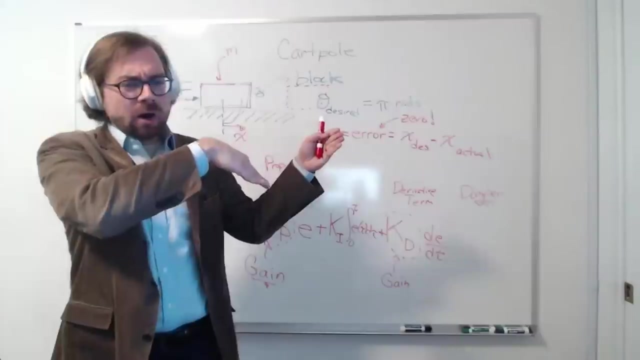 you want to go, or at least it gets you there pretty quickly, probably pretty close there. The D term slows you down The I term: it's useful when you've run your controller, but you are not all the way there. Here's an example. Imagine that this block we're trying. 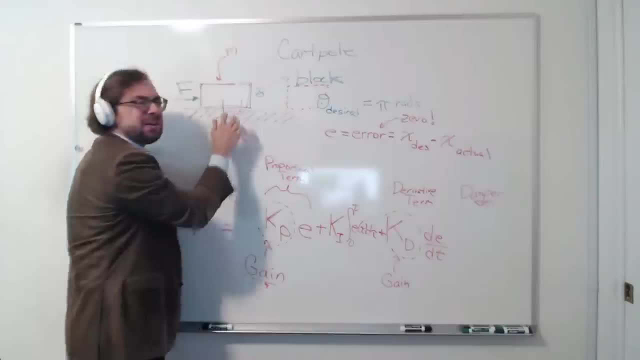 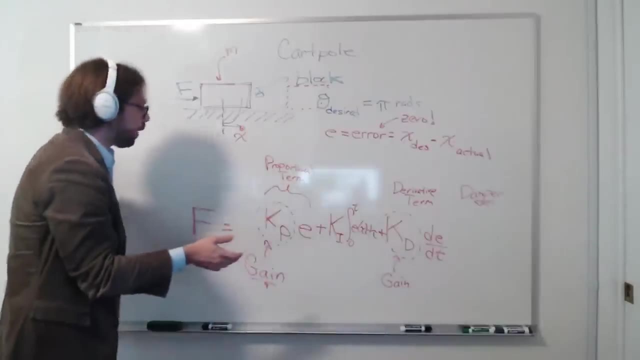 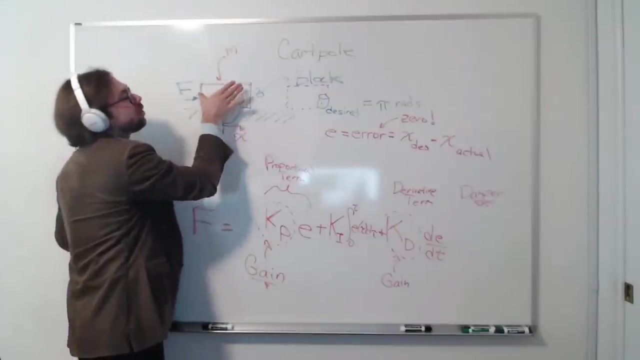 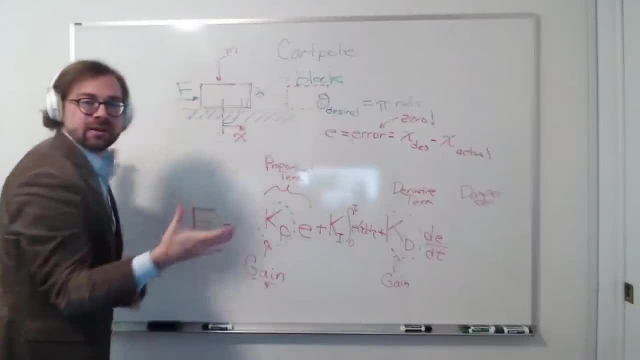 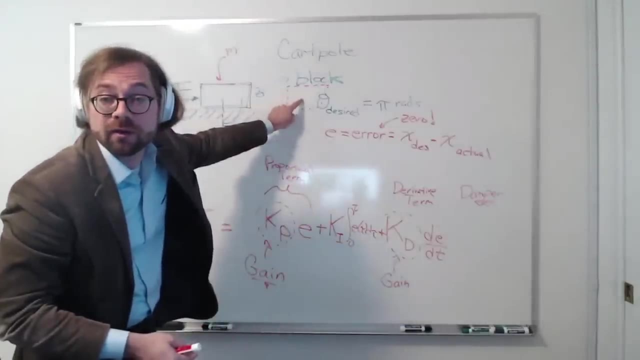 smaller. At some point the force will be small enough that the friction with the ground will stop you before you want to get there, before you're all the way there, And it'll just sit there. It's not going to do anything, It's just like: well, you know. 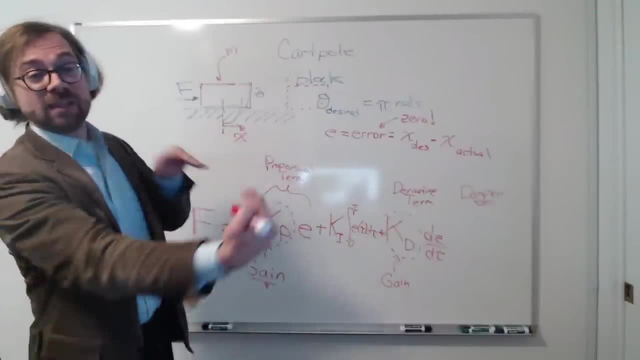 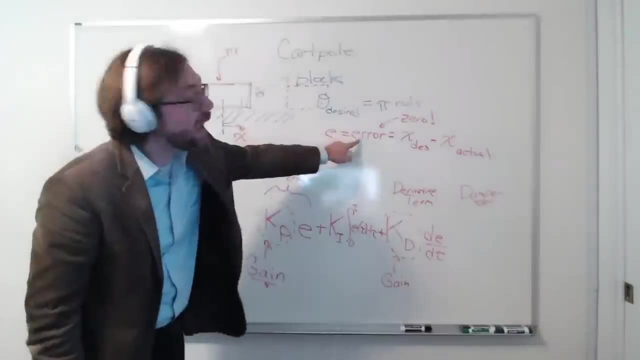 I say I'm going to apply this much force and then the friction is going to fight me and I'm just going to hang out there and just forever And we call that- and that means we'll have an error, that isn't zero, forever. We call that a steady state error. 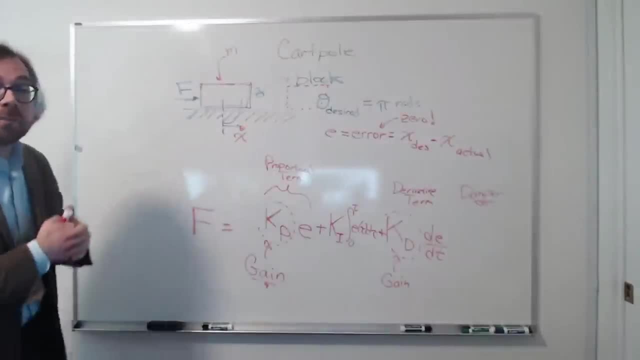 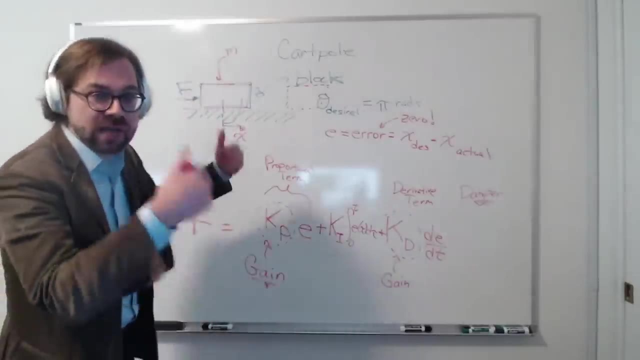 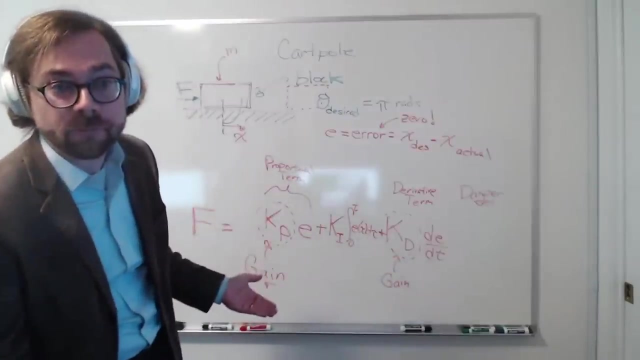 okay, in controls, All right. And one of the most common ways to get rid of steady state error is this integral term okay. And for those who have not done calculus, an integral it's just really adding up the past to get the future, okay. So if you are, and here we are, 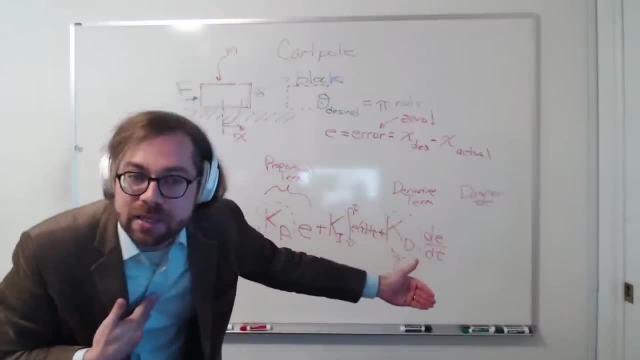 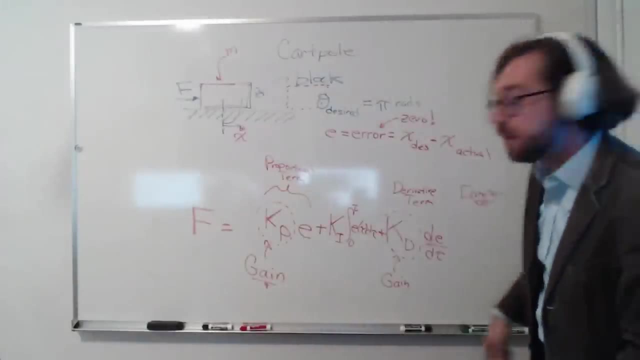 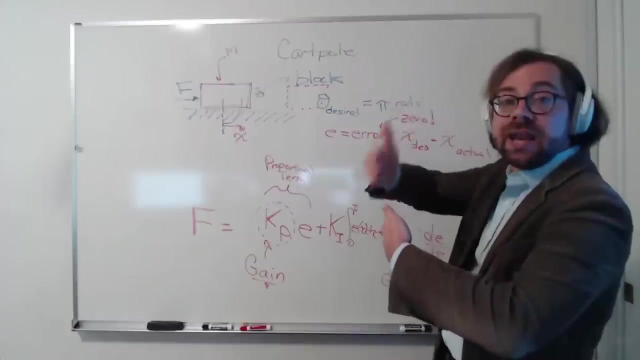 it's hard to see because my equation spacing is terrible. This is why I wish that they did PDI control, because then when I do this lecture I can do the I at the end, the point of space. But it is doing the integral of the error, meaning it's adding up all of the error from the past. 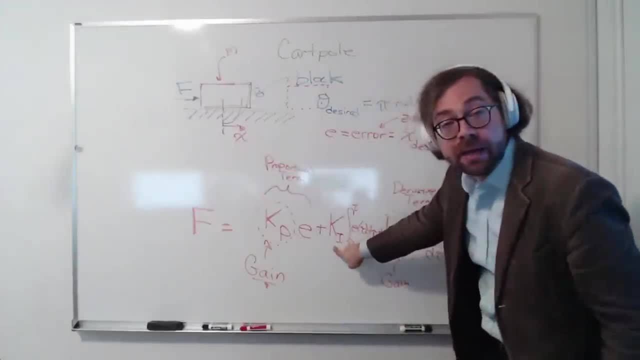 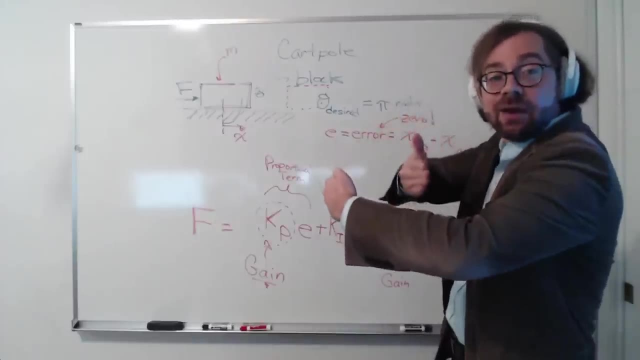 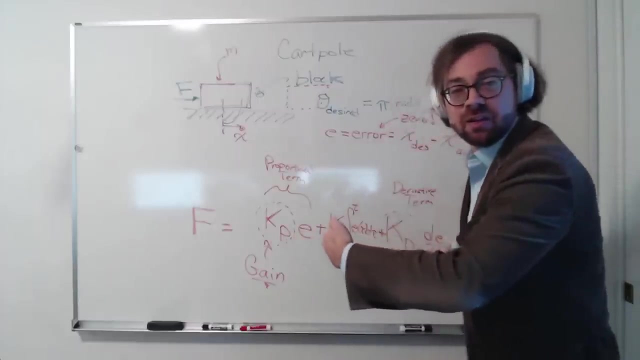 and then multiplying, Multiplying it by another gain called KI. So if you are sitting with this steady state error for a long time, okay, all these other controllers- they're chilling out, doing nothing new, But this I controller is saying there's an error. I'm going to keep adding that up. 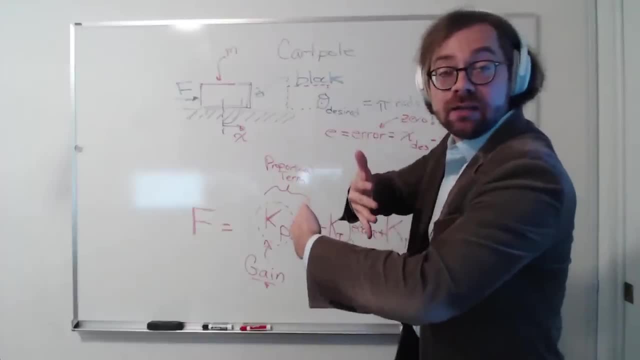 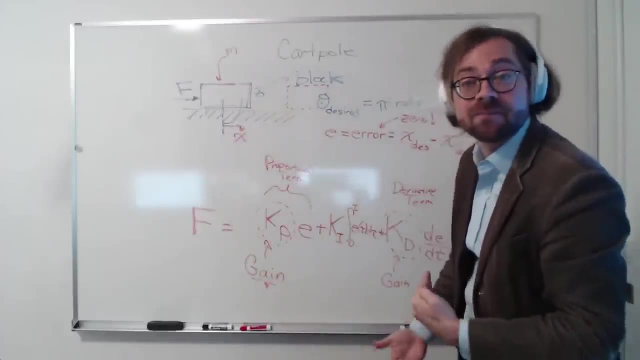 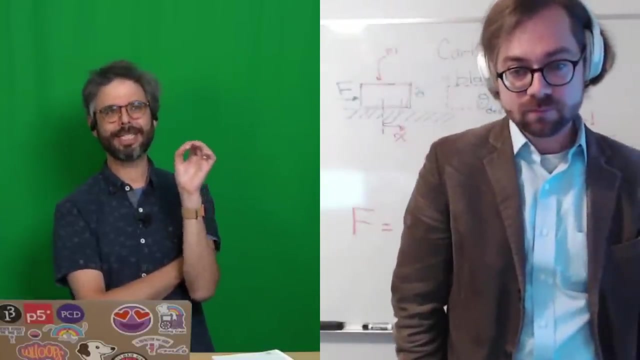 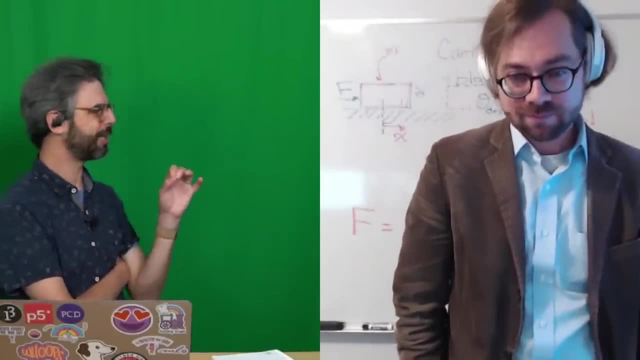 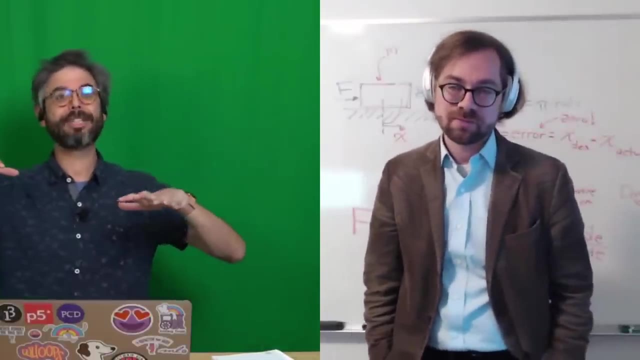 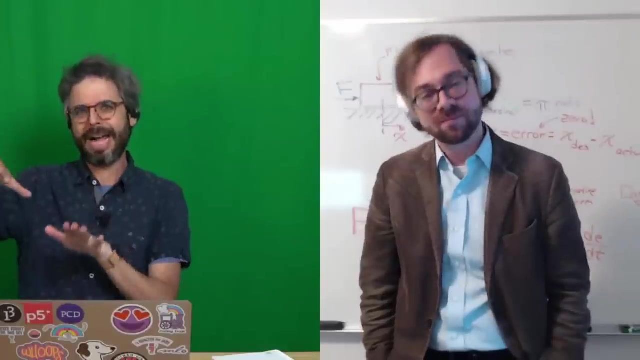 used heavily in a lot of tutorials and projects is this flocking simulation where birds are attempting to. well, these pseudo birds called boids are attempting to match various. match their neighbors in certain ways, like: stay together but don't get too close. match their. 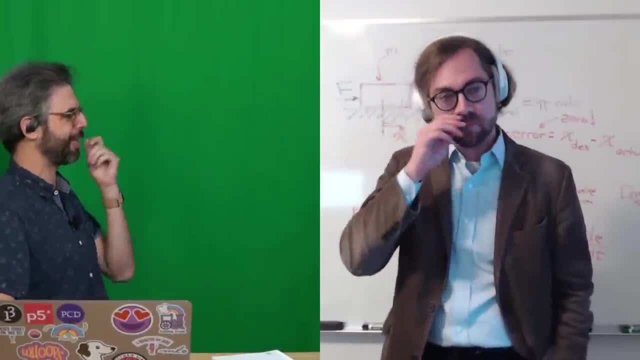 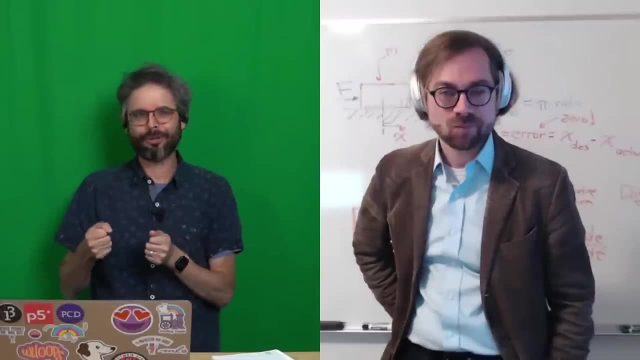 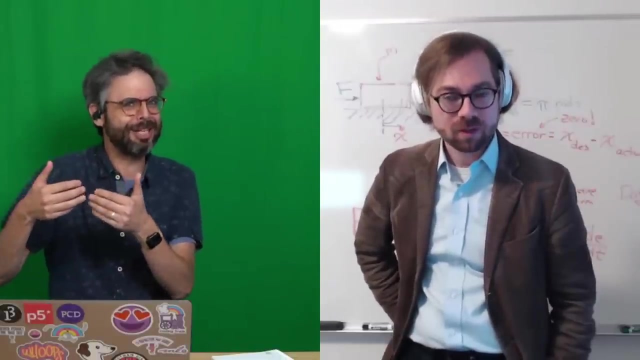 velocity, And I think I was watching one of the PID videos that you sent me and I was, like an explanation, had this example of if you're driving a car and you want to drive at the exact same velocity right next to your friend's car, if you don't have the integration, you might always 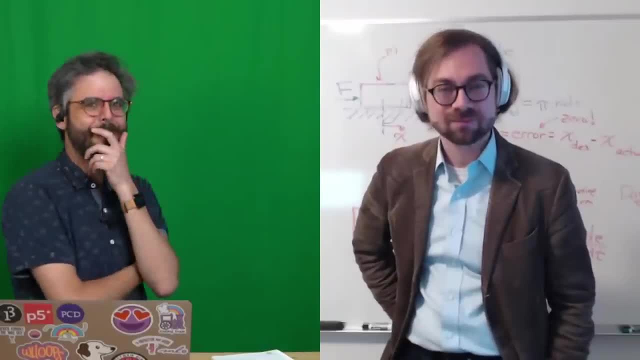 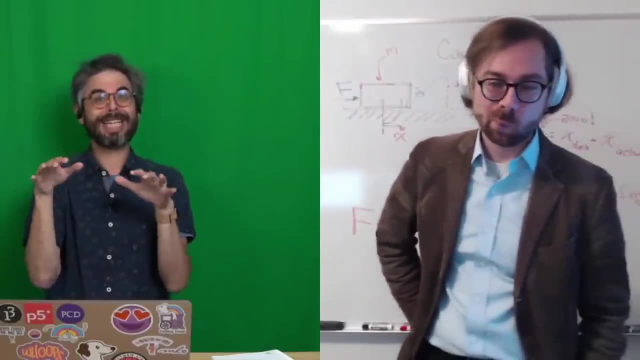 trail right behind them, I don't know because you're yeah so, and so it's kind of like with the birds flocking. we don't use integration in flocking because the idea is just to match the velocity but stay actually like a little bit behind your neighbor. but I'm imagining that's. 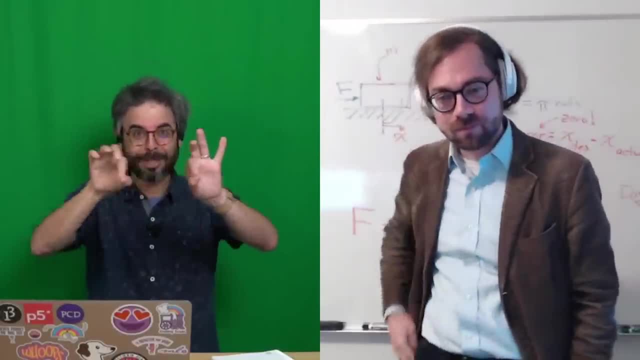 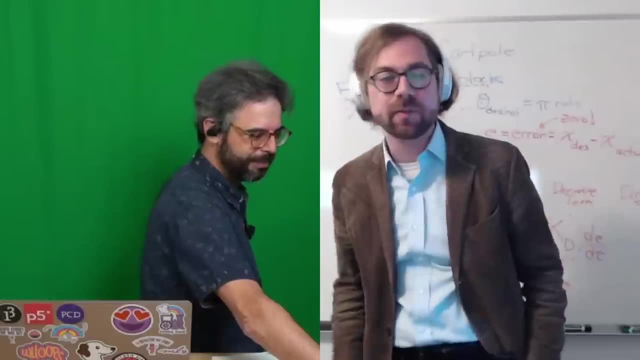 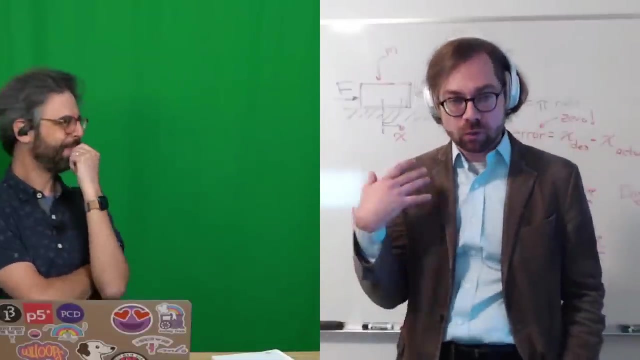 the idea I'm imagining. if we wanted to catch up and be in some type of perfectly horizontal formation, we would maybe need that aspect. Yeah, And there's these. these concepts have extended, extends beyond, well beyond robotics. In fact, you know, these were invented before there were robots. One of the things was the. 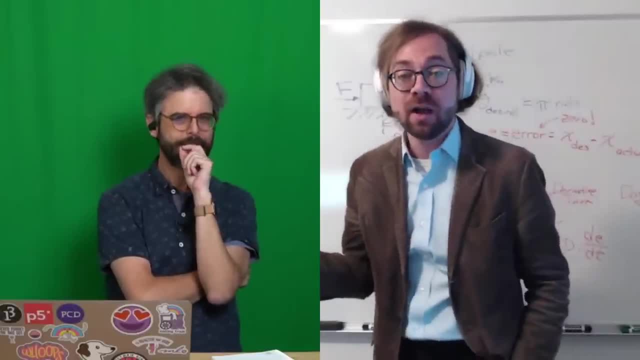 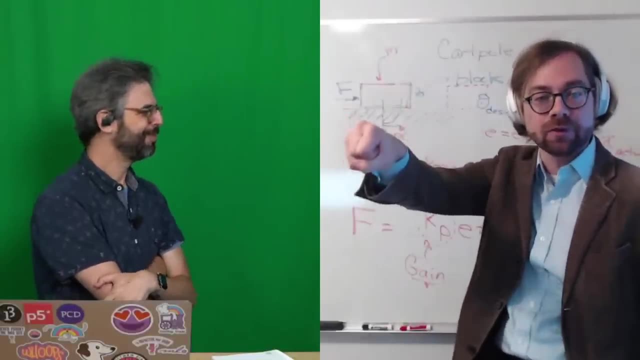 initial applications of PID was ship navigation, for trying to keep a ship on course, for an autopilot. So you don't need some, some, some, some Navy sailor sitting at the wheel the whole time. You know that's a, that's a. that's that. that loses interest for me after the first 12. 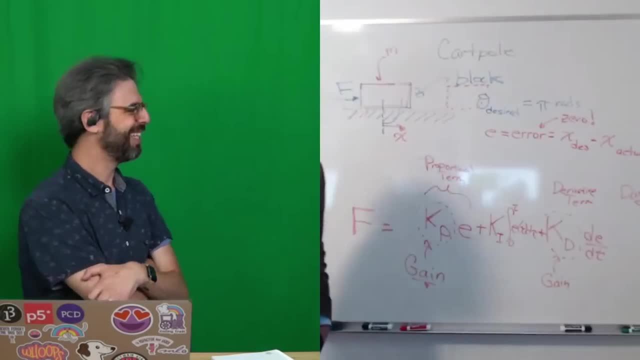 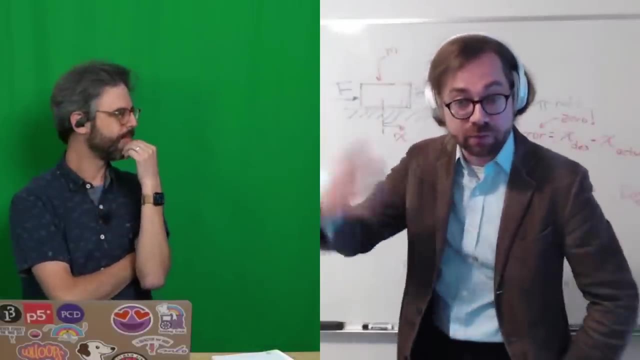 hours or so you know, But that's but. so that's what these things are used in a lot of kind of automation tasks, but also in modeling how, how organisms move around. I mean I, I, I have the good fortune of going to biology conferences every, every year, just about each year, And 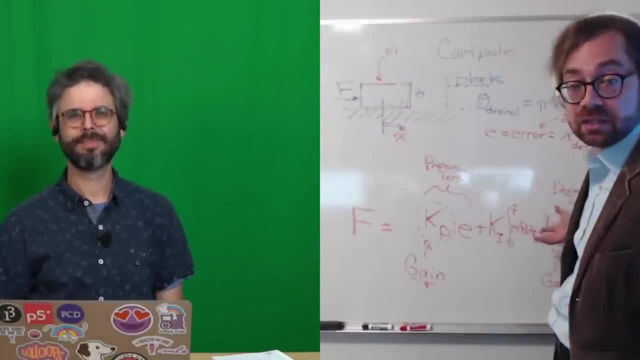 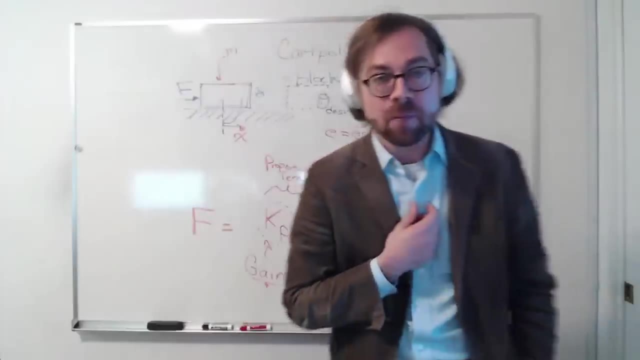 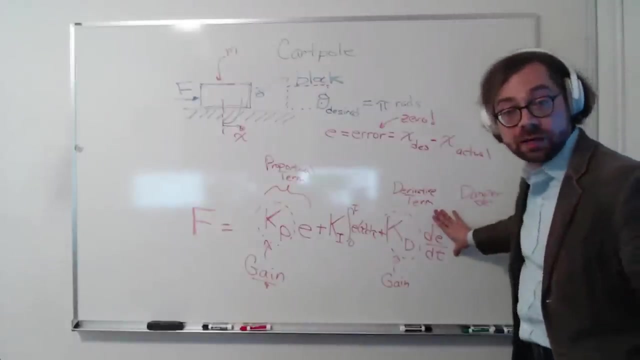 they people will use control systems like this to model animal behavior at times. So that's the big picture. That's what we're going to try to implement today with a, with a primary emphasis on the P and the D control. We can do the eye control as well, But the P and the D will get a lot of your job done for. 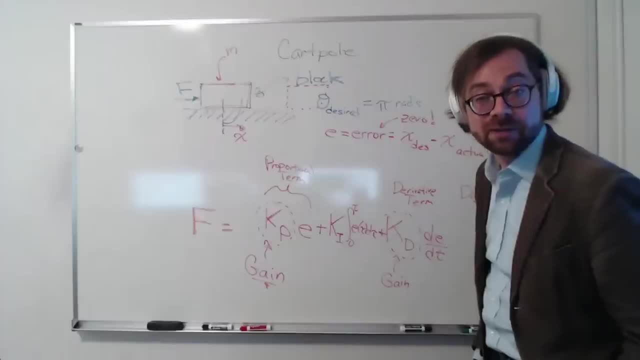 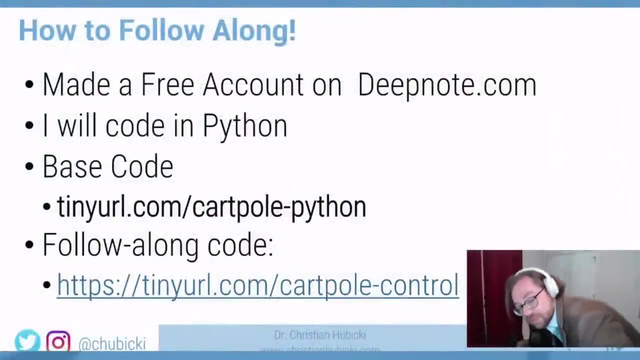 you All. right, cool, Let's go back to the board. So, just so we have these links up for you all to look at, I'm going to be building a top- this base code here from cart poll, slash the high pipe and Python here. Okay, That's going to take you to. 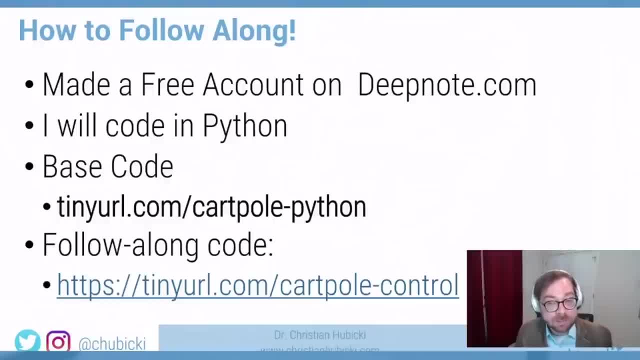 a deep note link which should be publicly shared And you should be able to see. let me know, Daniel, if you have a hard time getting to it or anything. Um, but if you feel free to make a free account on deep notecom, you have, like, I think, a hundred hours a month or something you can use. 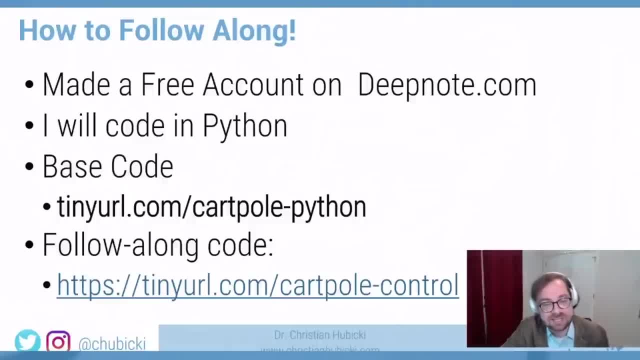 for free, which is normally plenty, uh, for the tasks that I need to do, And I'm going to be going to cart poll type of control too. Yes, There's a question in the chat which is which asks um. just to clarify: the constants are. 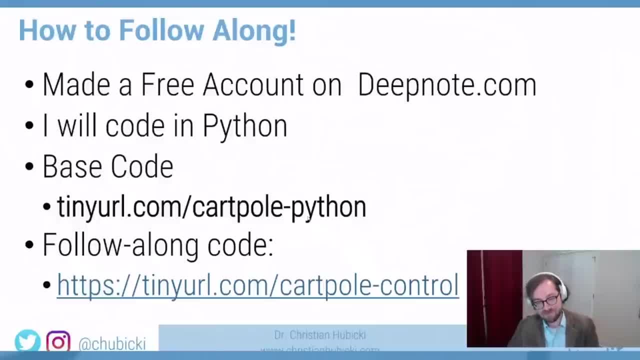 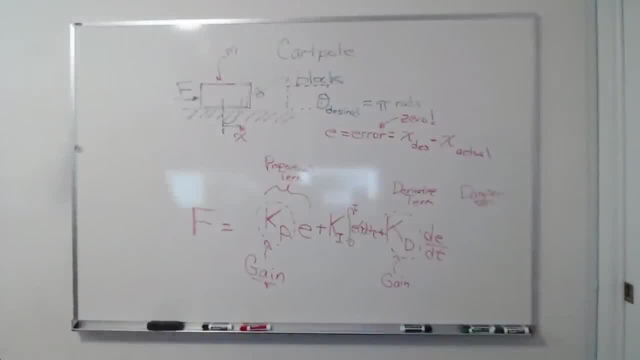 positive, right. Are the constants always positive? Obviously they need to the air, the. the direction of the error is what sort of controlling the direction of the force? but are the constants always positive, I guess is. my question is the question. 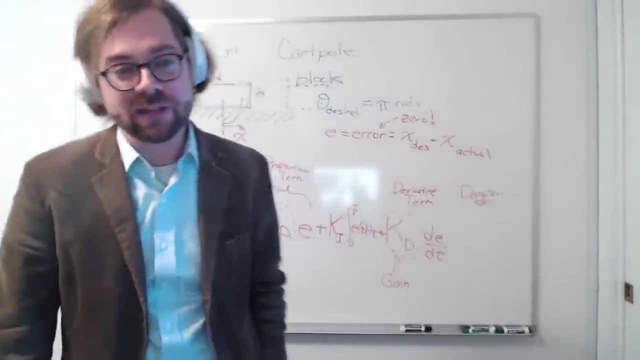 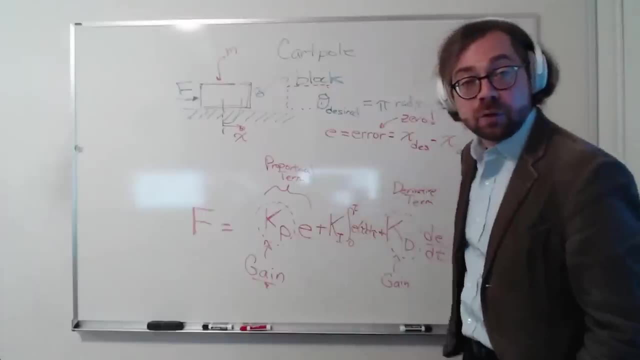 The constants should almost always be positive. I just, in fact, I will go say it always positive, All right? Okay, That's a great question. So we will be dealing. if you are, if you are dealing with negative gains, you probably 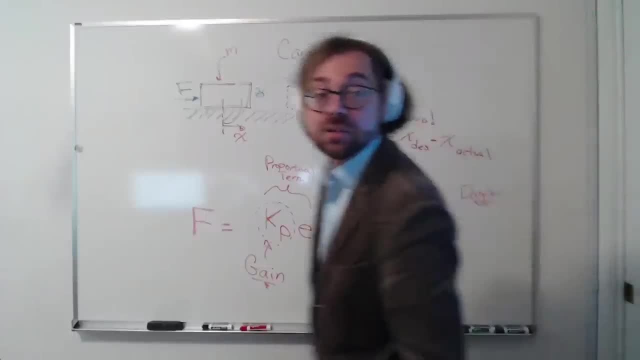 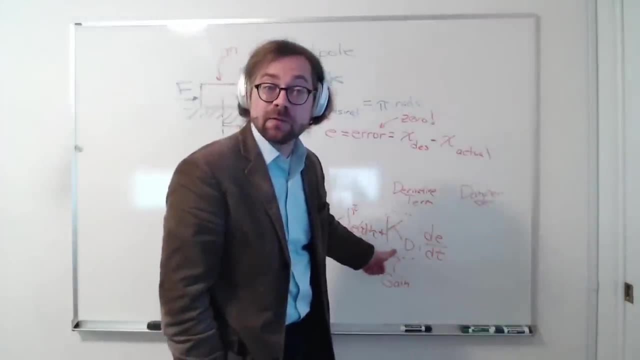 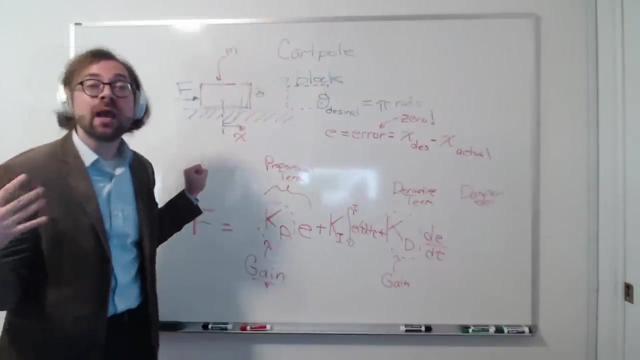 flip the sign somewhere else in your code. Uh, so the reason being: um, let's just take this D term. Okay, This D term, if it's positive, it is always pushing against the motion of your object. Okay, Should be trying to slow things down, which is good, because then you're taking energy out of 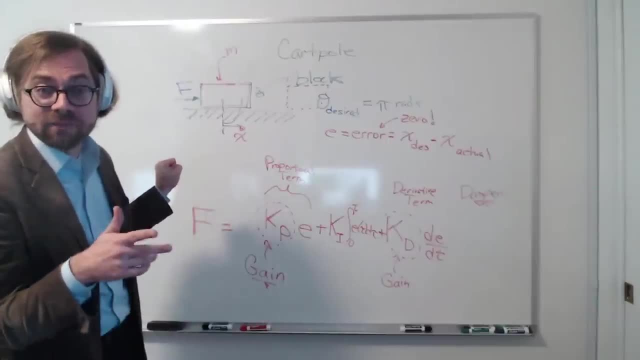 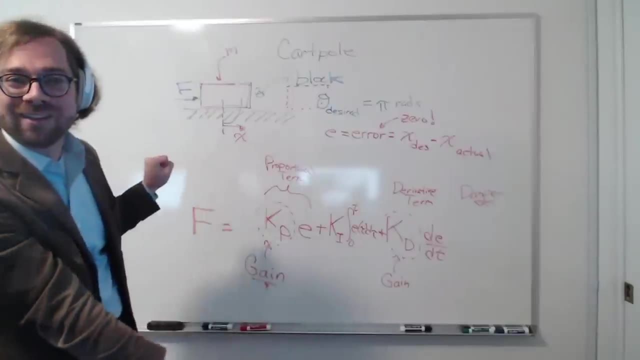 your system. Okay, If you ever had a negative damper, those things don't exist in real life because they basically just shoot energy, Yeah, And and we'll drive things to be unstable. So negative gains tend to be unstable, I think. 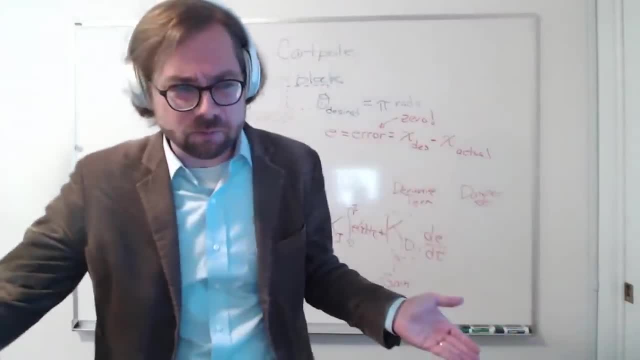 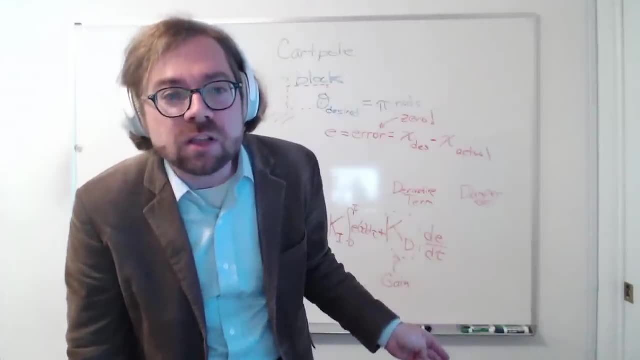 there's the classic. there's a joke that uh is like the most professory joke I've heard in a while, which is the story of the uh, of, of, of the curmudgeony old controls professor, that the 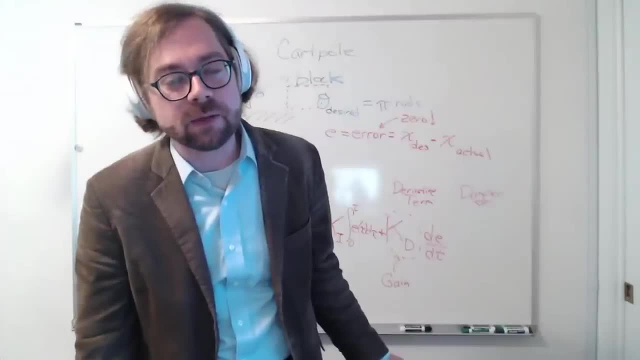 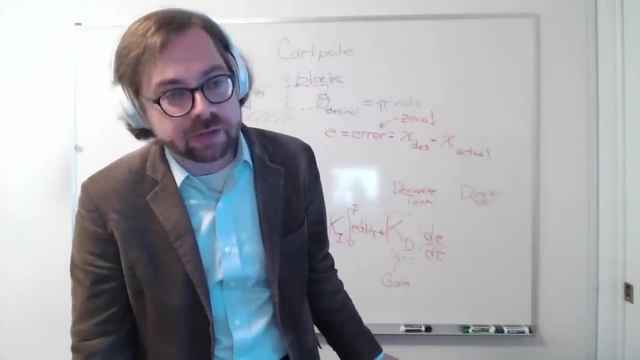 controls professor was always- you know like it was- was really hard on their students And and and by the end of the term the students we worked really hard didn't understand why they were still being you know taught what- why they were still being. 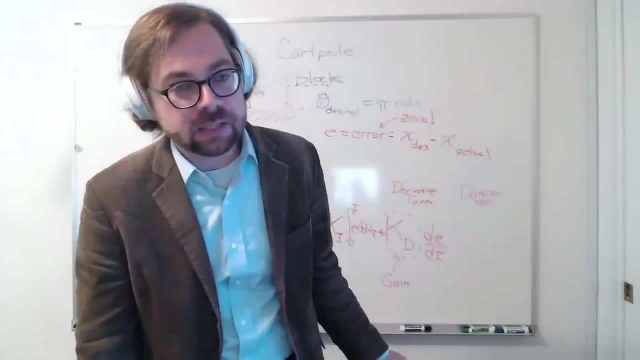 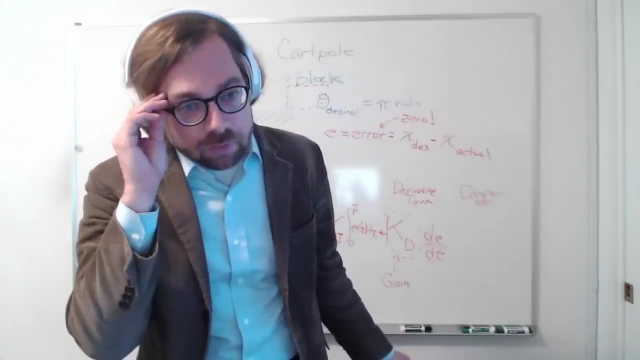 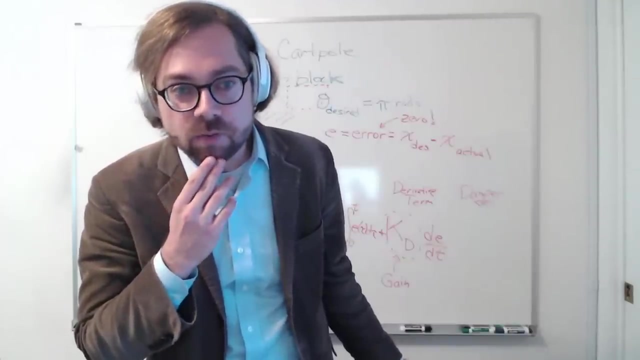 berated for not doing well enough, And the and the controls professor said: well, when you are- uh, when you're- in a control system, if you have a negative gain, that leads to positive feedback, and positive feedback is always unstable. So that's why I only give you negative feedback. 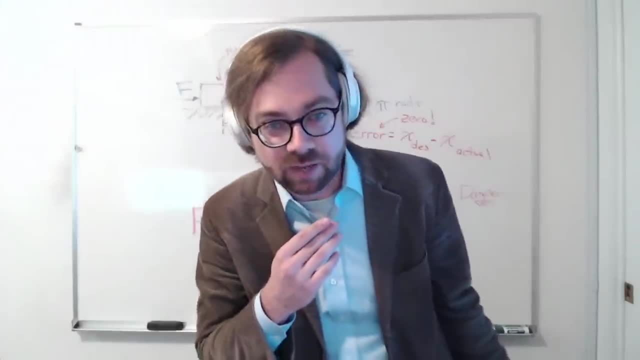 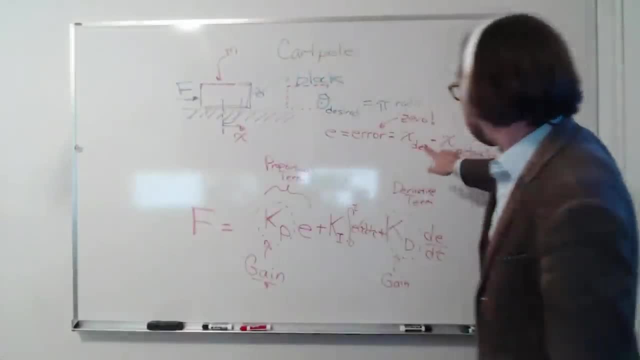 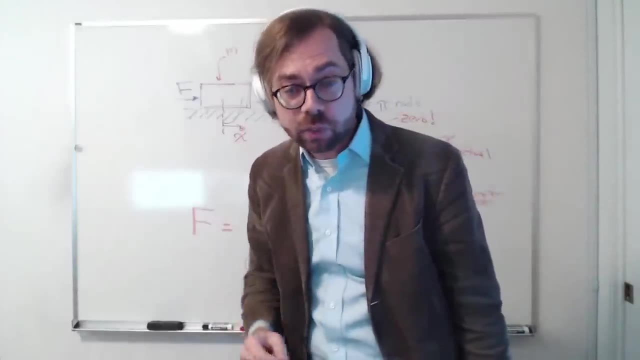 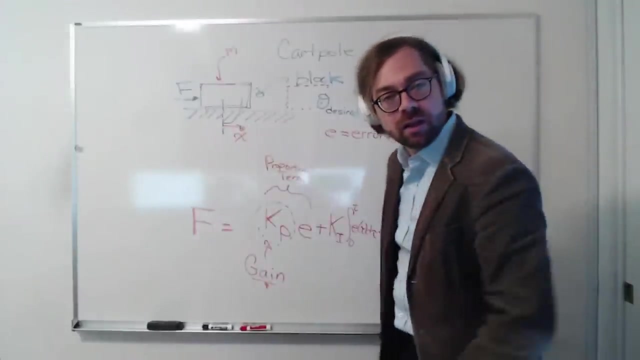 Yeah So, but like it's so the basically uh it, it. it creates unstable systems when you make the game negative and for how you choose games. we're going to do some strategies today that are good heuristics, good rules of thumb, but you can take entire courses in engineering. 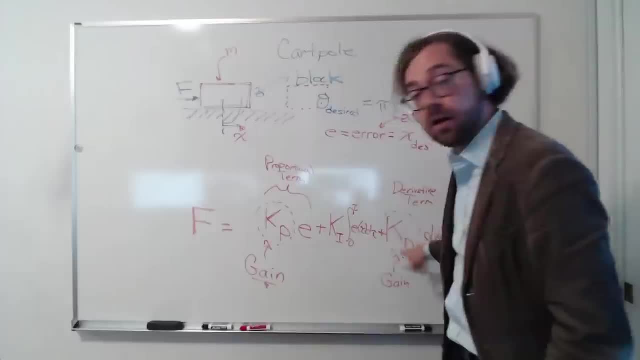 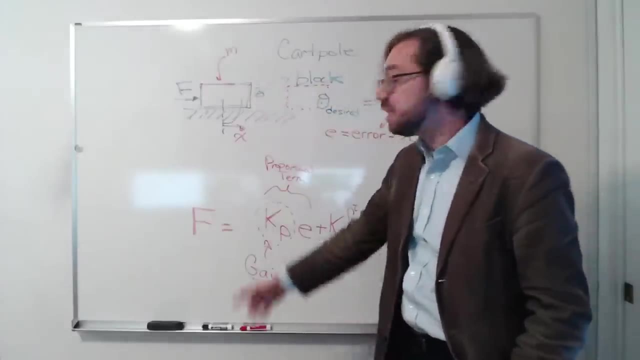 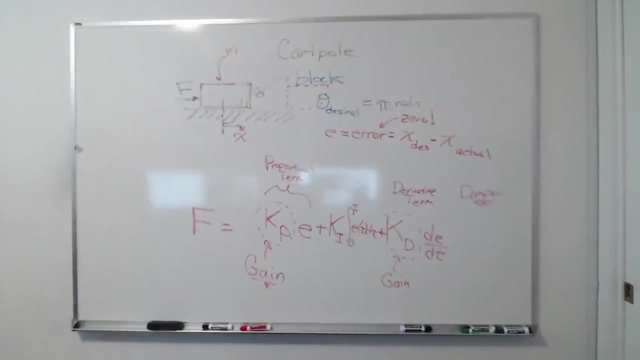 departments and math departments on how to choose these numbers. There are some really sophisticated mathematical ways to to take your system, take your task And then these numbers pop out, these games. but today we'll do it with rules of thumb. All right, Thanks for the question. 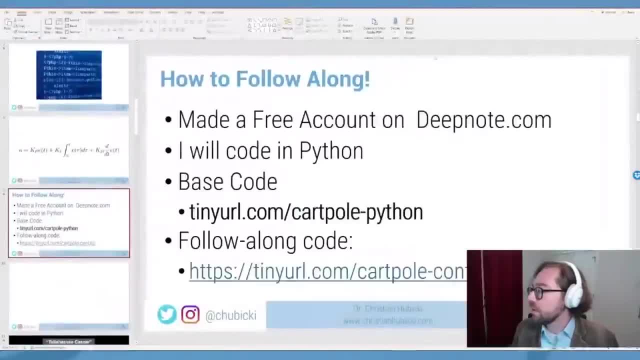 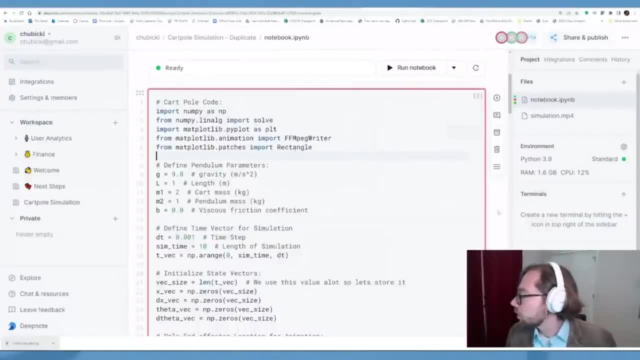 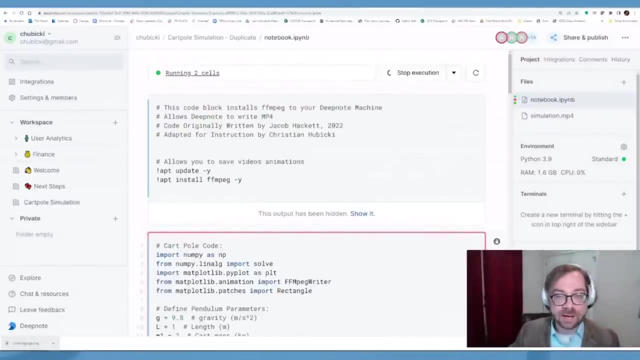 All right, So let's go away here, Okay. So now, if you go to the your URL that I had before, you should see some kind of interface like this, where this is deep notes and deep note has notebooks in Python that you can write up codes and just execute the notebook. 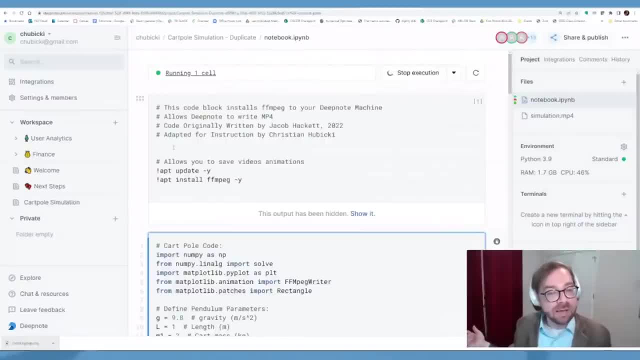 And this prevents you from necessarily having to have your own interpreter on your computer. This, so this way you can just go to a web browser and just start working on things. It's also deep note is good for for sharing books, for collaboration. I know a lot of people like 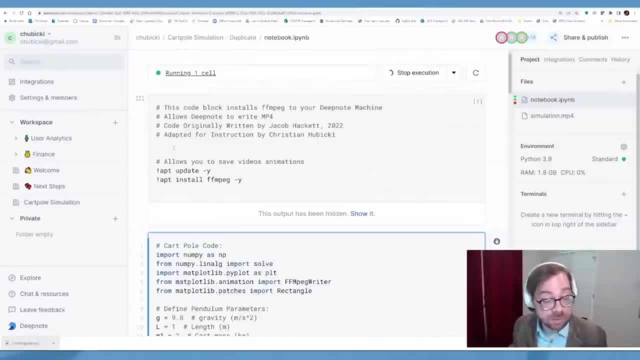 Google co-lab. That's great too. That's a great way to do that, And then the other thing that I'd like to say is that you can use your mouse. If you want to switch your mouse, you can say: it's going to. 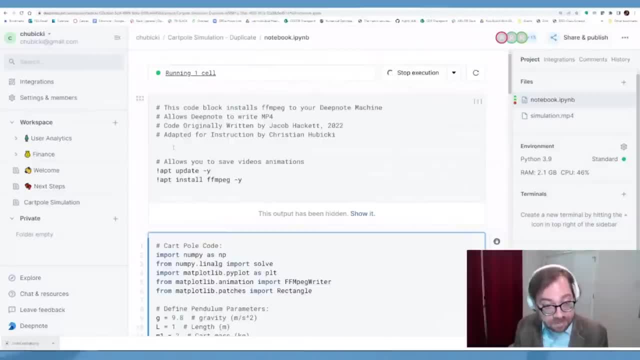 auto, not the mouse. it's going to auto pause. I don't know how many of you use it, So that's really something that I would like to stress to you. And then I have another one right here, So this is sort of coming up here. So this is. I did this quite a few times and it's 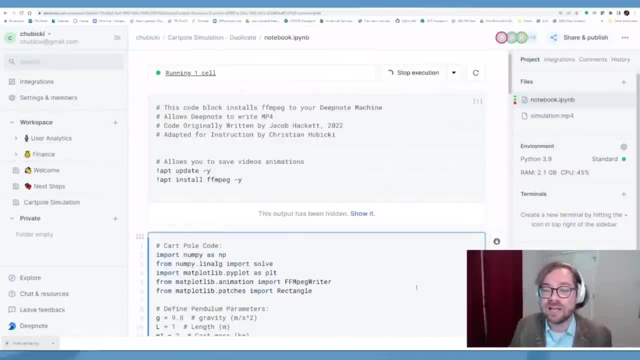 still a little bit more mature than before, but this is kind of- I guess I'll name it. this is my first computer I've used. I've used it since I was a freshman in high school, So basically it's two different devices And this is just one of them And this is just one of my. 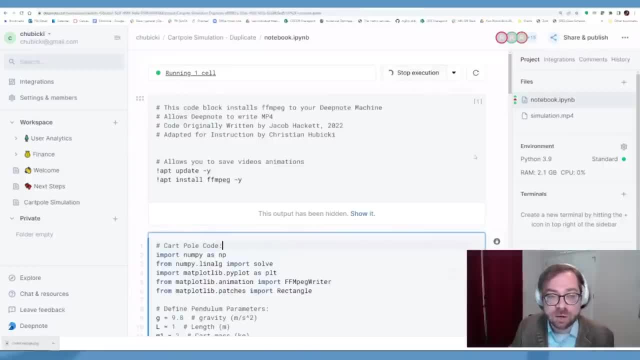 devices, and that was just a second level, And so if you were going to use your mouse, you have to do this with your mouse, and then it should run the code at the link that you're at, And what you'll see is that: 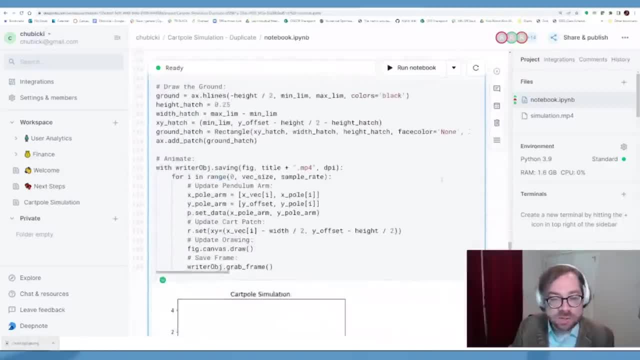 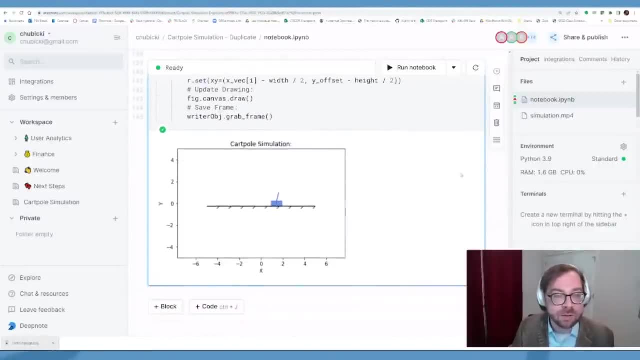 it looks like it should be done, Okay, and it will run all this code. And this code is our cart poll. You'll see at the bottom there's just an image of what the cart poll looks like, But when you run the code, 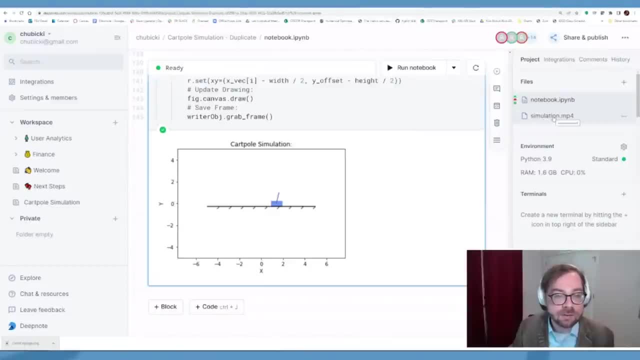 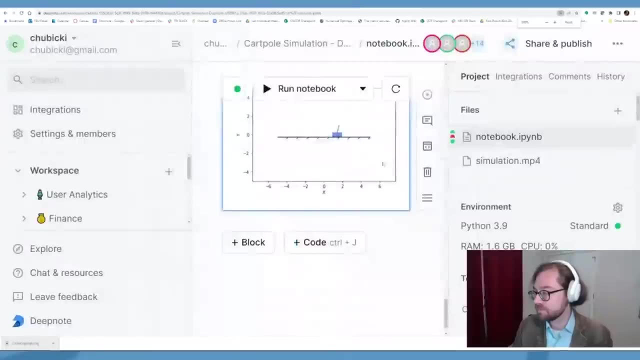 you'll notice on the right hand side. I'm sorry. a couple people are saying that the font size is a little bit small for them. Is there a quick way to zoom into the page? Sure, there you go. Thank you, Good to know. 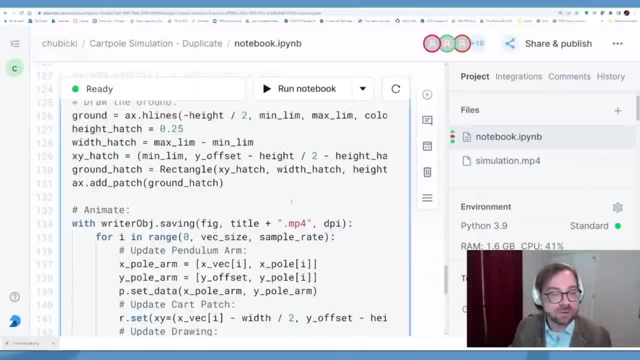 All right, so let's see if I can get rid of that so that we can see it a little better. Thank you for letting me know. See if I can make this a little smaller over here. Well, hopefully this will be a little bit. 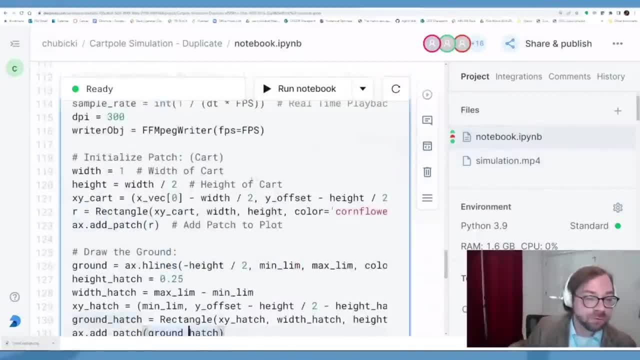 Good, thank you very much. So yeah, so anyway, this is code. Thankfully, I was not explaining any part of the code specifically, but if you click this run notebook button, it'll run it over the course of, I think, about a minute. 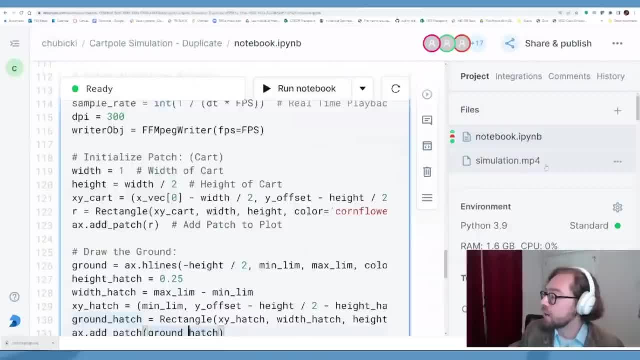 just because it has to get the servers to do it, And over on the right it'll pop up this little thing that says simulationmp4. And that's going to run as an animation that you can then download. This is why I especially look forward. 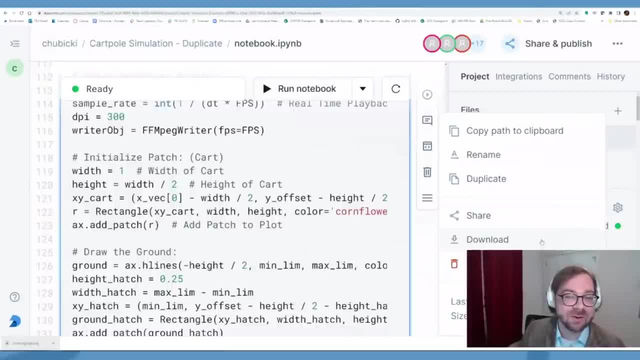 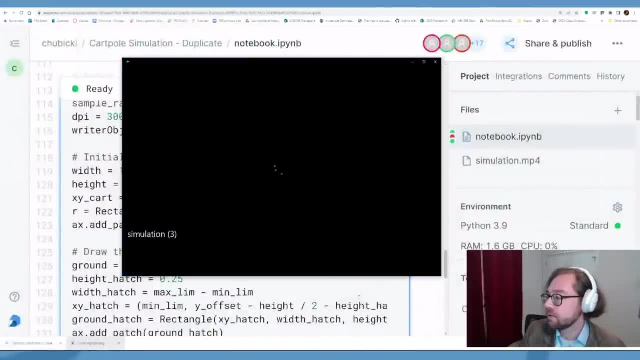 to seeing how you handle this. Daniel, You have a much more real-time way of getting your animations up here, And so I'm gonna download that, gonna run it, and it'll give you an mp4 file that you can run on your computer. 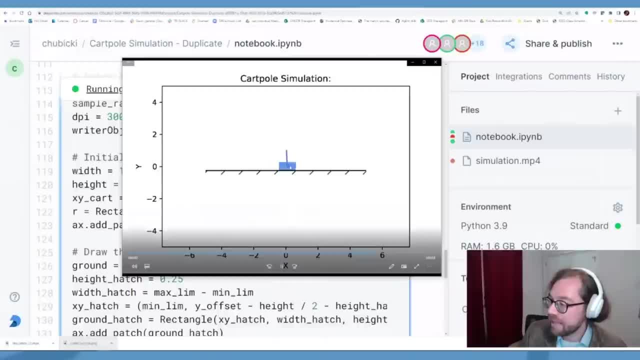 And there's this little cart poll where there's a mass to the cart and then there's a mass on the end of that little poll and it just swings around. See that Cool, right? Currently zero control in it, though, right. 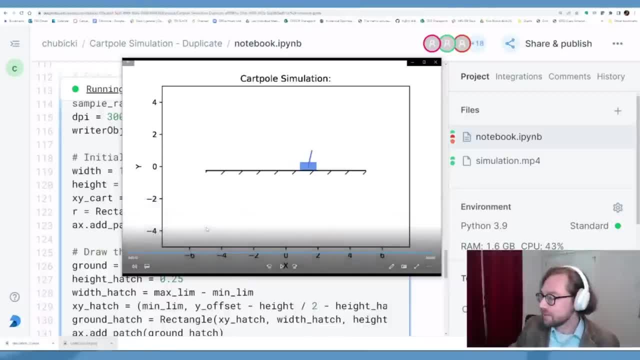 Zero control. So that's what we're gonna add today. So the first thing we're gonna try to do is we're gonna try to control just the cart. okay, We're gonna move the cart from where we start, which is at like zero. 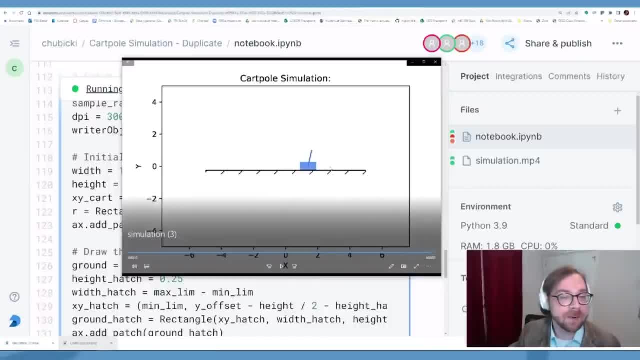 and let's move it to like position of like three. okay, And we're gonna use PID controller to do it. So we're gonna use PID controller to do it. So let's go for it. So we'll go back to the code. 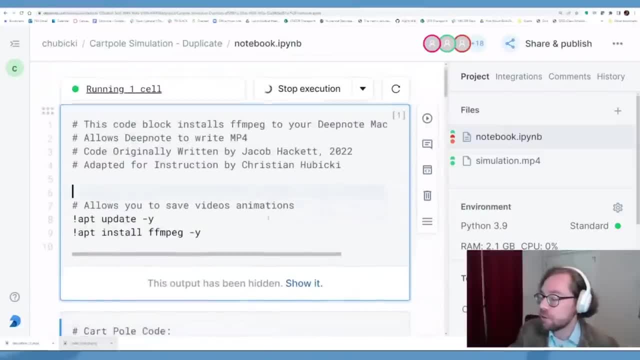 and I'll give you a little tour of what's going on. okay, So this is code that was originally made by my PhD student, Jacob Hackett. thank you very much to Jacob. that is set up to automatically generate this simulation of the pendulum on a cart. 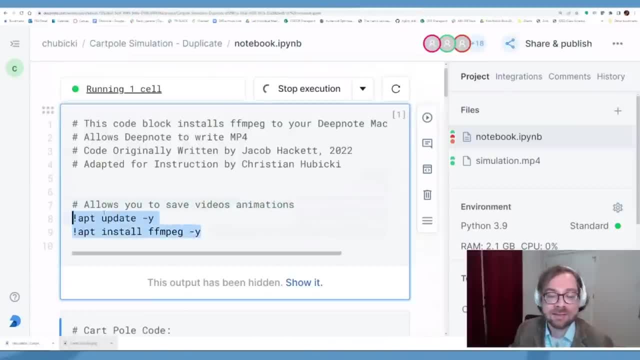 And up at the top here is some code using FFmpeg. It's just baseline code to start making, setting up how to make a video in code. That's all it's doing. You don't have to worry about any of that. I've carefully partitioned out. 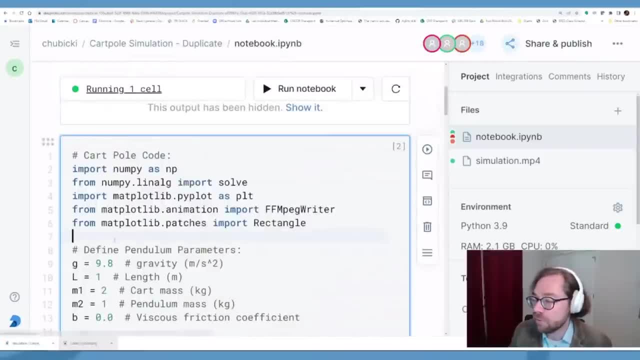 where you do have to worry about stuff. So here you have all of your libraries in Python, and in Python, a super popular one is called NumPy- NumPy or I don't know who pronounces it in what way, but this is how you do a lot of your good numerical. 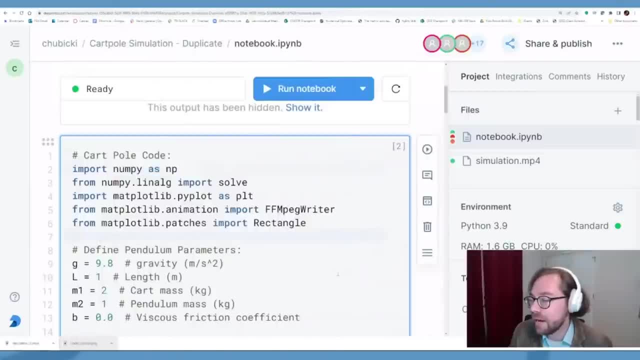 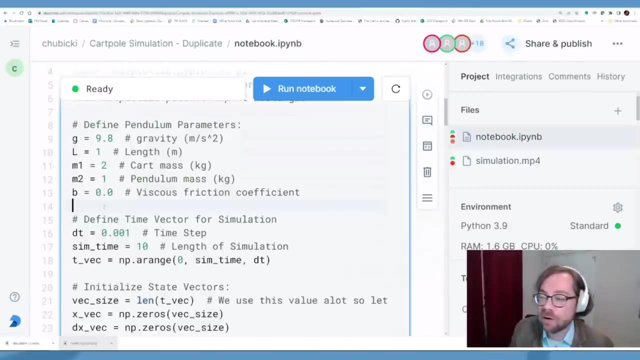 numerics and mathematics in Python, okay, And a number of other things that we use, and that's all gonna go into, basically, the simulation part, the thing that is simulating the mechanics of this thing swinging around. okay, Then we're gonna define the parameters of our cart pole. 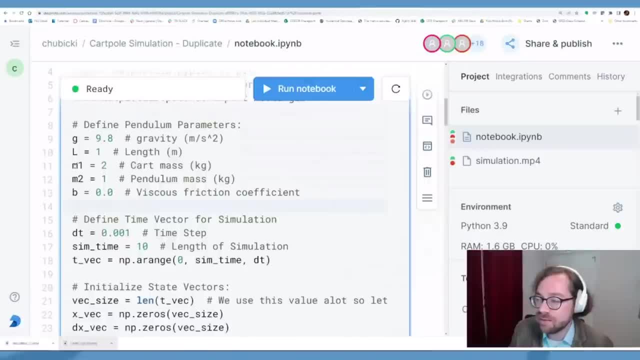 And you'll see that there's gravity, there's a length, there's the mass of each cart. ignore the little pop-ups that keep coming up here. They try to be helpful. We try to be helpful with these pop-ups And so you can change those parameters around. 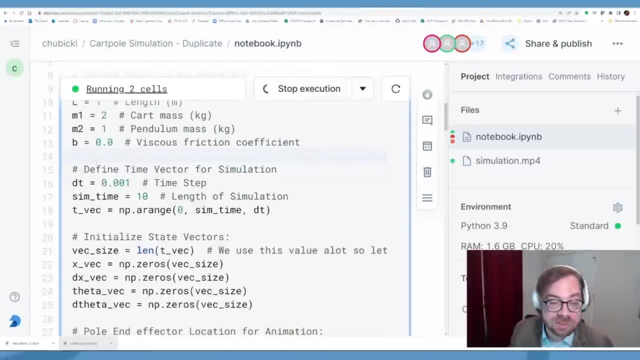 as you would like. okay, And here are some parameters of the simulation. For those of you who don't know how these computer simulations work, they work by taking little time, steps in time and saying, hey, I'm currently at this position and this speed and I'm gonna use 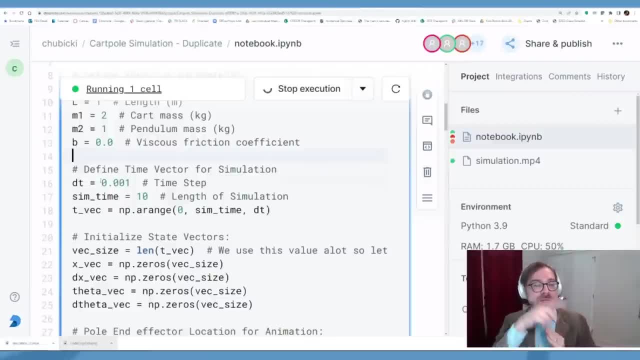 what I call the equations of motion, and compute how much this thing should move over the next tiny bit of time, some little time step, And that's what this DT is okay, So, and then it will compute how it moves over that time step. 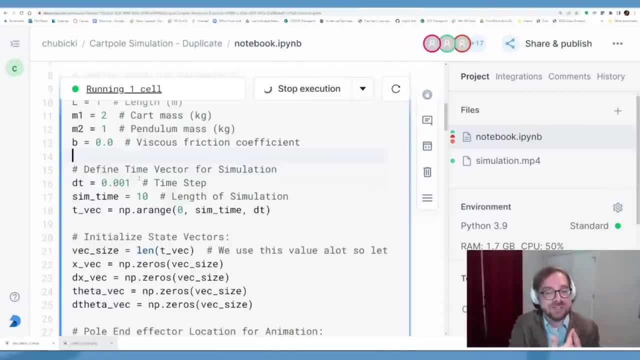 It says. this is where I am now. reuse those equations to figure out where I need to be next, and then next, and next and next, and then repeat until you have a full simulation of the motion of your system. That's what this little time step is. 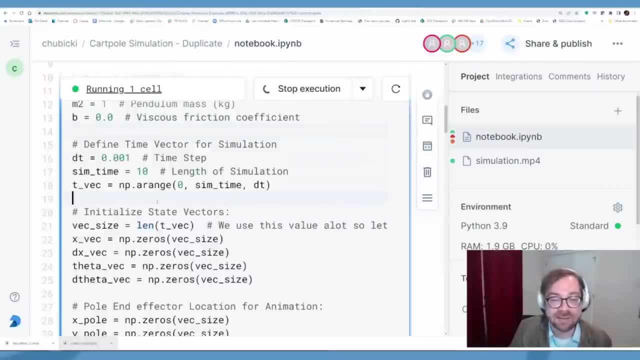 And there are many ways to do that. We're using a fairly simple method called Euler's method. That's for another time. Did you ever cover Euler's method on your stream here, Daniel? is this a thing that I imagine? you have to simulate things. 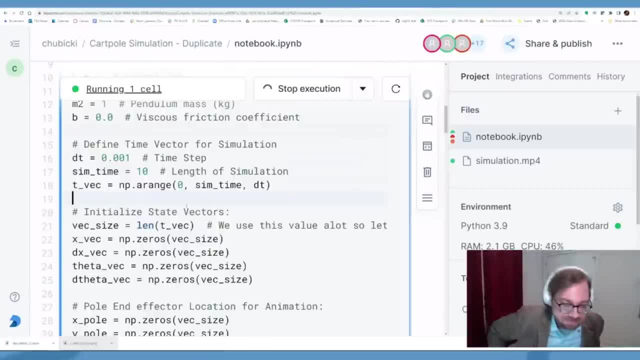 This is a frequent discussion And so, yeah, Euler's integration, that's the primary integration method I use in almost all of my examples. yes, And we've talked about various other techniques, like Verlet integration and there's like the Runge-Kutta. 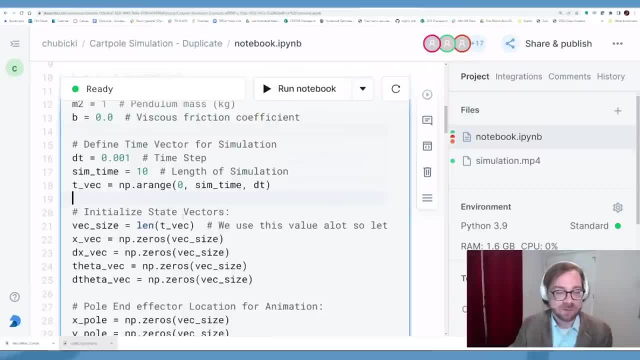 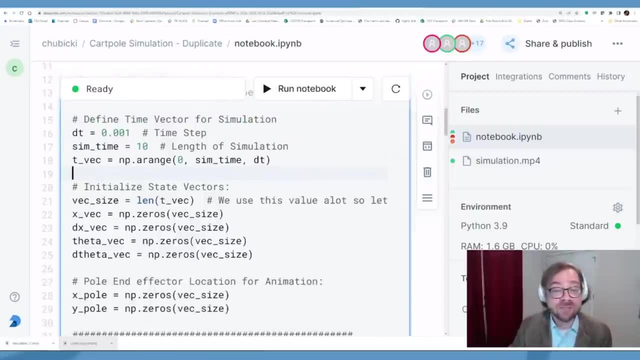 which I'm always mispronouncing. So it's come up before and is also a big aspect of the various different kinds of physics simulations I've done Great, so yeah, so that's what's happening here, So nothing you haven't seen before. 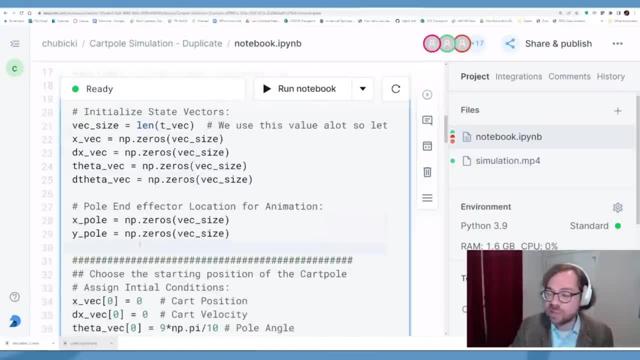 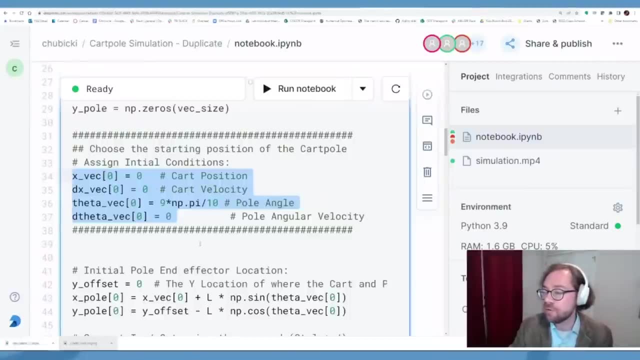 And we just initialize. we do some initializations of our variables And I think that one of the things that we do change is we can change our starting position of our pendulum and we can change our starting position of our card. OK, 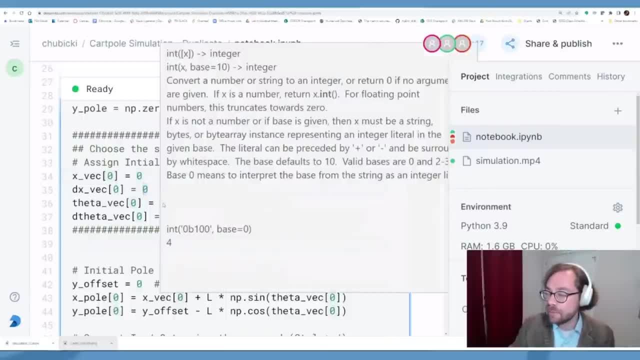 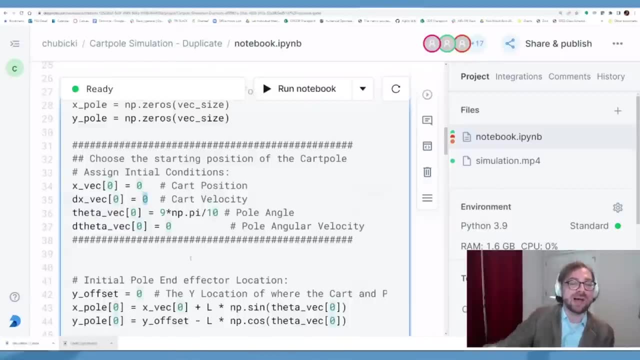 I said that I'm going to start it at position of 0 with a speed of 0. And then I'm going to change the pole angle, excuse me, to be 9 pi over 10, so like 9 tenths of pi. 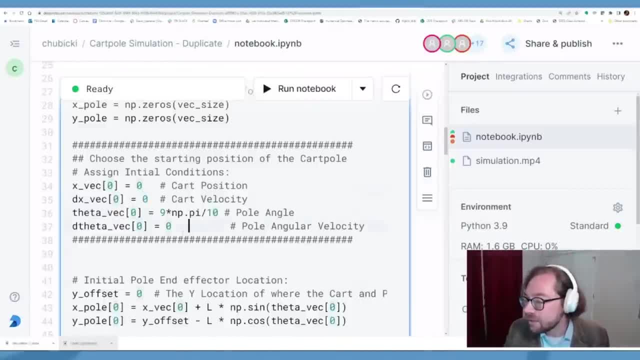 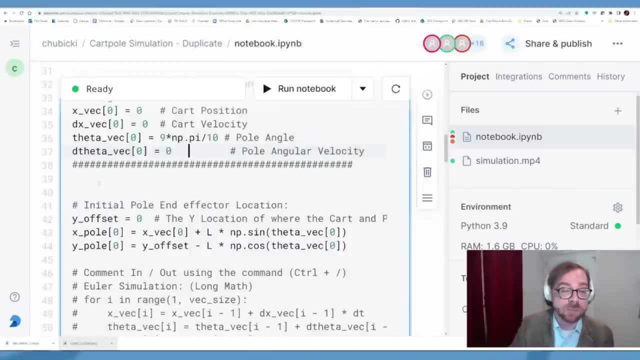 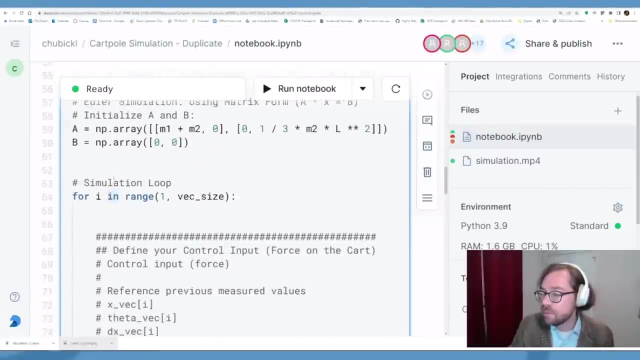 so very close to pi kind of. so kind of close to pi and with an initial angular velocity of 0. So we set those initial conditions there, And so that's how we set where the card starts, And then we get down to the simulation loop. 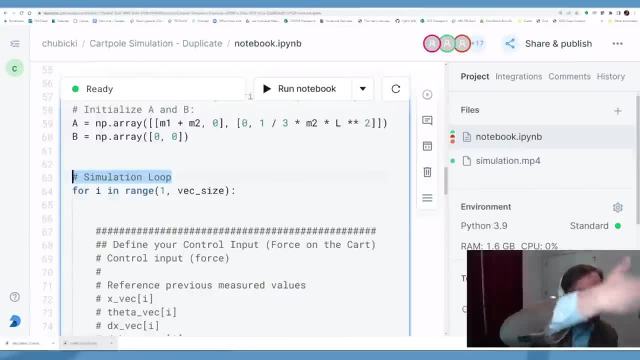 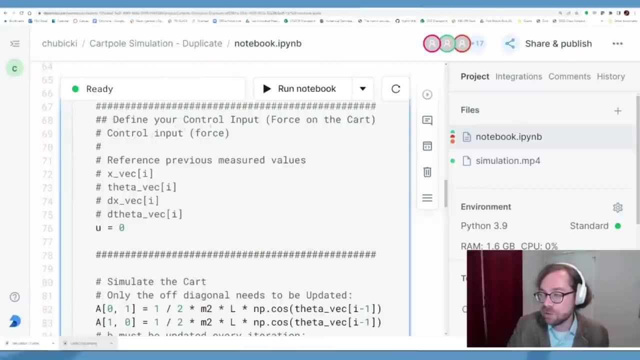 This is where we are taking steps through time to get our simulation, simulation, simulation. I've blocked off this handy dandy little section here, for this is where we're defining our control input. So that's going to be our control, our control. 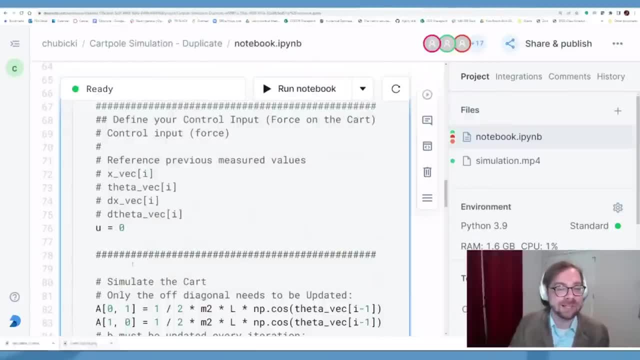 order right here. all right So, and the level of Python we'll need to use is very simple, So you don't have to worry about it too much if you haven't learned Python before, But if you have, you can tear it apart. 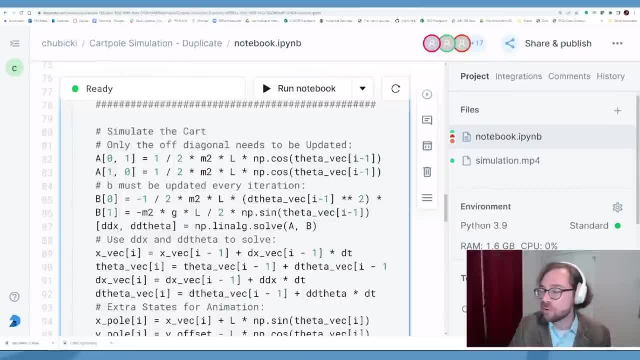 and do what you want with it. And then down here we have the actual simulation calculations for the pendulum on a cart, And I know that you simulated the double pendulum in the past, which is a pretty darn complex system, So there are a number of ways to do it. 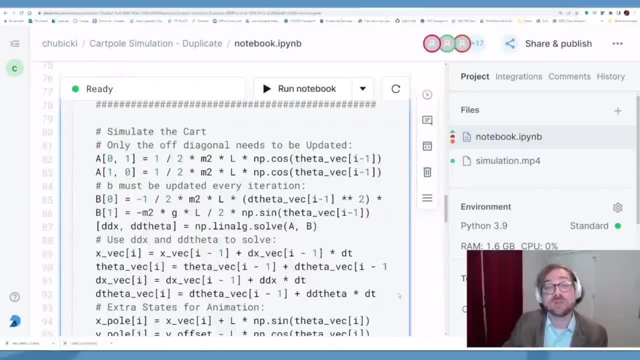 Here we actually set up the equations of motions as a matrix operation that we then solve and then come up with our accelerations for our equations of motion. That's what we do here, And then at the end there's all of the stuff. 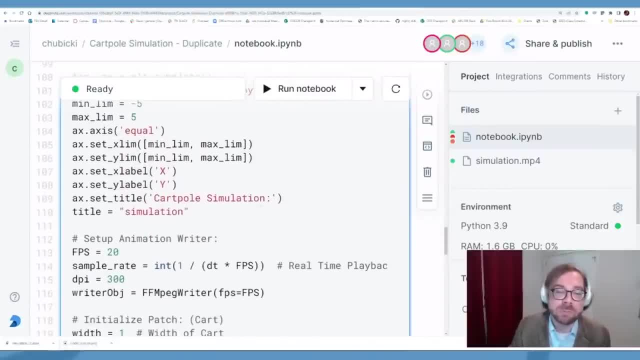 where we define our animation. Any Python wizards or Python enthusiasts or Python learners want to mess around with how the animation looks. put a cat on the end of the pole, by all means. So that's all that's going down at the end. 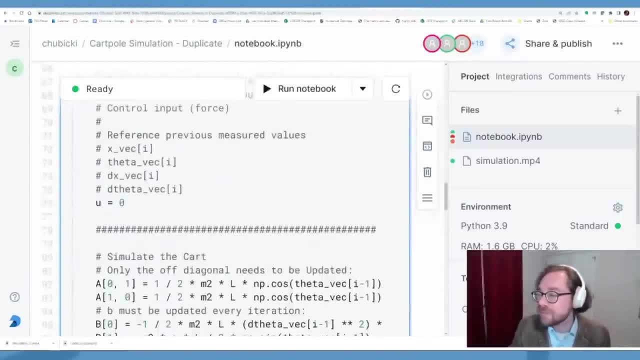 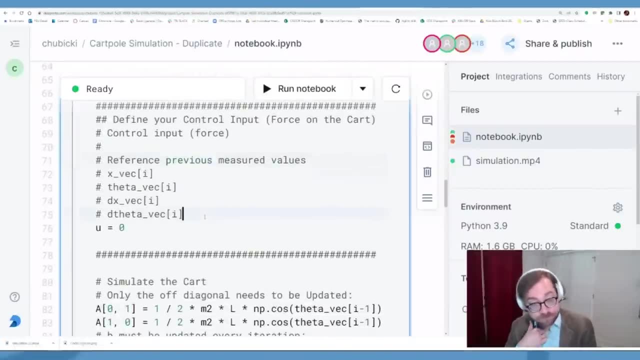 So what we're going to clearly focus on, though, is the controller, So let's go back up to our controller- And I've commented this up already, so that way you know how to reference what variables and how. OK, So let's start by just controlling, but by just 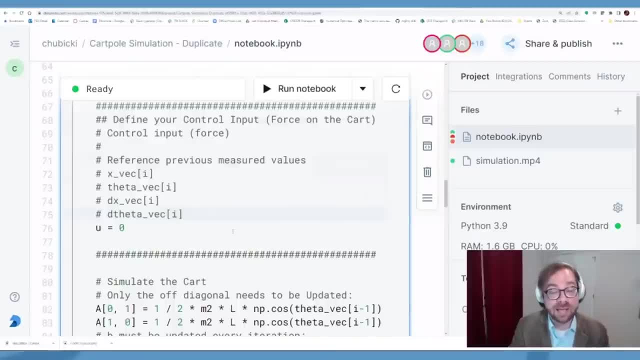 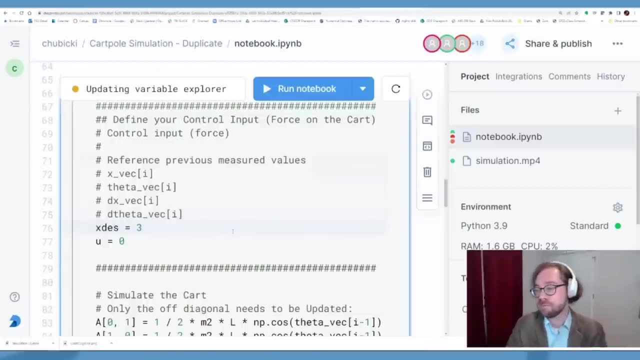 moving the cart to that position, 3.. So let's have a desired x, which I will label as xdes is equal to 3. And I'll resist not typing a semicolon for my other languages. OK, All right, So we have. well, this is our desired cart position. OK. 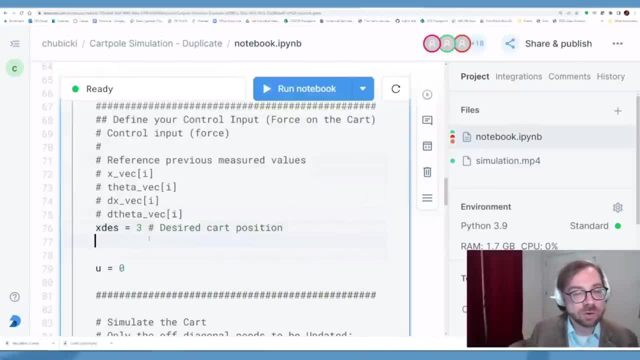 All right, And we're going to do a p controller to start. So let's do a kp And we're going to do a kp And let's just set kp equal to 50,. all right, kp is equal to 50.. 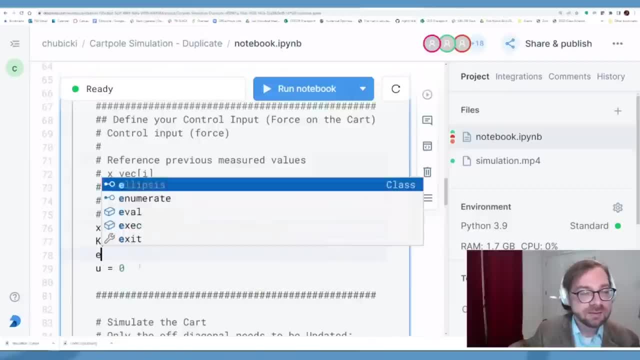 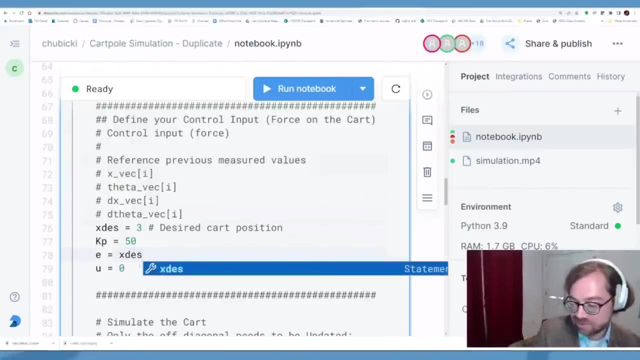 Now we need to know what our error is: e. So I'm just going to define e as being our desired minus actual. I always remember desired minus actual, like district attorney by some mnemonic device: Desired minus your actual. So our desired is xdes. 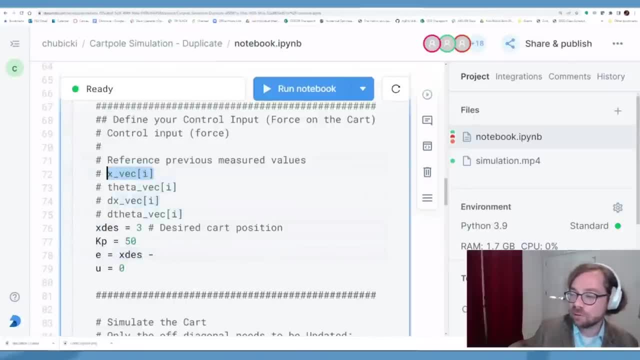 And our actual. I gave you a convenient little thing: You can grab xveci, which you have to do minus 1.. Put it in here: minus 1.. So basically, it's our last measured position is what this is. so: xi minus 1.. 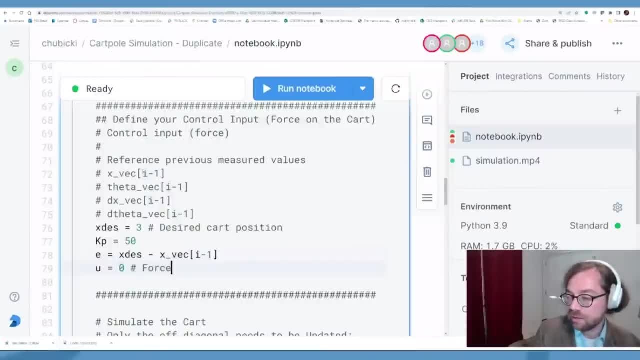 So here is our actual force. You'll notice it says u And you're going to say Christian force doesn't start with u. That's correct. In control theory, control inputs are often designated as a u. That's just a convention we like to have OK. 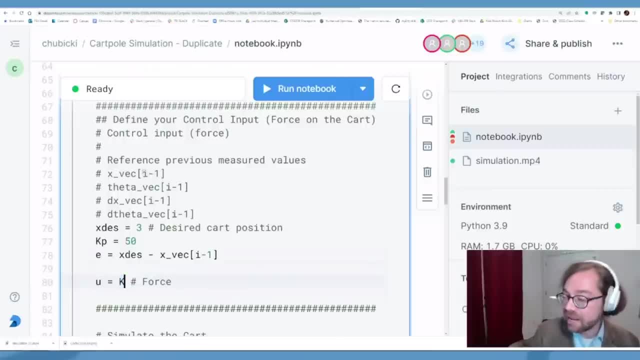 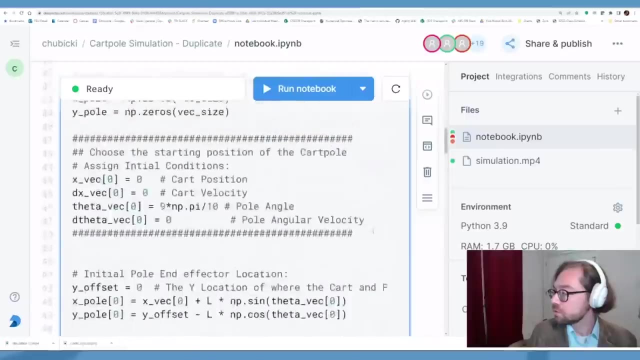 Control inputs are u's, And so we're going to say k. So our proportional controller is going to be kp times error. Simple enough. So what I'm going to do is I'm going to scroll up and just run this block. I'm in. 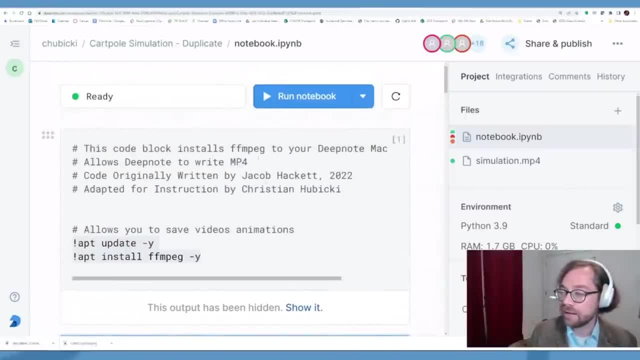 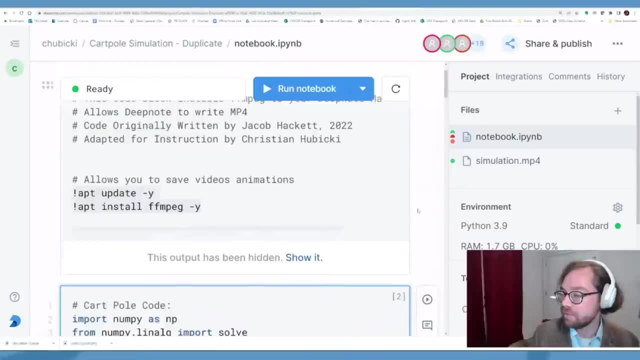 That'll save you. I'm having to run this block. You don't need to run this top block every time. This just installs FFmpeg so it can make animations, So you can run the whole thing. That's fine. I'll just redo this. do this command. 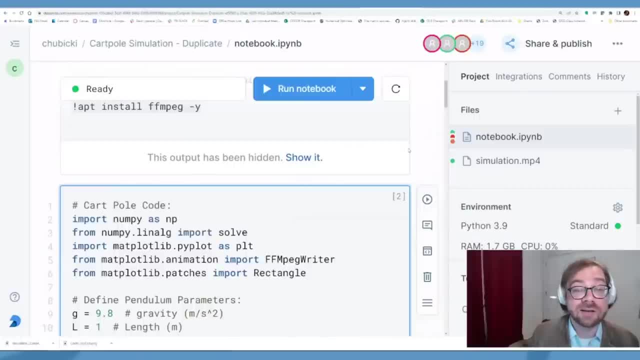 And that's not the best. And are people able to see the text OK enough, Or should we do? It looks good, I think. Good, Great, OK, I can always make it bigger. I just wish I had a bigger monitor. 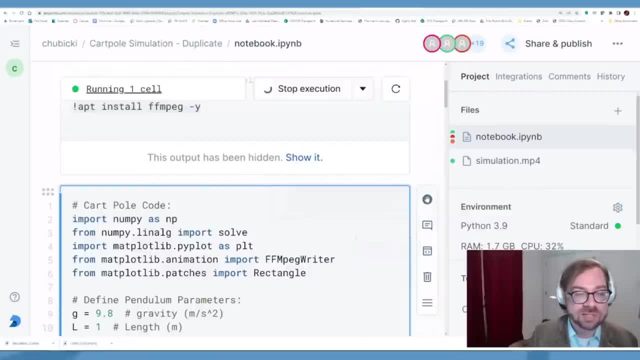 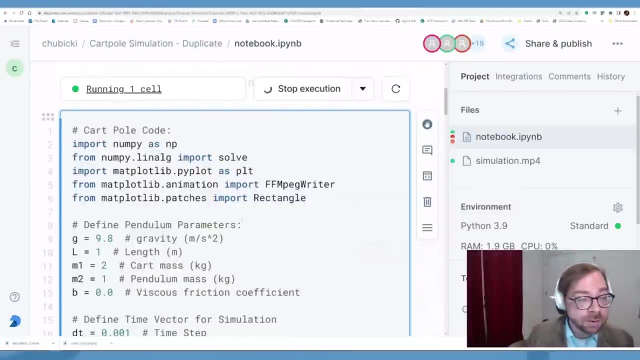 That's all. So I'm going to click that little arrow- that was right there- And it's just going to execute everything in the second big block, which has the simulation. OK, This will take a little bit And while it's waiting for the server to run, our code. 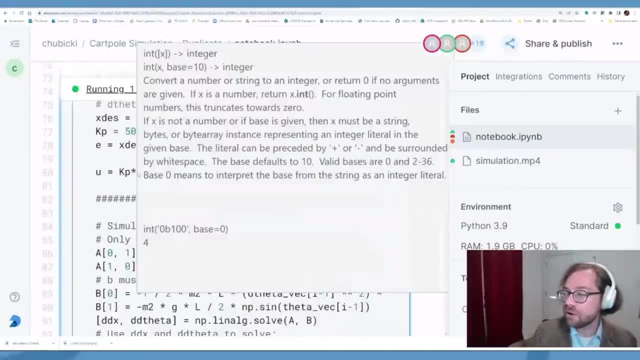 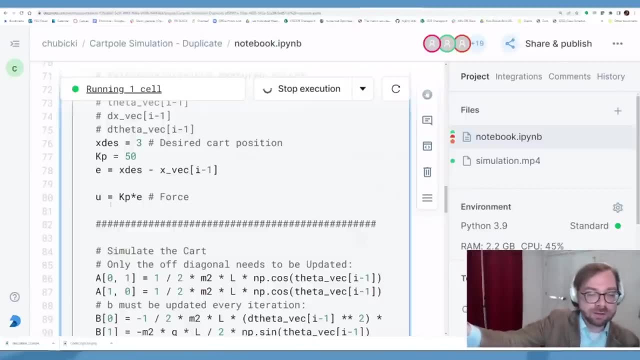 I'll point out that this is going to try its darndest to keep the. it's going to try to push the block toward that position, But it's not going to know how to stop. This is the spring attached to our block. 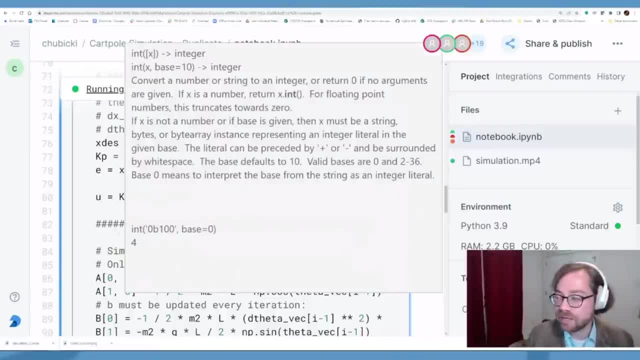 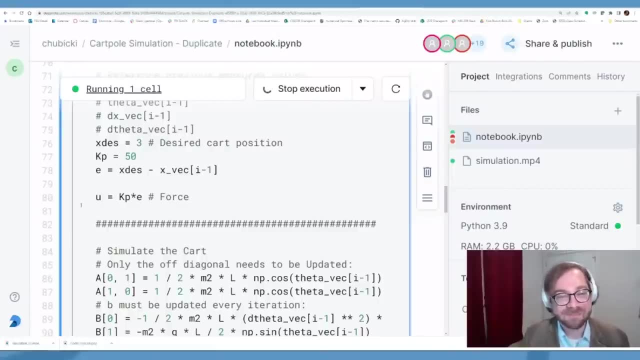 And I chose 50. And people say, hey, is that big or is that small? It honestly depends on your system. OK, And is this a sort of idealized system? Is there any friction between the cart and the ground or other forces at play? air resistance. 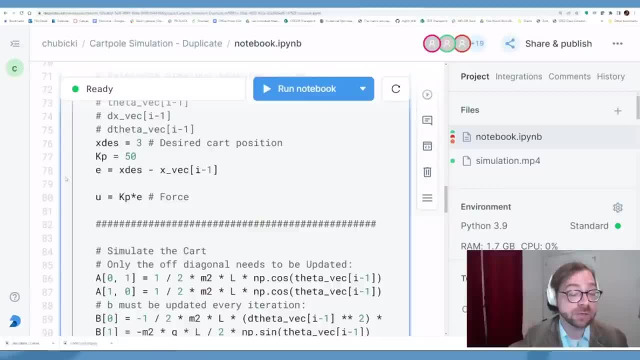 This is a pretty idealized system It has. there is friction with the ground, but I turned it off just because for demonstration purposes. But a very idealized system, Daniel. All right, Looks like it's done, So I'm going to download. 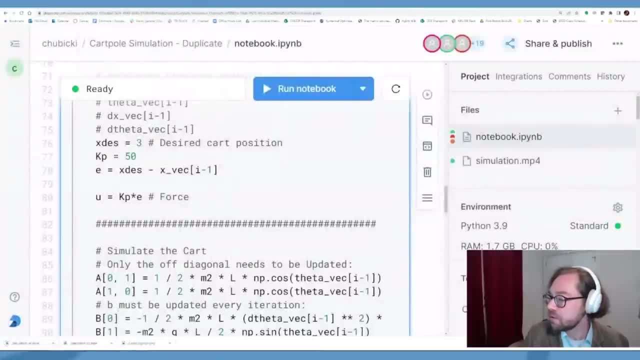 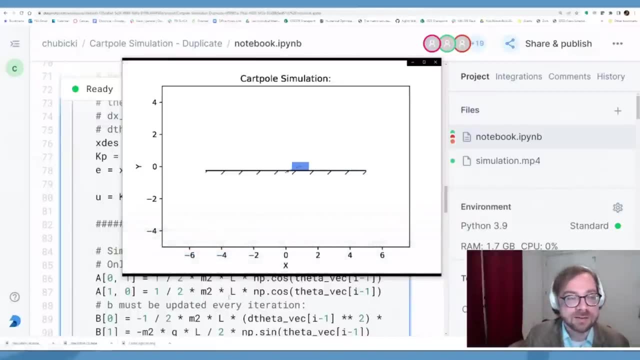 I'm going to download this and cross my fingers See how it goes. Whoa, Hey, look at that. It's a spring, just like we anticipated, with a little pendulum swinging around Again. we don't care about the pendulum. 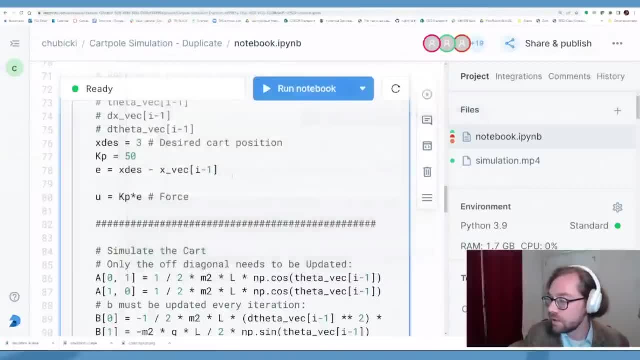 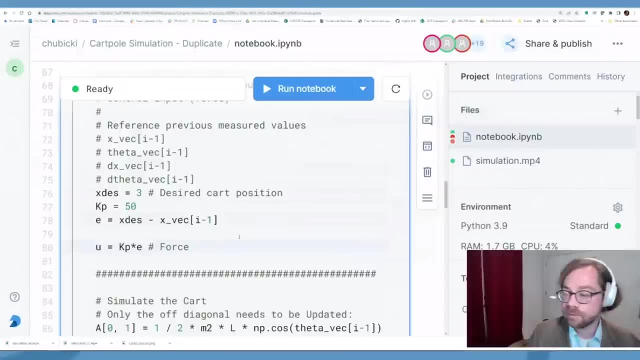 So pretty much as we anticipated. So that's the P control. Let's add the D controller here. OK, So we have a proportional game. Now let's make a derivative game. Now. my rule of thumb is: I try to make my derivative gains. 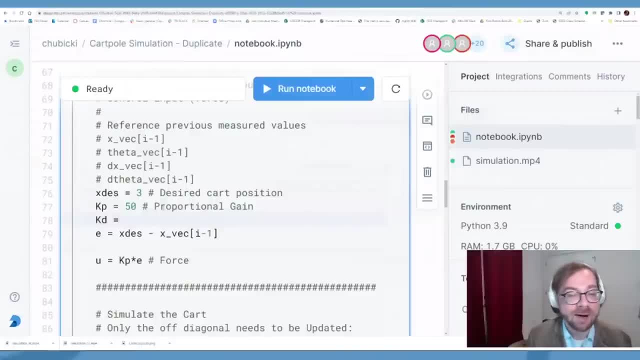 about 1 fifth of the proportional gain. if I'm just messing around, If I don't have any math to tell me otherwise, it's a good starting point. OK, So I'll make it 10.. That's our derivative game, The thing that's going to slow us down. 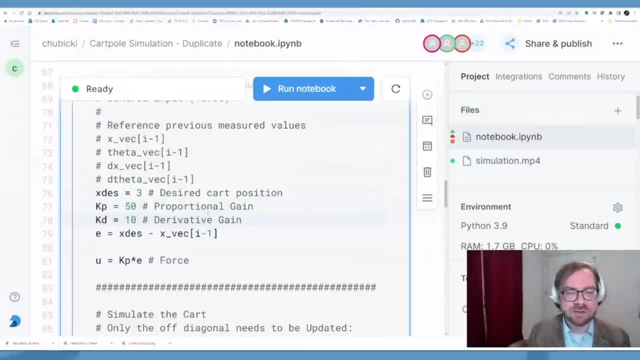 OK, And that's going to be proportional to the derivative of our error. OK, And so just I'll go back to the board and say, well, what's the derivative of our error? And I'll do just a little basic calculus. 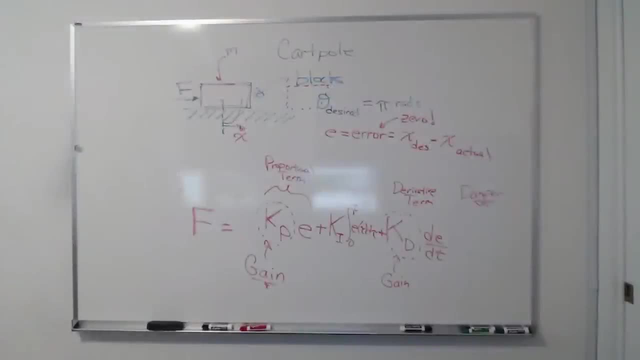 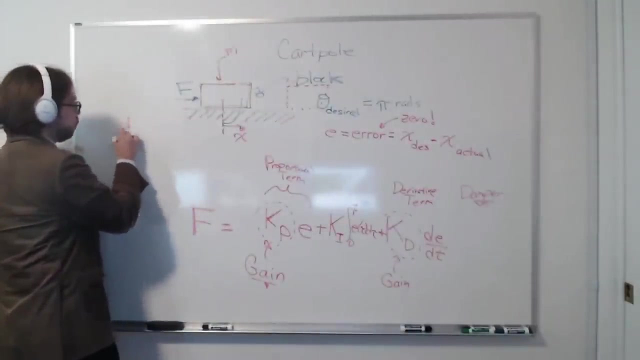 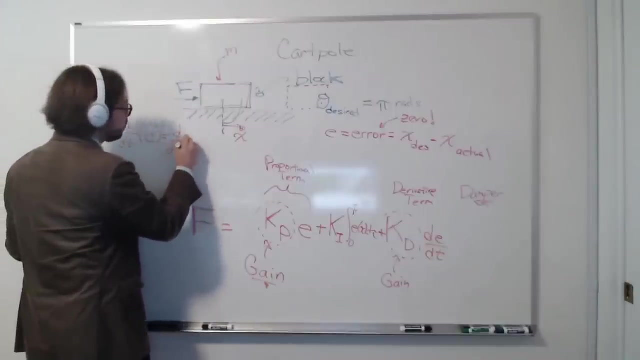 Don't fret if you haven't seen calculus before. OK, That if we are taking the derivative with respect to time of our error and our error swing my microphone around and our error is your x desired minus x actual, that's. 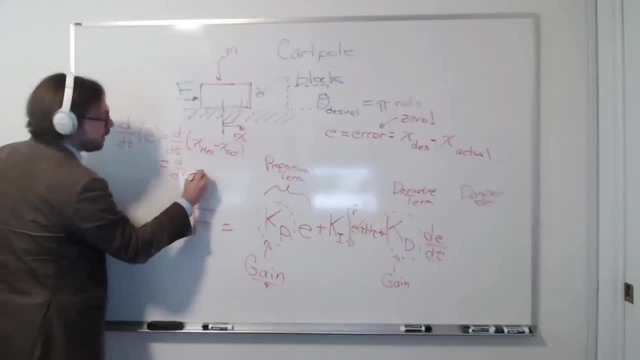 equal to taking the derivative of each of them individually and subtracting them. This is just a property of calculus. OK, So this is the rate of change of x desired And this is the rate of change. This is the rate of change of our x actual. 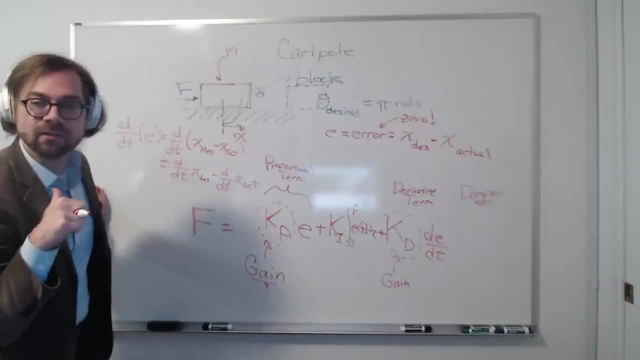 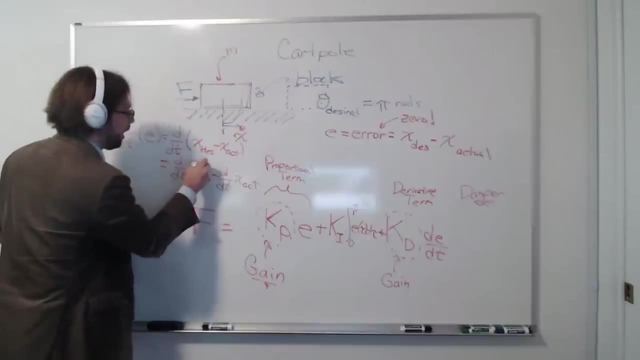 Now our x desired. who decided it? We did. Is it changing? No, It's just a constant. So we draw a little arrow that goes through it and says it goes to 0.. That's 0.. Now the rate that our actual position is changing over time. 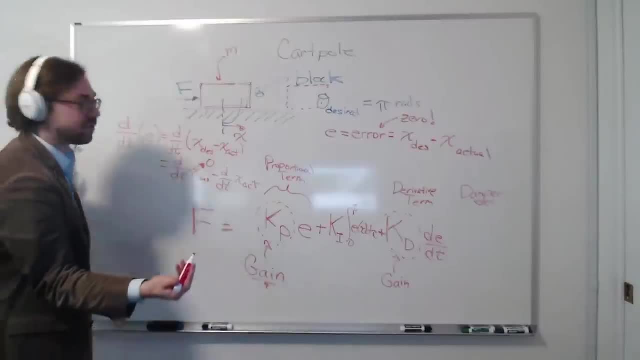 we talked about this before. That's the velocity right, That's the velocity term. So So our time derivative of error is equal to minus d dt of our actual position. so our measured velocity, And in our simulation we've measured that information. 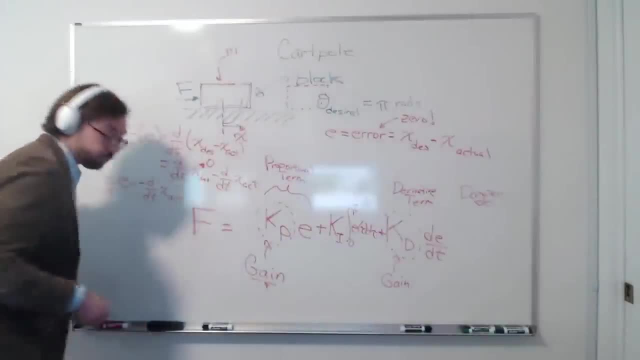 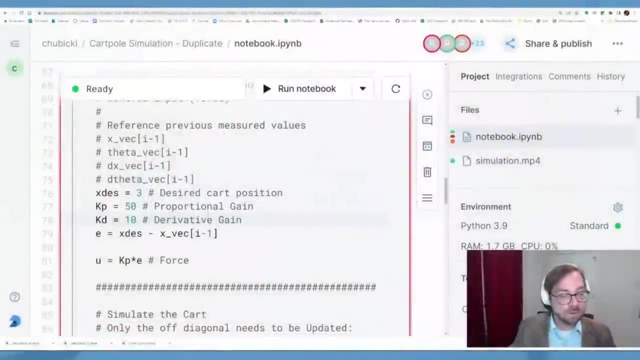 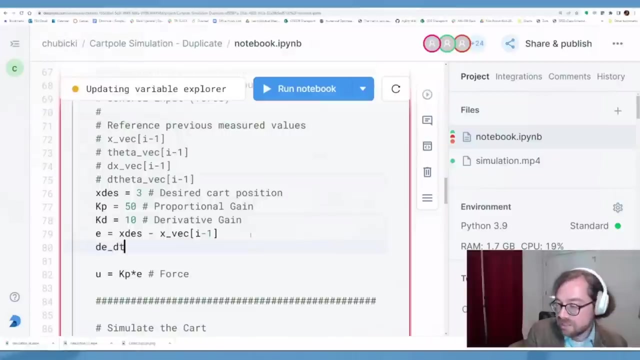 So we can use that directly. So back to the code. All right, So we're going to create de underscore dt. That's our derivative. Sometimes we would say e dot. Whenever you take a derivative with respect to time, sometimes you just put a little dot above it. 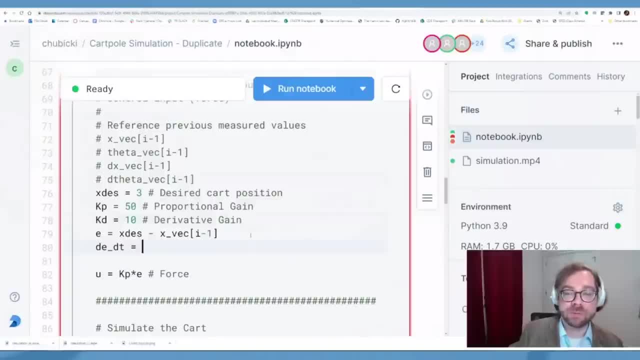 It's easier, Saves us precious marker space, marker stuff, marker magic. And so it's equal to minus the derivative. So that's it. We have that stored in dx. So right there, That's the velocity Minus that. 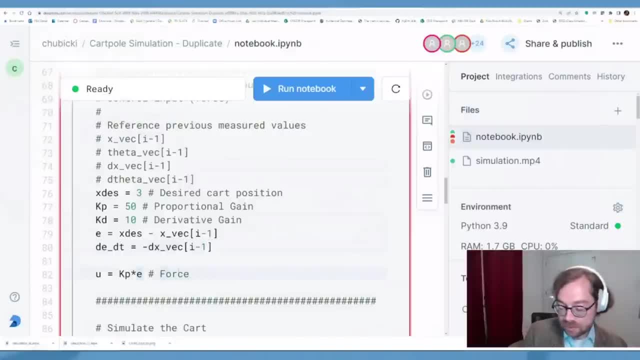 So we have d, dt. Now we're going to add together, We're going to add our d term, So we're going to say kd times, d, e, dt. See what happens. I'm just going to rerun this block of code. 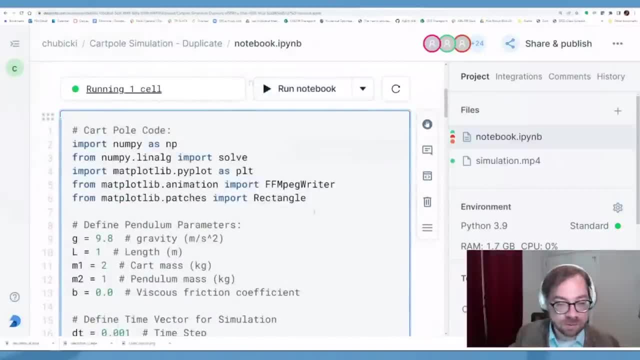 I hope I didn't screw something up. I know it'll be the first time anyone's ever screwed up a lot of code on your screen, So I don't want to be setting any records here, But I guess, if I'm going to do something on 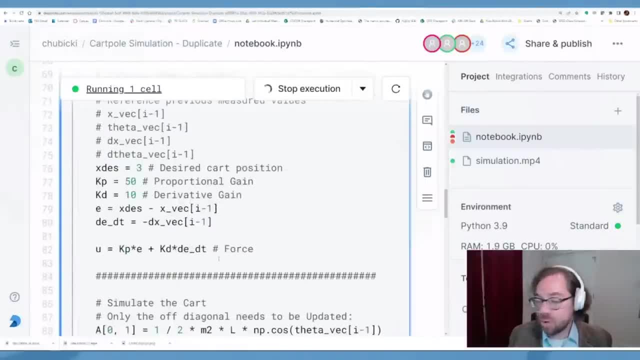 OK, But you can see how simple that controller is. as we're waiting for this to go. You might have thought a robot controller might be a bunch of if-then statements, a bunch of catches, a bunch of cases, a bunch of do this, then do that. 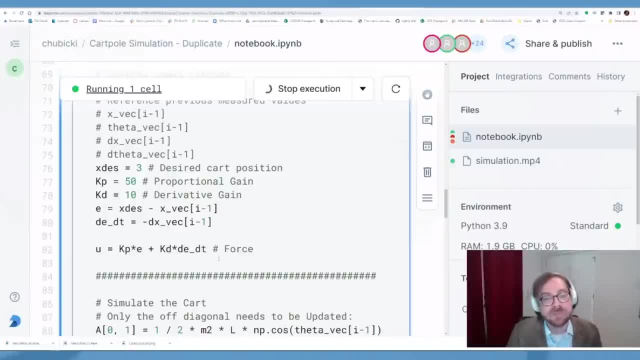 And that can be in a robot controller, But it doesn't have to be. It can be. It can be these continuous little math equations, And while this is running, I'll say that, hey, there's theoretically nothing stopping you from making these gains enormous. 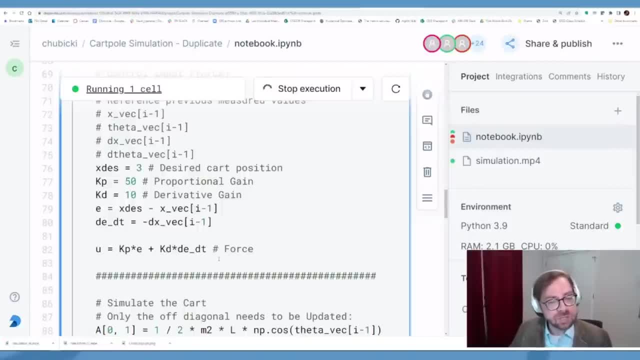 You can make them a million. OK, And in the simulation sometimes that works really well Sometimes. But on real robots the reason you don't do that: What did I screw up something? We have that d? d They're running it. 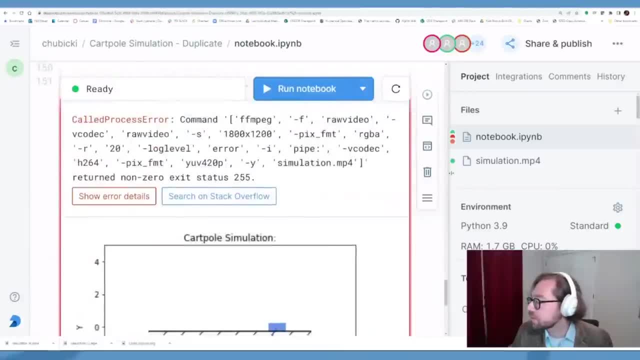 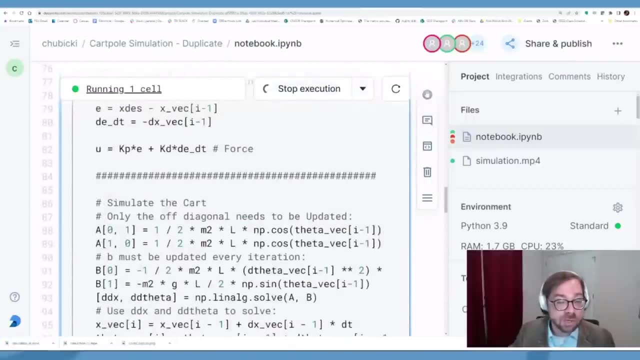 I see an error going on here. Oh, it didn't like something. Let me just give it a little bit. Run that again. So yeah, Is yours working? I see you put it in here. It's still waiting here. So you can tell if it says it's still running. 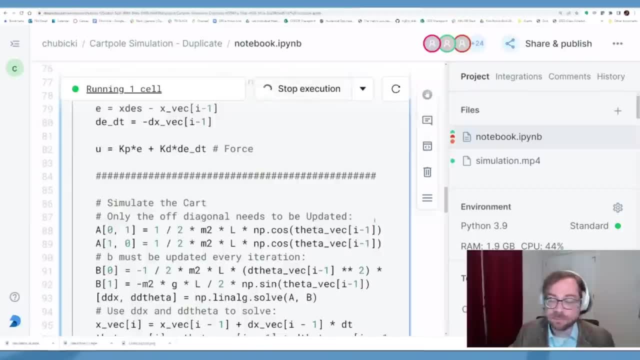 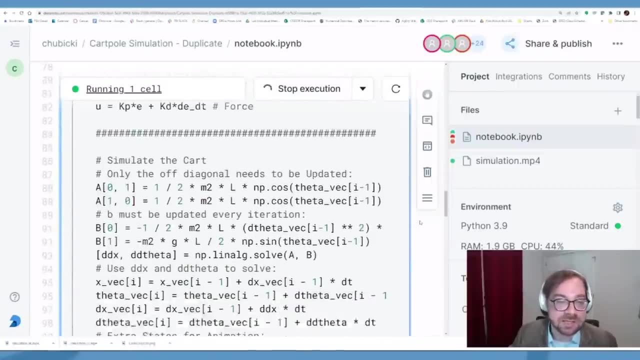 You can tell if it has a little stop, little swirly swirly wheel right And it should go through. It looks like it errored on the making of the video part, which I sure hope it didn't, because that's. 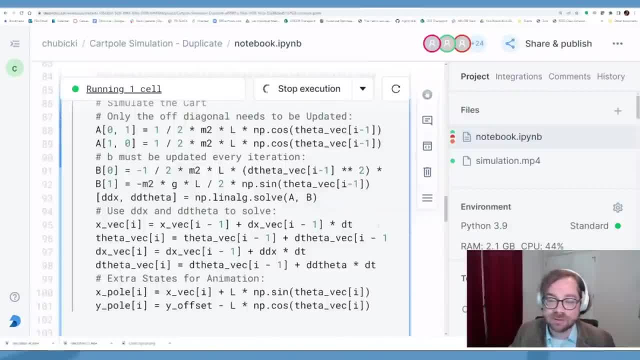 the part I'm least happy to debug and it's working fine While it's running. I had a question actually in my mind and some people are asking them. I have a good sense of how I tune these kinds of parameters. 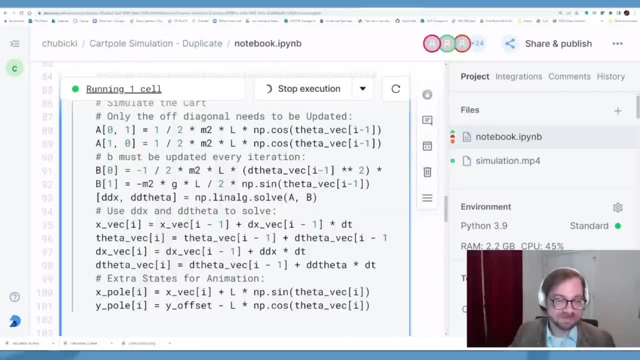 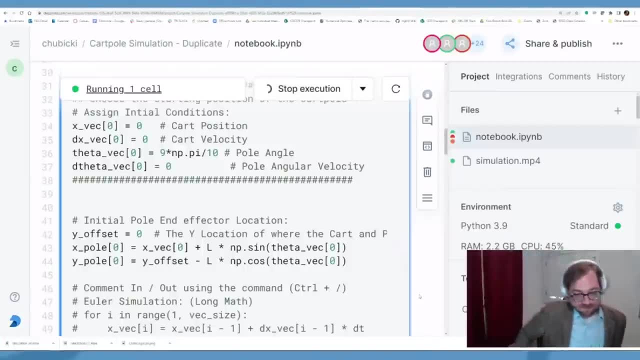 these constants in a simulation that I might be doing for a code example that goes on a website or in an animation. But you're dealing with- and maybe this is what you're getting to- real physical objects. You have it on too big. it could crash and break. 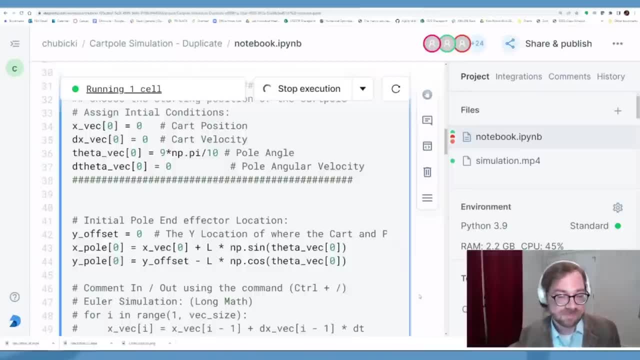 So how do you? How do you? What is the process? What is the process for tuning all of these parameters? Do you actually do a lot of simulating first on a computer before you apply it in physical reality? So the short answer is yes. 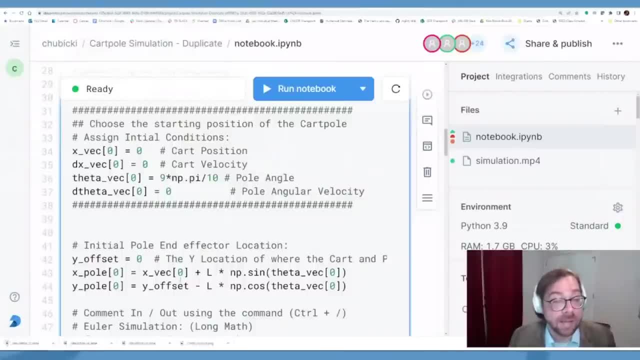 When we can, we try to build a simulation of a robot and try to get gains on it. Now we know that that simulation will be imperfect. I don't know if this has been said on your channel, but I know it's been said a million times. 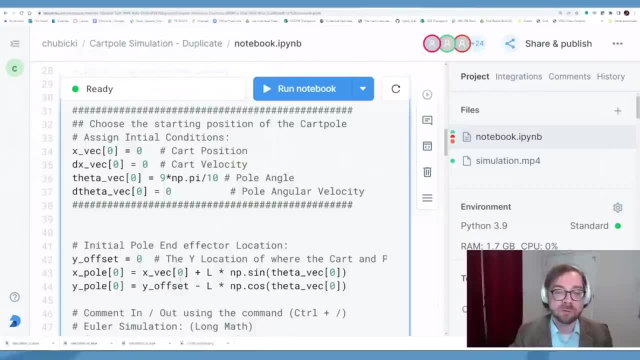 in all kinds of engineering and sciences. But all models are wrong. Some are useful- They're useful, yes, But some are useful, right. And so we'll have a simulation model and it'll tell us if we're in the right ballpark, right. 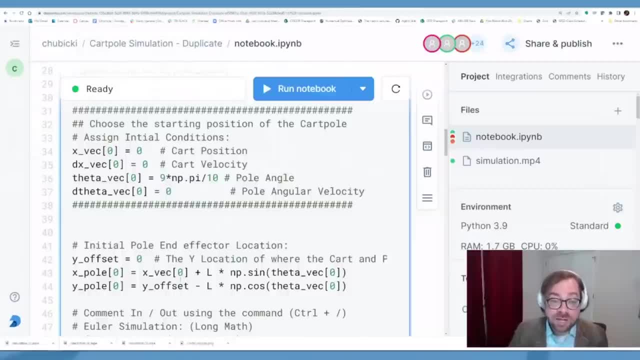 So that will give you a good first guess for the gains. But I will say- and we do this with our robots all the time- some of the robot testing is exciting when it's trying to walk. Some of it's incredibly boring where. 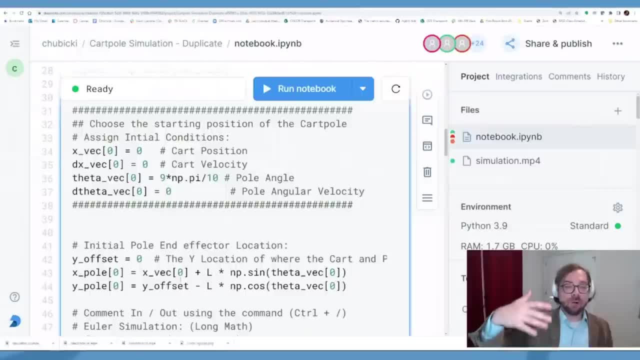 you'll have this hardworking student will go to the robot and it'll take its arm And we'll just be like try to jerk it like a little left or to the right a little bit. And what is he doing? 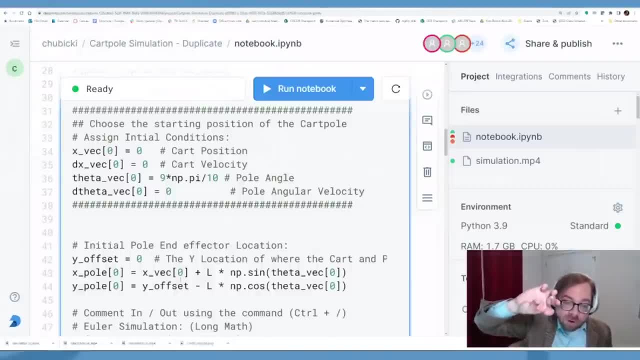 He's tuning up the gains. He's starting very, very small, so it's applying almost no force and then just almost with a knob, dialing them up to where he expects them to be good and where she might say, OK, that's good. 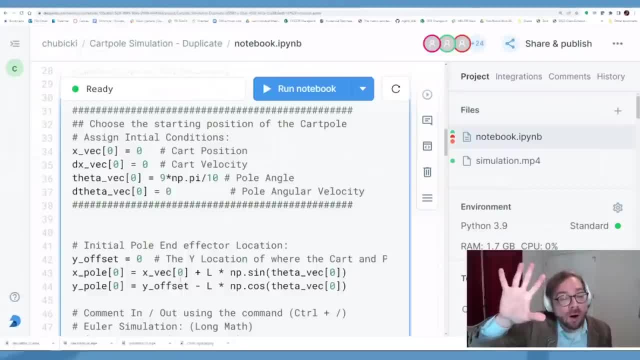 We're getting about to the range where I expect that they'll be good. But is it good? Does it need to be a little tighter? Does it need to be a little looser? So there's often in robots a little bit of manual play. 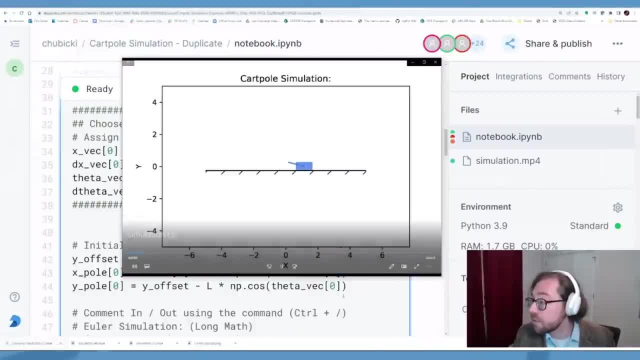 And that's fun. So let's see, Do we just run here? I just ran my simulation. Oh, look at that, Look at this, Look what's going on here. This is awesome. OK, look what it's trying to do. 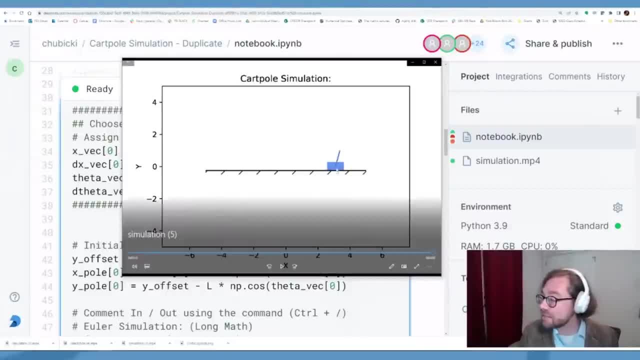 So it is trying to keep it in that position there, but it's actually got a little disturbance on it. You see that It's the pendulum being whipped around at Mach 3.. And it's still trying to hold that position, even though it's jittering around. 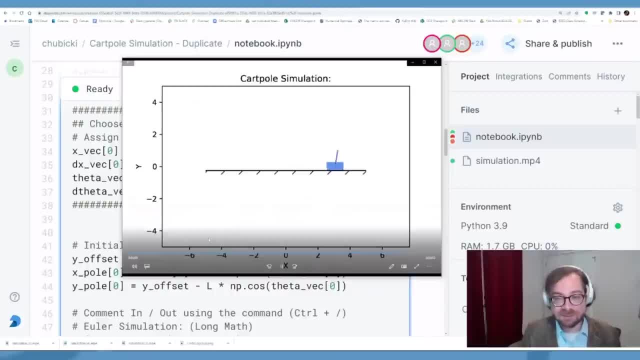 So it's trying to do its best to hold it there. So we did it. I would say we effectively did it. If we didn't have that pendulum on there, it would be almost perfect. So that's a very simple control of the cart. 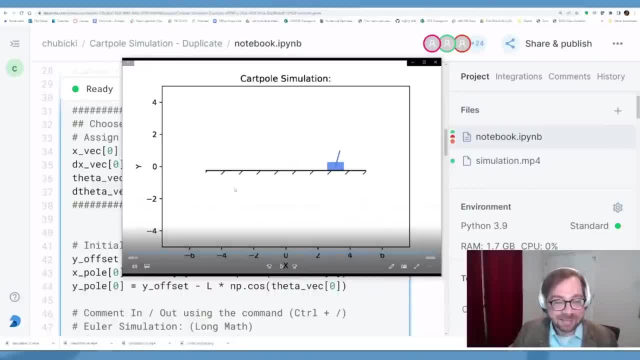 Now, what we really want to control, though, is the pendulum, And this can be a trickier proposition, or it could sometimes be a simpler proposition, where we're going to say: we want to apply a force that is proportional to the error, not of the cart. 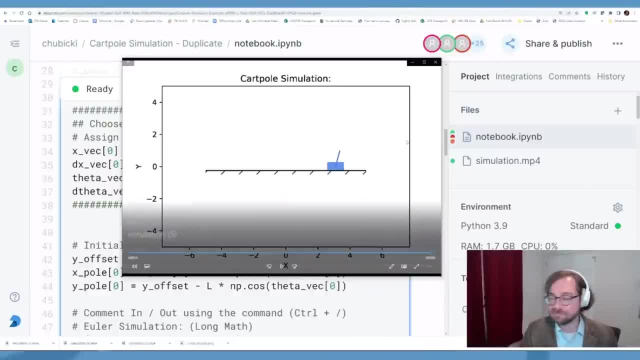 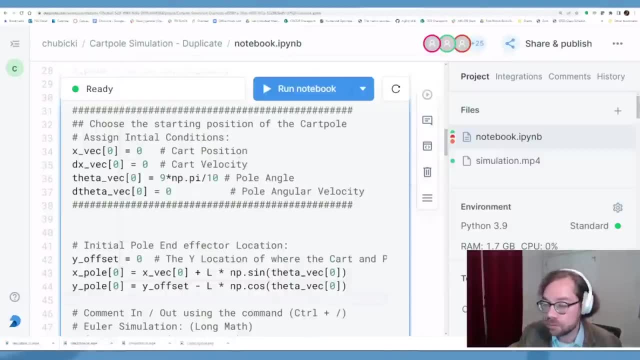 but of the pendulum and derivative gain. Sorry, can you show the tiny URL link again real quick? A couple of people were looking for it And I failed to get it into the chat. I will put it in the chat So you can find me. 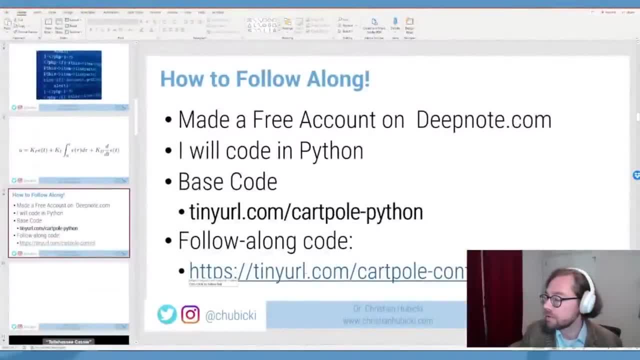 So right here, currently I'm coding on tinyurlcom slash cartpull control. The base code you can edit is at cartpulls hyphen Python. Oh, actually my face is in the way. Let me get that out of the way for you. 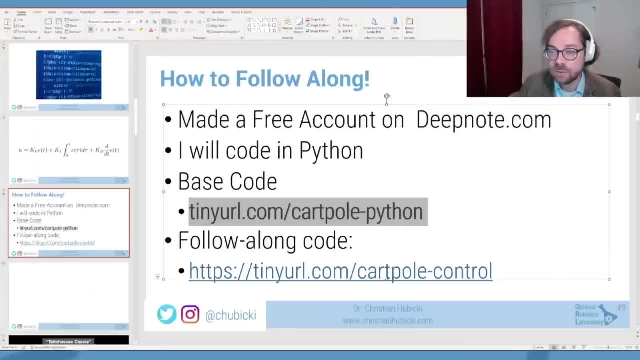 Cartpull, I'm putting them into the chat now. Yeah, So we can put that maybe in the description or whatever we want to do. These questions are great. I welcome them. Another question came up. actually I was saving some for later. 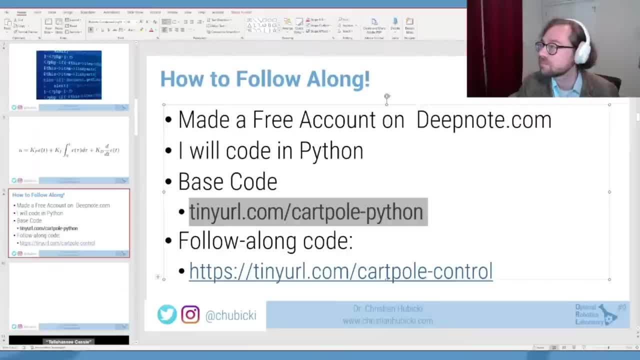 But since we took a moment to chat here for a second, a lot of my viewers, I know, are people- at least I would say viewers- but also students that I work with at NYU, in particular work with Arduino a lot. 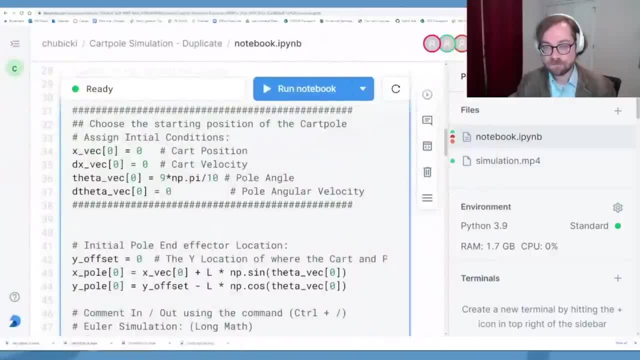 And is this a particular? is that a microcontroller that you work with at all in your lab, And is the PID controller algorithm something that could be applied to an Arduino controlling a servo motor or something like that? Yeah, So yeah, we do use Arduinos all the time in the laboratory. 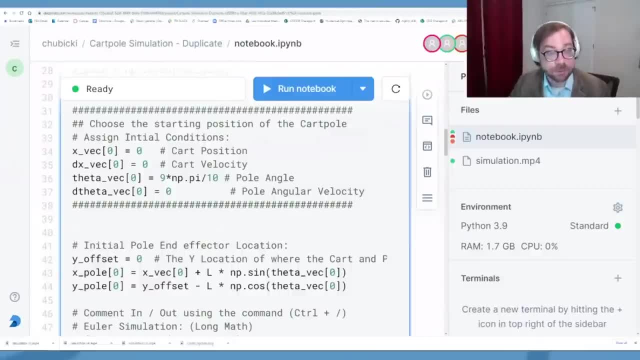 They're great for especially small robots when we are just trying to prototype something And or a proof of concept robot that might be for a scientific test. I remember I had to make a. maybe this is a story that would tie a few things together. 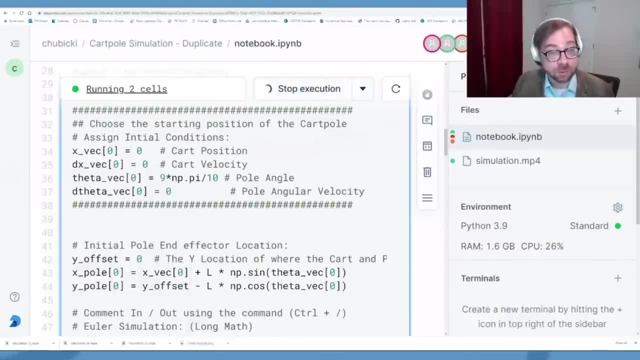 I remember when I was on Survivor, as you were mentioning, there was a challenge where it went on for hours, So I had nothing to do but talk, And one of the things: if you watch the episode of this, if you're watching the show, you can't miss this challenge. 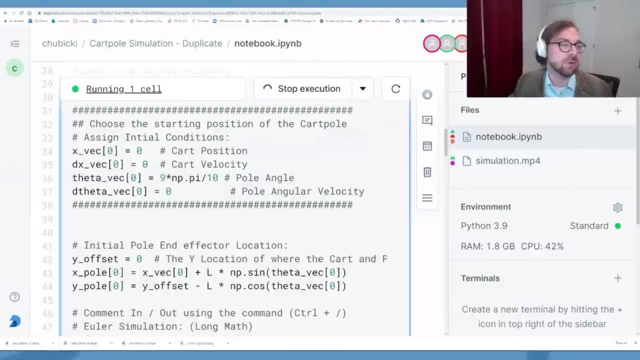 At least it'd be hard to miss this challenge. Just if you're watching, you'll get it. You'll know which one I'm talking about. And I mentioned that I had to design a plant root robot, a robot that was basically a growing plant. 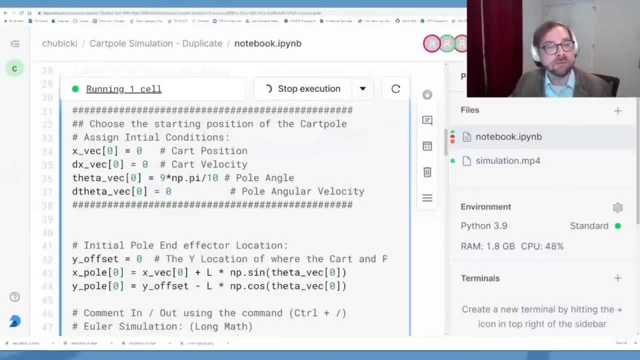 root that would move in the soil, And this was a scientific study for trying to determine what strategies for how roots grow would be best for penetrating through different materials, And it was specifically in collaboration with a group at Duke that does genetic knockout studies of plants. 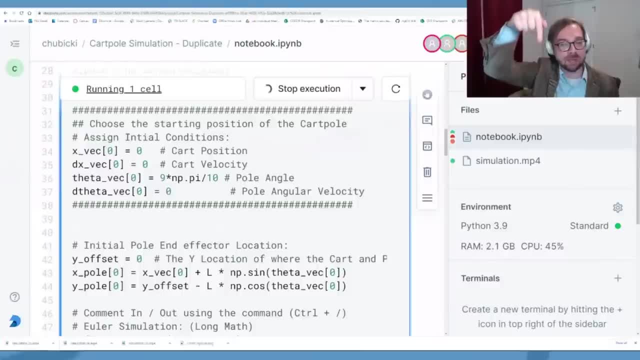 And notice that there are some ways that plants grow, that they grow straight, and sometimes the root little wiggles at the end And there's that wiggle, And that wiggle was something that showed up in plants that they could knock out and try with real plants. 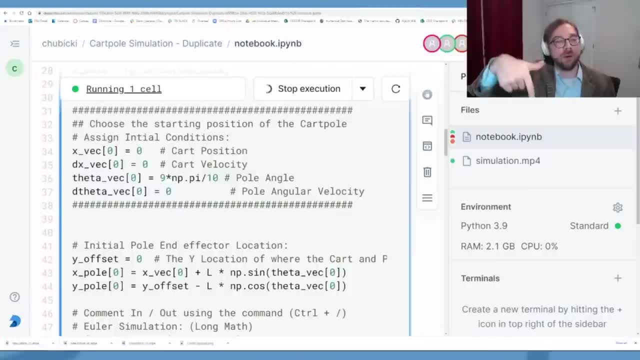 to see if it's better at growing. But they wanted to also try it with a robot, And so I made a in this motion. this wiggle is called circumnutation- circumnutation, And so we used our Arduino to control the wiggle. 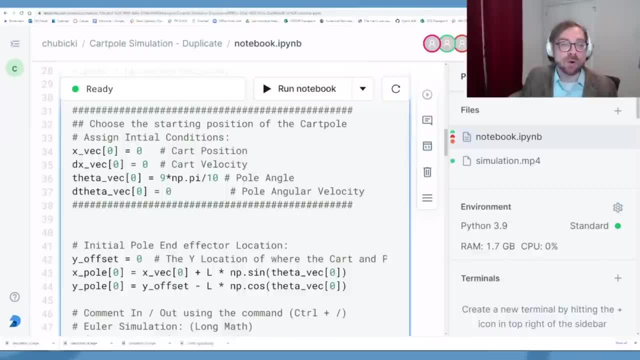 The wiggle of the plant, And there we use something called a stepper motor. And a stepper motor, you can just tell it to click one wheel at a time. It'll just click to a position, And so you don't need a PID controller, just. 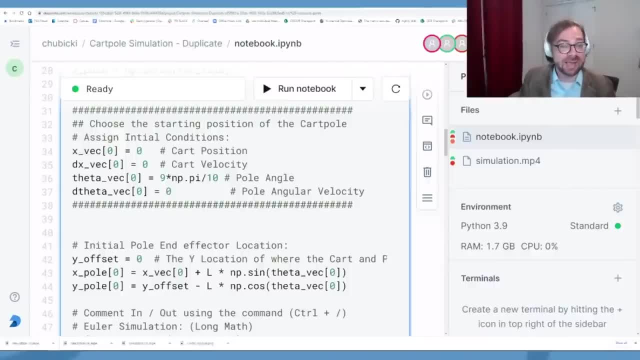 to do that, to click to a position. However, if you have any kind of motor where you're applying current or a torque or a voltage that you control up or down, PID control is great for that. But the project I was talking about during that challenge, 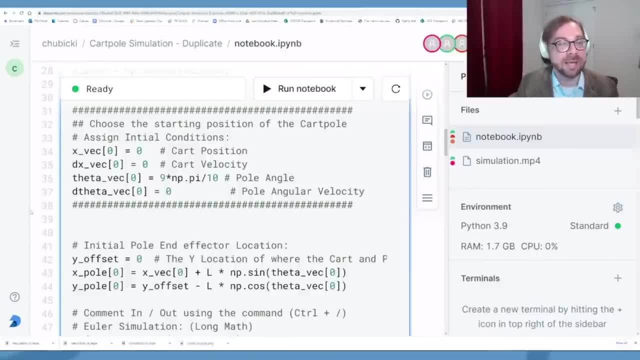 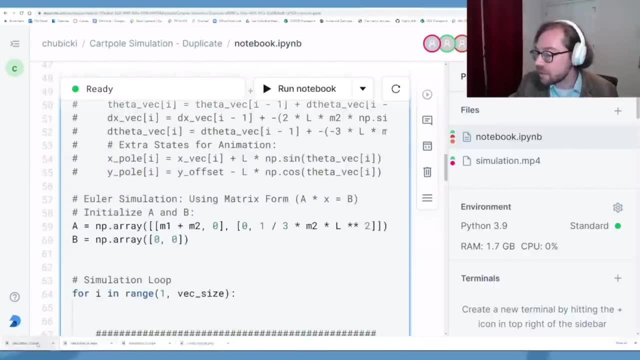 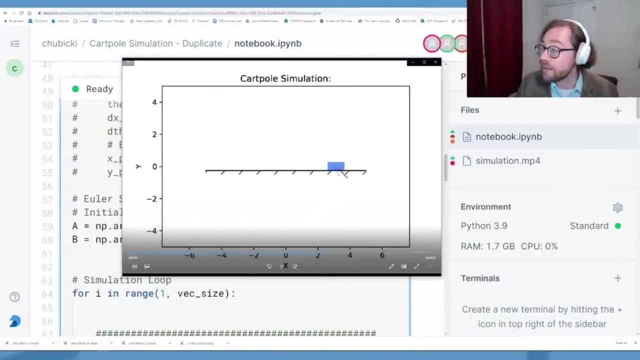 was using an Arduino to control the circummutating plant robot. That's what. that was, OK. So yeah, All right, So it looks like that. so that ran And it managed to hold that position at roughly 3.. I bet if we didn't have, if we could turn off the pendulum. 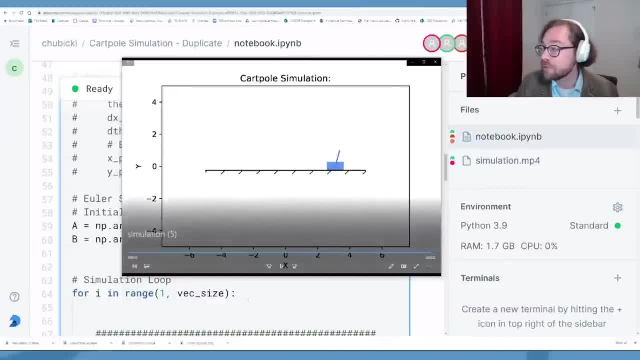 by making it massless or very, very close to massless. if you went up to the top, if you went to the top of the code and changed the pendulum, If you changed the pendulum mass to like 0.001,. 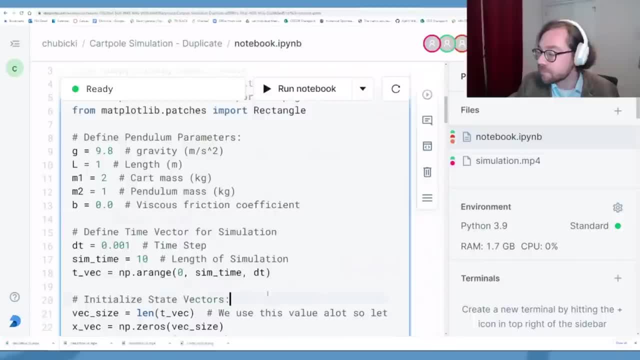 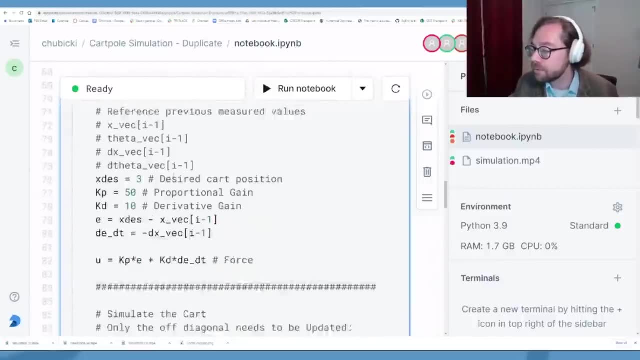 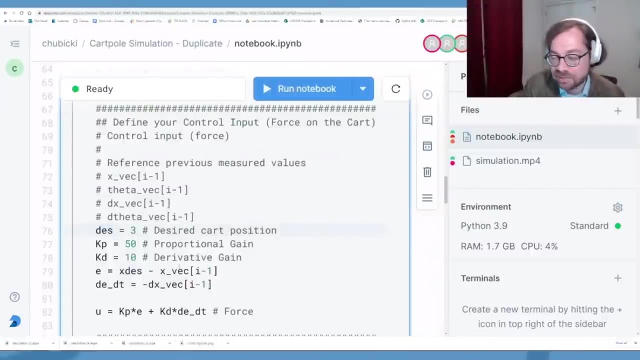 it would probably do extremely well. OK, So now let's try to control the actual angle of the pole. All right, So let's go. well, maybe we can make this super easy. So, instead of having an x desired, let's just have a theta desired: an angle. 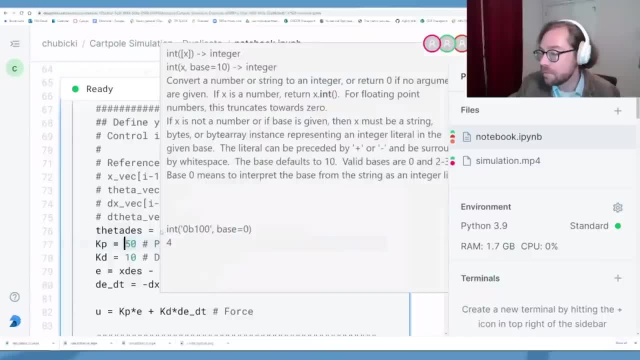 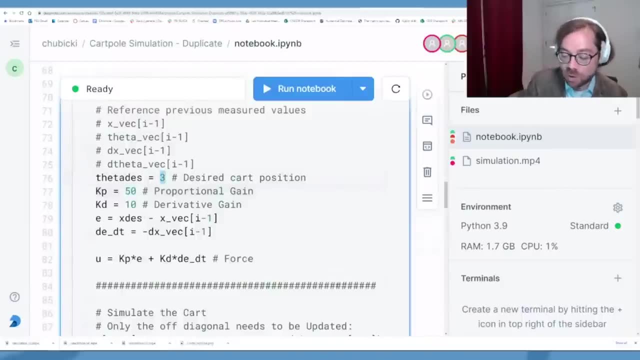 So theta des? all right, And we're going to make that theta darn. it teleported me in the code, All right, So theta des. So where we want our desired theta to be, pi. So down to 0, up is half a rotation. 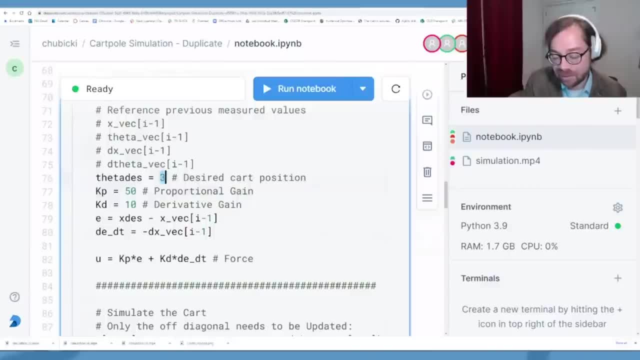 Half of 2 pi is pi. So in Python you have to say nppi, because the numpy package is the one that tells you what pi is. OK, So all right, And now we're going to come up. so now we just say our error. 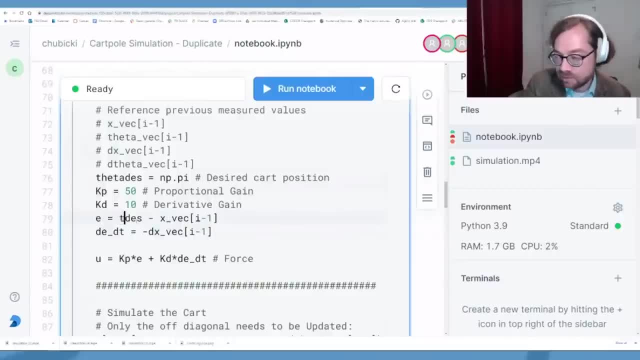 now, instead of being xdes minus xvec, it's theta des. All right, So theta des minus theta vec. and dedt, instead of being minus dxvec, it's minus d theta vec, And we'll see how this works. 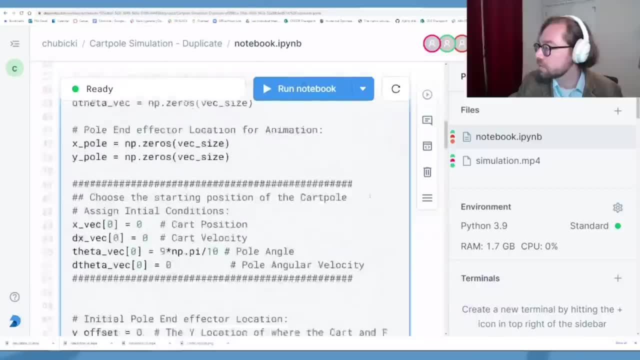 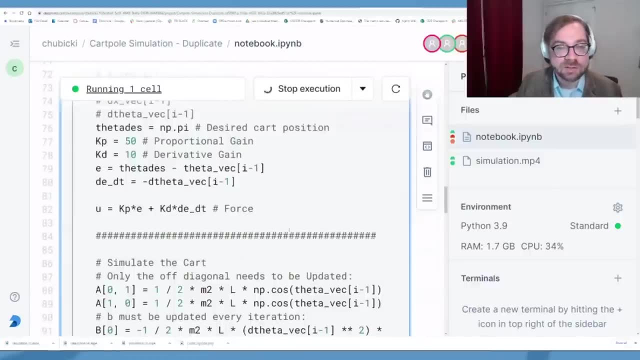 We'll see how this goes. I'm just going to run this block of the code. I don't need to scroll up, I can just click that little arrow over there. We'll see how this works. I haven't tried this set of games before. 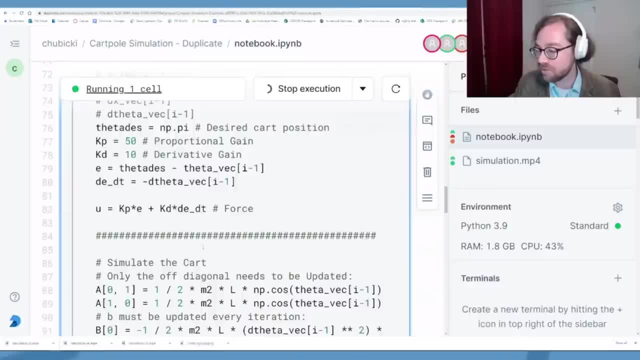 so your guess is as good as mine as to how this goes. But yeah And you sorry, I was answering questions in the chat while I was sort of half listening to you, so I was curious. So you had to change both obviously. 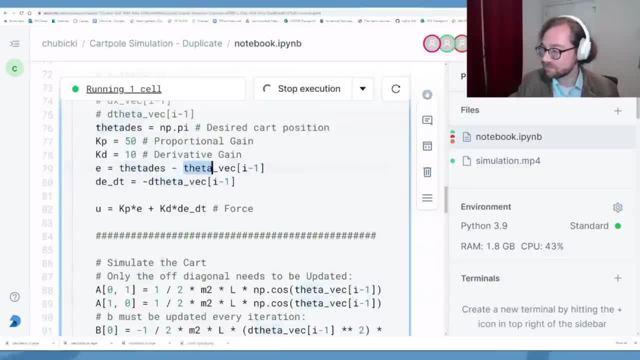 you're changing the desired and the error to calculating based on the angle, but now you're also looking at the angular velocity of the pendulum, no longer the velocity of the cart itself. So the cart's position plays no role anymore. its position or velocity. 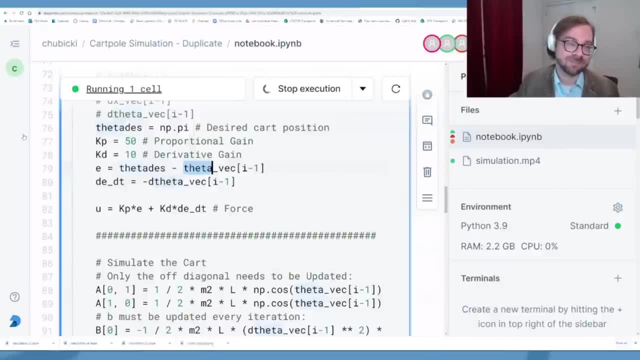 You're only looking at the, you're sensing basically just the movement of the pendulum. That's exactly right, Daniel, And so yeah, so we've now changed it. so we're just caring about that thing staying up, We don't care where the cart goes. 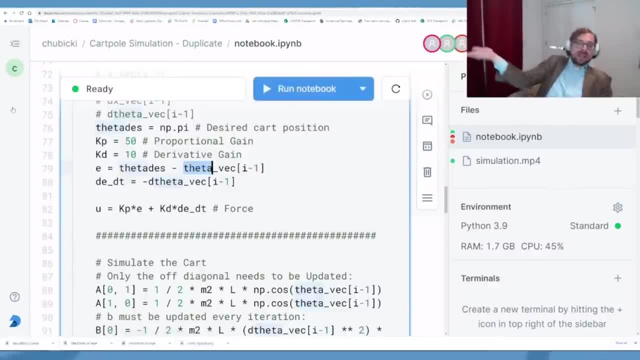 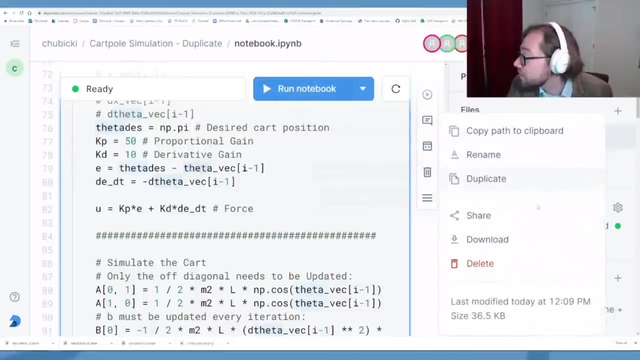 It's like if we are balancing a rod on our hand. we can move our hand all over as long as the thing stays up. So all right, it looks like it ran. This time it did an error in that weird way that I can't explain the first time that's happened. 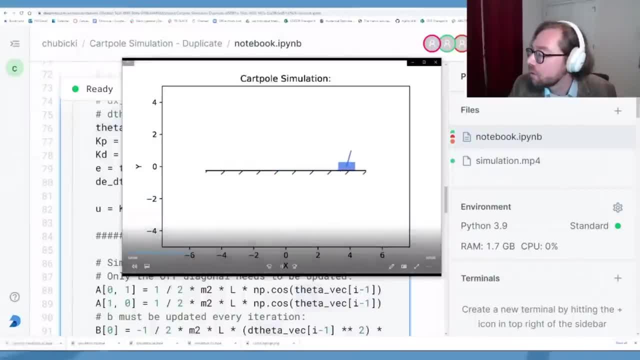 Let's see, all right, let's see what happened when it ran. Oh, it's trying to catch up. There we go. It really doesn't care where it's going. It really doesn't care, All right, So yeah. so hey, it didn't fall down. 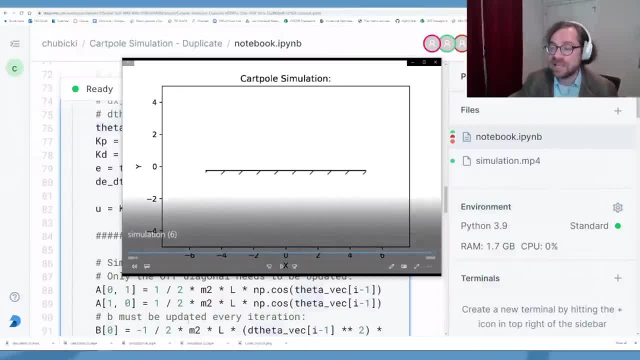 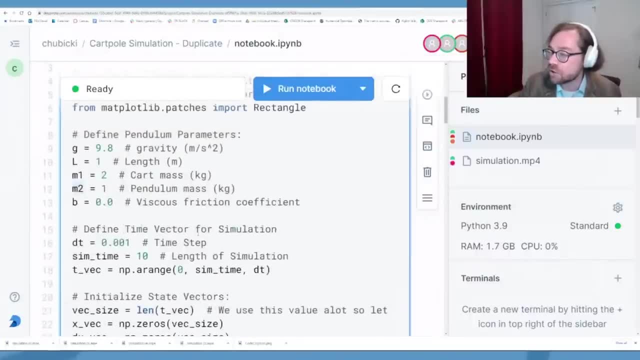 at least as far as we knew right. So we can mess with the gains a bit more And we can also start where let's have the cart start a little bit closer to the top, So maybe it doesn't have to make as much extreme maneuver. 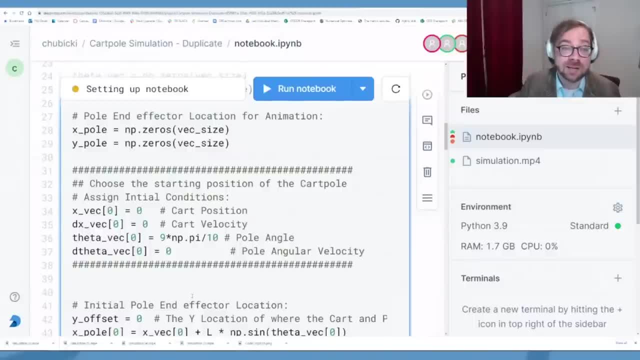 while we're trying it out. And this is a good strategy: if you're trying to test out a controller and you want to know if you just got it right at all, try to get it start off really close to where you want to go and see if it'll get it there. 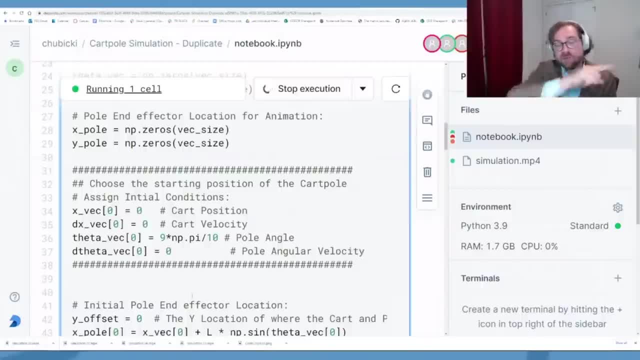 And so, and then if it goes wild, any, if it flails around anyway, you know you probably are doing something wrong. 50% chance it's a sign error somewhere, You have a negative where you shouldn't. So I'm going to make: oh, did I rerun it? 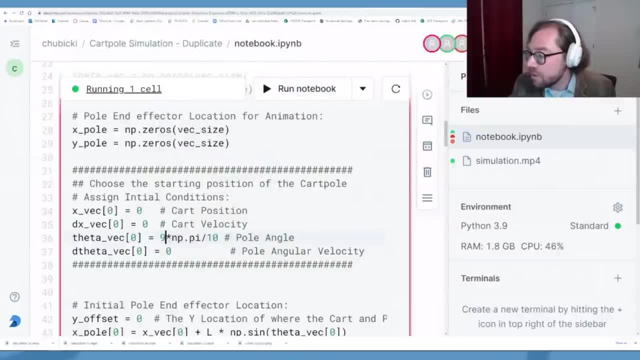 Okay, I'm going to stop execution. didn't mean to rerun it, So I'm going to change instead of not. I'm going to go up to my initial starting position where, instead of having nine over 10 pi, I'm going to change it to 9.5 out of 10 pi. 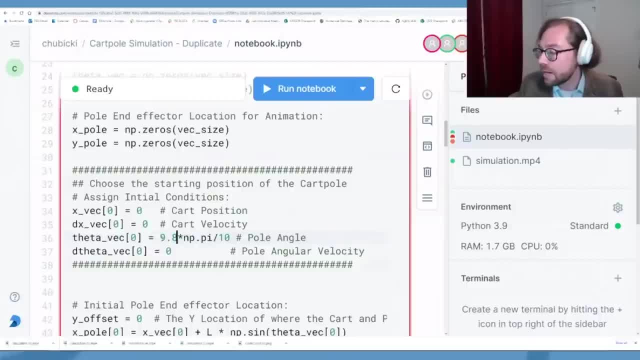 Okay, so pretty close. we can even go 9.8 out of 10 pi, just to see if it works. So I'll rerun this code here. So, and what we should expect, at least what I'll expect to happen, 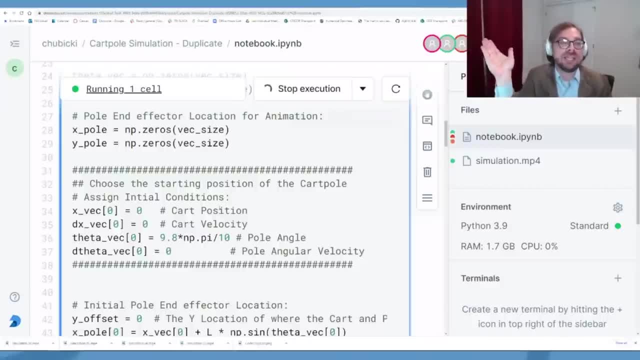 is that it's keeping the system pretty close to up. It keeps it from going down. Now, if it runs off to the distance, what I'm going to first try to do is increase my P gain, Because what I want the system to do 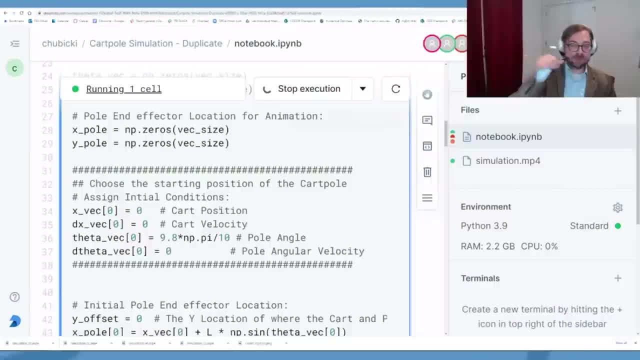 is to push harder on the cart when there's an error, So that way it might push it past where the pendulum is And so it might start going back. but we might have to play around with that a little bit. But I will point out, the thing hasn't fallen down yet. 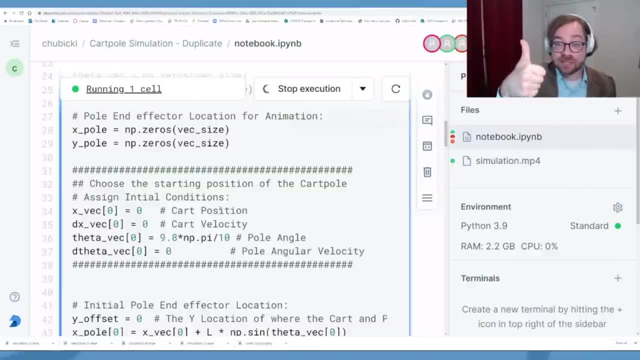 So good, that's not too bad for games. we just we just plucked out of nowhere. you just need infinite space. yeah, it's infinite space, right, yeah and so. so this will be the game and the one thing i think will be fun when you're doing the. 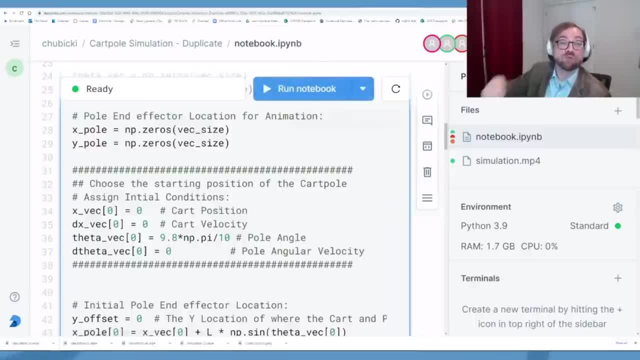 the javascript version of this that we have the ability to rapidly try new things? yeah, no, it's. this is kind of i mean, uh, i am learning so much and fascinated and just enjoying this so much, but the the amount of time between changing a variable and seeing the result is is very painful to me. 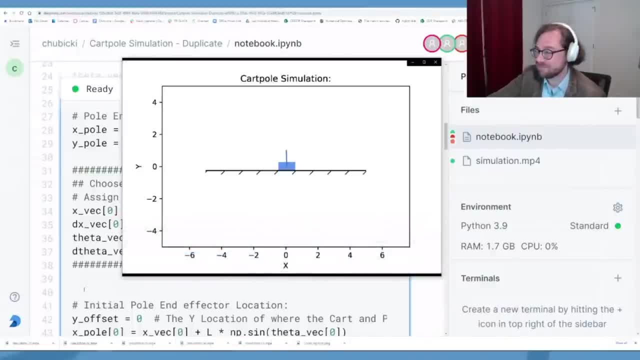 uh, because that that's sort of, and i'm so. that's why i'm so excited for this collaboration, because i think there's some. well, javascript and the browser obviously have a lot of limitations in terms of scientific computing- um to be able to quickly demonstrate and change. you know, we 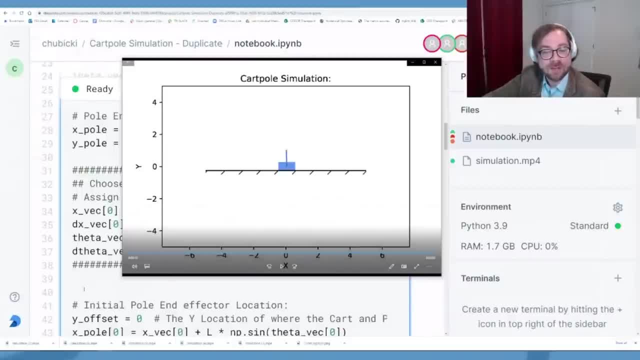 could interactively change the game, with a slider, for example, and have it continue to run. so anyway, we'll get there. no, it's fine, and i'll point out that. hey, look there, you know, managed to balance the pendulum. it was a little bit of an error and managed to actually. yeah, looks like i managed to. 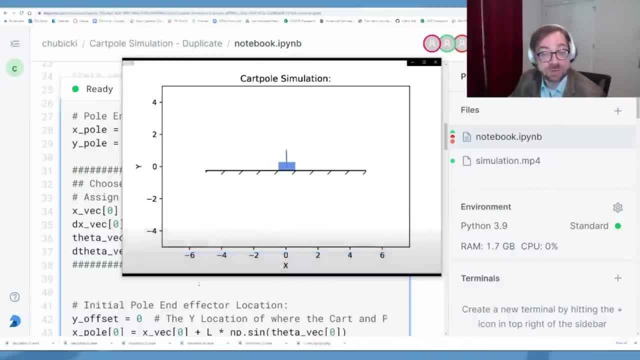 stick it there. yeah, so so it balanced it and so we, at least those gains at least worked in principle for the small error. now we can tune them up, um, and and in in the, in the, in javascript, and uh, that's maybe will be our next step, i think. but before we go there, i'll talk just a little bit about the integral term. 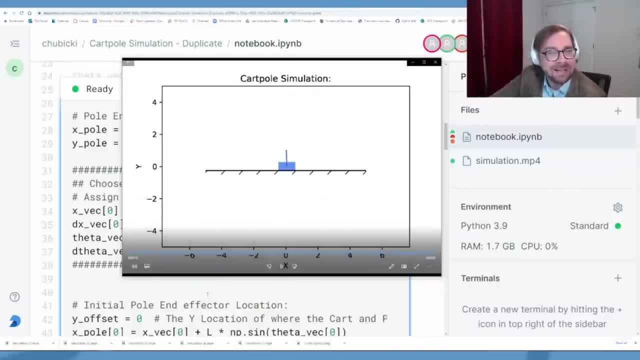 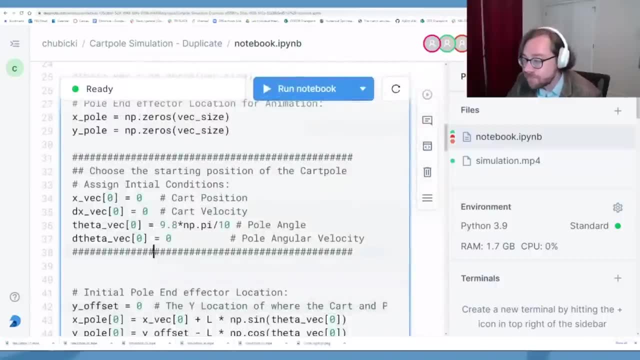 the integral term, just because sometimes people are like: how do you, how do you do the integral? you know, you know dodgy, kibiki, uh, and there's, that's often the one that that gets people just a little bit confused. okay and so, and justifiably, because it's a little bit more complicated, because you actually have to start. 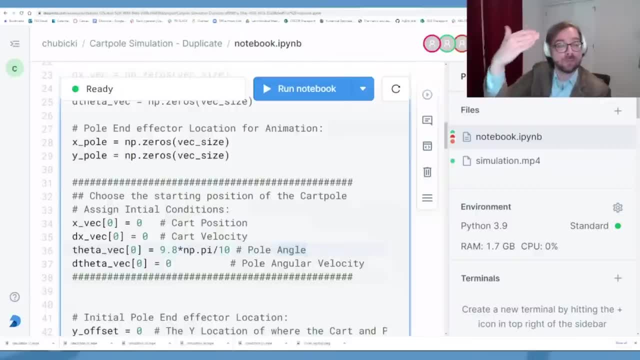 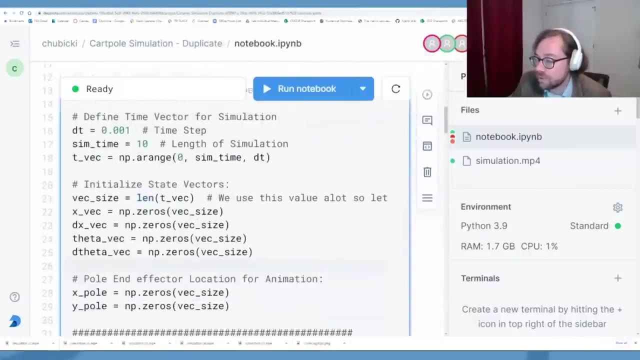 keeping track of how you're adding up, over time, this error. so you need some kind of variable in which you are storing this added up error. so let's do that and i'll- and i'll- add this to our um. i'm going to actually make some changes to the base code in order to do that. 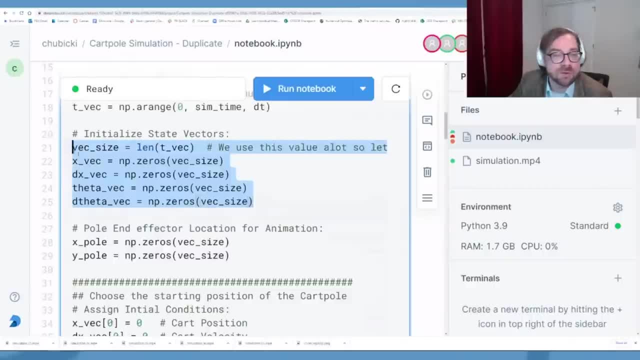 so what i'm initially setting up here are what i call sort of state vectors, and these are these. these are vectors, just lists of point of, of numbers that are storing the position over time, the velocity over time of all of the, of all the things that are moving around. 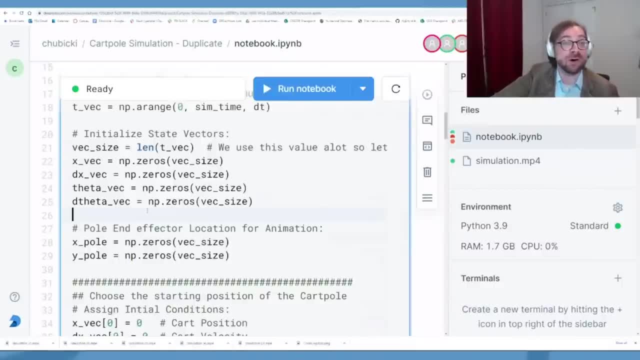 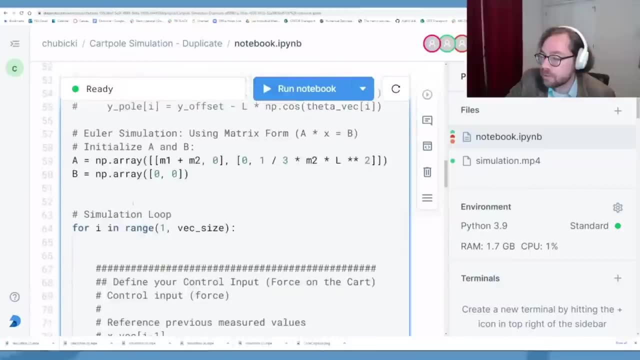 we're just going to add another one for the integral of our error. okay, so i i would say you can, you know, we can even simplify this a little bit more. so we're going to say, right before the simulation loop, we're going to say our initial. 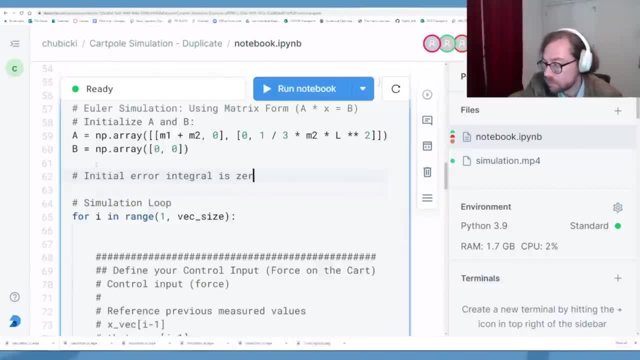 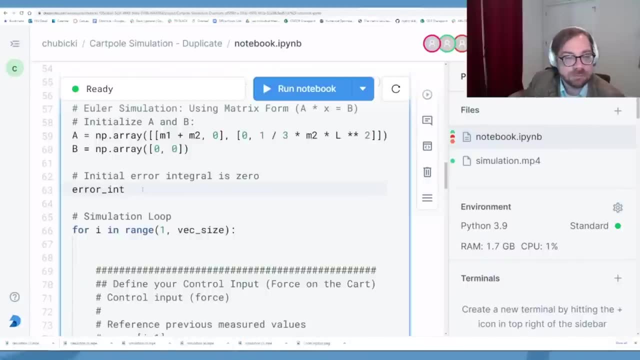 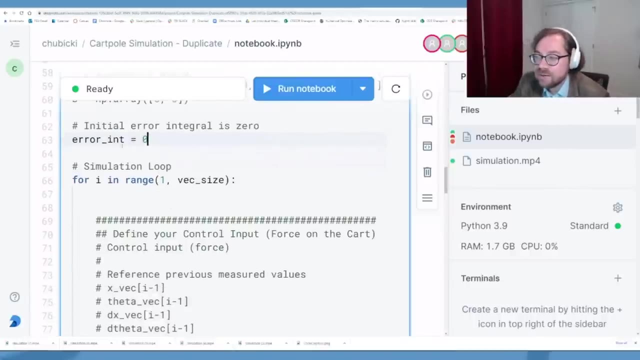 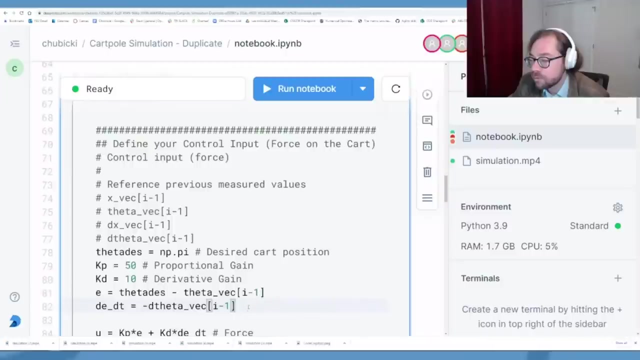 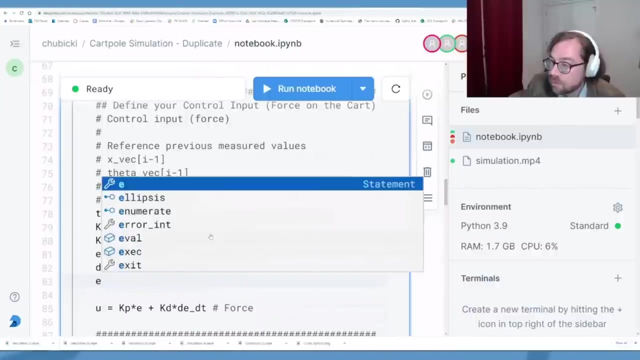 error integral is zero. create a variable called error int- and this is just above the simulation loop. that's where we're doing this- right equal to zero. and then, inside the loop we're going to create, we're going to update our error int. what do we call it? error int? 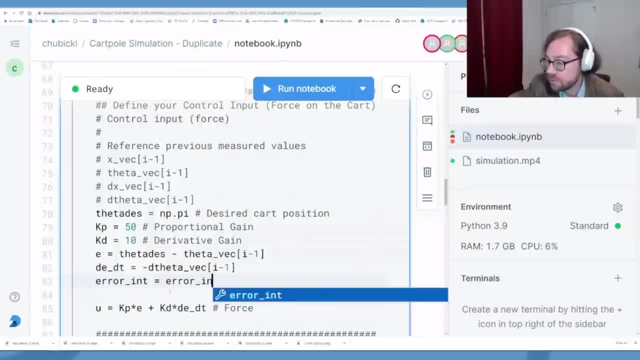 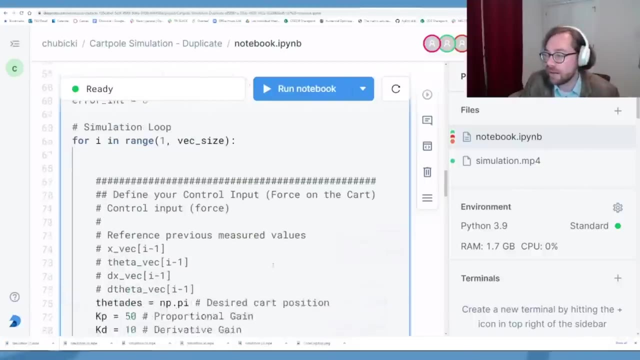 as being equal to the previous error int plus recurrent error times. you remember that little time step that we talked about in the simulation, for how this tiny little step of time we're going to multiply it by that, i believe, is dt. i'm just going to check and make sure that's the right variable thing: dt. so a thousandth of a. 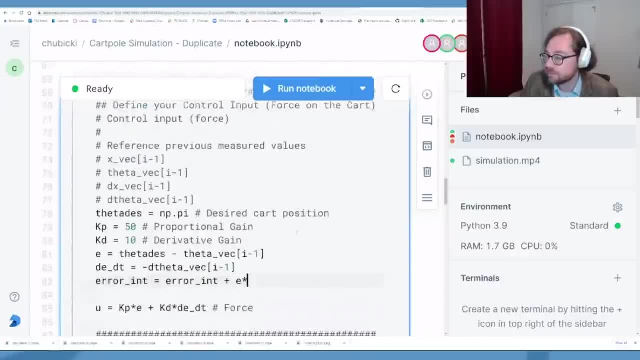 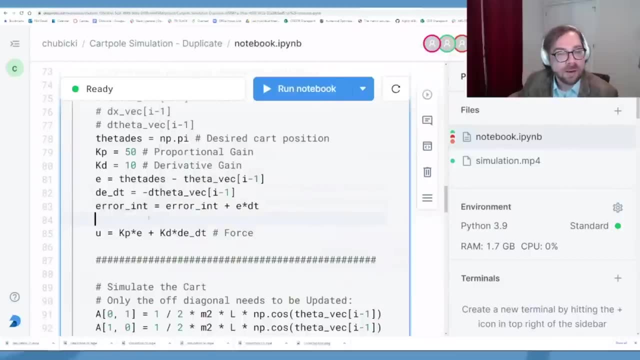 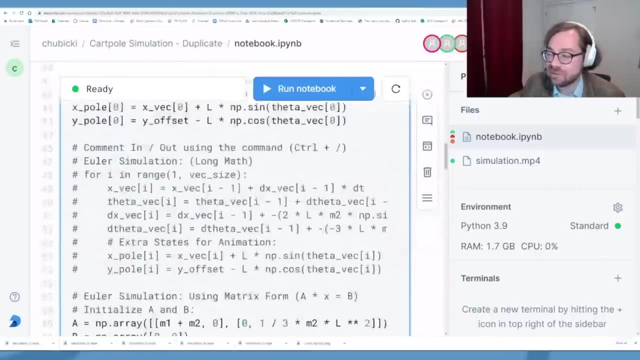 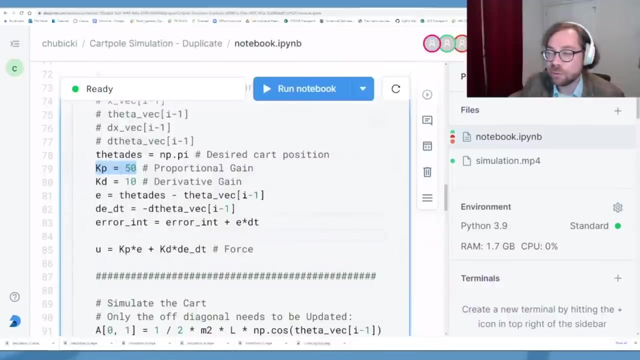 second this tiny little period of time. dt. there we go. there. you have your error integral. now what else do we need to add an integral term to this controller? well, we have a k. we have- goodness teleported me again. you have. you have an error. you have a. you have a gain for your proportional term. gain for your. 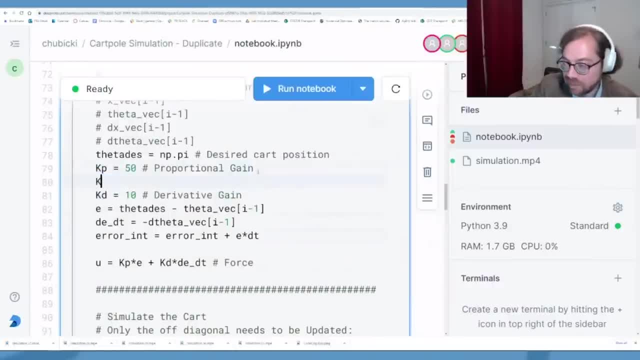 derivative term. you need a gain for your integral term. so ki, and we'll make it one. this is often my smallest term, my smallest game when i'm doing pid control. if i, if and when i want to use it, it's the inter integral game which i have a disorder in which i can only spell it integral. 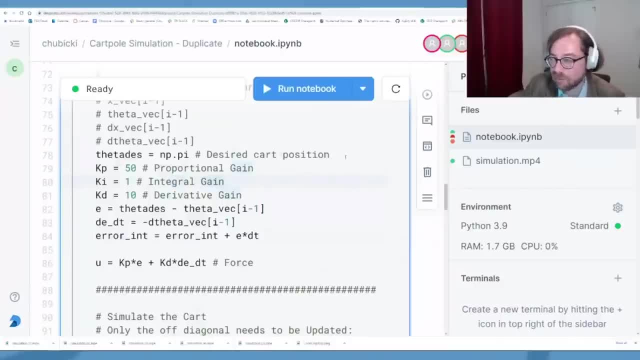 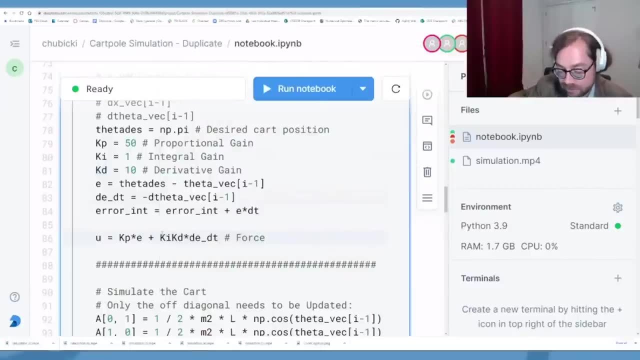 every time integral. every time i spell it wrong. so integral game. so then we add this term, so they say: ki times error, integral. done, that's our integral game. okay, so now we have p, i, d, all three components, and if we decide we don't need, i guess what we can do. 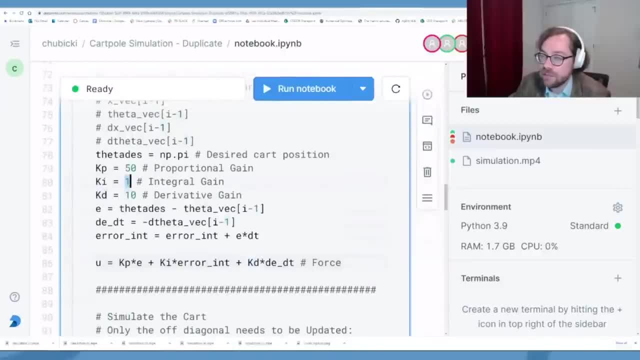 we can teleport away and then come back and then do what i was going to do in just a second. we can make the integral term zero doesn't exist, turn it off. so i'll do one quick run of this, and i think that that is the core of what we need to start doing. 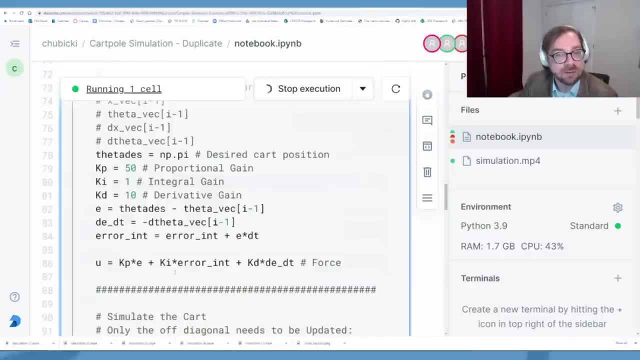 this job script. yeah, i've got a few questions that i'll that, that i've been noting down once once. well, i guess, like while it's running, maybe i'll ask you some of them. yeah, perfect, um somebody. i have no idea what this means. when somebody asks um about if whether this relates to something called. 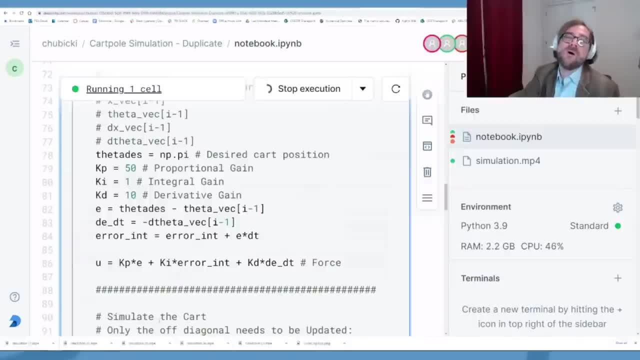 an lqr regulator. is that something you recognize? is that a term you recognize? it absolutely? is i, we got we- we have some ringers in in the chat today- the lqr regulator, so, um, so the the short answer is yes, and i mentioned before that you know we're picking gains right like, and there are these. 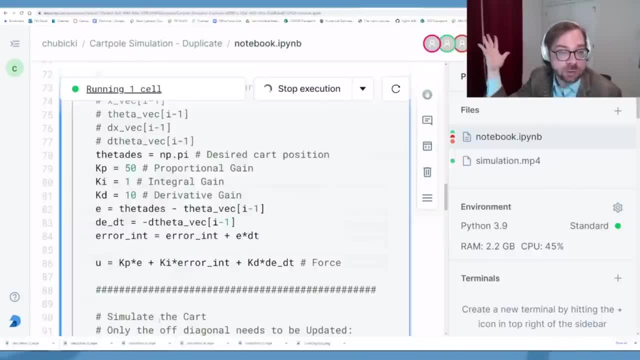 these rules of thumb we're using, but there's an entire mathematics to choosing gains more intelligently. so that way- i mean that way theoretically- you don't have to get guess and check like with a robot. i can do a little bit of guess and check. uh, but what if i was doing? 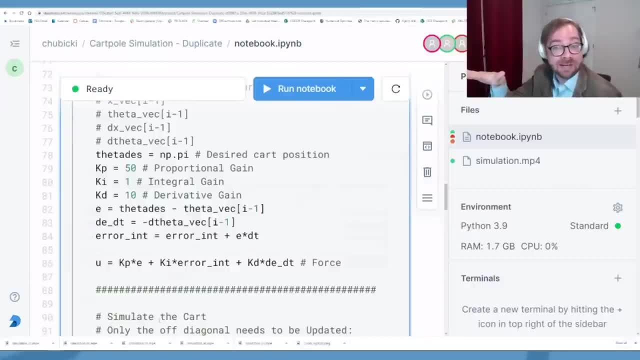 gains for a power plant. uh, and you know of sure being how much i'm going to open the valve that's going toaga. i'm just going to save. fuck these two, put them on a stack and just use that. uh, and i know i'm going to use and coming here and doing stuff from every one end, but i afraid that i can do something like that. well, i feel like i'm abandoning myself if i've got CPUs on every�E. 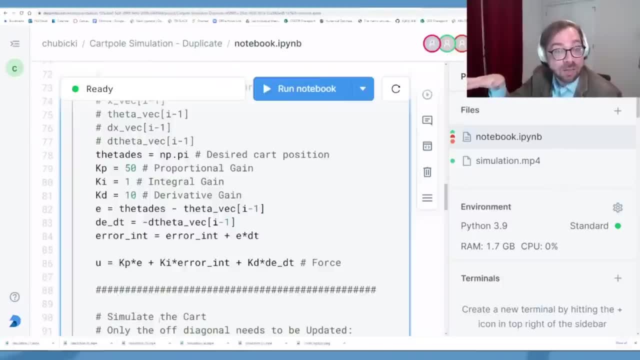 to the coolant. you know you don't want to guess and check on that. however, if you have the equations of motion, the system we'll call the system dynamics of your system. you can use this, use control theory, to come up with the gains, and one of the, which is called lqr, is one method for doing. 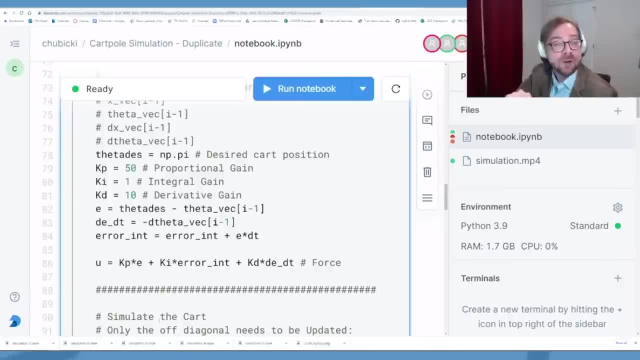 that that's a method of what we call optimal control, where we, instead of defining, um, just where we want to go, we define what we call a cost function, which we say, oh that where we define how much it costs to operate our controller. and so that could be saying that you know, we have a cost. 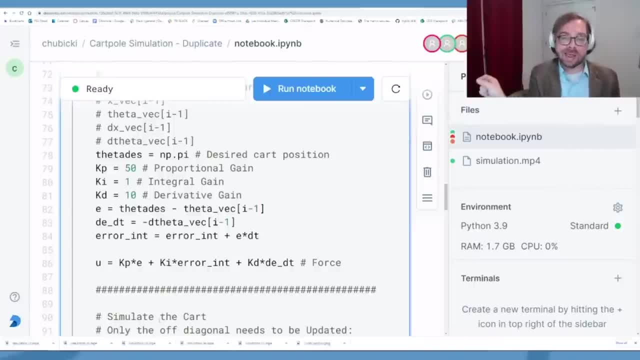 that penalizes how far we are away from where we want to be, but also penalizes how much effort we get there, and this is the proportion that we want to care about both. and, theoretically, lqr, if you run this system, if you baik, this process, will give you the optimal best gains to minimize that cost, and that's what lqr does. so 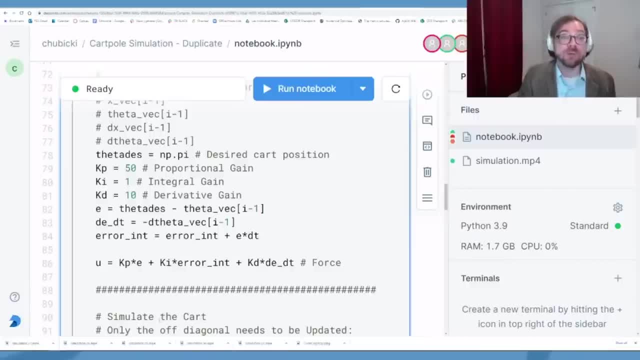 it will give you the pid. that's absolutely best, yeah, but we would take. yes, but it requires us to do a little bit more math and to take the system, the, the math that's of this pendulum on a cart and do some a little bit of you know, trickiness with it. yeah, it's interesting one of the things when 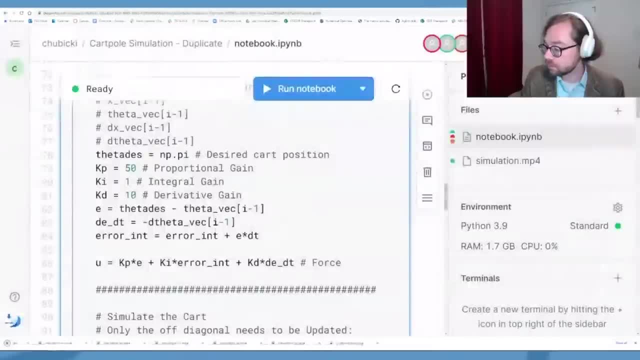 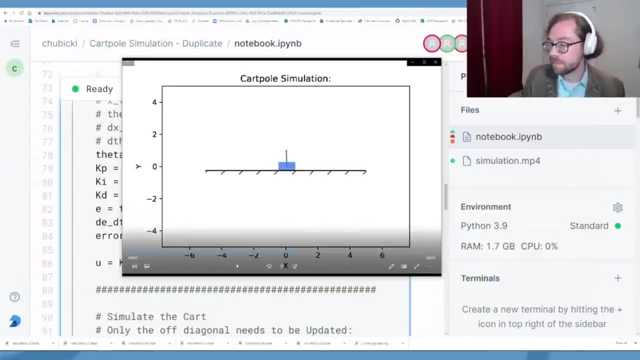 i was poking around looking at, uh, this topic, i saw a paper about using genetic algorithms to evolve the optimal um gains for pid. so i think there's lots of interesting methodologies you could use to sort of like tune those parameters. yes, and they all have strengths and weaknesses. 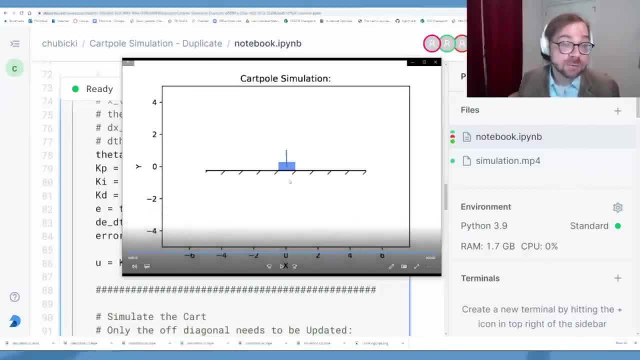 so these, the lqr, uh, as it stands for linear quadratic regulator, it's a, it's a, it's a, it's what it stands for. but if we break down what that is, that first word, linear, says that your system should be what we call a linear system. 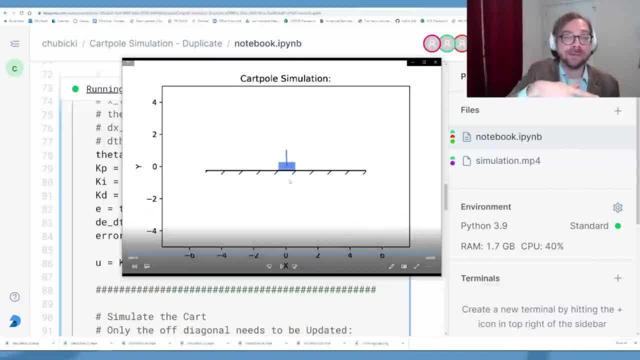 meaning that you put in a little bit, you get out a little bit. you put in a lot more, you get out a lot more. um, but the pendulum part of this is not a linear system. okay, it's not linear because, um, if i put in a little bit of effort when the pendulum's at the bottom, it'll move a little. 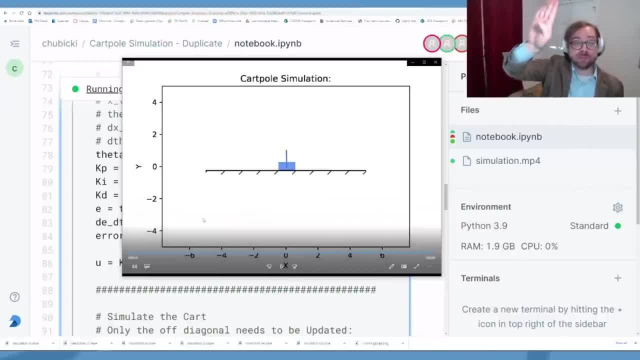 bit and come back right. if i put in a little bit of effort when the pendulum's at the top, it's gonna go crazy right, so it's not linear, so you can use uh. so so theoretically, my the lqr doesn't work now in practice we're. 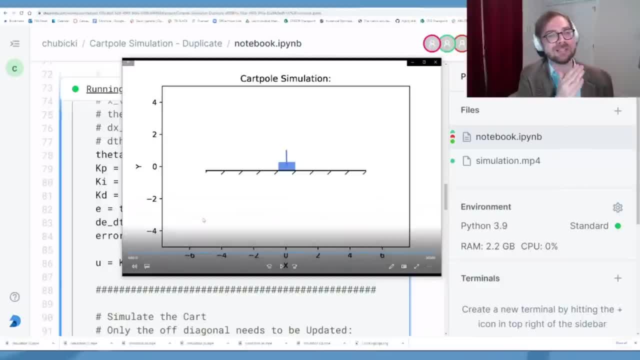 good at making it work. in control theory we learned the ways to linearize the system. pretend it's linear, uh, but genetic algorithms don't care. right, much like the honey badger, the genetic algorithms we can, you can get, you can give it whatever you want and it will try to come up with a solution, but it you. but you don't have those guarantees. 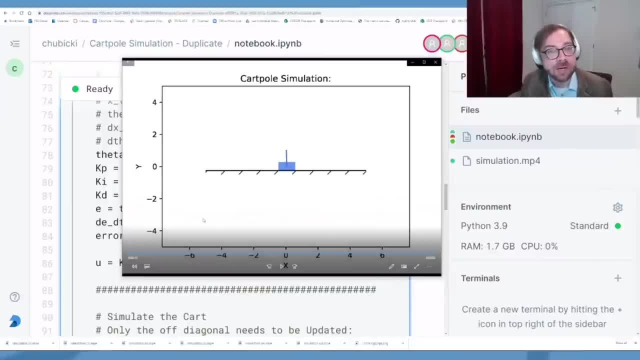 like lqr, mathematicians from 100 years ago figured out how to the the proof that says these are the best gains for that system. so it's this balance between what you can prove and what you can do. so it looks like the i term didn't do much, didn't kill the system. 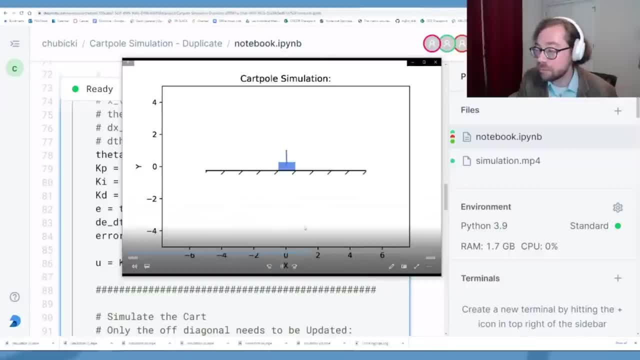 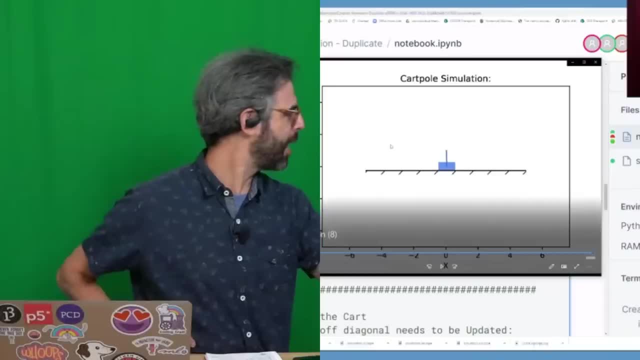 didn't do much either, still going, but i think that, but we can balance. i think this is a good time to hand it over. what do you think? yeah, no, this is perfect and and a good uh segue here in that. um, oh, and i've, i've a good segue in that. you know there's some other. 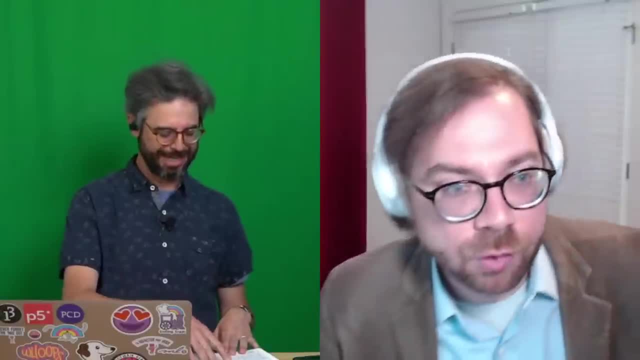 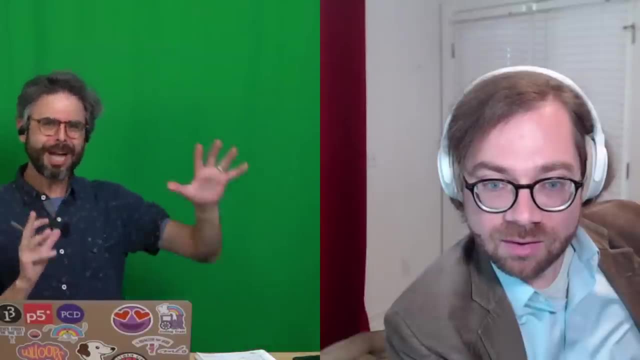 questions that maybe we can come back to towards the end. um, that i've been noting down here. um, but a lot of the discussion in the chat, which was super interesting to read, was: oh, i've been, i think i saw somebody try this in unity, or oh, you know what you could do? you could 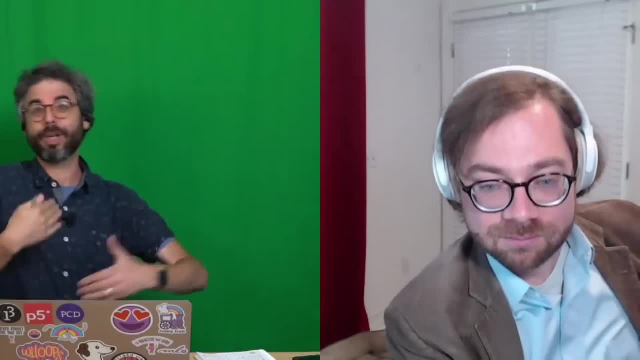 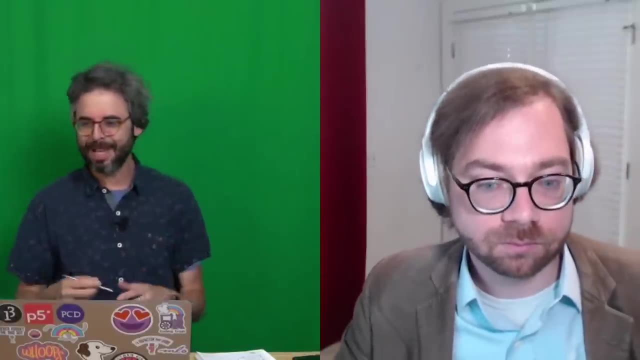 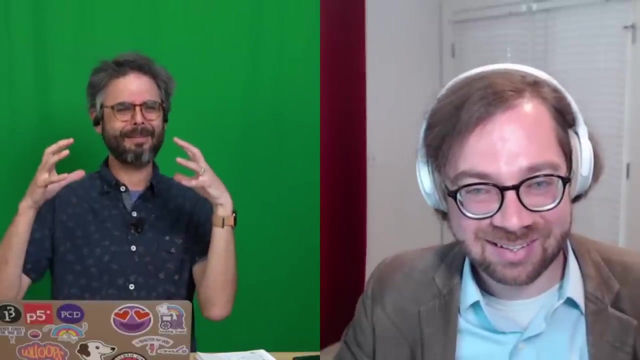 use pygame. so if you wanted to have it in python but have it be real time and interactive, you can use pygame for that actually. so this, this is really like kind of i think where we're going now with this stream. I'm just so excited about this topic that I have to kind of my eyes are. 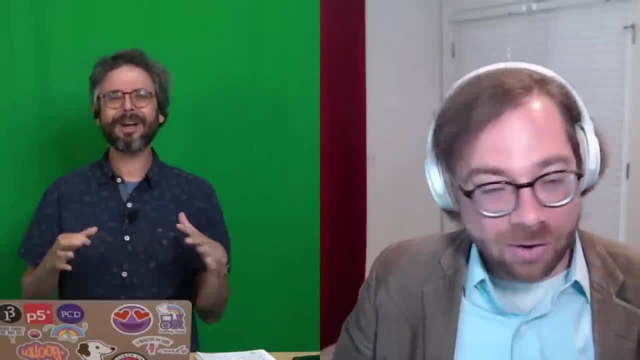 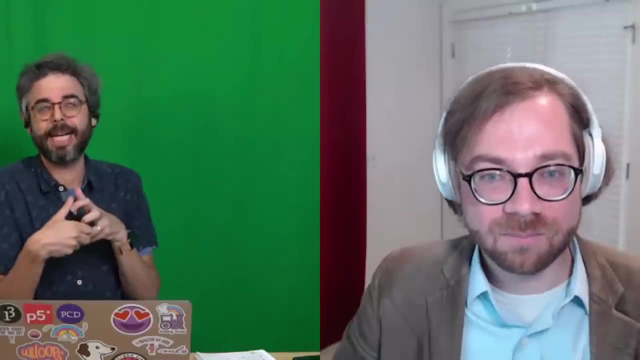 too big for my stomach, I think, is the right- maybe- metaphor here that I just want. I want to try to work in JavaScript and P5 to take a few steps towards beginning the idea of an interactive simulation around this topic, now that we've been taught about in such detail, But I do think it's. 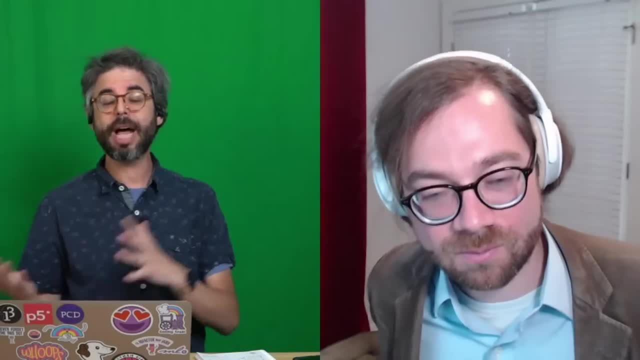 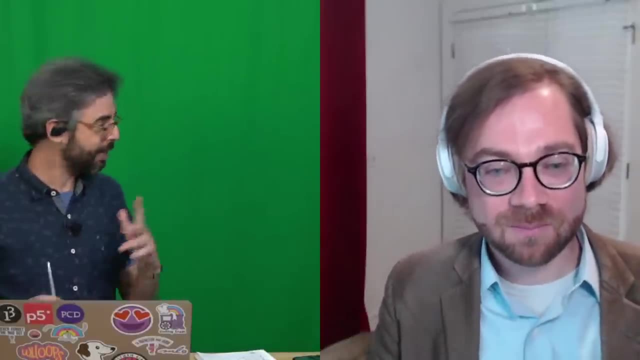 something that I would really like to come back to, and we can maybe do some additional live streams, or I might make some I really hope to do, like a specific coding challenge video about a PID controller. So yeah, so I think this is a good time to segue. Let's see if I can press this. 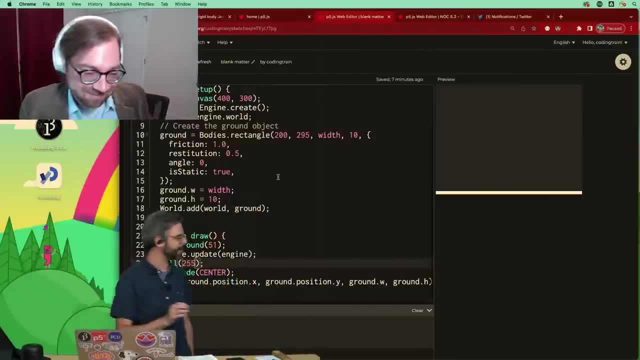 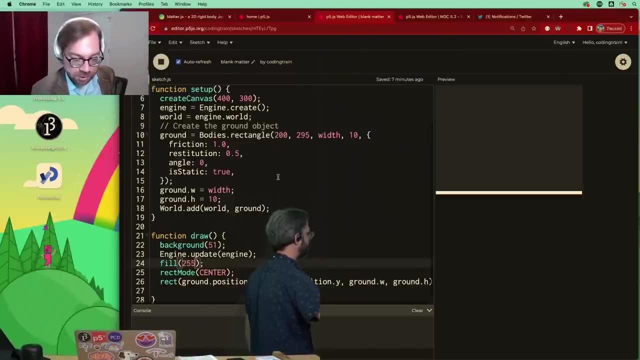 button. Hopefully this works Great. So now what we're looking at is- and I'm just going to make Christian a little bit smaller here- to not block the code. Does my voice pitch get higher when you do that? Yeah, no, no, I, it's funny. I have a video about that. there's a JavaScript. 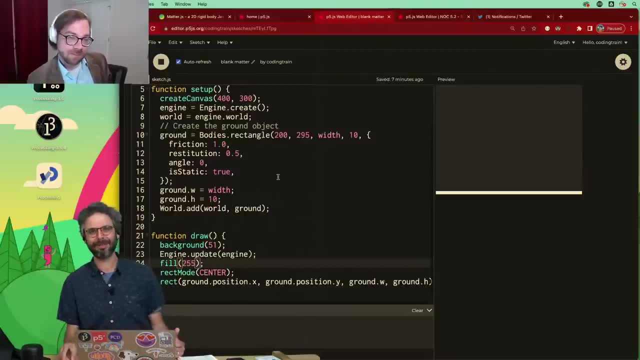 array function called reduce, which is a way to sort of like summarize an array of numbers all into one value, And that's a very sort of crude way of describing it, But it's like stick, where I keep making myself smaller in the video. Anyway, nobody should watch that one. It's really I should. 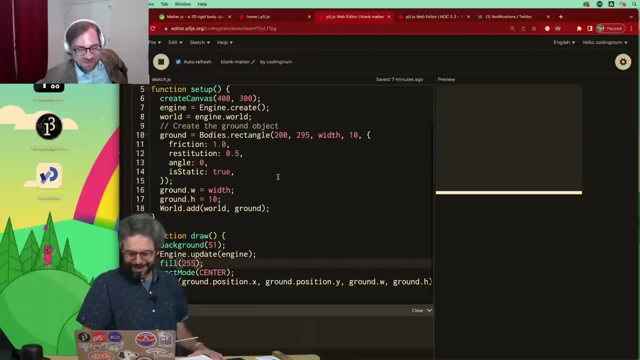 that should be deleted from the internet. But so let's see. So a couple of couple thoughts here that I want to just begin with. So one is: oh. so, before I go on, though, just you know, everybody, stick with us. If you have somewhere to go, don't worry, this will all be archived. 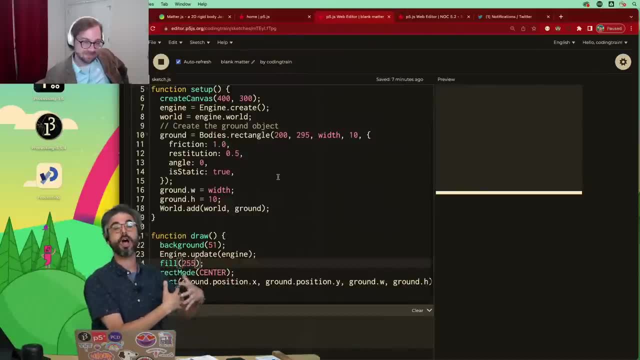 you can come back and watch it later. After the stream is over, I'll make sure to update the video description with all of the links of Python code that have all been demonstrated, as well as any other sort of extra material, And then we'll also make sure we sort of share. 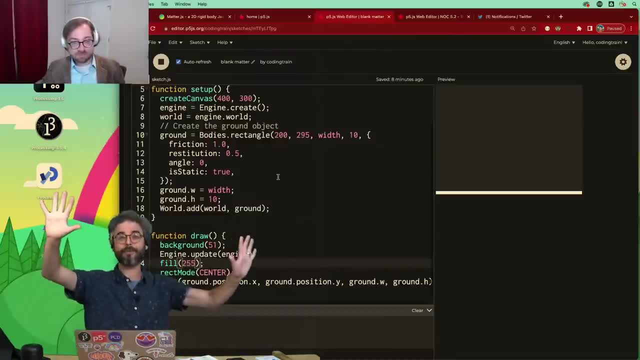 on social media. Speaking of which, just so we get- I get this now for anyone who's here. If you look at the video description currently, you will find Christian's Twitter Instagram. probably what I really like to highlight is Twitch channel, where, if I'm not- 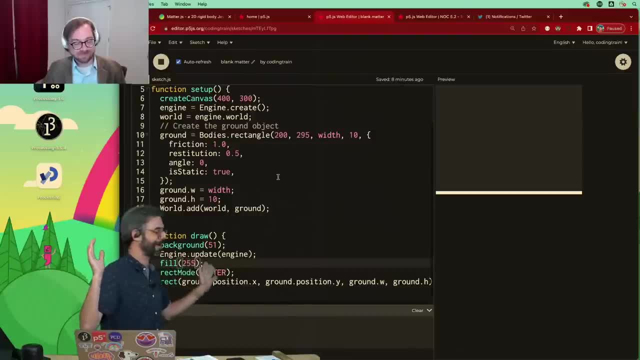 mistaken. you do a bunch of different things, but sometimes pop up lectures on various topics related to science and robots. Yeah, I should, I should, I should plug those things. Yes, So so I do do occasional Twitch streams, which I I'm still figuring out how to save videos. 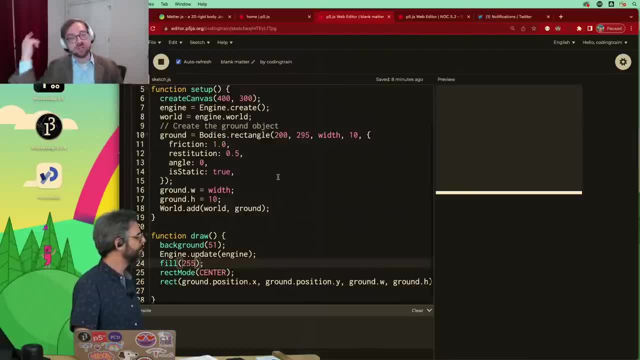 on Twitch, but I'm doing it as well. I'll sometimes I'll just run to the whiteboard and I will put a concept up there and we might throw together some code or just, you know, turn it into a lecture or just a Q&A. 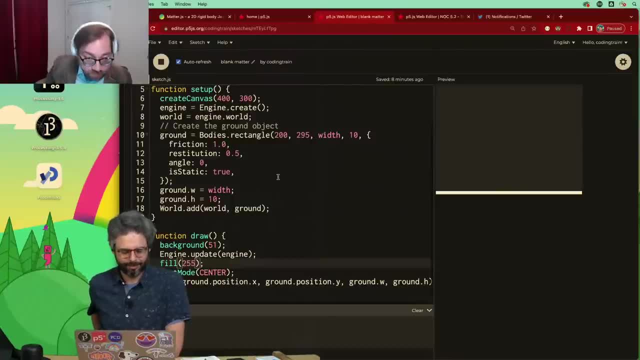 session about a number of topics. So so feel free to follow me on there And- and I look forward to hearing your feedback- on Twitter or any or any or any of these platforms, And I encourage you to use all kinds of ways of adapting this code. I mean, I'm doing it on Deep Note, for because we 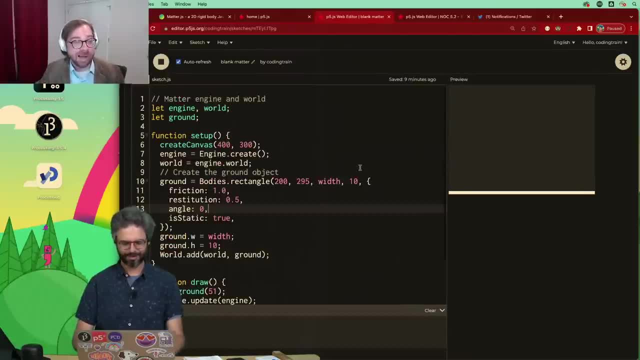 use it for other things. but copy that code You can put it on your own PyCharm or your own computer, whatever. whatever will run it faster for you, That's all great. So I welcome all that. So I appreciate your patience and listening to the lecture. 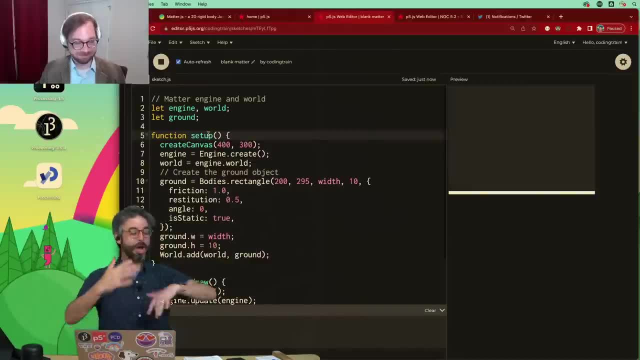 No, this has been fantastic And we're not saying goodbye. I just wanted to make sure because I know sometimes these streams they go on for quite a long period of time And I try to wrap up at the end. But I wanted to make sure that people who wanted to know more about Dr Hubecki's work and 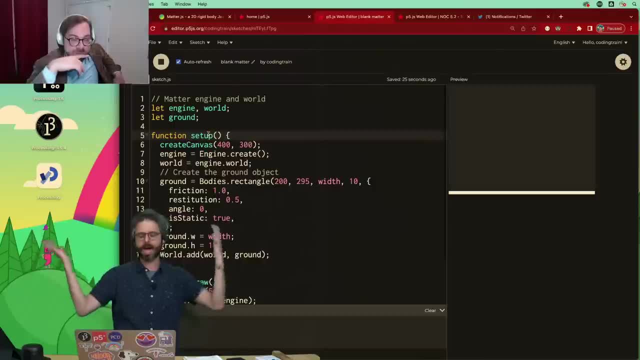 follow the labs research, you can find all that And again, after the streams over, we'll make sure to update the description with all, all the stuff. And of course, you can join the Coding Train Discord, where we have discussions and share. 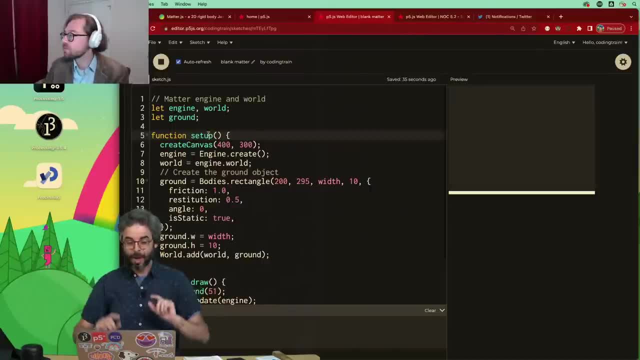 sharing about the various topics So you can ask questions and things there. Okay, but so I'm going to start to jump in. You know, I don't know what the ratio of people who came here from like Python and robotics control, versus people who came. 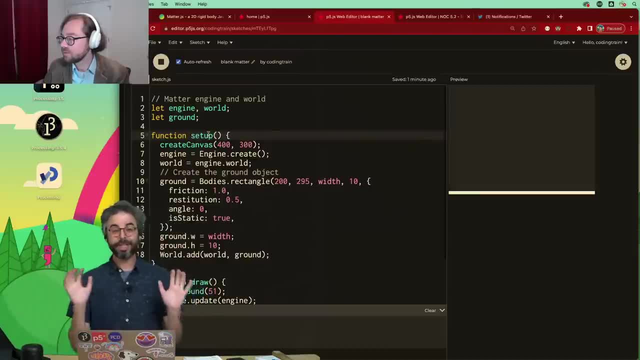 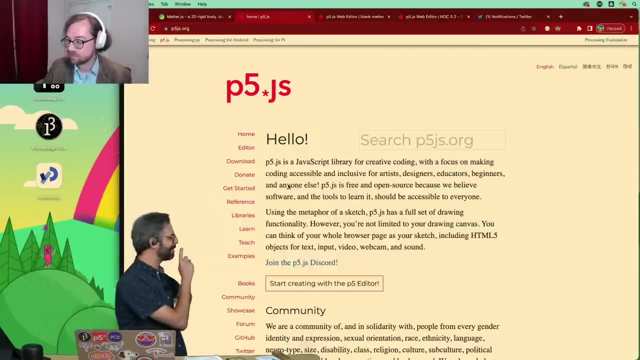 here from Creative Coding and P5.js. But just to set the stage for a moment what I am going to transition into doing. it's funny like I think that, like my output is a little bit, it has like the night shift on for some reason, So the screen is a. 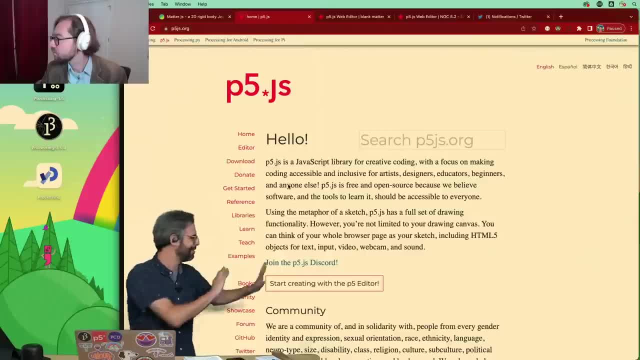 little bit. this is: I've never seen this before, I've never seen this setup, But anyway, it's fine, You can see it, But I'm going to use a library called P5.js, And P5.js is a. 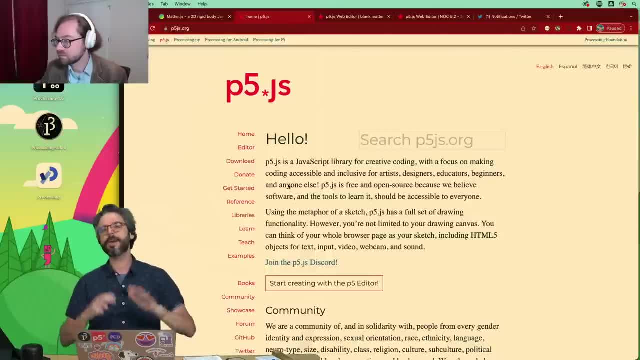 JavaScript library for what is referred to as creative coding. It's a very broad term But essentially, if you're interested in art and design and animation and play and experiments and games, it's a very beginner friendly environment for doing real time animations and 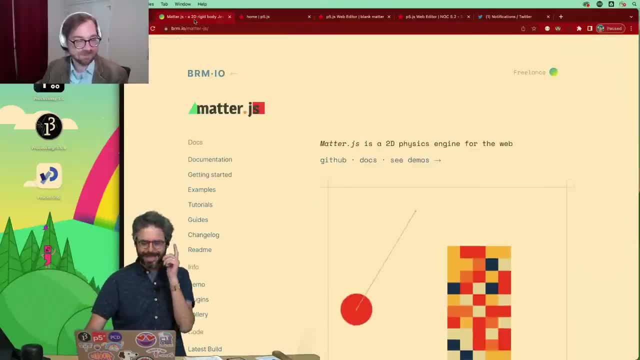 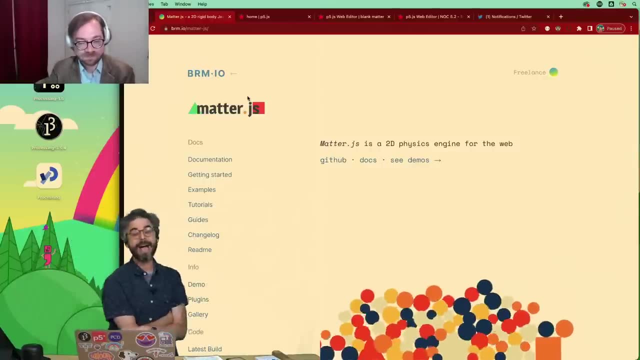 graphics and more in the browser. I also think- and I'm a little bit torn about this, but I'm going to talk a little bit about the P5.js, But I'm going to start with this physics library called matterjs. So I've been going back and forth in my head all week about this. 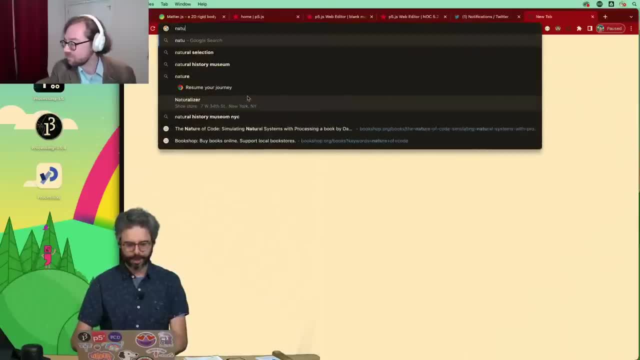 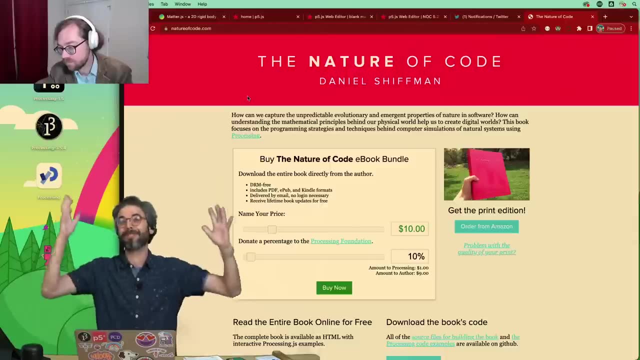 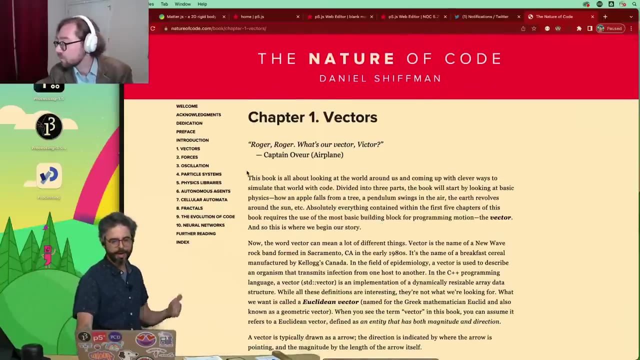 If you look at my- I'll just pull this up here in case you're not familiar with it. But if you're, if you're kind of new to the world of physics, simulation in JavaScript, you can take a look at this particular book that I have online: all about vectors and forces and oscillations and 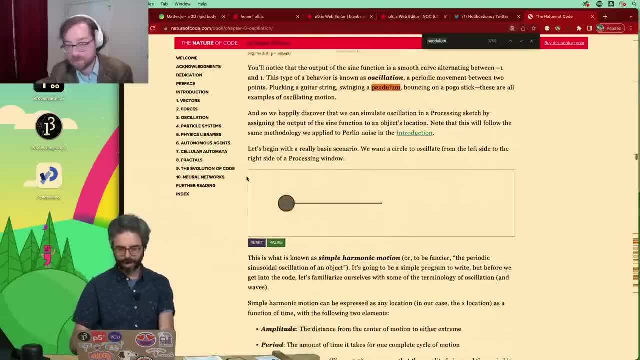 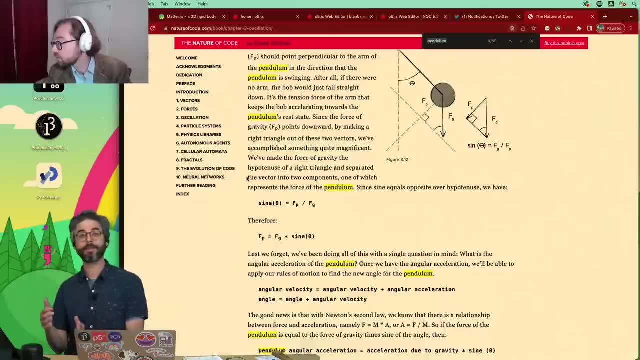 And you know, if I scroll down in here, we're going to find you know all about pendulums, And so this is a whole book that is sort of the foundation of a lot of the coding examples and tutorials that I do. 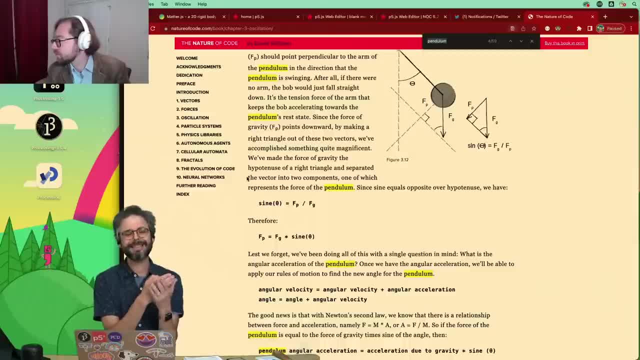 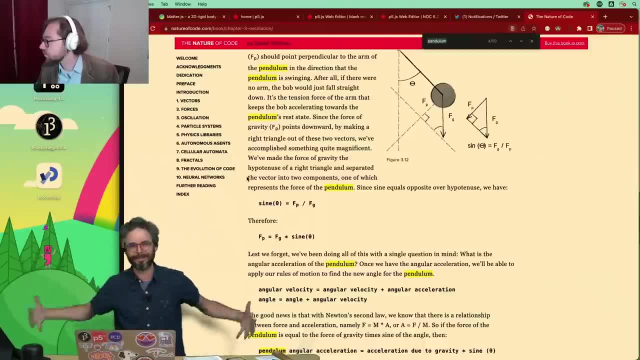 And for the most part I am always coding- these is wrong to say from scratch, because I'm using P5 and all sorts of other dependencies and libraries. But I'm not using a physics engine. I am doing the what what Christian referred to as Euler integration in the code. 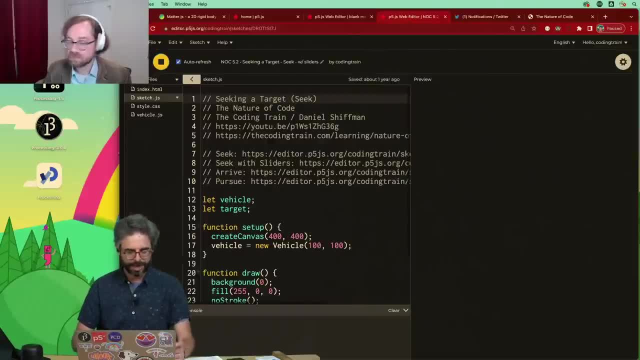 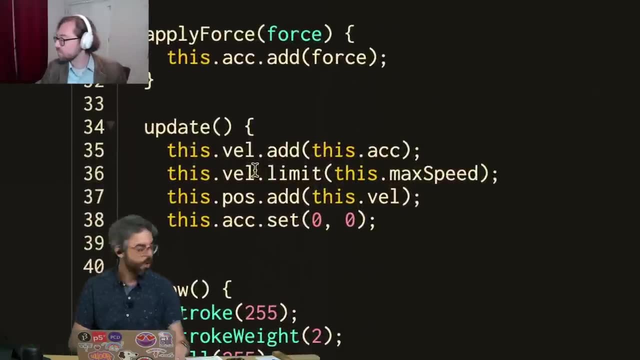 And in fact I'm just going to pull up this example really quickly, which is about the seek behavior. If we look here this: where's the update function? right, This is Euler integration. We take the acceleration and we add it to velocity. We take the velocity and we add it to position. Right, 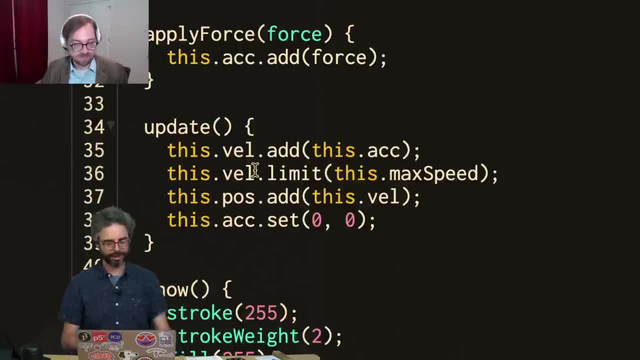 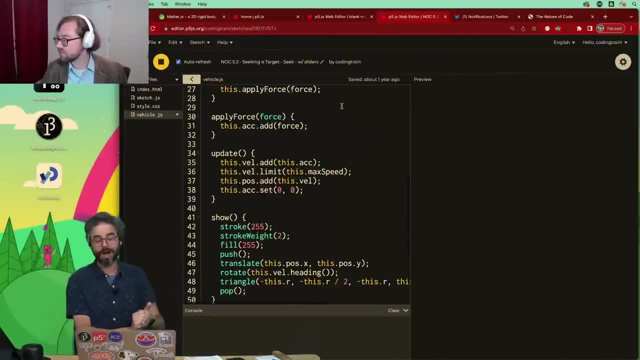 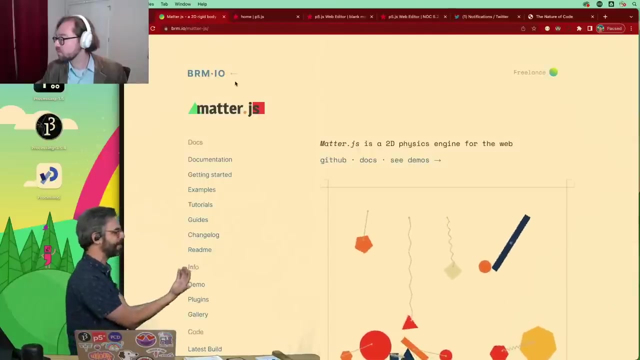 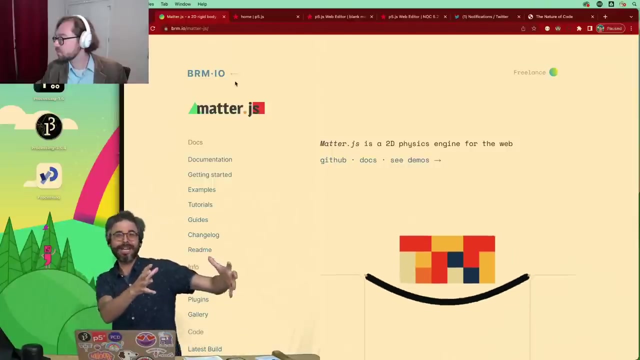 And we're accumulating all the forces in the apply force into the acceleration variable. So I would like to investigate PID controllers as they are connected more to the sort of like raw Physics simulations in nature of code. but I think I'm curious to see how does just applying this concept in a very quick and dirty way to a basic example that uses a physics engine- and to be clear what the physics engine is doing- is, I'm able to just say like hey, there's a round thing over here, there's a square thing over here, there's gravity, and I'm going to put this force in the system, you know, go. 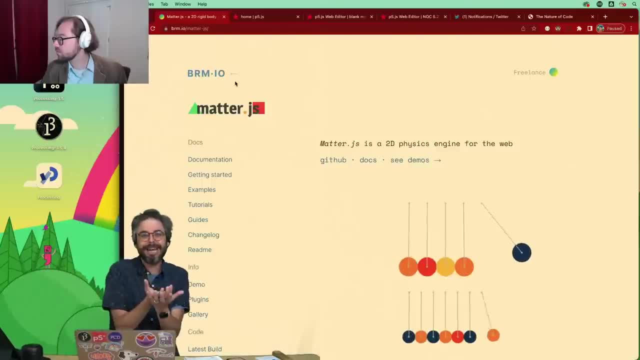 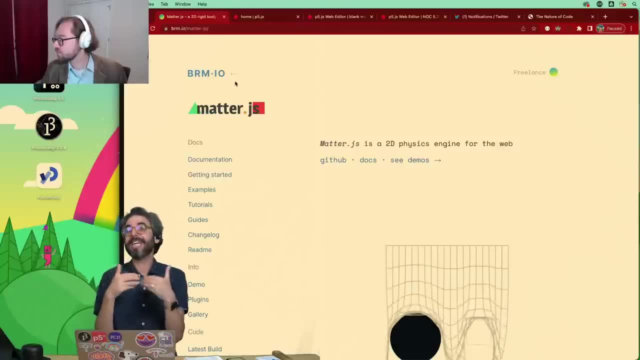 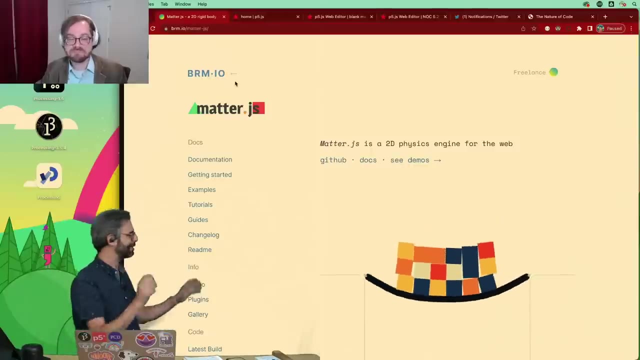 So we'll see how well this works. but can we set up a little cart on On the ground? can we apply forces by pushing it left, you know right or left- and giving it a calculate those forces based on PID control? So that's kind of my goal. I don't know Do you have any comments or questions about that, Christian, as I'm setting this up here. 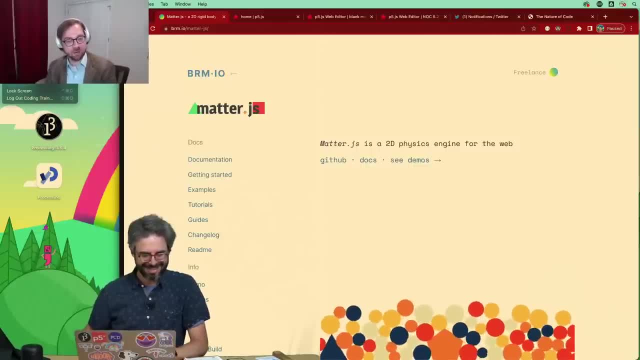 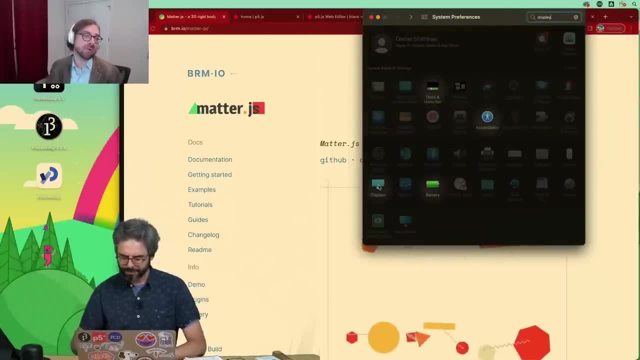 This is great. I'm very excited to see new ways to I mean, and as you're, as you're getting it set up. I mean, sometimes you know some of the bring up process, for when I'm trying a new system is the time it takes for me to code up the simulation. 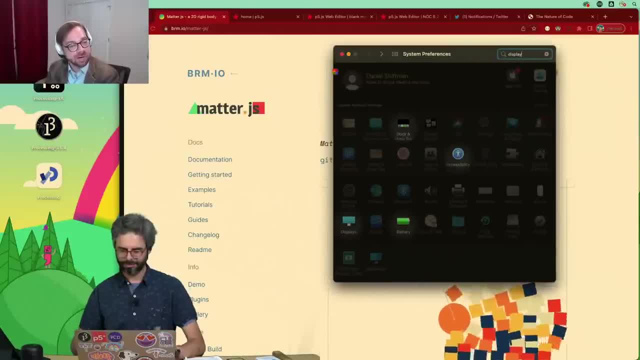 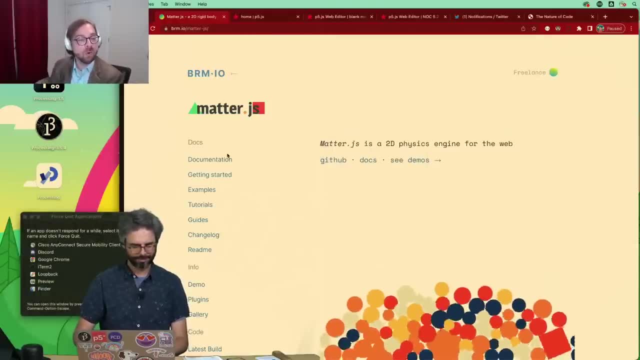 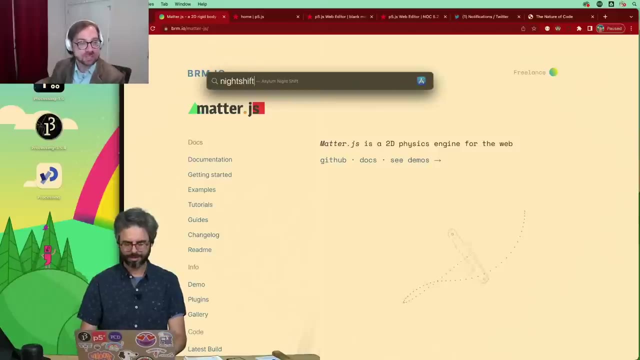 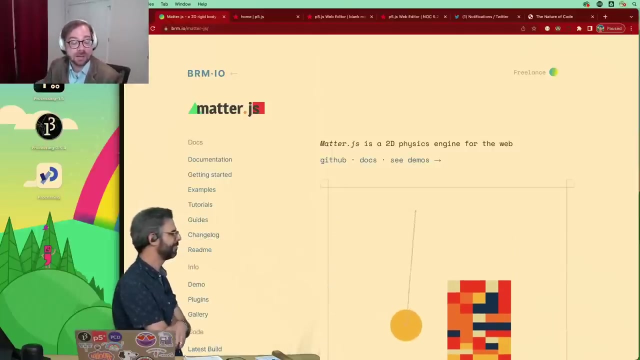 That's the first step That you have to do. when I want to try to code a new robot in a simulation is I need the simulator, And I think there's a lot of room for interesting ways to to generate physics simulations. I mean, sometimes I'll go straight to the equations, but geez, you know, be good to to do something where you pop in the, pop in such in the system and it just and they just bump around and go from there. 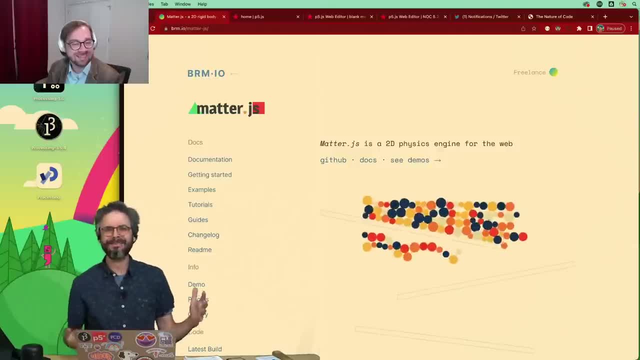 So that's exciting, Great, Yeah, I'm. I'm really stuck On the fact that I'm going to have to just let it go. But if something is going on with my screen, like look how, like look at the top right here. 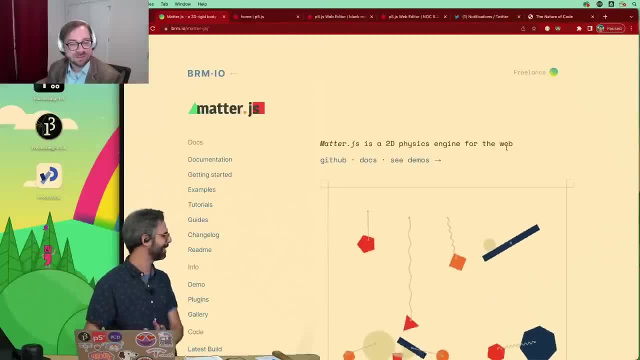 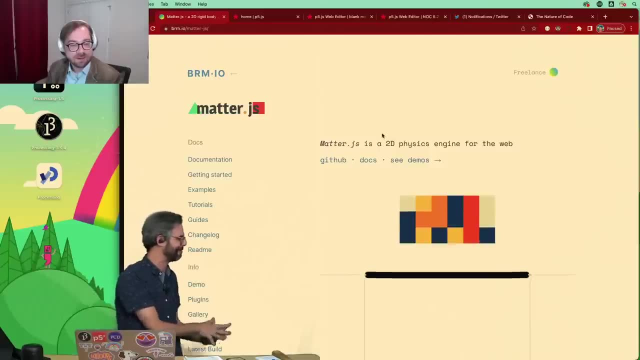 This is not the correct like back bar. like some weird glitch just happened and night shift turned on. It's like it thinks it's the middle of the night. I should be sleeping, So it's it's made. it's reduced the blue light or something in the in the, but I think we'll be able to keep going. 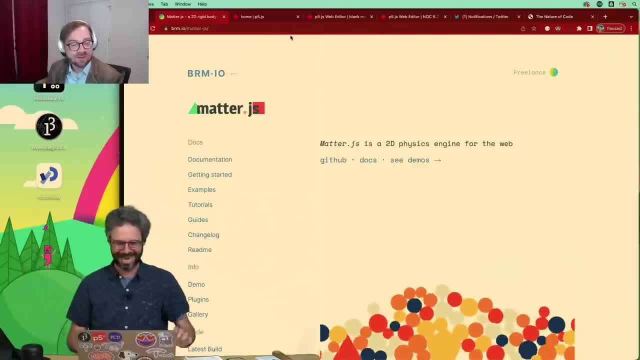 I'll think. if anybody knows where that setting is and wants to pop it into the chat, I'd like to fix that. But OK, well you are. you're a professional that cares about that sort of things. I was like I didn't notice until you told me 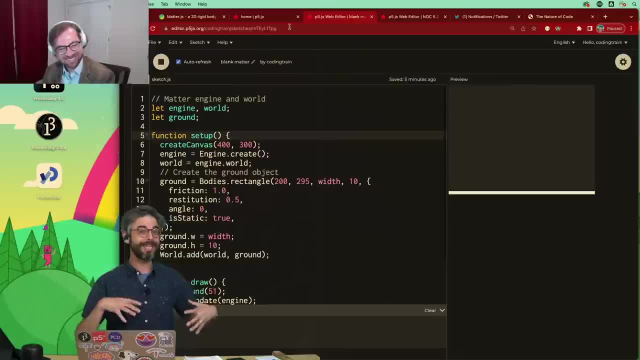 But yeah, Yeah, Well, you know, yeah, I'm recording everything to disk, also from today because, as as the viewers know, I often take content from live streams and remix it into sort of like a shorter edited video, So which I was thinking about maybe doing. so it'll bother me forever that the recorded, you know. you know I could do that. 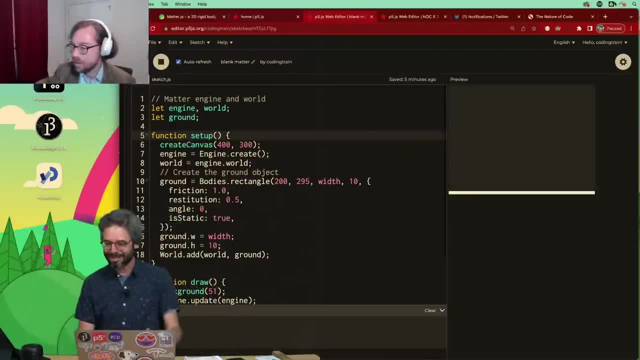 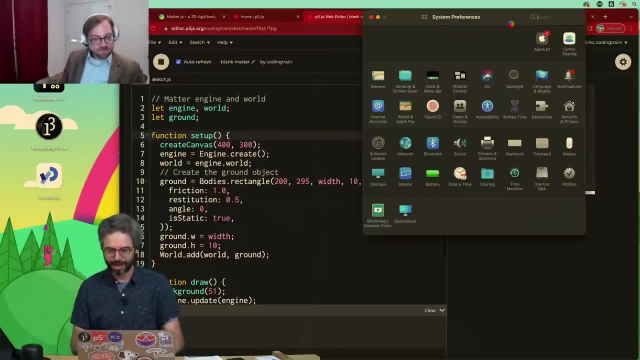 I'm going to let it go, though It's going to be fine, because I knew where to turn this off. But look it, it this: if this is the only totally wait, wait, wait, this disappeared. So my system preferences- see, my system preferences- is like frozen. 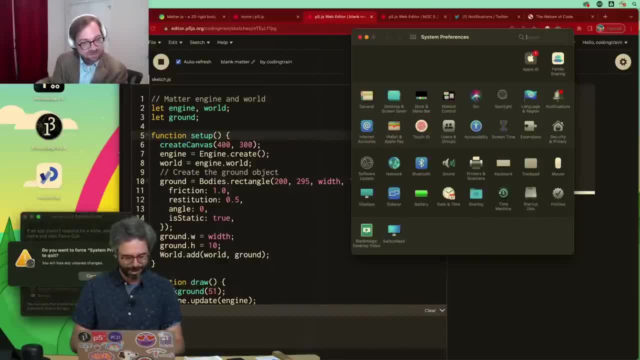 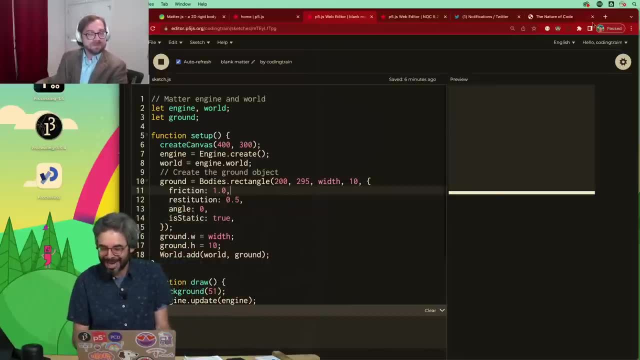 I have the rainbow of death here spinning rainbow of death, So I'm just going to force quit out of that, not worry about it, And you can change it in the control center. I know, But look, the control center button is missing. 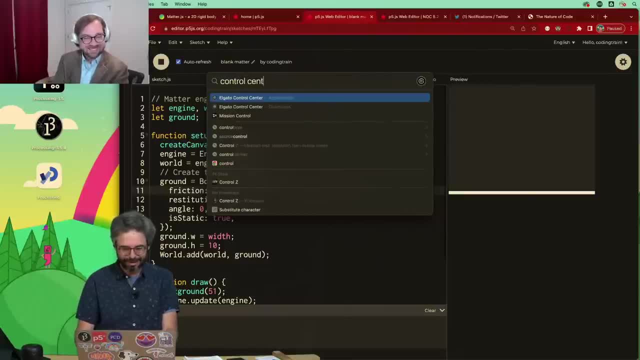 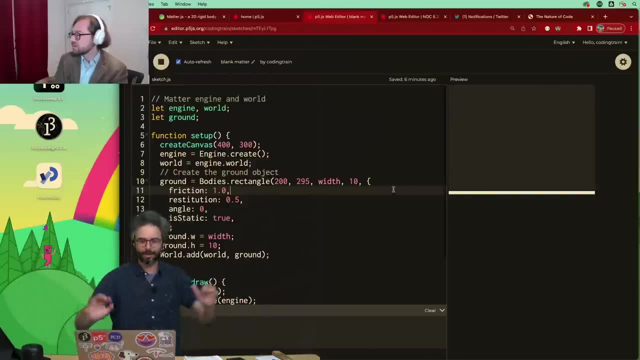 It's disappeared. control center. OK, now I've got OK, so I'm going to. if everybody, if anybody has trouble seeing what's on the screen, let me know. I think we're fine, All right, So I have put in the pin. comment in the chat. 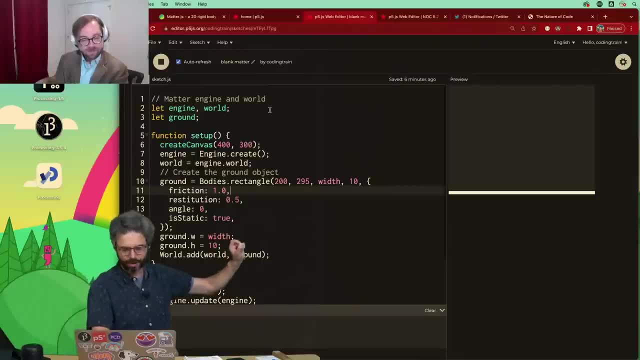 And I have put in the the pin comment in the chat And I have put in the pin comment in the chat. I have put in the pin comment in the chat and I should have done this, for the tiny URL link from earlier is a link to this particular P5. 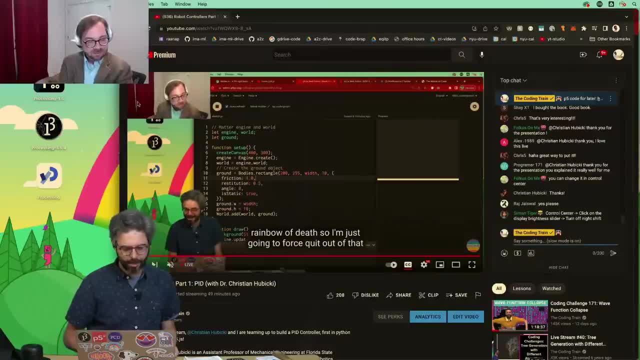 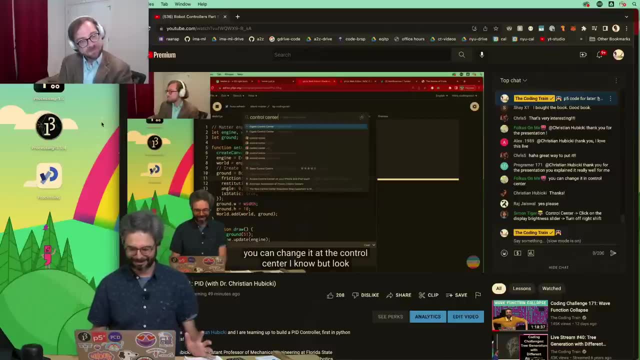 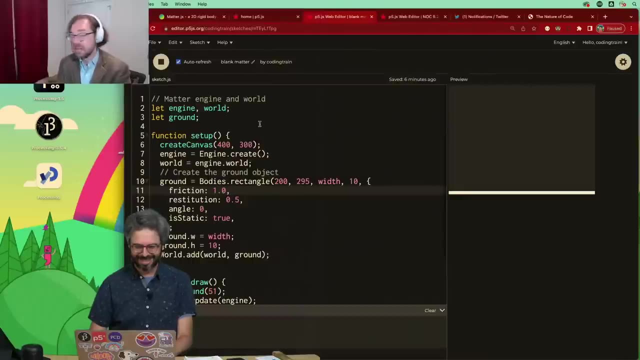 sketch. So again, you know, I oops whoa, look what's just like. things are just appearing like out of nowhere. I wonder if I should restart my computer. Look at that, That's interesting. I mean, if you wanted to handle that, I can always I'm engaging in the 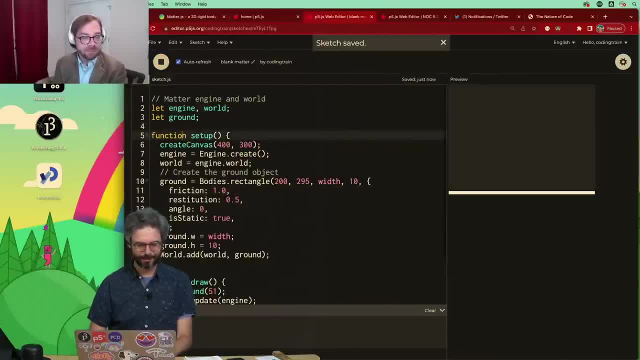 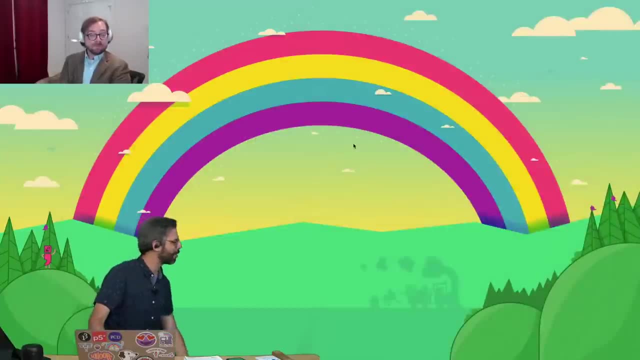 chat right now. If anyone wants to jump in and if you want to handle that business, I can. I can talk about this sort of thing. I'm going to restart and I'm going to ask you one of the questions that came up which I was kind of curious about. Somebody asked, like whether you 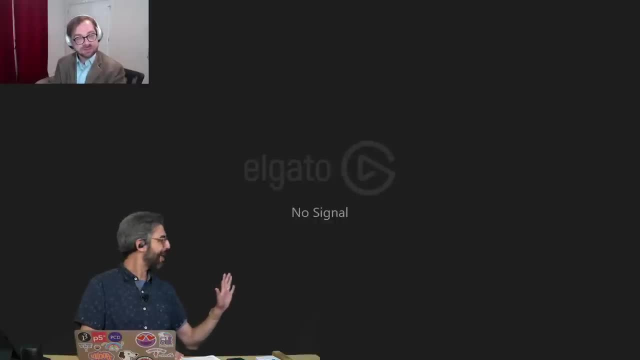 could use PID to like land a rocket, like a SpaceX rocket, And I was actually curious, I don't know. you know I've been following the James Webb telescope with all the images that have been coming out And I know there was so much that went into the design and engineering and production of 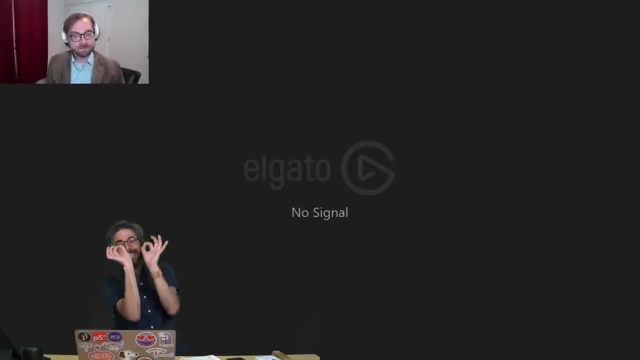 the telescope, you know, and the fear of sort of like any little, like slight angle of a mirror setting. But do you know to what extent does the work that you do in robotics research apply to these kinds of mechanics that happen in space? I guess that's. 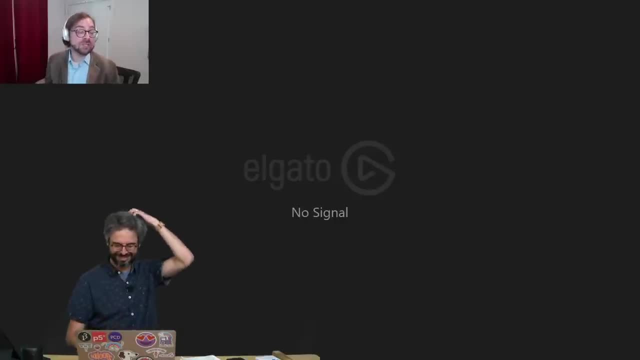 what I'm asking. So so, so yeah, I mean I, I am interested. So the short answer is like: like I mean, reliability of controllers in space is super important And the and I need to be more. 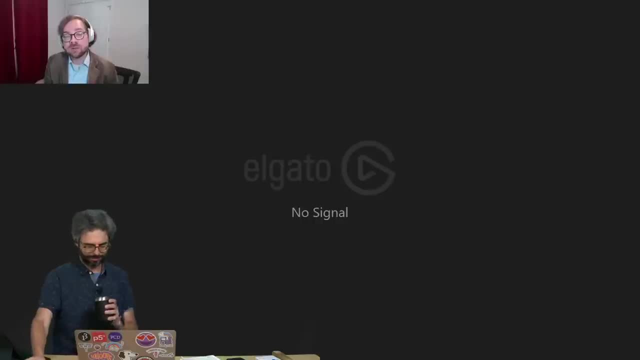 up on what is actually being used on some of these particular spacecraft. But but somebody landing a rocket, I mean you look at how that like, if you, if you watch, like a SpaceX self-landing landing rocket, you could almost see the PID in action. that now under the 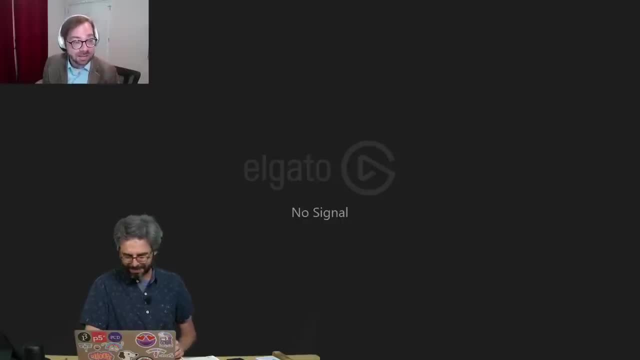 hood. we don't know exactly what's what's being used, necessarily, But, but, but. a lot of different control techniques. even if they're not explicitly PID, they end up acting like PID- They'll, they'll. if you need that, a lot of you need to be slowed down. we'll start applying a force in the opposite. 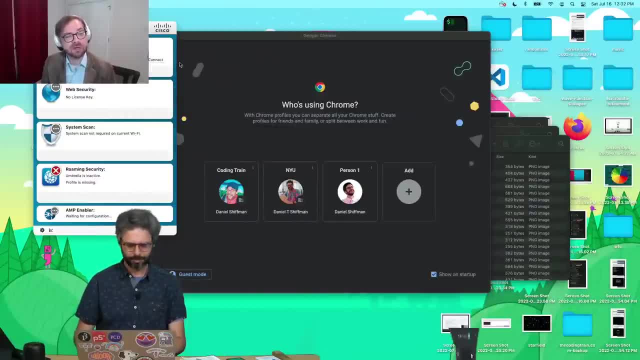 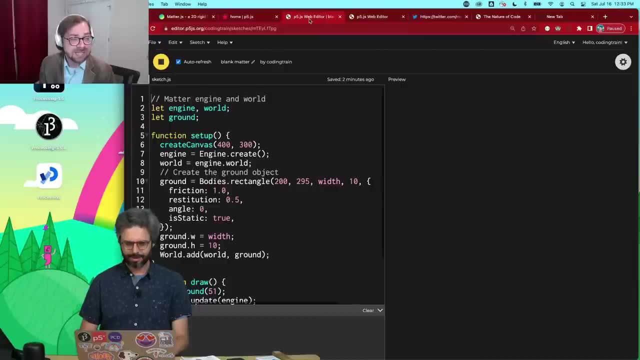 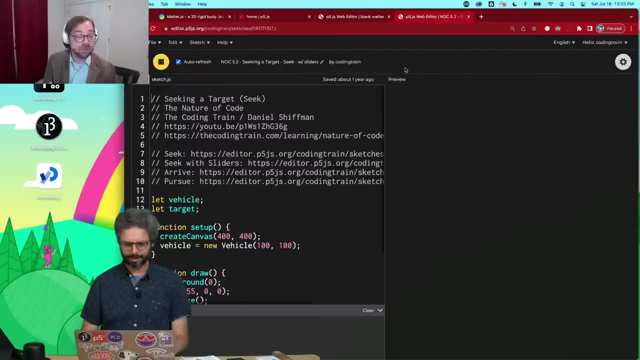 direction I was seeing in the chat. there's something called MPC, which is like what's called model predictive control. But what MPC is is it's basically more or less acting like PID, except it's able to reason about the fact that you might have limits on how hard you can push. You know. 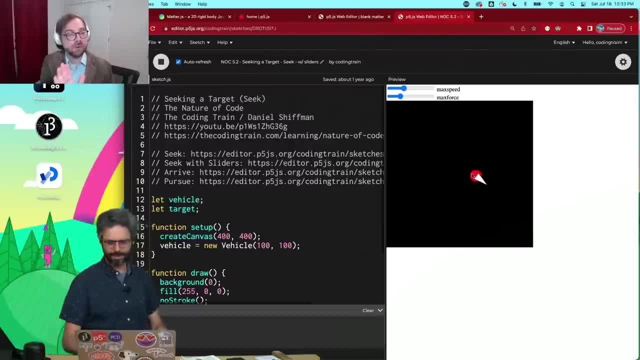 if in on our PID controller, if you had a limit on how much force you could push, it would try to ask for things beyond that limit Now and it might not be able to do it, but it might be able to do. 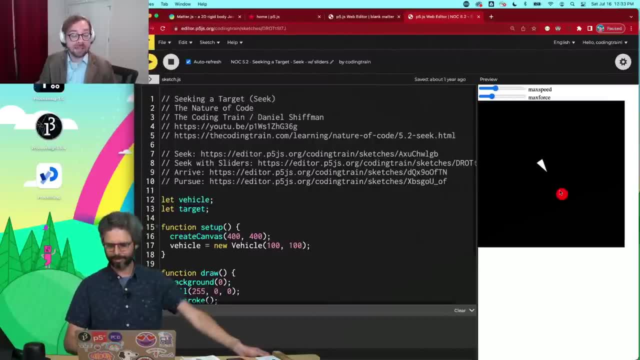 it and deliver, and it'll you know so it'll do the best it can. However, there are methods that will understand that I am limited how much force I can do, And once it, and that's going to require me to think ahead and push more later, because I have to push less now, for instance. So even 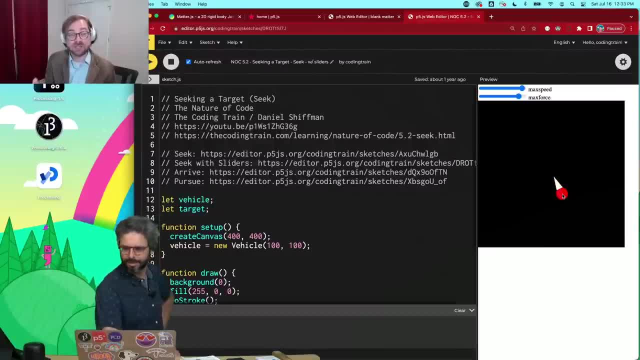 if PID isn't used directly, in all of these cases, the core principles of it are often present And I would not be shocked at all If that, if in the space thing, in the, in the, in these, in these space settings, that that you need to, that that they will be using PID to orient. 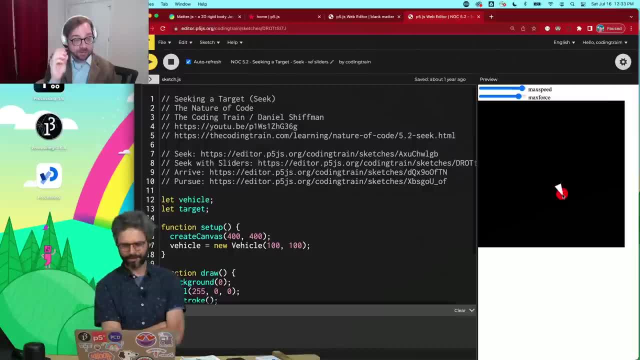 different, different elements of the of the spacecraft, But they also one thing that they also want to be careful about is if, if something fails on the spacecraft, that it still works. So if you, if you can. one thing that a PID controller requires is that you have sensing that you can. 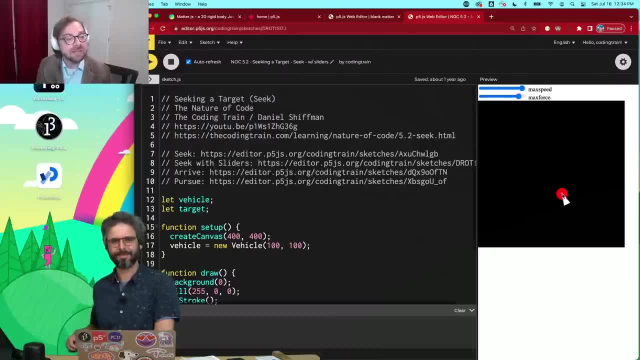 sense that what your angle is. And I guess what happens if that sensor is is gone. that sensor is gone Like what was the whole spacecraft down. So a lot, a lot of the very bright mechanical engineering things is that they'll they'll try to make this sort of idiot proof that, even if the sensor is, 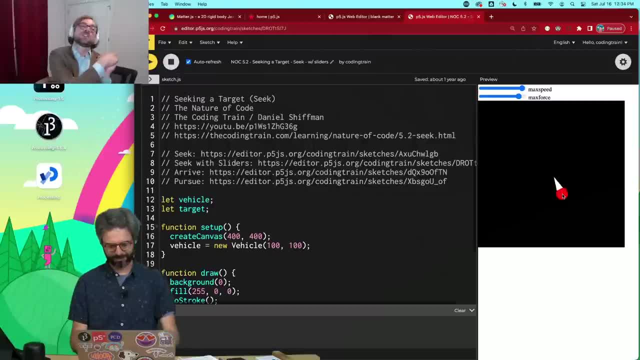 gone. you just have to apply a torque and then it'll go against the hard. stop. That way. you don't have to have a sensor right, It just deploys right. So one one one. so if you can, so things, and this is not just PID control. 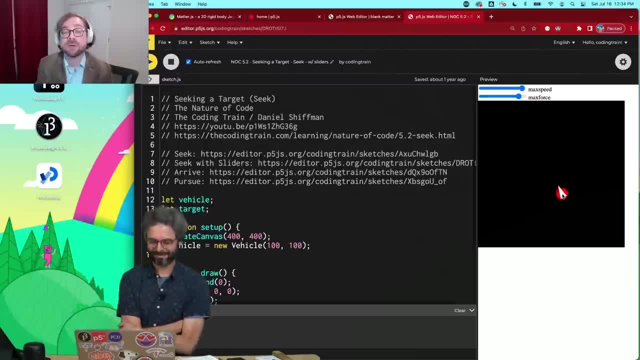 this is any form of what we call feedback control, where you're getting feedback from sensors, you're getting information from the sensors. uh has that component and inherently adds at least a little bit of complexity. Yeah, That's great, Thank you And and look in that thank you for. 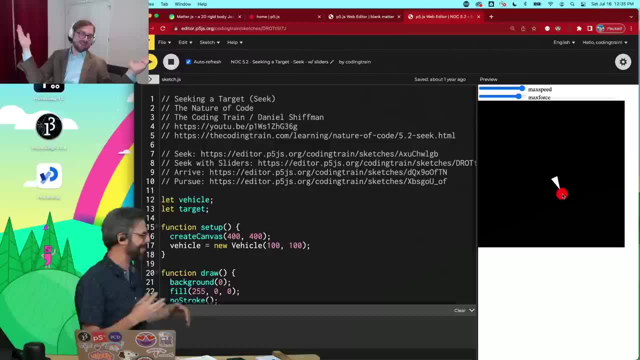 uh, talking through that in that beautiful amount of time, restarted the computer. the- uh- the menu bar thing is looks correct And I've no longer have that slight tinge to the hue of the screen. So we're back and ready to go. 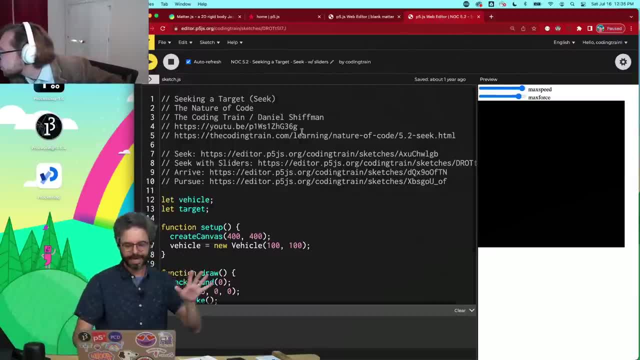 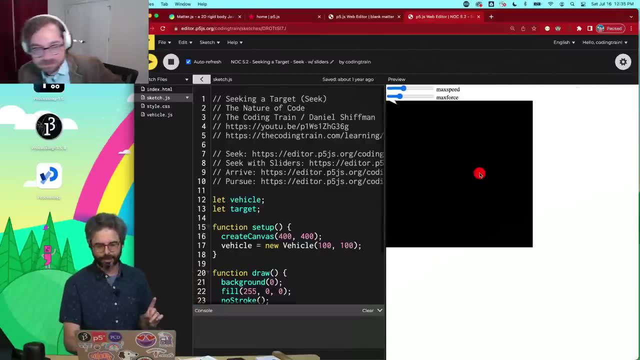 So I also just wanted to. I'm gonna jump back into that matterjs sketch, but I just wanted to show here um that this is the seek example I was referring to, which is this simulation of this steering vehicle that is attempting to seek this target. 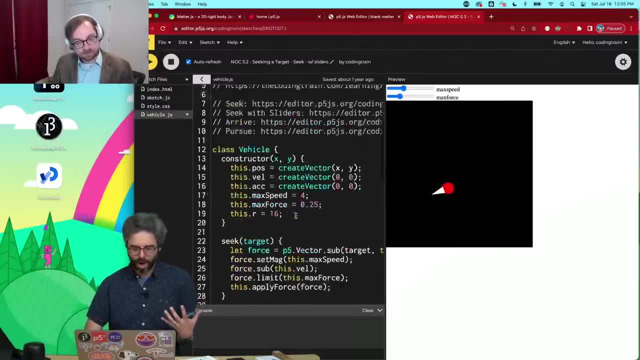 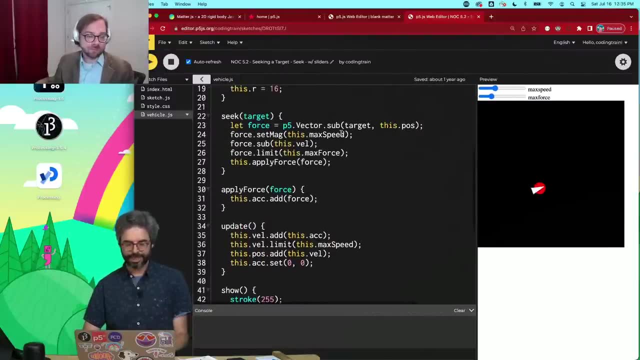 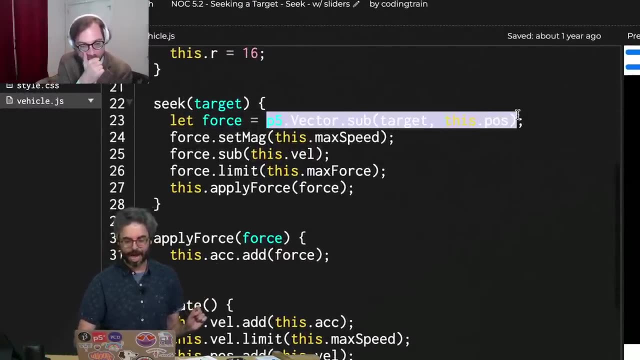 which is a red dot, And little did I know really all along that ultimately this um uh seek function is essentially uh w, which is what I've covered, like in great detail in many videos. is this error? I am looking to find the difference between the target's position and my position. 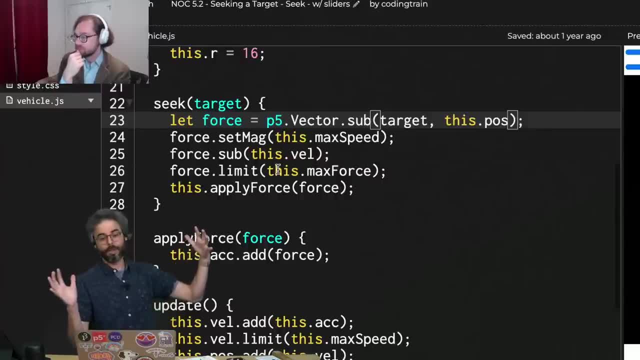 and creating a force out of that, scaling that force according to this max force variable, which is much like the gain in the P controller, and then applying that force. So we're going to do something similar, but I'm going to switch over to using matterjs. 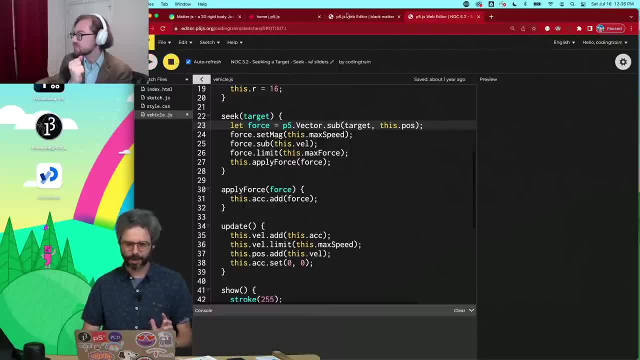 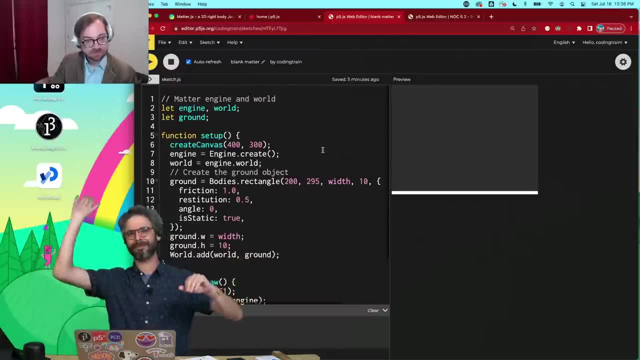 and looking at the cart poll kind of scenario. Okay, so let me stop this. So if anyone is interested in that, hit me up after. I'm sure just through some nice online searches you can find the nature of code book and the nature of code videos, and 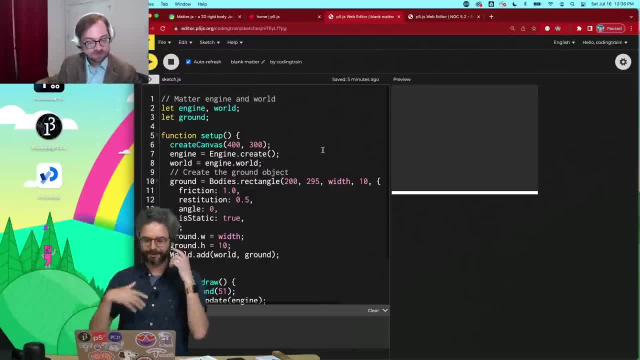 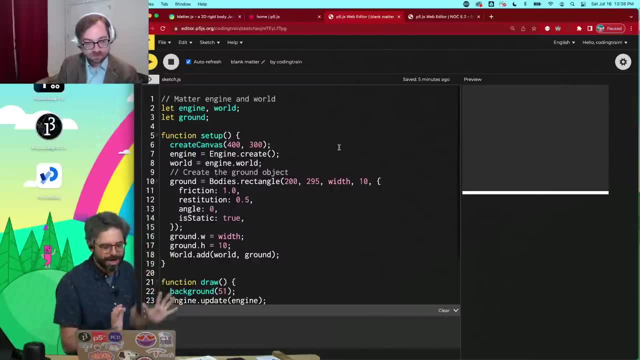 all of that. But if you're interested in going down that road and you can't find it, let me know in the comments or in the chat and I'll be able to answer that later. Okay, so let's take a look. I've started. I put a little sketch together at first, just so we didn't have to in a lot. 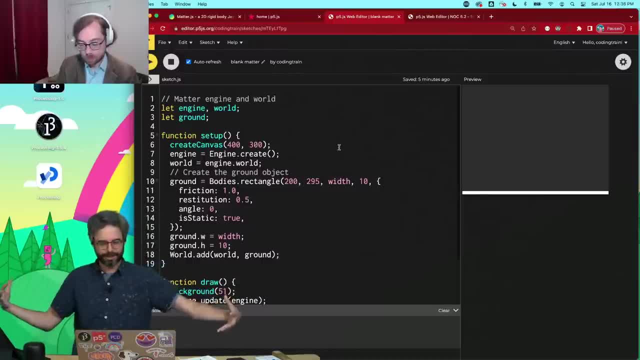 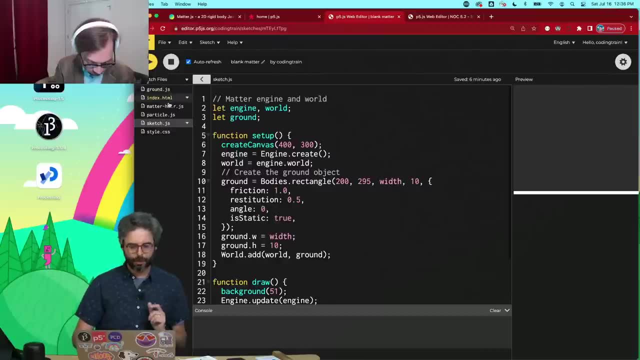 of my video tutorials. I always like to try to show the entire process of coding something, but I wanted to at least have a little sketch. I have a foundation to start with. to try to save a little bit of time here, Let me show you probably the most important piece of this, which is that- and I'm actually 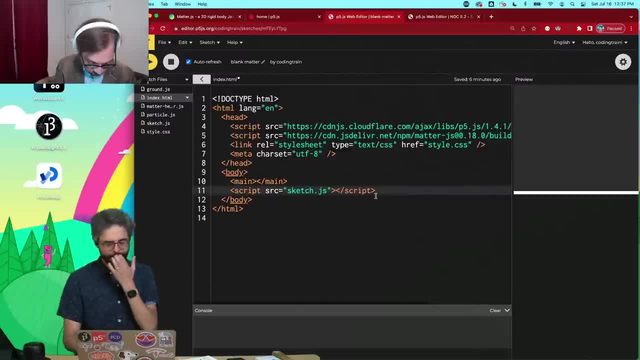 not using all of these, So I'm going to take these out now just to simplify. whoops, maybe I was using one of those and I didn't realize it. but let's, I'll just leave that in there right now and I'll figure it out. 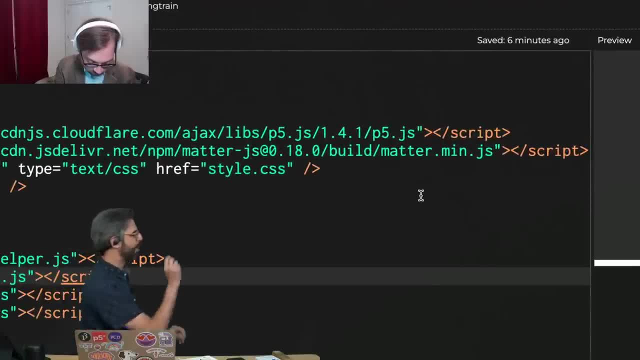 But the important part that I wanted to show you is you. I'm importing both the P5 library here as well as the matterjs library there, Okay, Okay, So you can see that the P5 libraries are hosted with a link to the Matterjs library. 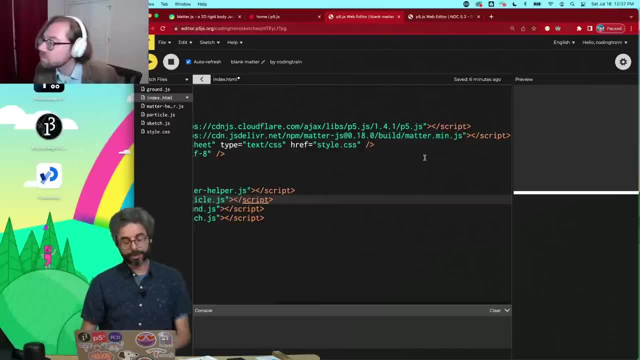 So the P5 libraries are hosted through the CDMs or content delivery networks, where the JavaScript libraries are hosted online. So you know this merits a longer discussion in terms of how you build all the components of a web page, but the P5 web editor, for the most part, will really help you along. 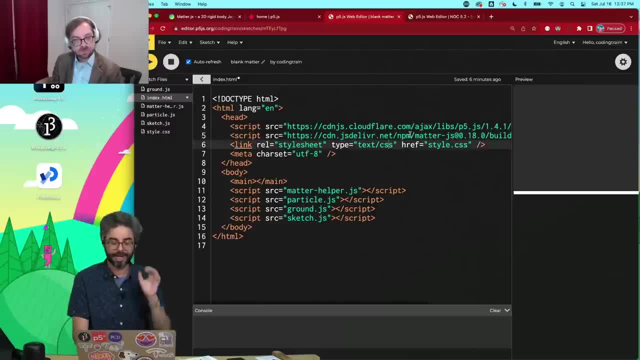 The only thing you would need to add if you were starting from scratch with the P5 web editor is this link to the Matterjs library, and hopefully folks in the chat can help answer questions about that if you're struggling with that. Oh, I need Matter helper. 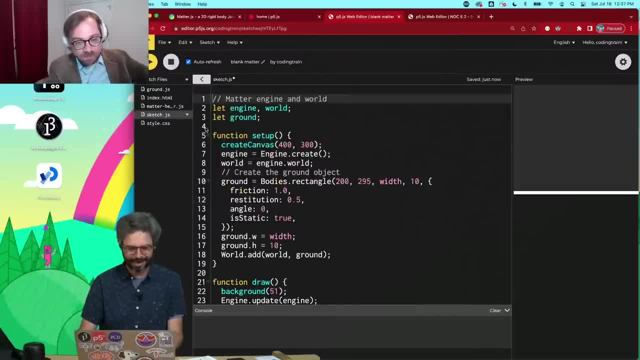 So I was simplifying this sketch and I left a couple things in here that I'm going to take out now from a previous example. Okay, so one thing I'll also note is that there's this JavaScript file called matter helper that I made. 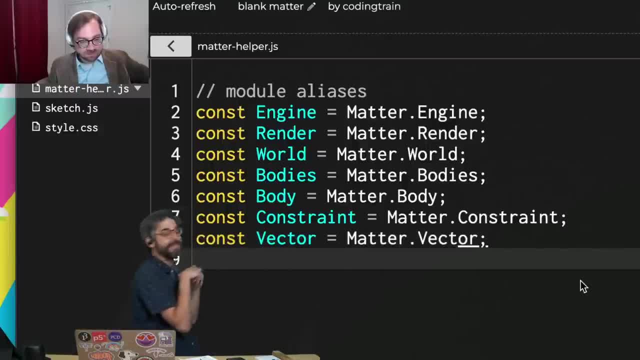 It's a little bit silly, but anytime I want to refer to something in the matter physics world, I have to access it via the matter namespace, like matterengine, matterrender, matterworld, And so I made all these little aliases to each one with just the single word. 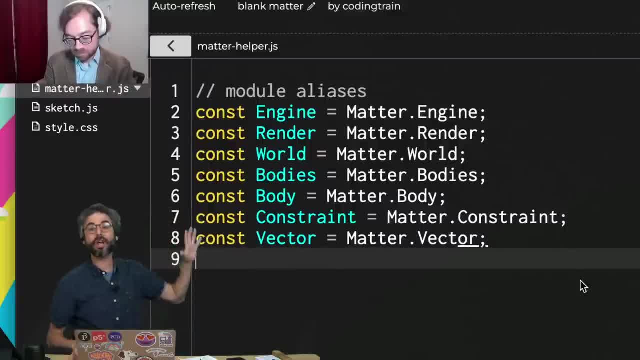 engine or vector or constraint or body, And I'll talk through what each of these are as we start to build the code example itself. But this just allows me, in the code as I go back to here, to say things like create an engine as opposed to matterenginecreate. 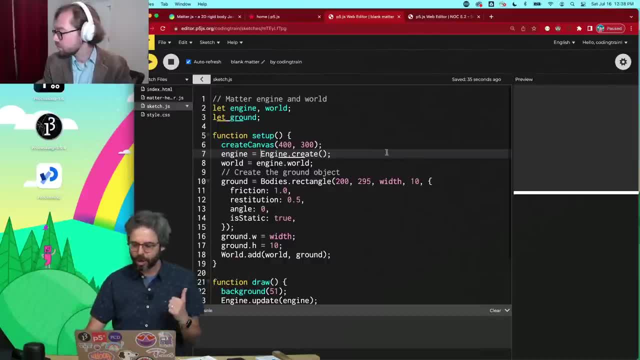 Least important detail of today, but a little helpful thing, Okay. so let's look at what's happening. So this is the setup function And, you know, actually I made the font a little bit smaller than I usually do, because some of this code is kind of long. 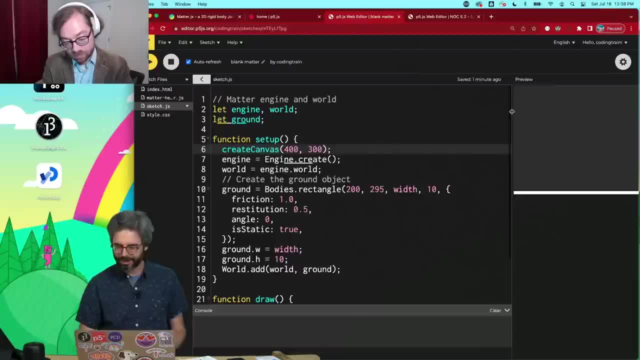 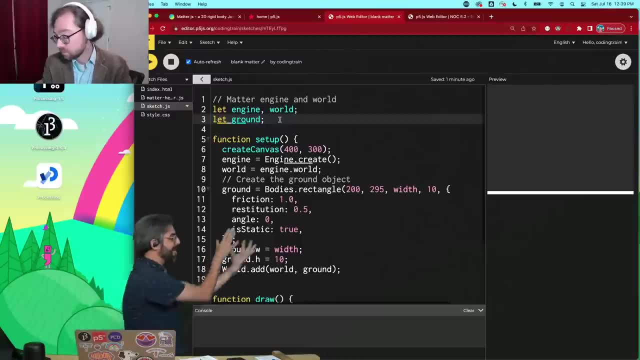 Let me see if I can up it just one couple points. So let me know if anybody has any trouble reading the font. But so the only variables I'm starting with right now is I have an engine That's the physics engine that's going to handle that Euler integration. 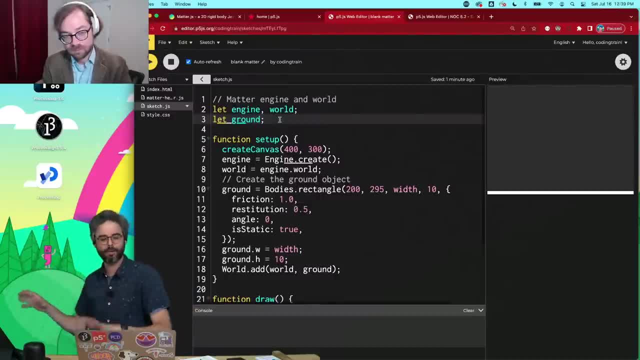 and all of the figuring out where the bodies move and how they move for us. I need to also store in a variable the world associated with that engine. The world is basically like a variable. I'm just holding on to a big list of everything that exists in the world that we've created. 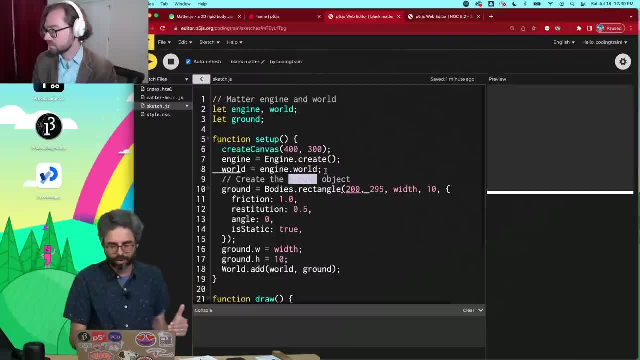 So you could have multiple worlds and do all sorts of interesting things, but we just have one world, And then any time I want to make something in the world, I need to create it as a shape. It has to have some geometry. I don't know what these weird underlines are showing up now too. 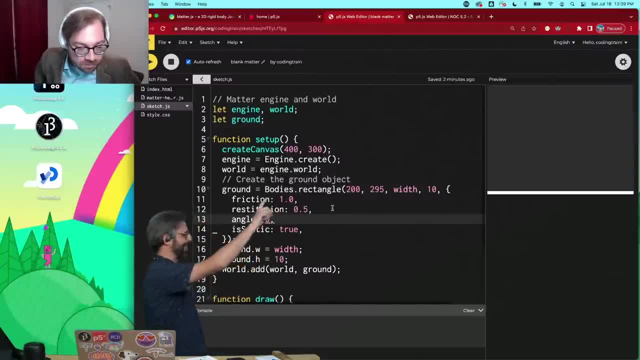 There we go, But I'm going to ignore that, All the weird extra things that are happening today. So I want to make for the ground. you can see I'm drawing it there, this rectangle, And you know this will be very familiar to any of you who use it. 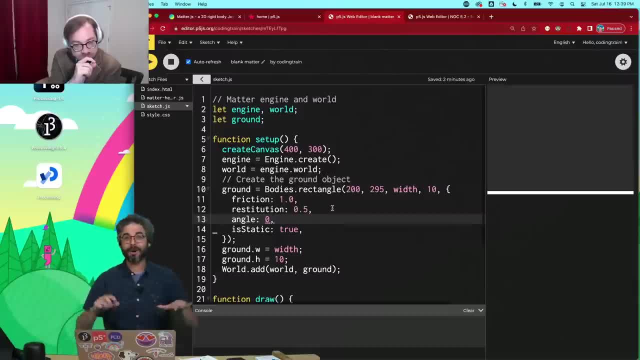 You use P5 regularly, but for Christian watching or anybody else who comes from maybe, a world of sort of more true mathematics, this canvas that you're seeing on the right here. it is a Cartesian plane, but it's a very odd one. 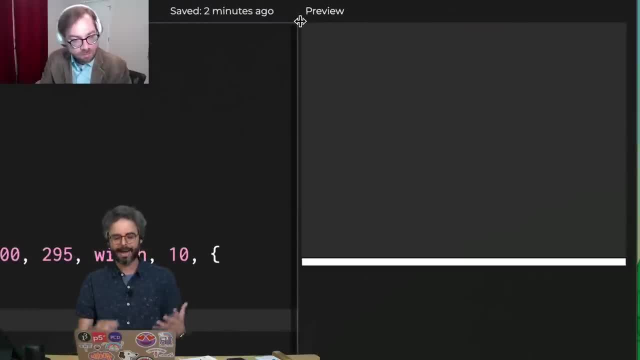 First of all, it's very typical of computer graphics, but odd in the sort of mathematical sense. 0, 0 is up here in the top left, not in the middle, And the y-axis is pointing down in the positive direction. 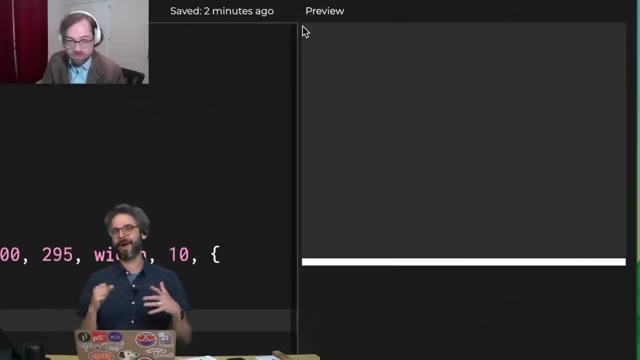 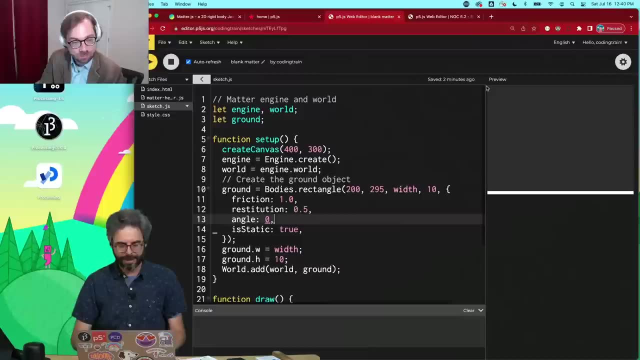 So that's quite standard for computer graphics, But odd. If I were doing like a lesson about you know, a pendulum, we would draw a Cartesian plane and point y up and have 0, 0 in the middle. 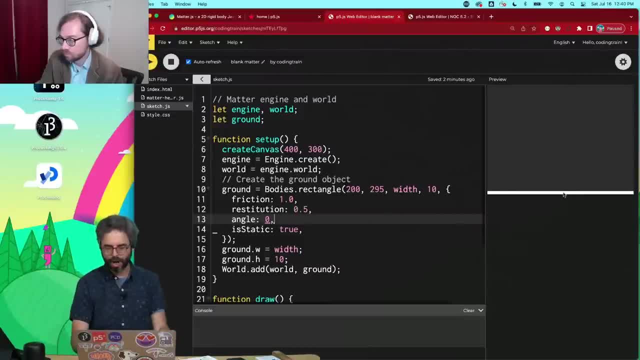 But so that's where this rectangle it's positioned at: 200 is the x, 295 is the y, very arbitrary number. It's about there Because I want it to be the ground, to be the full width of the window, the canvas, and 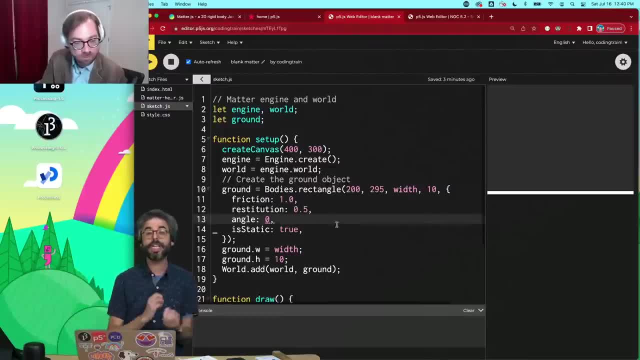 have a height of 10.. I gave it a little friction. Restitution is a variable that refers to the sort of bounciness of it, the elasticity of it, if you will, And then I'm saying it's static, It's a sort of something. it's like an object of infinite mass that can never be moved. 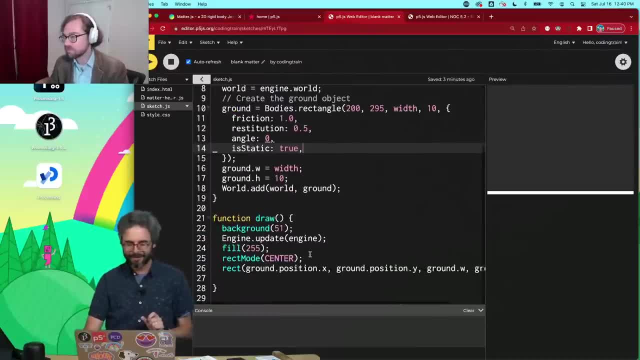 So that's the ground And that's where we're going to put the cart. I also just added a couple variables to this ground body so I could store I don't. there might be a way to access them through matter. If anybody knows, feel free to like let me know in the chat. 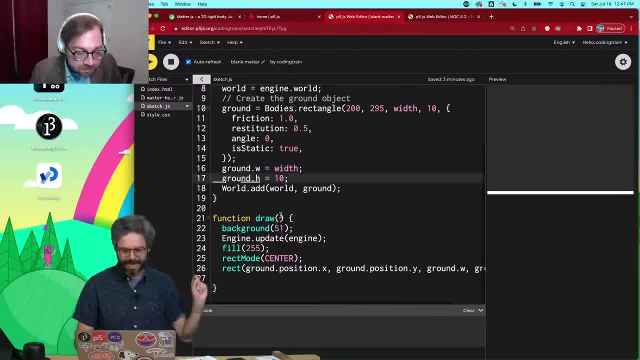 But I just put the width of it in a variable called w and the height in 10.. Because what I'm doing here in the draw loop, The draw is that same animation loop that Christian had in the Python code, that for loop, But here with P5, because we have a- you know- animation program that's showing us every. 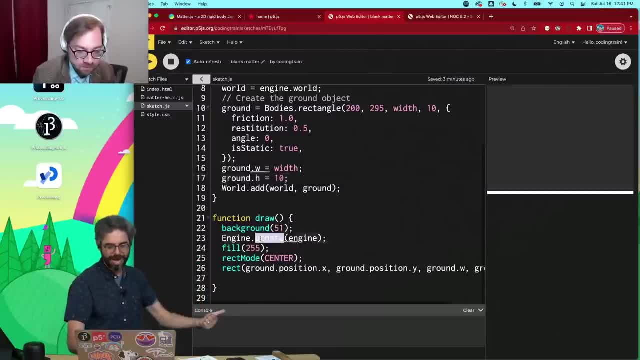 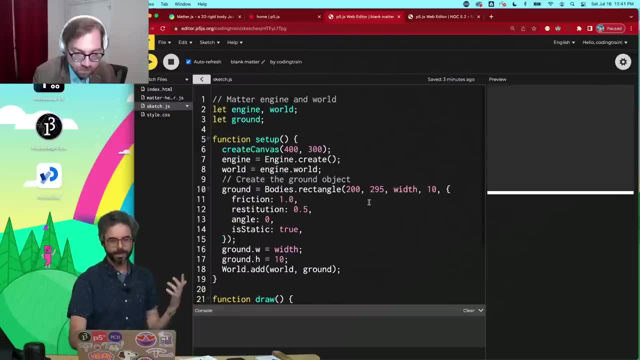 frame draw shows us each and every frame. So every frame, we want to update the physics engine and draw the ground at its X position, its Y position, with its width and height. So let's look at just adding a cart to the system. 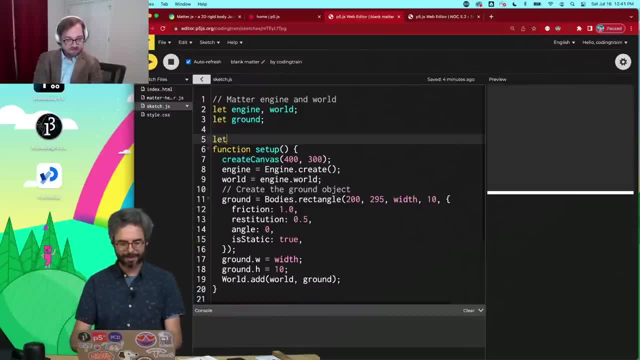 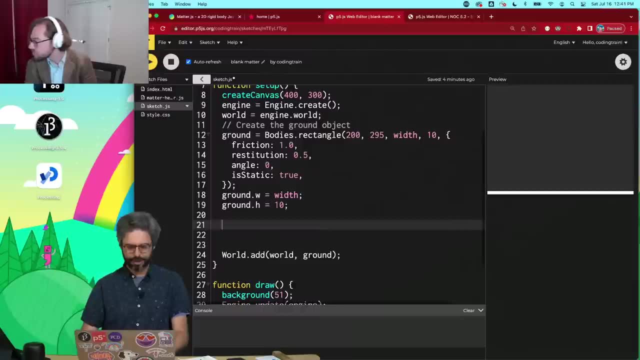 Yeah, And Christian, you should absolutely stop me if you have a question or if you notice a question from the chat. I'm not keeping as close an eye on it. So let's add a cart and I'm going to do the same thing. 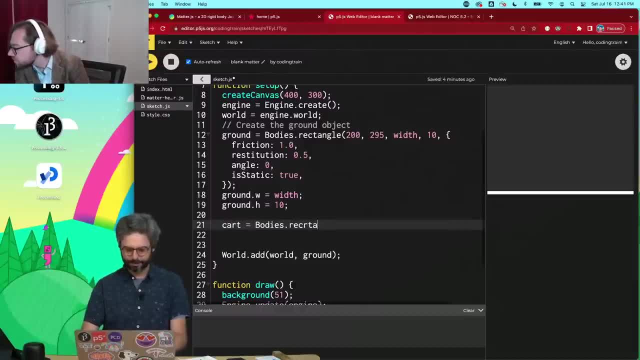 Cart equals bodiesrectangle. Let's put it in the middle. Let's put it So. I'm going to do a little like mental arithmetic, which is. I don't know if you've ever experienced this. It's really hard to do when you're suddenly like live broadcasting. 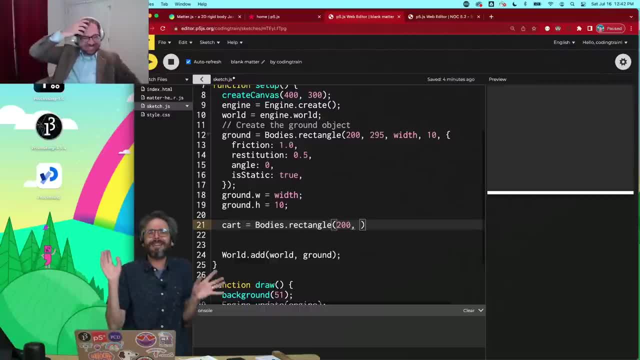 You know you're sitting at home drinking your tea. 295 plus five equals 300.. That's like you know I do that. you know you could tie all my hands behind my back and, you know, tape over my eyes. 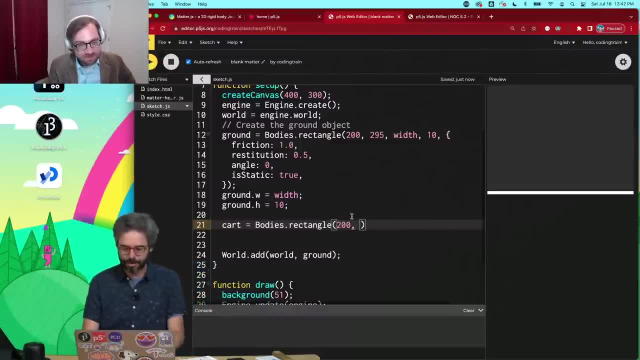 I don't know I could do that, But all of a sudden here I'm drawing a little bit of a blank, But let's put it at 290.. So five pixels up from the ground And then we'll give it a width of about 20 and a height of about 10.. 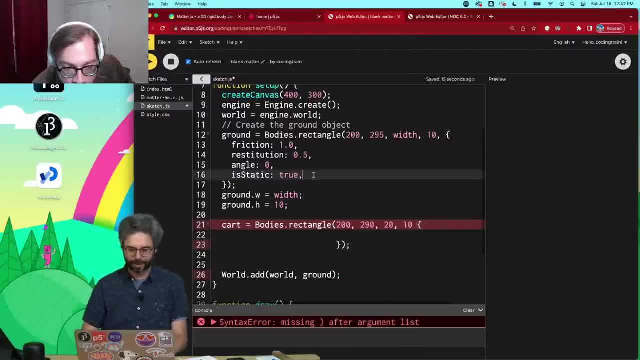 And then I need to also set these, all of these parameters. So I am going to just sort of like I've got a little syntax error here, which I'm missing a comma. I am going to, I'm going to, you know, maybe we'll turn the friction off at some point. 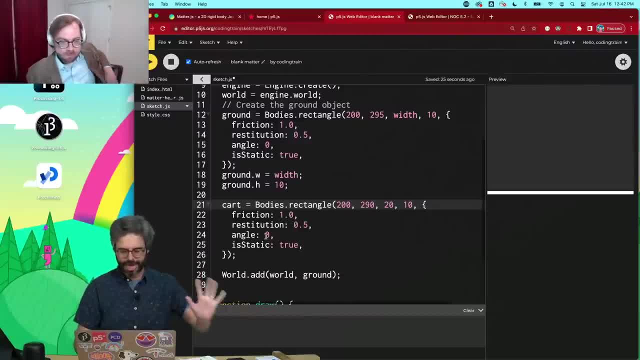 but we'll leave it for now, Just sort of base friction, base restitution, angle of zero. This is very important, though False is static, because this is not a static object. We want this to move. It would, And in fact, maybe just for the sake of argument right now, let's give it to y value 250, because 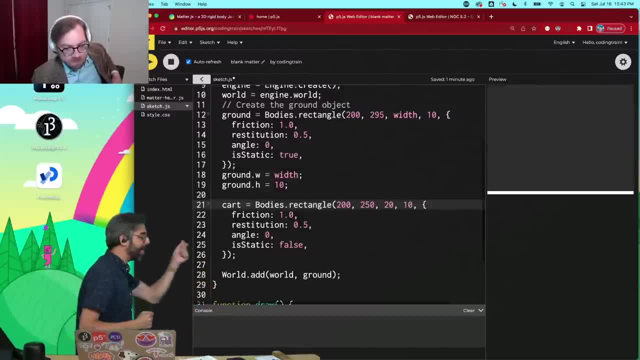 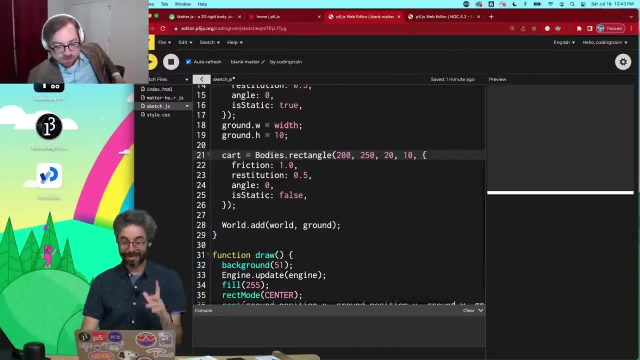 if everything is working, it should fall. Now two things. we don't see it on. We don't see it on screen. There's two things. What am I missing? You can think about what am I missing right now. I'm going to go. 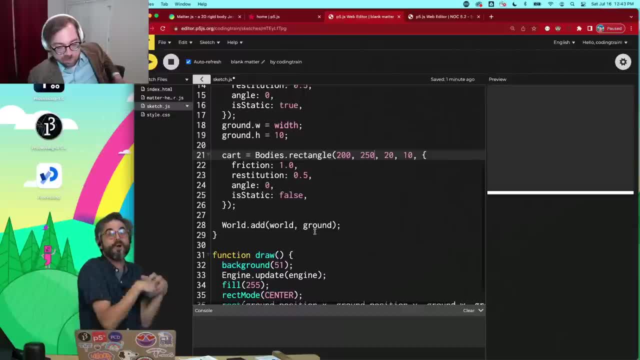 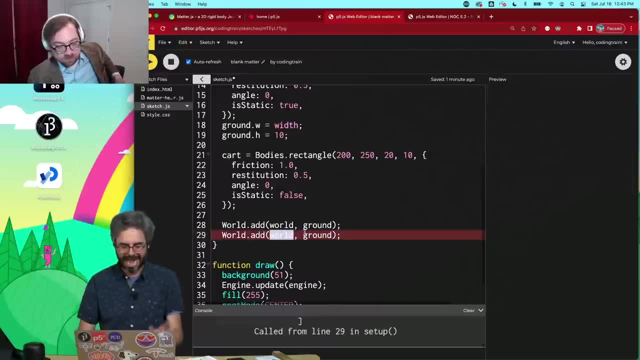 The first thing is, I can make a body, but it's not actually part of the physics, unless I add it to the world. So let's do world add and add this cart. Oops, no, no, I add to the world the cart, but we also don't see it because- and matterjs, I believe. 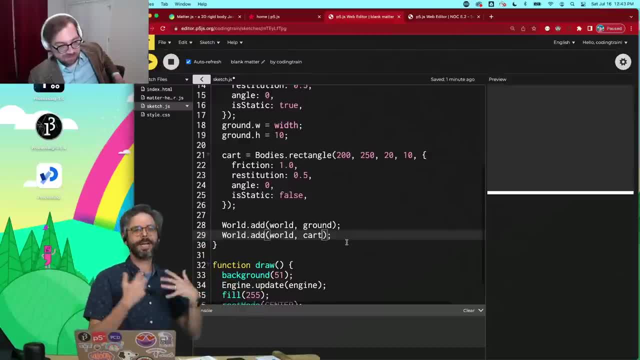 has some functions that will sort of draw things automatically to you. But again, the sort of ethos of the coding train is: I'm demonstrating sort of algorithms and behaviors And you, the artists of the world and programmers, will put your own creative twist on this. 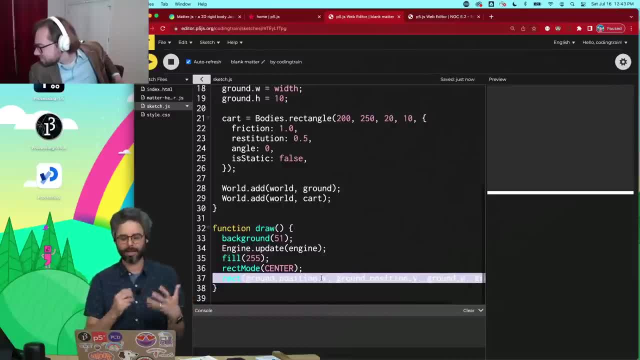 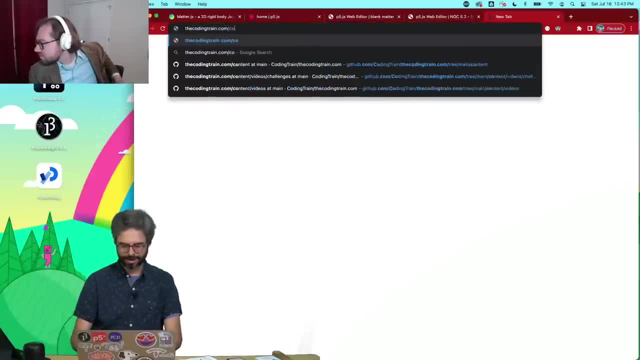 So I think it's sort of good practice for me to always be, additionally, drawing the elements myself. So let's draw it with a nice. we'll use the coding train colors. So I have this little website which has a bunch of colors we'll pick, and maybe I could. 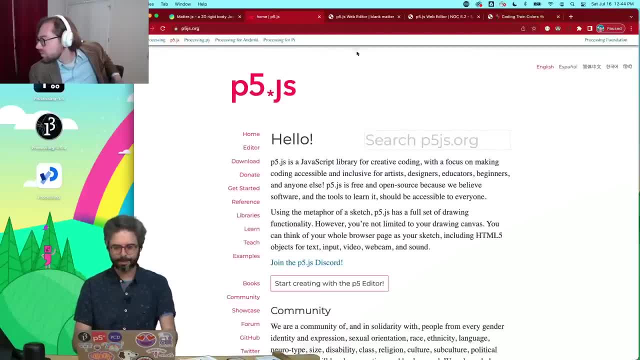 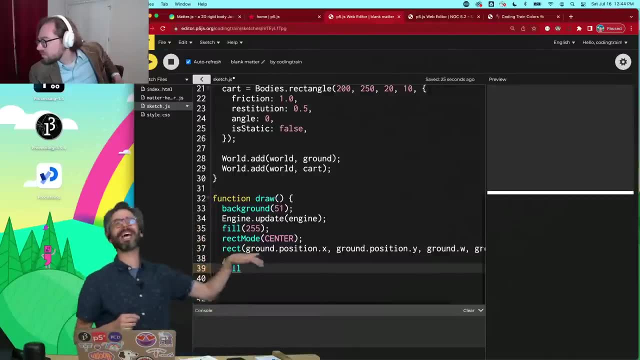 let's pick this nice blue and we'll set that. Oops, We'll set that to be a fill And I, by the way, I totally forgot to duplicate The sketch, So if you go to that link at any point, apologies for this. it's actually going to be where. 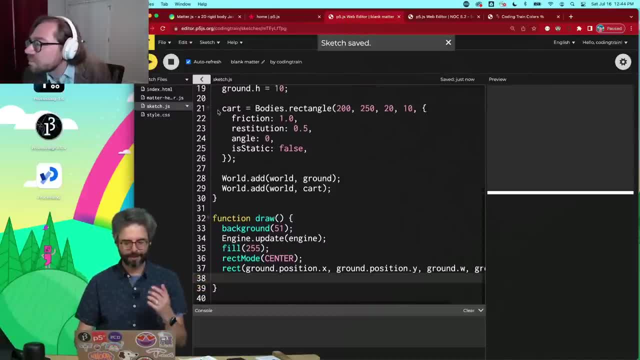 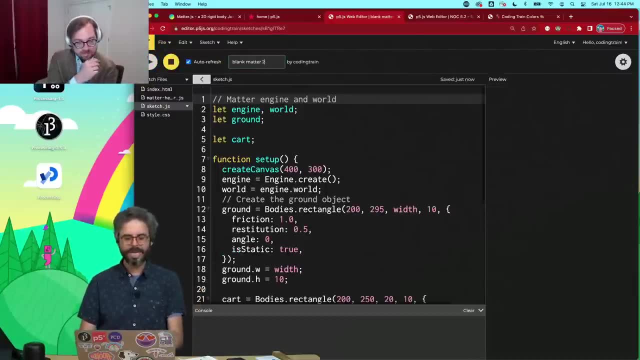 I am with the code now. Why don't I duplicate it now? That way, this is the sort of new base code. if somebody wanted to actually start along, So I'm going to do, I'll just call this. I'll rename all these to something more that makes. 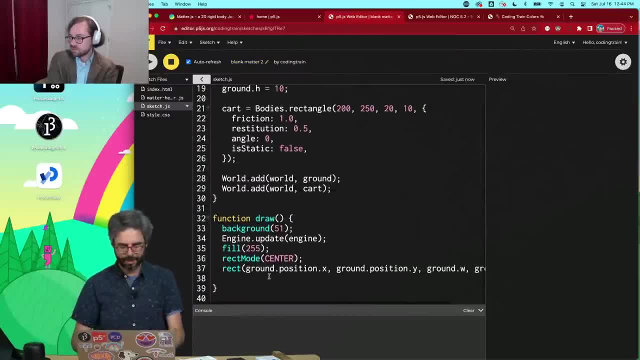 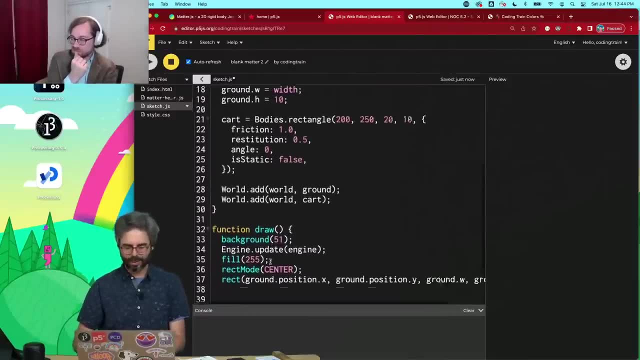 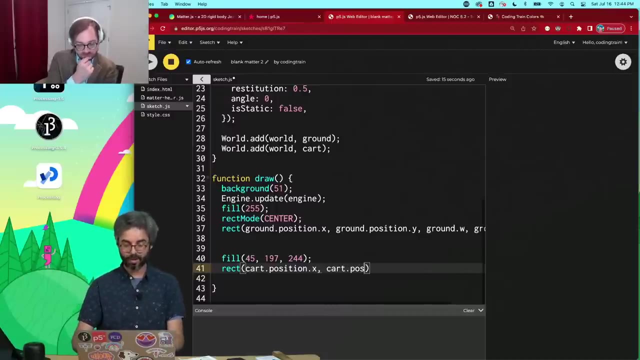 more sense later and link them into the description. Okay, So let's add a fill of that color. Let's put a rectangle at now. What is it? The cart position is very long winded, One of the reasons why I don't. if you, if you've been paying, if you're like a, a person. 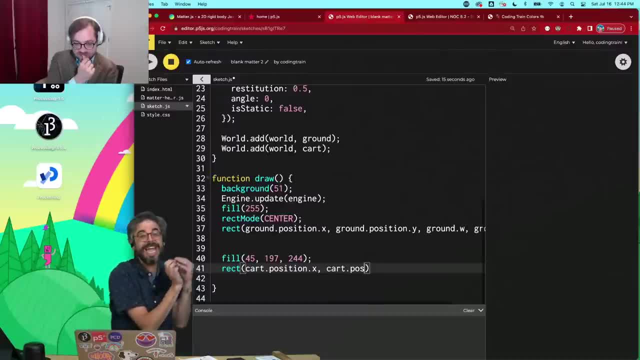 who's seen every coding train video ever. you would know that I usually often take these matterjs objects and wrap them inside my own class, my own objects, to be able to have more control and authorship over them and kind of keep the code a little bit more concise. 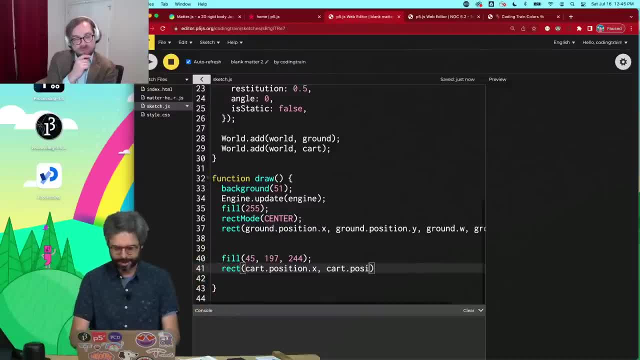 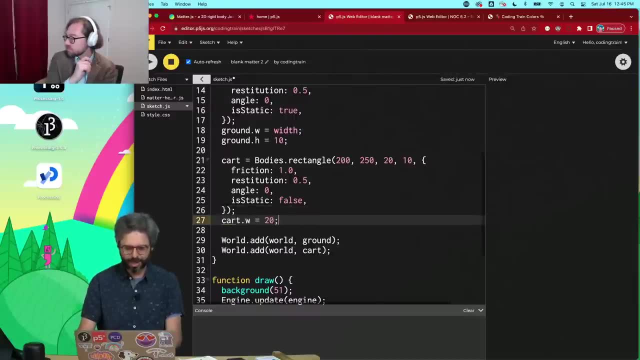 But I think for today's demonstration, it's simpler just to use it directly. So we're going to draw it at the Y and I'm- this is a my little weird hack- where I'm going to give it a width of 20 and a height. 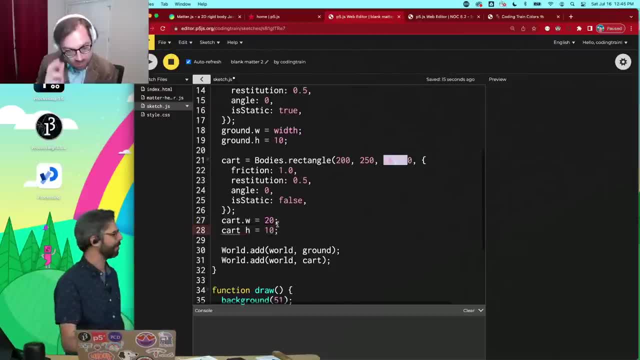 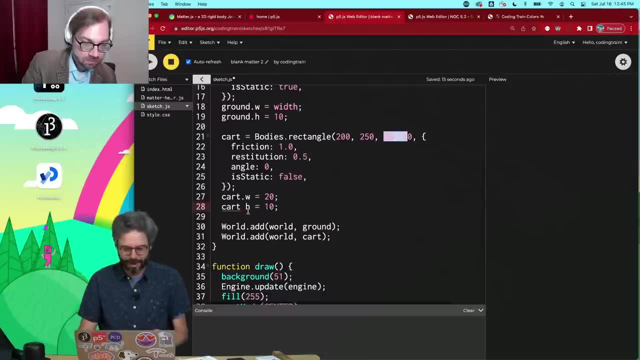 This is sort of bad practice in that I have these kinds of redundant variables And if I update one and forget to update the other one, it's going to cause problems later. but you know, we'll refactor this later. Maybe I'll look into how matter works a better way to. I know it gives you the vertices. 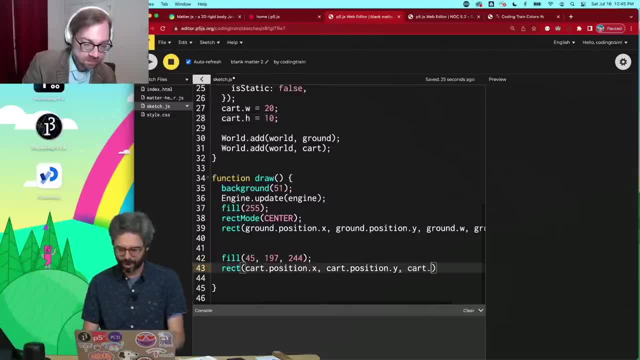 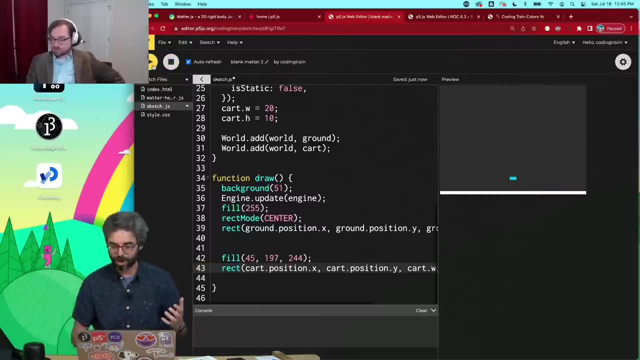 of the geometry so I could sort of pull that dynamically. but now we can just say cart, W, carth, And let's run this, Okay, And we can see. there we go, So we can see the world. Things are working. because as soon as I run the sketch and I'm at the, the cart is falling. 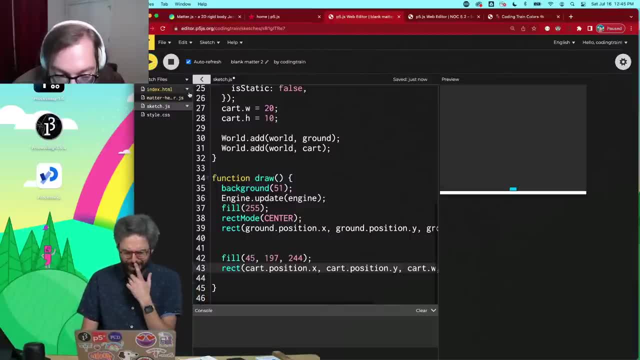 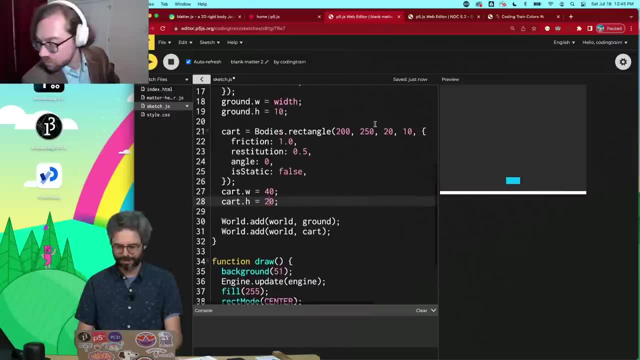 So we could always have it fall. but let's position it, and it's so small. Let's, let's make things a little bit bigger And we'll see what I mean. I have to now change everything everywhere in its position so that it's actually falling. 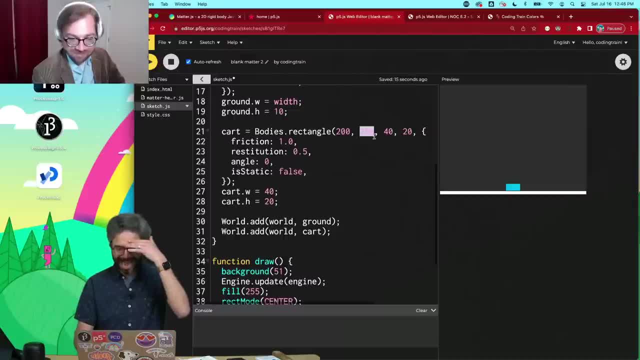 It will actually settle in the right place. Let's put it at what- Oh, I've lost track of. the ground is like 10 pixels from the bottom. This is 20 pixels high, So I think the bottom is at so height minus 20,, which would be like two 90.. 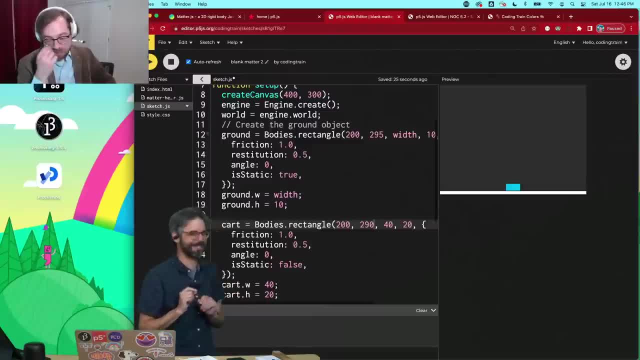 That should give us a good plot. All right, Anyway. And it's going to adjust itself because matter is like smart being like no, no, these two things can't physically be in the same space. Let's push them apart, Okay. 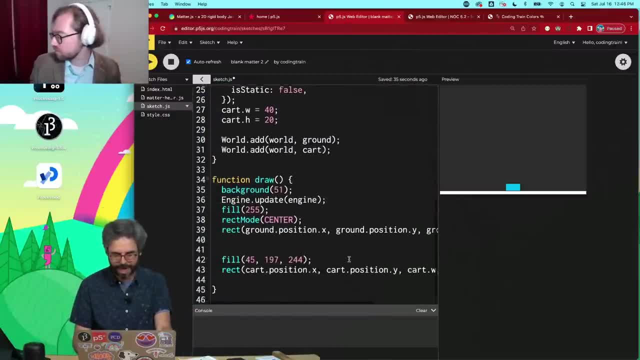 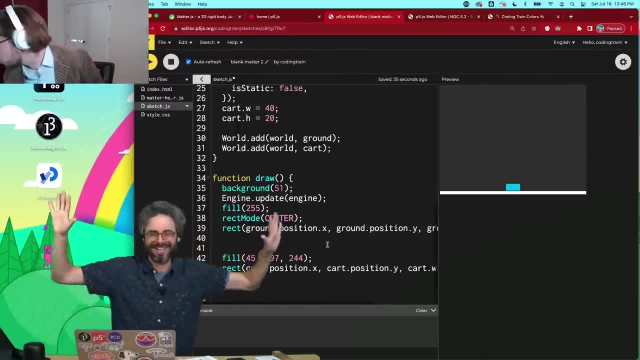 A carth. Did I forget that somewhere? Somebody's saying in the chat: no, it looks like I'm good, Okay, So great. So we've got cart pole. I'm not, No, no pole, We have cart. 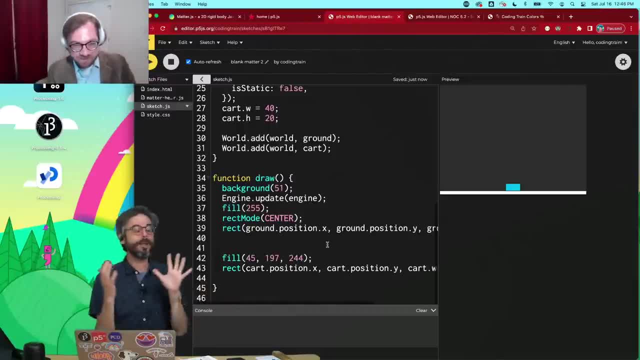 We just have cart We're. we're maybe going to get to cart pole. We'll see I had. by the way, the planned amount of time for this stream was till 1pm, which is about 15 minutes from now. 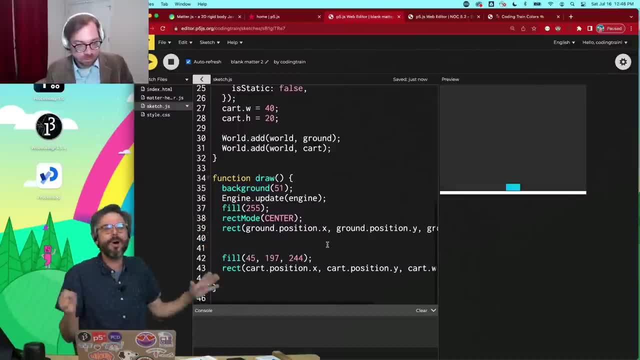 Do you have a time that you have to go by, just so I could keep that in my head? Okay, I don't want to look, I always I'll grab a drink of water, if that's all right. Yeah, So yeah, you can. you're, you can go have a little break to yourself at any point. 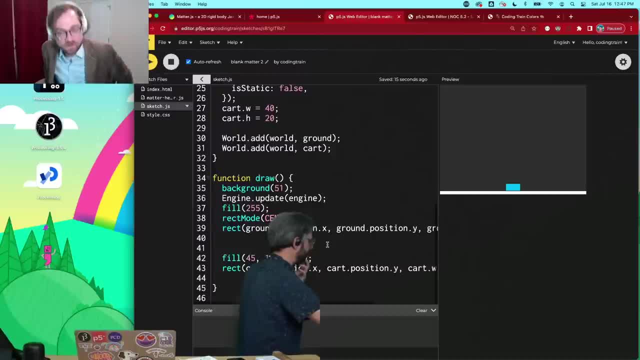 I can actually also, uh, remove you, Um, but just bring me back in a minute. I'll, just as long as you're okay, Be jumping, Yeah And talking about the controller. That's cool, I'll just grab it. 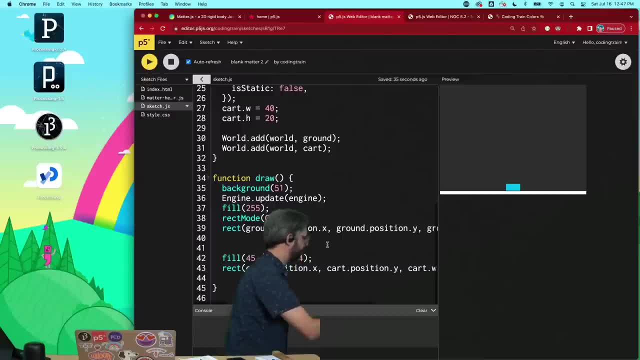 I grabbed my, my water bottle. Okay, You are off. Uh, Christian, you might be able to hear me, but your audio and video is no longer on stream. Okay, Uh, so Johnny is making a good comment, which is: maybe we should start the wrapping into. 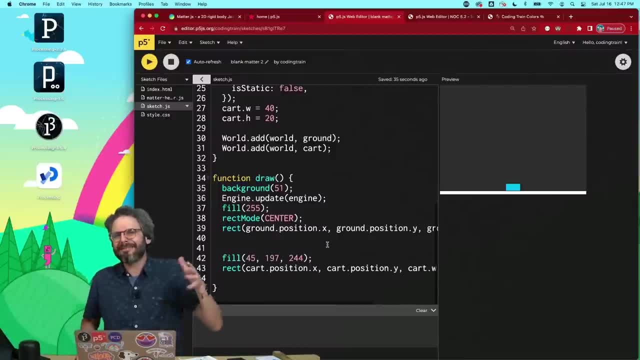 classes sooner rather than later. I would agree with that. Really, I mean, that's a very good point. I think I'm just going to hold off. I think I'm just going to hold off because I ultimately, I think I might come back and 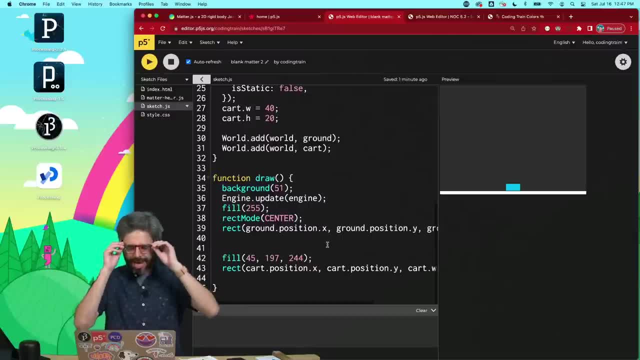 record, do this again as more of a coding challenge video, And I might think more about it, might do it without matter, but let's, let's, let's keep going here. So I'm going to now add a force, So we're going to create a variable. 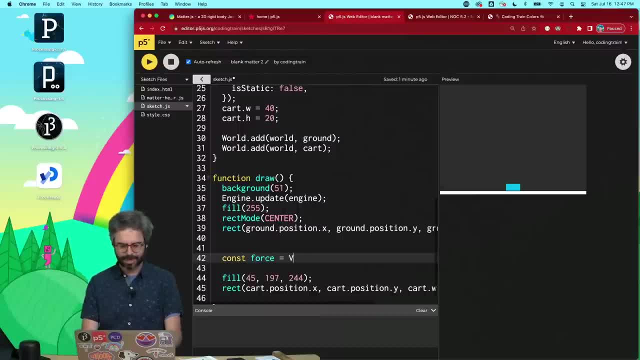 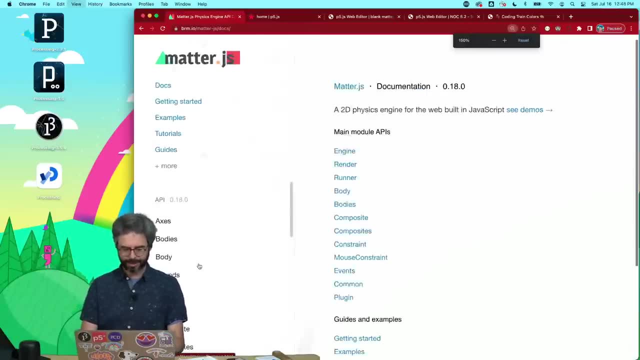 I'm going to call it force, I think, the proper way to do this. let's let me just show you how I figure out how to do this stuff. If I go into the documentation here and let's make this a little bit bigger and I go under. 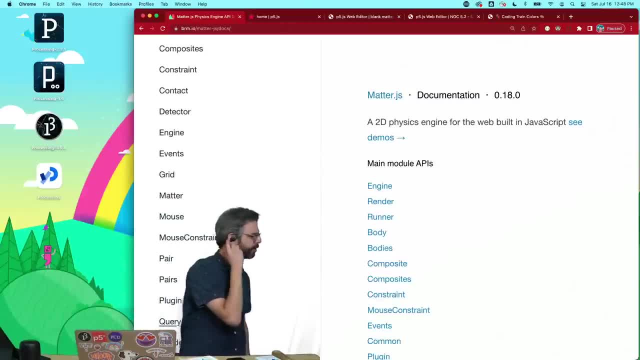 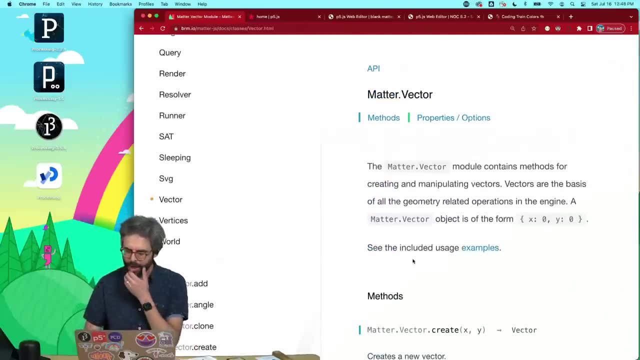 a vector And, I think, Christian. hopefully I can still hear you So when you're back just talking to my ear or I'll just check in a bit. Um so um, basically I want to create the force as a vector so I can use mattervectorcreate. 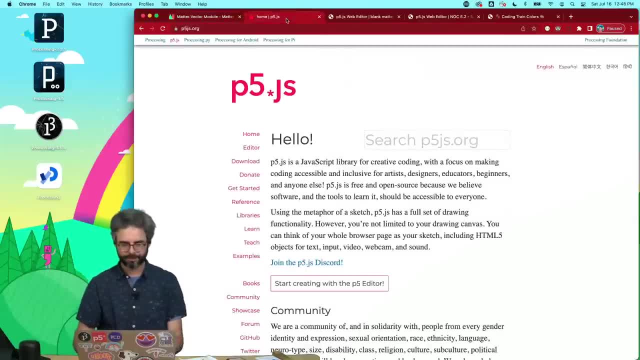 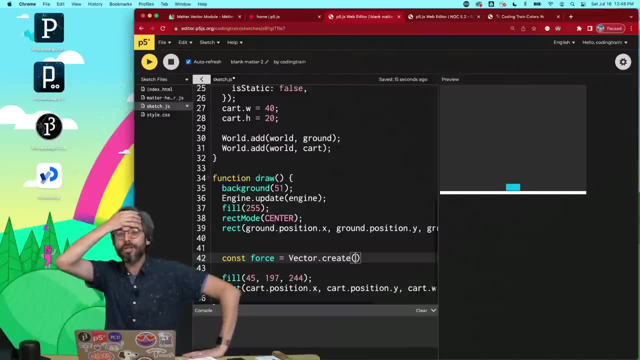 or, in my case, just vectorcreate and let's go back to here. vectorcreate and let's make a force. Now again, what are the units of measurements? Uh, the units of measurement are pixels, And we're going to have to just make our best guesses as to what makes sense. 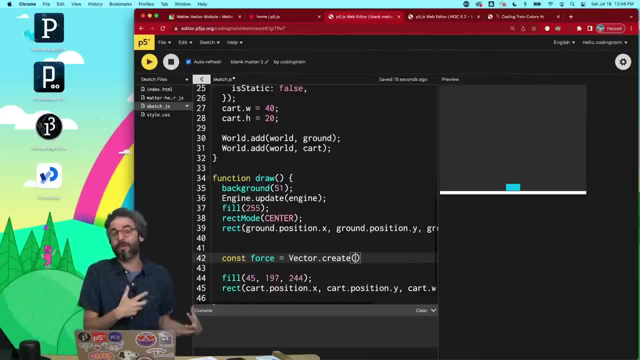 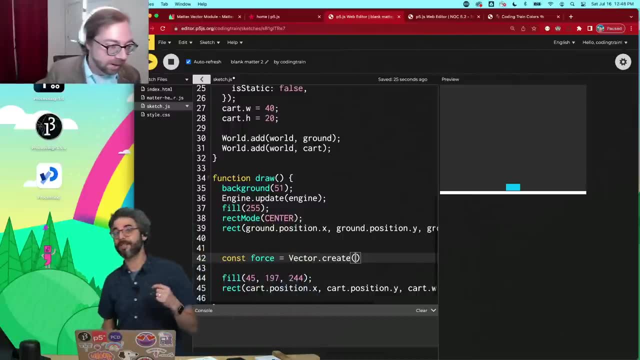 Uh, uh, you know I've talked about this before when using like- and I'm going to bring Christian back here- Um, let me just press this button. Great, I've talked about, like, the physics engine box 2d, which is uh, was famously used for. 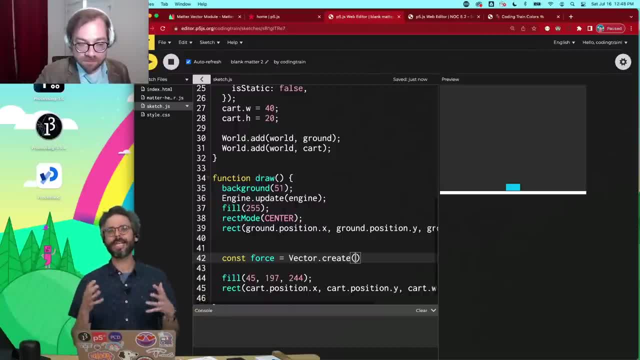 gay. uh, you know it's probably still used, but at least for early kind of casual physics games like angry birds. Um, and that is a physics engine where the units of measurement are real world. They're meters, They're seconds. 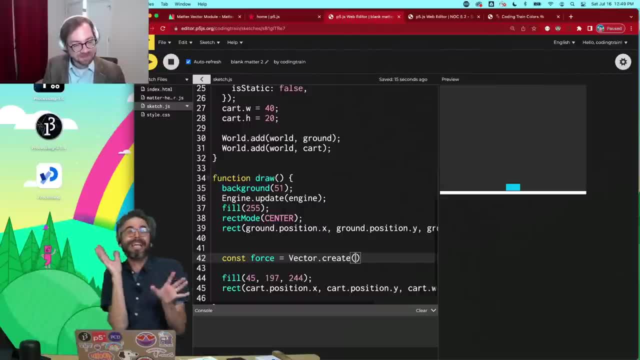 And then you have to do all the conversion before you draw them into pixels. I like, I actually like an engine like matter, because of the simplicity that I can. just my unit measurements is pixels. So again we have some issues in terms of real, you know, stimulating true, physical, 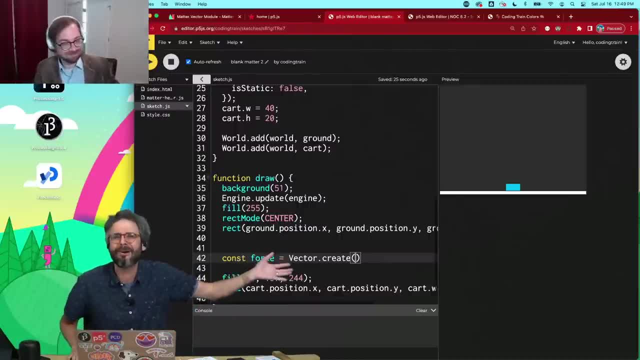 reality. but you know again, this is only a 2d world, so that's not even a real thing anyway, Although I, uh, uh, uh, I, I'm, I'm getting off track. So let's make a uh, a vector, that just uh, one zero. 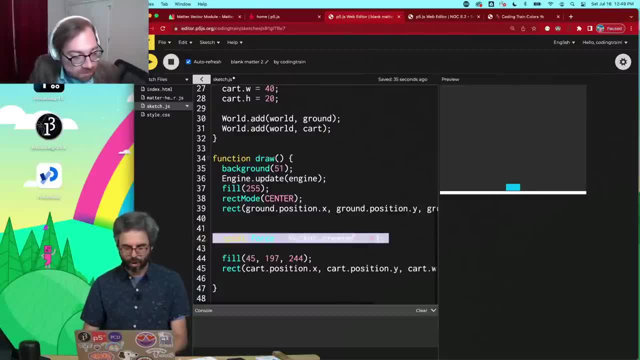 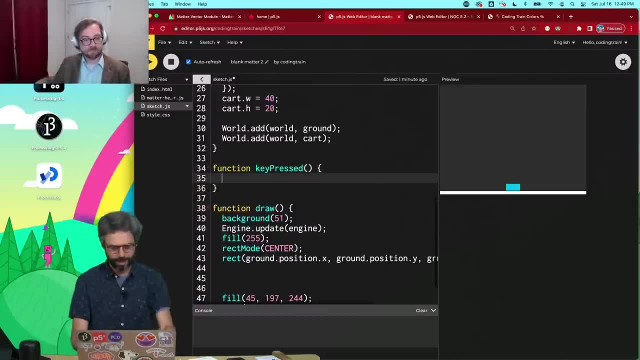 And actually what I'm going to do is let's see if we can control These, force, control the cart, just to get started through key presses. So I'm going to add a key pressed function. I'm going to check if the key code is right arrow. 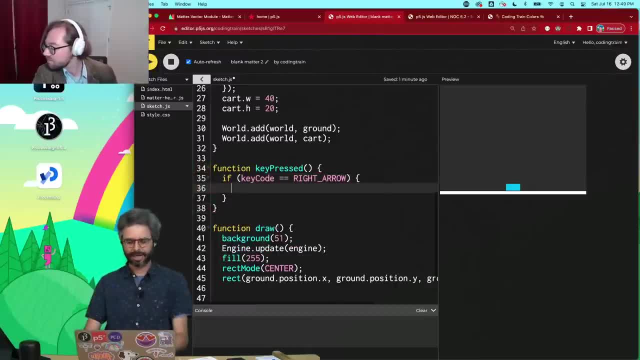 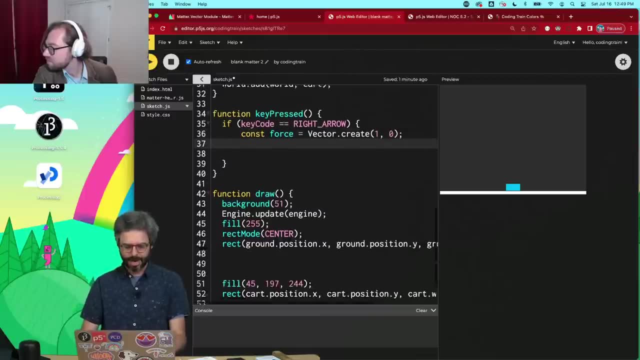 And these are all built in variables to P five that let me build an interactivity really quickly. Um, you know, I could put buttons on the screen and do other things. I'm going to create this force and then I'm going to say: and I now I don't remember. 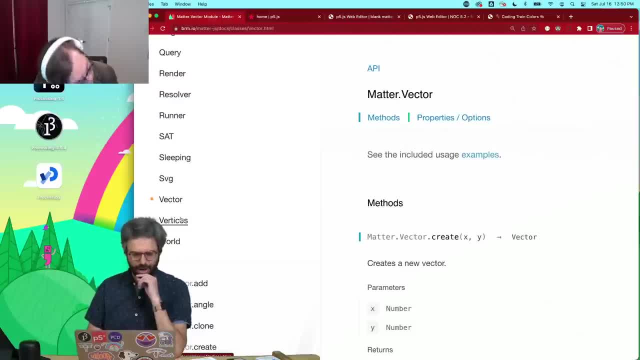 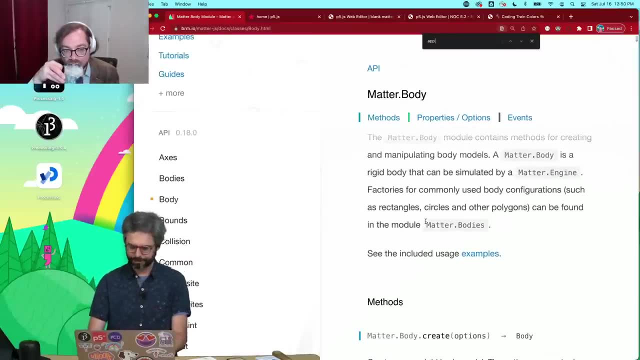 how to do this. So I think it's under uh uh, uh uh, by default. Uh uh, body. Let's take a look. Uh, I think there's a body: apply force function. Yeah, So I need to apply the force to a particular button. 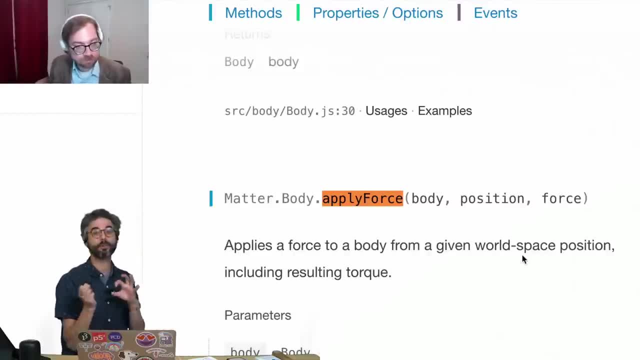 So the force is the vector I'm applying. That'll eventually be the force We calculate through PID or just our PI PD. I don't know. I don't know that we're going to get to the eye here in the JavaScript version. 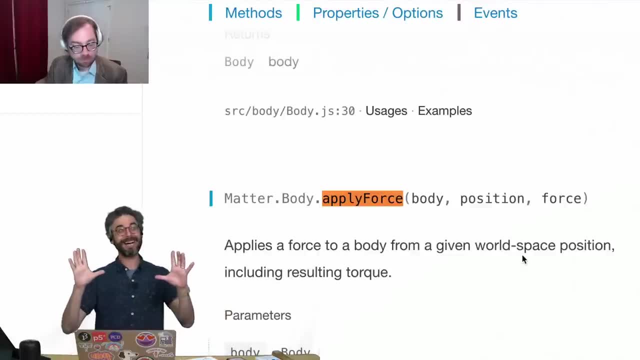 Um, the position uh is interesting because, uh, while in a lot of my examples I just consider all objects Like, Like a single point mass, So it's like there's no geometry- We can actually apply a force to like the top left edge of the cart or the bottom right. 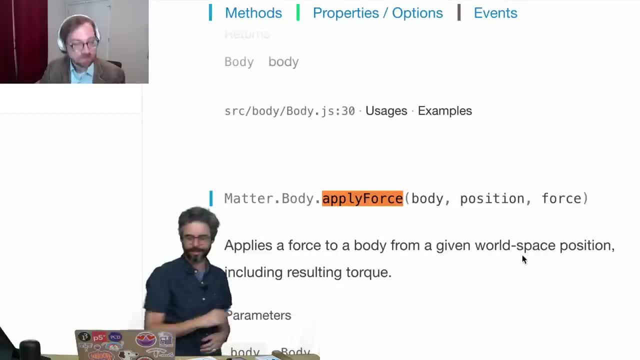 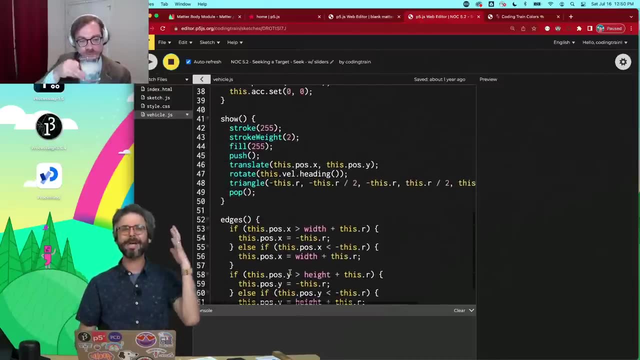 edge. But I'm just going to apply the force to the center of the body and then the body, So I can go now into the code and I can say whoops, um, every time I say whoops. now I have this like I can't help, but stop for a moment. 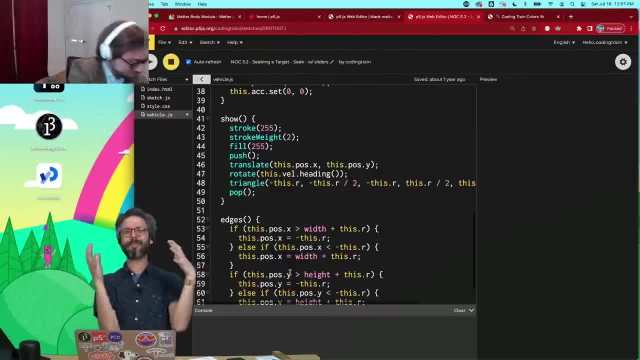 And then imagine cause I have- I don't know if you probably haven't seen these, uh, Christian, but I have these like super cuts of me. It's over and over again, with all these different videos, that I make a lot of mistakes. 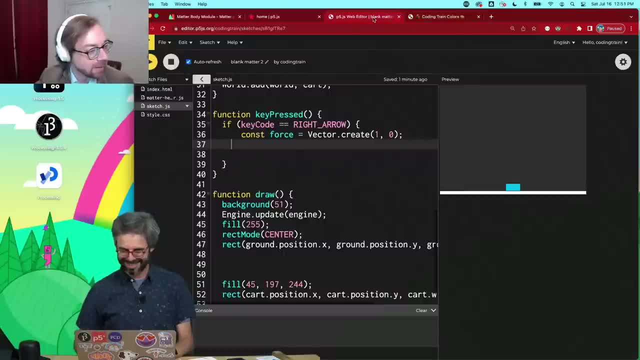 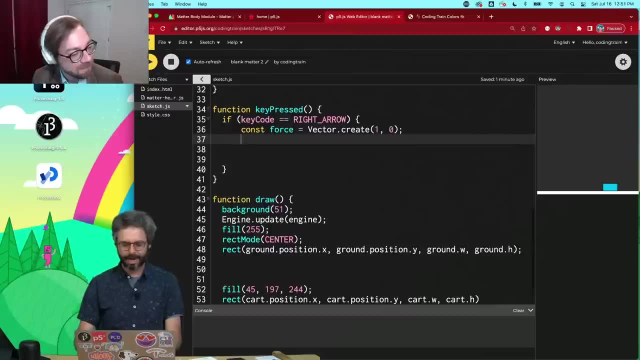 I say whoops all the time. Okay, Where am I? I pray no one does that for me. too long of a video, Yeah, Uh, okay, So force. then we're going to say a body dot, apply force. We're going to apply it to the cart. 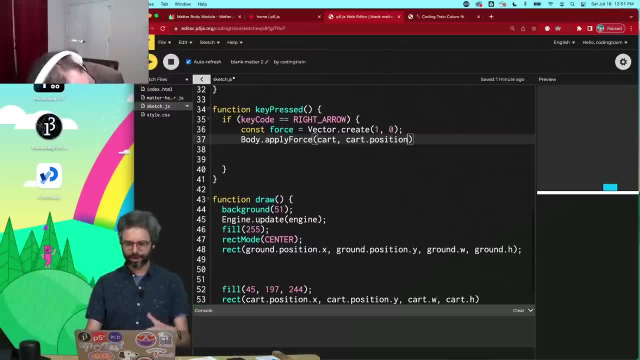 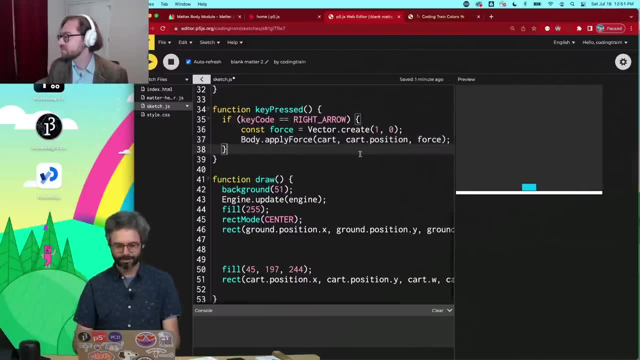 We're going to apply it just to the cart's position, So the center of the cart, and I'm going to apply this force. So I'm assuming, if all goes well, Okay. And also just note I have this auto refresh on, which is a little bit risky, because if 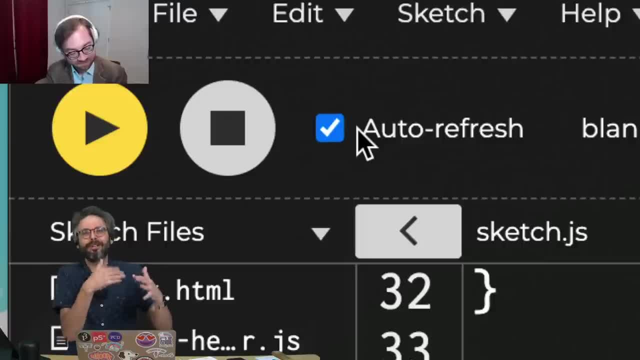 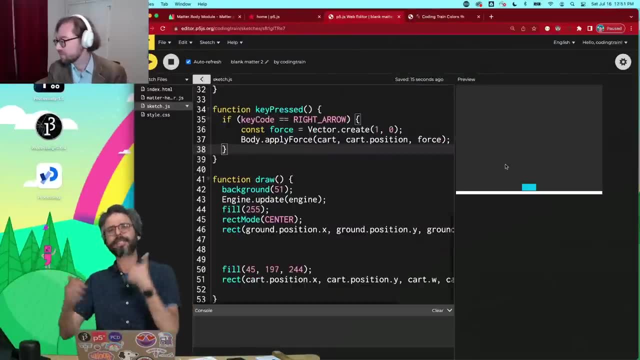 you if you write, if you're writing a for loop and you have auto refresh on and you don't get the exit condition in there, sometimes your code is going to restart and then get stuck in an infinite loop, but it allows the sketch to like continually update as I'm editing. 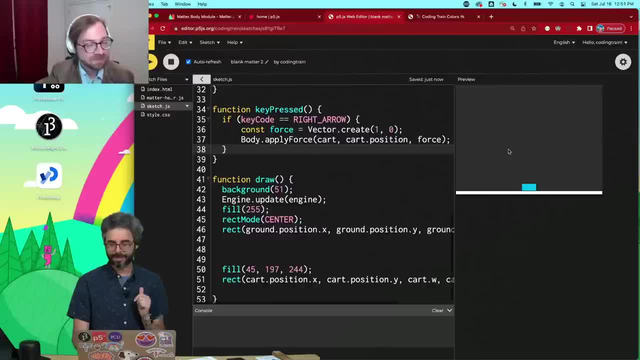 the code, which has a lot of convenience for it. So, let's, let's see what happens. Whoa, That was kind of a big force. So we know that the, the, the uh values we want are should be much smaller. 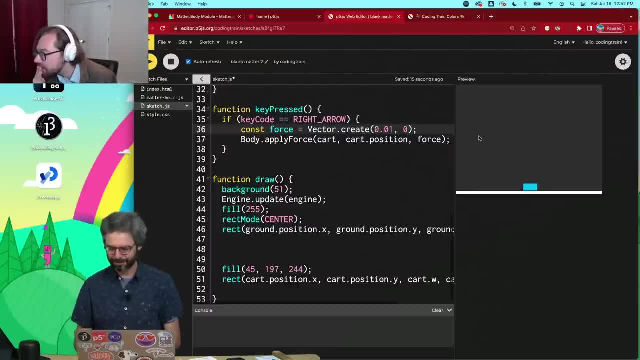 So let's try, uh uh, a smaller number. There we go. We can see I'm kind of like pushing it along here. now it's kind of like jumping up into the air. I'm not going to worry about that too much there. 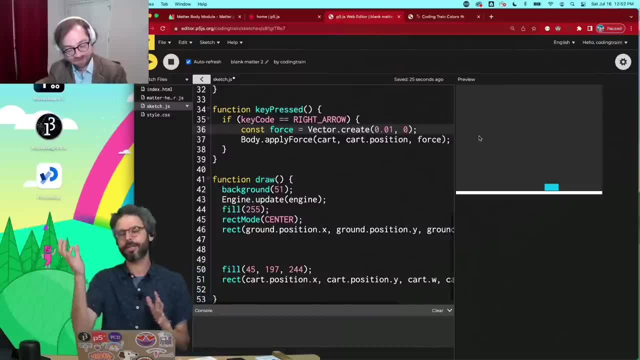 There probably is a way that, uh, you know there are constraints. I'm going to use a constraint if we get to the pendulum, Um, but there are all sorts of ways that I could think about it more as like it's got. 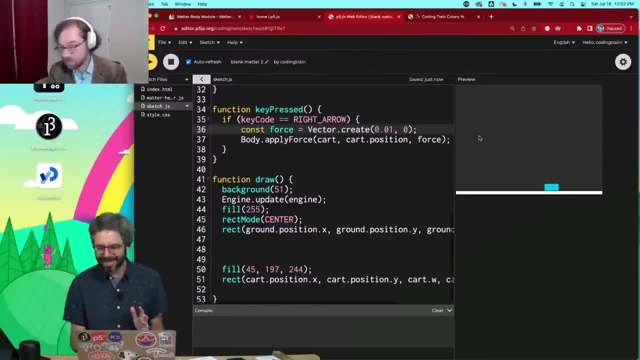 wheels. it's locked to a track. What's the friction, what's the grab? but I'm going to let this be a very raw and sort of just whatever kind of matter does by default. Um, So let me see, this is working. 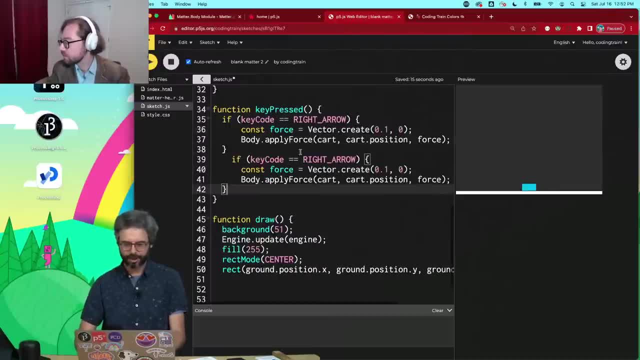 Let's make the force a bit stronger and let's also, uh, just add in a force for the left arrow. Obviously, there's a lot more sophisticated ways we could do this, but just hard coding in a negative force. Oh, look at that. 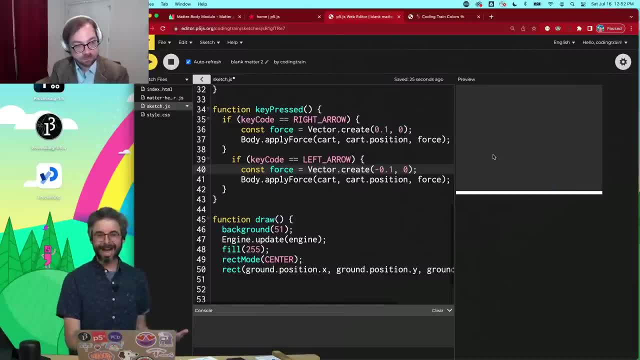 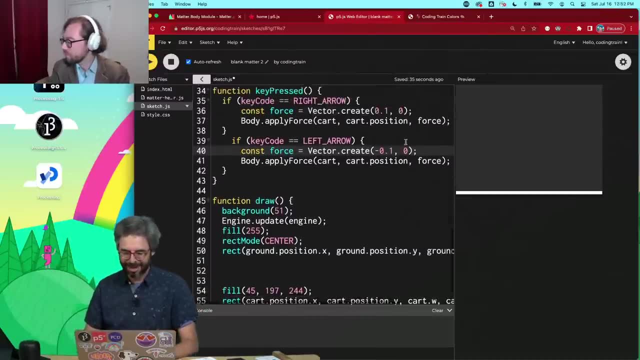 Whoa, Look at it, Maybe I'm like it's a flying car, Like I. uh, we've got space X going on here just with like a little, uh, horizontal force. I wonder what the lift off is from. uh, it's interesting that that it's uh, uh sort of. 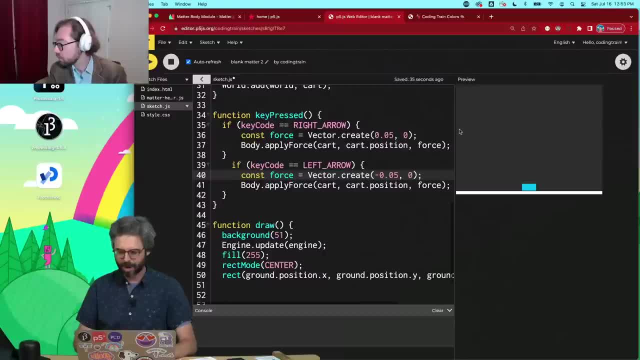 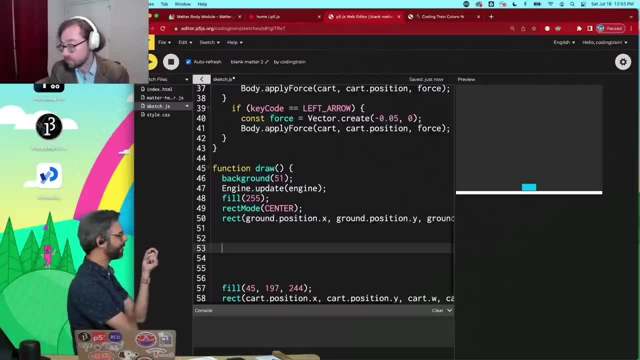 occurring and let's. so I'm going to stop worrying about uh tuning this Cause we're not really there yet. So the idea now is that what I want uh is to have to, if I'm recreating, and stop me. 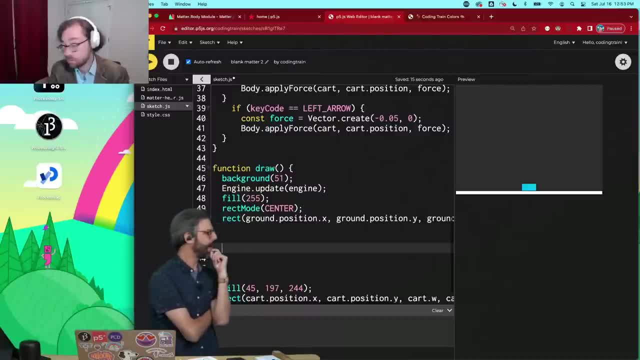 if I've got this wrong. um, uh, what I want to do is say, like I want to have a controller move the cart to a desired X location. So let's say, uh, my desired X, And I'm just going to call it desired for short. 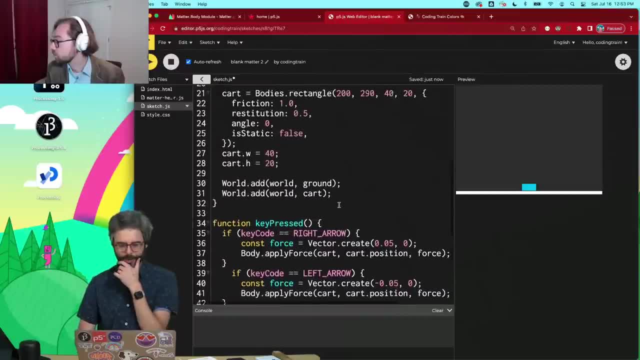 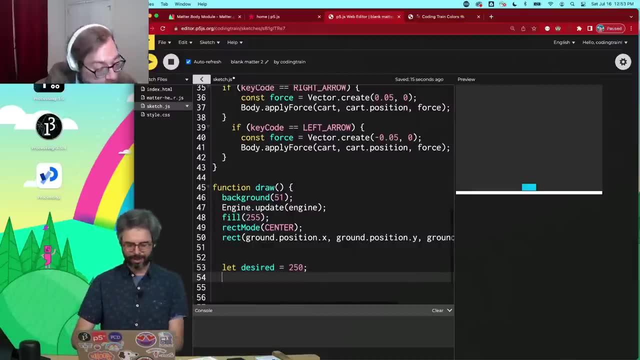 Okay, Because I'm not going to use a Y in this case. uh, uh is um 250.. Okay, So now the next thing we need to do is calculate the arrow, which would be the desired minus the cart's actual position, but getting this right. 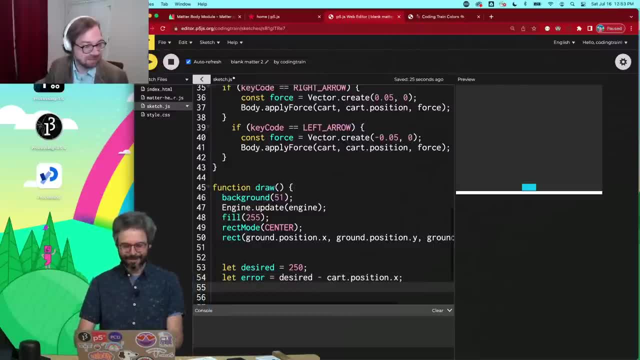 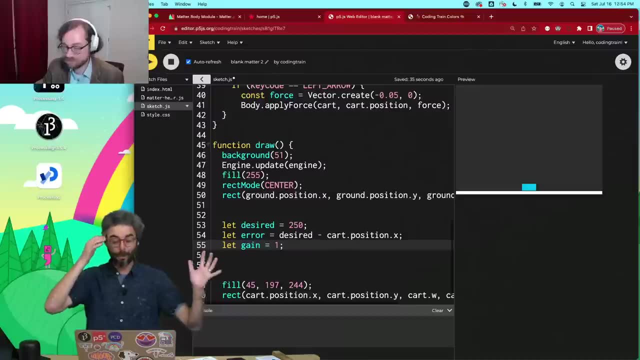 So far, Okay, Perfect, So far. now we need: now we need a game. Now we need a game, right? So let's just try a game. Let's just start with it, Okay, So let's start with this. 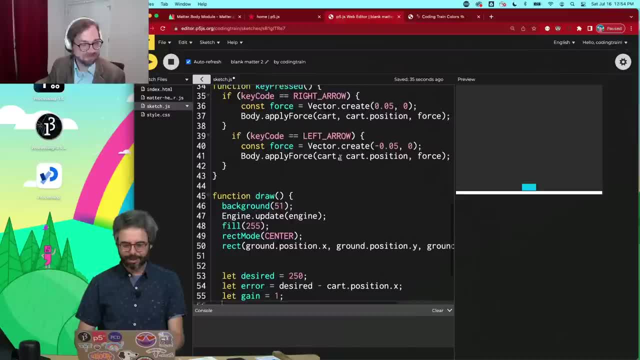 So we're going to start with it. We're going to start with this value of one right, Because I have no idea what it should be, And then the idea here is that I'm going to create this force now, not with keyboard control. 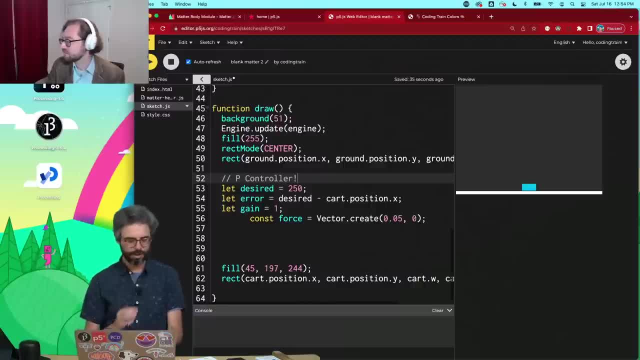 but with my P controller. So this is the P controller I have the desired position in. in one dimension I have, which it could be a vector That's, I assume, Correct, Right, Uh, a two dimensional vector, That is a three dimensional vector. 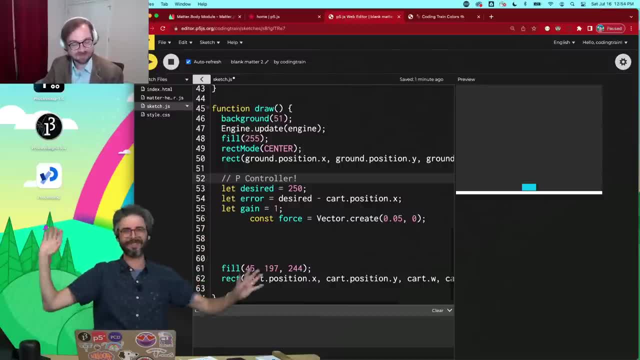 I look forward to seeing all the posts of people doing this in unity or three JS, hopefully, uh, that you'll share back with me. I have the gain, and then the force is just going to be and I'm going to just make a. 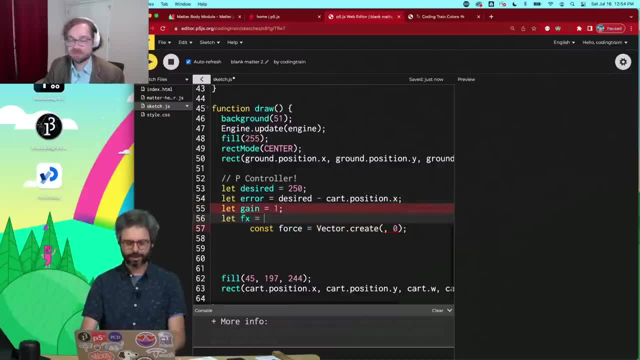 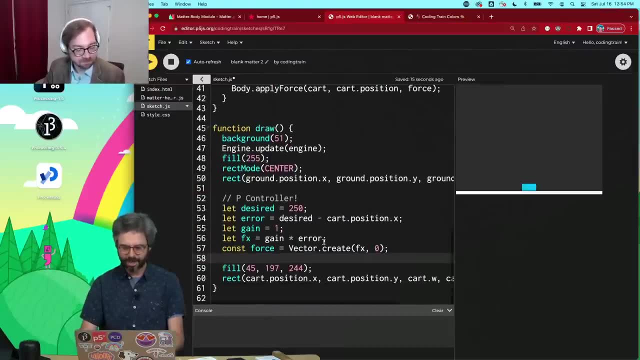 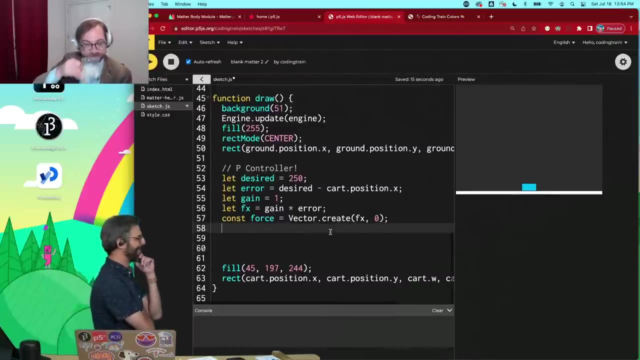 variable called fx, which I'll say is the gain times the error, And then I'll create an actual vector- Again I'm oversimplifying here- to just eliminate having to deal with any vector math or the why. but how's this looking so far? It's looking great so far. You got me in the perfect. 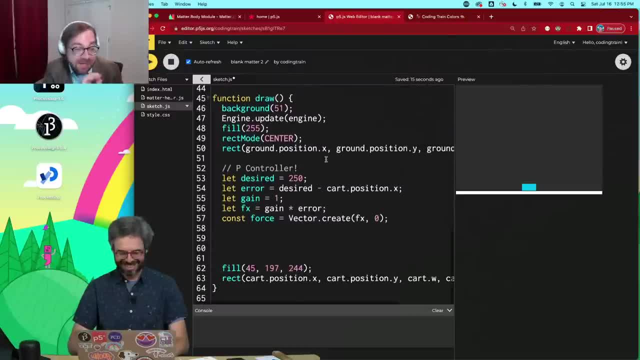 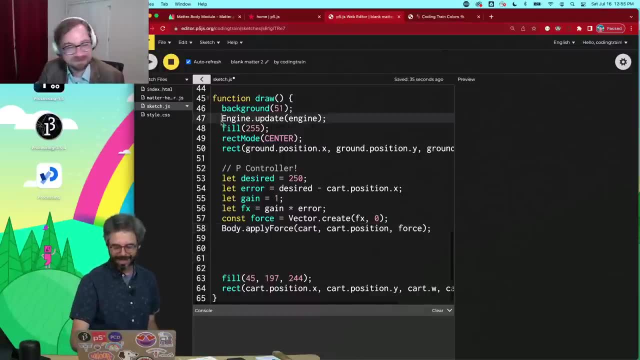 time, Let me drink my water, Sorry, Yeah, Yeah, It's perfect. This is yeah, Okay, And now I'm going to apply that force, So I'm first thing I'm going to do. I like to do is I often just? 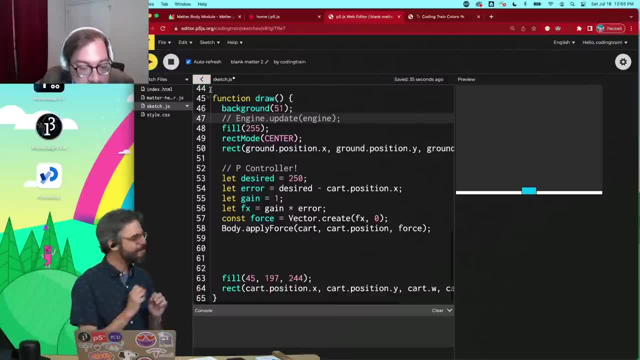 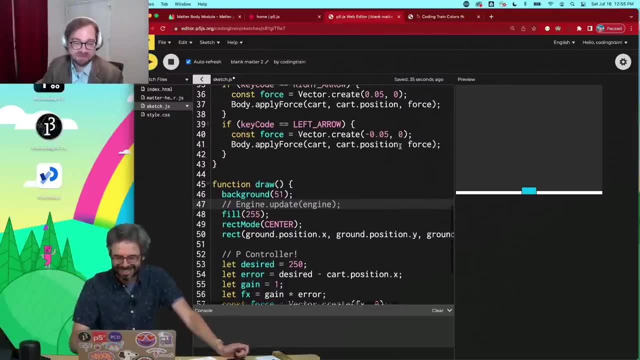 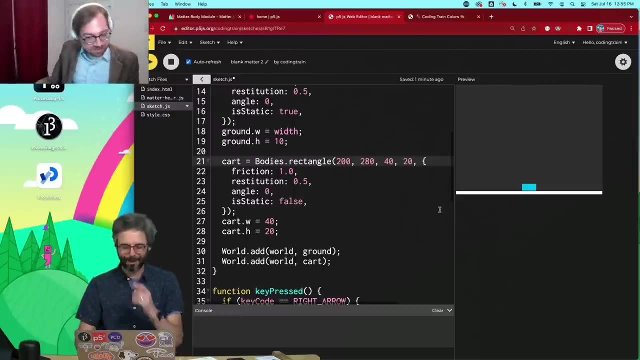 turn the engine off. So okay, So, ah, I see why it's jumping up in the air. These are the. see, my, my, my little bit of arithmetic was off, So let's move this up. Just, I just want it to start more at the. there we go, at the proper spot on top of the ground. 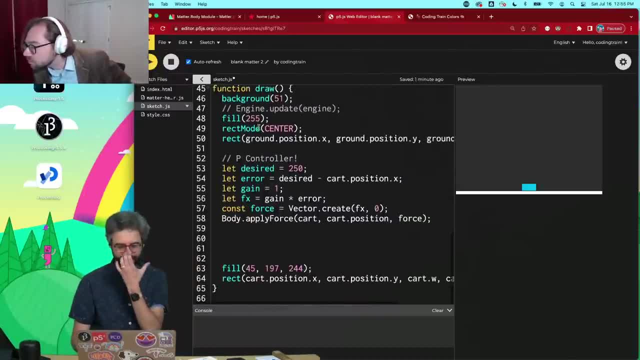 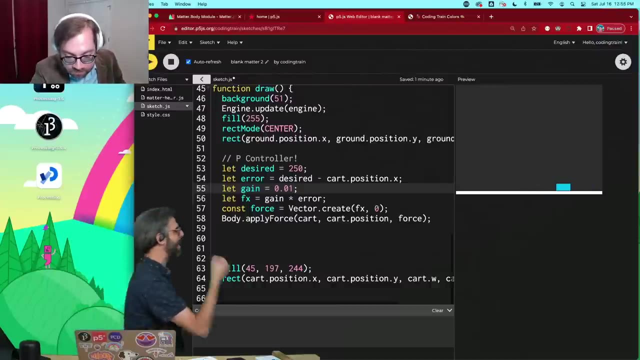 So now that the engine is off, so no physics are being applied, And as soon as I turn the engine on by uncommenting this line, it's gone. So this gain is clearly much too high. Let's give it a lower gain and we can see we've got this unstable oscillating behavior. That's what you would. 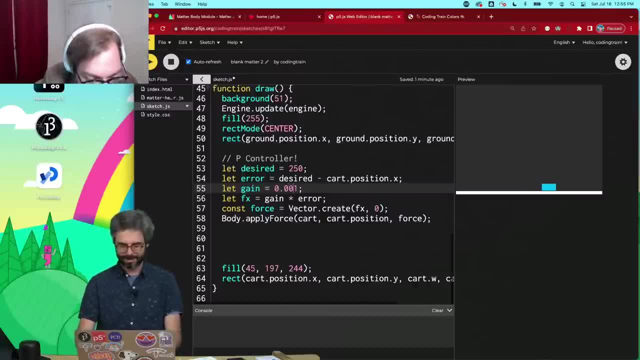 expect, right? Yeah, Yeah, Yeah, So that's a, so the gain is currently 0.01.. Oh, there we go. Yeah, It's probably because I imagine pixels is a very tiny unit, Yes And so. so, as a result, it's not meters, It's like. 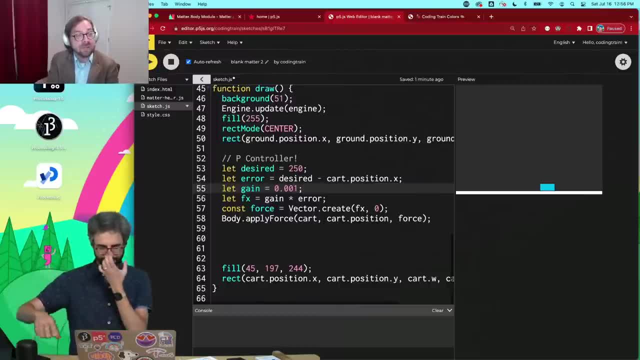 there's probably a ton of pixels during that on that thing. So that makes sense. So so people have to consider what the units are of their gains. It's like force per unit, distance for the P gain and distances in pixels, And I'm guessing when you get the velocity it's going to. 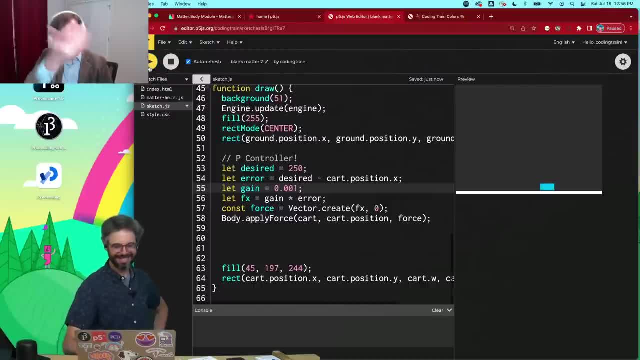 be pixels per second. Right Is what we're going to get. So that's perfect, It's. I'm kind of fascinated by this levitating behavior we've got Again, even though I'm choosing to ignore the Y value in terms of this, this world, this physics world, is not a one. 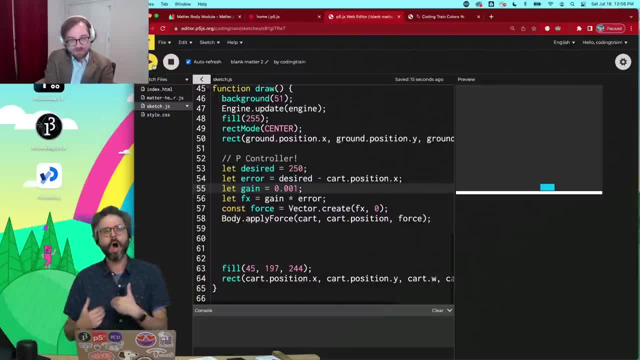 dimensional physics world. And again, if I were doing this more with my own custom baked physics engine, I would have more control over simplifying it, but I'm curious to see where we get with matter, So I think we'll just have fun with this extra Y that's happening right now. I probably 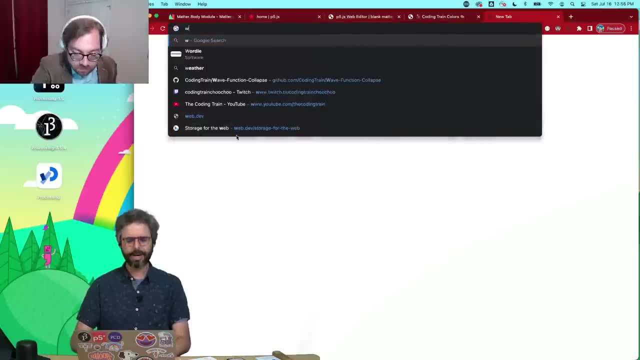 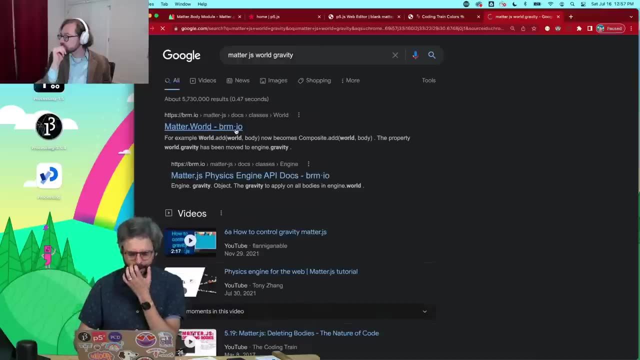 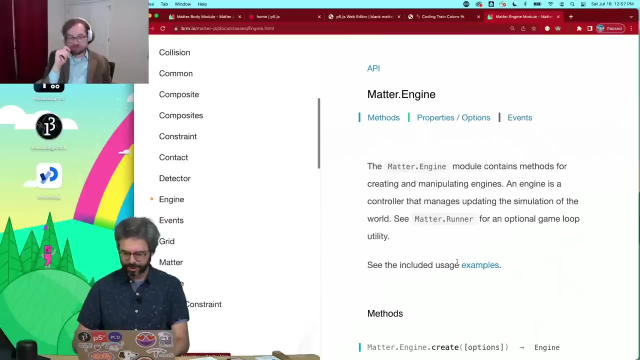 could increase the gravity like matter. Let's just look. I'm just curious if we want it just so, we have the matterjs world gravity, So I assume there is a world gravity has been moved to engine gravity. So engine gravity- is that something that I can just set directly, or do I need to call a function that's? 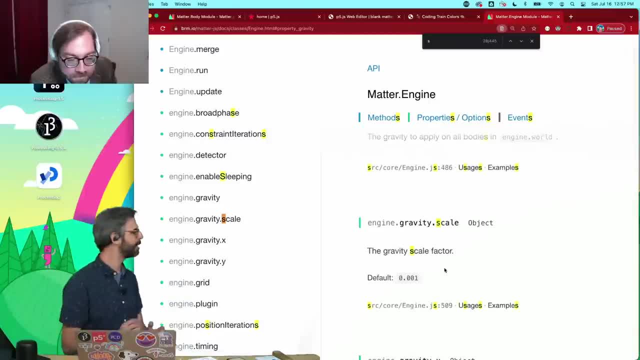 like: oh, there's a scale factor, So this probably it's probably internally got this sort of like scaling that it does between the two. So I'm just curious to see where we get with that. Now I think this is kind of not I'm not sure, I'm not sure if it's actually. I mean, 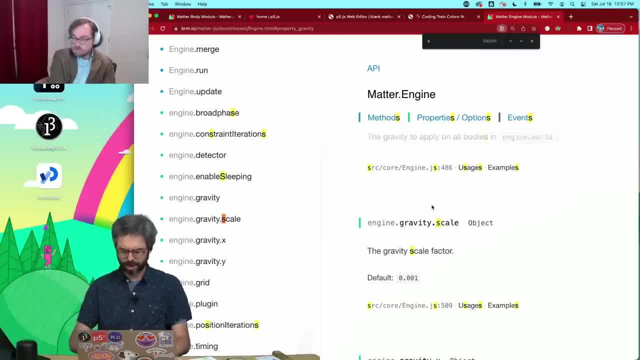 what would be real world measurements and pixels in some way, Okay, Although this is the scale for just the gravity, So I'm not sure I'd have to do a deeper dive into the ins and outs of this physics engine. Is there like a set set gravity? No, So let's just try hard. I'm just curious. Let's just 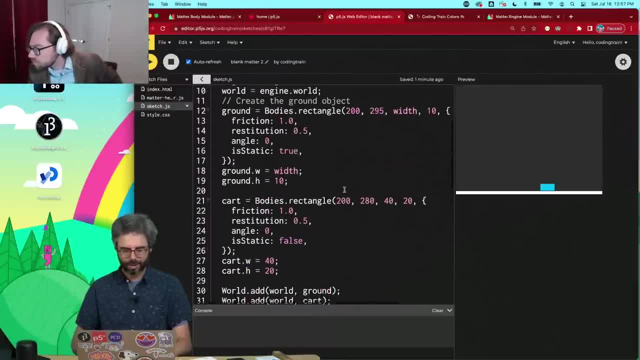 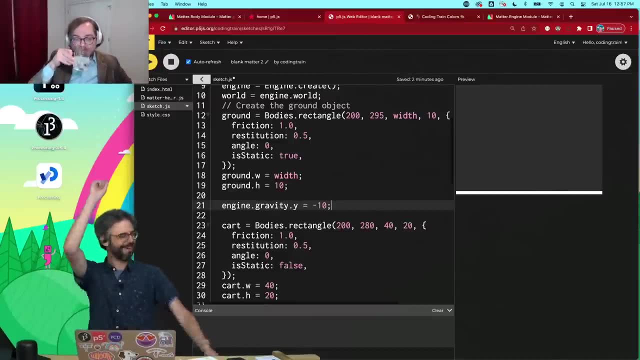 try hard coding it. Let's go to engine gravity. dot Y equals like negative 10.. Like what just happens? Yeah, See, okay, So I made a gravity in the inverse direction. I'm not sure, I'm not sure. Yeah, I guess. Okay, So, I'll just try this. So okay, So, let's just try this. So, let's just try this. 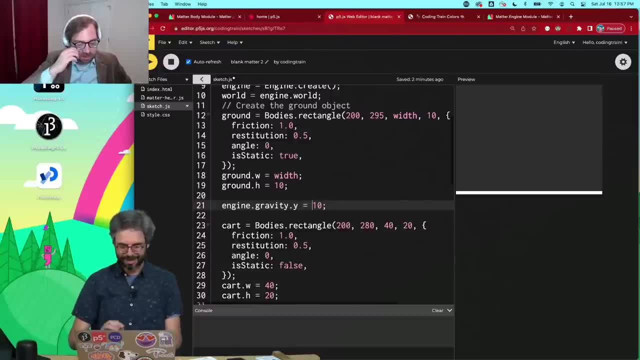 So I made a gravity in the inverse direction. Here's the gravity pointing down Right. So with like stronger gravity, whatever sort of weird anomaly that caused it to lift up into the air- is not really happening as much, But I'm going to let it stick with the default. 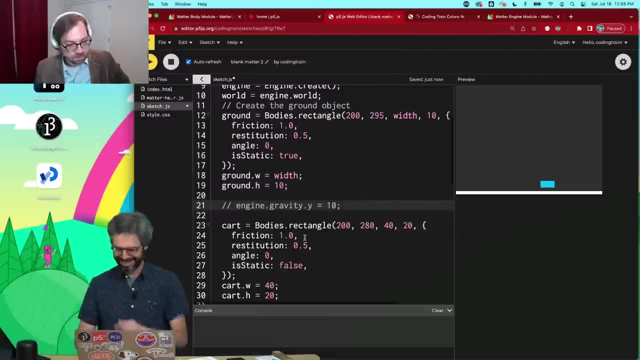 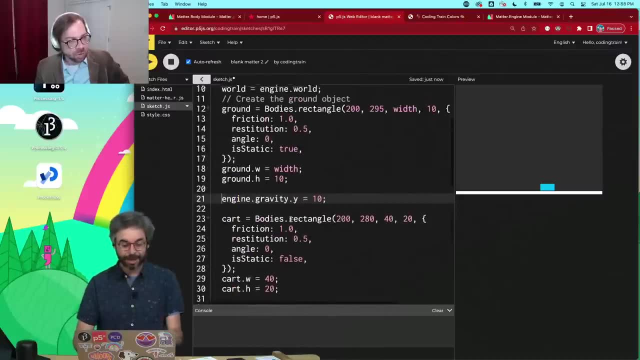 But if we need to play with that later, we can Okay Levitating. Actually, maybe let's keep the gravity a little bit stronger. Yeah, It looks a little bit more realistic And actually we'll really know when we look at the pendulum as well. 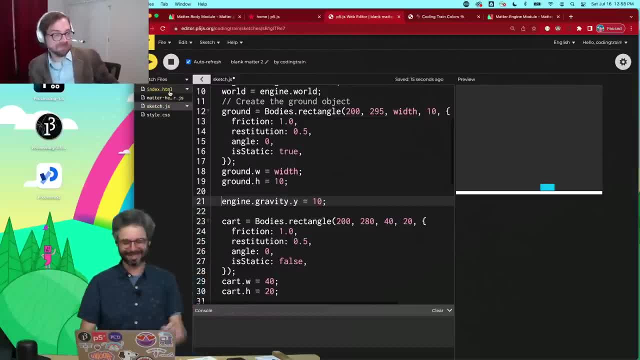 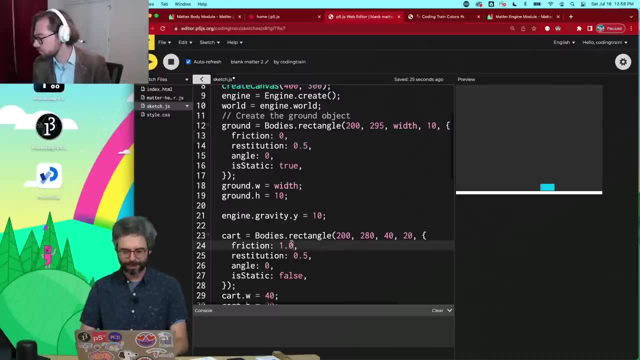 Right, If we get the pendulum, that'll be pretty clear. Right, The pendulum is going to have to deal with the gravity a lot more. The other thing is, I think I should turn the friction to zero, because right now the friction is probably playing a fairly large role in how it's able to slow down and stop at the proper location. 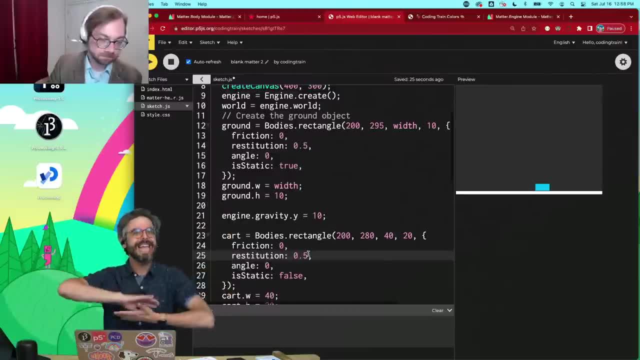 You can see now, And in fact the restitution that might be how it's levitating into the air, because I have each of these as slightly And I don't know if you know that there's a little bit of bounce between them. elasticity there. 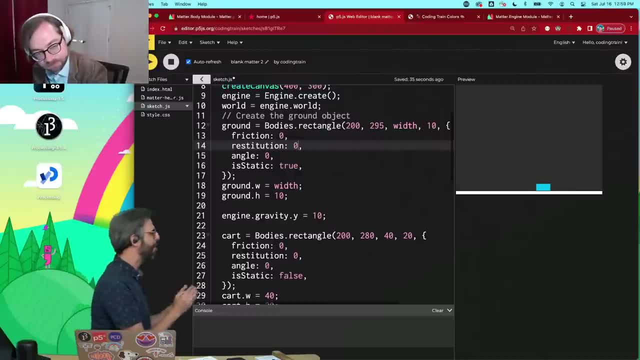 So I think, actually, by setting the friction to zero, the restitution to zero, we have a much more idealized scenario here. Oh, I'm liking this, Okay. So am I right in that if let's turn the gain up a tiny bit? 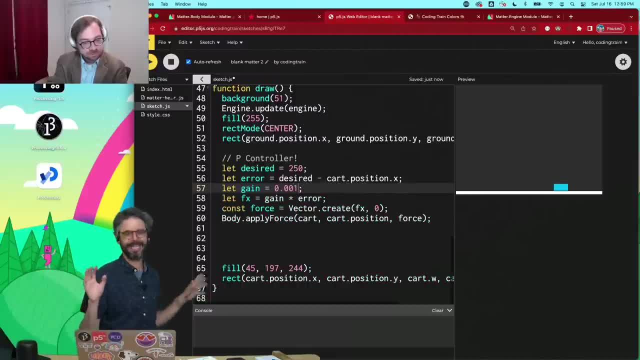 And actually, because we're in an interactive place, let's just go for it right now and immediately attach a slider to the air, So that we can demonstrate that we're already leaps and bounds ahead, not in terms of the math and, you know, accuracy of the simulation and the ability to code the simulation- than the Python version. 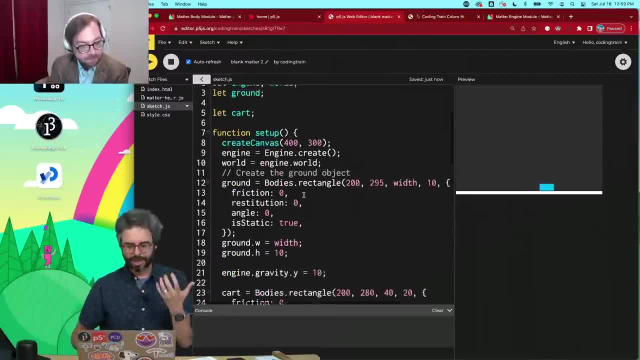 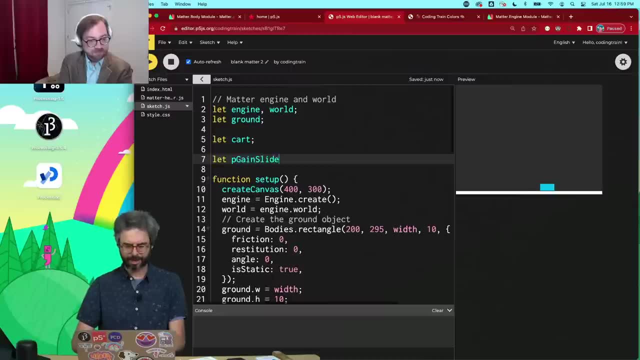 But we're leaps ahead in terms of being able to run it in real time. So let's, even just by changing a variable and having it run, But let's create a gain And I guess I'll call this P gain slider, in case we end up making a bunch of these. 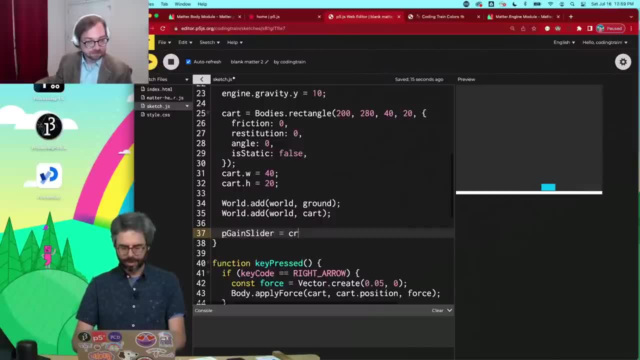 So I'm going to make a P gain slider And again, P5 has all these nice hooks to doing this very default interaction, GUI interactions. You know any of you who are CSS wizards and have done a lot of web development, you might have ideas about a much more thoughtfully designed interface and I would welcome those. 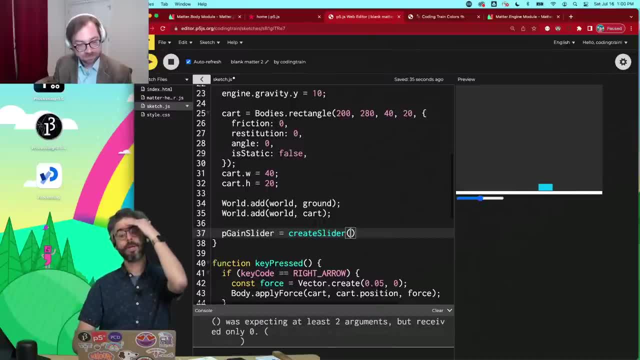 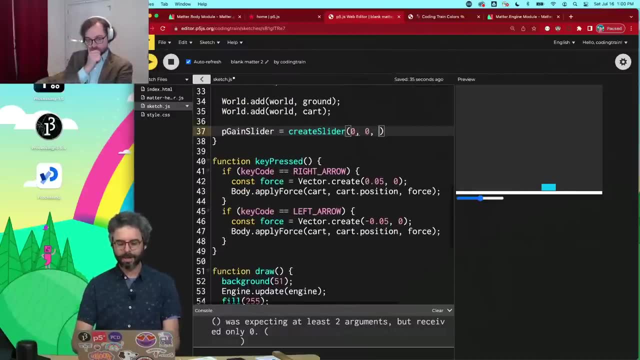 But for right now I can just make a slider. I need to give it three different values: The starting value, which let's make the gain zero, just to start, and the minimum and the maximum, And then actually I do also need a fourth value, because the default step is a unit of one. 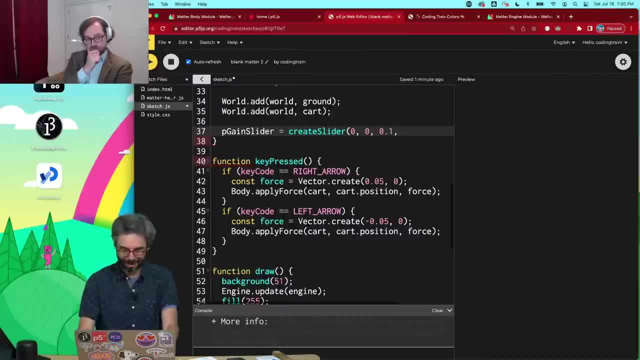 So if I want to be able to slide between zero and point one, I need a smaller unit of measurement. So let's do point oh one. And this should allow me to now Come on. If I could, if I could figure out how to use a mass mouse, what is good? 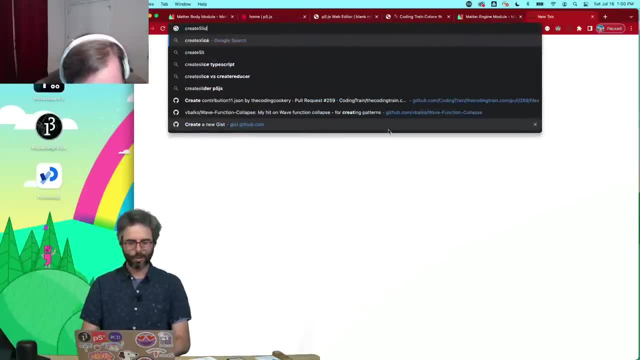 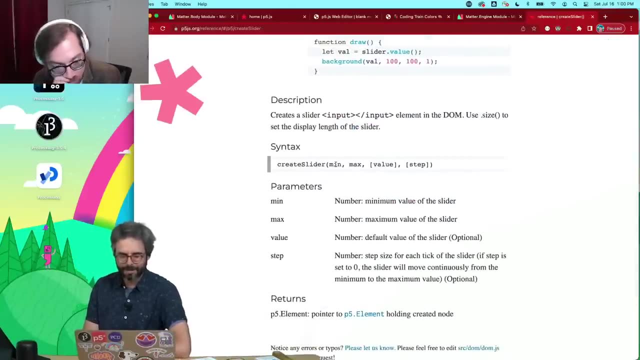 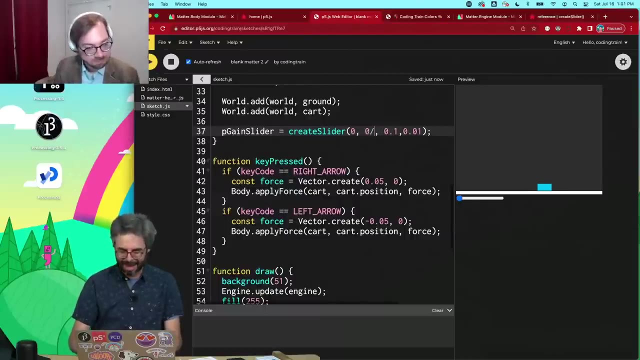 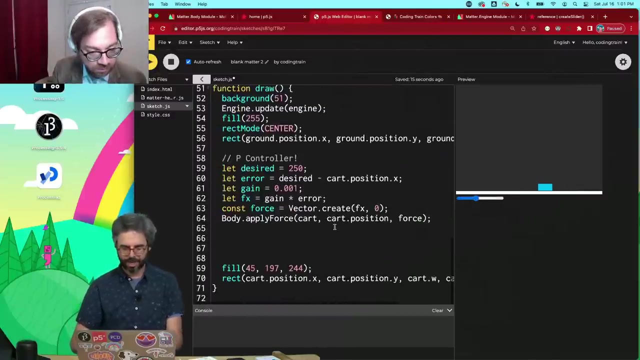 You know I must have made some weird mistake in the order of these parameters. Create slider P5.. Let's look: Minimum maximum, minimum maximum, then the value, then the step got it. so I did make a mistake. minimum maximum start at zero, then the step. there. now I can use the slider and all we need to do is have this be P gain slider dot value. 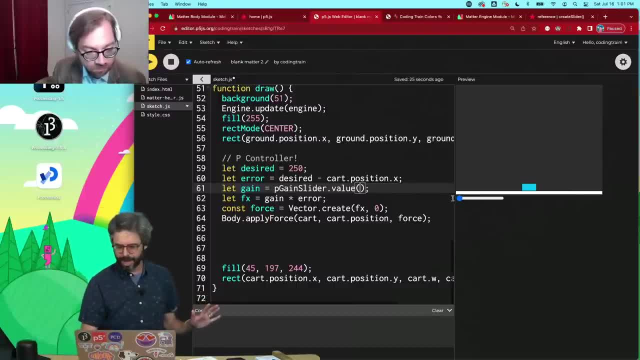 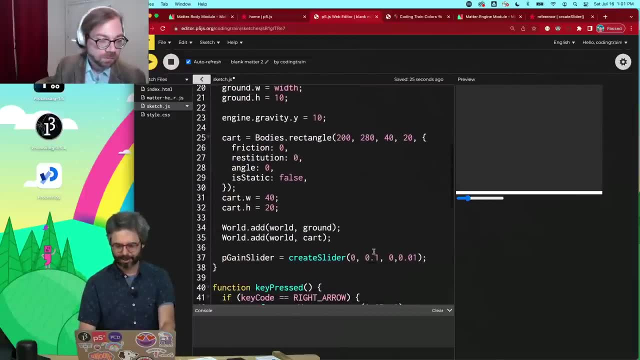 So when we start there's no gain, I can ramp up the gain. It's way too High. Um, let's, let's. let's give the let's. I think that's too high of a maximum value. Um, let's try this. 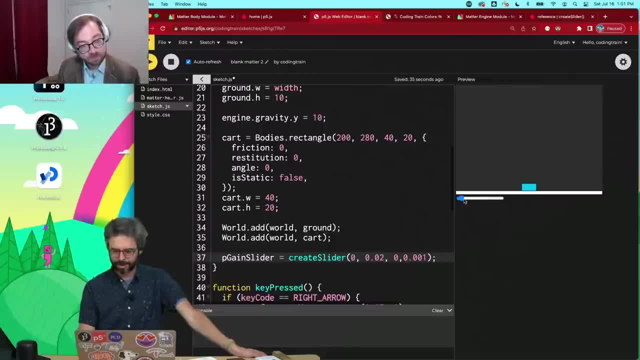 I've never- I don't usually- work with such small numbers and sliders. Uh, let's. yeah, there we go, So we can see it's way too big. I, uh, I need a like a reset button to put it back. 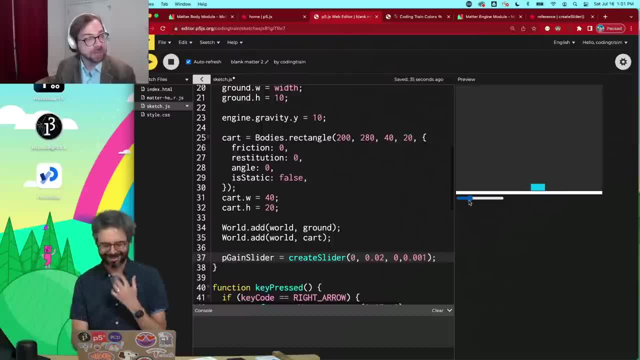 I was just going to say, I was just gonna say a reset button would would would really help you here, especially when we get to the cart pole. It's great, Let's. let's add that in, Let's add a um. 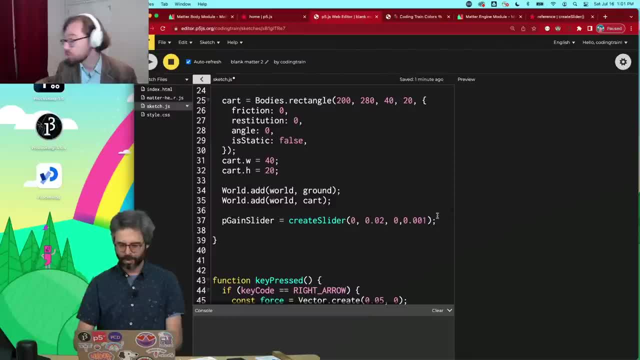 Actually, I don't need to have a global variable for it, because we'll just do it this way: Create button, reset uh, mouse pressed. So what I'm doing is: and it's going to add a button, Whoops. 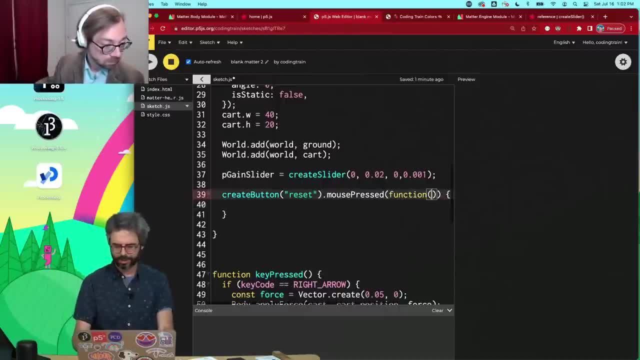 What did I? oh uh, mouse pressed function. I've forgotten how to use javascript. Okay, Uh, great, So you can see now, uh, quickly, um, and I'll zoom in here just to make a little bigger. 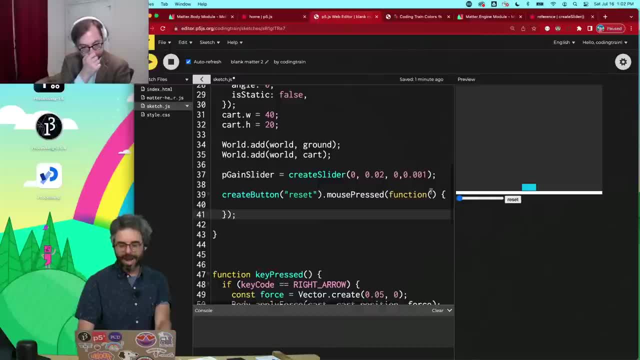 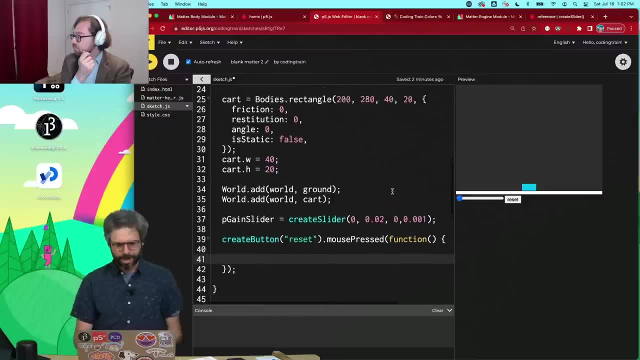 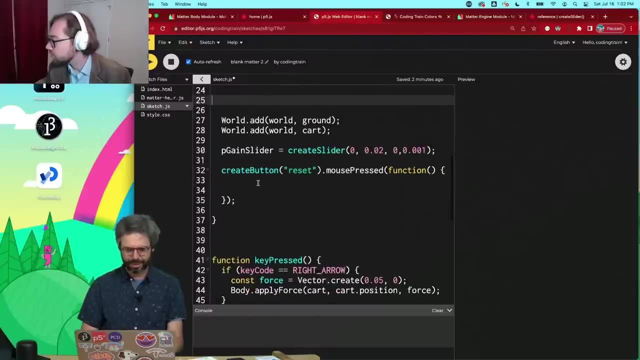 There's a reset button. Anytime I click this button, whatever code is inside this anonymous function, that's inside the mouse pressed event, will execute. So, uh, I suppose this is a little bit of a weird way of doing it, but let's actually just uh, let's write actually a function called re um reset cart. 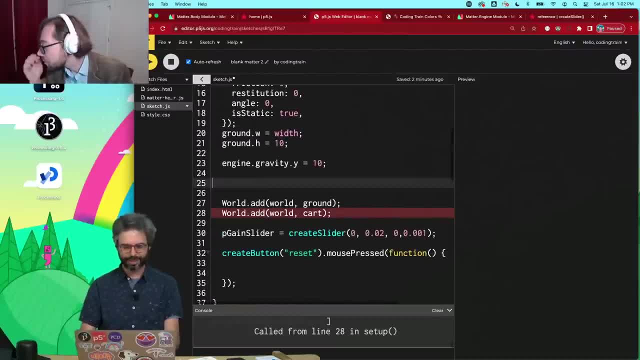 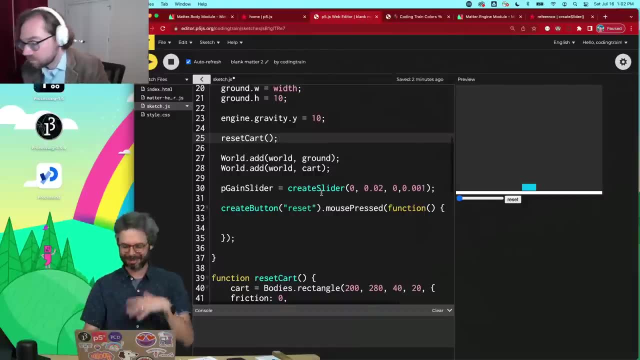 I'm actually just going to put it in a separate function and then I'll call reset cart. Just by making A new cart I could probably go in and set the velocity to zero and set its position back, but I think it'd be easier just to recreate the cart. 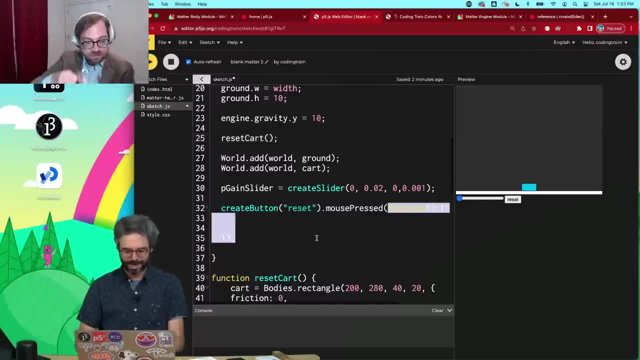 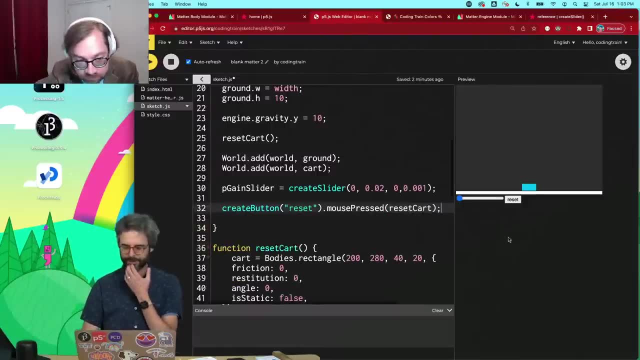 You know I can always just rerun the sketch, but it's nice to have a reset button And then I can just say right here, whoops um, reset cart whenever I also press that button. So if I make this big reset cart, 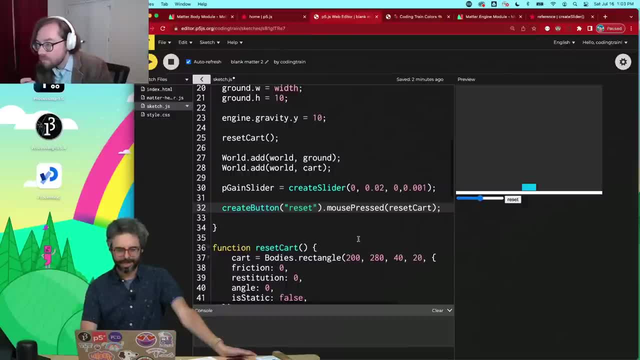 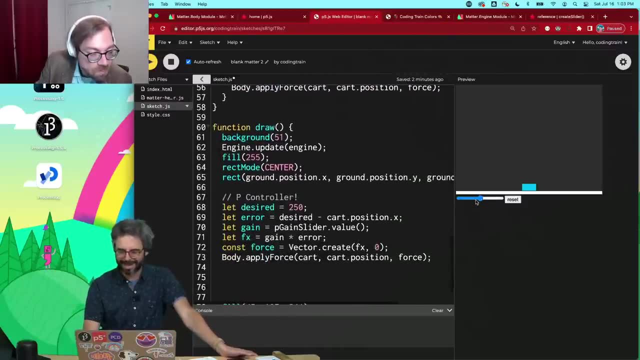 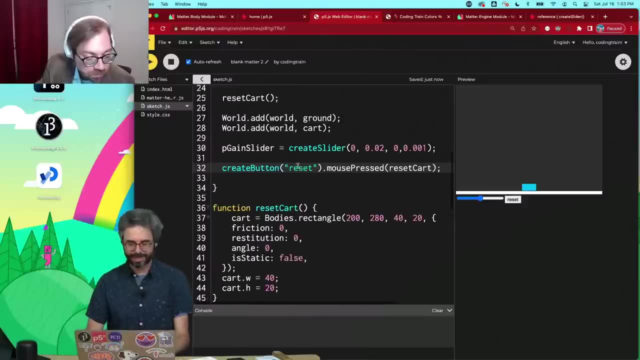 Oh, interesting. Now why? what did I do that caused it To no longer apply this? I'm- I'm- at the moment, I'm stumped here, Like I recreate the oh. you know what it is? adding the oh, adding the oh. so this is actually a I've done a terrible thing. 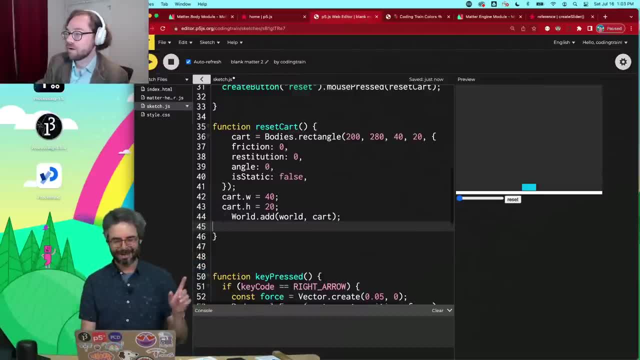 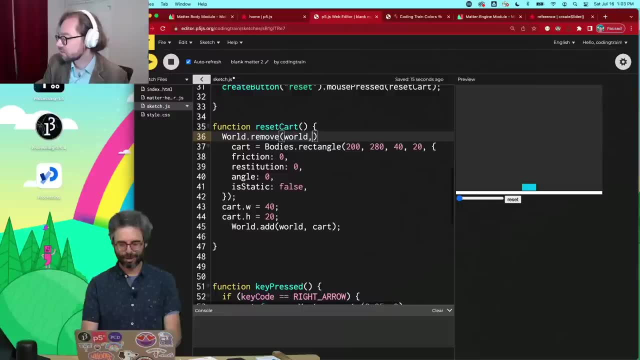 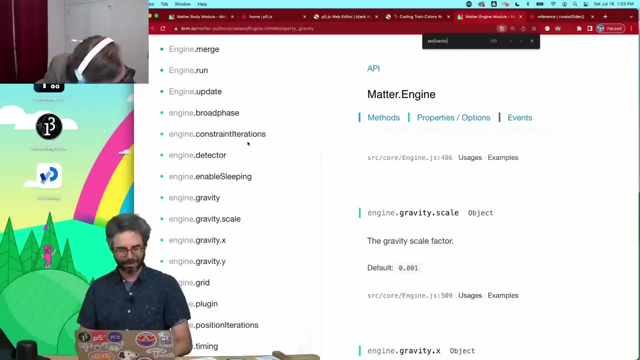 I can't do this. This is how I usually do things, but I would have to remove the cart. Let's see, Maybe it's as easy as doing this: Remove the old cart, Make a new cart. Uh, let's see, we'll have to look into um, uh, we'll have to look into the world. object. 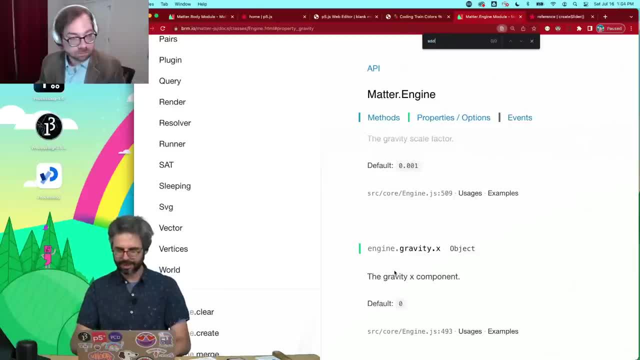 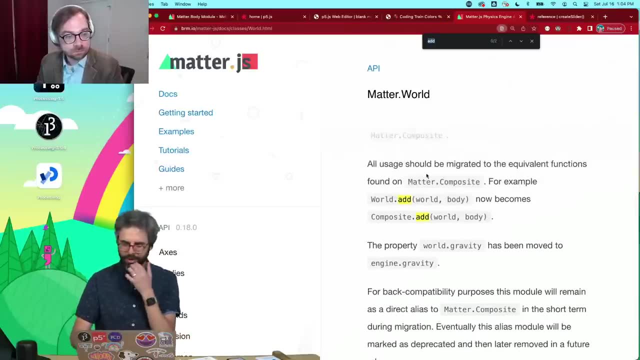 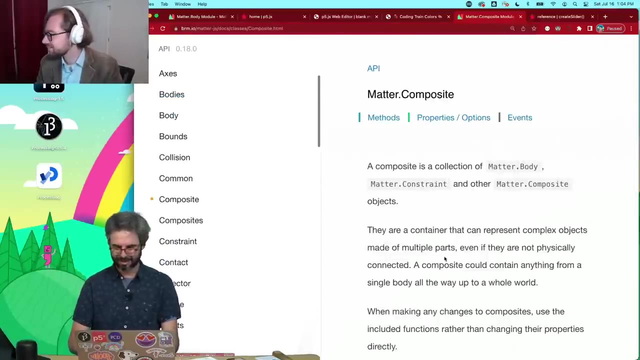 I don't want to get too off here on a tangent, but here add um. world has an ad. Oh, uh, usage should be migrated to the matter. dot composite: That's fine, Uh so uh, is there a remove composite, dot remove. 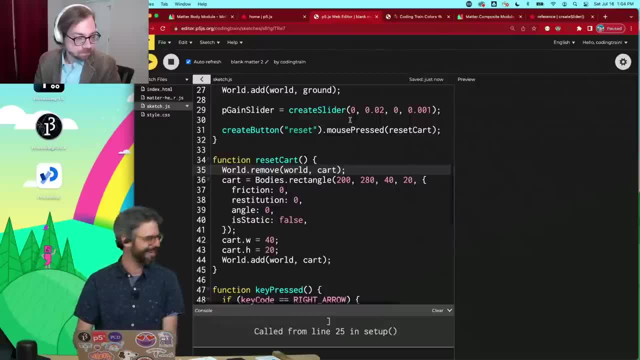 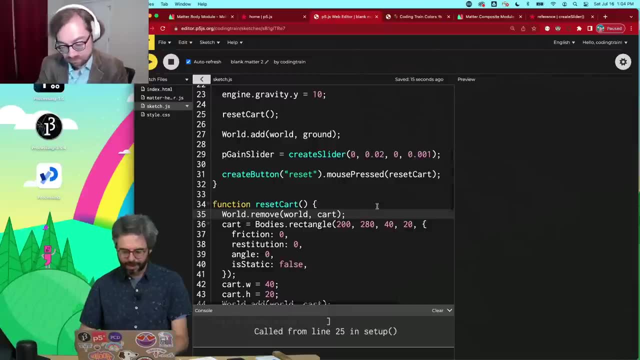 Interesting. Um, let's do it a different way. I'm going to invest. I'm looking at the chat. uh uh uh. reset, Let's just see reset cart. mouse press reset cart. Um, let's just see matter dot composite. 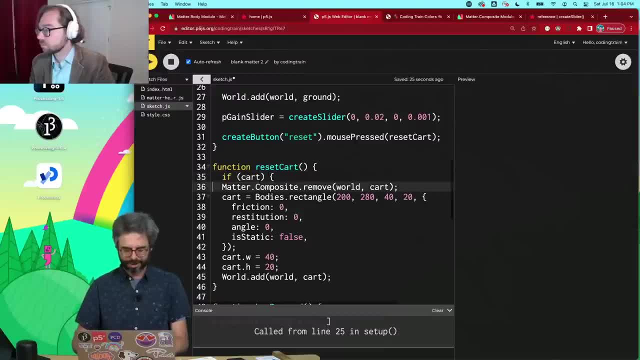 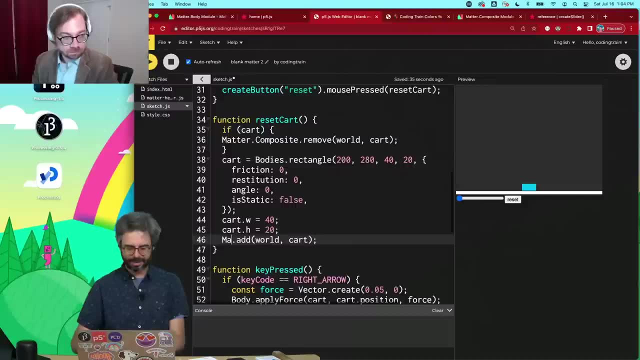 Oh, if, if the card exists, you'll have to bear with me for a second as I try to sort this out. Um, and then let's see. uh, let's, let's go. I guess it's changed. It's changed to matter. dot- composite dot add. 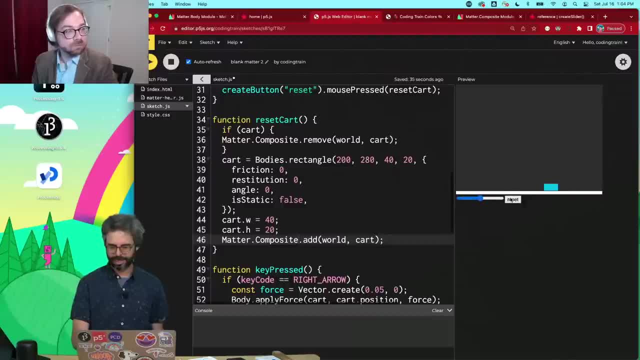 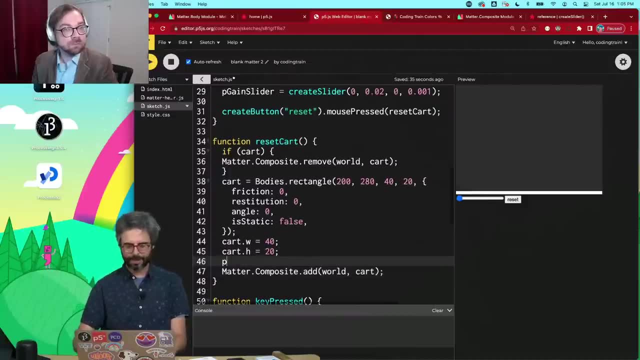 Okay So, let's see And then reset. Yeah, Okay So, and I might as well also reset the slider. uh, P gain slider dot value. I'll reset the slider to zero. So anyway, that was a lot of oh, uh, and I need to make sure this happens after I've. 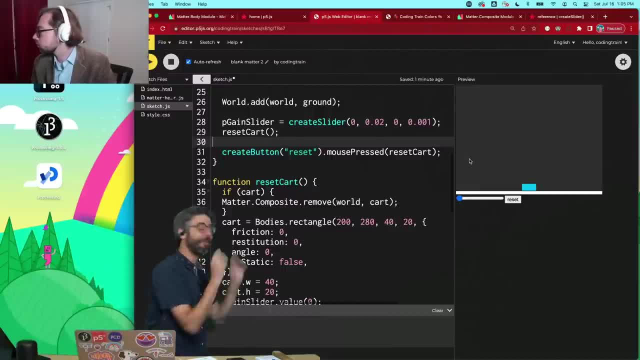 made the slider: Okay, So that was a lot of extra. Well, one thing about adding interactivity: Okay, So interactivity. is we easily so easy to lose our way from the actual simulation that we're trying to focus on because there's so many little extra edge cases and things that 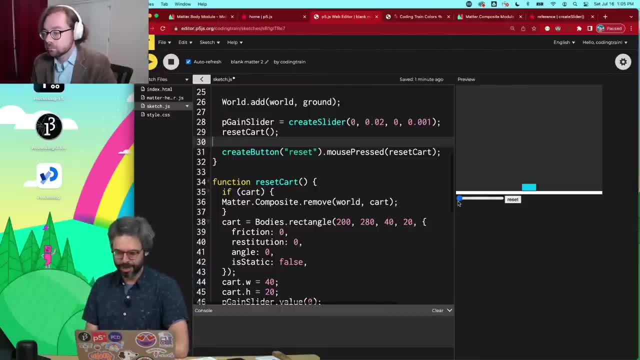 come up with the interactivity, but that's what we're here for, So we'll go with it. So I'm going to um add a little bit of gain. If I hit reset, it sets everything back to zero, And I think this. I think maybe, um, we'll leave the maximum gain a little bit lower. 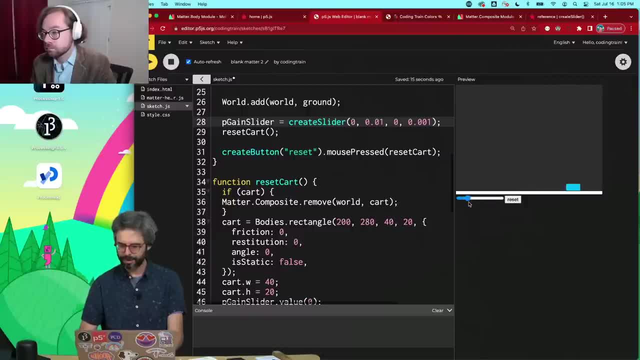 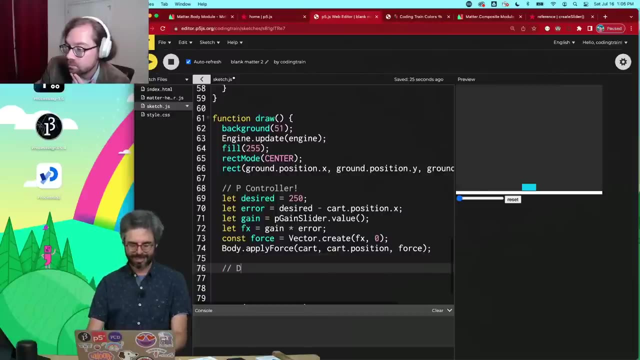 so we can see: uh, all right, great, All right. So we now have a P controller moving the cart to a desired location. Now I want to add the D, or so here's the question. Here's one question: the force. 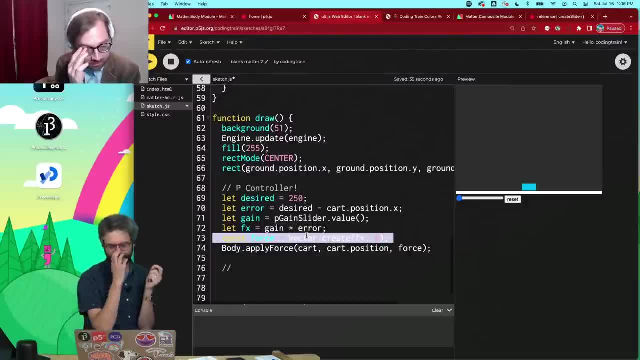 So this is where I guess I'm still going to. uh, if I'm following um the earlier Python code, what I'm doing is I'm adding the you know. Okay, Let's just hit stop here, so we don't get errors. 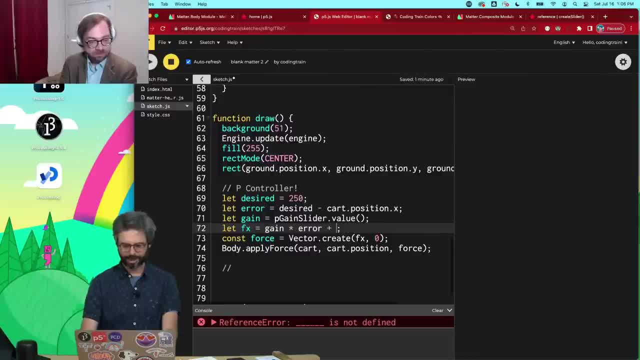 This is the D. you know, this is like a comment here, like a, not a real thing: D control. I'm going to add that here so I can leave it as one force, uh, and then apply that same force, the same way. 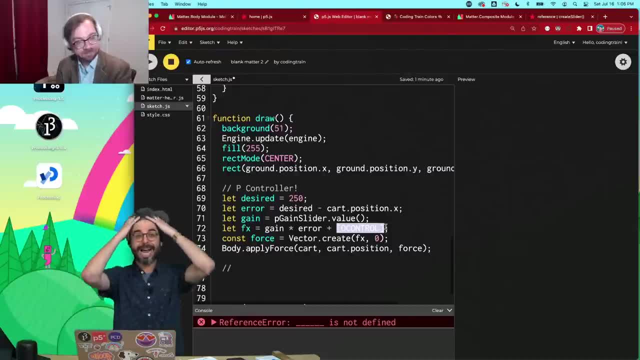 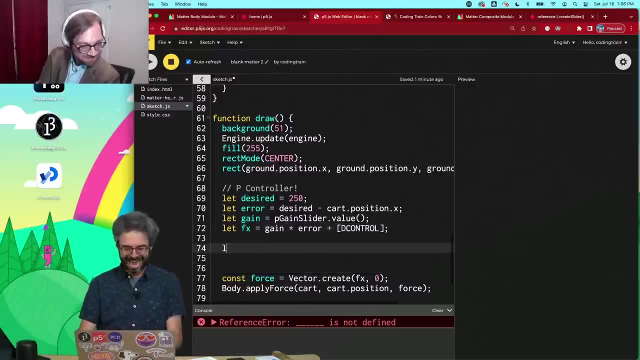 It's just a matter of adding that, And so in order to do that, I need to look at the carts velocity. Is that correct? That's right, Okay. So let's look at um. So first thing first. I uh an. you know I haven't used matterjs other than a few. 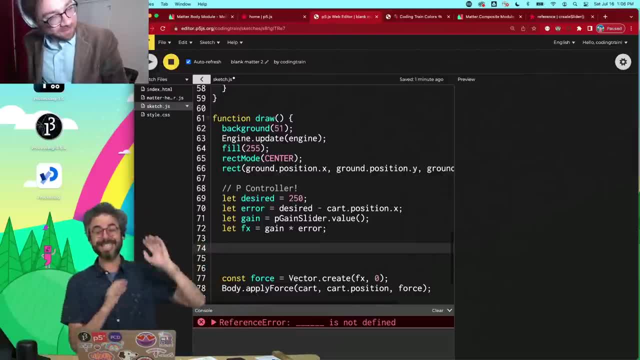 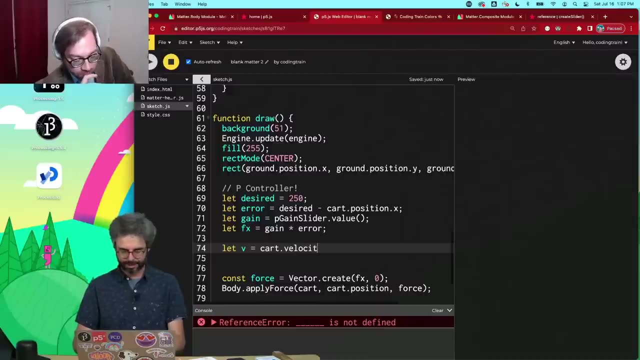 tests yesterday in probably a couple of years. So I didn't go. this is as far as I got basically in the tests, so we'll see how how this goes now, uh, and how far we get. Okay, So I need to get- I'm just going to call it V the carts, uh, velocity. 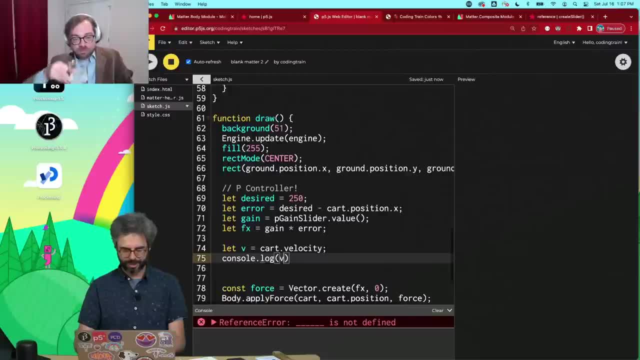 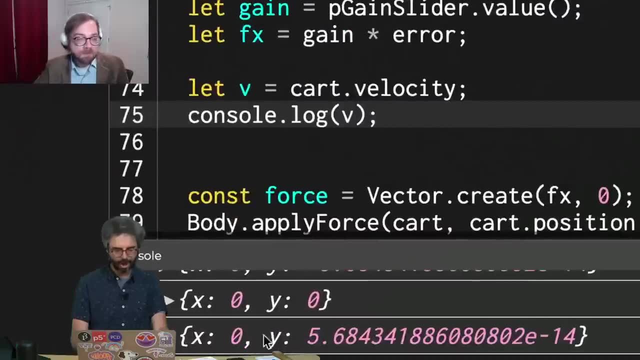 Uh, let's console log that and see if that shows up. Great, So we can see here that I'm getting the carts velocity. Now there is this, like you know, a tiny, infinitesimal Y velocity, which I will choose to ignore. 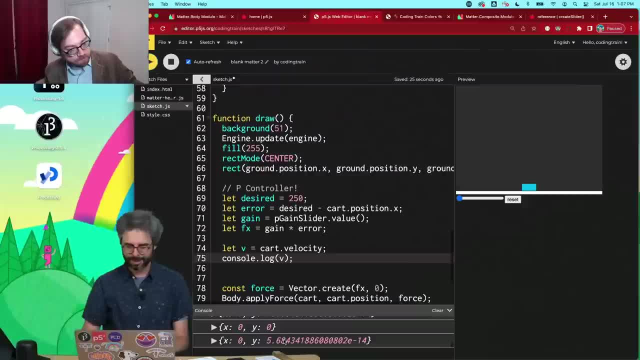 I just want the X component of that carts velocity. Um, okay, And this actually often occurs in JavaScript. One of the pitfalls of JavaScript is the way that it rounds floating point numbers is a really odd behavior. So you know, you can add three points. 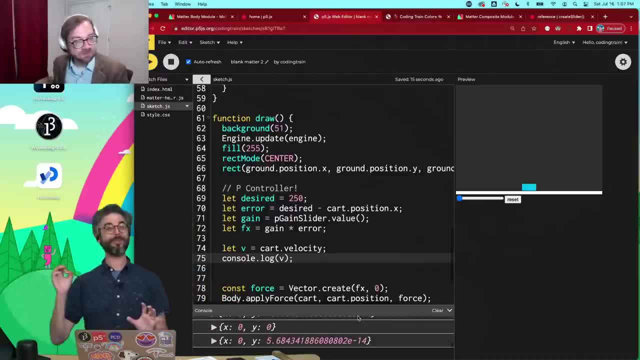 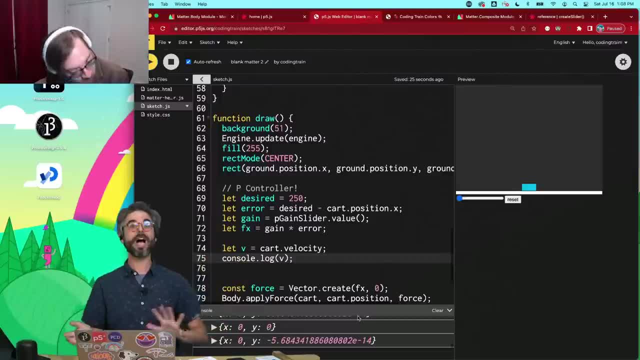 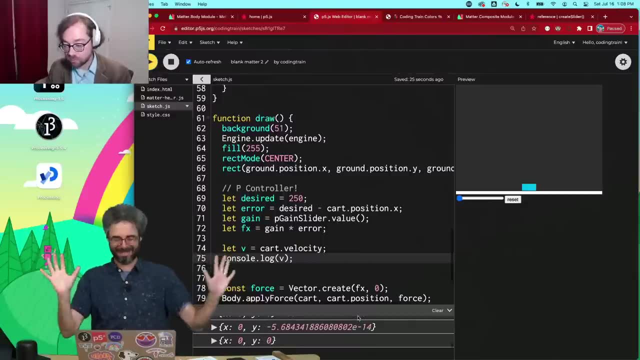 2,, 1,, 4, like all sorts of weird stuff can have in a JavaScript, because you know we're not, we don't. this code is not going to help us land the space X rocket. It's just for us to simulate the browser to get the idea of it going. so we can live with. 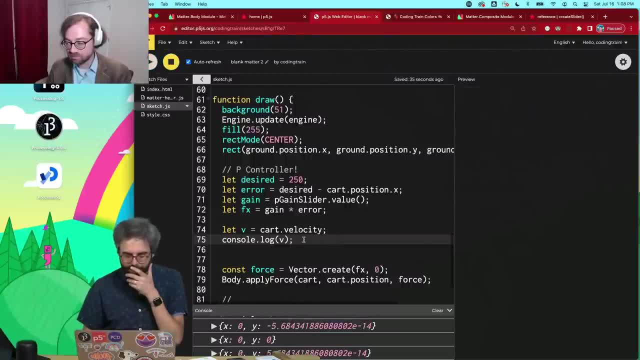 those kinds of errors. Okay, Um, so now I need a um. you're going to have to Talk me through this a little bit here, Christian. I know that I need a um. we'll call this the P gain. 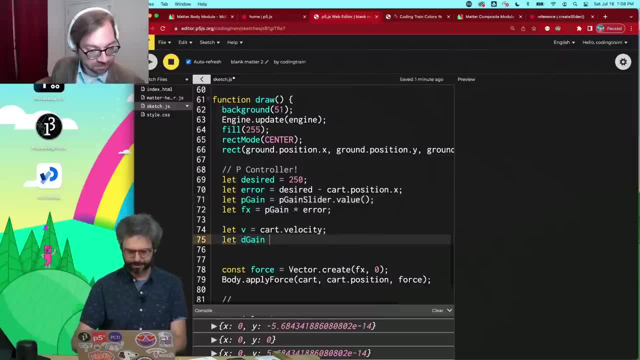 Now I need a D gain, That's right, Uh, which you had said something like 10% of what your gain usually is. Is that right? Yeah, I go, I go for 20 for 20% generally, So I'll go 50 for you. 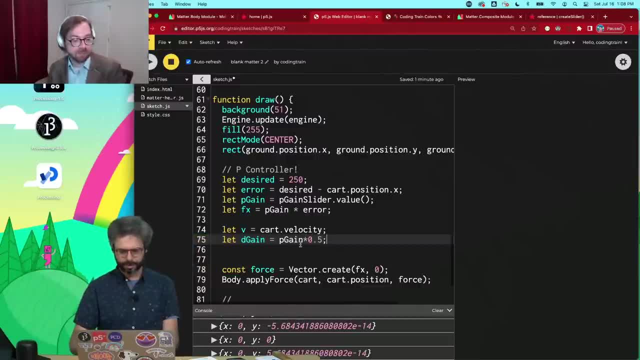 So, yeah, Oh, sorry, Sorry, That's not a game yet- 50.. Yeah, So I will make this its own value, but just to have something in there, Let's start with it as half, whatever the P gain is. 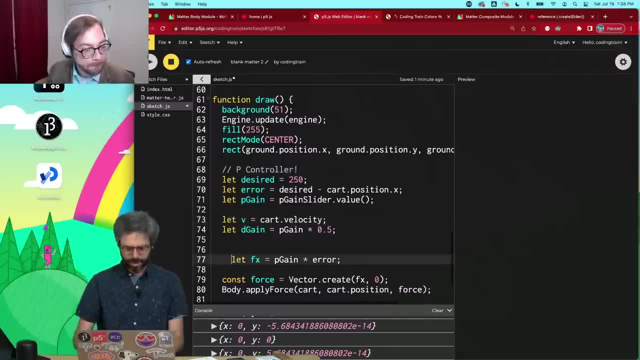 And then the, the L and I've- now I'm blanking here because the elements that I want to multiply together in the equation help me with this part here. So you- so it was going to be- first is your D gain that you just defined. 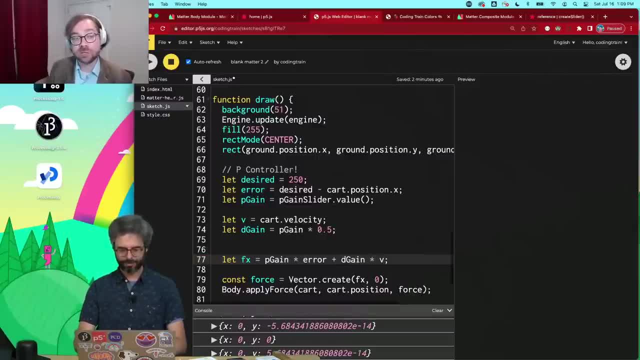 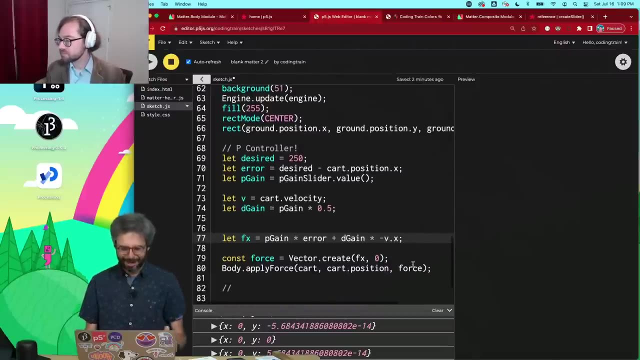 They going to want to multiply it by the derivative of your error, which is going to be negative velocity. Okay, And, and just in the X direction in this case, Yes, Yeah, Okay, Great, Perfect, Um, okay. So let's see, I'm like no, it can't be that easy right. 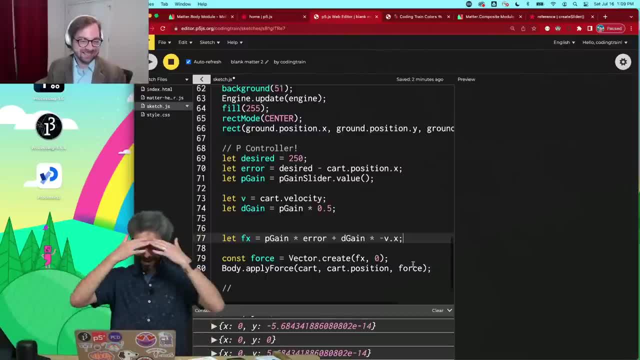 The derivative of the error is the velocity. is the is the negative of the velocity right? Because velocity we're talking about derivative as a way of describing the change. the change in a position is the velocity. incidentally, the change in a velocity is the acceleration. 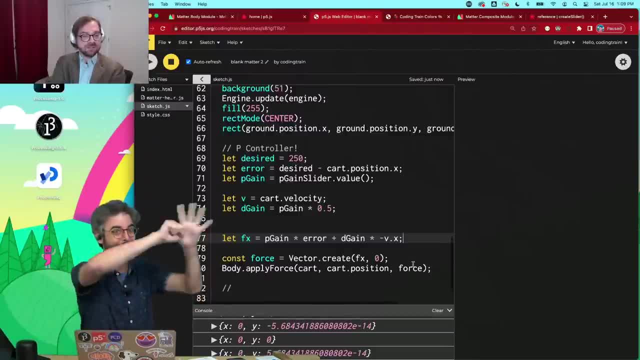 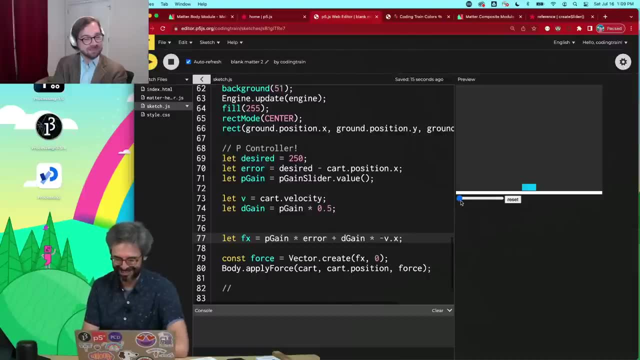 and force. Yes, It's the acceleration. This is where all that oiler integration stuff comes together Beautifully. Okay, Here we go. Oh wait, I got to turn off the game, I'm afraid. Look at that, That is fantastic. 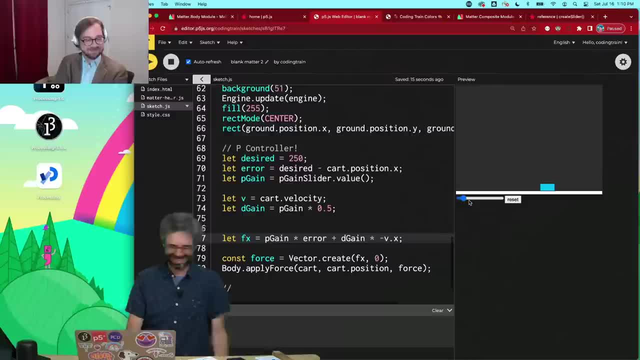 That's a PD controller. We did it. See you all tomorrow. Okay, No, no, we're going to get going, Uh, but that's great. So let's, um, let's give the controller, just so as it continues to rerun itself. let's. 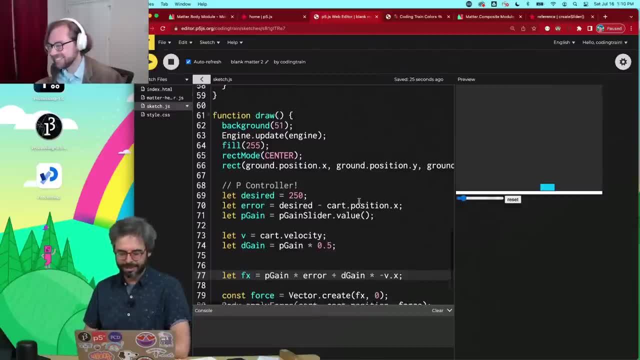 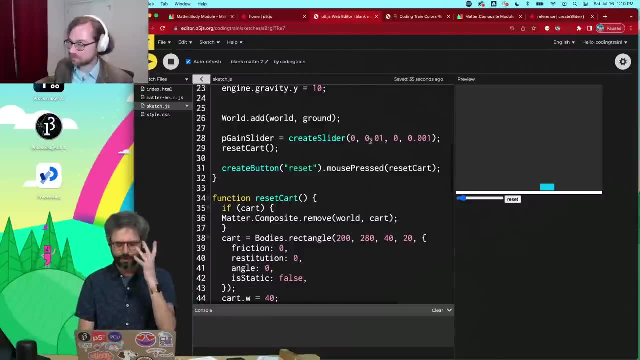 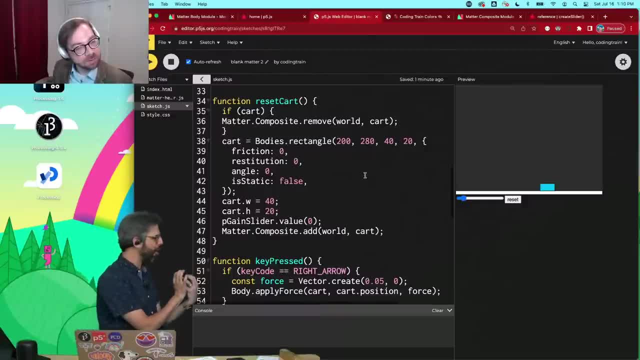 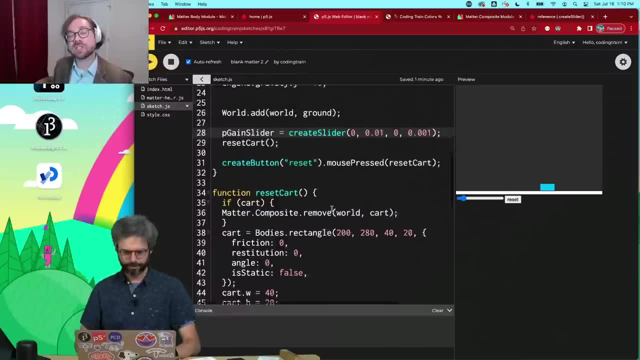 Should we leave the um D gain as a ratio, uh, as calculated from the P gain, Or should we give it our own control over that? I I'd say it'd be very informative to put a slider on there cause, then you can see you. 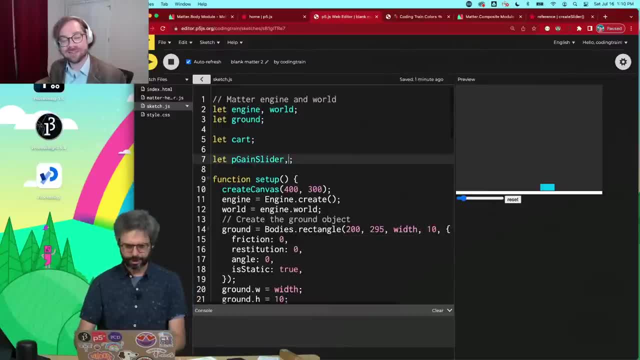 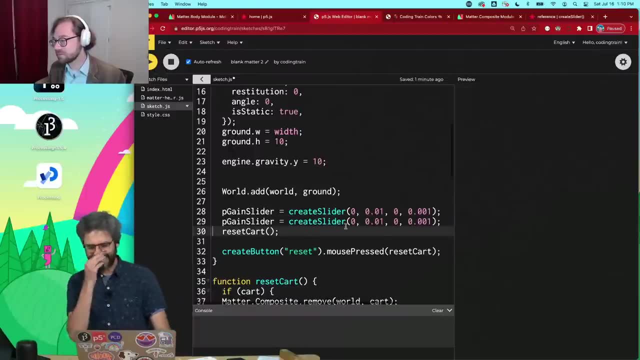 can see the reset. Yeah Yeah, It'll be interesting to see how that behaves. Okay, So let's do a D gain slider. add that Now. I'm not going to add any labels to the slider, so we're just going to have to. 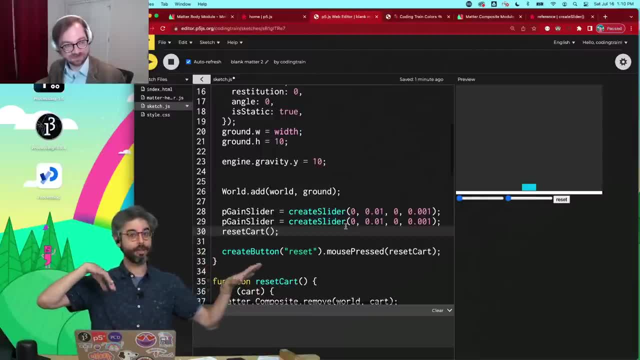 remember which one's which- One of the things that maybe I'll do after we're done today, which is I'll put this in a GitHub repository and accept pull requests for people to help improve the interface and add things to it. I don't know if you saw this. I'm going off on a. 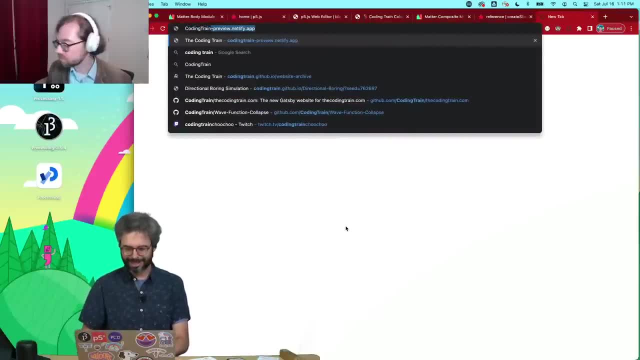 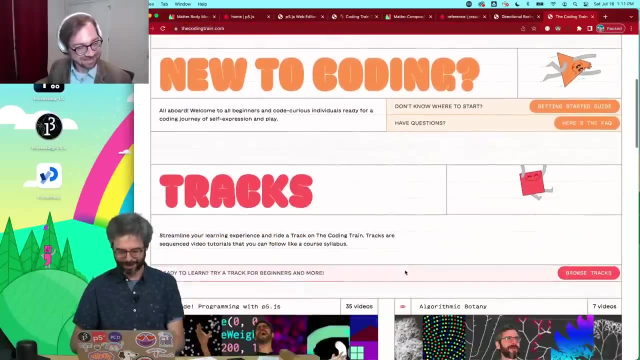 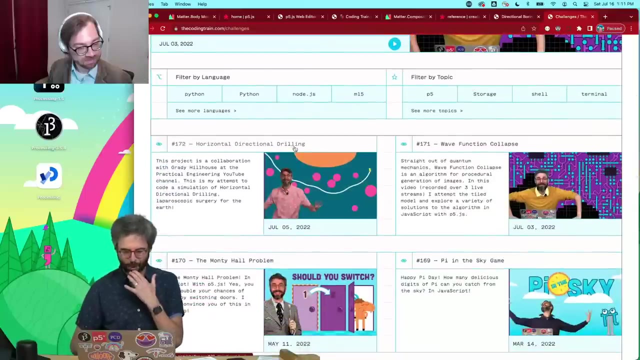 little bit of a tangent here, but I just want to show you an amazing example of this is. let me just go sorry for the slight digression, but I want to show everybody what's possible. So I'm going to go to one of my recent videos about horizontal directional drilling And this: 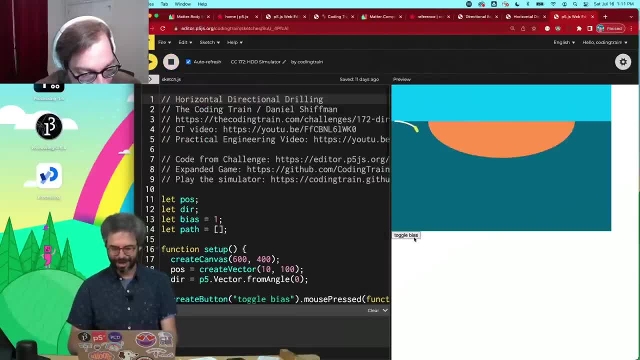 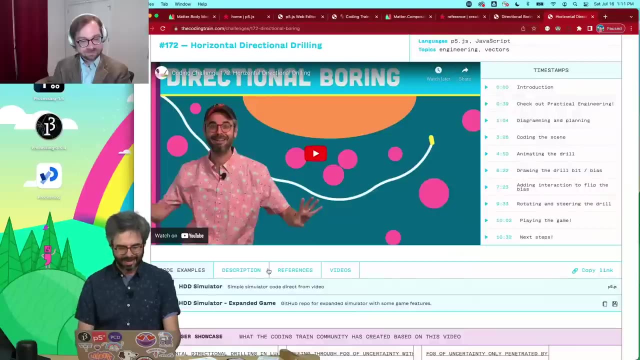 was a really basic simulation of how horizontal directional drilling works, with changing the bias of this particular kind of drill and turning it, And this was the basic simple code example from the video. And then, if I go here to the expanded game which the viewers contributed to, 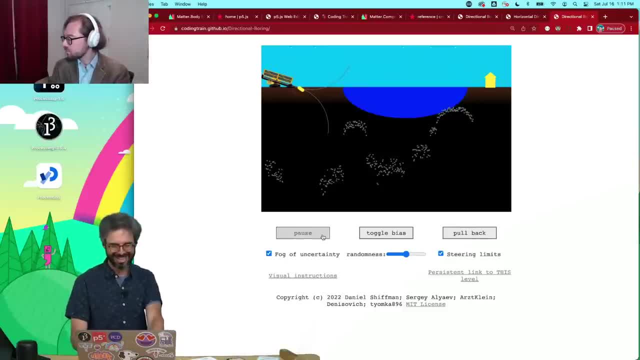 and I try it here. you'll see like this is what it looks like now. It has like this animated drill. It has like these: it has this: you know these obstacles that are hidden, but you sort of get these clues. It has a goal, you get a score, So we don't need to go down the 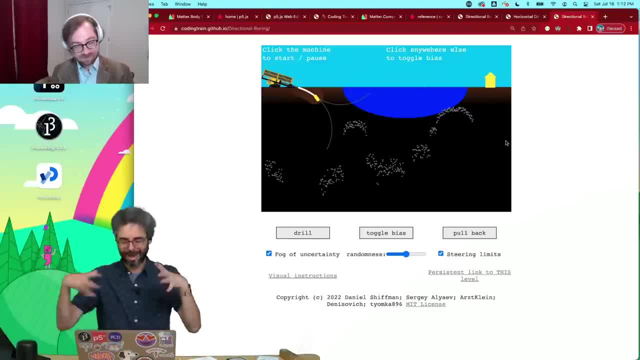 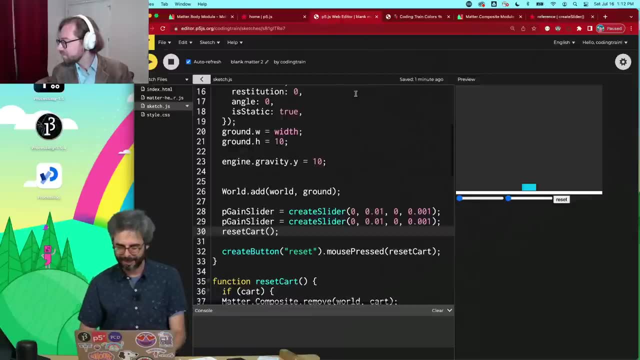 road, but I just want to encourage people who are interested. anybody who helped with this. if you want to help augment whatever simulation we do here, I would welcome. I'll put this all up afterwards, Okay, So now I need to get back to where I was, So let's think. 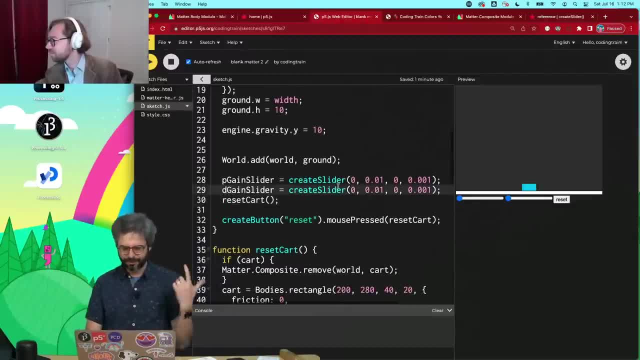 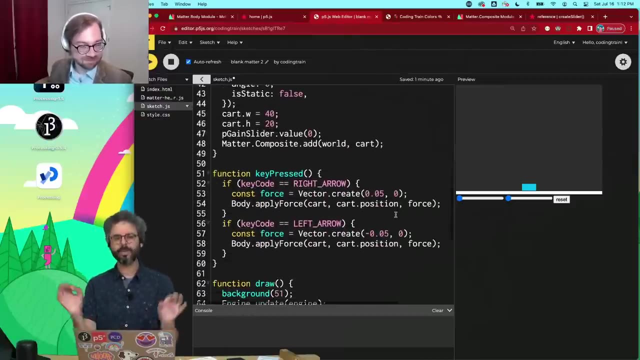 about this. The D gain slider will have a default starting value of zero Its range. let's have its range go to half. We can actually just make it the same because we can. let's just make them the same for right now, So we don't. we'll see what the gains are by their literal position along the. 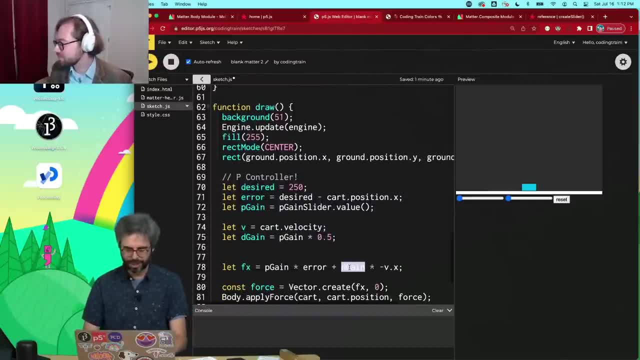 slider, And then we will do this: D gain. Oh yeah, sorry, Yes, sorry, P, this is D gain slider. I have a lot of redundant variables here, but I think it helps us follow what's going on: The value of that slider, And then right. 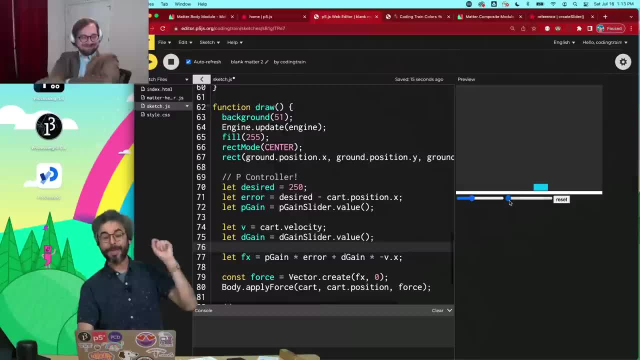 This. ah, so now what we can see here is this is with the P gain on, And as I turn up the D gain, it's like this: dampening or damping. I can never get that right. Do you have a nice way of remembering the correct terminology of damping versus dampening? One of 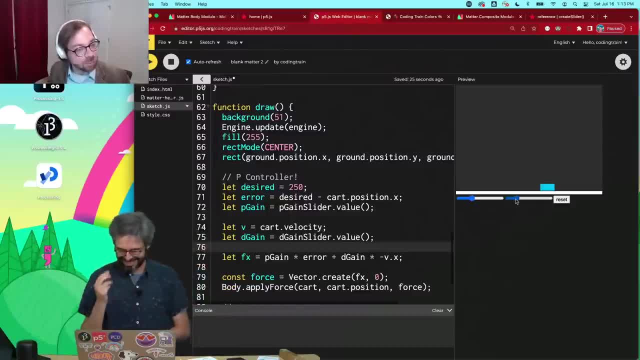 those is making something wet. Yeah Yeah, Dampening is the wet thing. Ah, you know you dampen a cloth, you know dampen. but the problem is because something's damp in the rain, So people think damping. So it's yeah, Dampening is the is the. I got to come with a great mnemonic. 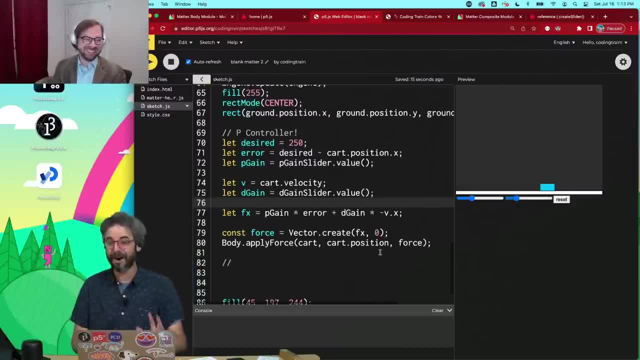 device for you Until next time. Until next time. Yeah, I'm always getting that wrong. It's like the other thing that I always get wrong Is modulo versus modulus: Modulo is the operator, The modulus is the result of the. 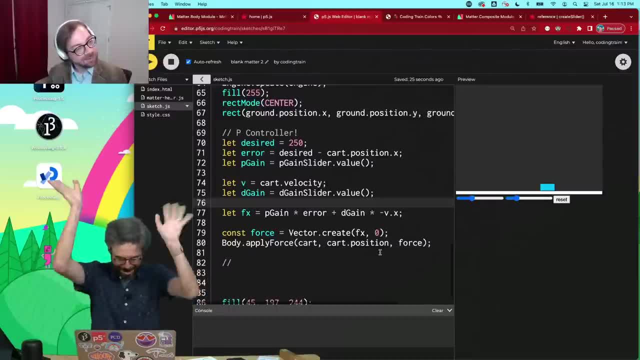 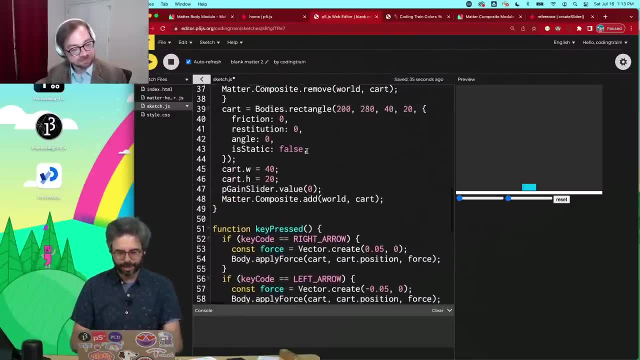 you know of the, you know this value, modulo, this other value. Anyway, I'm off topic, Okay. So I think we're in good shape here. Um, let's add, just um, let's give these some default values. 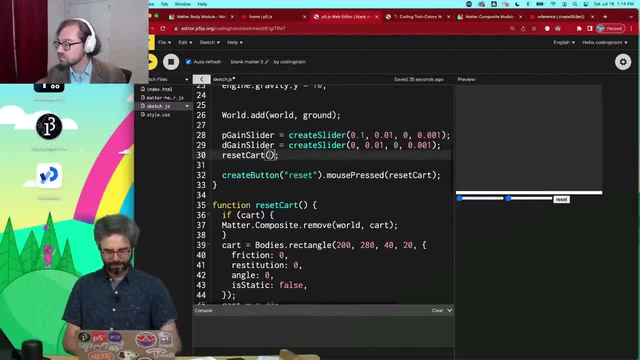 that we can sort of see stuff happening as I'm um, whoops, no, not, not point. um, let's do 0.05, 0.025.. So every time the sketch re: Oh, no, wait, Oh, again, this is I. I have the order of this wrong. I can't seem to remember. 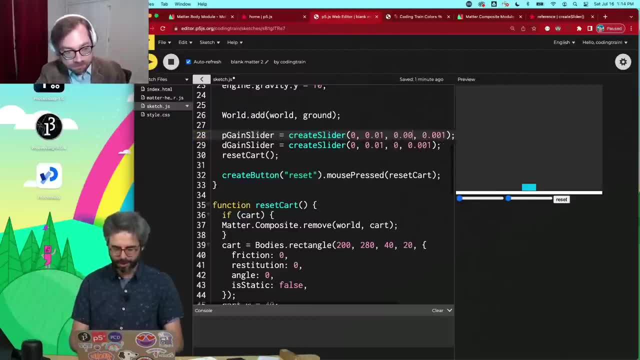 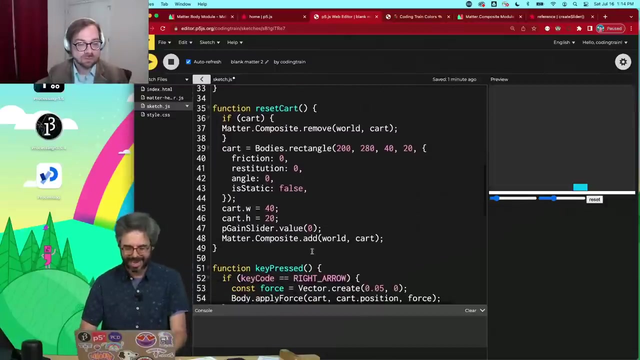 that this is 0.0, 0.05 and then 0.0025.. Did that work? Uh, oh, wait, D gain slider. What have I got wrong here? Uh, P gain. So why is the P gain slider? Oh, because of the reset. 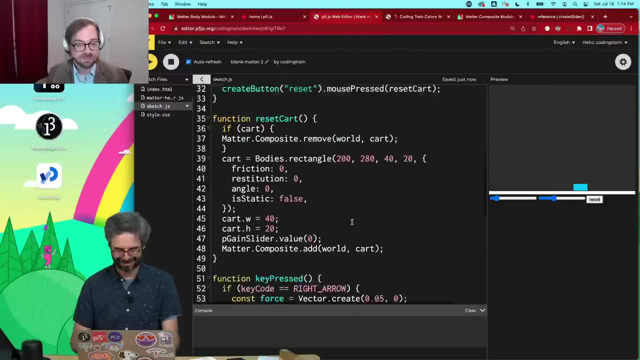 Ah, this is. this is a very awkward thing that I've done that I'm just going to uh, uh live with. So this actually okay, great, Okay. So I just want it to every time I change anything in. 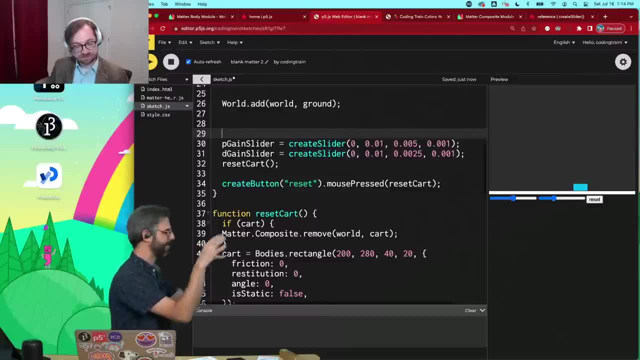 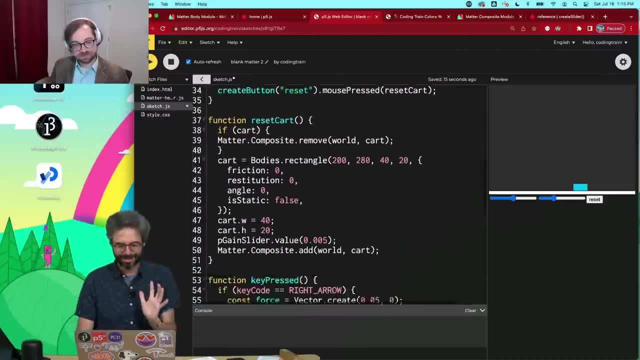 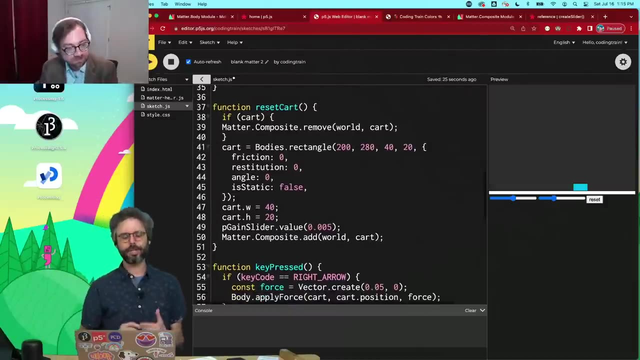 the code, it's going to automatically start and resettle it. Uh okay, Min max. Oh right, You think maybe I should have a variable for the default value. That would make sense, but this is fine. I want to add the pendulum, the, the pole, if you will. So the way that I'm going, 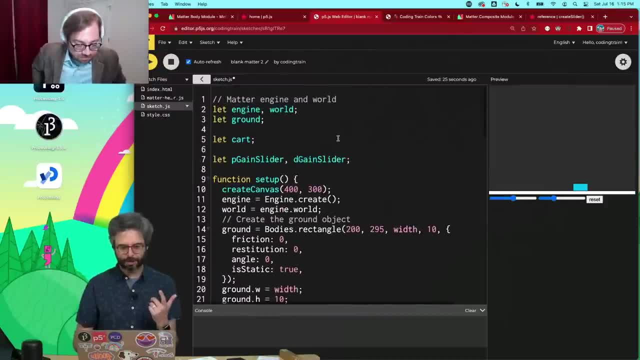 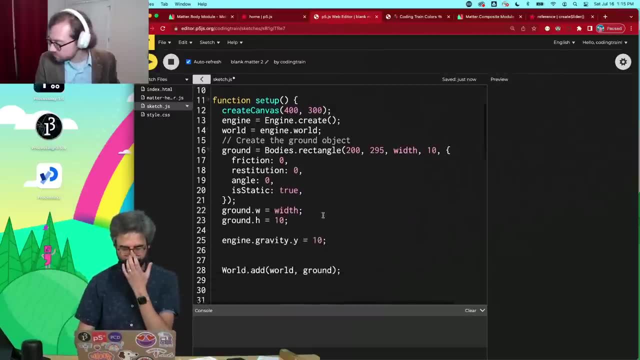 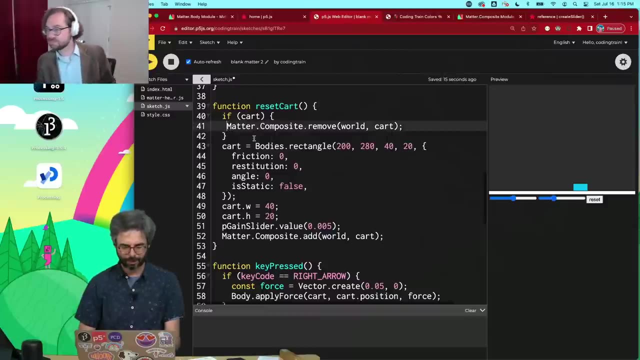 to do this is by first creating a circular body, So I'm going to call this the Bob, as in the thing that's hanging on the end of the pendulum. So let's have a variable for Bob We're going to create, and I suppose this should go in the reset. I've really locked myself into a corner here with 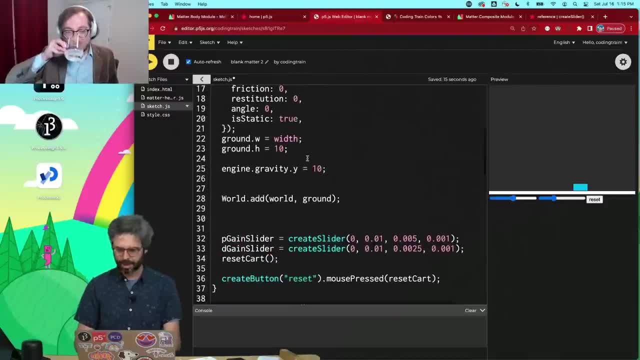 this, but let's not worry about it right now. Uh, you know, maybe I won't use the reset button. uh, much of that thing I can sort of refactor later, Cause there's so many things now that need might are going to start to need to be resettled. So I'm going to call this the Bob, as in the thing. 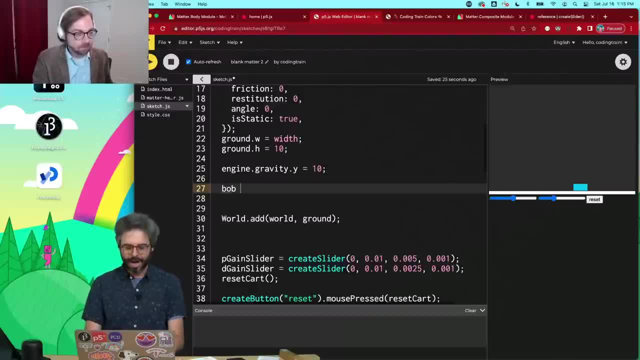 that's hanging on the end of the pendulum. So let's have a variable for Bob. We're going to create- and I want to reset- Um. so the Bob is a body, creates um body circle. I think it's um. 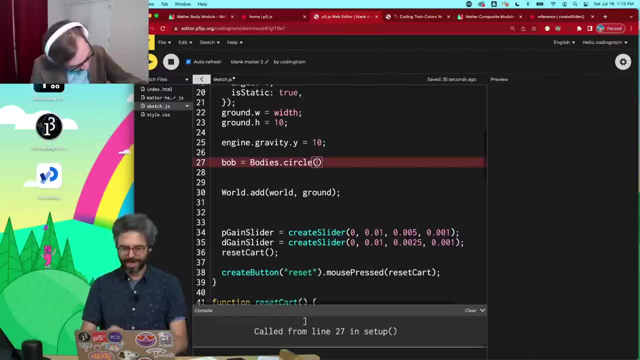 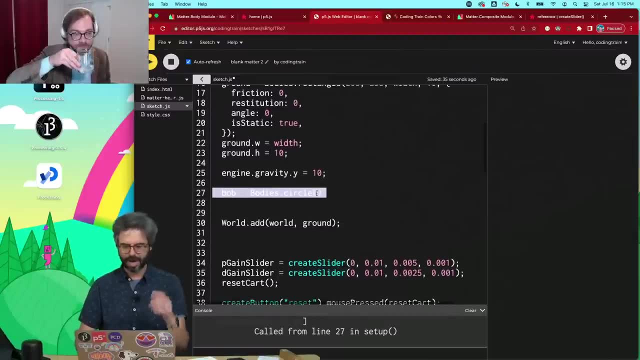 bodies dot circle, and then I give it an X and a Y, So let's have it be at the um. I want it to be at the carts location, but that's let's see. you know what. let's put it in reset. 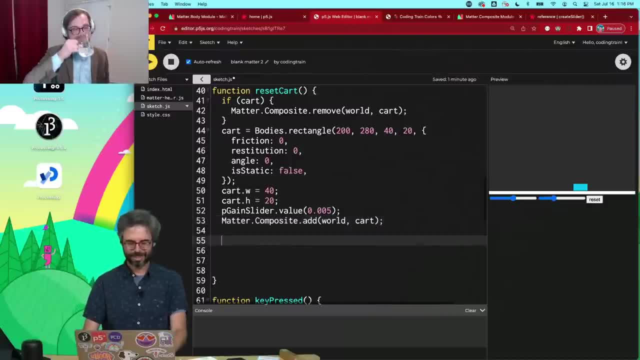 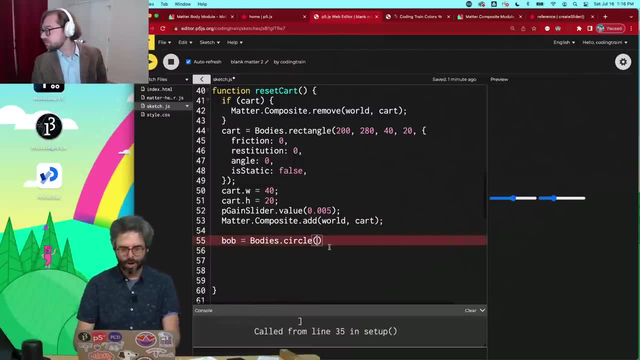 and realize we're going to have to fix this later. So, since this is kind of our like build world function now, so I'm going to re create the Bob um, because I want it to be directly above the cart, So I'm going to say the cart position dot X, and then I will just use, you know, a hundred. 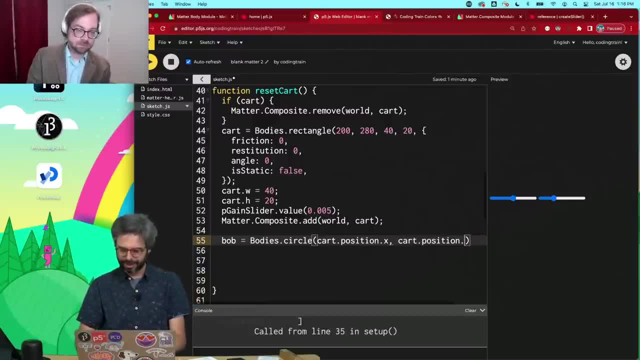 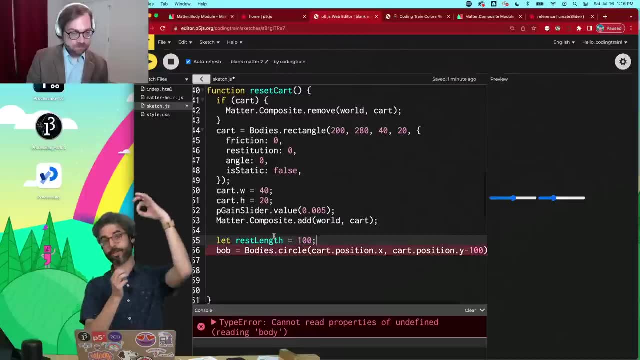 pixels. I'll. actually this is kind of silly, but let's say Y minus a hundred Cause let's have a variable for, like the rest, length of this, What's going to be the pendulum. It's, I mean, I'm. 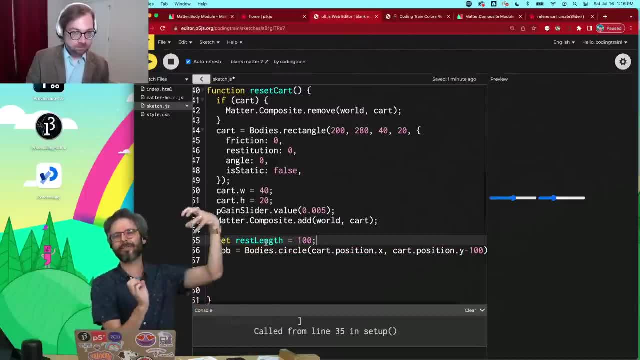 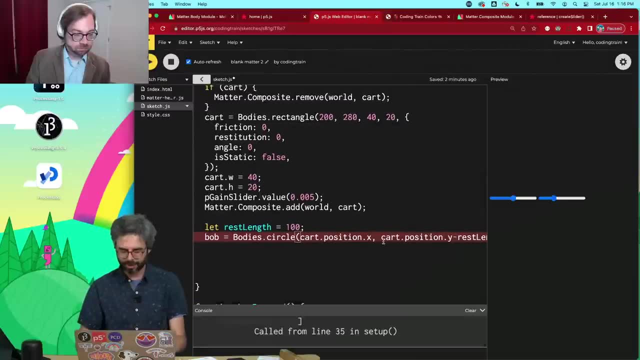 thinking of it as a spring. It's ultimately I'm thinking of it as a spring. It's ultimately I'm making a like, idealized, fully rigid spring. That's what the pendulum arm is, So that's why I'm using the rest length term. And then, what else do I need? Uh, we need an X. Oh, we need an R. 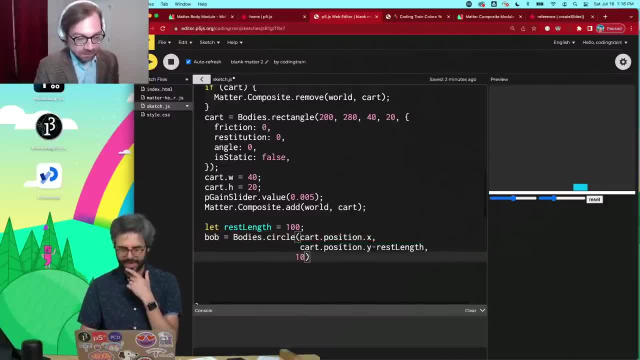 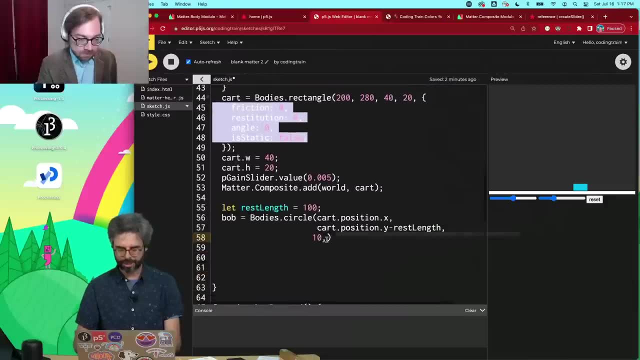 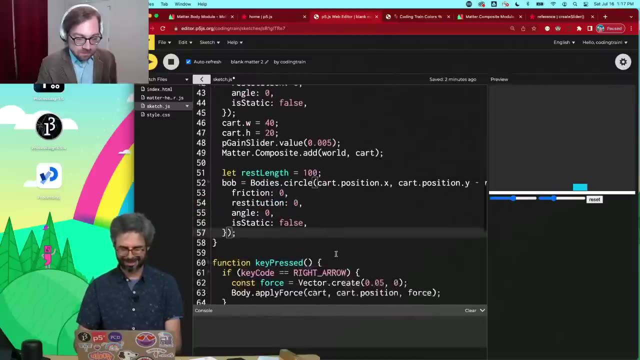 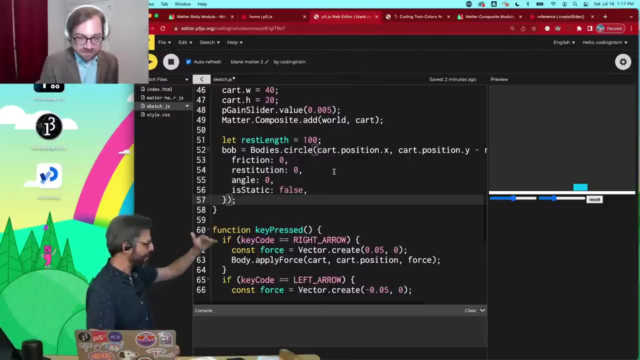 Let's have it be um 10.. And then, uh, I need all the options, these same options which I probably could just um again. I will refactor this later, But this is the Bob Now. it is a Bob that exists at the cart's position, but a hundred pixels higher. 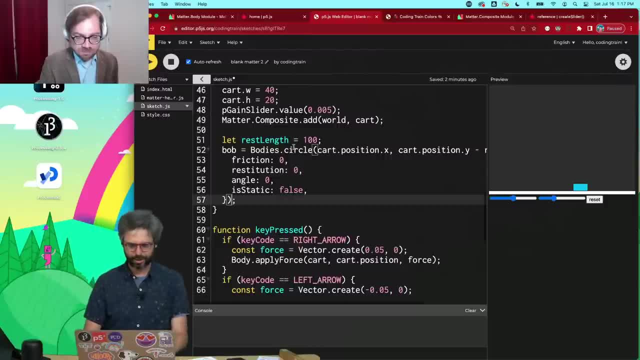 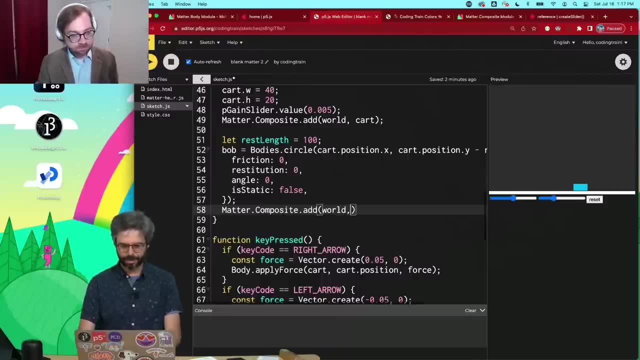 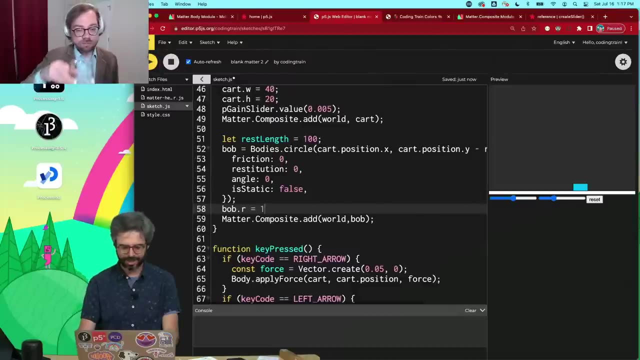 Um, and it is not static and I need to say matter, dot, composite, dot, add to the world The Bob. let's also just store that radius value again. kind of silly that I'm doing this. Let's just store it in a variable attached to the object. 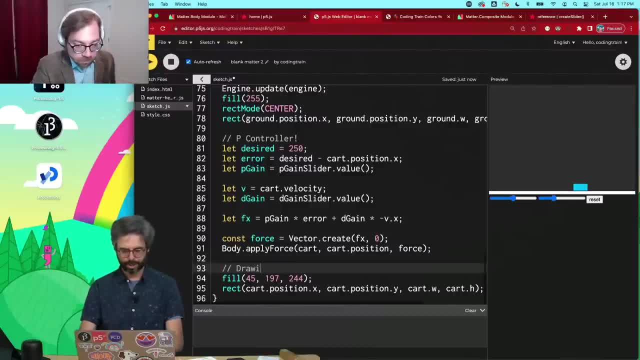 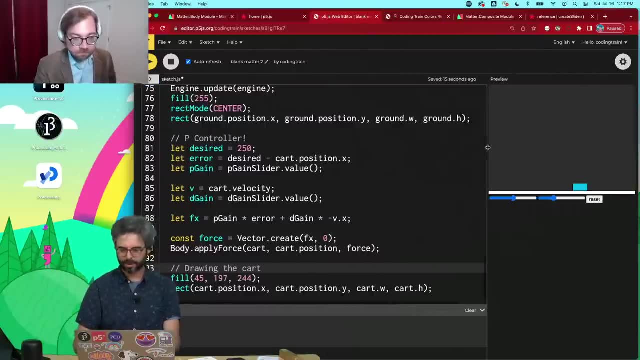 So now I can draw. this is drawing the cart, And I think I have more room here that I can put this here. Right, Make my coat a little bit wider. Right, Make my coat a little bit wider. I think you could. I'm slightly And if I stand over here, 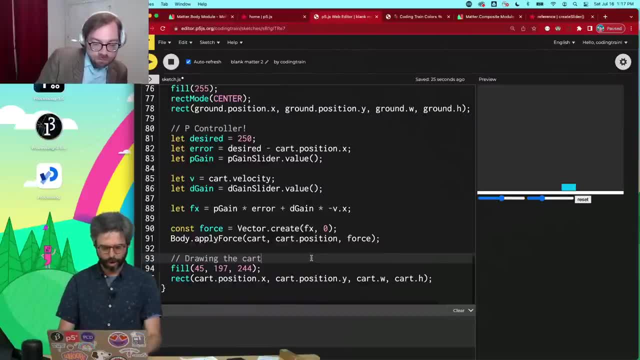 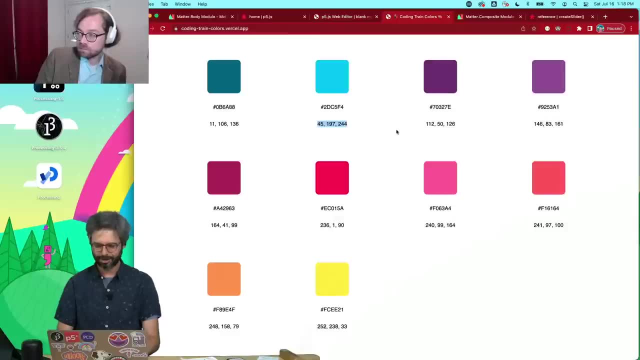 okay, My set up's a little bit better now. Um, drawing the cart: now let's draw the Bob. Drawing the cart: Now let's draw the Bob, We'll get a different color. Drawing the Bob, We'll get a different color. 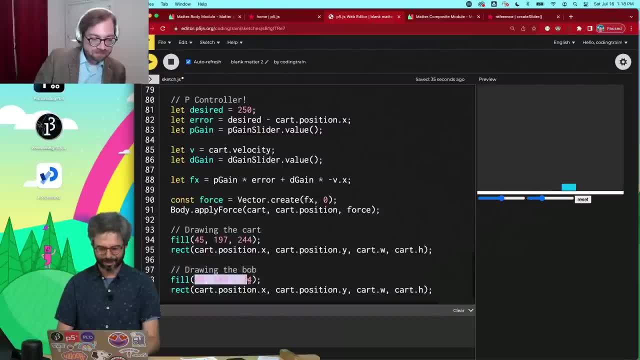 Drawing the Bob, We'll get a different color. Oh, actually, I'm going to have to do something else. I'm going to have to do something else. closed it. but that's fine, we don't really. the color is the sort of, is not the important detail. 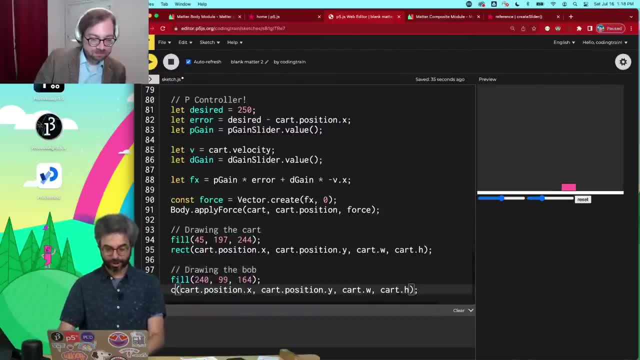 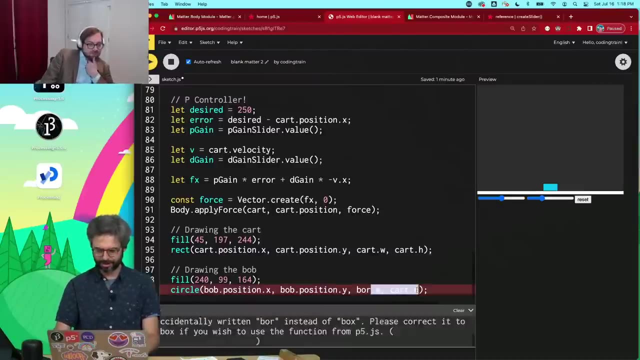 here, uh and the. it is a circle which is at the bob's position and oh, why did it fall through the ground? that is strange. um, we're gonna have to figure that out. bob dot r times two. okay, what did i miss? oh, did i not add it to the world? 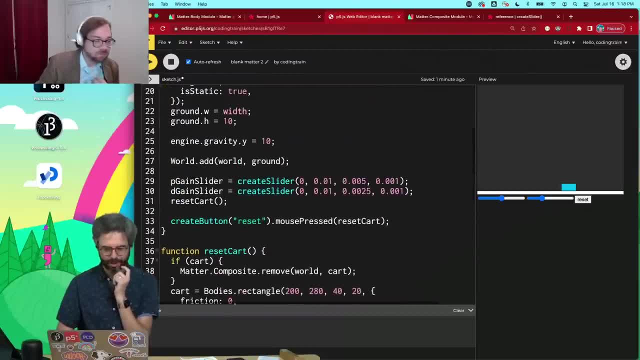 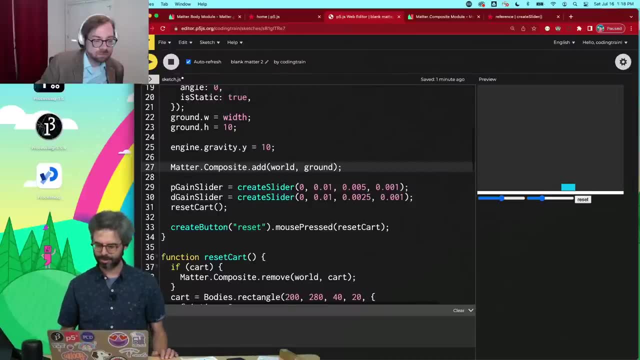 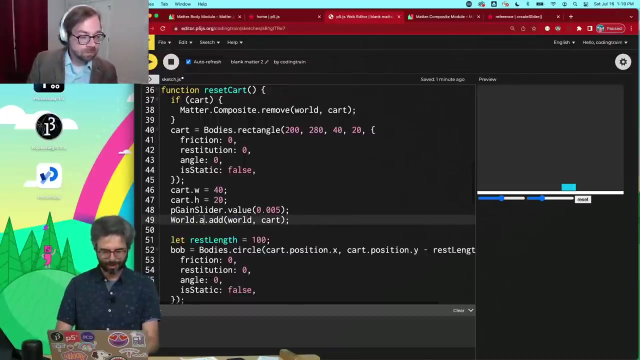 no, i added it to the world, did i not add the ground to the world? oh, you know what it is. i wonder if. all right, let's go back to. i'm just curious because the uh, let's this is. i'm just going to go back to my old-fashioned worldad. 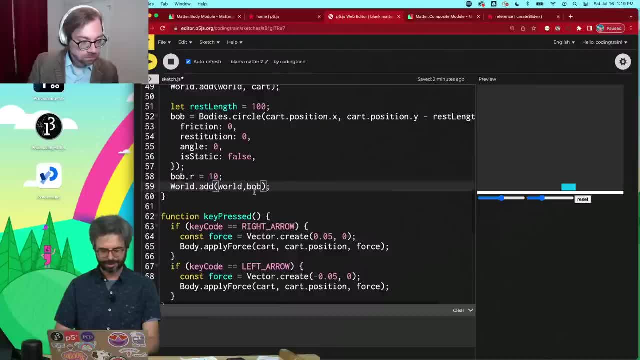 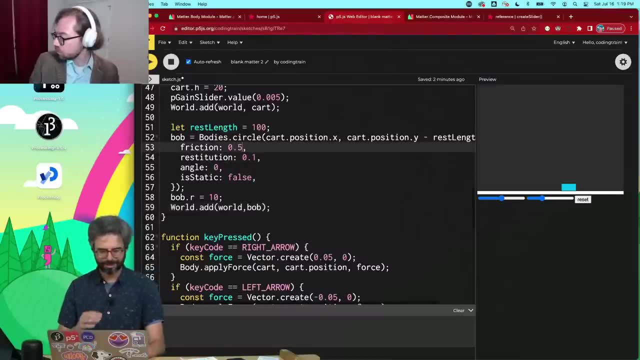 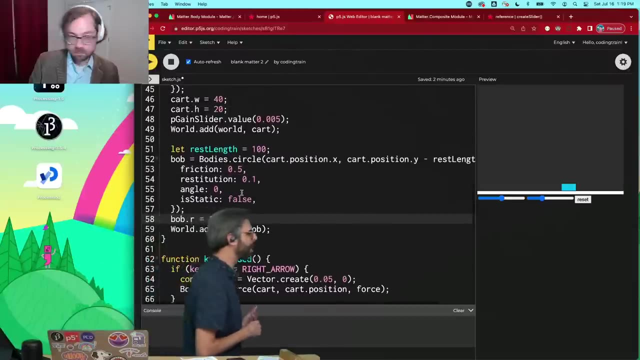 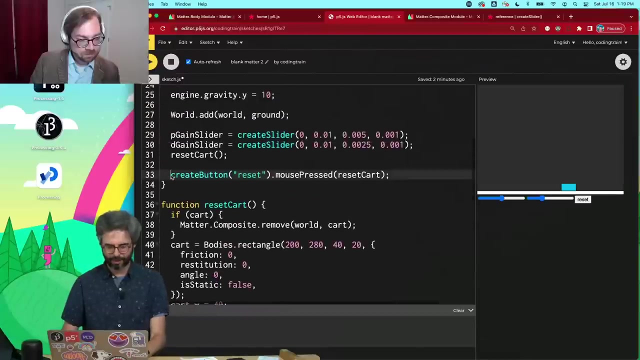 and let's see what am i missing here? let's give it a little restitution and friction. this is strange i'm trying to think of. i'm going to look at the chat. you forgot to remove the bob after resetting. no, all right, i'm going to take out this idea of the reset button right now. 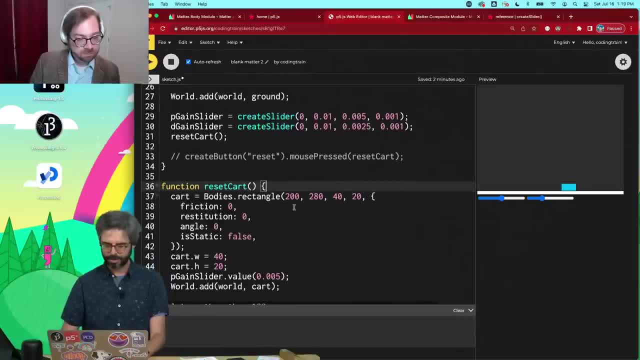 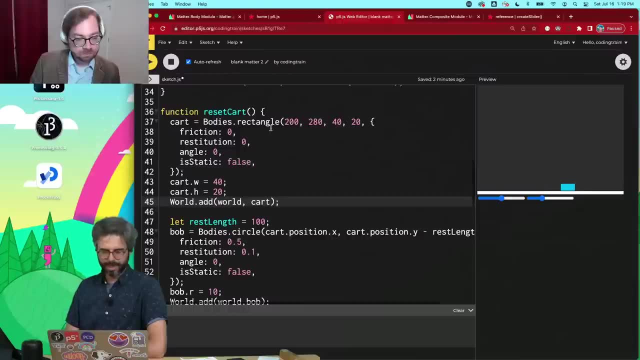 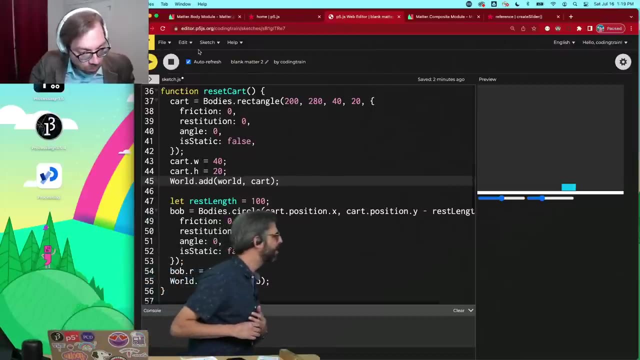 and take this out. so this is just creating the world. let's take a look at this we are. we make the rectangle bodies dot circle. all right, i'm going to go to my code, for i'm looking at the chat. i think the gravity is so high that the euler integration is starting to mess up. i have seen this. it's i'm back just hard to keep up with thiselethe görüş dicho kau, an activation that the oiler integration is. 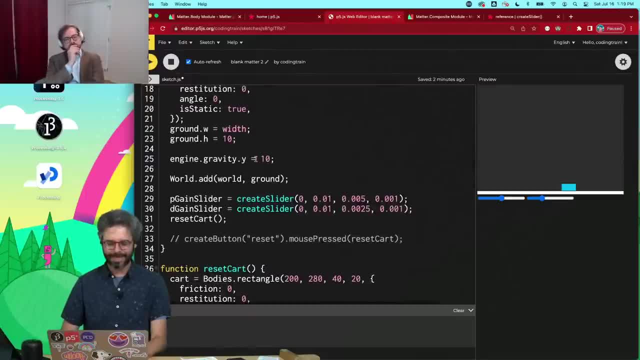 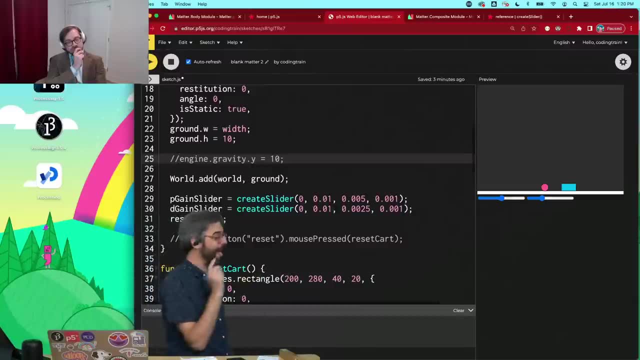 starting to mess up. i have seen this it's i'm probably need to change the time step. let's change the gravity. oh yeah, so that was simon, a great comment in the chat. so this is something that i we have seen when i write my own physics engines. 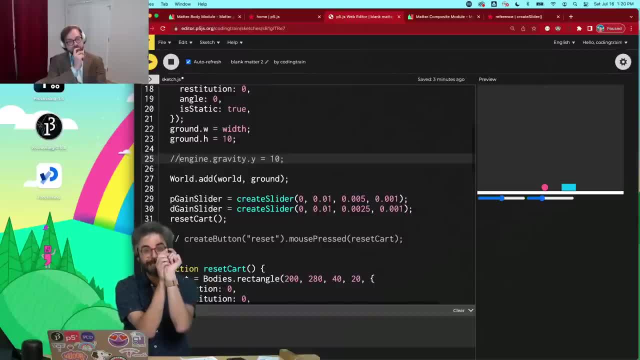 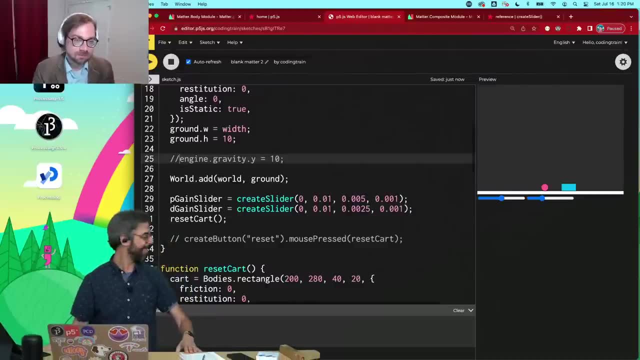 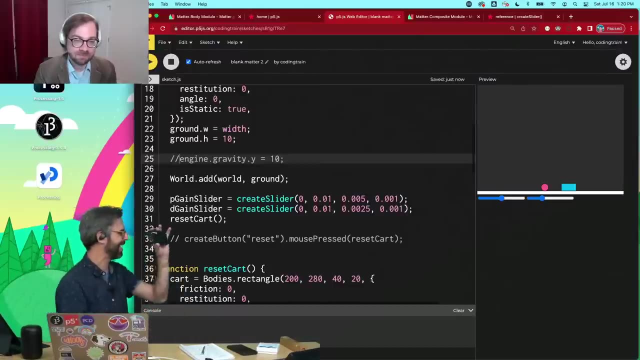 that if, and in christian's python code there was a variable called dt which controlled the time step, and you can imagine, like, if this desk here, right, i'm gonna raise this up a little bit- if this is the ground and this little elgato hdmi capture thing is the bob, if i were to drop it, right, it's. 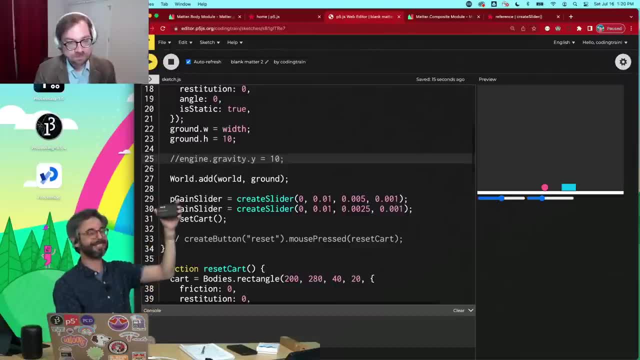 really following continuously through air. but our simulation is doing this: calculate a time step and then teleport it to here, then teleport it to here, and so if those time steps are really big, boom, it's going to like skip past the ground. it will never actually make contact because it's. 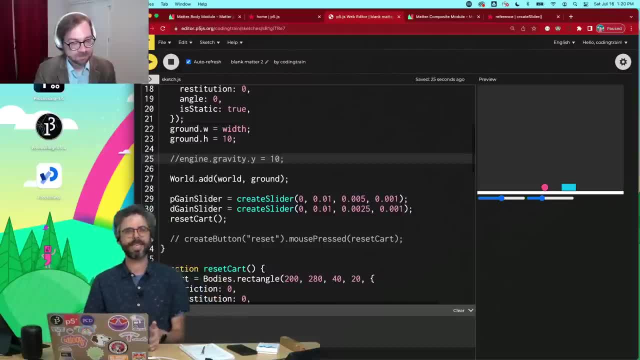 able to leap over it, and there are all sorts of ways in programming physics engines. box 2d is a very sophisticated methodology for this. um, i think there's probably a way for me to alter the time step. but i'm actually just right now. i'm just going to leave the gravity by default. 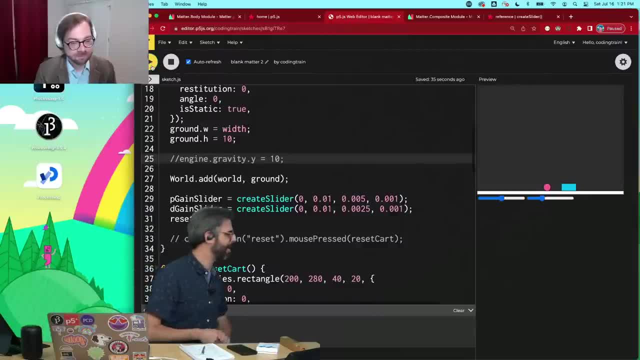 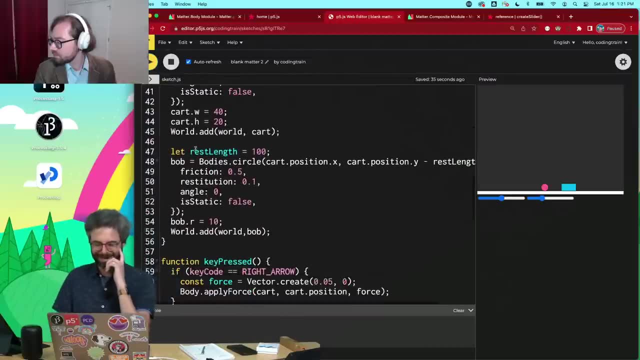 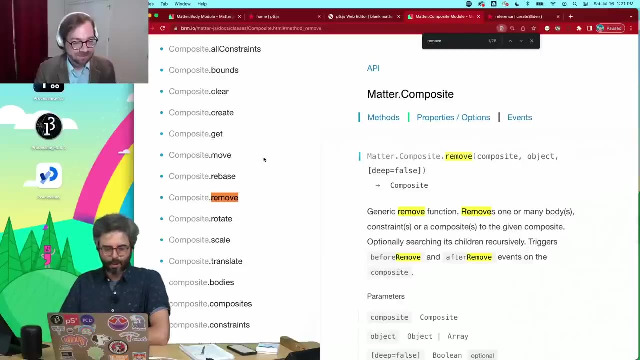 and we've got it working. okay, looking at chat: okay, the gravity, the gravity, all right. so, but now we've got that working, uh, and i i made some unnecessary changes trying to debug that, but i'll just leave it as is. the next thing we need to do is create a constraint, so let's go to the matter. 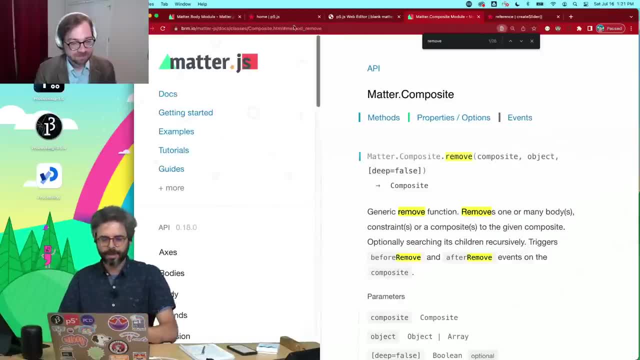 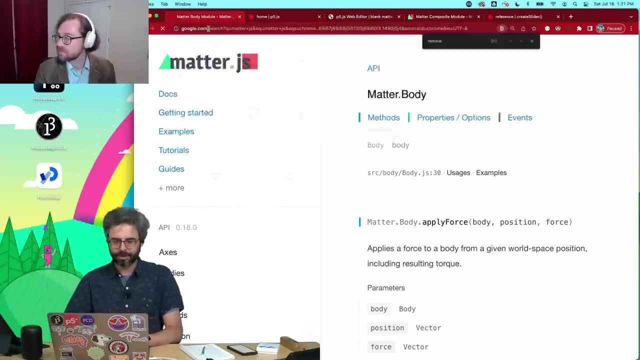 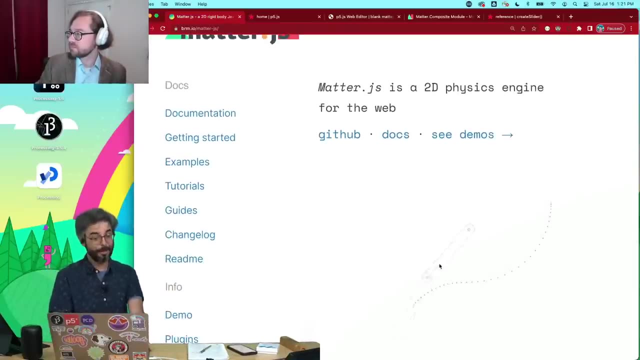 website, the constraint by. so if you go to, um, the home page of matterjs, um, let's just see, uh see, these demos, like we have this newton's cradle, we have this like this double pendulum right here. anything, we have these springy things whenever two bodies are attached to each other via a spring. 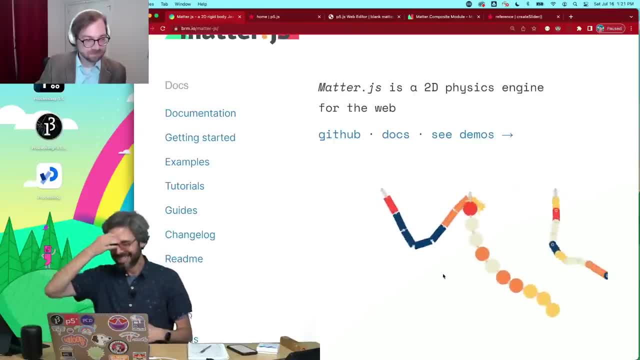 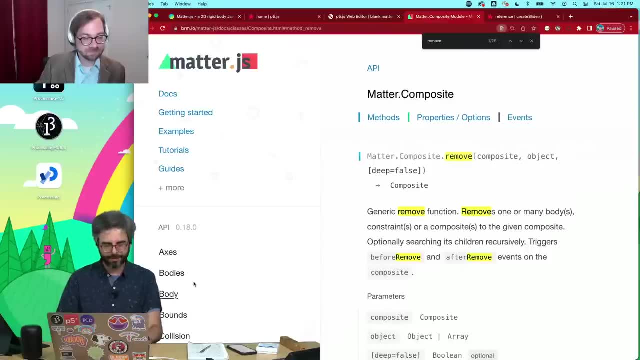 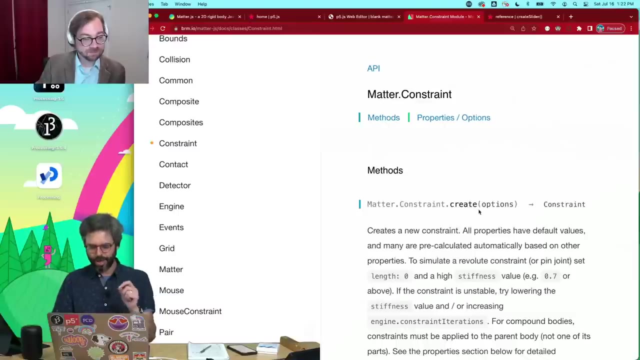 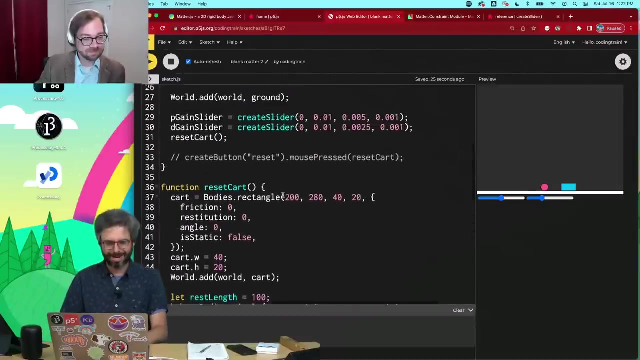 however, uh, springy, it is. um, oh, look at all these wonderful examples. uh, that's called a constraint. so i'm going to look at the documentation under a constraint and basically, i want to create a constraint with a set of options and let's do that here. so i'm going to do this in my um, i'm just 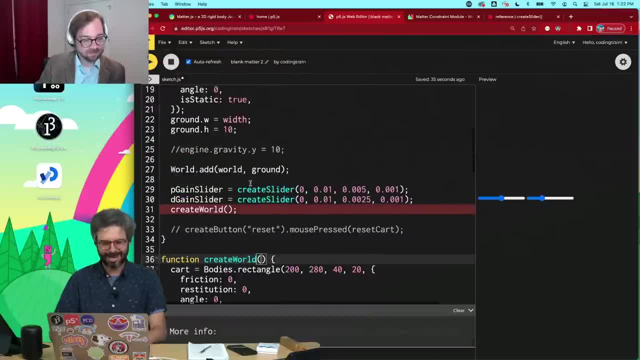 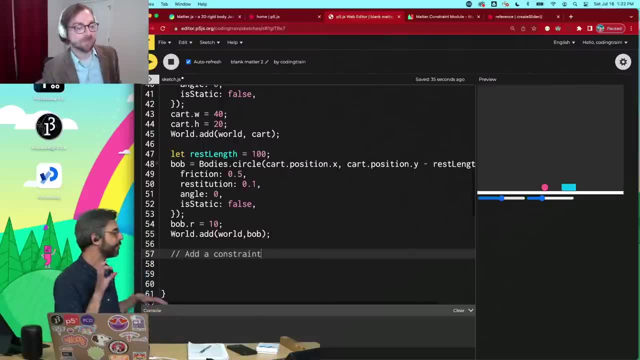 going to now call this create world, this function, and i probably should put the ground in it too. but we can fix that later. let's add a constraint. and again after the stream today i will go to the code and then go through and kind of comment all of the code so that the released version has more. 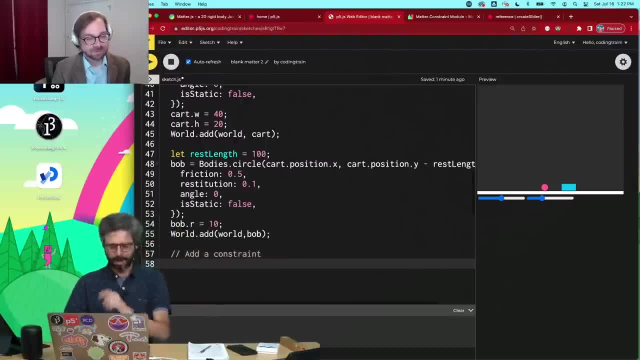 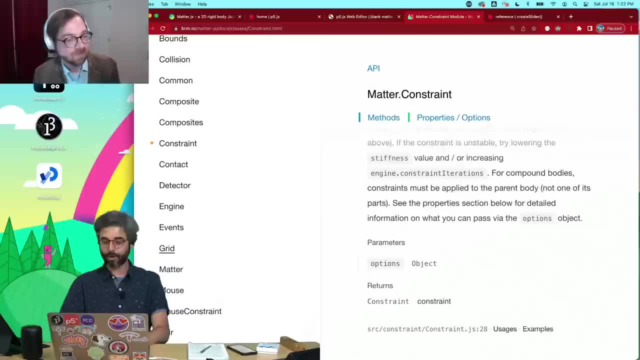 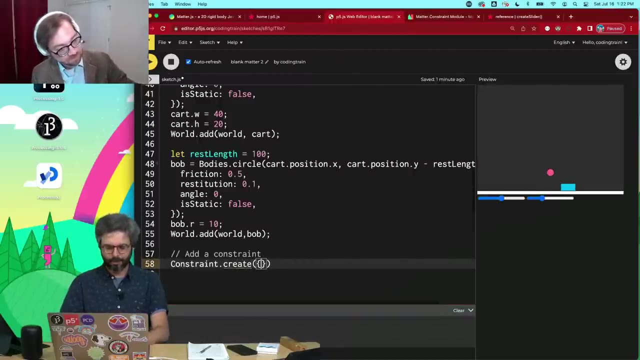 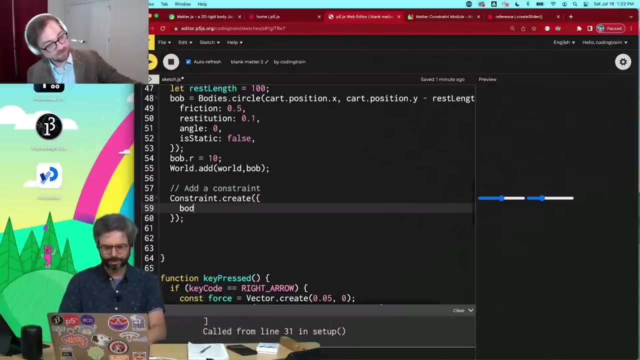 explanations in it, and you know i'll do some cleanup as well. um, so we need to say: um constraint, i already forgot create, constraint, dot create. where is that? uh, cut, create, create, and then i believe we give it a set of of options. so now i think it's just assuming. it's giving me an error. 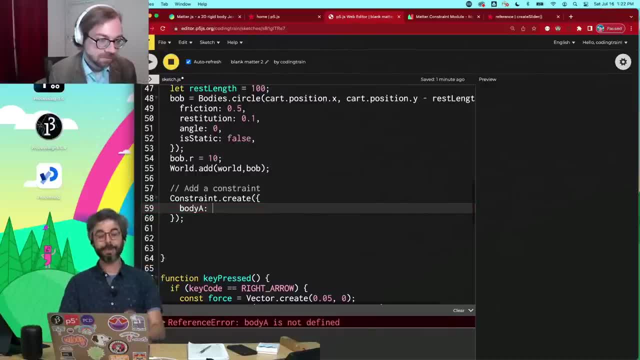 Let's turn off auto-refresh for a second. Now, body A: I believe the first thing you do with a constraint is you say which two bodies are attached. So body A is the cart and body B is the Bob, And somewhere in this documentation. 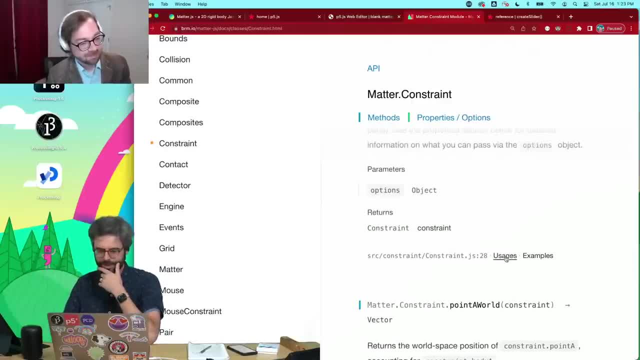 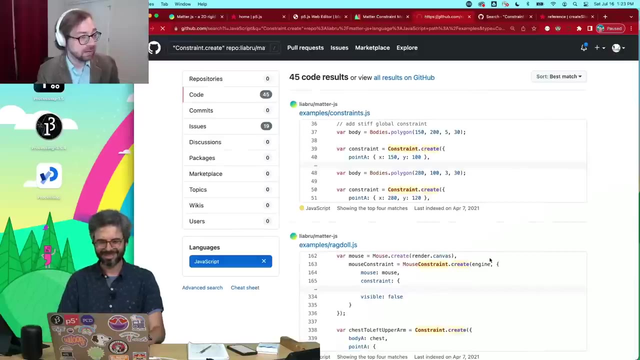 I should see all of the usages or examples. Let's try here. Let's go to examples While you're looking that up, Daniel, in dynamics- multibody dynamics- when we add a constraint, we add something that's called a variable, called lambda. 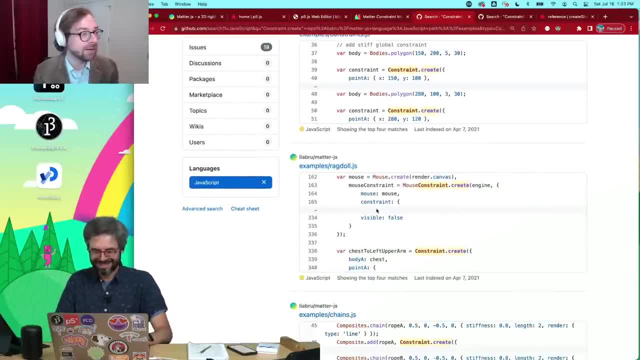 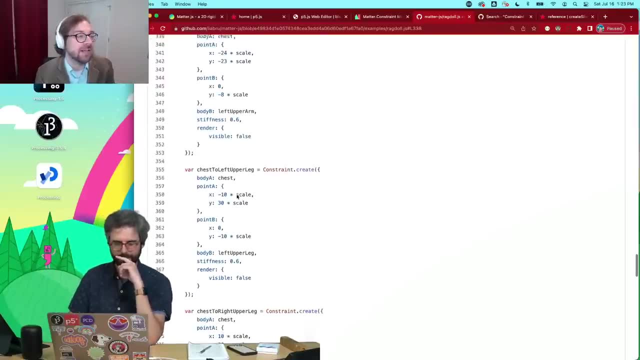 for every constraint and it's called a Lagrange multiplier And that's how we handle the math and deriving the dynamics. Basically, it's the force that makes this constraint happen. Obviously, that's not relevant in any way to you fixing your problem. 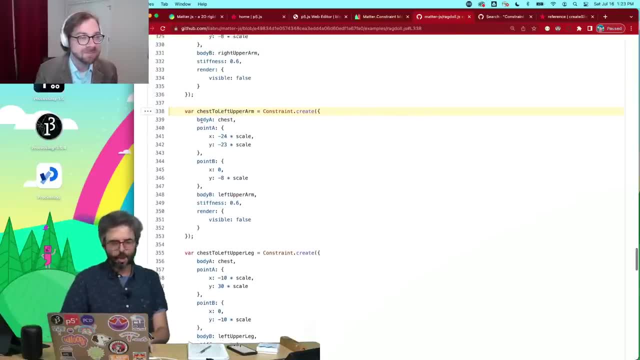 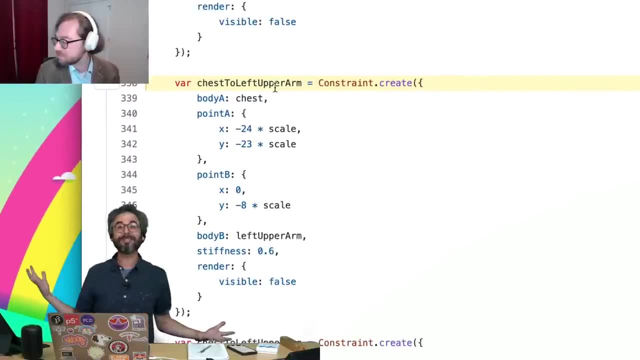 but it just ties back to how we do it in robotics, So there's probably a better example. I just sort of clicked through and found this example and we can see this is actually. I found an example of a ragdoll simulation with matterjs. 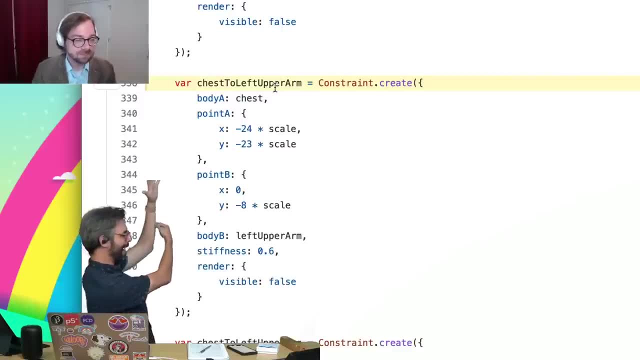 And you can see, here is the chest to the upper left arm, or maybe that's, I don't know. I don't know what part is what- an actual anatomy here. but you can see we have two bodies and then we have a stiffness. 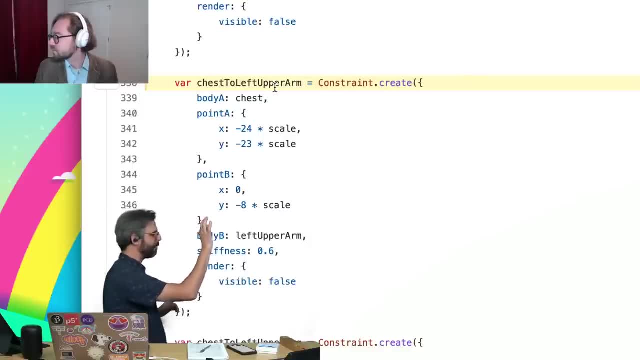 That should be all I need. I think There is a point A and a point B. I think that's just if you want the constraint to be attached to the offset from the center of the body, which I don't need for this. 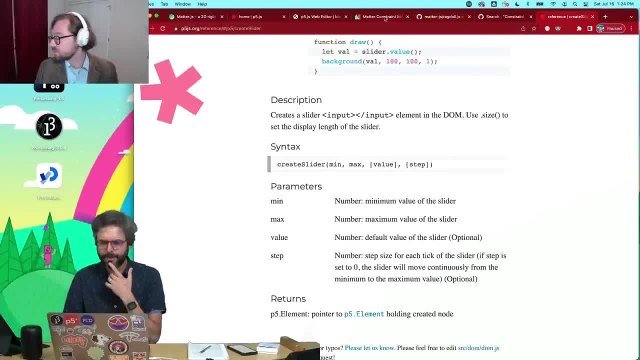 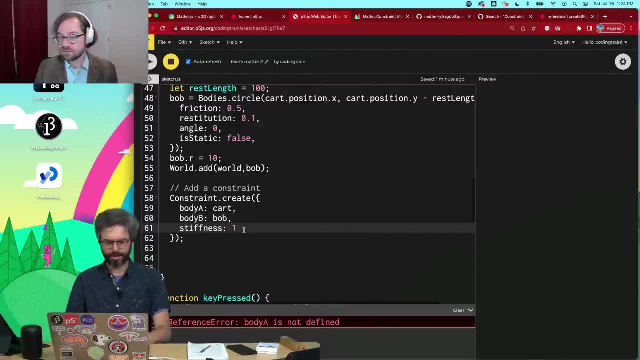 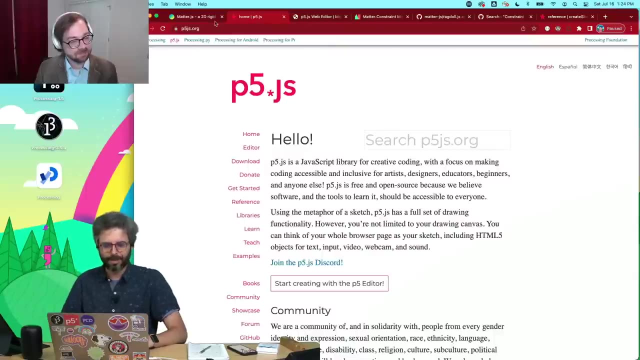 So let's see if that's all I need. Like, where's my sketch again? Body A, body B: stiffness of one Body A is not defined. Oh wait, no, no, All right, you know what I'm gonna do here. 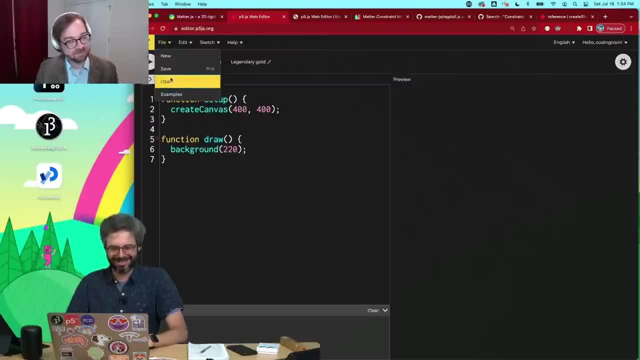 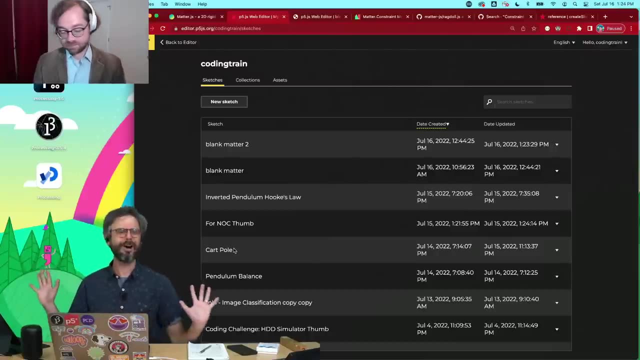 Is. I'm just gonna look at the thing that I was making yesterday and see what the constraint code is there, because I think you know we've been going for a very long time and so I'd like to kind of get this wrapped up here. 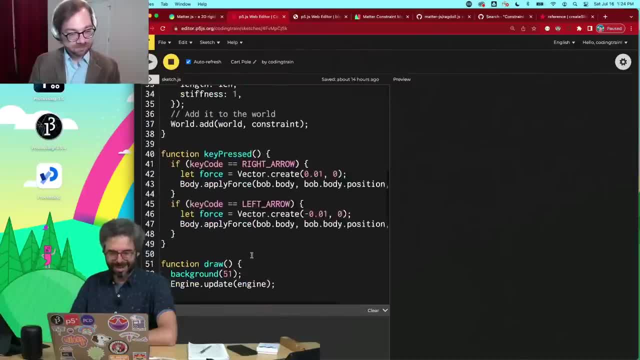 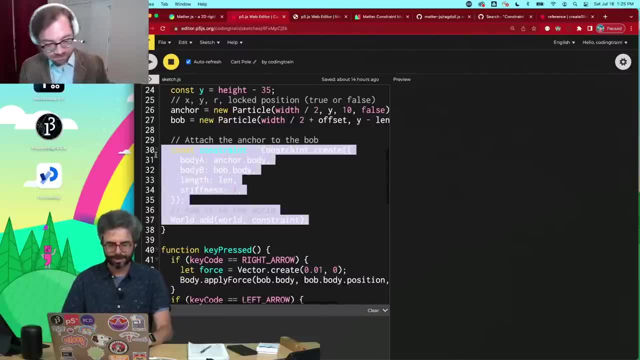 and I think this will help us get there a little faster. Constraint body- oh length, I'm missing Constraint creates. let's just take this. Let's grab this code here that I wrote yesterday as I was trying this idea out: 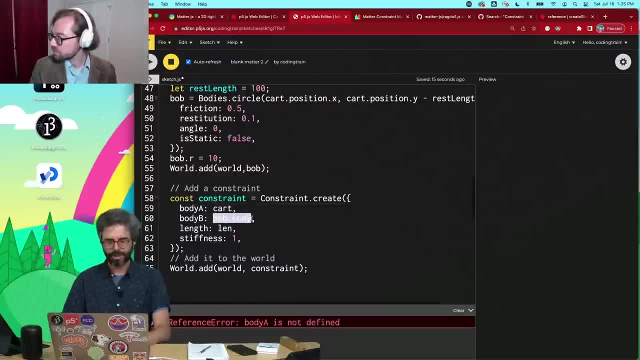 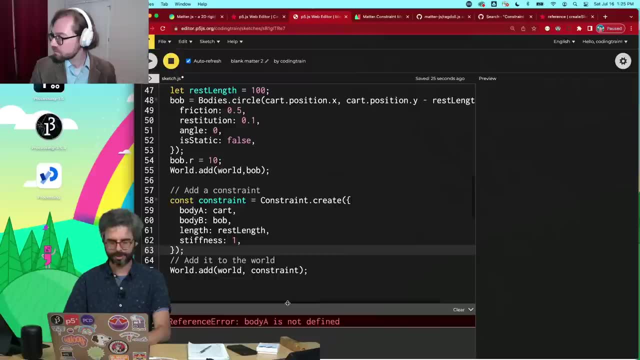 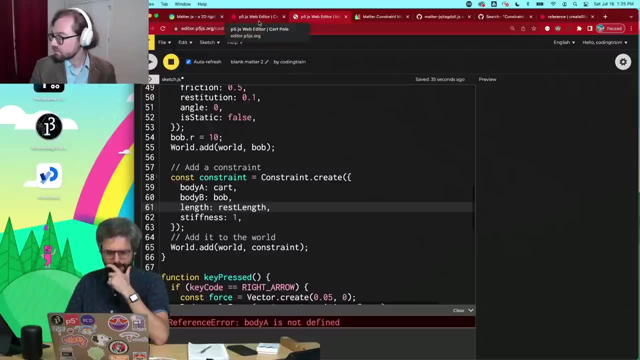 And so we're going to go to the cart, the bob, the rest length which I set up here, and the stiffness. Why is it saying body A is not defined? So let's take a look at. what am I missing here? 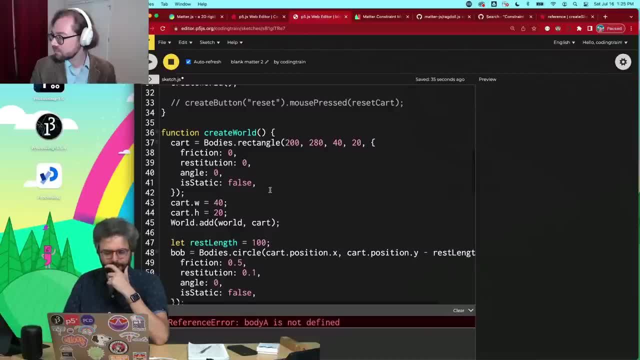 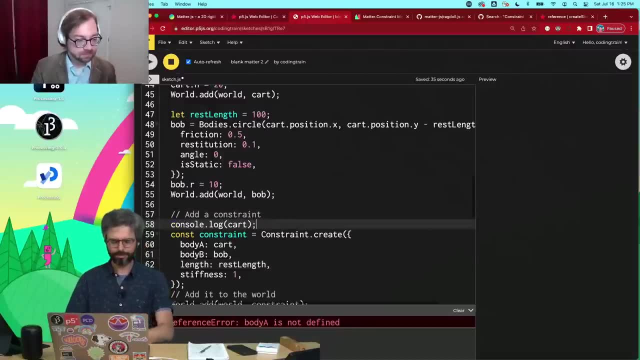 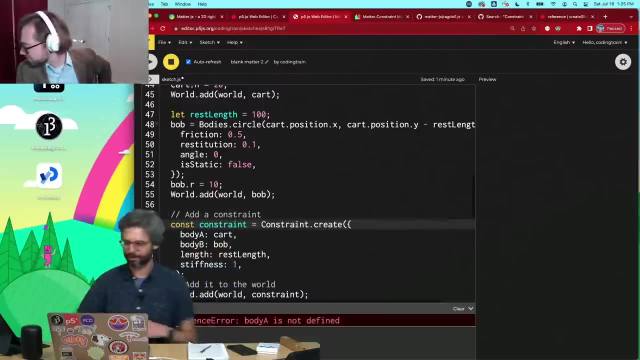 Is cart. oh, is cart not made yet? No, cart is a body, Bob is a body. Hmm, This is where the chat always comes in and helps me out. I disabled auto refresh. Yeah, yeah, yeah, Oh, okay, no, we're fine. 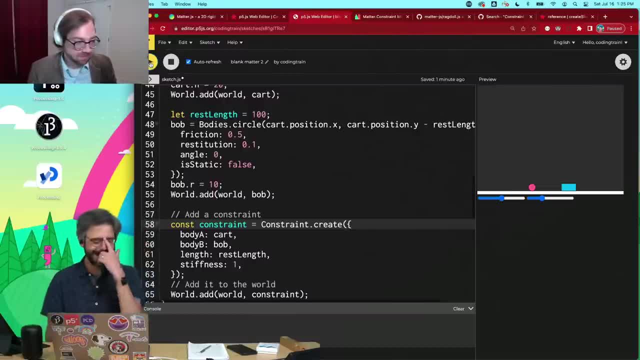 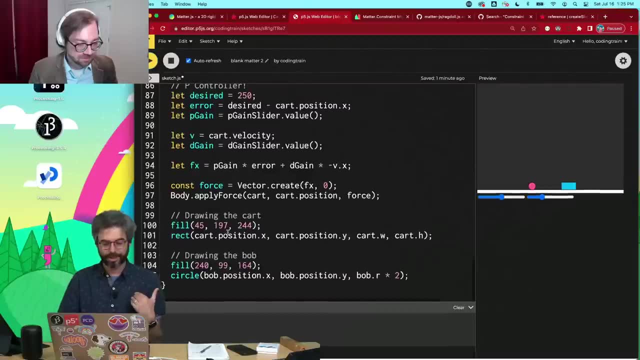 The constraint is there. okay, The constraint is there. I think I just- I don't know I hadn't fixed it and run the code in the right order. Okay, the other thing I want to do is render that constraint- That constraint, by the way- by default. 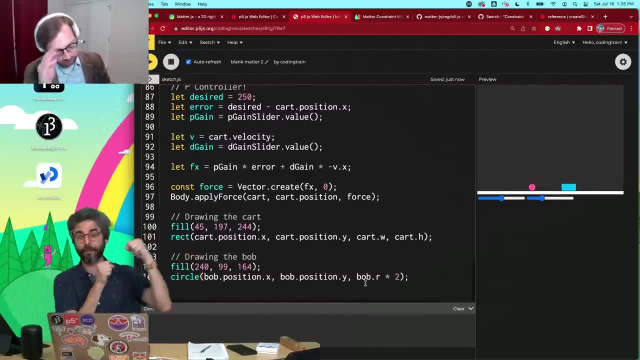 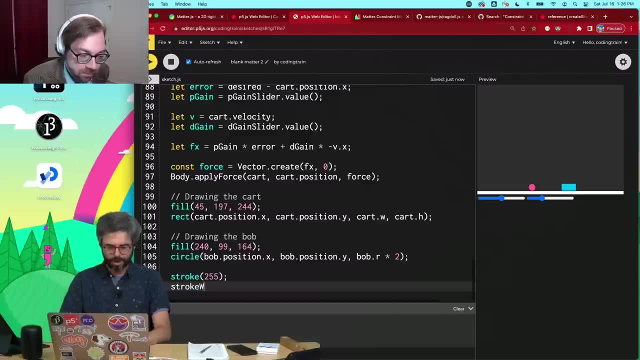 doesn't have any mass, It's not. there's no geometry associated with it, It's just a force. But for our purposes- let's not worry about color here- Let's draw a white stroke with a thickness of four pixels, And we'll just draw a line between the cart and the bob. 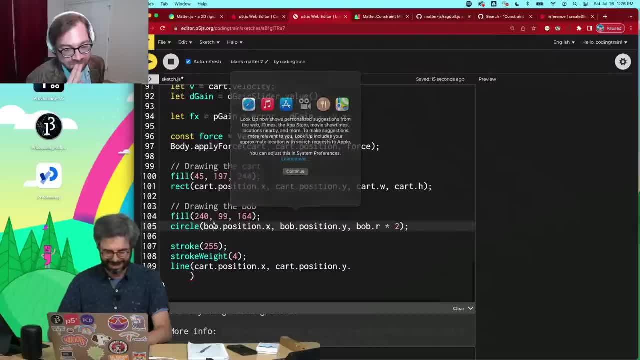 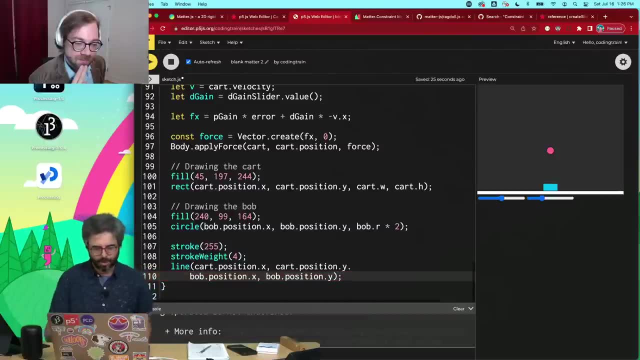 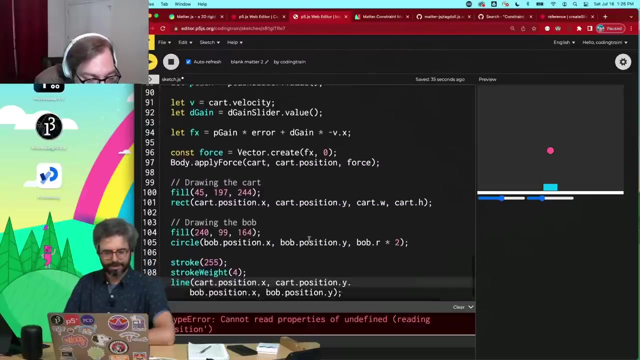 Oh, Oh, No, okay. So what am I? what's wrong here? Stroke cart position X: What is undefined Cannot read property of undefined line 110.. Hmm, Oh, look at the chat again. Look at the chat again. 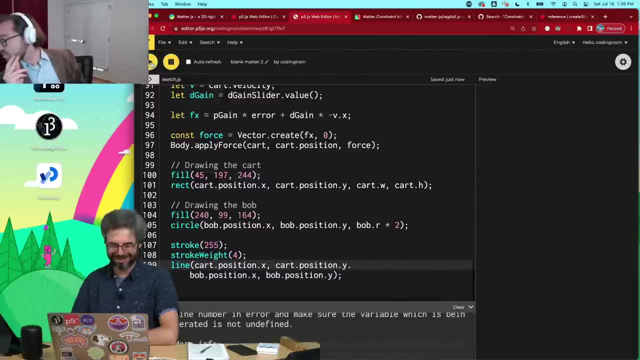 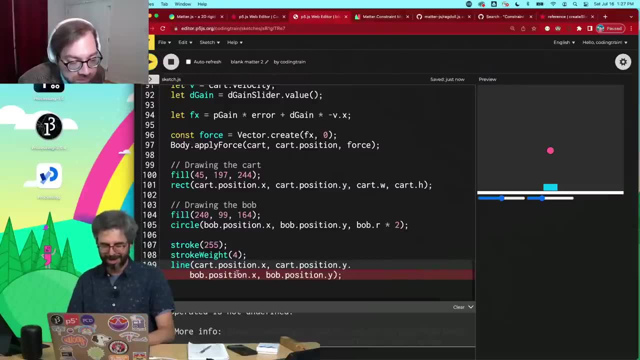 out again And everyone's telling me I forgot to press play. but that's not the issue here. What is going on here? Cart position X. cart position Y. Bob position X. We just drew a circle there. We just drew a rectangle there. 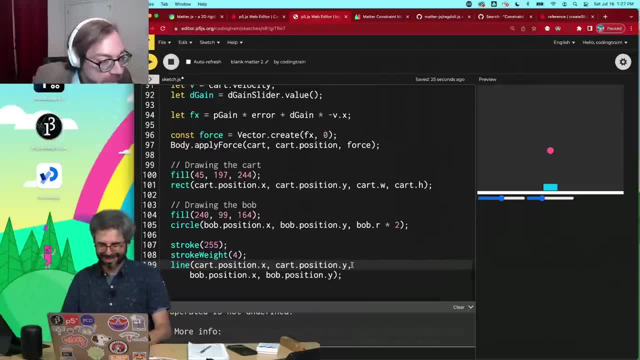 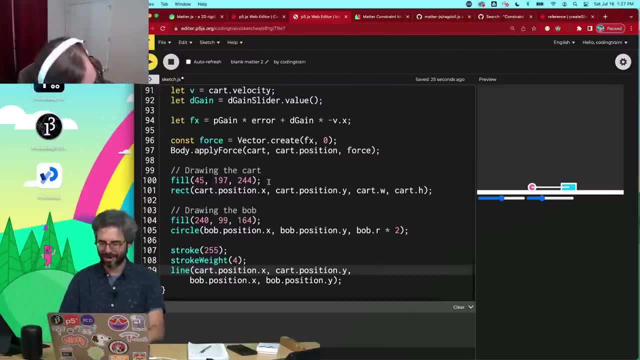 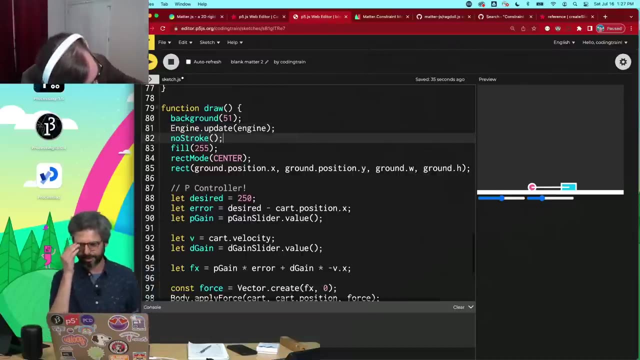 Oh, there's a weird typo. No comma, That's a comma. There we go. Yeah, Okay, Here we go. Oh, and I've added this like very thick stroke to everything now. So before I draw these elements, let's put no stroke, Okay, And I put auto refresh back on. 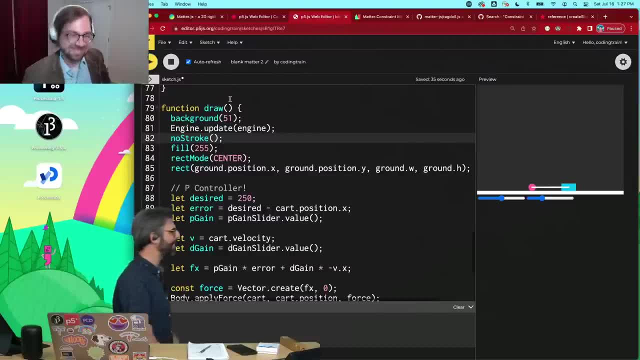 There we go. All right, Look at that. Now, of course, our pendulum is just falling over because my controller is not attempting to balance the chat, by the way, So the chat is 30 to 60 seconds behind us. 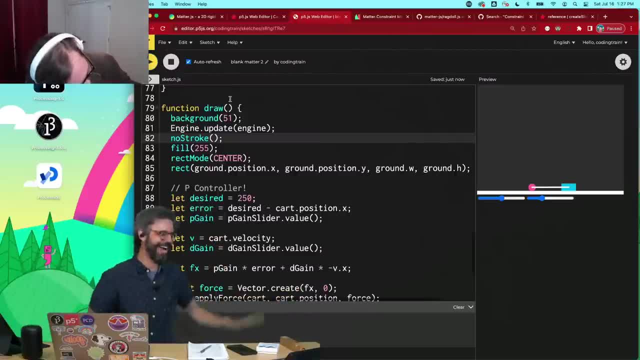 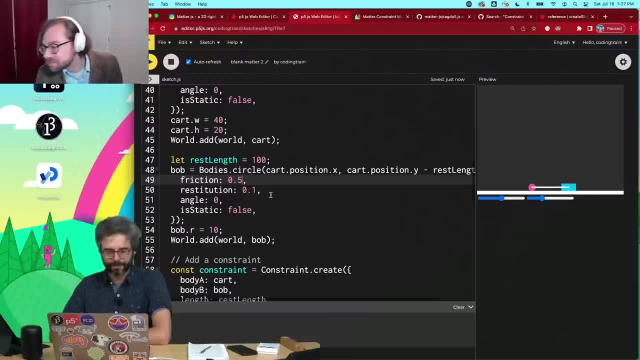 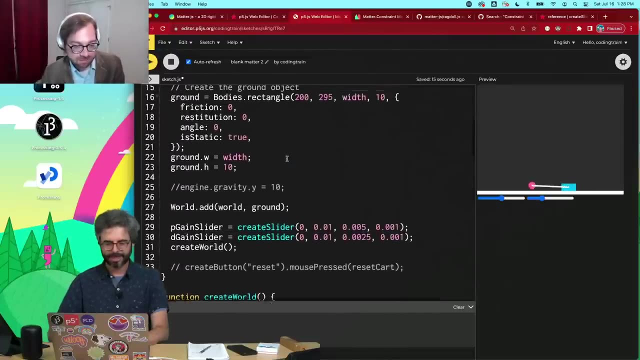 So you can see like comma, comma, comma, comma, comma, comma, comma. Okay, I got it, Let's add, let's take out the friction, but let's put a little bit of bounciness in there, just because I think it'll be kind of nice to see it, the pendulum bounce when it hits the ground. 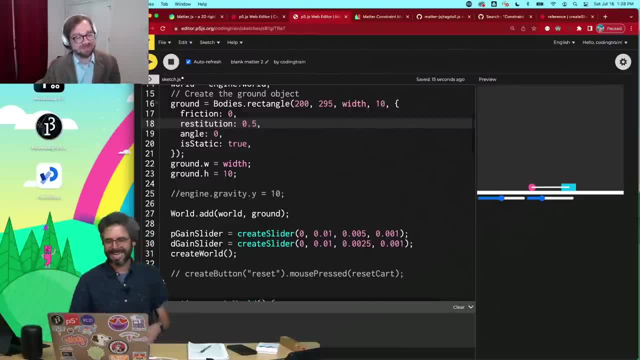 Let's see. Yeah, there we go. That has a nice kind of feeling to it. Again, I need to really do some tuning to my controller. I need to really do some tuning to my controller So it doesn't go flying off into the air. but so be it. All right, We're getting really close. 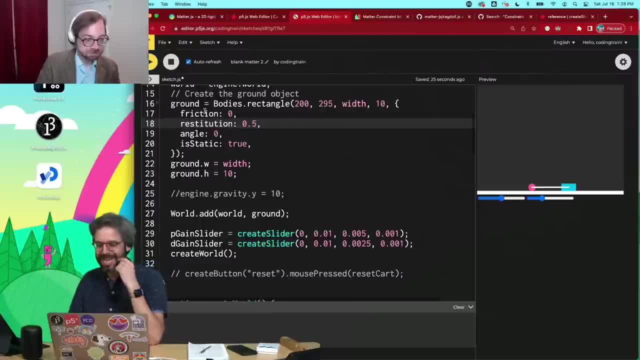 to the end of this, I think: right, Yeah, So the next thing I need: yeah, go ahead, Go ahead. I'm sorry, No, you're you're, you're, you're, you're the. why don't you tell me? 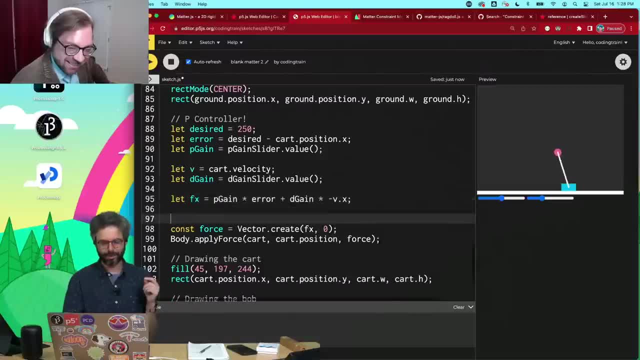 Okay, So I need to. only the thing that I need to do is the calculate the error now, as not the difference in X positions, but the difference between my ideal angle and what the current angle is. So my ideal angle, if, if my reference point is the Y axis, would be zero. Now, 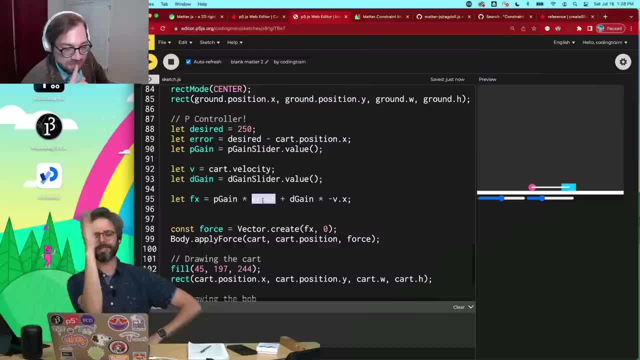 how I get that angle might end up being that might be 90 degrees or negative 90 degrees. So let's see. The question is: is matter going to give me the angle or should I calculate the math for the angle myself? I think I'm just going to do it myself in a very ridiculous way. 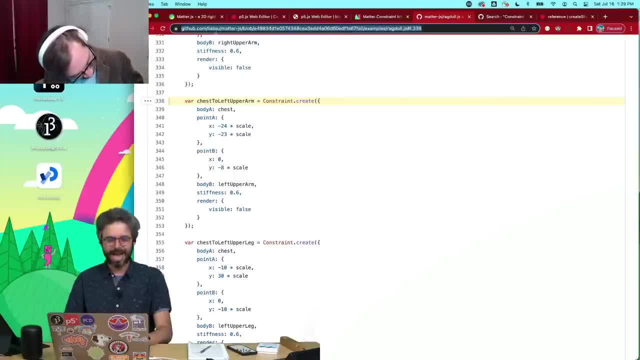 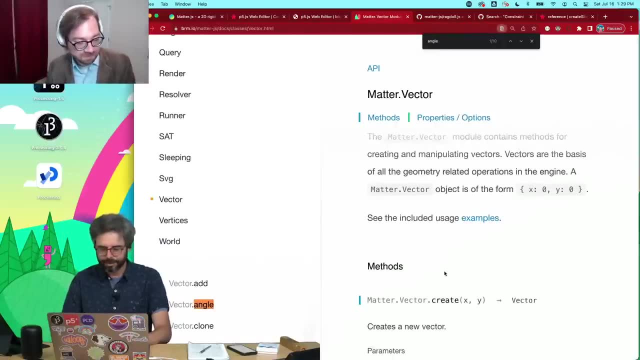 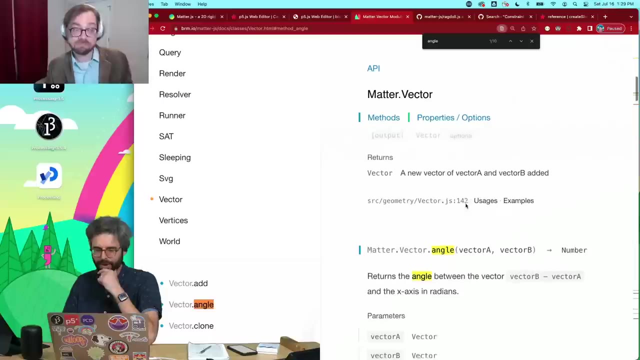 Unless. let's just check the math Matter vector, Let's check the matter vector object, because maybe it has like a heading function in it. Oh, like an angle Vector angle. Yes, Oh, that gives me the angle between two vectors, which I could certainly use, but that's not what I want. I want the angle of just the. 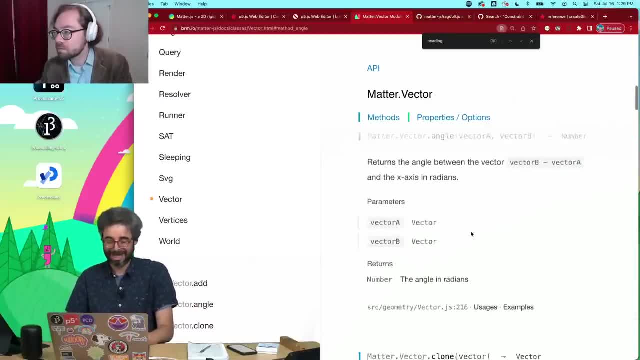 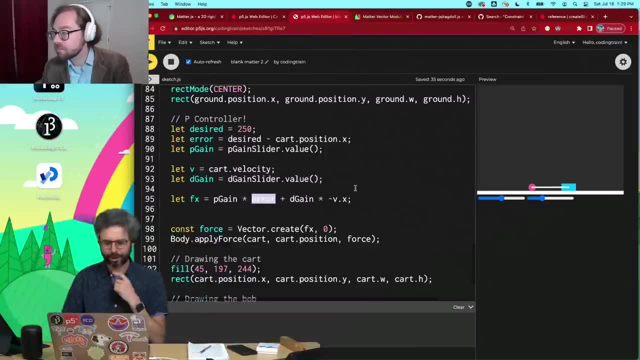 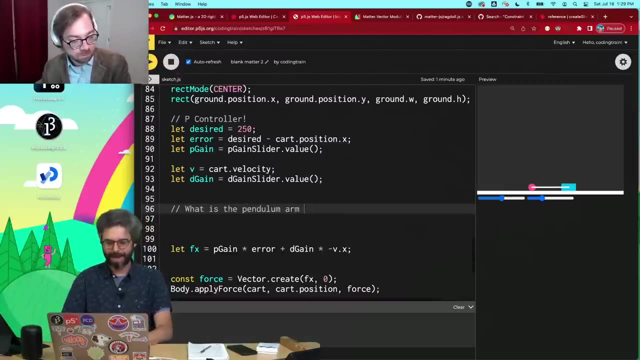 heading of a vector. I know how to do this myself. I was just wondering if matter would give it to me. So maybe somebody in the chat will tell me. but I'm going to just do this in a very, very crude, raw way myself. So let's, let's add a comment here. What is the pendulum arm angle? 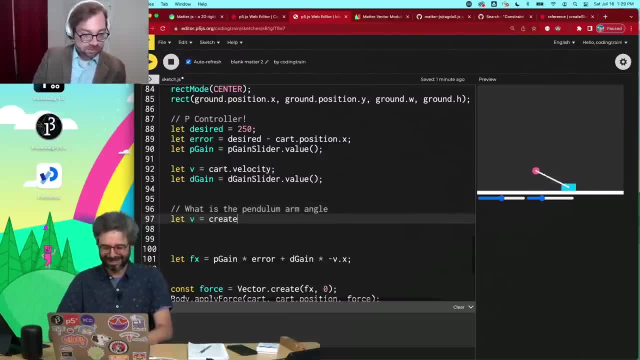 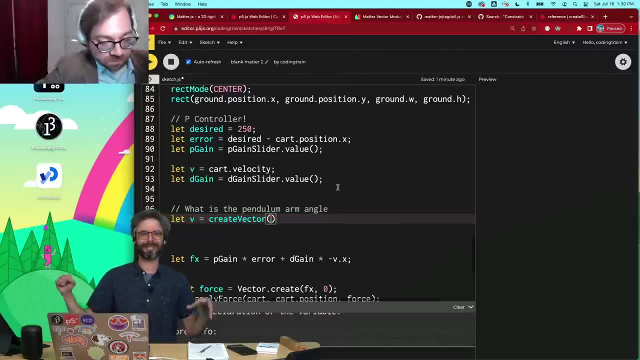 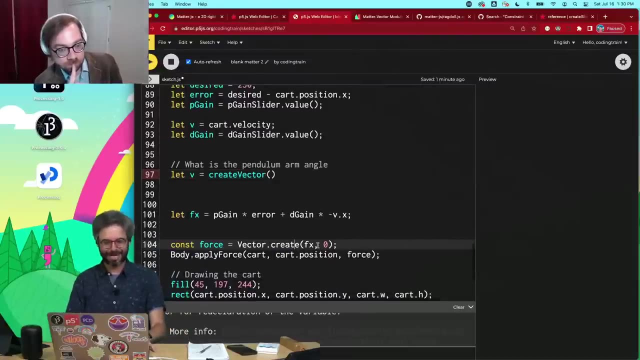 So I'm going to make my own P5 vector. So here's a really terrible idea that we will correct later. but I'm mixing, I'm not mixing metaphors, I'm mixing physics libraries in that matter. has this vector object called vector dot create? but I know the P5 vector object like in and out? 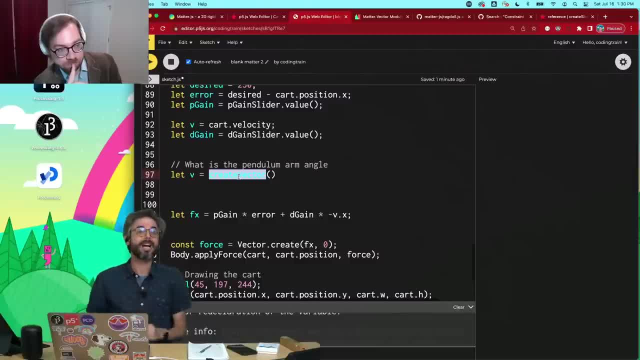 like it's burned. I'm going to mix this into my brain so I can get an angle from it really quickly. I could also use the, a arctangent function. so many ways I could get this, but let's just do it this way. So I want to. 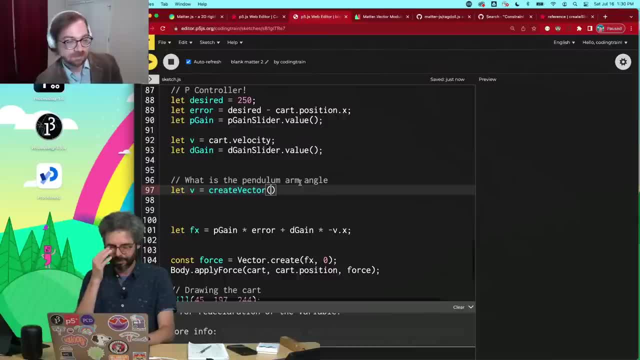 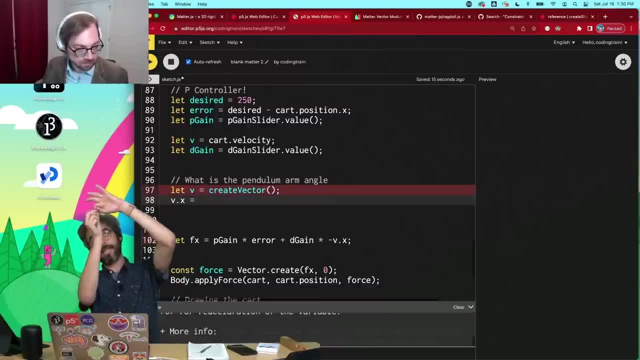 create a vector which is the. I'm just going to create an empty vector And then I'm going to say V dot, X is the Bob's position minus the cart's position. And I could go over to my whiteboard here to diagram this, but I don't want to do that, So let's just do this, So I can give it a. 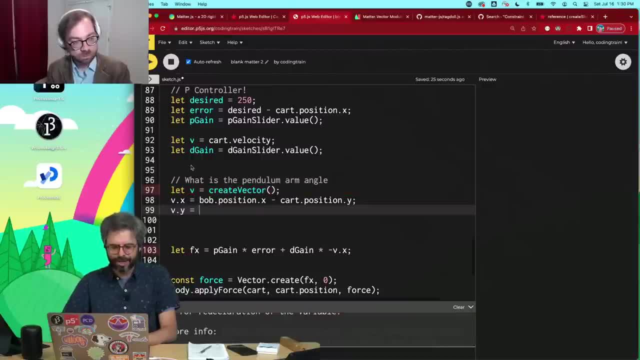 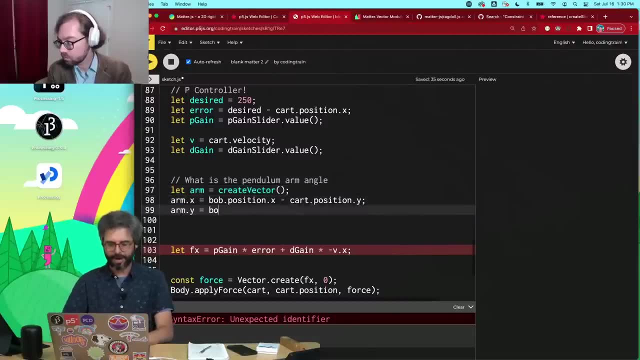 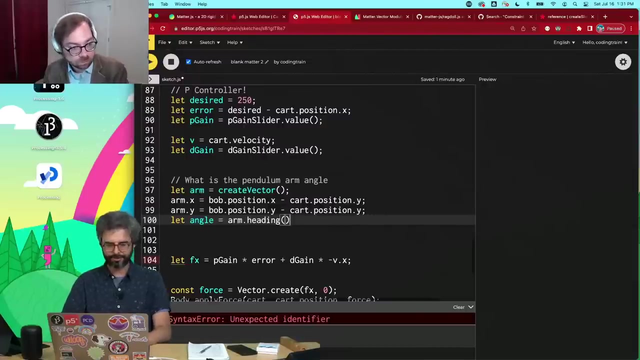 I used v already. Let's just call this arm. It's a vector to describe the arm. And then bob position dot y minus bob cart position, dot y, And then I'm going to set the angle to be the arm's heading, So again I could do this mathematical calculation. 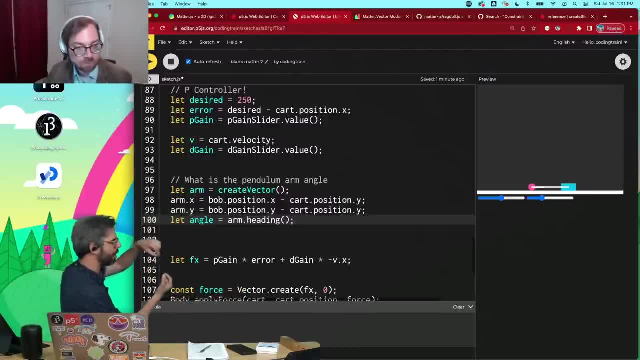 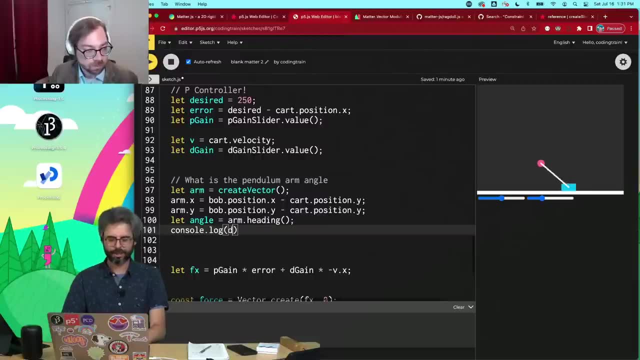 myself, but basically I drew a vector pointing from the cart all the way up to the bob and then I'm getting its angle. Now let's look at what that angle is And I'm going to convert it to degrees, just because my ability to understand what 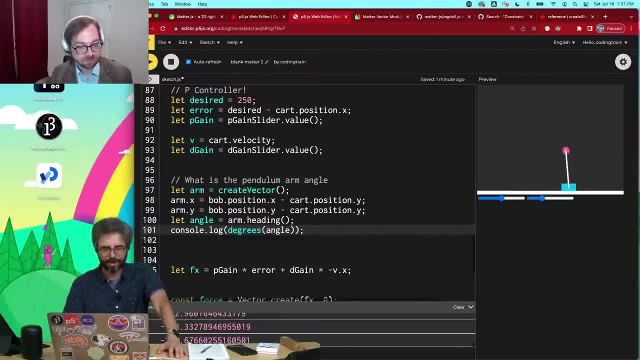 an angle is in, radians is, So we can see it's about. well, it's at negative 180 degrees when it's there, which is correct. So what did it start at? Let's turn the engine off so we can see. 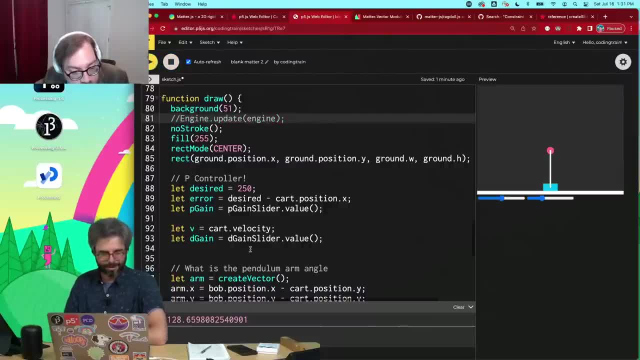 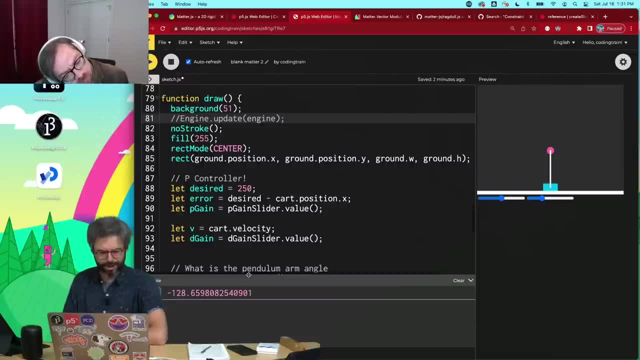 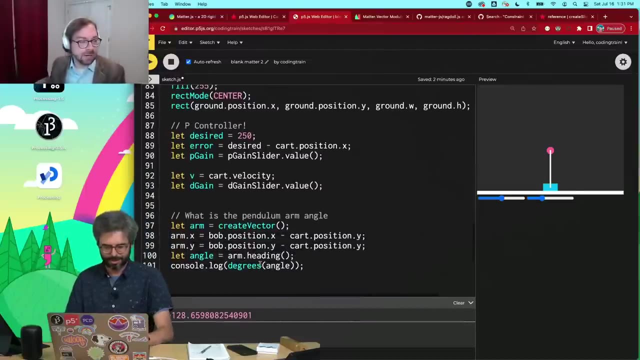 What is it? What is it? It's correct angle. It's correct angle. is pi divided by 2, right In radians In radians, In pi over 2 in radians? do you think it's degrees or not? Because pi over 2 is going to be like 1.7.. 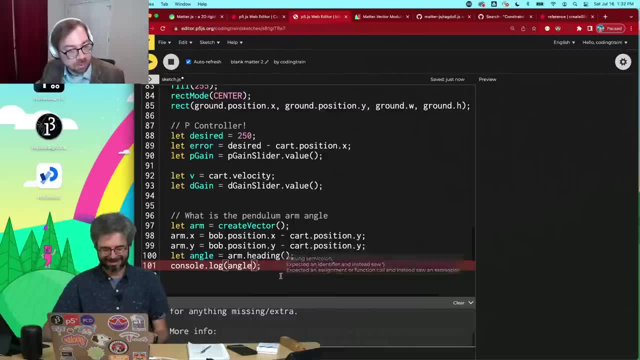 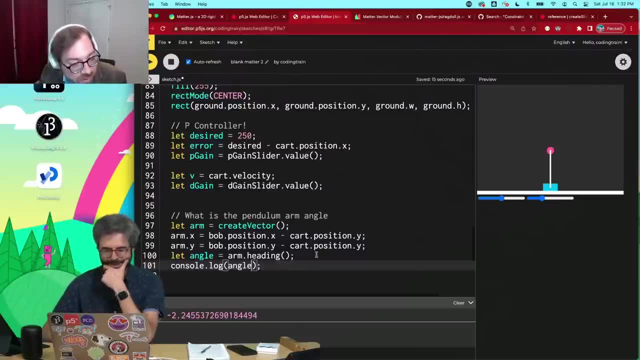 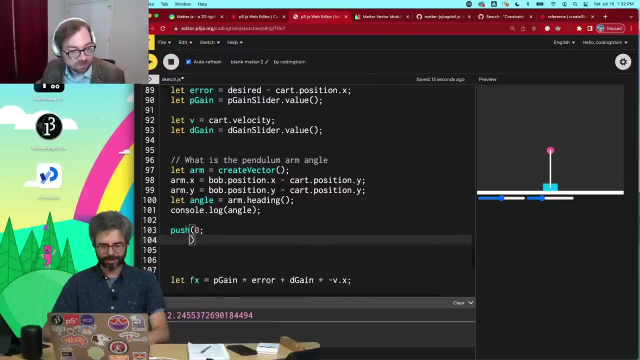 Yeah, I converted it, and then I converted it back in my head. OK, What Do I have something wrong here? OK, Let's see. Hold on. One of the ways we can debug this is: I'm going to do this. 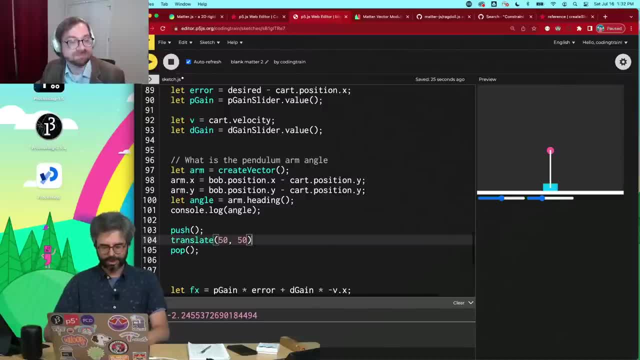 I'm going to very quickly translate to a little spot and draw a line. I'm just drawing this line here and I'm going to rotate by that angle. Weird, That's weird, That's weird, Yeah, weird, Okay. So I definitely have a mistake. Oh, there's a Y there. I make so many typos There. we. 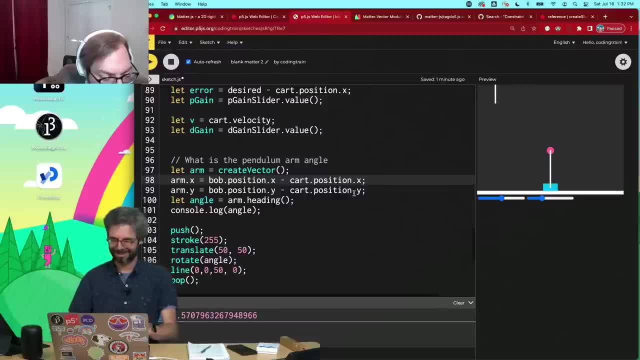 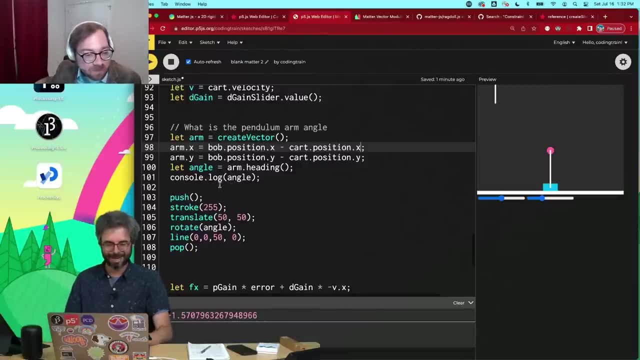 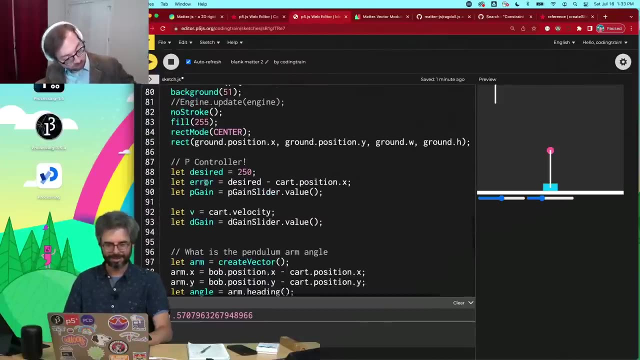 go. I knew like my math is not right. Okay, There we go, We're good, We're good. I'm sure the chat, like the chat's- already got this. Okay, This is actually nice, though, to see this, because if I turn the engine back on where's that, It's kind of fun to see, like that little extra dial. 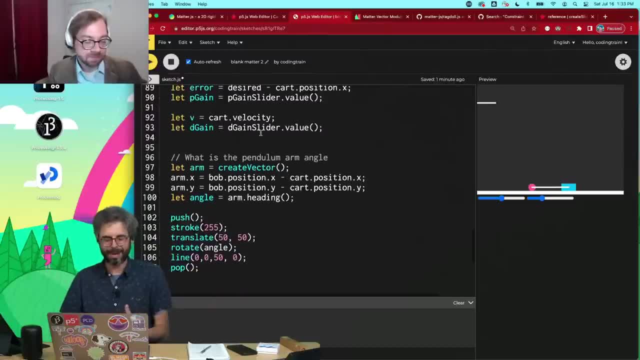 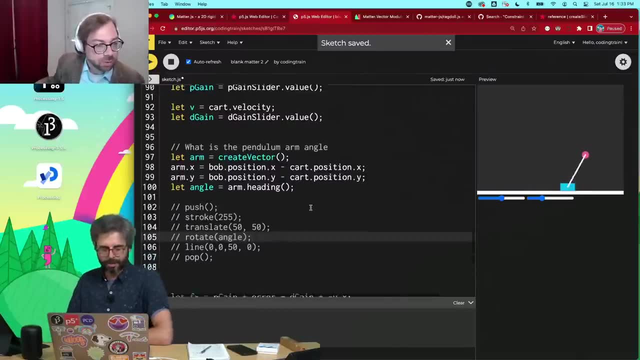 kind of rotate with it, It's like. but I don't know that we really need that debugging because we have the actual pendulum arm, but that's going to be useful. So I'm going to just comment that out, though for right now. Okay, So now-. So one thing I want to alert you to is the fact that 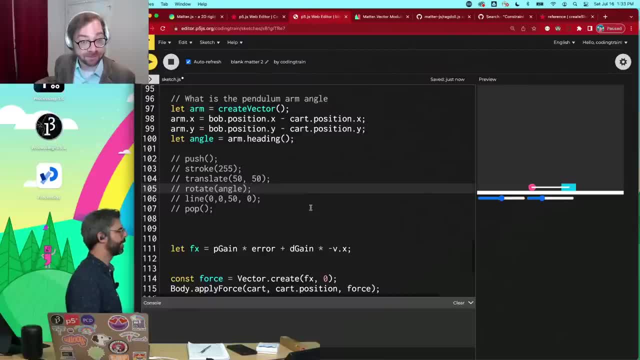 we're going to have to get the derivative of that angle that you're measuring numerically Right. So I know that you have a plan for that, but we can certainly come up with one, if I'm sure you can. I don't have a plan for that, So you can start thinking about that. Yes, I guess I. 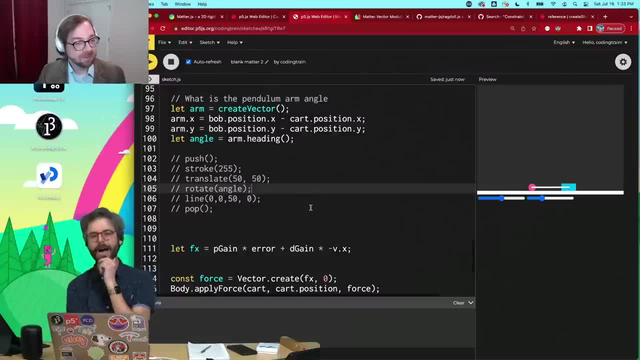 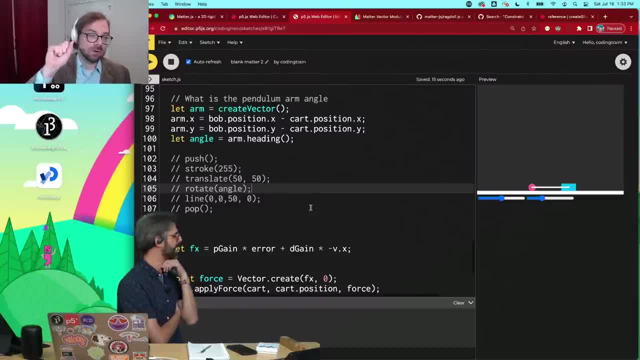 track that angular velocity myself, I guess by looking at the change. Yeah, Yeah, That's what I was wondering. Can you store something or grab something from the previous loop attempt variable that you can derive? Yes, That's what I'll do. 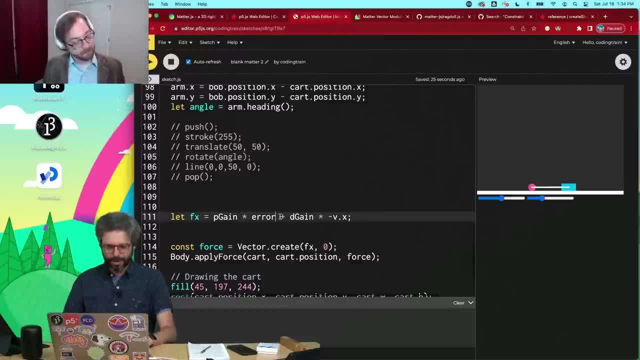 That's what I'll do. So first, let's so. one thing I'm going to do right now is I'm going to just comment out the D gain. So this is now, it's just got a P gain. It's only, this is just a. 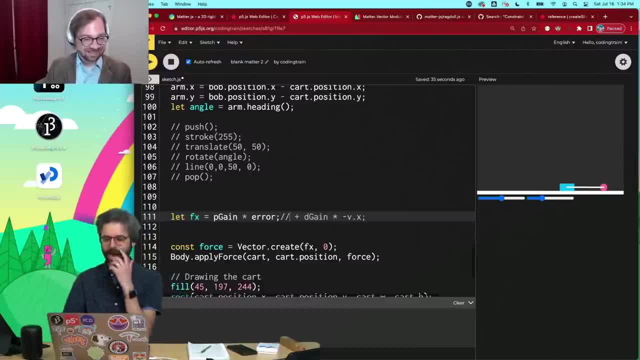 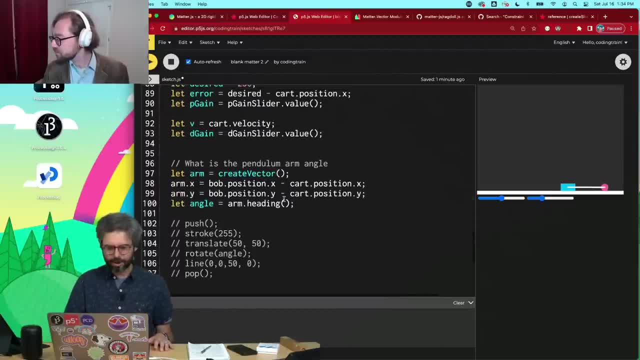 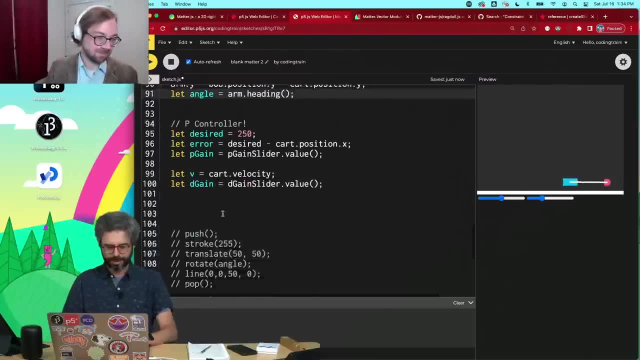 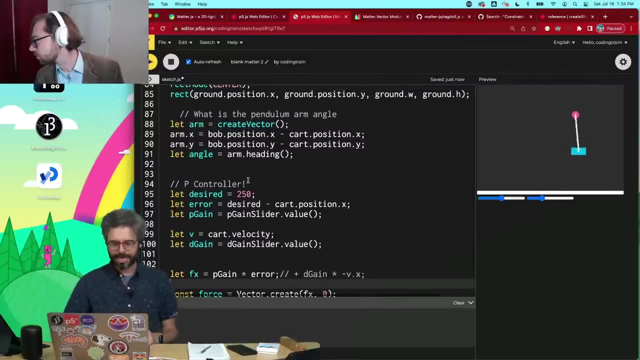 pendulum. Okay So, but the error now should be: where did I calculate that? Okay, So, this isn't. let's. let's move this up to here. Let's take- actually just take- this out so that we can see things more in one place. And now what I want to do is change this error calculation. 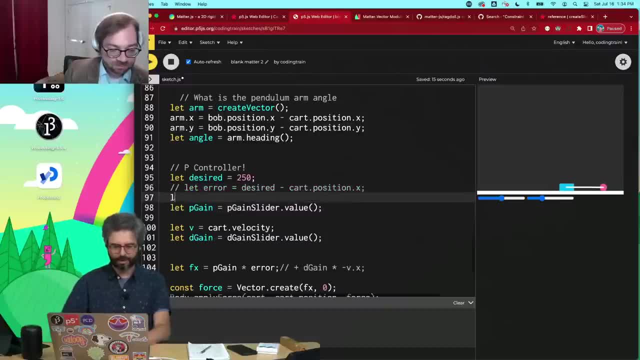 So this is. I'm going to just leave that there for reference. This is now the desired angle, which I said was: what did I say? It was pi divided by two. I mean pi divided by two should be the. uh, assuming zero is horizontal, right? 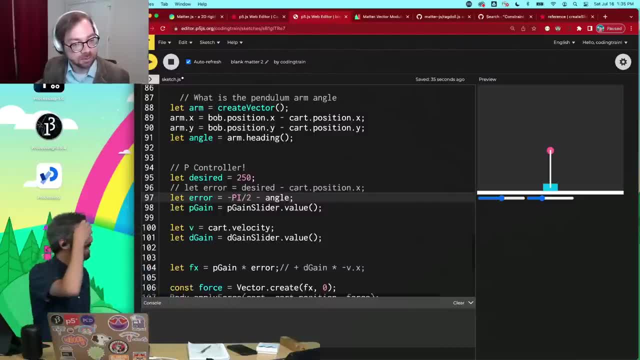 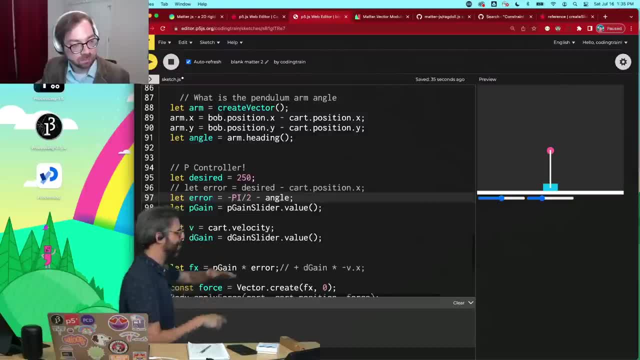 pi divided by two, because the Y axis in my world is flipped, So rotating down along the horizontal axis is nine degrees. So you know, there there could be some reasons for, in a different kind of demonstration of this, to actually make the world, with the Y axis pointing up, to reduce these kinds. 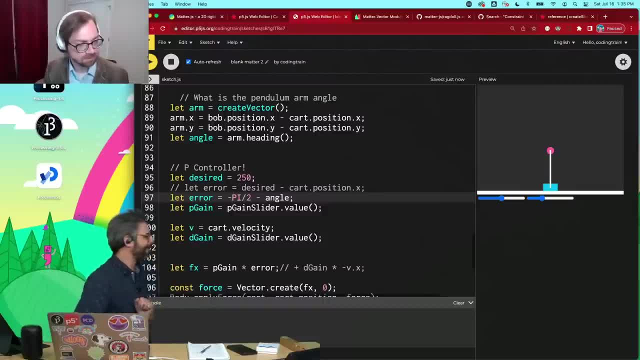 of problems. But, like you know, in in, in my world of like just getting this to work, like, Oh no, I just remember we need a negative here. Okay, This is cool, All right, So it's perfectly. 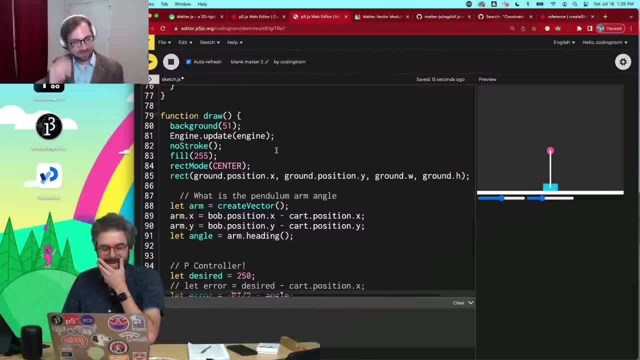 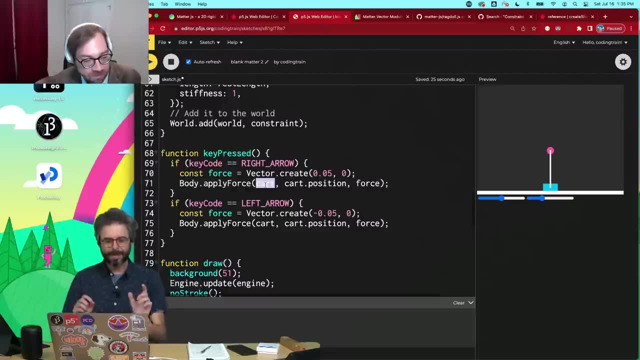 balanced because there's no offset. So just to see if what the P controller does remember these forces I had here, let's- actually I'm going to be able to, with a key pressed, apply a little bit of wind, almost as if a gust of wind. 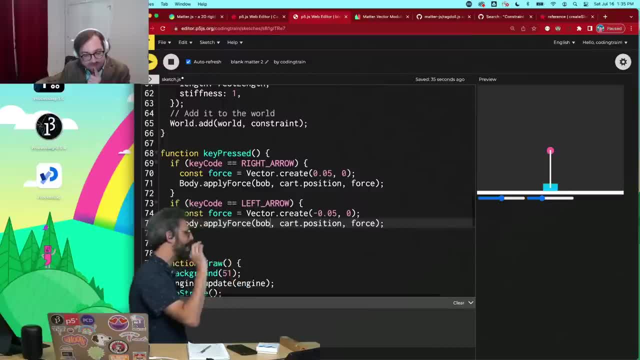 comes or somebody flicks the Bob. It's not a wind, because the wind would push the cart conceivably as well. So presumably now, when I press the key press to the right, a little force is going to act on the Bob, pushing it to the right, And that should cause every P controller to start to move. 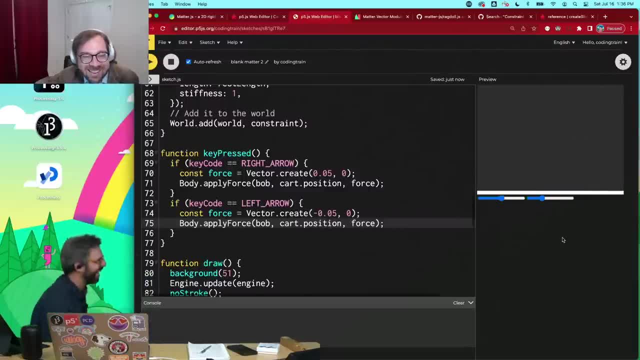 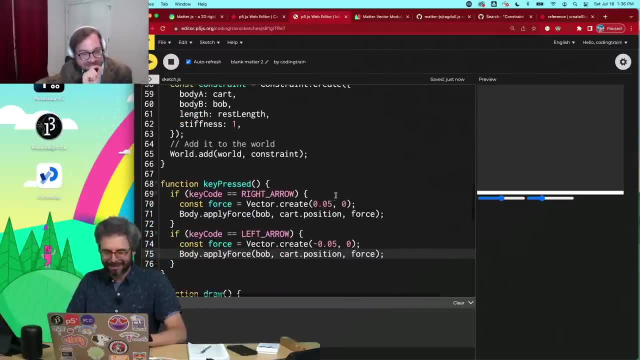 the cart. All right, Maybe we should. a little less wind, a little. a little less. a little less wind and maybe a little less restitution, a little more conversation. What's the song that I'm somehow referencing now? I wish I do? There we go. Okay, Now it went in the wrong. 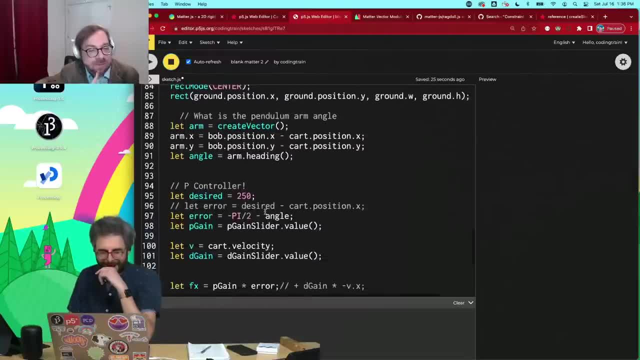 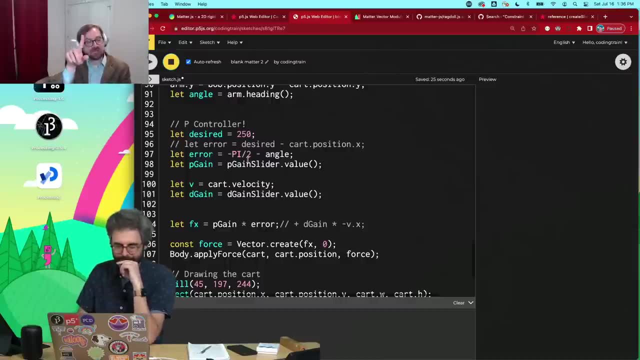 It compensated, but in the wrong direction. So I must have something flipped. Well, it's possible, Like I the. I mean, I know you had to have to change the direction of PI over two as your desired angle, but theoretically it should be okay. It shouldn't require. 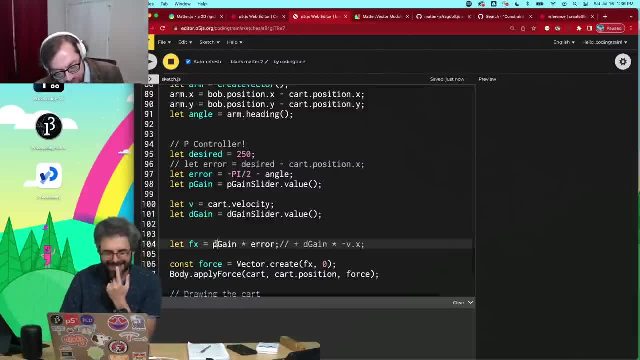 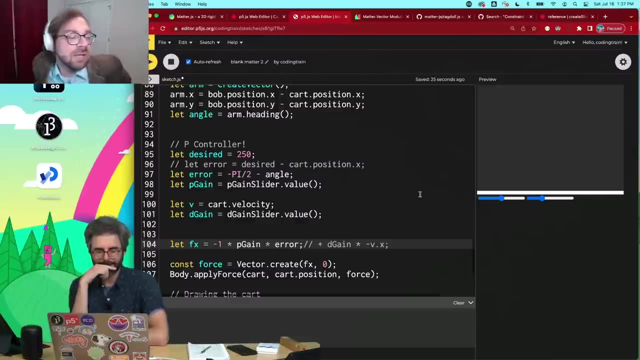 maybe it's the fact that it drives it in a different direction. You could try flipping the gain, even though it technically should be positive. but we can give that a shot. There we go. So why is my direction wrong? Interesting, I mean. 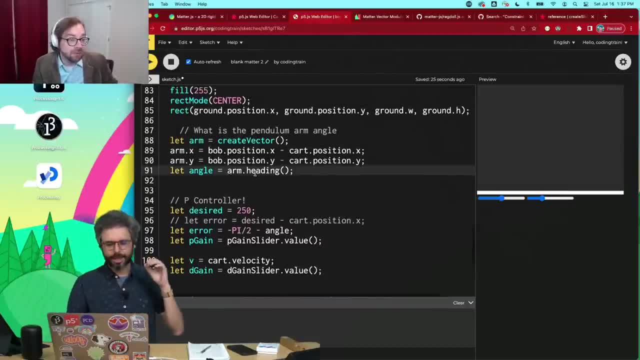 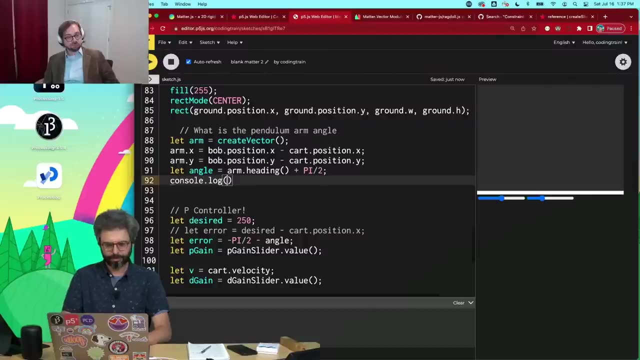 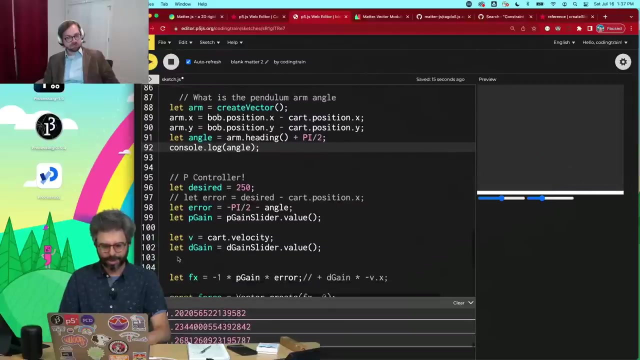 it has to follow how you were defining your angle. So, let's, let's, consider zero being the Y axis, in which case, oops, Oh wait, Okay, Hold on. Hold on, Let's not. uh, let's turn the engine off for a second. 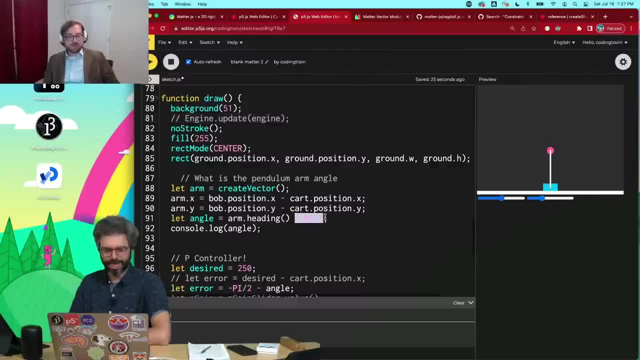 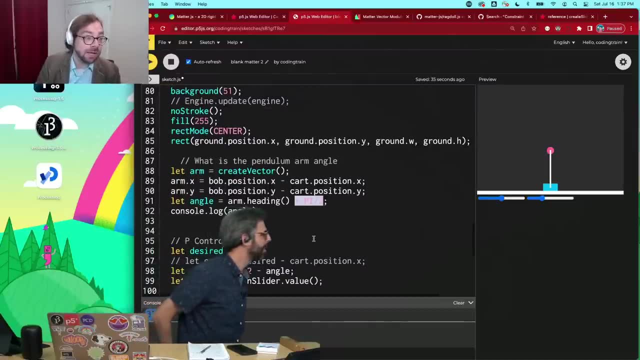 So right, So this angle is now zero because I'm offsetting it by PI divided by two. And one thing I also point out is people are saying that we didn't, that the D term might still be on and still working based upon the cart position. So mismatch, that's something that could. 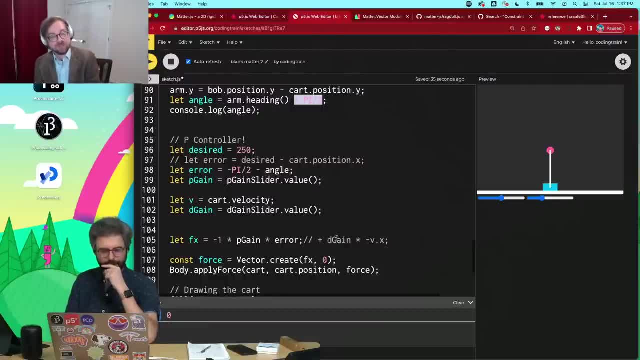 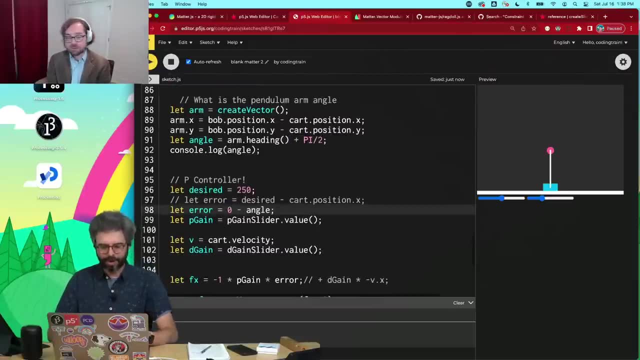 be mismatched. It is- I commented that out- Pretty sure. No, Um so, and then this would be: the desired angle is zero minus the current angle. But if the current angle is, I go, let's see. So now let's do it. Did I turn the engine back on? No, we don't have to get stuck on this. We can sort of 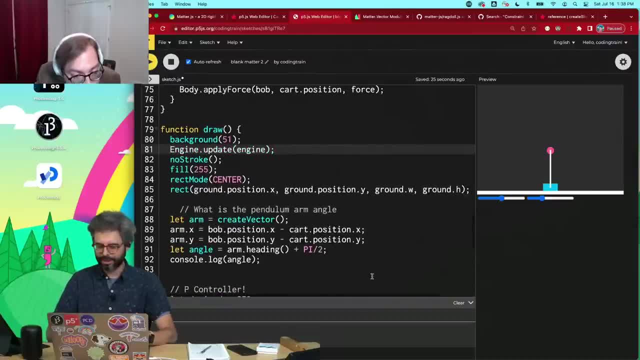 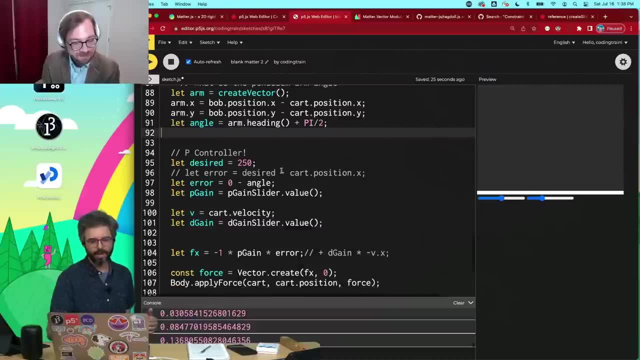 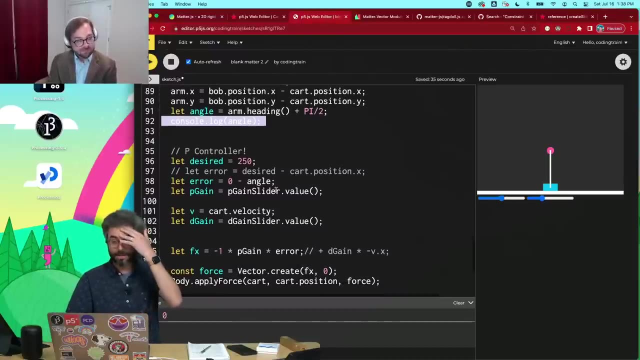 think it through more later I'm sure it will. Yeah, Oh, there we go. So there's something. this is one size now. Oh no, I still have the negative. I didn't realize that. the negative All right, So I'm not going to worry. about this right now. Um, let's, we'll. we'll put our heads together. I'm sure it will appear to somebody. All right, Let's just cut this precisely And then we're going to look for when we were matching it to the address value, when we were matching. 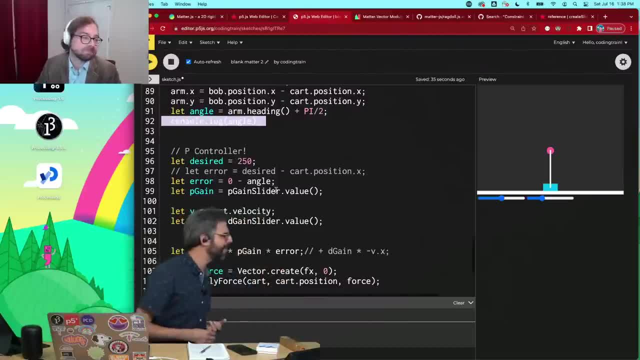 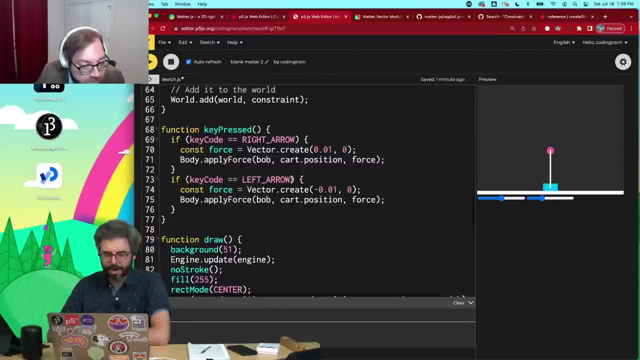 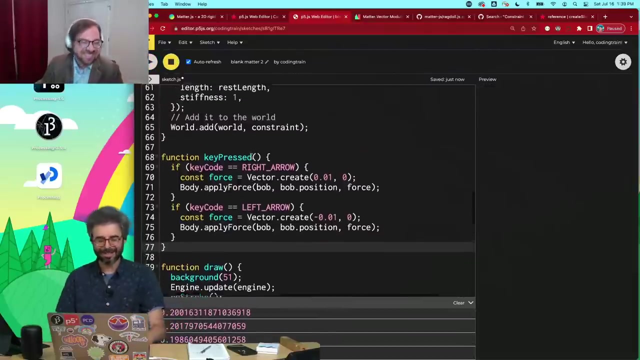 somebody who — So it happened at this address. Okay, somebody line 71, 75, 71, oh, cart position, that's not a big deal, but that is a problem. so if I look at this, you know one thing I can do here that I've done. 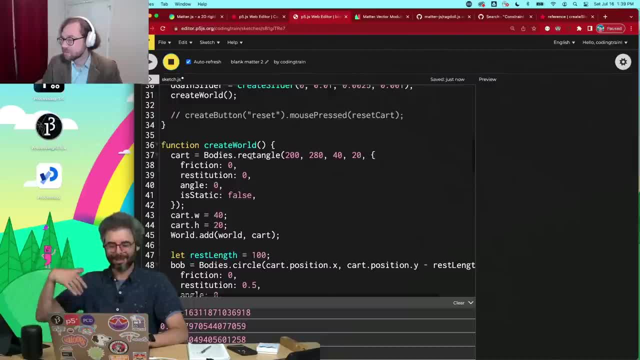 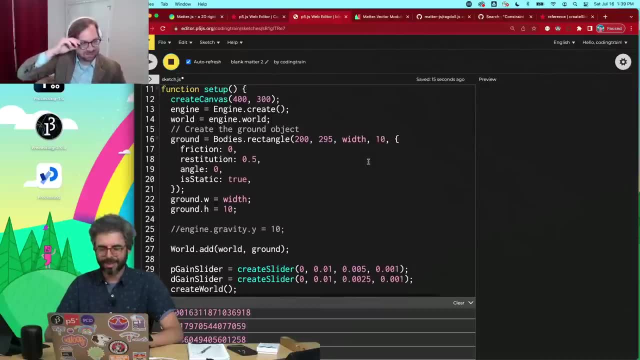 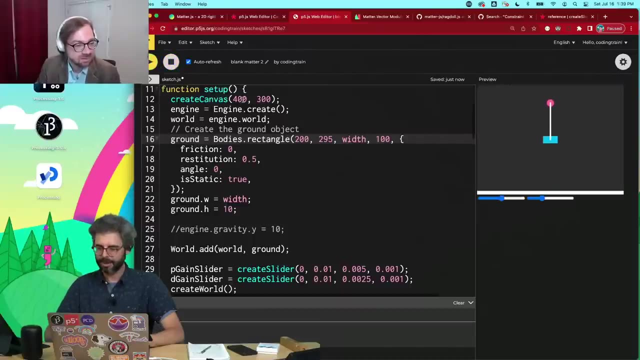 before is: I've you can, we can make the ground much, much higher. so basically the ground, so that it can't skip past it as easily. thicker, thicker, yes, so the ground could be like a hundred pixels thick, and then obviously, now it's, and the H is a. 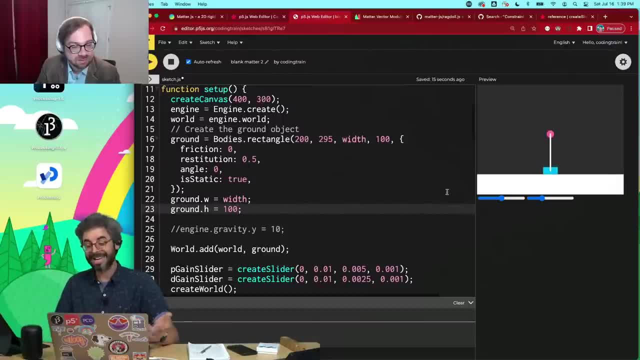 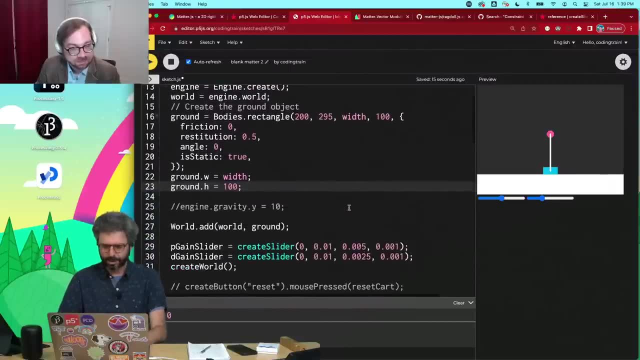 hundred. so it's obviously, it's there. but oh, actually, you know, that's kind of fine. I was gonna say like, oh, I want to have to shift it down, but let's just, that's actually much sort of nicer to see it there anyway. so let's, now I just need to adjust. it would be nice to adjust where. 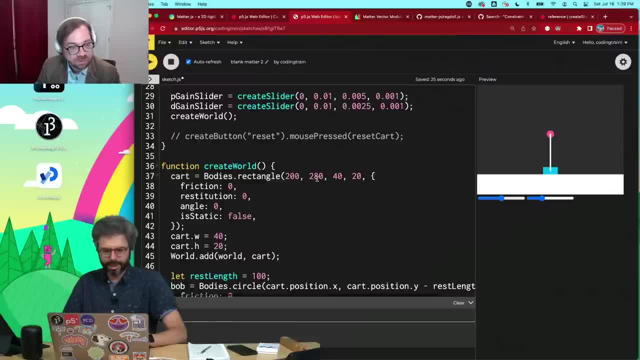 the cart starts which is like around- I sort of forgotten. I'm just like there we go, perfect, okay, I don't remember what it was. so okay, so great. so now, and let's make this cool. so now I can just like we now, yeah, go on. I'm sorry, but I was gonna. I was gonna mention that like we. 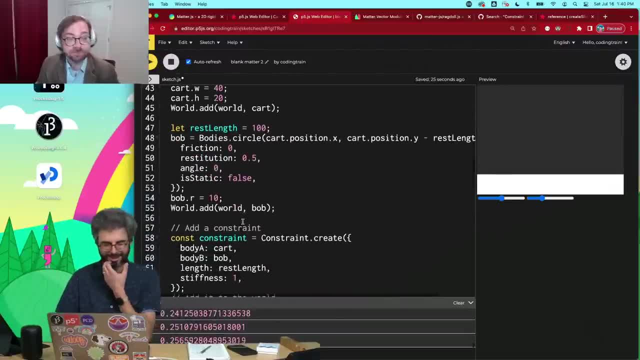 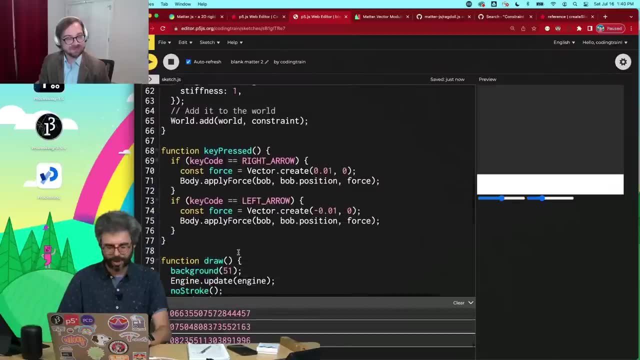 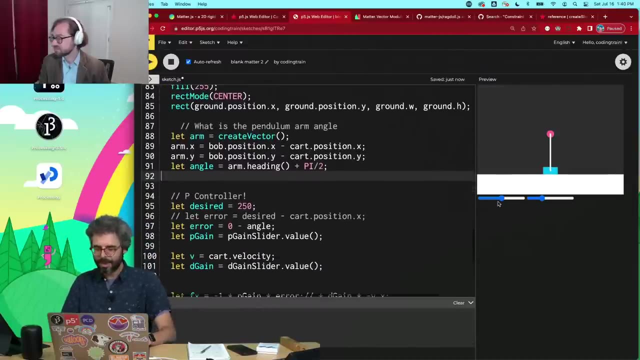 can up the game now and say: yes faster, yes, yes, yes. so where is? I just want to see where this console log is that is filling up the console there. it is okay. so let's now put the gain higher and hit a little force to the right. yeah, you. 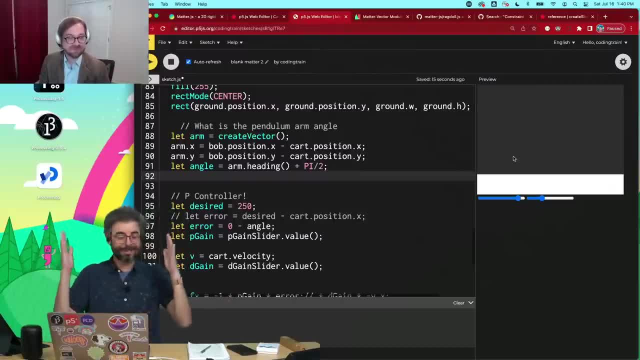 could see. I mean it's it's you know. one thing I could also do. I was doing this in what I was doing. test is I could add little walls on the on the sides so that it's like forced to stay on the screen. it'll bounce back and have to readjust. maybe we'll do that just for because I 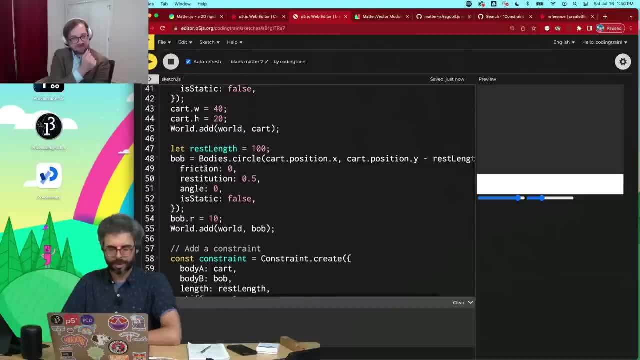 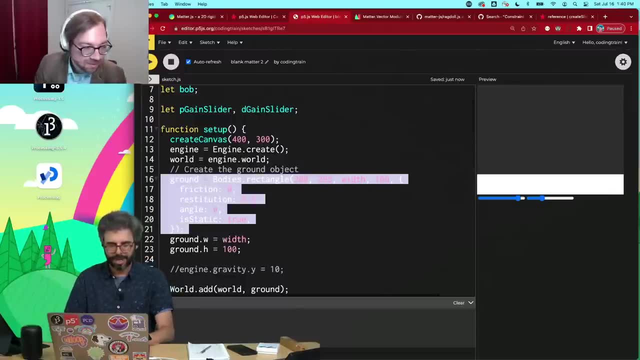 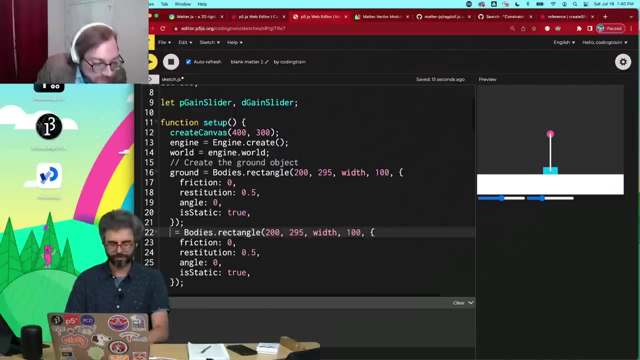 think it'll make the simulation kind of interesting. I don't want to get too stuck in this, but let's do, and I don't even have to draw those necessarily. we can just say like, hey, let's make a left, left, left wall which is a rectangle at the width, at the. I'm going to just 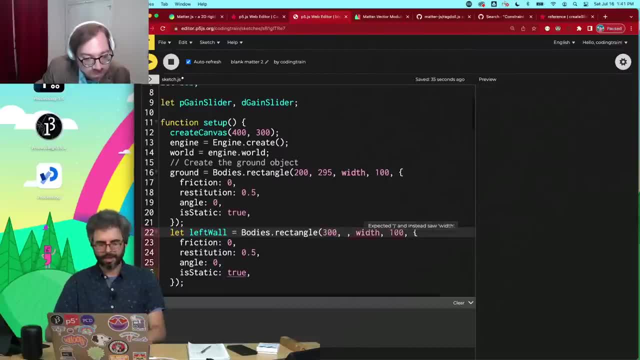 hard coat this in, because it's a little bit more concise right now. at 200 pixels down, it's just like 10 pixels wide. it's the full height. so now, okay, and let's make it a hundred pixels wide, just like this. oh, I didn't add it, no, it's just I. 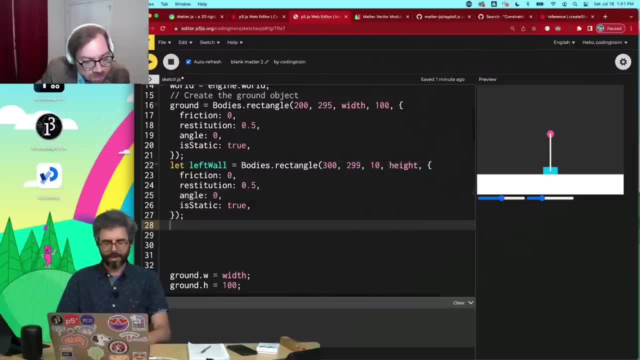 didn't add it to the world dot. add world left wall and that's the right wall. by the way, this is I. I was uh saying this to Christian earlier this week. I try never to stream for more than two and a half hours because that seems to be the threshold where my brain 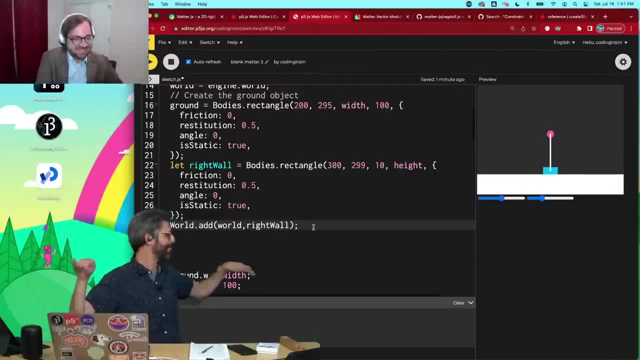 completely starts to shut down. it's like my classes at NYU are two and a half hours long, with a good 15 minute break in the middle, which we did not take, which is uh. I guess I had a little bit of break because we were, we were, we were. 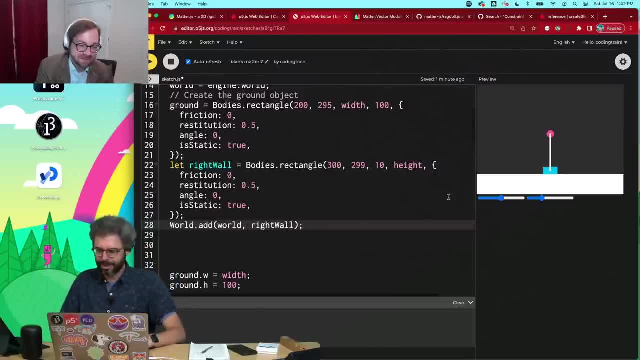 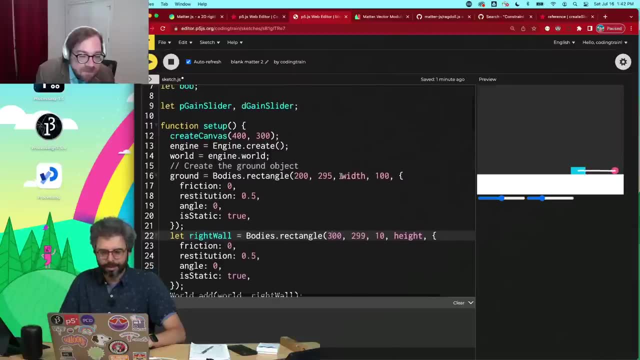 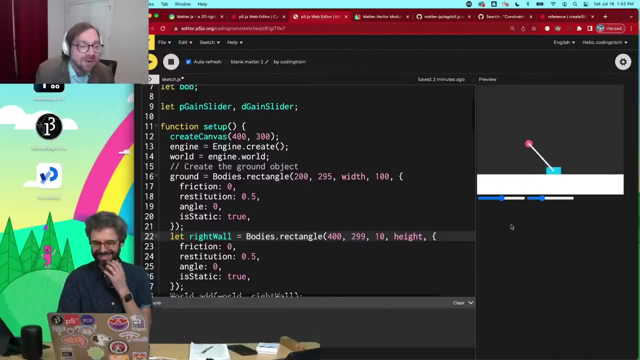 just back and forth, but uh, um, okay. so let's see here. oh, that's the giant, the wall. oh, the wall should be at a 400. sorry, this is the problem with not drawing it. I don't know where it is there. we go, there, you go. so okay, and let's just add a left one. 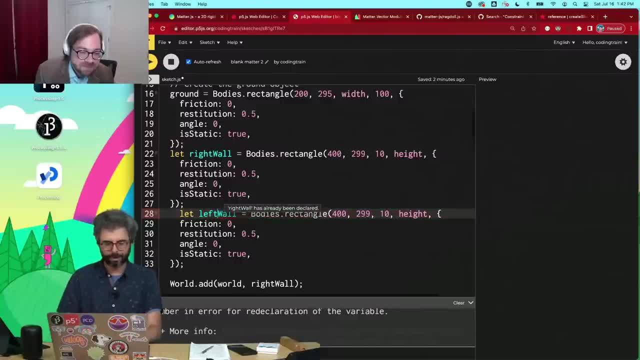 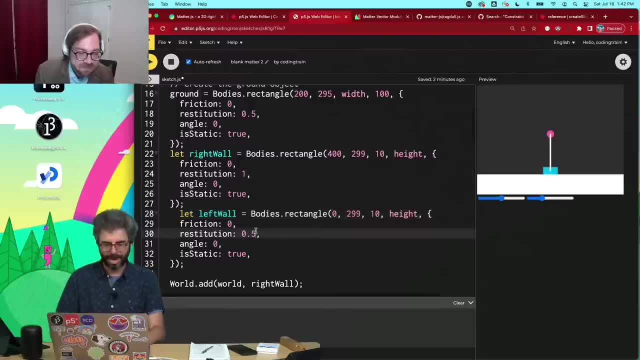 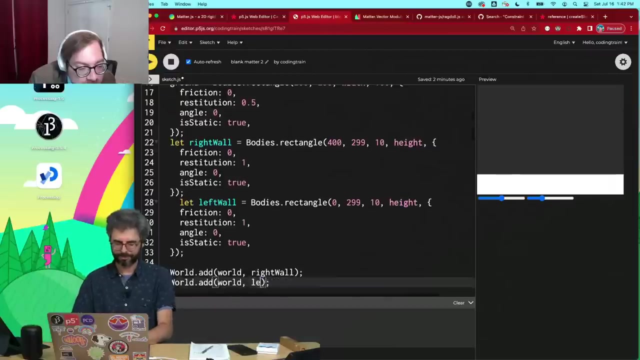 maybe this is a a different kind of problem I'm introducing, but at least we'll have this option. okay, so now, and if we can make them very bouncy so as to force the the things to bounce off them more, okay. oh, let's see left wall zero tonight and got to add the left wall to the world. okay. 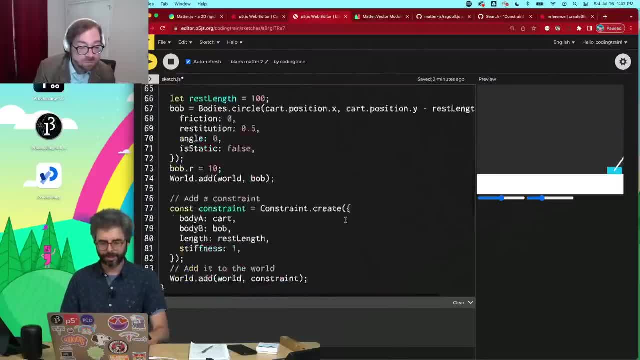 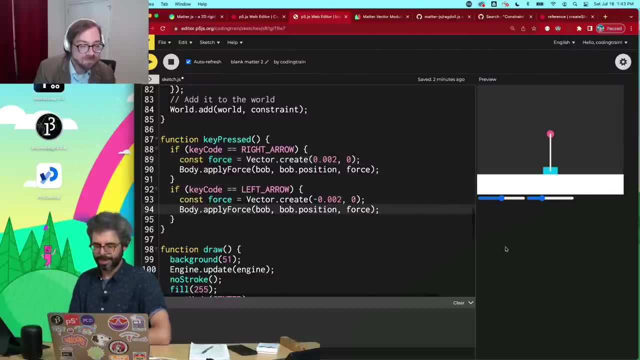 and I think I also might like to. I think it'll help us sort of see what's going on by having this force be even less let's- I'm gonna just many magnitudes less right, because we can see now it, there we go, we can see it more, trying to balance it and I don't know why it decided to like this, this, you. 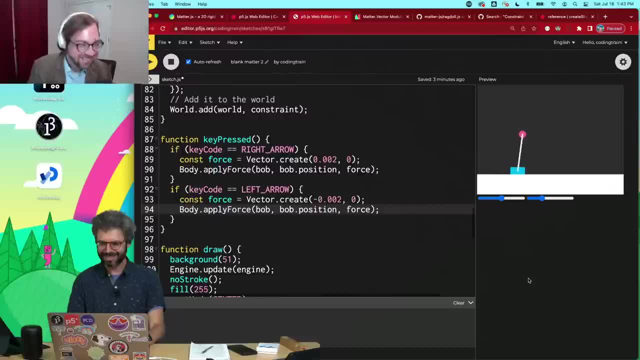 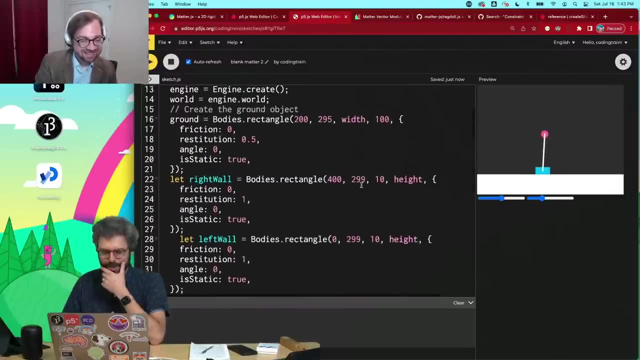 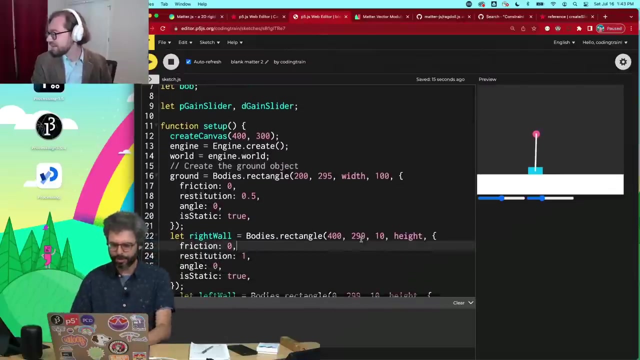 know this killed your walls. I don't know what happened, yeah, but I love that. I love the way you're. you're uh winding it back and forth. I think you can suck up the end. I might be. I wonder if the walls are actually in the wrong place, because 290, oh, what am I doing? yeah, the wall should be. I. 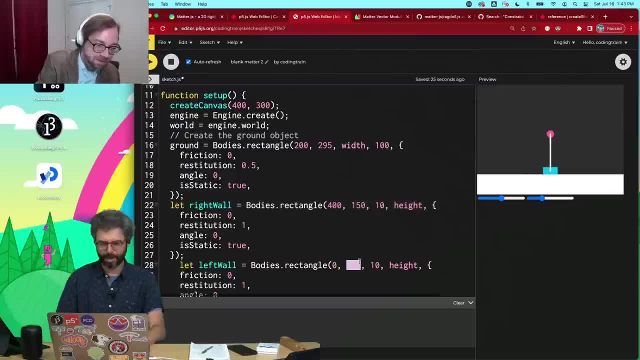 don't know what I was doing. this should be 150, the Y position. this is the problem of not drawing it. the wall is actually not was like I had it all the way at the bottom. I don't know what, why I did that, but this will and we can up the game. but yeah, uh, okay, great, yeah, so we're, we've got a nice. 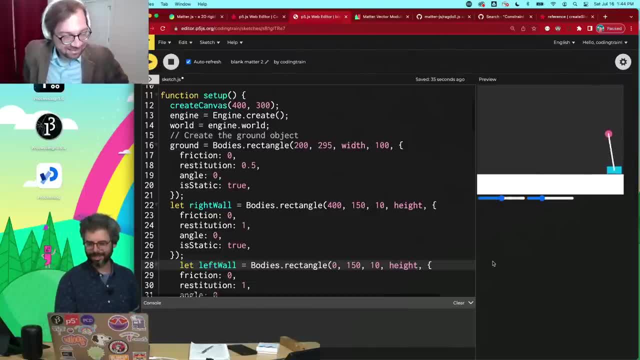 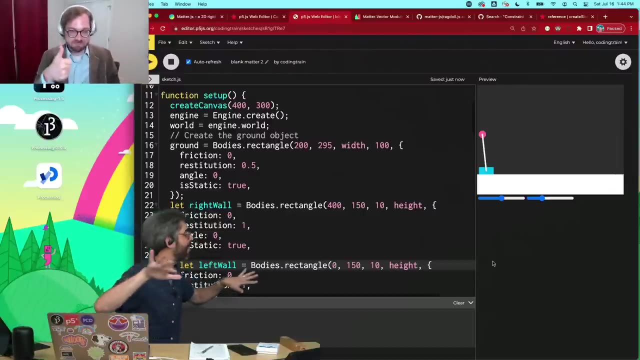 P controller. I can like push it and it'll sort of try to like get it balanced. look at that, that is awesome. yeah, okay, this is, we should really stop here. quit while you're ahead, okay, um, so I'm gonna, by the way, I'm gonna, put a hard stop on us at two o'clock, so that gives us 15 more minutes to maybe. 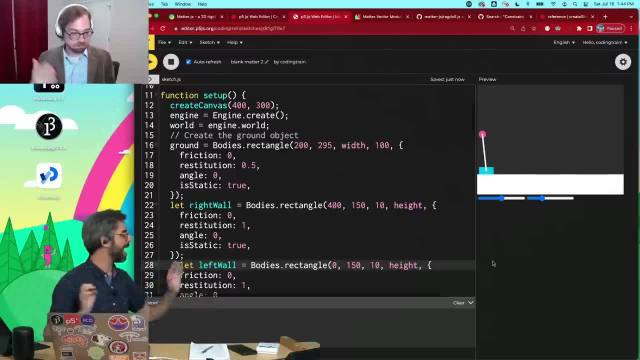 see about adding the D controller and maybe one or two short questions. we can always come back and do this again or be available on social media or Discord or in the YouTube comments if people I mean: uh, Christian, you're, you're welcome to. we'll go back to your life, but I will. I will pass along any questions that I can't. 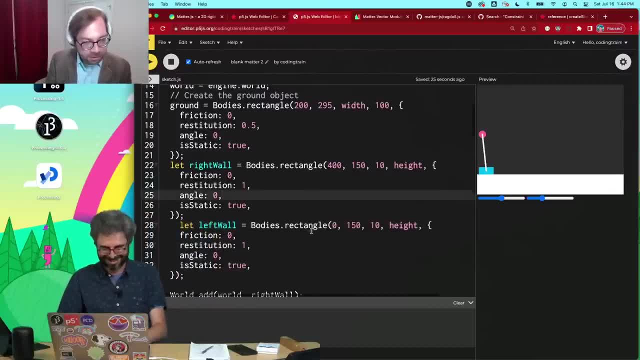 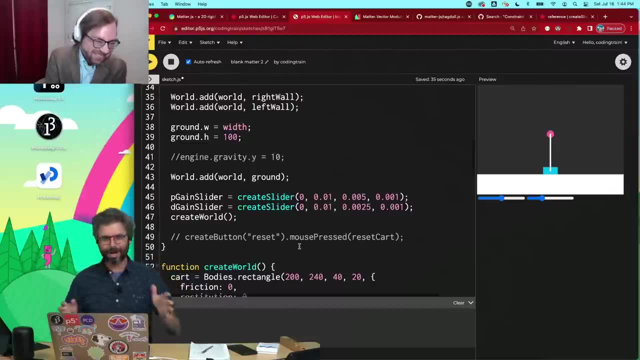 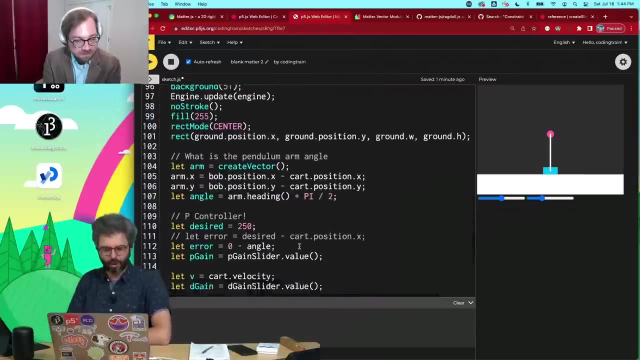 answer to Christian and and you know what, you're working so hard, I'll stick around to 2 pm, I you know, to moral support for your challenge here. okay, okay, okay, we're gonna, we're gonna wrap this up. we're not going any more than 15 minutes, um, so let's start adding the D control here. 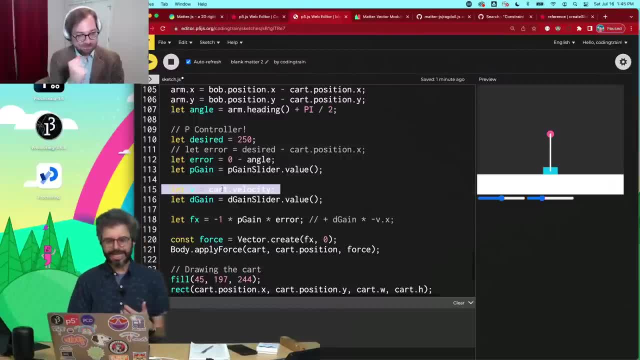 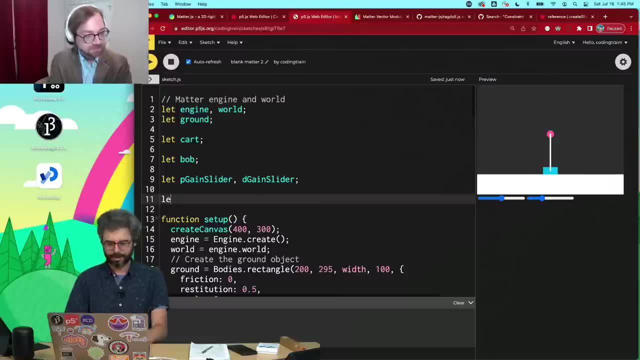 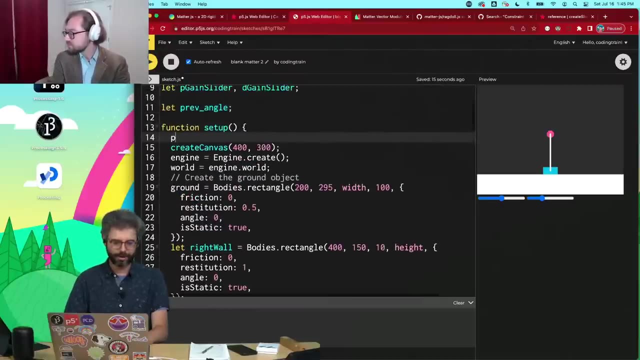 so we need is the angular velocity, and the easiest way to do that would be to just store the current angle and the previous angle. yes, correct, so let me create a variable for previous angle. we're going to have the previous angle start. I don't need to put it in setup and I'm mixing different code. 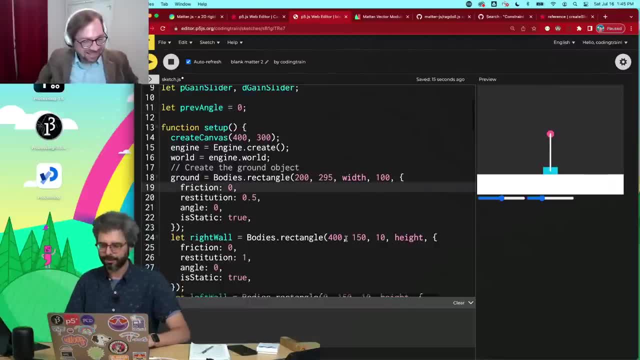 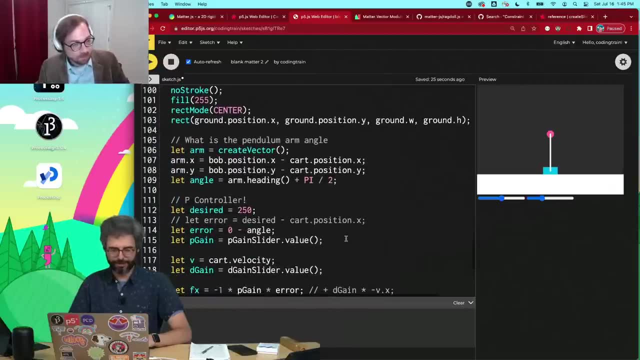 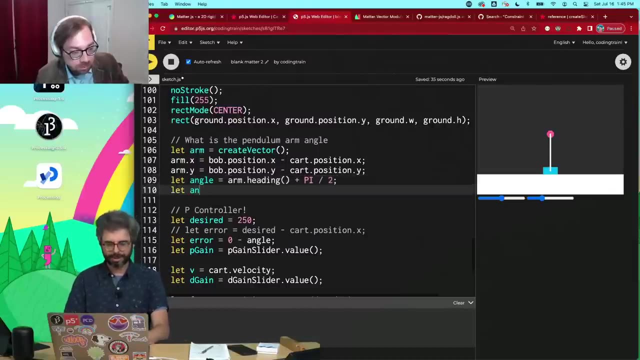 styles here I will go back to what I usually use with the camel case for JavaScript. previous angle is zero. so this is me. where am I calculating? this is actually going to be pretty fast as soon as I calculate the new angle. the uh angle velocity is the current angle minus the previous angle. 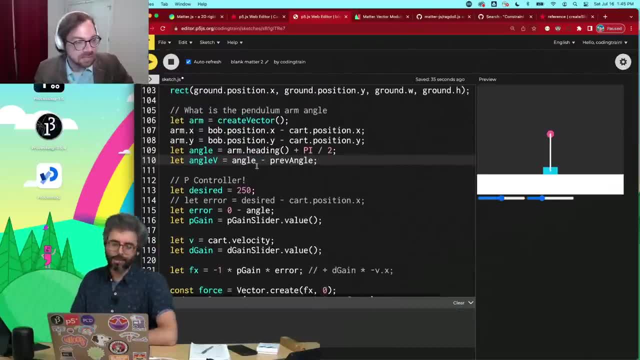 right. so in my case, Delta T is uh one, but we we might need to match it because I'm just using the frame rate. basically, every frame is one of them. there might be an issue with that in terms of how we scale things, in which case we can and how matterjs is working. but let's start. 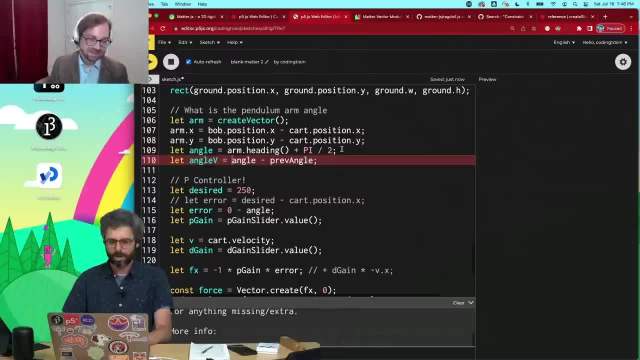 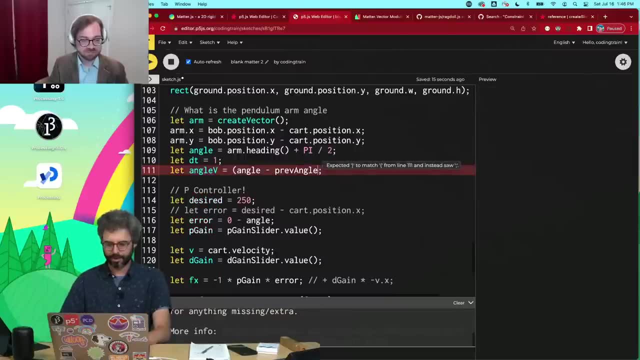 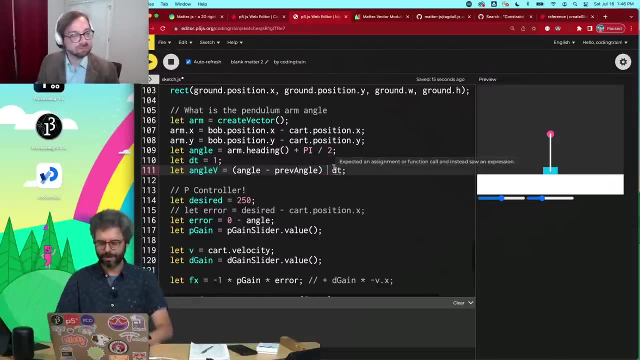 with that. but yes, we should. I guess, to be more to be correct, I should have a variable for DT and take this and multiply it by DT. is that correct? divided by DT, divided by DT. yes, sorry, that's what I meant. um, okay, um, so we're going to leave it like that, that way, that that is a. 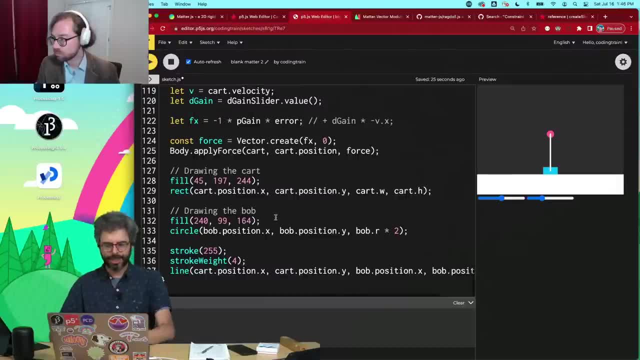 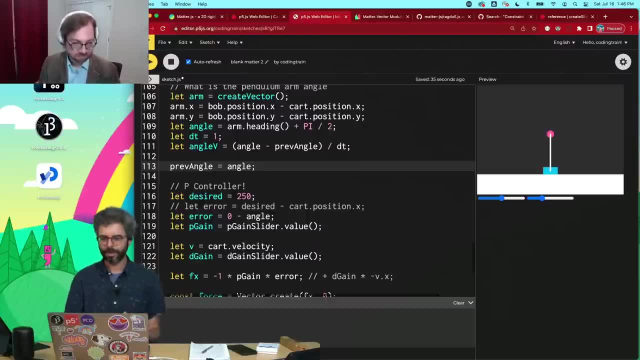 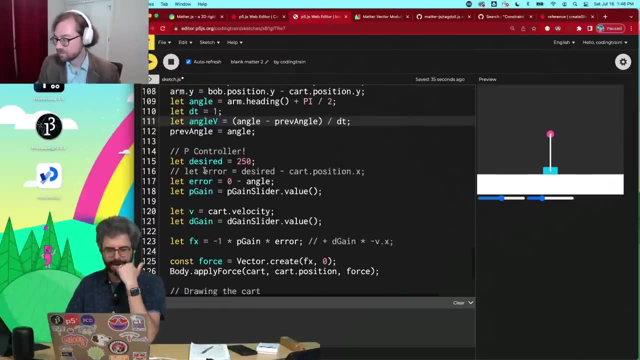 parameter we could adjust if need be. I just need to as soon as I do, that previous angle is the current angle, so that I pick that up for the next time. so this should give us the angular velocity, and then I guess I don't really, just to be consistent. 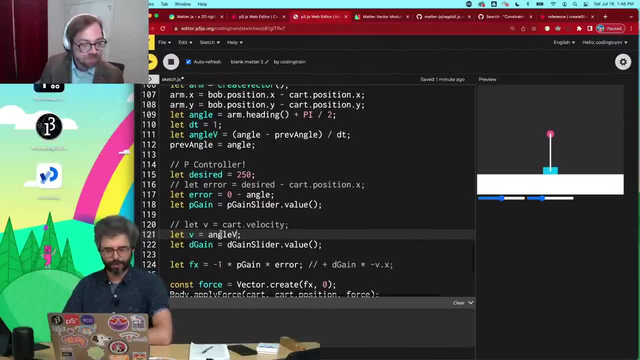 I'm I'm having many extra unnecessary variables here, but I'll just put this as the angular velocity. Oh, and there's no, it's a scalar value, so there's no X component I'm dealing with And so I have no idea. 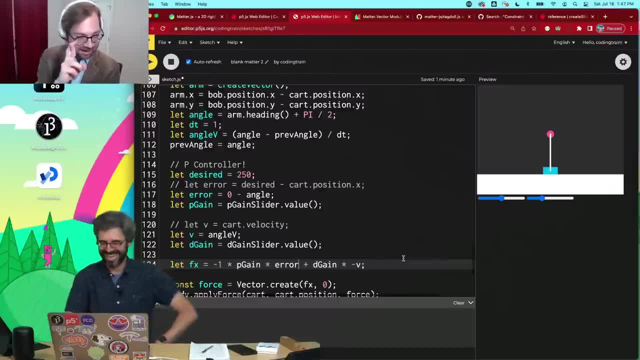 I think I put everything in the code. Okay, Fingers crossed here. Oh yeah, I mean, it's hard to tell how much of a factor that's having, but let me ramp that up. Wow. So we might want to. it's possible we might want to. you know, keep in mind we have to change the direction of the other gain. 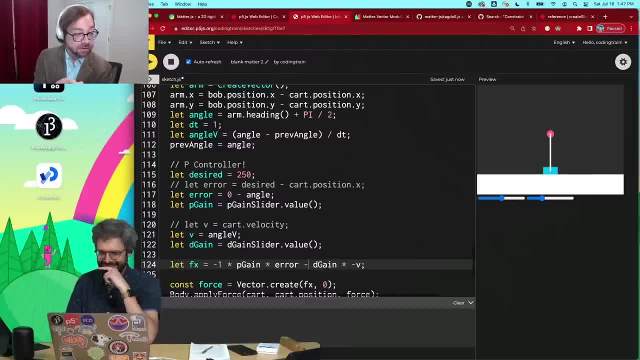 Right. So we might want to change the direction of this other one, which is not a theoretical problem. It would be like what, if you're forced, you define as operating in the opposite direction, for instance. So that's not a crazy thing. 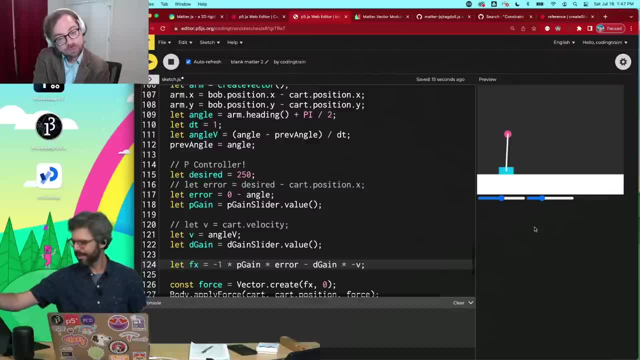 So let's look at that. It's coming to a stop here And it sways slowly to a stop. How about that? Wow, Now it's gone. Oh, you're doing that. No, I'm sorry, I'm pressing keys. 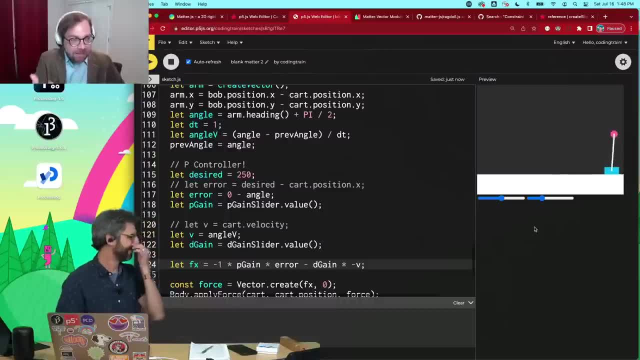 Yeah, Okay, What happened? The math said it shouldn't do that. That's why we better have like a buttons or some interface or like the four I could use. like something that we use a lot on the channel is something called Perlin noise, which is this sort of smooth noise which would be nice for like just this kind of like arbitrary wind. 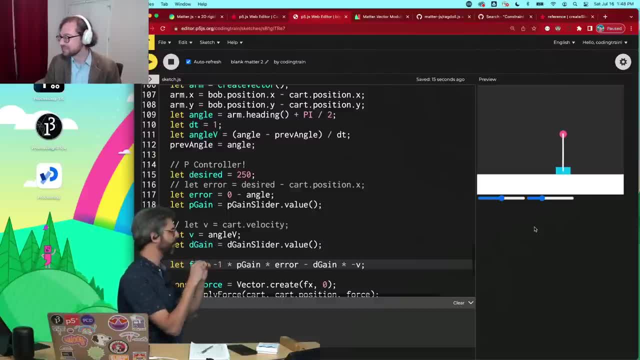 That's kind of like rant sort of chaos. There's a little chaotic wind into the system. That's not just Totally random but sort of smoothly changes over time and have it always balance. According to that, KD can always absorb DT term. 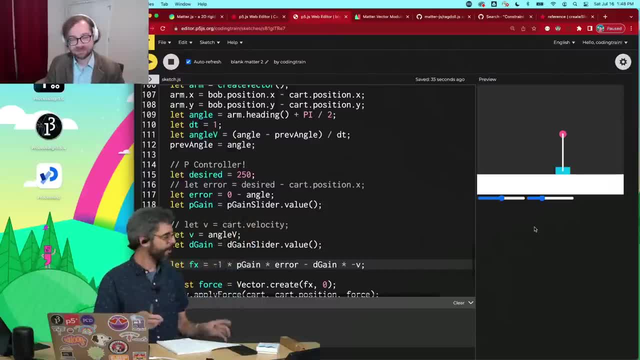 Okay, So I'm going to make a list of things that I look at: this, this, this we're going to, we're going, we're wrapping this up. I was going to say 10 minutes early, but not really. 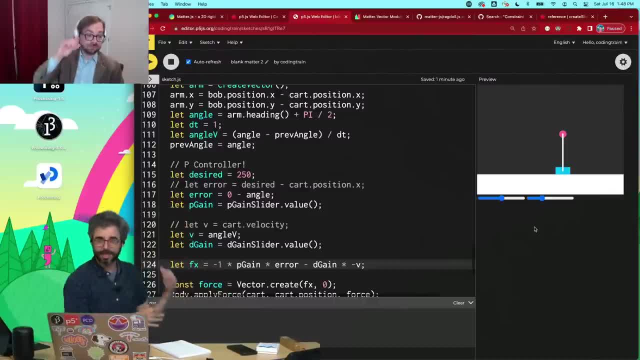 I just want to make a short list of things that I want to address, So I remember them And then what you know. it's not going to happen immediately because I got to go back to the Christian. I'm sure you do as well. 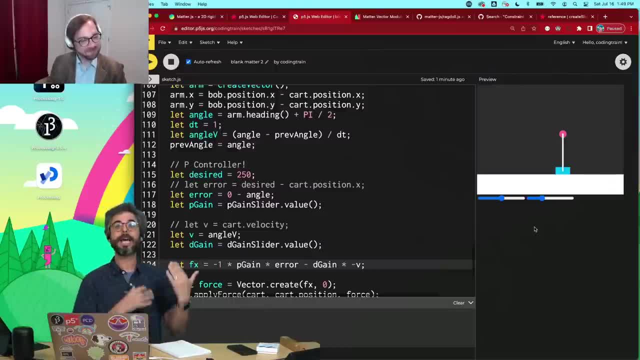 Go back to regular life for a little bit of today, but sometime later this weekend, or certainly on Monday, I'm going to add the code to get hub. Let's investigate the direction of the of the gain constants. Like I have some error there, maybe related to the axis being flipped or something that I just cannot. I cannot find right now in my head. 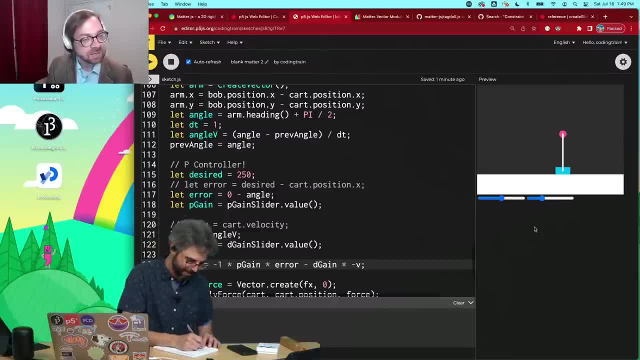 So we'll investigate. I'm almost certain. I'm almost certain That's what it is. I mean, yeah, that's what I know. I talked. I know I talked about how the gains should be positive, but that's, it could be dependent upon which you direction, you put your at your force. 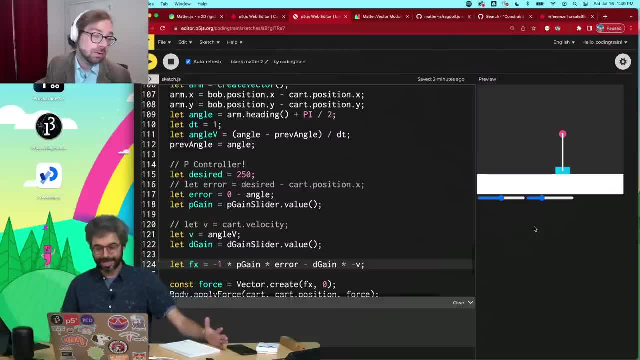 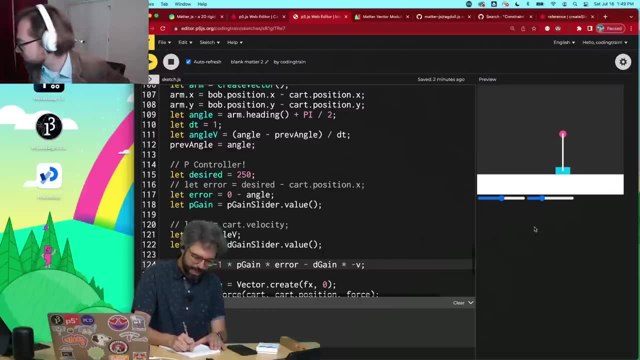 And then I don't know, Does anybody else quickly in the chat- There's actually not, I mean- and then I'm just going to do some like clean up and commenting of the code, Okay, But like we're not going to keep going with this. but I would just out of curiosity, if this were a- let's say this were a demonstration for a lecture you're doing. 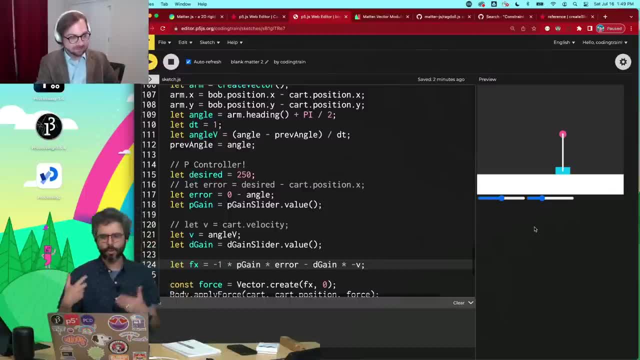 Okay, Like what would you be giving in one of your robotics classes? Like what would be? I mean, I guess the adding, the I could be something. next, but what would be? what would be sort of like the follow-up to this? 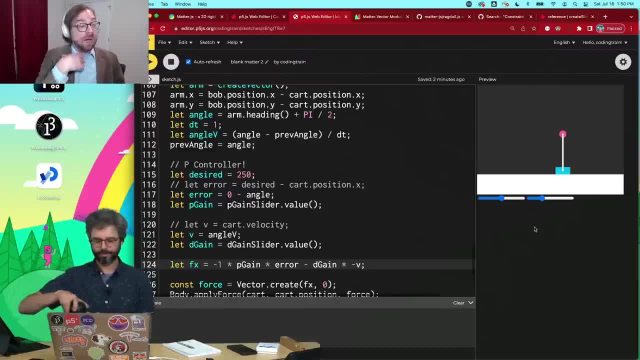 Well, I think what you would do, So in a robotics lecture, like we would learn what the margins of stability are Like. there's like we have these methods of knowing not just what makes the controller perform better or worse, but there are thresholds for what's stable and not stable. 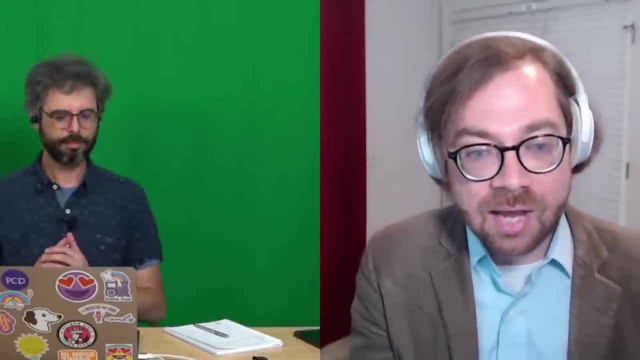 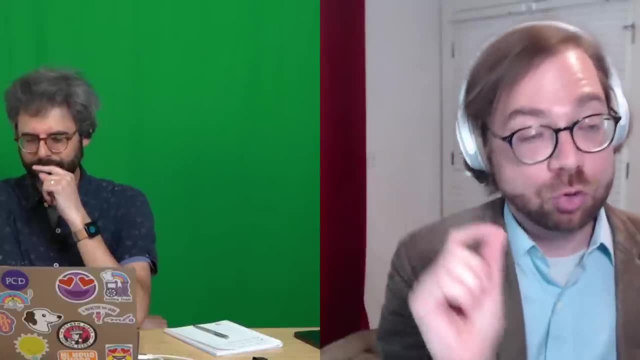 And you can technically test those out. Now, that's not a super necessary thing for for what we're doing here. We're kind of tuning it up. The I term would be interesting to show. The tricky part would be getting it to not only balance but also hover back to the right position. 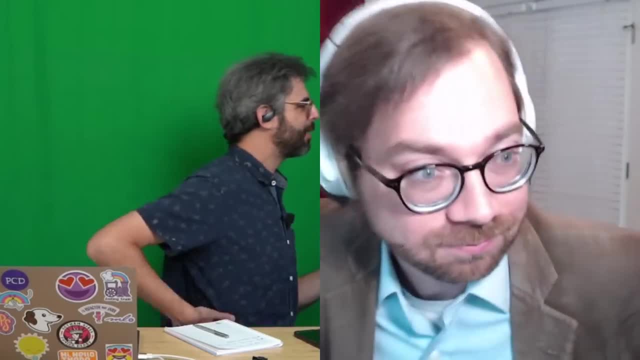 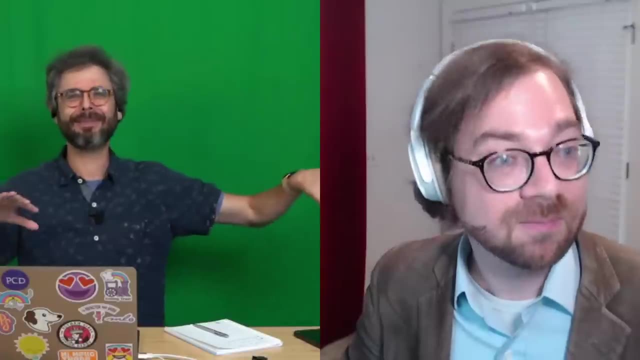 Right, Ah yeah, And someone in the chat. someone in the chat just said that would like to see the desired position of the Bob, not angle. So people are arguing like adding various comments to the chat. but that's interesting. 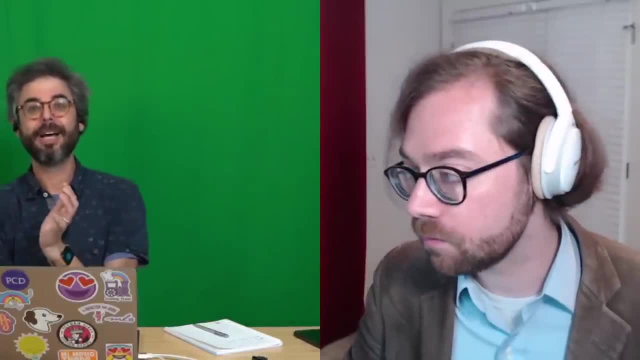 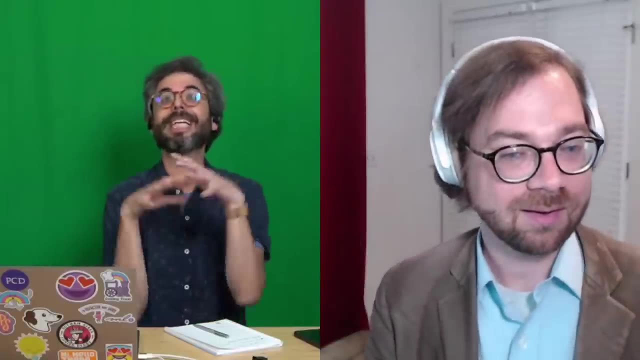 So not only does the robot need to balance the pendulum, but- or the pole, if you will, But it also needs to balance it in the sort of center of the space that it inhabits. Exactly, Exactly, And there are ways to do that. 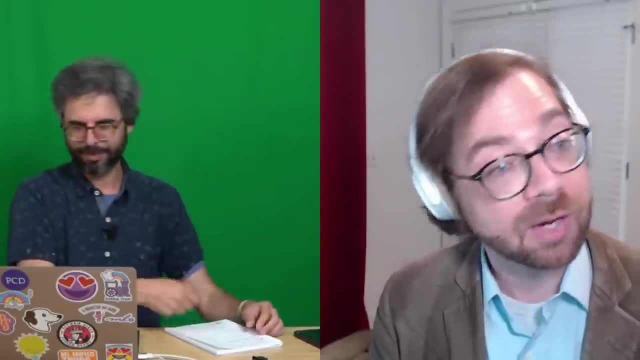 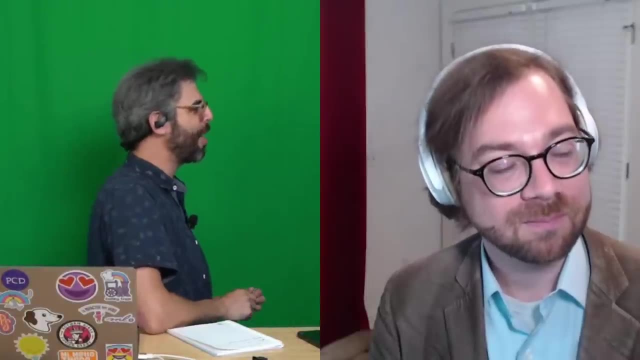 It's a little trickier, but you can still do it with the PID control framework. Great, So one more. I'm going to take one or two more questions from the chat before we wrap up. One is: what is your favorite control algorithm? 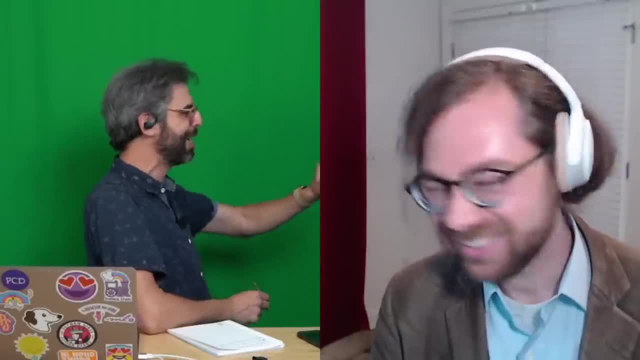 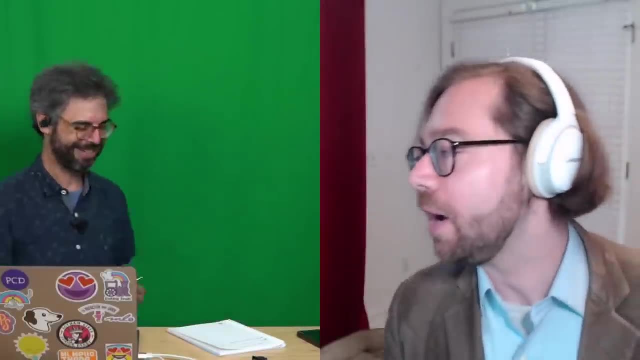 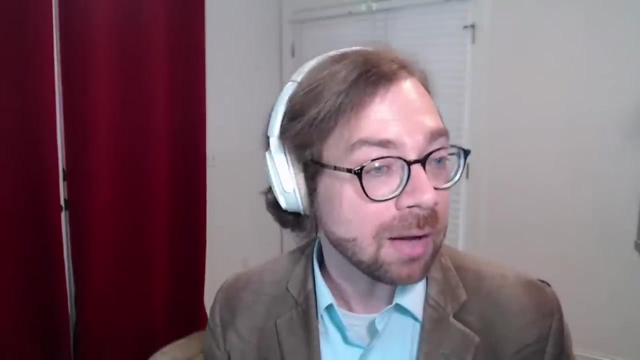 And the options. you can go off this list of options, but the ones listed in the chat are LQG, MPC, sliding mode, et cetera. Do you have a favorite? Yeah, yeah, So just I'll zoom in on this one that's called MPC, which stands for model predictive control. 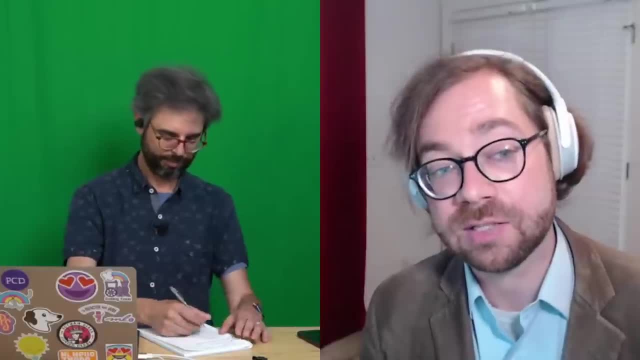 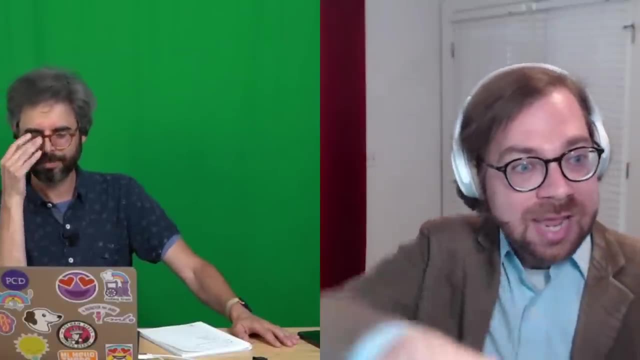 I mean they all have. the short answer is: they all have their uses in different things. The thing that's interesting about model predictive control is that it is not just taking the current state of the system, like what we're doing with PID, and saying: do this based upon the current state of the system. 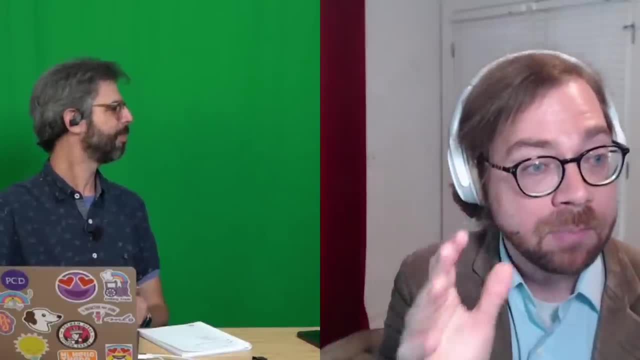 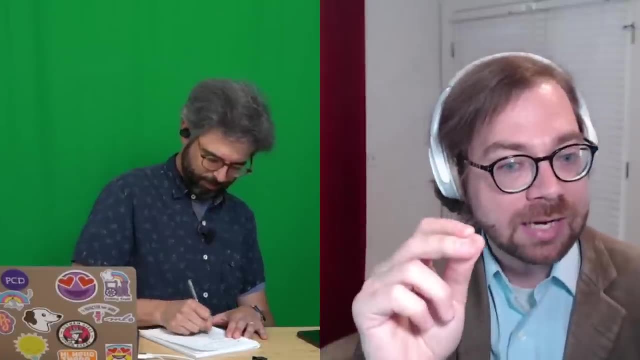 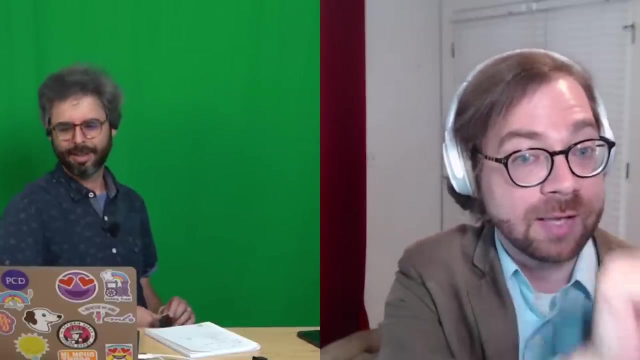 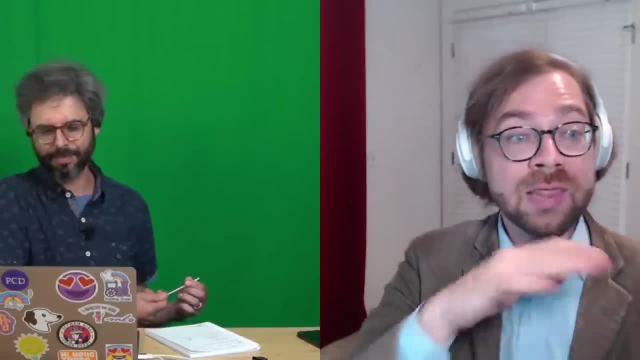 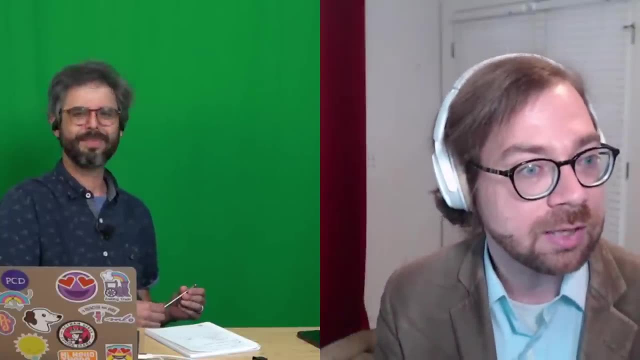 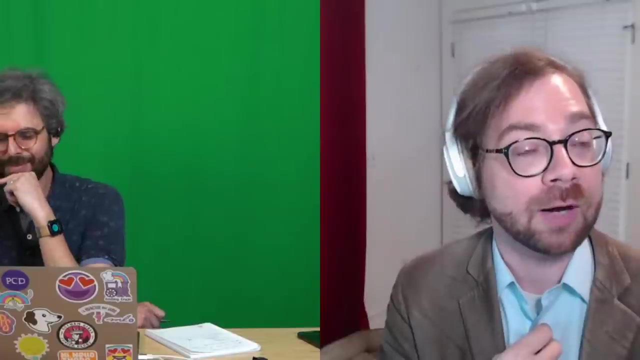 It's doing what we call a trajectory optimization on the fly It is, and one of the sort of undersold to the public tools that we do, that we can do in robotics Now is we can run really fast optimizations called quadratic programs. 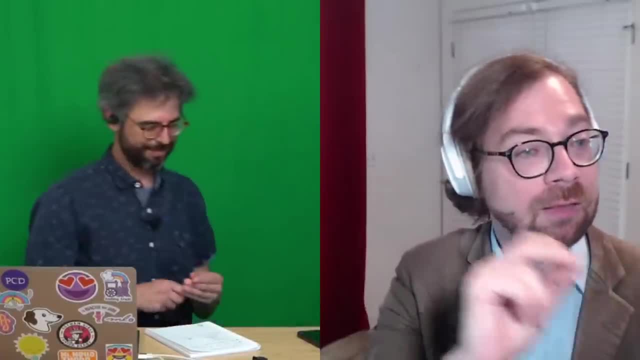 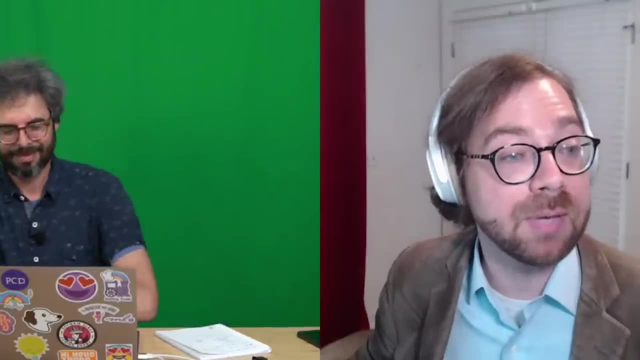 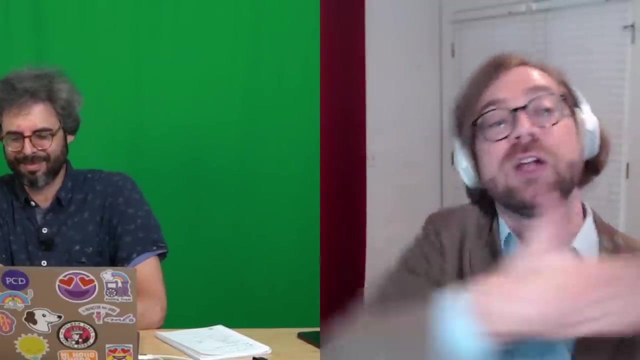 And they will generate on the fly the best trajectory it can, not only for now but into the future. And so you can do really cool stuff with MPC because it is just rapidly changing its prediction. You can push it around. It's like, oh, I should do this now. 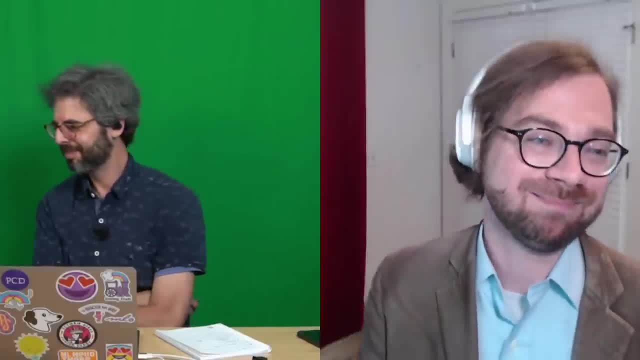 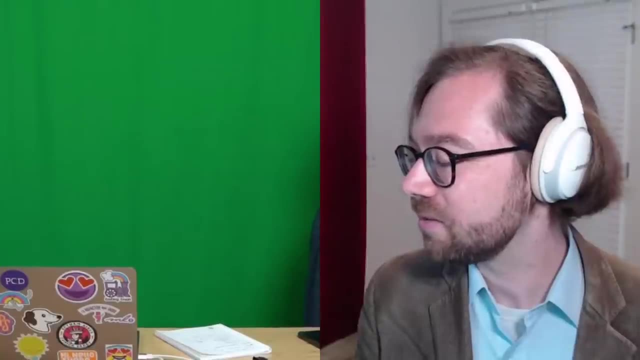 I should do that now And we use that in our robots now. a lot Wonderful. There's a great. Oh, now I lost the comment. There was a really nice comment in the chat that said if we added friction, that would be a nice way to demonstrate the need for the I 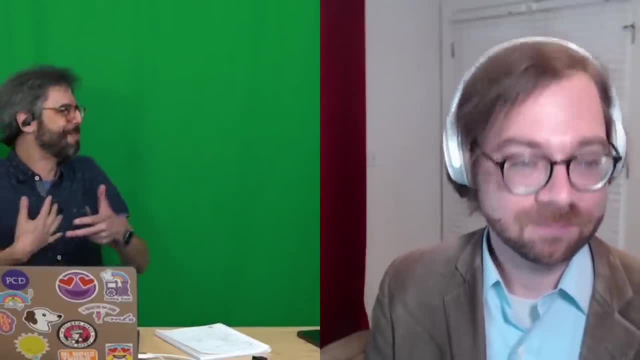 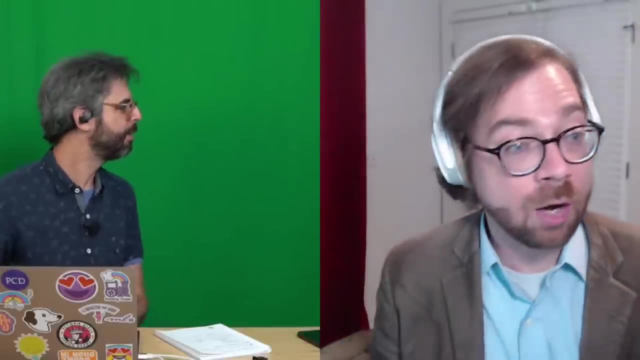 Because we would have to push harder, I guess in a way like accumulate that error to know, to get it to balance properly. Yeah, And I'll make a quick comment on the I term. Yes, that's a great thing for friction. 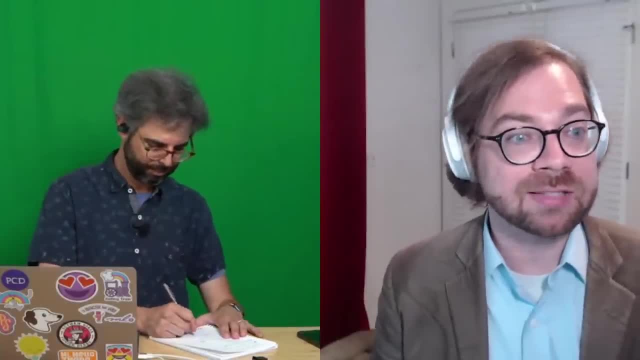 The I term is also the easiest way to make your system accidentally unstable. You've got to be careful with the I term. It could take something that was stable and then suddenly crank it up too high and it starts like it will go from like: oh, I'll correct this little bit of say state error to it will overshoot. 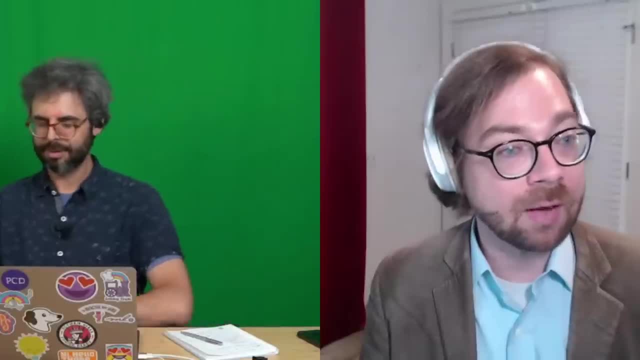 And then it will overshoot again, Then it will overshoot again and it goes wild. So that's what it will do, Right, Wonderful. So let's see here, Let me just check. So I'm trying to think of what else I want to say to wrap this up. 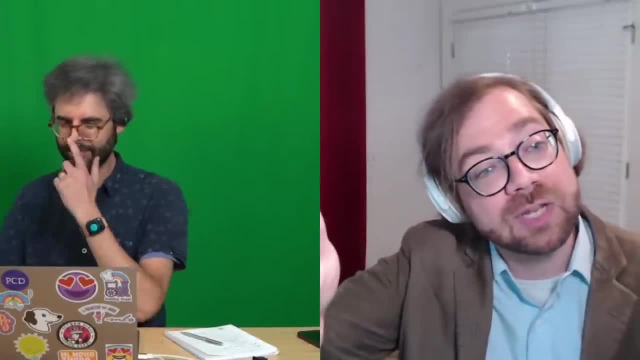 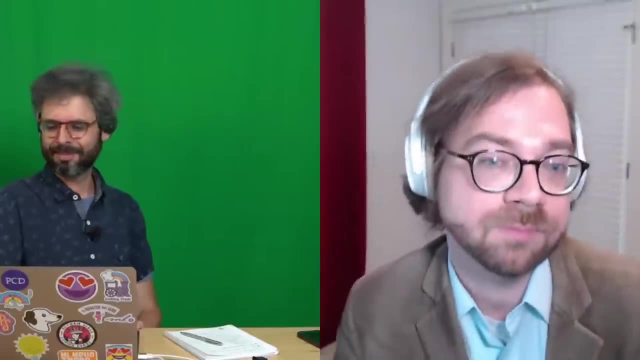 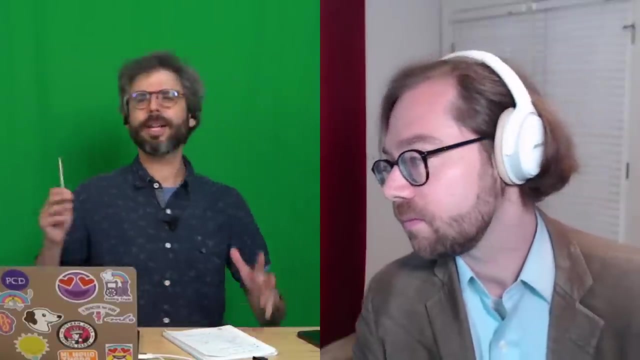 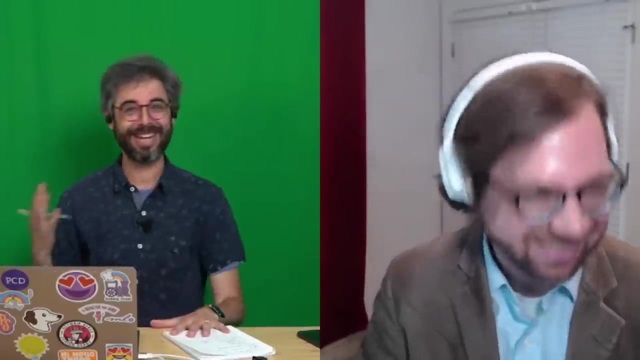 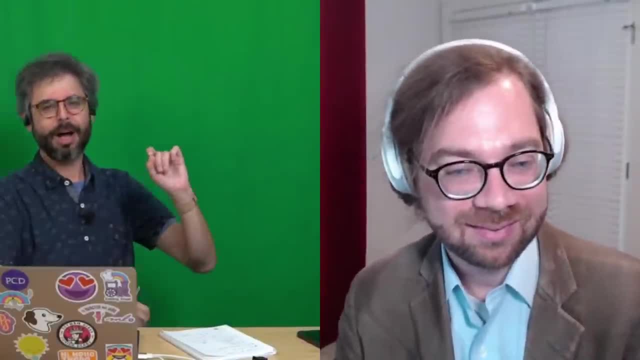 So, first of all, thank you so much for joining. This is really fantastic, Oh, thank you. Oh, I know what I was going to say, The only thing I wanted to add. So, one of the things that I'm hoping that I've been working on for a while, one of 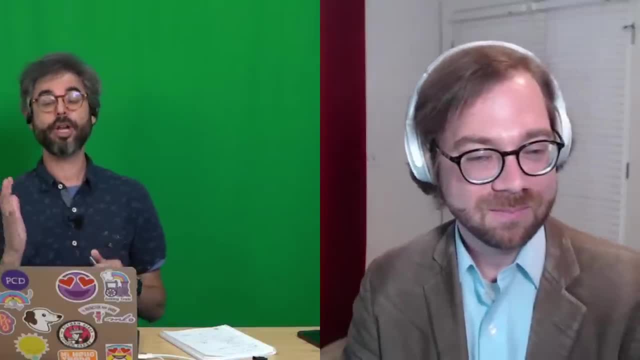 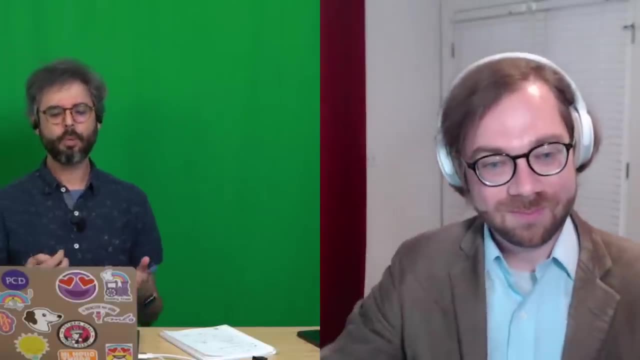 the reasons I'm so excited about this is I've been working on a new chapter for The Nature of Code book about neural networks And I've done demonstrations of this, where we use a technique called Neuro Estimation Evolution to evolve the weights of a neural network. 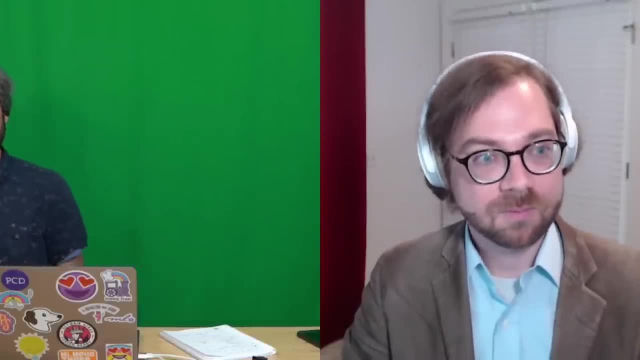 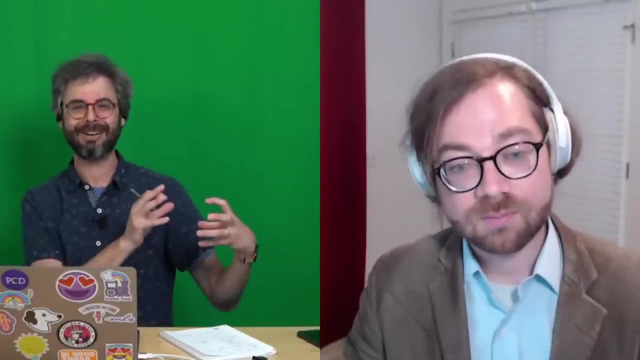 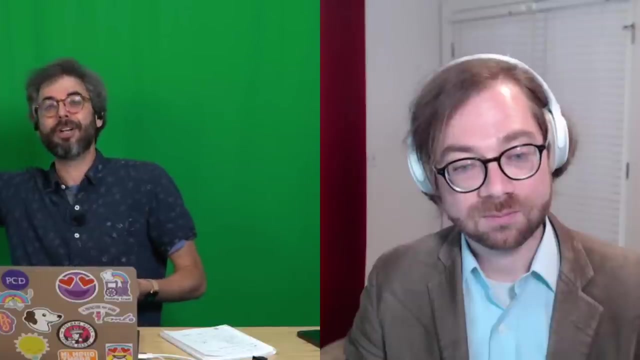 to control an agent in a simulation, And this, I think, would be a really nice example of comparing and contrasting that kind of like: what would the inputs to the neural network be? It could just be just the angle of the pendulum. 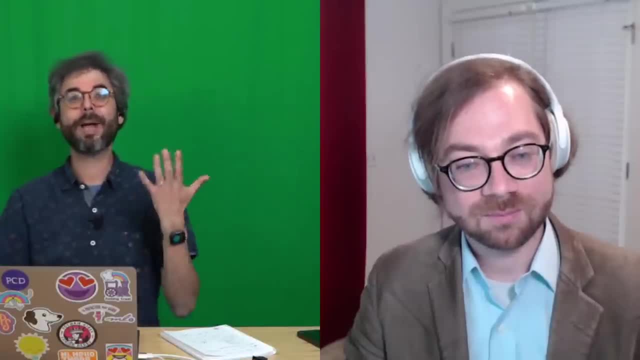 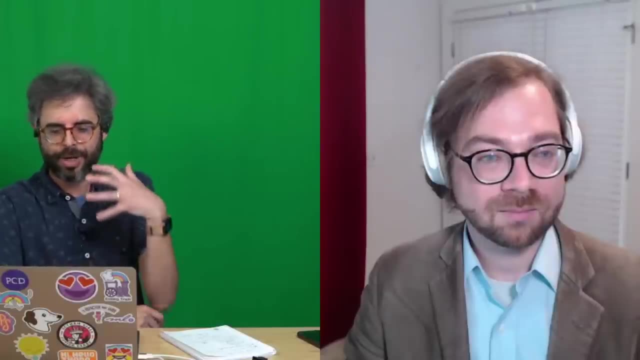 and the current velocity of the cart or something like that and sort of compare and contrast. But what I love about this is I often have students who are like, oh my god, I need to learn reinforcement learning and Q learning and all this stuff to be able to control my thing. 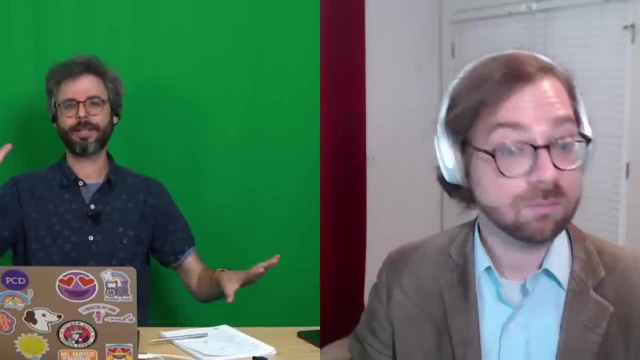 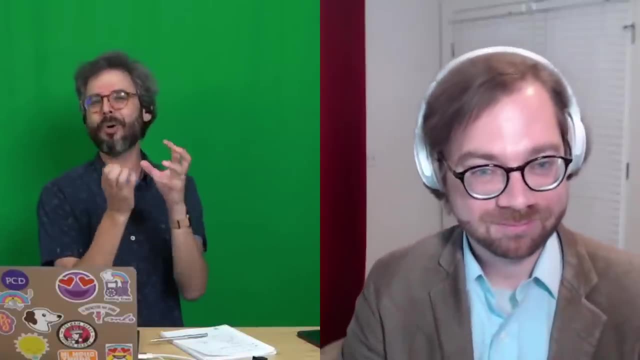 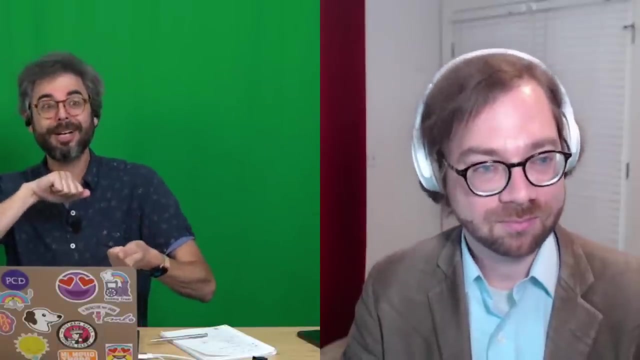 But no, there's something as simple and again, everything is relative. There's lots of complexity here and calculus, math, But something as simple as just looking at your agents, your object's position in the world, where it wants to be that error, and applying a force. 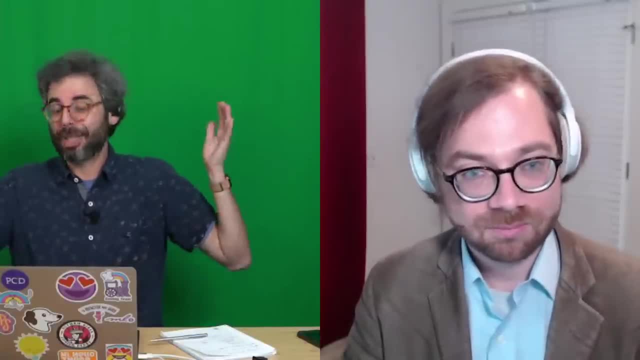 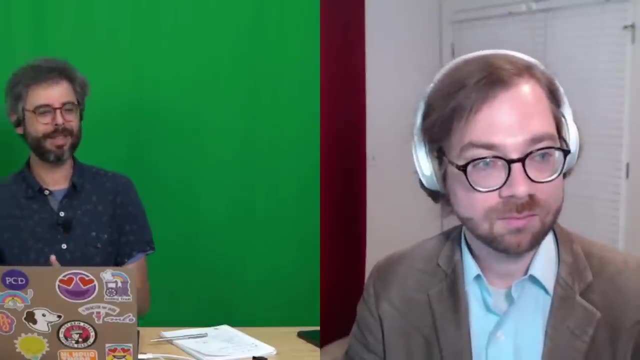 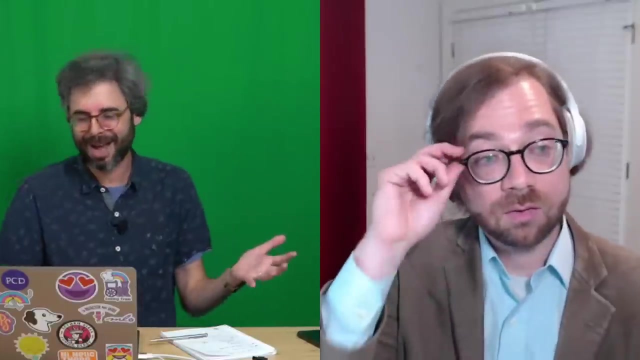 scaled according to that error And just that proportional controller is a really nice way to add intelligence into a simulated system, And obviously, with a physical robot that you built with an Arduino, sticking a neural network in there could be quite overkill, although interesting as well. 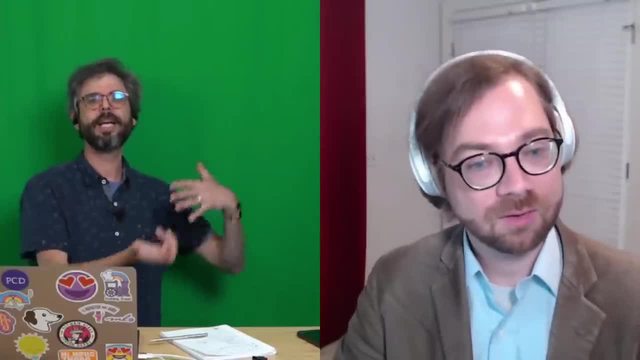 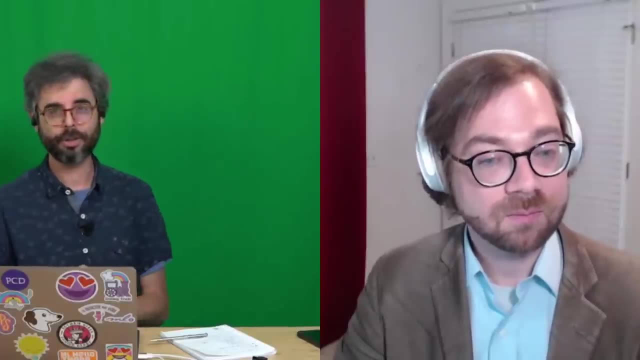 So I just think it's really exciting to see this as a complement and counterpoint to some of these other systems that I'm working on, And I think there's lots of potential here to continue and look at more controllers And hopefully we can stay in touch. 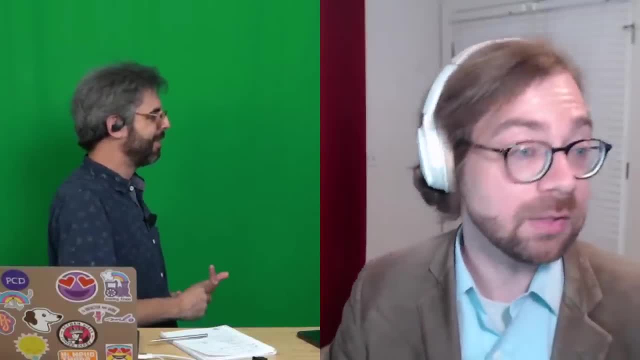 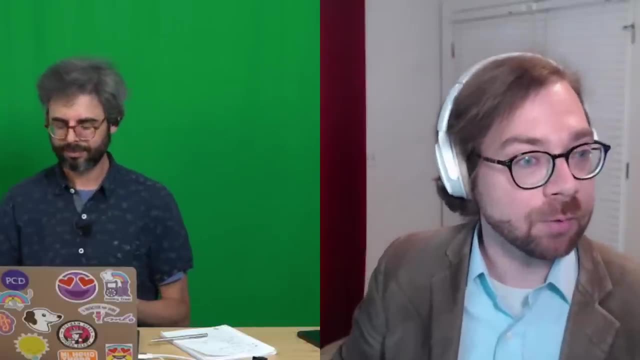 to work on this some more? Yeah, absolutely. I'll just throw a little point on the end of that. I was talking to you in the chat. I was mentioning that people were bringing up neural network controllers And it is a great complement because even 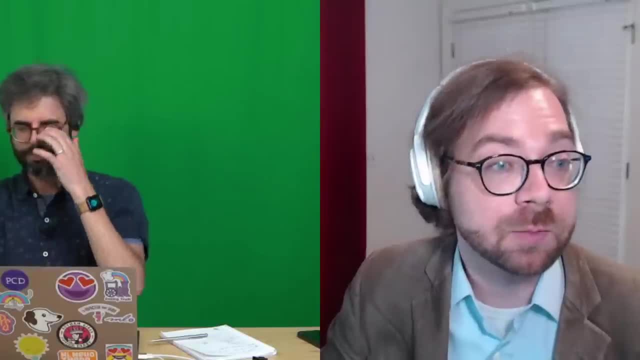 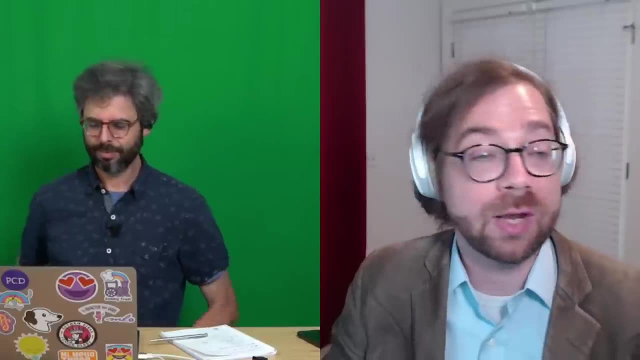 some of the really coolest robots you see that are using reinforcement learning. there's a beautiful example of taking the Cassie robot, the SpyPed, and people use reinforcement learning to train a good walking controller. It's amazing What they're doing the neural network, what it's producing. 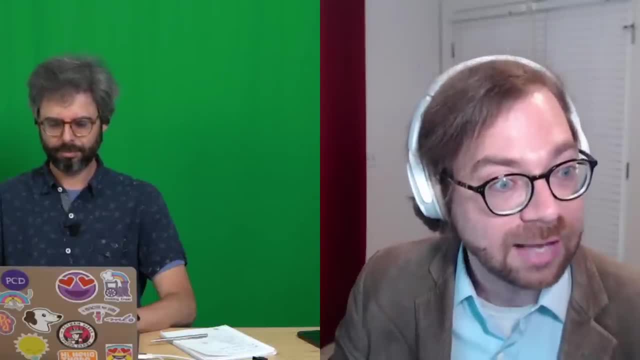 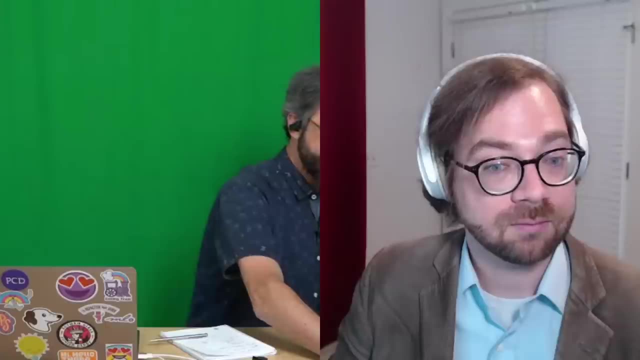 are the desired values for a PD controller. That's what it's doing. They work together and that's really effective. Great, All right, so I'm just going to go, Thank you, I'm just going to go over here just to show quickly. 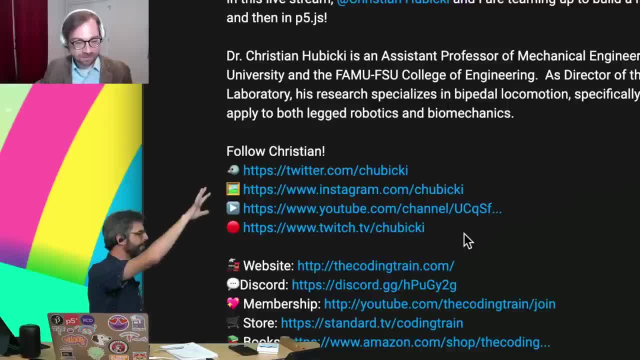 I've zoomed in here. This is currently what's in the video description. You can find Christian's Twitter, Instagram, Twitch and YouTube channels here, So please go and follow Christian. We are both on Twitter. I plan on definitely sharing some of the results here. 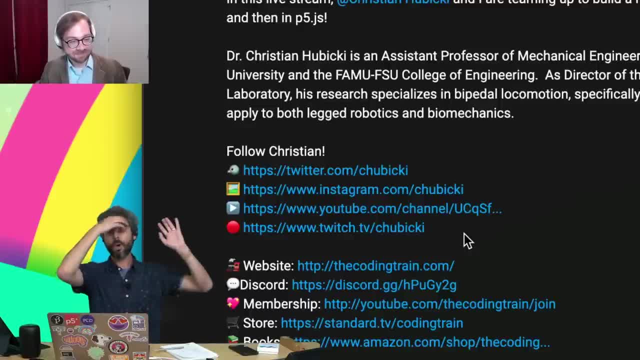 so maybe we can get a thread going with some additional links to explanations or examples And if you've made something. there's no page on the Coding Train website currently for this live stream. I might have one in the future and there's a way. 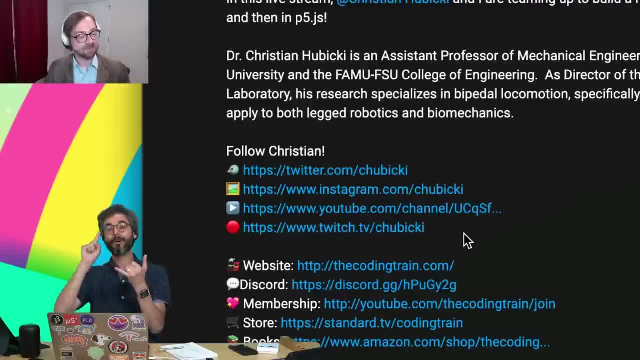 that you can submit things, But stay tuned because I will be releasing a GitHub repository and updating this video's description with links to all these materials in case you want to make your own. And I always say this, but very little in life. there's lots of things that make me happy. 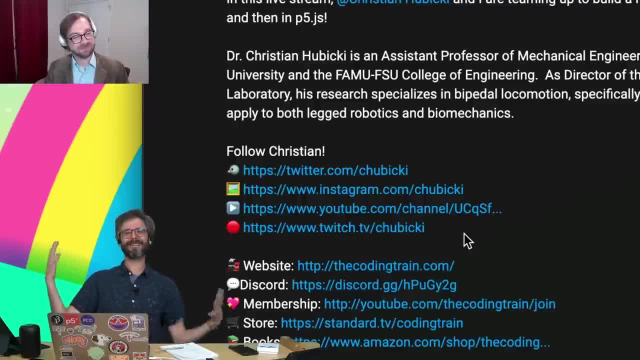 But one of the things that makes me happiest in life is when somebody sees something in a video and makes their own version of it. However, even if you just made it and you changed the colors and you added a little design of a cart, 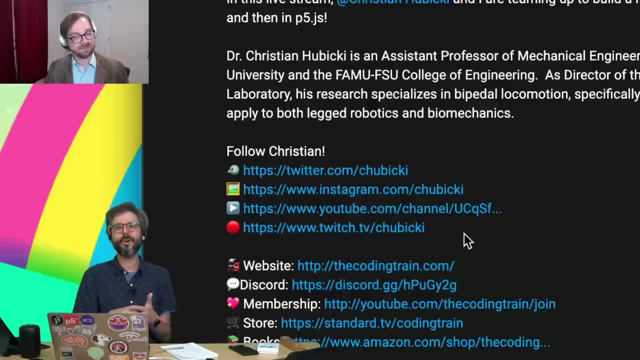 think, just whatever kind of creative fun you can have with this. Don't worry about accuracy of the physics of the simulation, Just have fun with it, play with it and share that back. I would love to see what you do. Is there anything else you want to say or plug or point people? 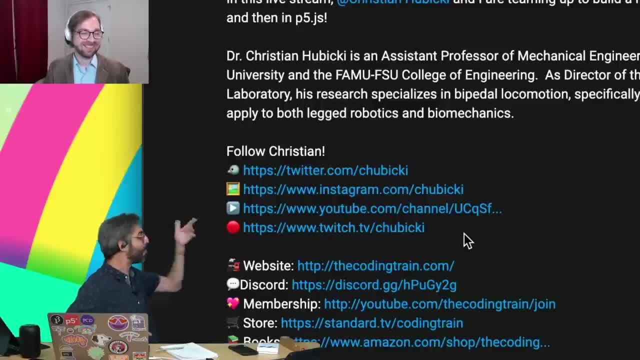 towards before we- Oh, I know I'm giving away a rabbit. One thing I did want to ask is because I do know that I do have a lot of students who watch the Coding Train, whether they're in high school or an undergraduate. 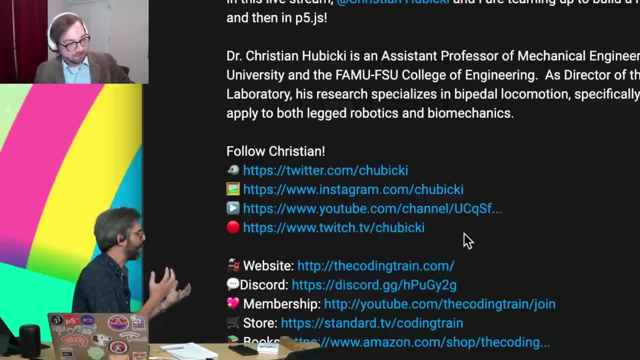 So if people are interested in- I mean kind of like the field of robotics or mechanical engineering, where would they look? What would you point them towards in terms of your lab and your program that you teach at would be one nice thing to mention before we wrap up. 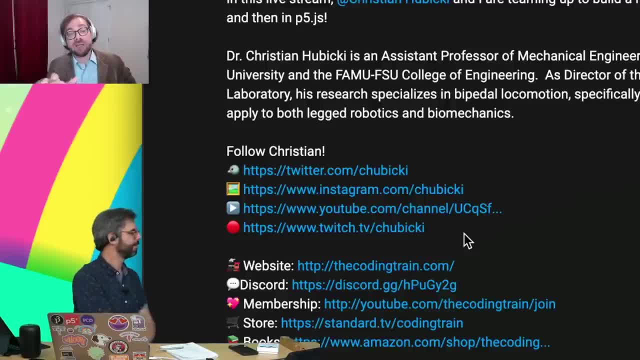 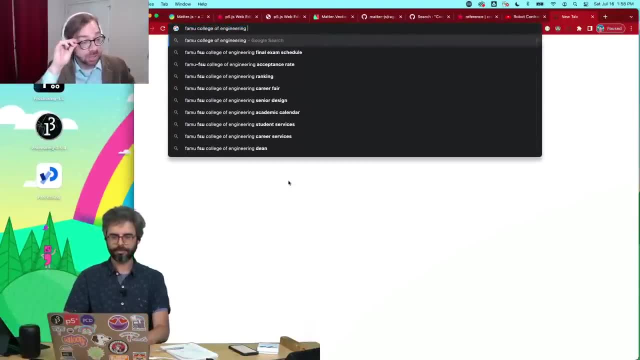 No, it's great. So I'm an assistant professor of mechanical engineering at the FAMU FSU College of Engineering in Tallahassee, So it's a joint college between Florida A&M University, which is a historically black college, and university. 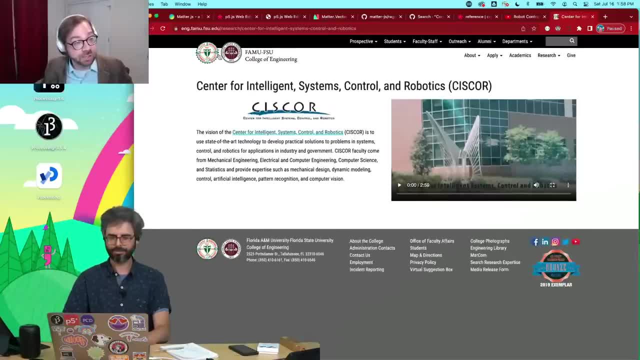 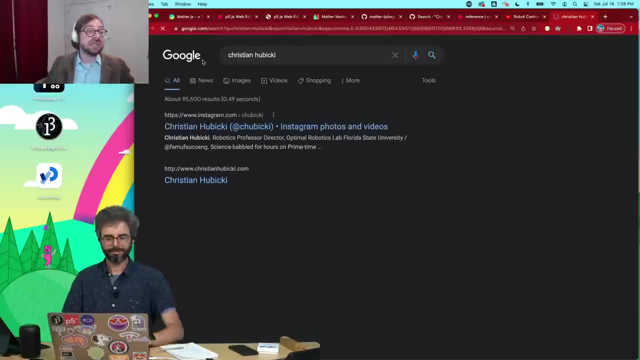 and Florida State University, which is a wonderful R1 research institution. So I'm down here in Tallahassee. You take engineering courses. You might take them from me. You can find me on my personal website at christianhubickicom. C-H-R-I-S-T-I-A-N. 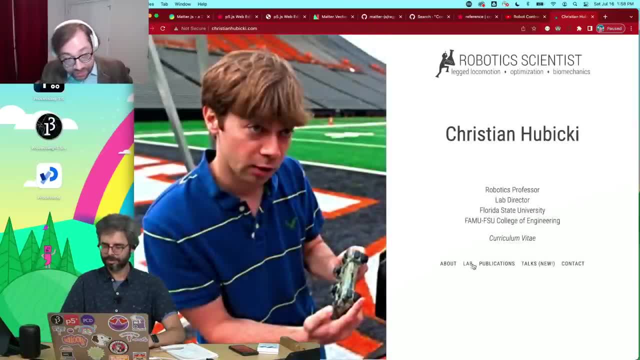 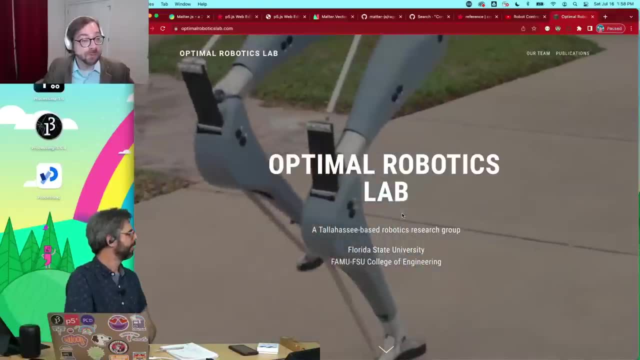 HUBICKI, H-U-B-I-C-K-I, And you can find me there. I've actually I give public lectures as well. Sometimes people pull me up And this is my laboratory, theoptimalroboticslabcom. 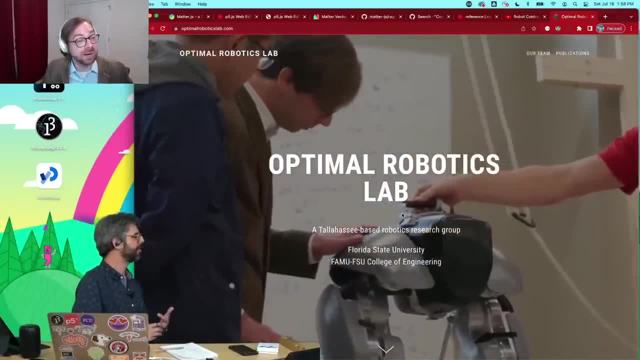 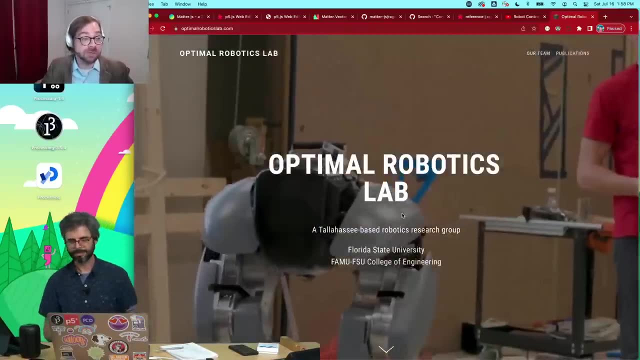 And so that's where you can find some of my work- And this is one of our robots walking around And feel free to reach out to me. You can find my contact information on my website and, of course, through Twitter, which is at Chubicki, which I believe. 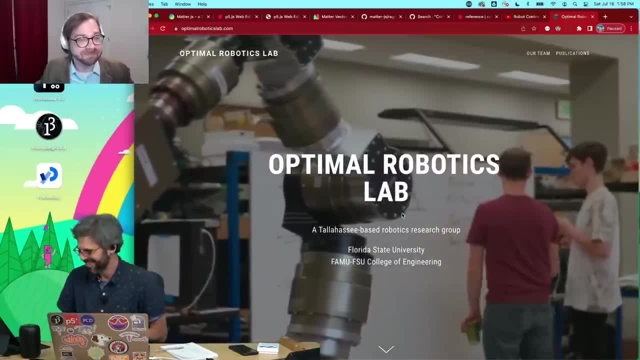 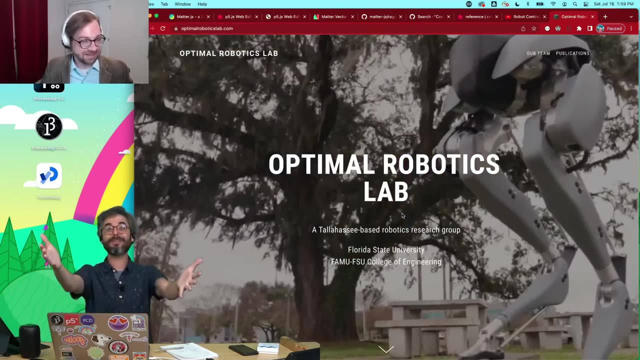 is Chewbacca's younger brother. Awesome, All right, Wonderful. Thank you so much for being here. This was great. I'm so glad the tech seemed to all work. Thank you everybody for watching. I don't have any particular updates. 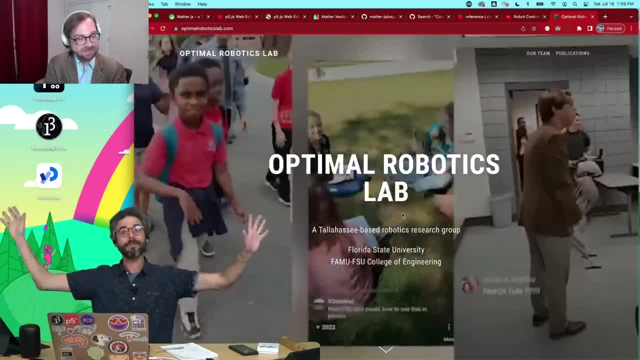 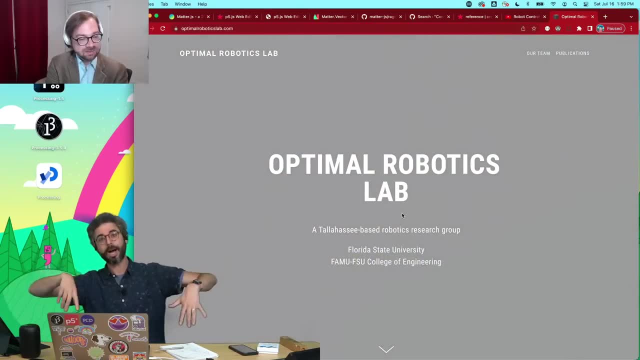 about when the next live stream will be or when the next videos are coming out, But hopefully something next week. I always announce everything on the Coding Train Discord So you can go to the Coding Train Discord. Join the Discord channel If you sign up for the notifications role. 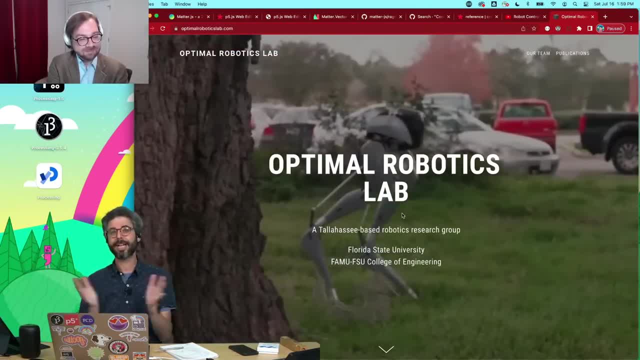 you'll get pings if you want, for when I'm scheduling things And I just appreciate all of you watching. Please go and enjoy making your own pings, You know? do something else. maybe Take a break from your computer. 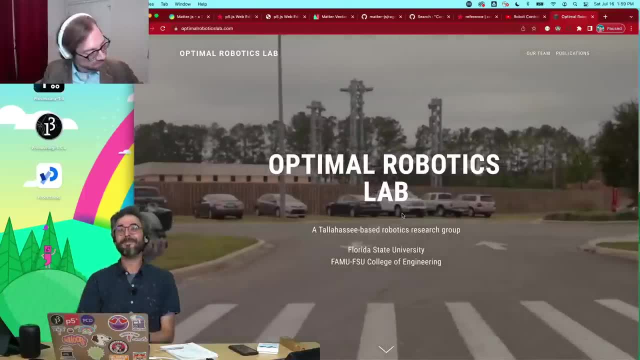 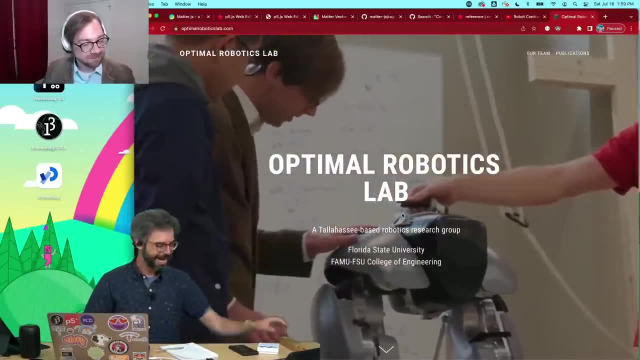 It's been like many hours, But when you come back to it, if you can make a PID controller in Python or in P5 or Unity, again, share it with us on Twitter And I look forward to seeing you next time on the Coding Train.